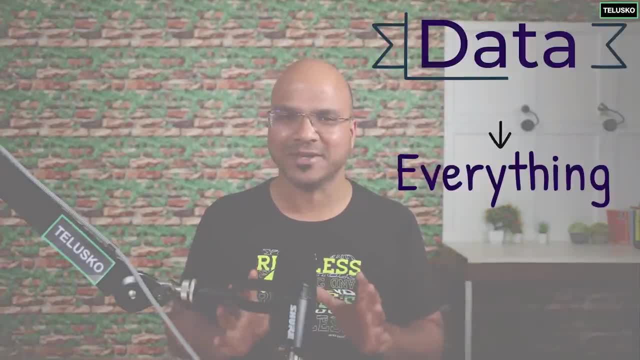 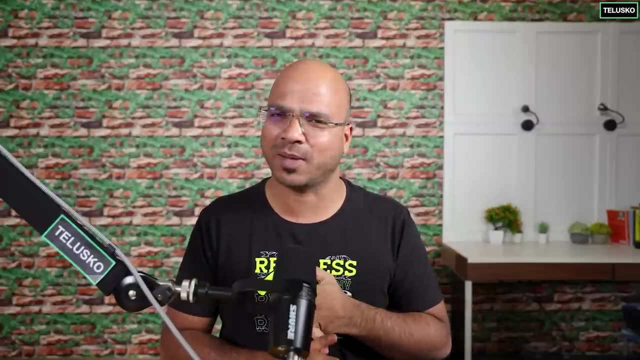 information. So data is everything. So it doesn't matter what technology you learn, you basically learn or you work on it so that you can work with data. Example: think about programming languages. Why do we use programming languages To process the data? Why do we use database to store the? 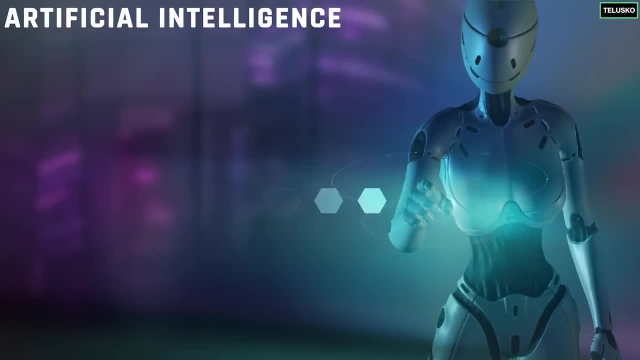 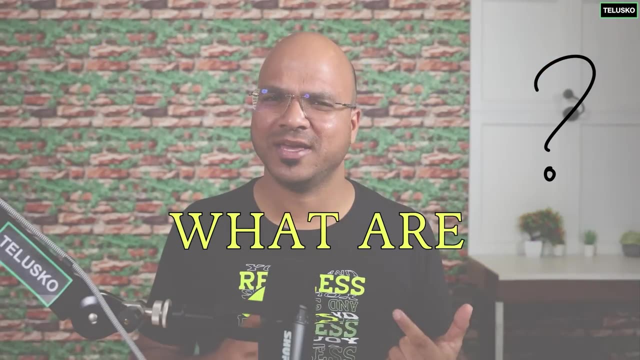 data. Why do we use AI to generate data or to understand data? right, I mean just to bring it down: everything is data. Now. then question arise: what is data structures? Now, if we talk about any programming language, we have something called primitive data types, If you. 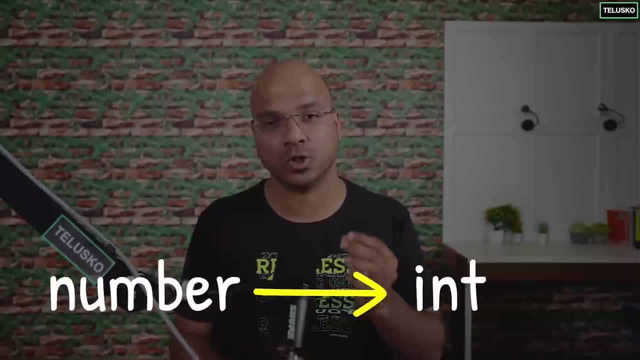 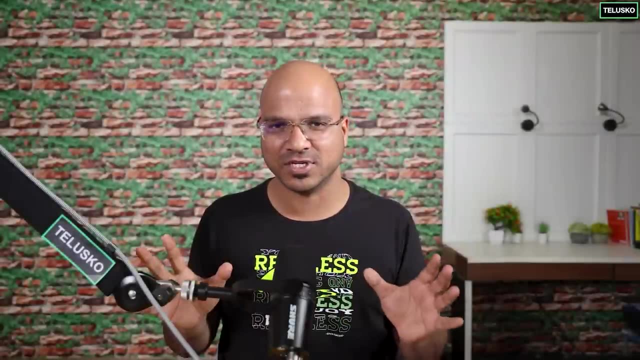 want to store a number, we store that in integer. If you want to store a text, you store that in a string. If you want to store a character, you store that in a character. Of course, depending upon different languages, the term or the way you store it changes, but ultimately you have. 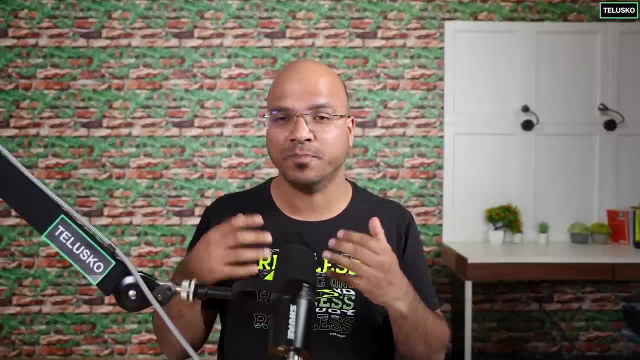 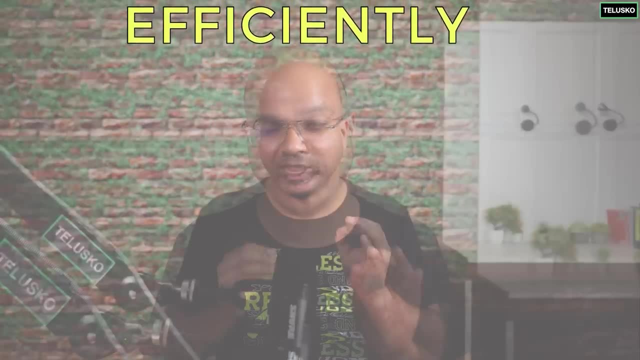 some types to it where you store the data. But what if you have a bunch of data and if you want to store them? It's not just about storing data. anyone can do that. It's about how do you store data efficiently and you can also save some memory. The thing is, if you simply 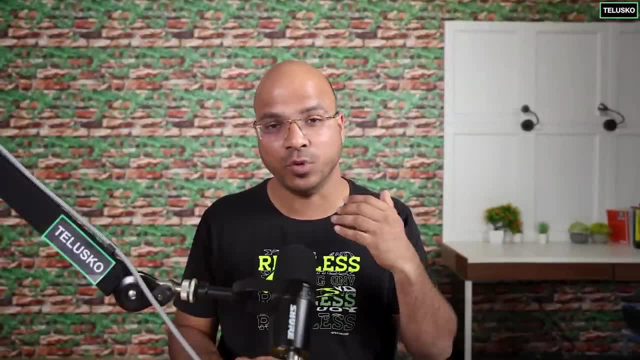 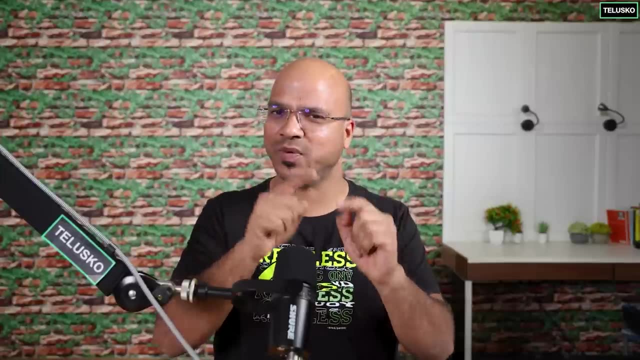 dump the data, you are expanding the memory and if you want to search something from the data will be difficult, and that's why storing that data efficiently is very important, and that's where data structures comes into picture. So data structure is a way to organize and store data. 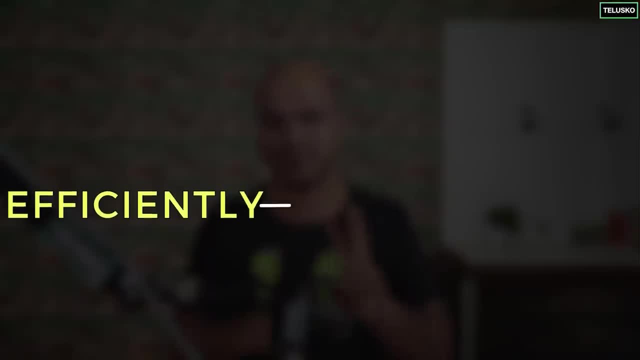 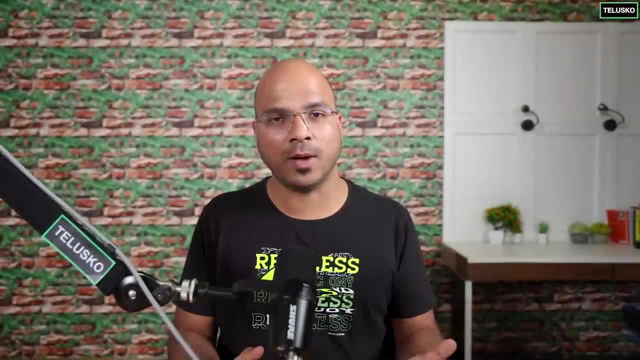 efficiently. Okay. so when you say efficiently, it means two things: First, in terms of performance and also in terms of the memory. Now, what about performance? Now, think about this: if you, if you talk about any software application which we use, it can be a normal. 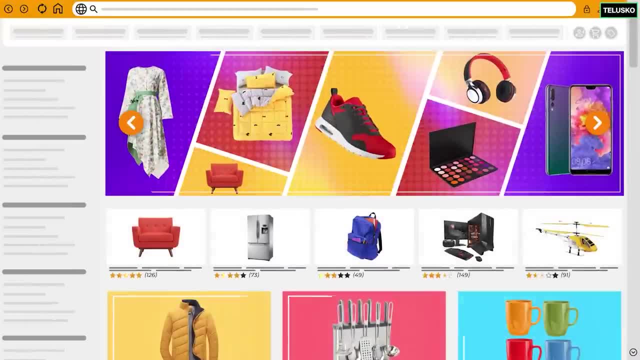 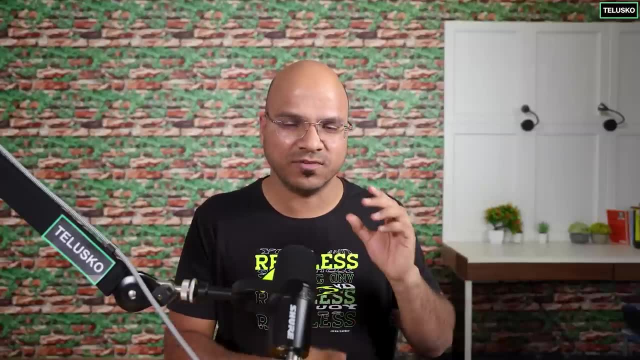 calculator, or it can be an application like Amazon website or any application which we use, a banking application as well. Now what we do in that application is we use some features using which you can compute something, you can process something, example on Calcutta. you calculate on the banking. 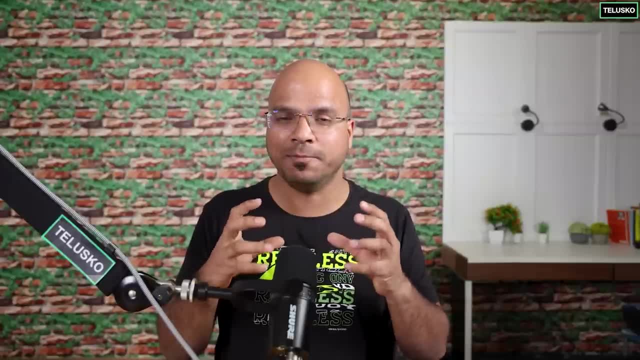 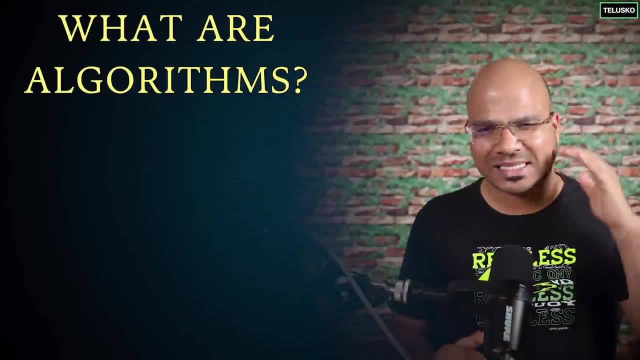 website you transfer money. so what you are doing is you are basically building an application which will do something in the application. So you are basically building an application which will do some processing, and the way you build an application is through algorithms. Now, what algorithms? set of instructions, let's say, if I want to add two numbers, it's very simple. you what you. 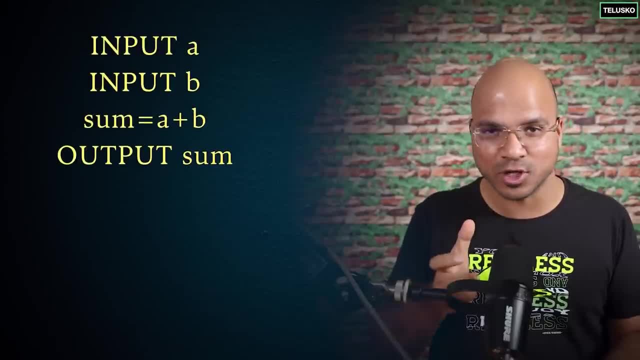 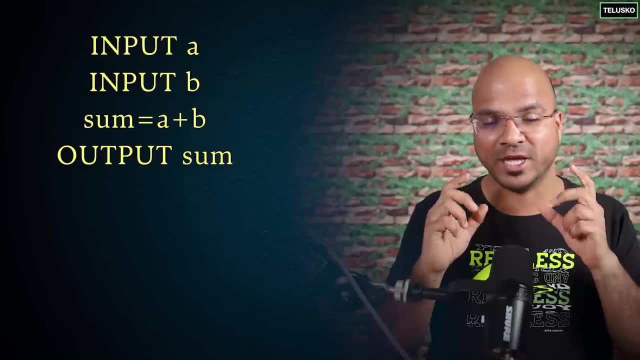 do is you say, take two values from the user, then perform the operation and give the value back to the user. Now, those are the steps, right, those are instructions. Now what I have mentioned, the instructions, those are called pseudo code, because we are not actually typing a code here. we're not. 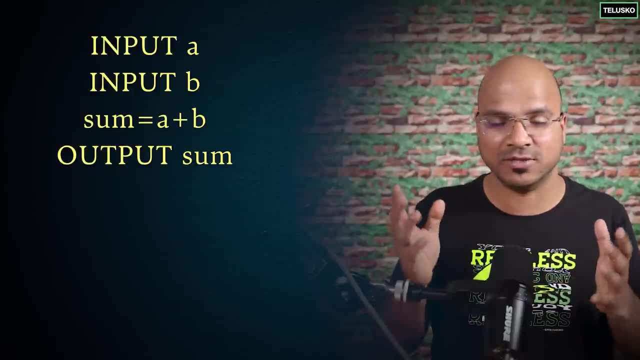 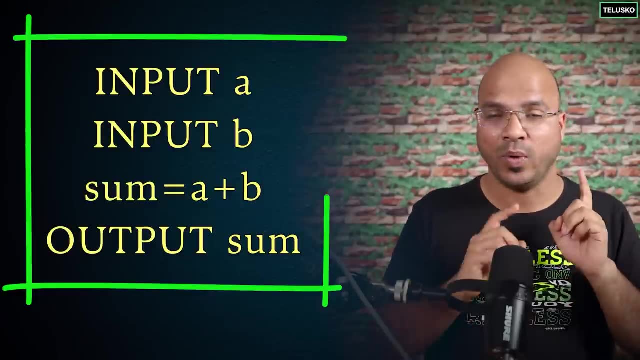 being specific to a language, let's say C, C++, Java, Python, JavaScript. what we are simply saying is: these are the steps you have to follow and that's your algorithm, right? but yes, when you want to make it work, you have to convert that into a code which. 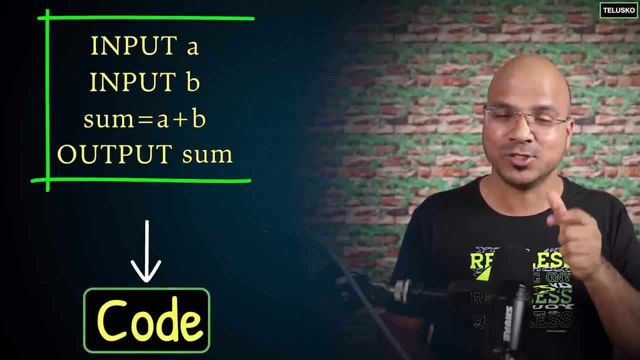 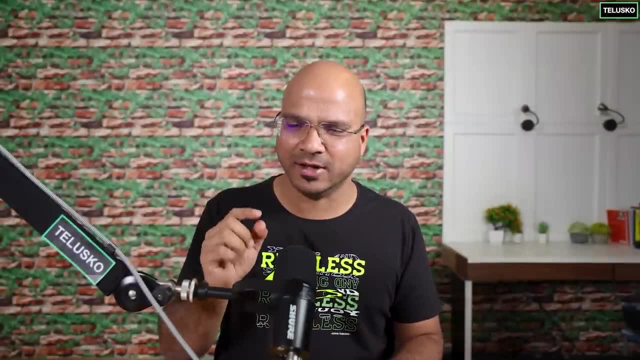 will run on the computer, right? that's your actual software code, and you can use any language, doesn't matter, right? but the pseudo code will remain same. Now, when it comes to processing of data for any task, it's important for us to make it fast and also save memory. Now, most of the companies are 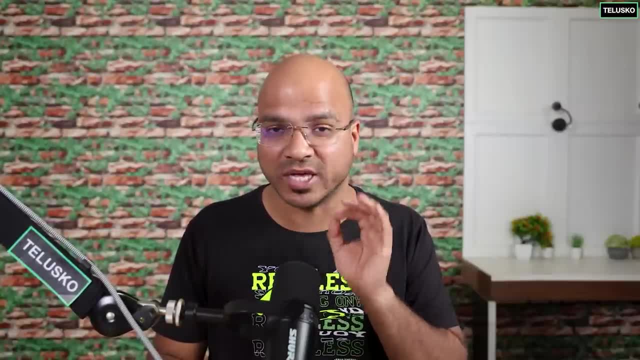 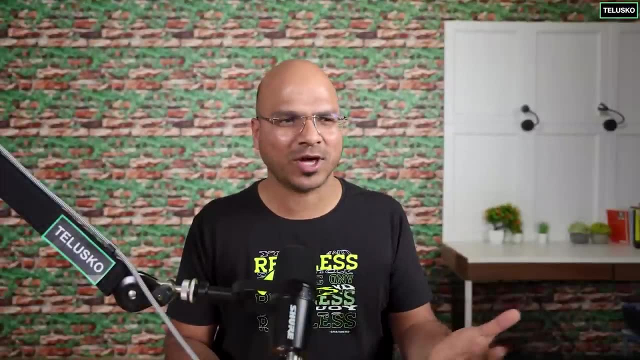 focusing on this concept of data structures is because they want to give a good experience to the user. Of course, right, if I'm using some application, I want it to be fast. Now you will say, okay, to make the system faster, you can increase the CPU speed, you can increase the amount of RAM. 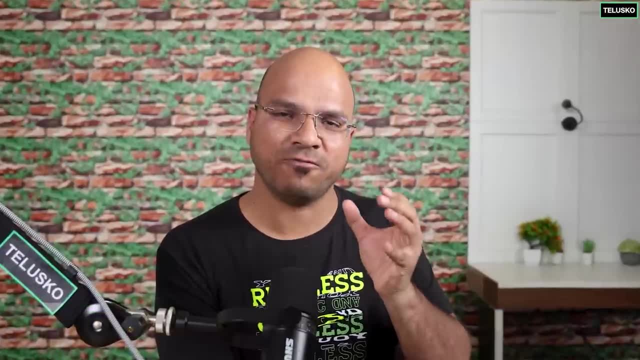 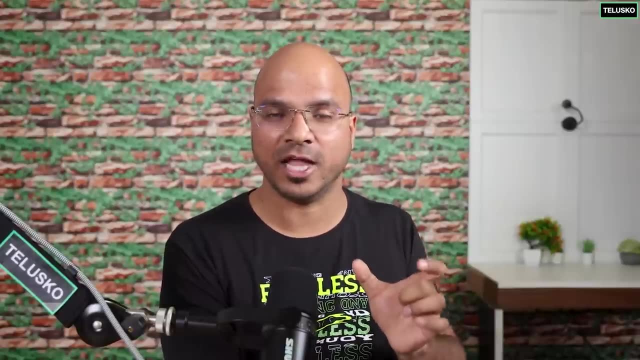 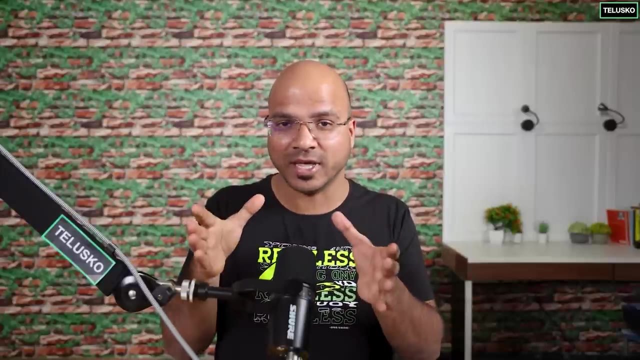 you can do that. but what if, with the same amount of memory, same amount of CPU power, you can still make it more faster? right, and that can be done with the help of data structures. Now, if you know how to use data efficiently in a proper structure, and by doing that you can make your application faster, 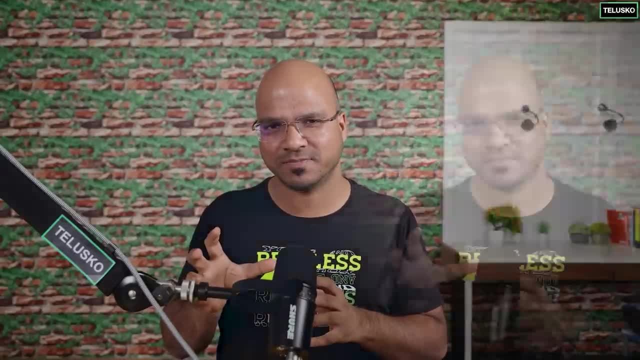 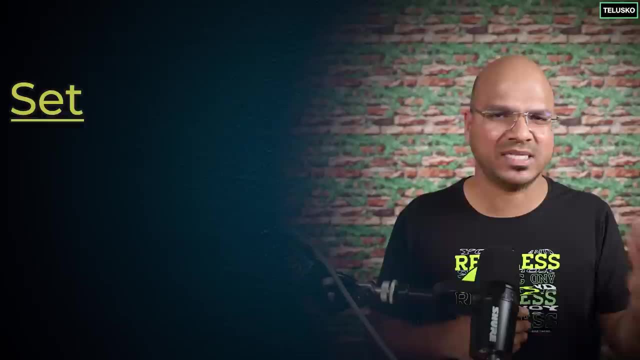 because in data structures we have different type of data structures. Example: let's say, if you have bunch of data, you can store that in an array. but apart from array we have other types as well. we have set, we have linked list, so when to use what. it's not that this is best or that is best, it's. 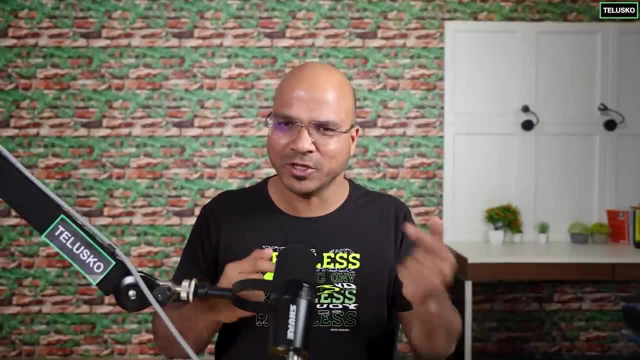 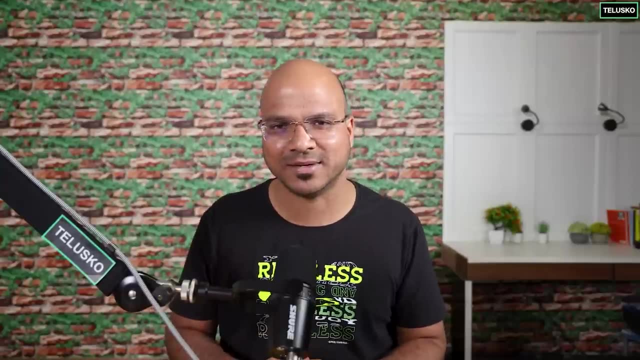 all about when to use what and to understand when to use what. you have to first understand what. this time you have to use array, this time you have to use set, and that's where understanding these concepts are very important. Now, these are not the only options we have. we have tree, we have 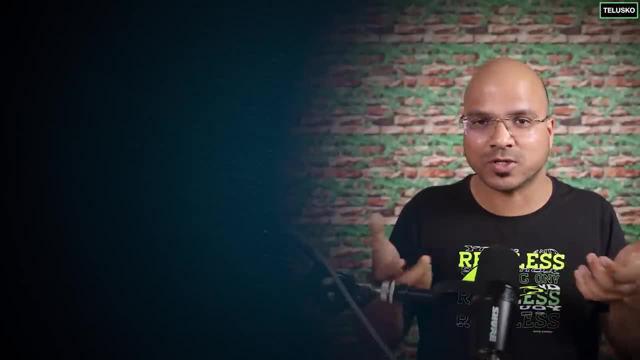 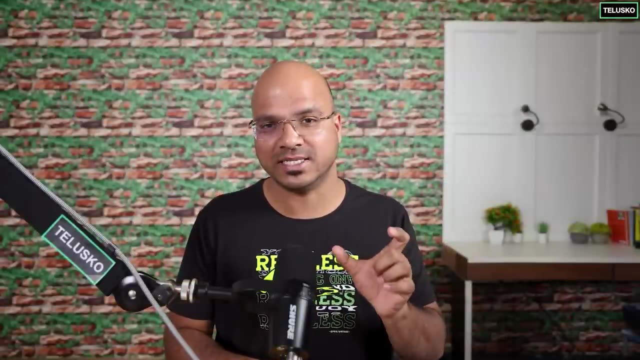 graph when to use them. so when you understand those concepts, then we can think about: okay for this situation we will use this and this is why companies are preferring candidates who knows DSA. it will help them in multiple ways. First, it helps them to reduce the cost is because every 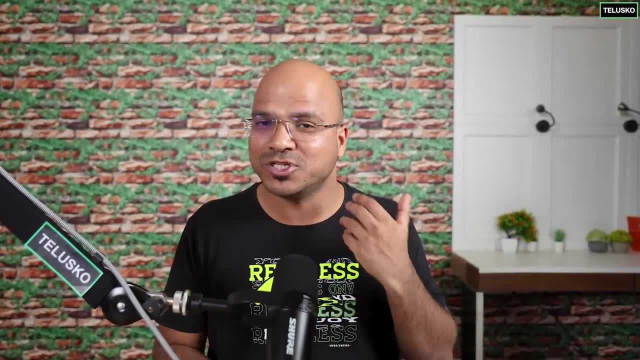 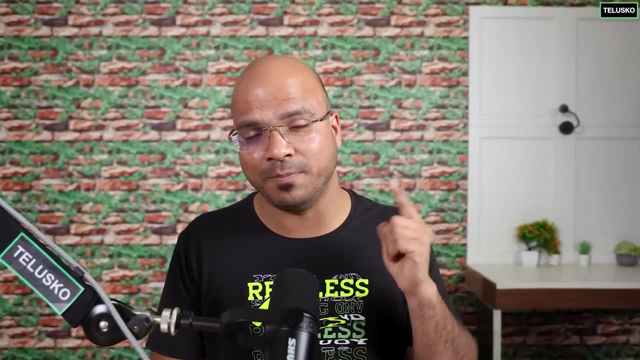 computation. see, I know you might be thinking, most of the application which we use are free. think about Instagram now. when we use Instagram, of course we are not paying for it, but then companies are paying for it, So the Meta is paying for you, for your account. 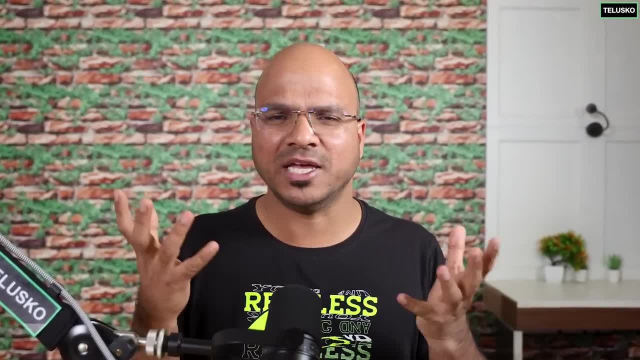 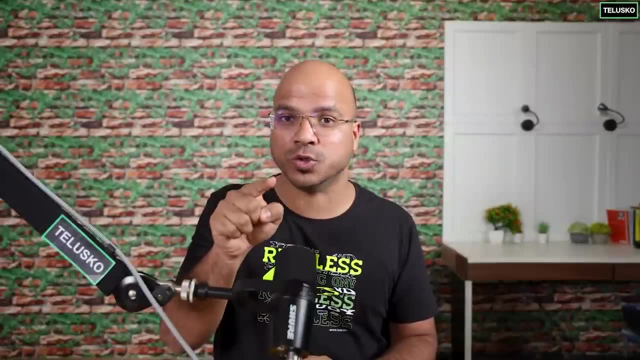 So, because those computations will be happening somewhere, some may be- Meta is using some cloud service, someone, and let's say Amazon is in this case. So Meta is basically paying to Amazon for every competition which you do. okay, of course, they earn from ads, but they will be paying for it. So 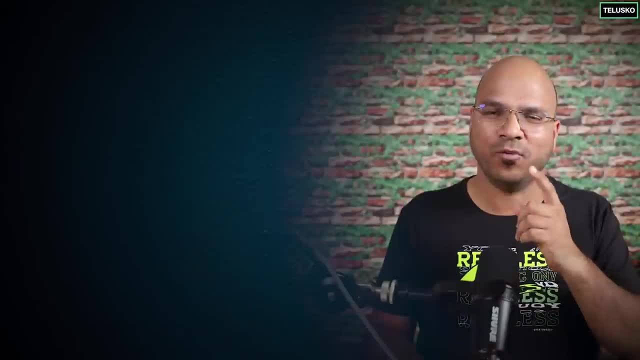 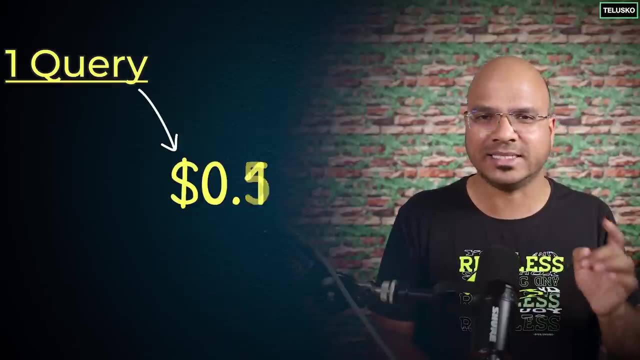 what they will do is they will try to optimize. They will say, let's say, if One query takes, let's say, $1 or maybe half a dollar, Can we just reduce it more? Can we just make it 10 cents? So that's the thing they are trying to do. 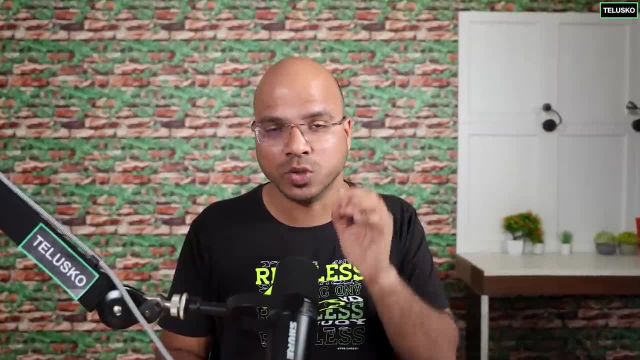 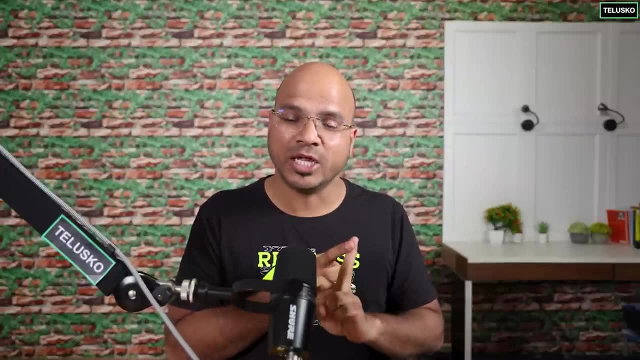 And the way you can do that is by making sure you use a proper algorithm with a proper data structure. So why companies are doing it? to reduce the cost. Second, to give a better customer experience, so that it will run faster. And if I search something, 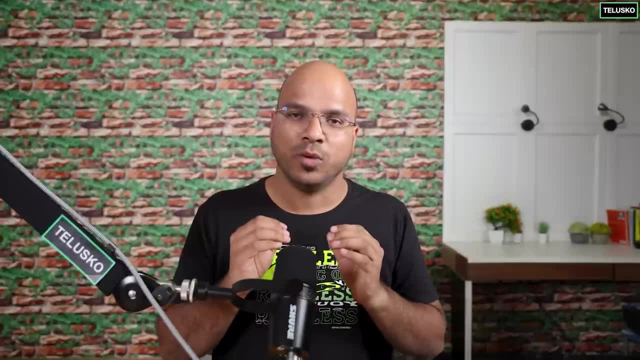 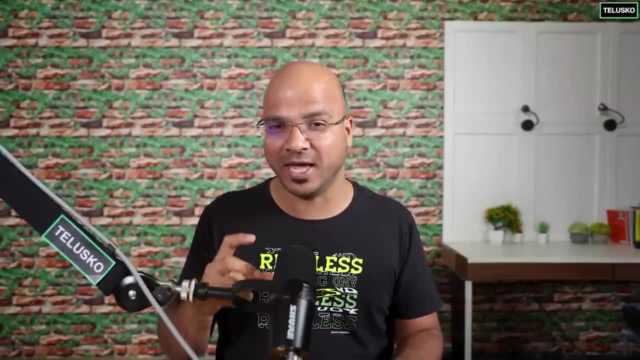 it should be faster for me as well as a customer. Next, when companies want to hire people, they have so many candidates right. How will they filter those candidates? Now data structure algorithm becomes one of the way to filter the candidates. 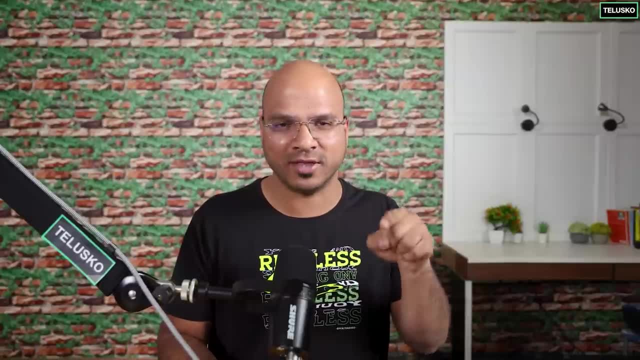 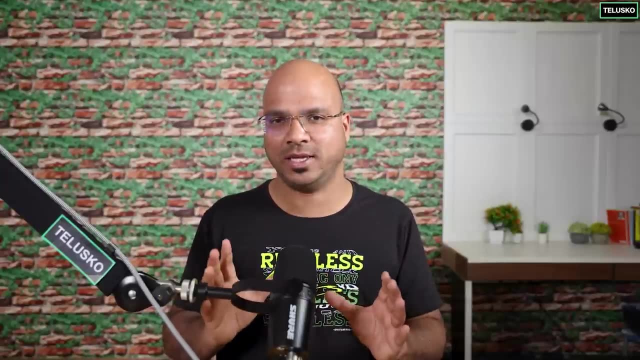 Because if you know data structures, that means you have worked a lot on that particular language and you understand how a particular system works. On the other hand, data structures are not the only thing you need to know If you want to be a good developer. 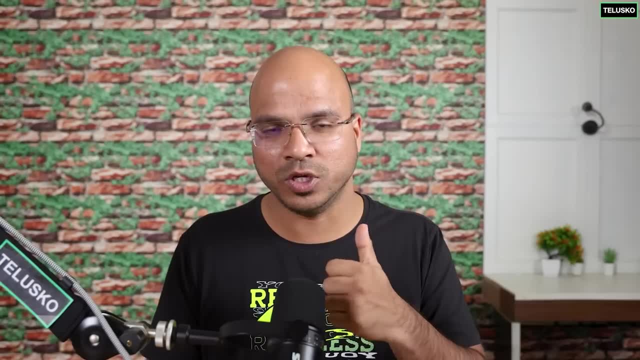 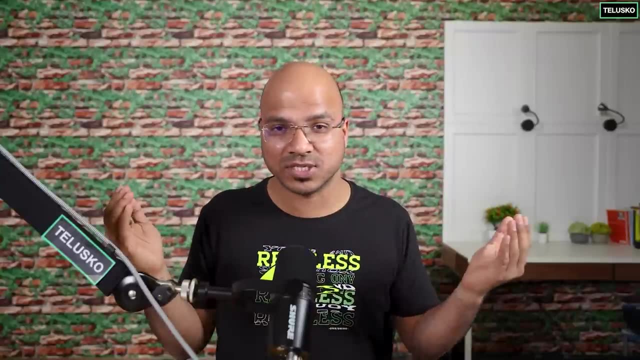 if you want to get hired, there are multiple things needed. For example, you need to have a good hold on a particular language, a particular technology. you should have worked on a few projects understanding the entire ecosystem, not just one language. 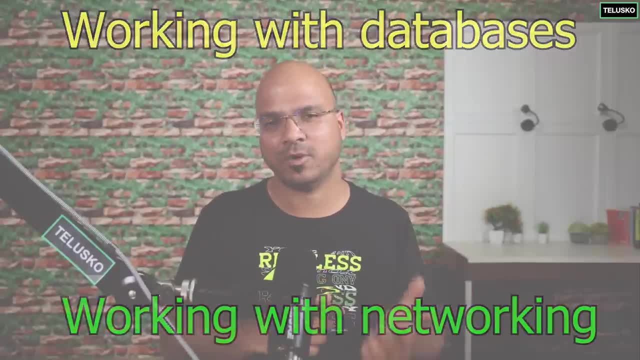 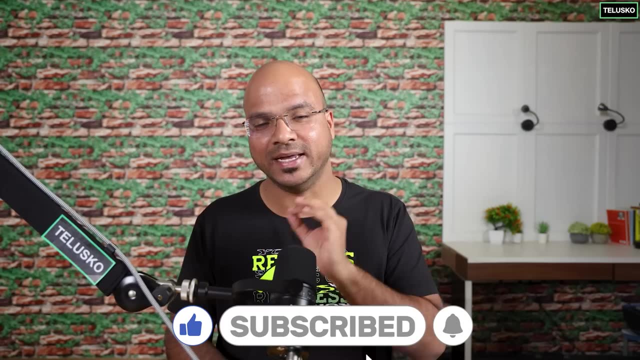 working with databases, working with networking, But then DSA becomes one of the important things there. So just to summarize, what are data structures? So data structures is basically a way to organize and store your data in the efficient way, And there are multiple data structures options available there. 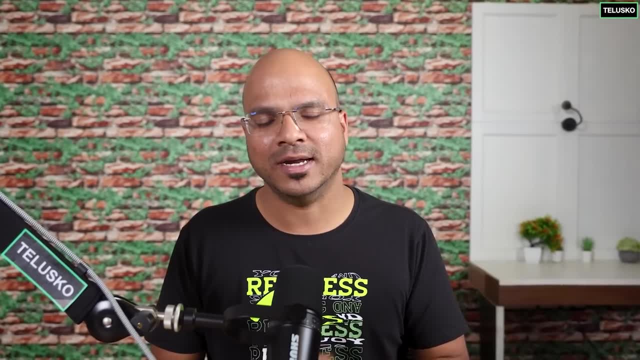 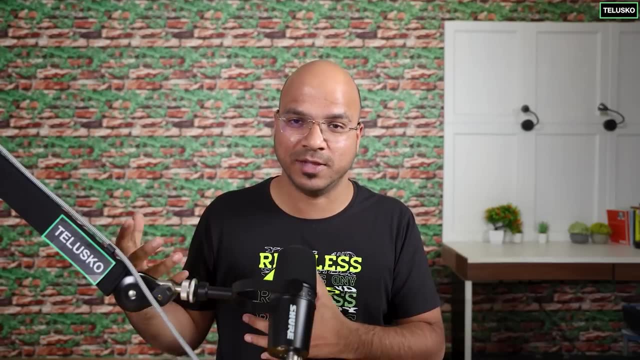 And you will understand that in the upcoming sessions we're going to talk about, In the upcoming videos, we will talk about what are the types of data structures we have, how to use them, when to use what and what are the algorithms available there. 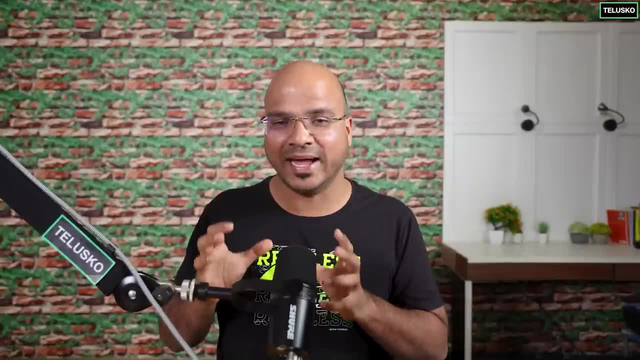 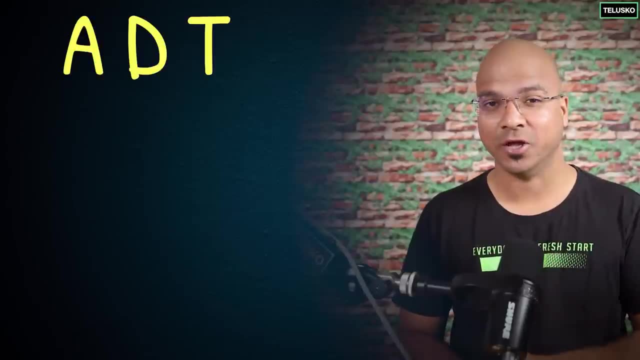 So I hope you got some idea regarding data structures. So, of course, entire cities is important to understand that properly. Welcome back aliens. My name is Devyn Reddy And in this video we'll talk about ADT, which is abstract data type. 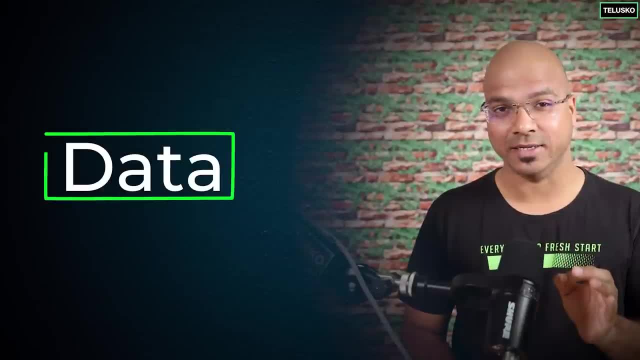 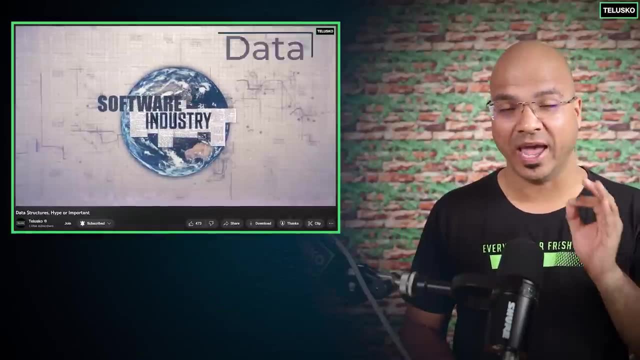 Now, before we move towards ADT, let's talk about data here. Of course, in the previous video, when we talked about what are data structures, we have talked about data And we also mentioned that in the software industry, everything is about data. 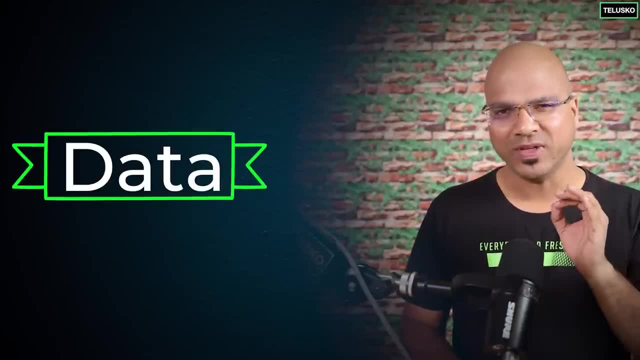 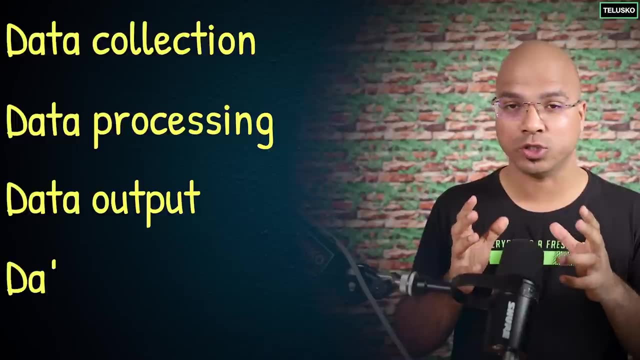 So, whatever you do, you're doing it for data right now with this data, basically, you get data from the user, you process data. You also give the output to the user, or maybe you want to store this data in the database for. 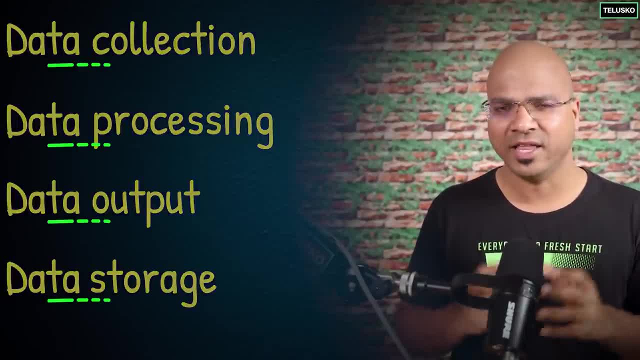 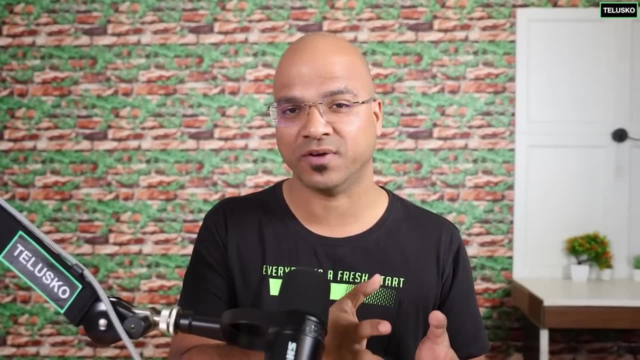 the permanent storage. But the thing is, it's all about data And whenever we use any language, doesn't matter which language you use. what you do is you store that data in your code somewhere. And to store that data we use something called a variable. 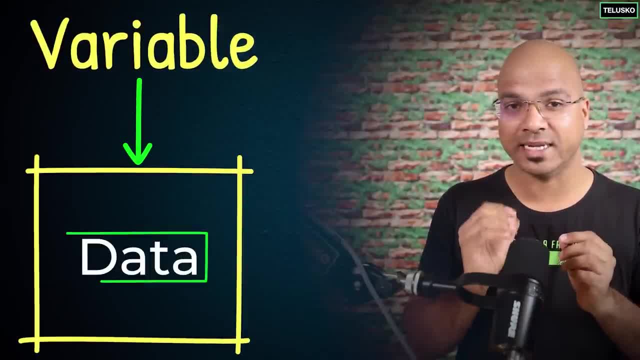 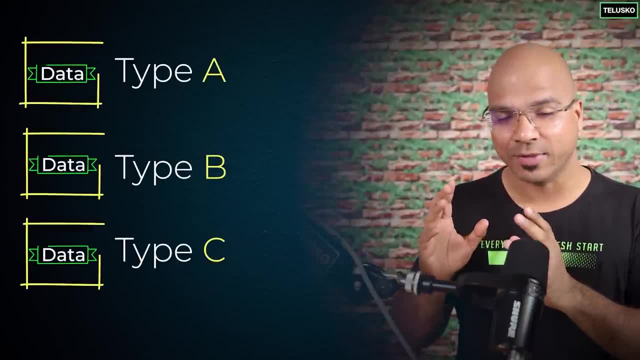 Now imagine variable as a box and you are keeping your data inside that box. The problem is, every box need to have a type. Of course, there are languages which are dynamically type language, where you don't actually mention the type of the variable. 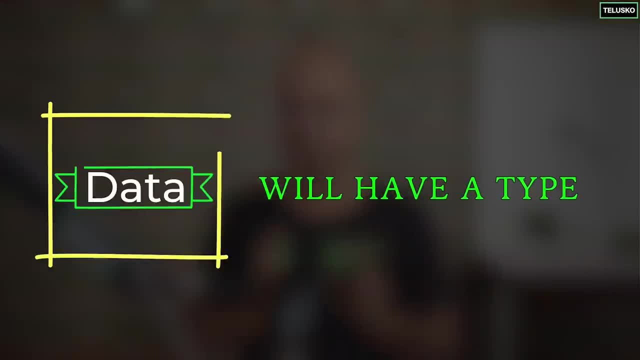 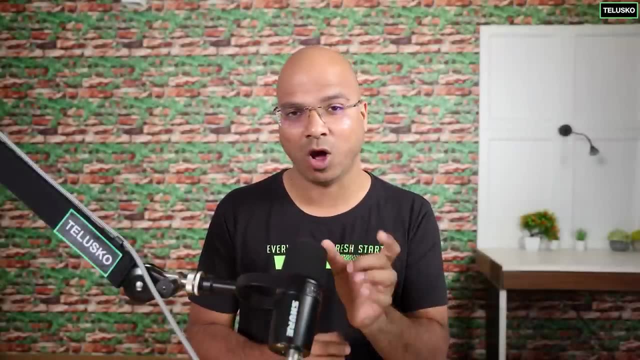 but in general, this box will have a type. So that means if you want to store the data, you need a box, which is your variable, And this variable also needs a type to it, or this box needs a type to it. 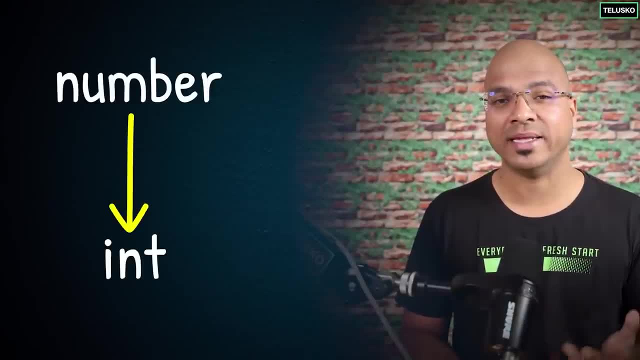 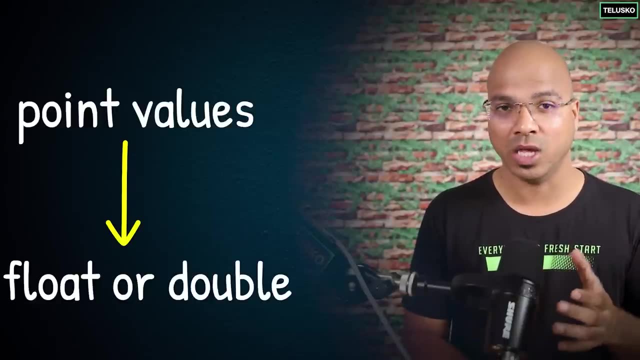 Now example. let's say if you want to store a number, so we can use something called an integer, or if you have any other point values, you can also use float or double. Now it depends some of the languages how they work. 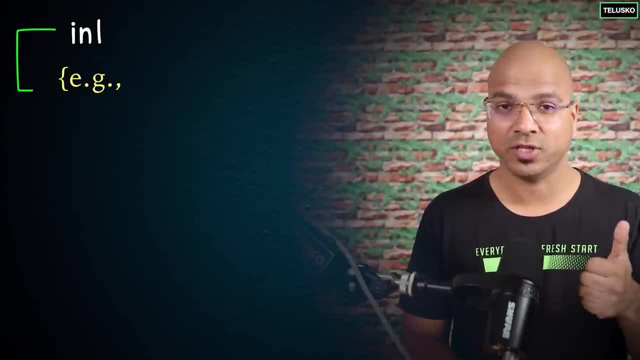 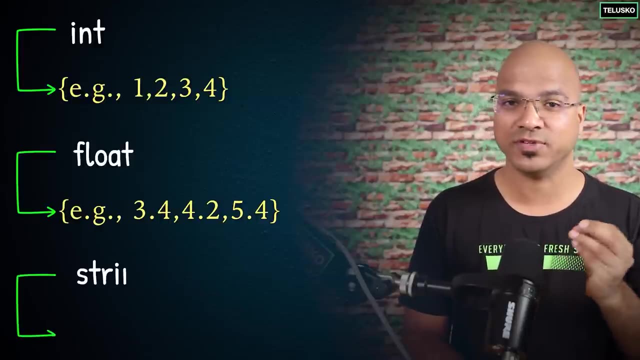 But in most of the languages we have something in common. We have integer for the normal numbers, We have a float for the point values And what if you want to store a text? That's why we have string, And in few languages 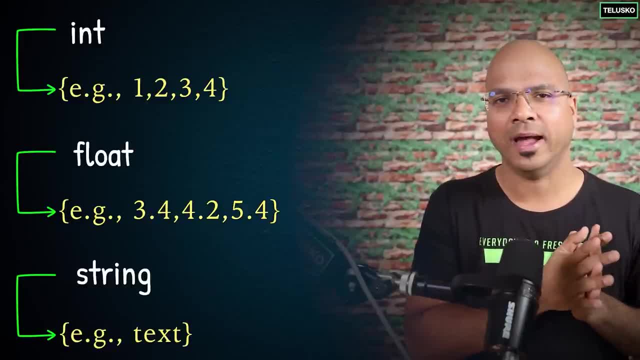 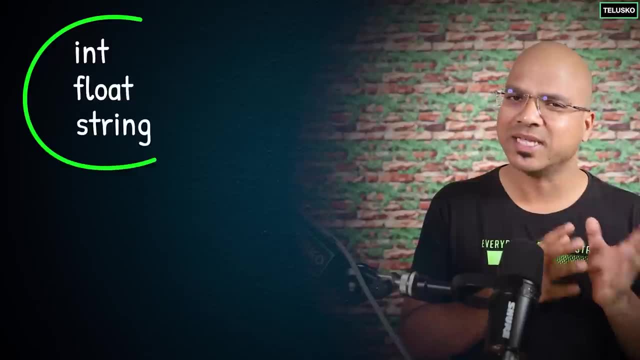 we don't have all these types. We have limited types and in other languages we have many, but that doesn't matter, right? In general, we'll be having a variable and a type to it. Now, all this type are called data types. 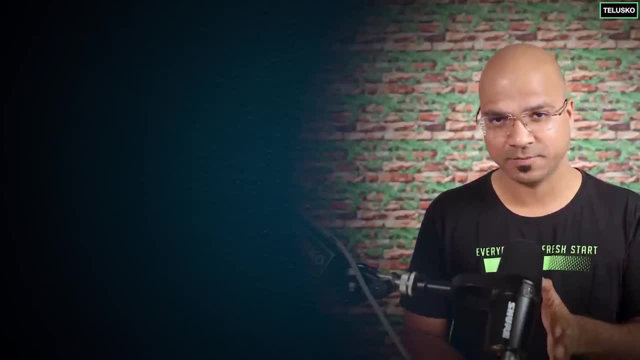 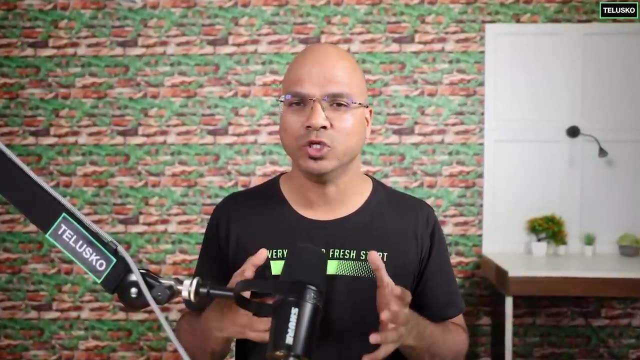 And they are the system defined data types, Or you can also call them as primitive types, is because it's there in the language itself. You can directly use them. but sometime you want to use some complex data type and we can create that with the help of some other concepts. 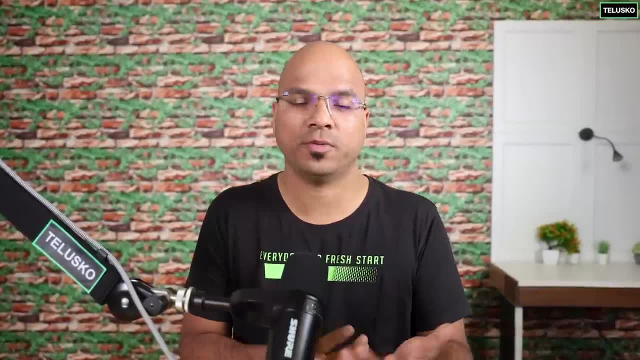 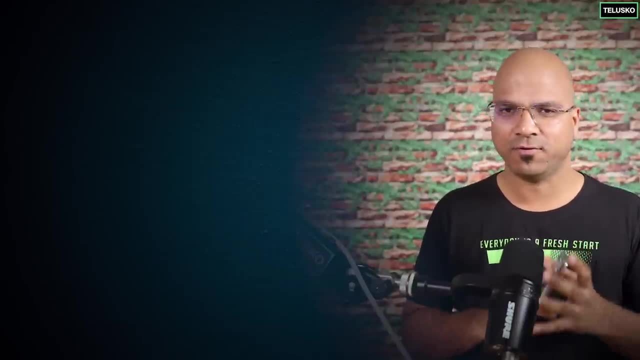 Example. let's say, if you want to represent a human or if you want to present a phone- Now I love phones- I'll be using that example. So if we talk about this phone here now, this phone will have a name to it. 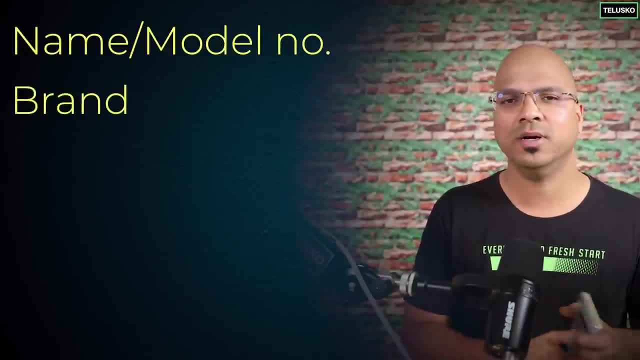 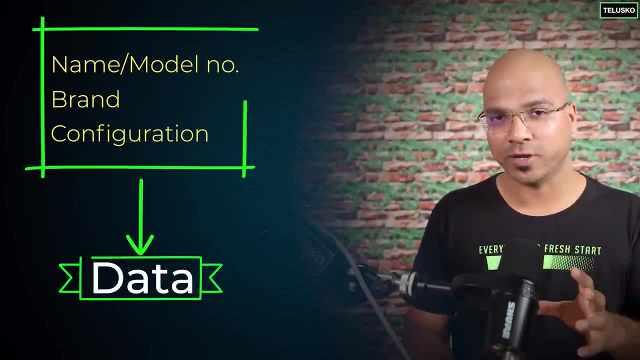 right. So it will have a name, It will have a brand, Of course. name is model number, Then brand, then the configuration, the amount of CPU RAM, all this are your data, right? So if you want to represent any physical thing in, 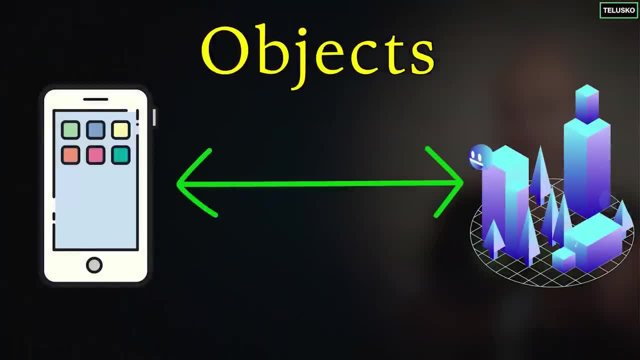 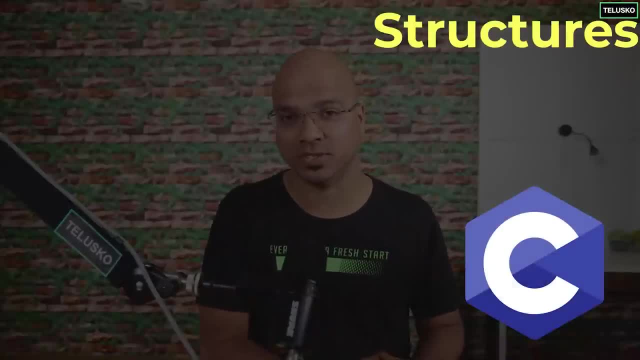 the virtual world. we use objects there. right Now, in some languages which are object oriented programming we do that with the help of objects. Example: in C we use something called structures, So we can define a structure name, let's say phone. 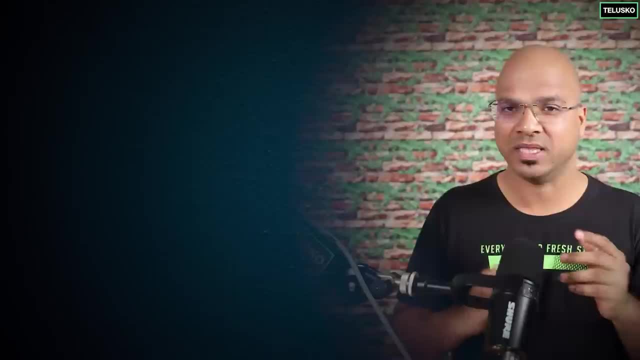 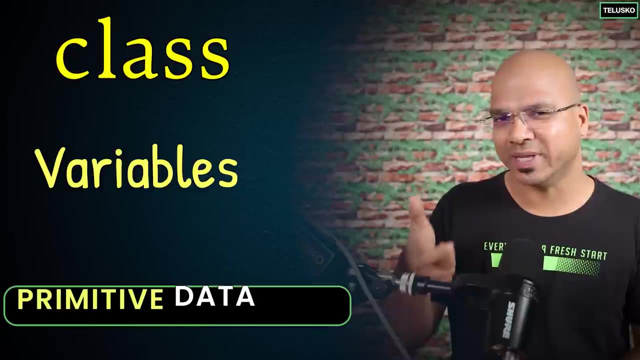 And inside that you can specify what are the properties that in the same way, in the object oriented languages we use something called class. In this class you create different variables with primitive type, And then the box itself or the class itself is your complex data type. 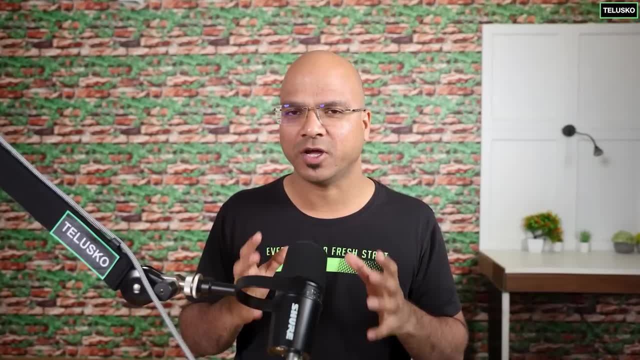 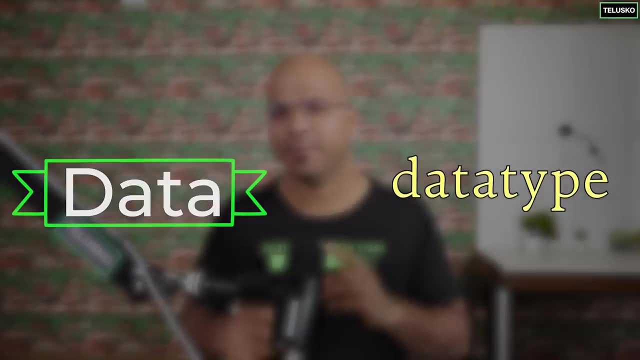 or you can say: user defined data type. User defined because system is not giving you. we are defining our own type, right, So that's about data and data types. But let's say, if you want to store a bunch of data, how will you work with that? 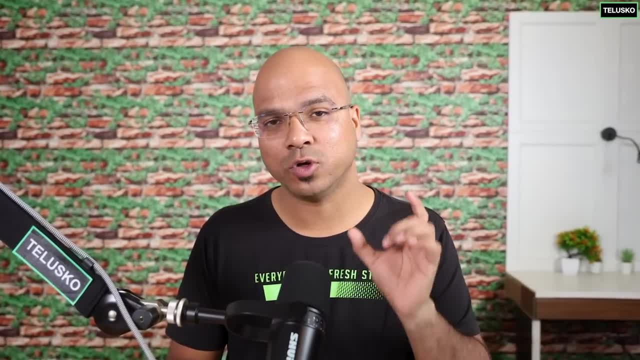 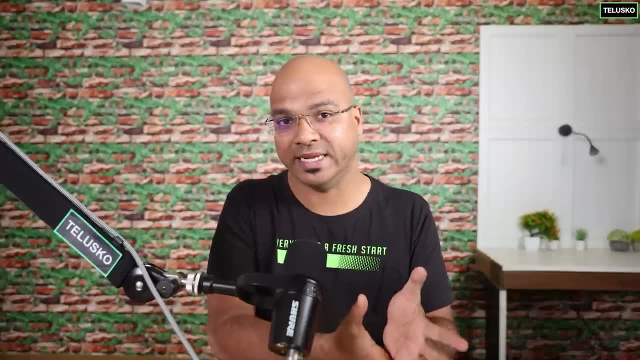 And when it comes to data structure, how will you store this data in a proper way? See, what happens is when you talk about primitive data, primitive types as well- every type will have a way to store data. Of course, that's what we are getting them. 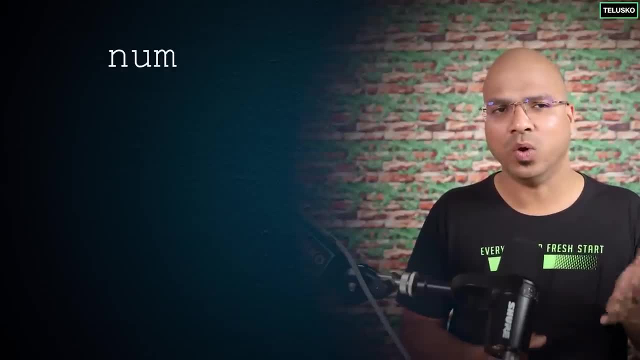 right. So example: if you are creating a variable called num, now let's say this num is of type integer and then you are storing a value to it. Now, with this variable num, you can perform operations as well. Now, what are the options you can do with integer? 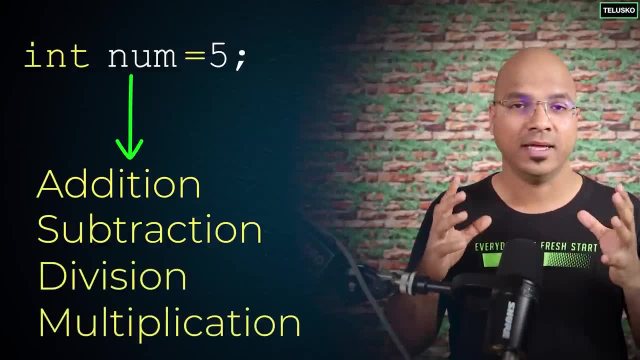 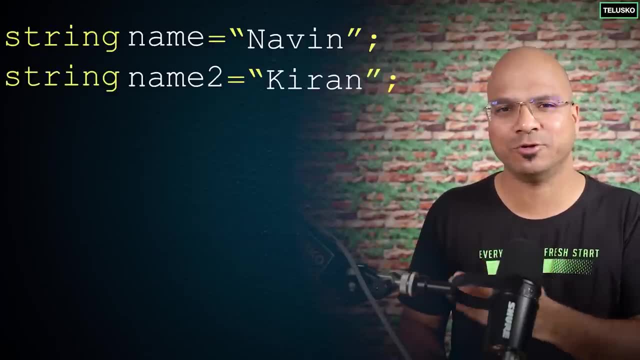 You can add two values, you can supply two values, you can divide, multiply, So you can perform those operations on the number. but let's say you have a string there. Now, with string, of course you will not be adding to string. 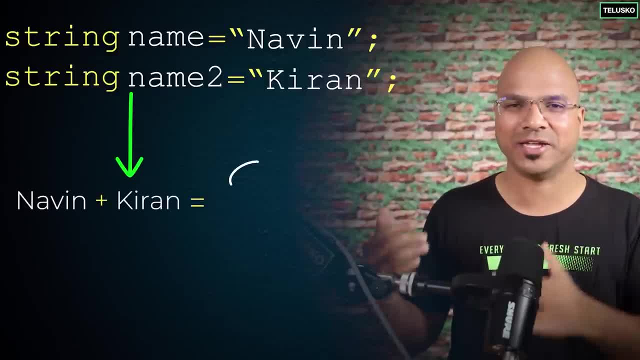 That doesn't make sense, right? Why? you will add two names, let's say Navina and Kiran. you will get a new name. Okay, A lot of parents are doing that for their kids, but that's not the idea here. 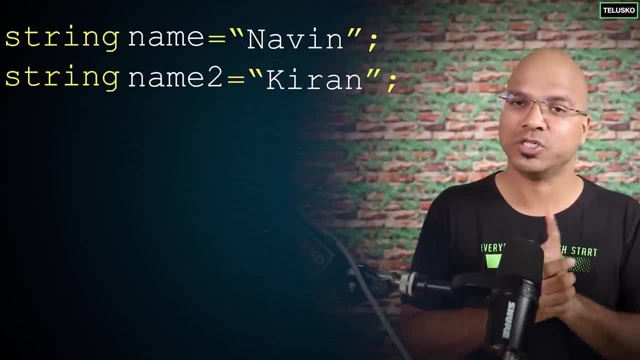 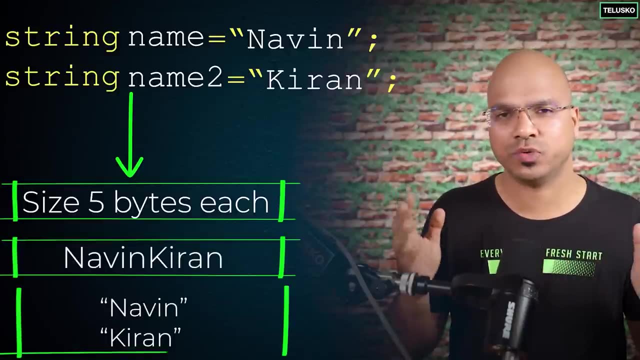 right, We can't add a string, We cannot subtract strings, but yes, which string. you can do something else. Maybe you want to see the size of a string, Maybe you want to concatenate two strings, Maybe you want to cut two strings. 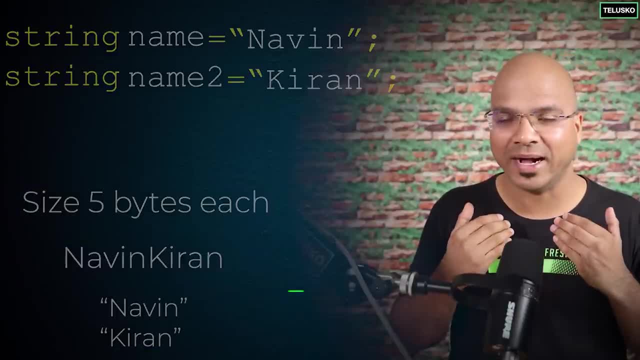 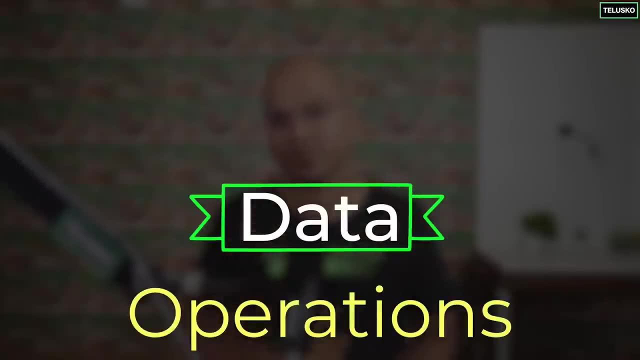 So string has different operations. in the same way, If you are creating your own type, this will have data, of course, but also you have to, you have to mention the operations which are going to perform. So we have two things right. We have data. 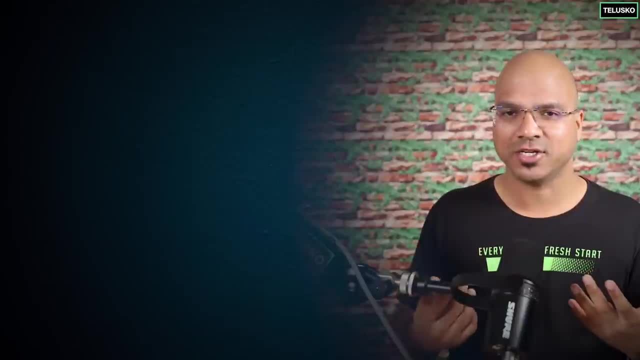 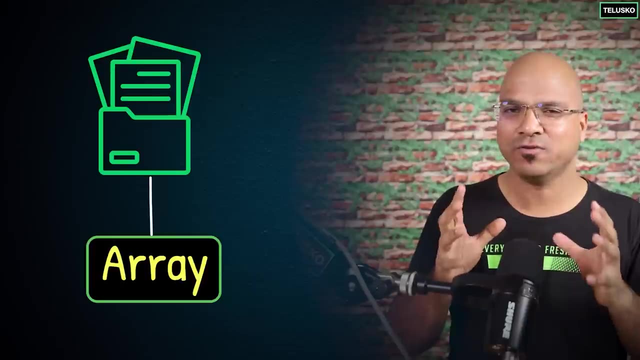 And we have operations. Now, let's say, in data structures, you want to store a bunch of data, as we mentioned, and you want to store it, So there's a concept of adding. So, if you have multiple data instead of showing them in multiple variables, 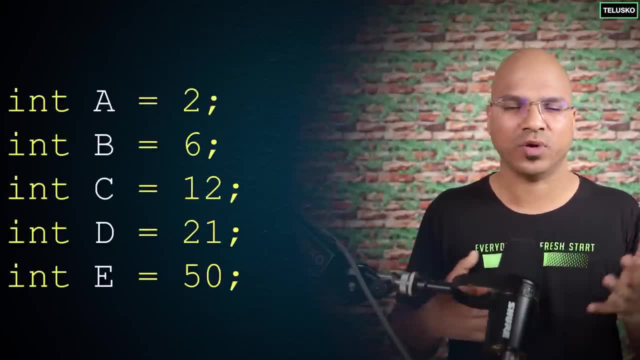 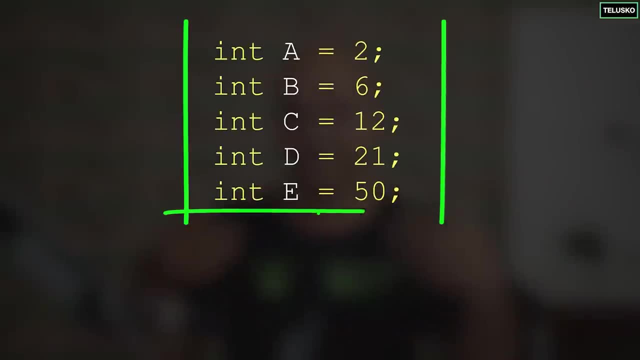 let's say you have five numbers, two, six, 12,, 21, and so on. Now, if you have all these values, you basically store that in five different variables, or you can create a single array and you can store all the. 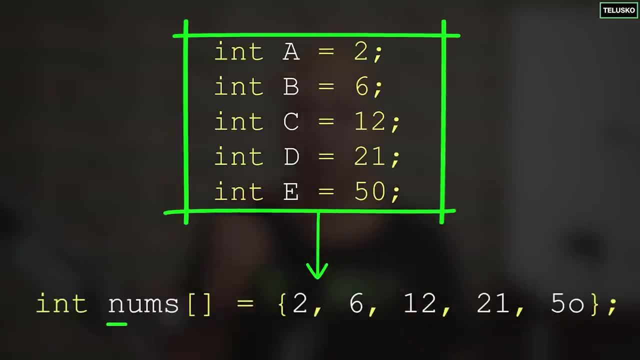 values there. The advantage would be you have just have to use one variable name there. So instead of saying A, B, C, D, E, you can simply say nums. You can use any variable, It doesn't matter. So what's important is you can use add a here. 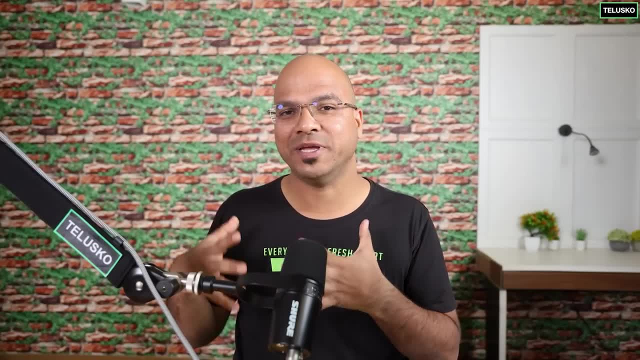 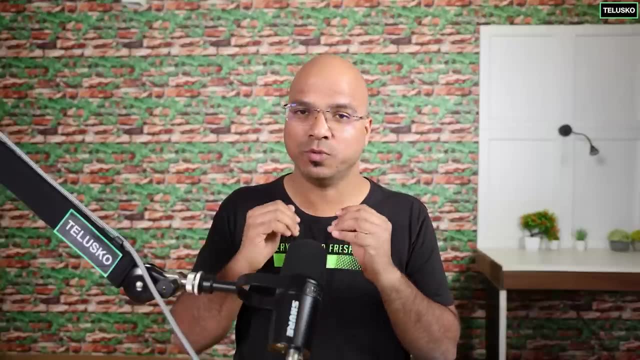 Now, when we use add a, we are not basically using a primitive type here. We are creating our own type here, own data type, which is an array. Now, in this array, basically, you should be also able to perform some operation. example. 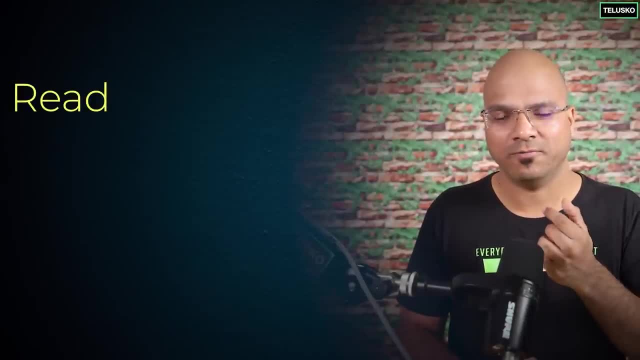 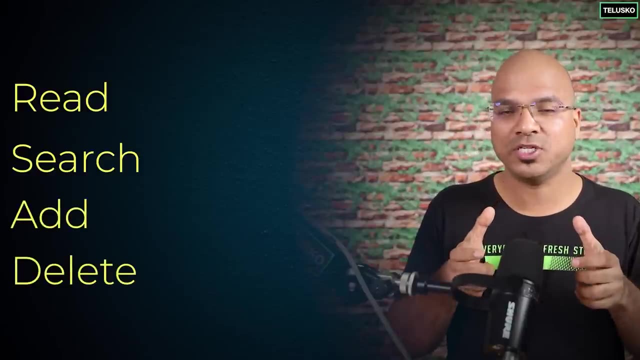 Let's say what, if you want to read some value, you want to fetch a particular element, You want to search the array, Maybe you want to add an element, Maybe you want to delete an element, So this operation should be possible on that type. 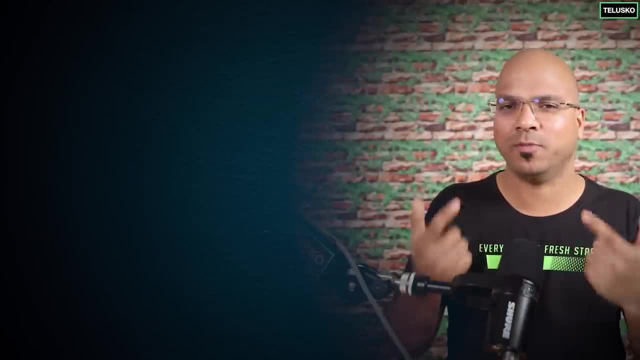 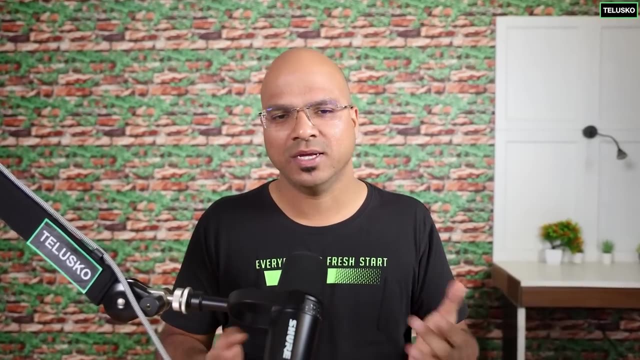 So in the concept way, when you have a type where you can perform some operation, we call them as abstract is because the implementation for adding changes from language to language And we don't just have added right. So let's say, if you want to store a bunch of values, 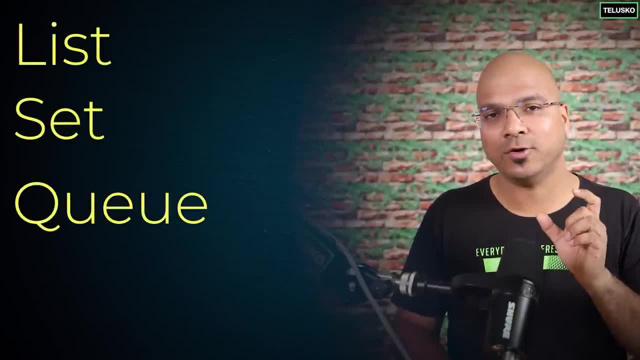 we can use list, We can use set queue. Now, when you talk about a queue here, let's say now inside queue, we have, I mean, we have one more option for that, which is stack. They follow different concepts. 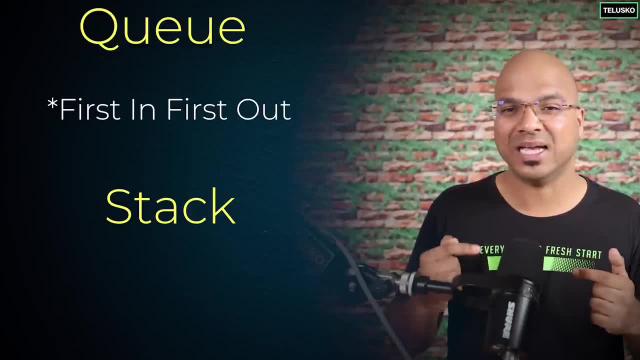 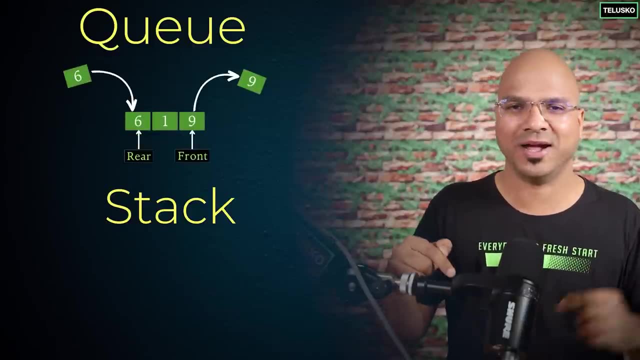 So let's say, if you want to add element, the queue which follows last in, first out, which means you have to insert from the end and you will get it from the first. Of course you can reverse it, You can insert from the start and you can take it from. 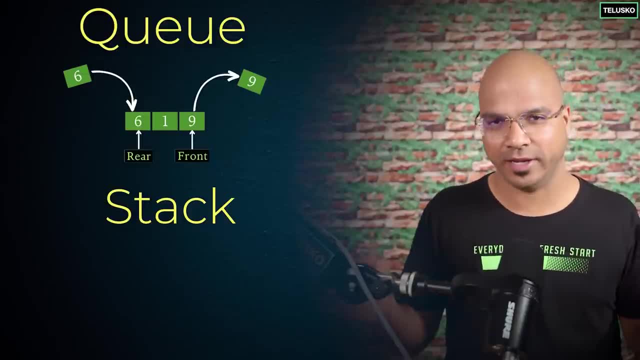 the end. The thing is you have you will insert from one end and you will remove from the other end. So that is first in, first out. in stack It is reverse: You do last in, first out. example. Let's say, to give an example: 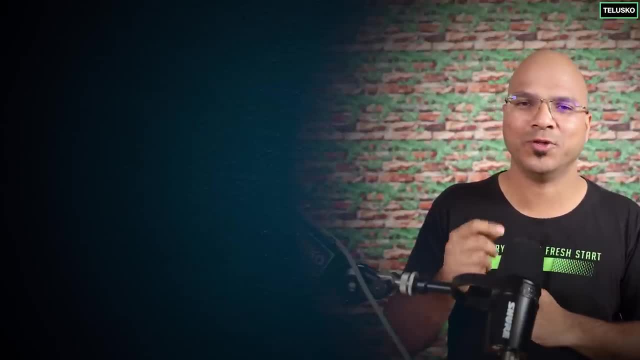 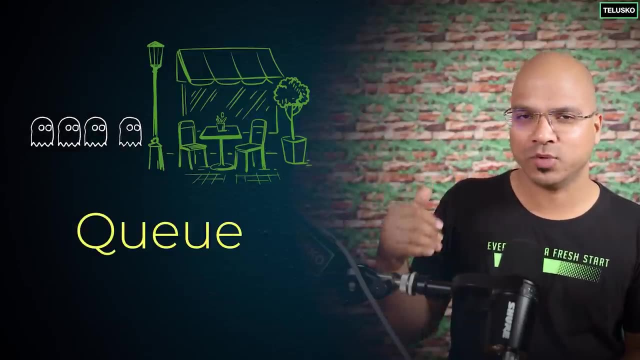 let's say, for queue we can say a queue which you follow right. example, If you want to buy a coffee from a cafe shop, of course there's a queue there. You have to stand in a queue And then, when your number comes, 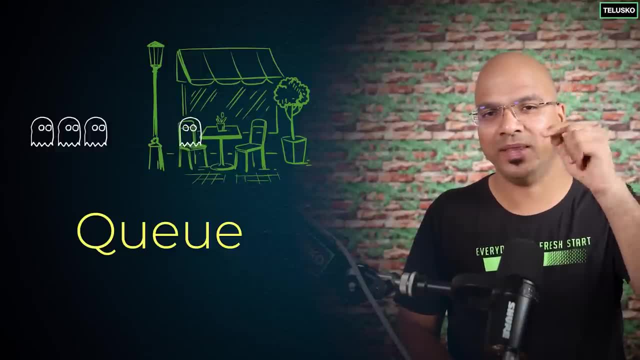 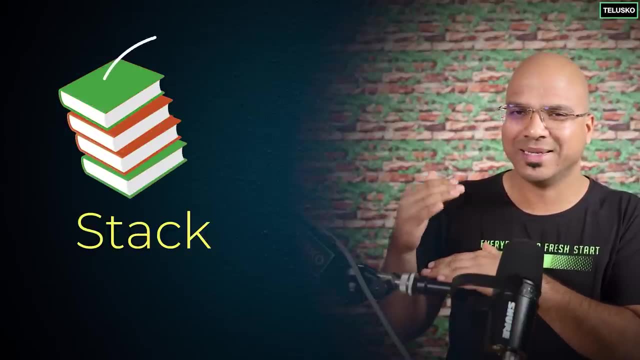 you will get the coffee. So basically, the first person who went there first we'll be getting the coffee first, right? In terms of stack, it is different. So when you keep multiple books, the first book which you can take out is the last book. 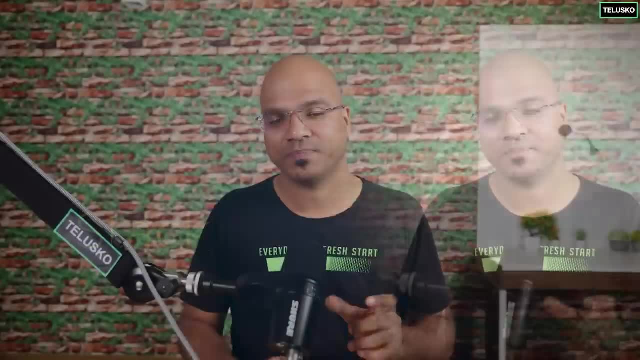 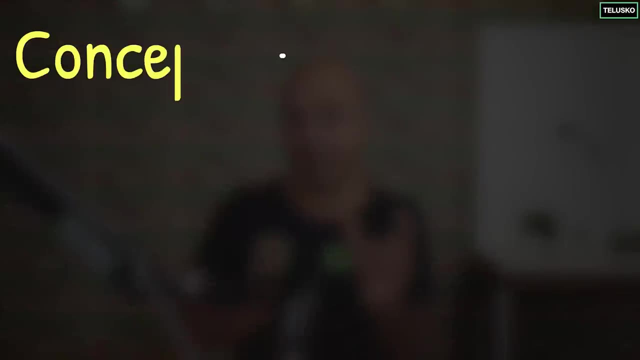 which you have kept there right Is the last in, first out. That is your stack. Now we have different way of implementing in different languages. The concept remains same right. So when you have a concept and the associated operations to it, 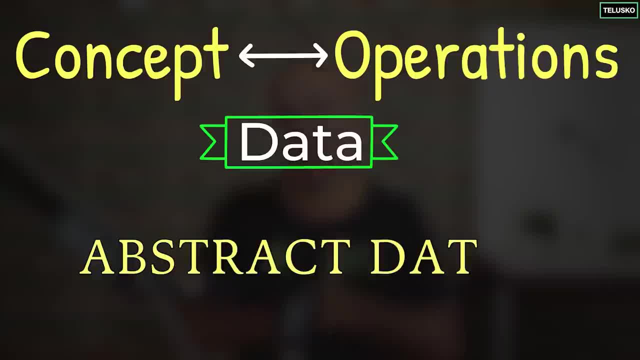 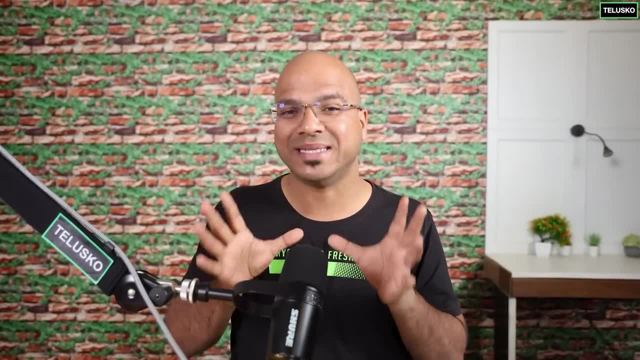 and, of course, with data which we call them as abstract, abstract data type. we also have map, but we'll talk about those things later. at this point, The point to remember is: we can create our own types, and which is a concept. 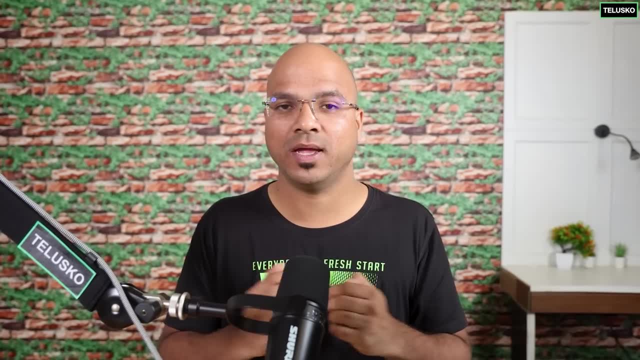 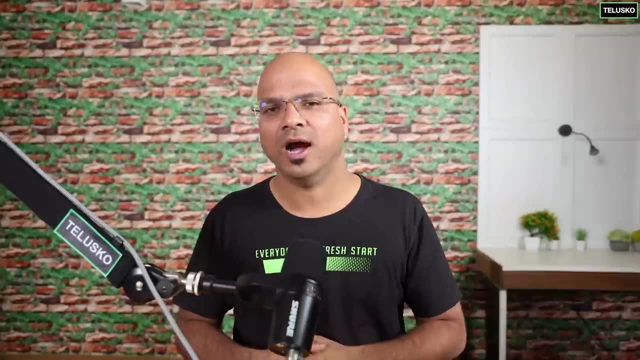 And if you want to have data inside that and also you want to specify what operations you can perform, that is your abstract data type. Of course, in the subsequent videos I will talk about how do you create them, How do you work with them. 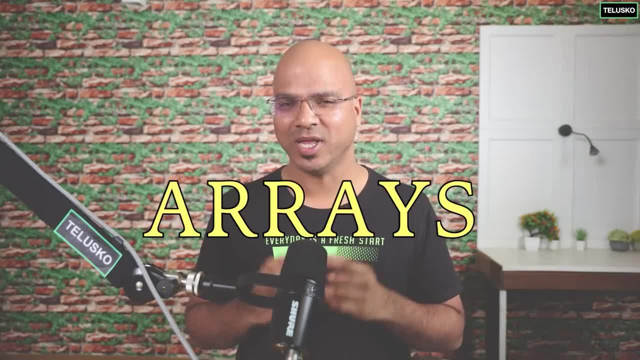 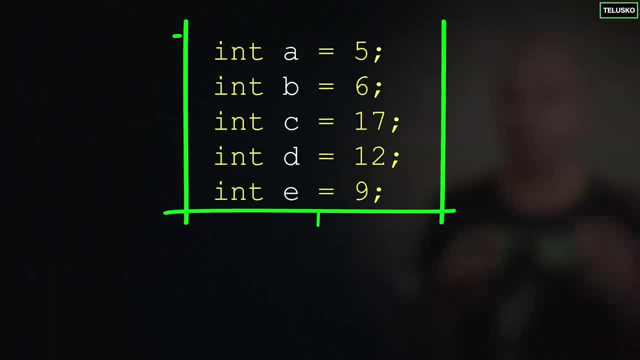 And it will be fun. in this video Let's talk about arrays. So let's say you have a bunch of values, Let's say five values. Now, instead of storing them in five different variables, we can store that in one particular sequence. 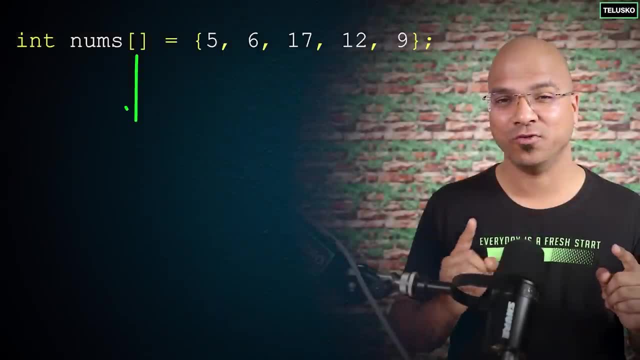 right, Or one variable. You can say: now, in this area you can store five values. So let's say we have this area here and then this will have a name to it. Now, of course, this data will be stored in a memory. 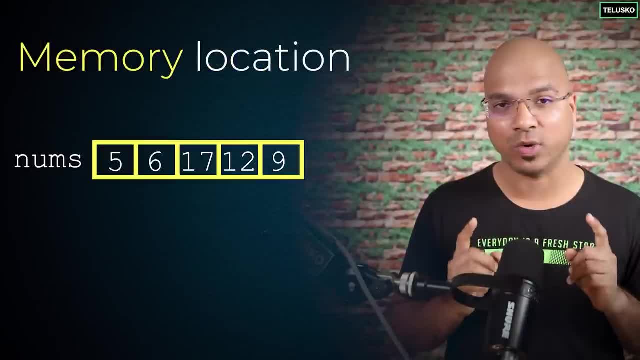 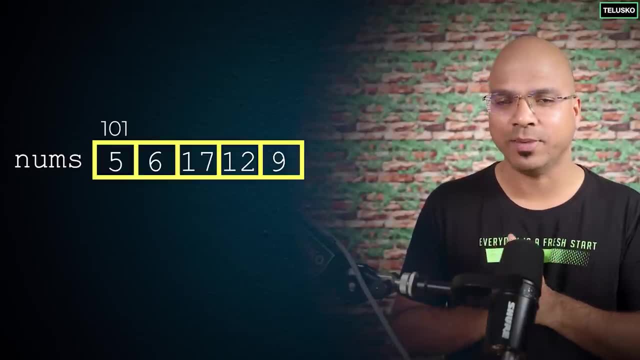 right, And every memory will have something called a memory location. So let's say we are storing this data in at a location, one, zero one. Now what happens is, every time you store a normal variable, let's say a premium, you type: 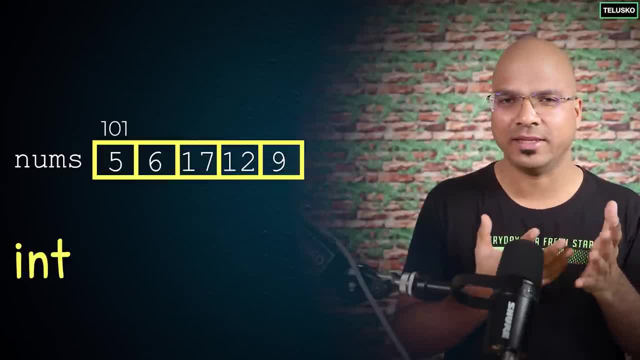 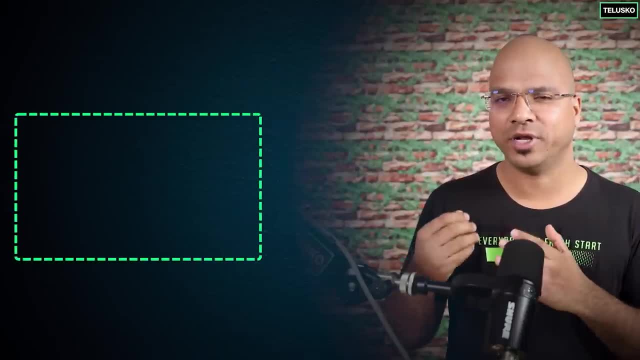 let's say ain't and depend upon how much sizes take. So every type will have a different size to it depending upon a language. But let's say we have two bytes now inside your memory. Let's say: if you create a normal variable. 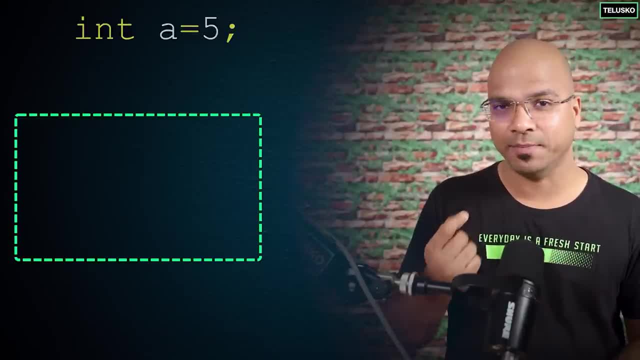 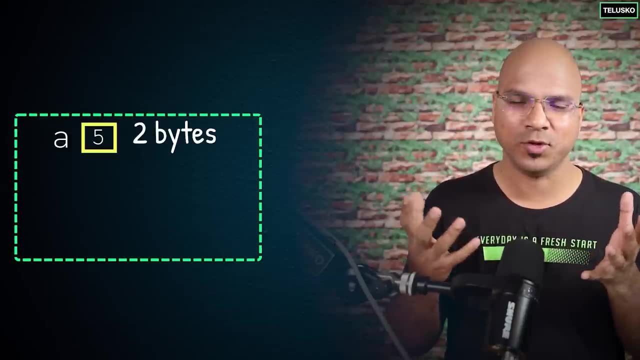 which is ain't a equal to five. Now, this particular a variable will take some space in the memory, Of course- let's say two bytes- and it will also have an address to it, right? So every time you, in your programming language, 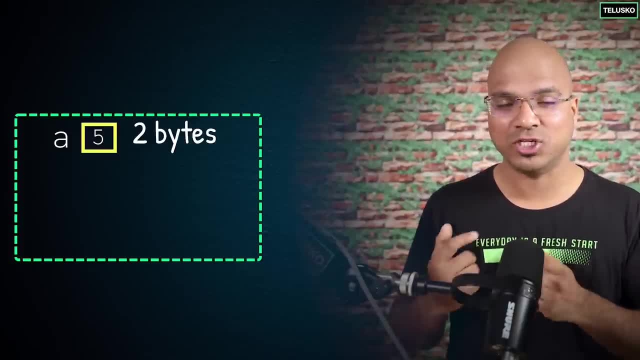 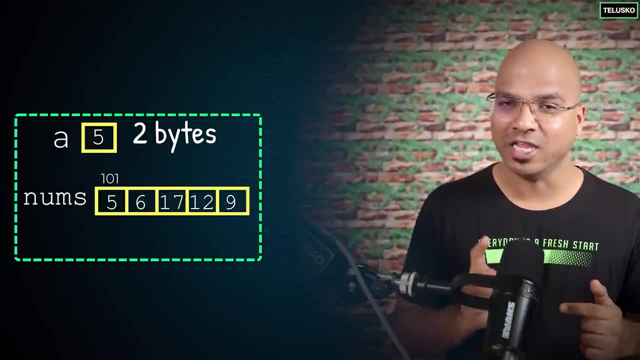 you say, Hey, I want a value for a, the program will jump to the memory location by searching for the address And it will get the value. But the problem is when it comes to adding, we have multiple values right And we only have one address. 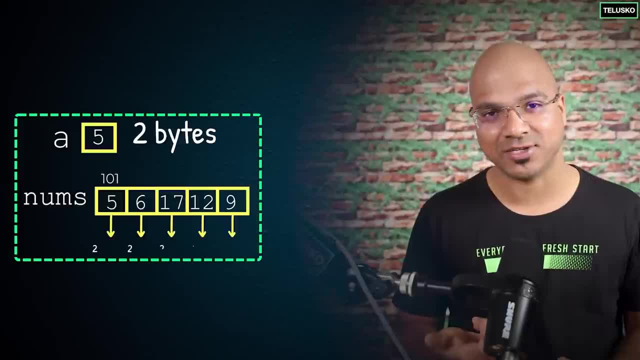 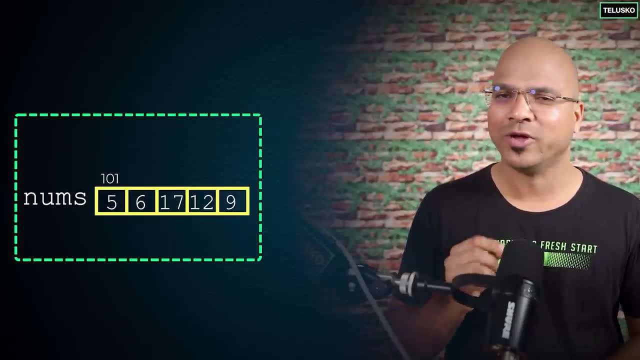 Now that's tricky. Of course, each element here will take the same size. If you say ain't to take two bytes, the complete array will take 10 bytes is because every element will take two bytes. How will you allocate memory now? 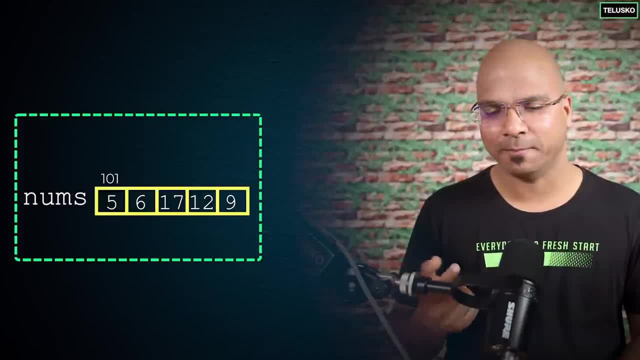 That's an issue. So what you do is the array will have a memory, but that will. that is only pointing to the first location, right? So if you say the memory for this is one zero one, the first element is one zero. 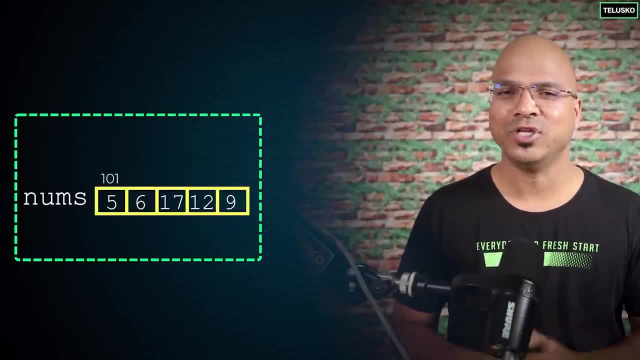 one. what about the second element? Now? that's where we have to use something called a index values. So let's say the first element is: look, is at one, zero one. So it will have a index value which is zero. The second element is one. 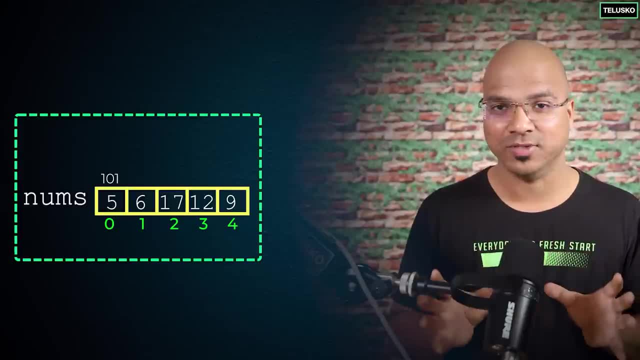 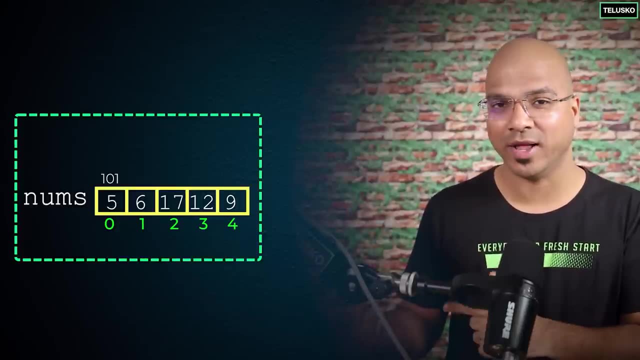 then two, then three, then four. right Now for five values. the index value starts from zero and ends at four. Now, why zero is because we're starting. we have a memory allocated right, One zero, one which represent to the first element. 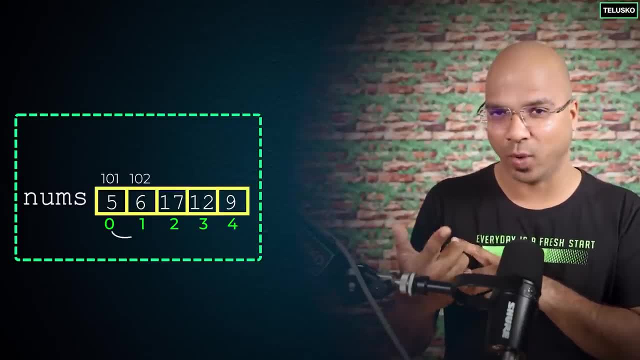 So we don't have to give one to it. So what you do is the next element is plus one. That's why one, two, three, and then you can just get it right. So one zero one, let's say, if you want to get the third element. 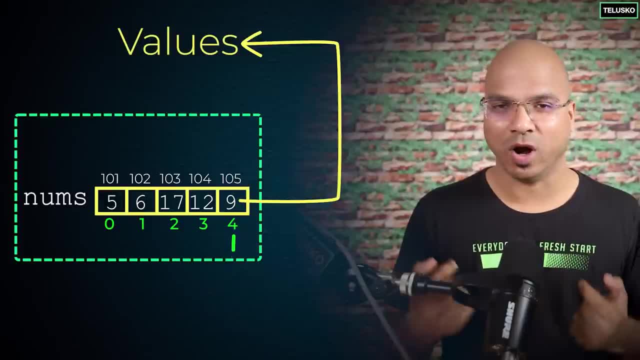 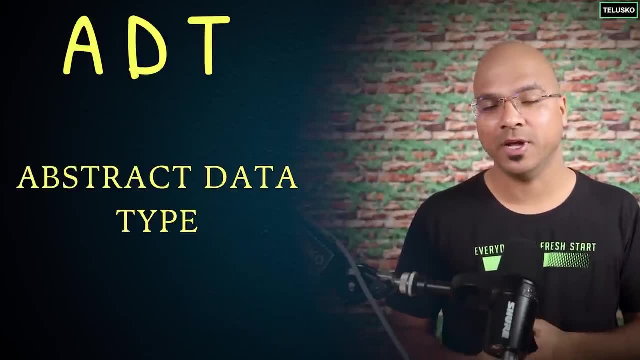 you have to say plus two. That's how we do it. So you got the values, you got the index and you also got a memory address to it. Now, with this, add a, as we already talked about ADT, which is abstract data type. 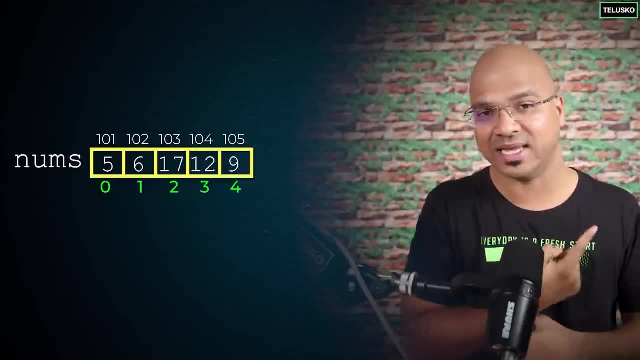 we should be able to perform some operations. Now, what opportunity can perform on this area? Now we can perform something called a read operation. So what is read? So let's say you want to get the value of index number three. Now what? 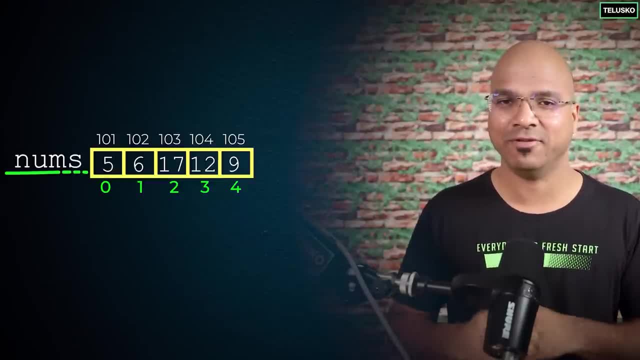 what? what you do in this case is you say, okay, my area name is nums, And then for this nums I want the value at index three. So in different languages we have different representation for this, but let's say this is common one. 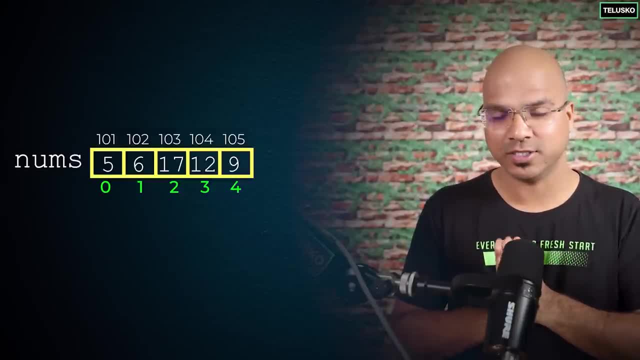 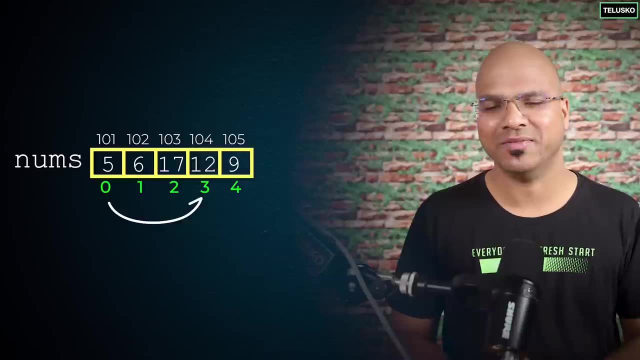 So nums bracket of three. Now what your computer will do is it will directly jump to the memory address. It's very simple for the for that right. So you will say one zero one plus three. you will get the value. So that's how you do it. 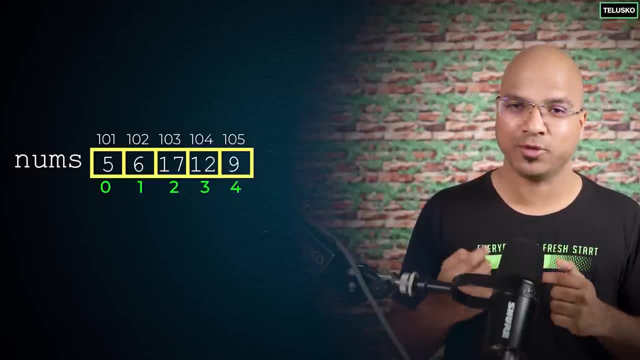 Now, reading is very easy and computer takes way less time to jump to that particular areas, because the computer knows the memory right, Because you, you are mentioning the index value, reading is good, It's fast. Also, what about searching? Now, this is tricky, because when you're searching, 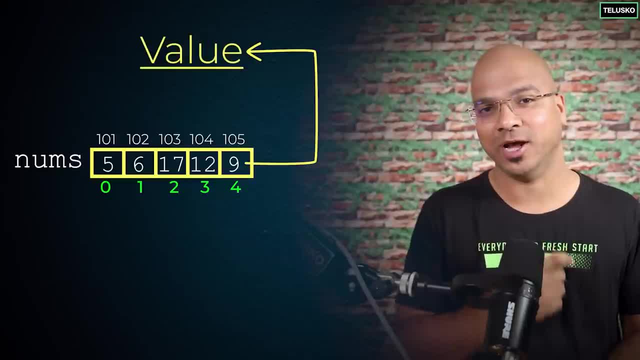 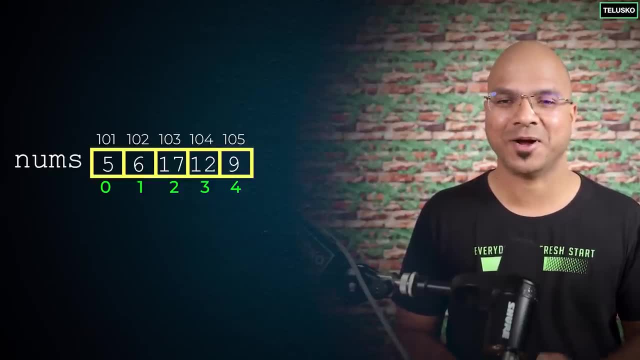 you're not searching for the index, You are basically searching for the value. now. So let's say, from this area I want to search what is 17.. Now, in this case, your computer has no idea where 17 is, because company only knows about the memory address. 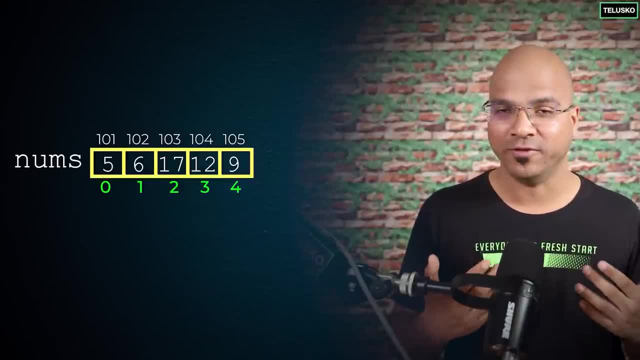 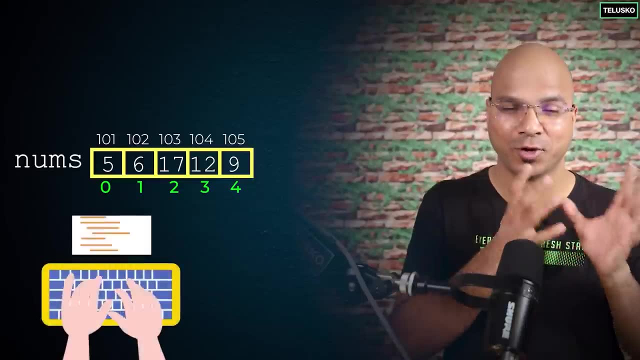 Of course the values are there, but computer has no idea in which location we have that value And do we even have that value? So what a computer will do is it will start on the first location. So basically you have to write a code to search from the first location. 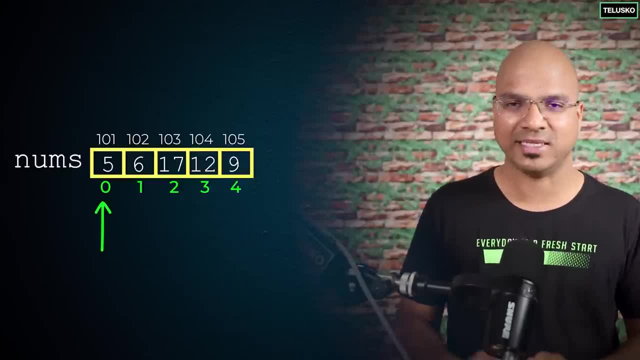 You have to check is the first one, 17.. If yes, good, we can exit. No, Then you have to jump to the next location. Is it matching? If yes, good. If not. next matching: yes, no. next. 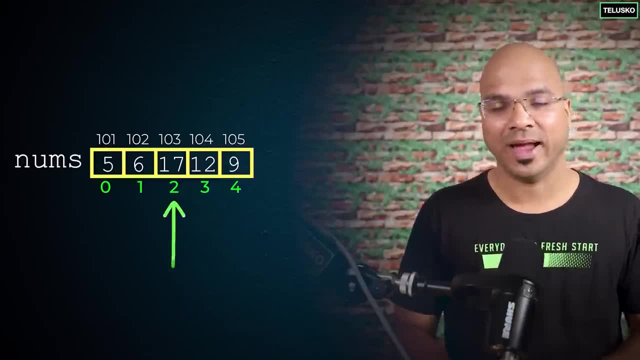 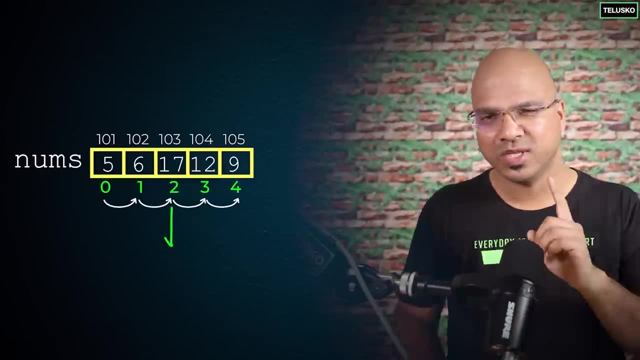 So, basically, you have to search each element, right, And let's say the element is at the end. You are searching, you are basically tracking to all the different locations. So this is time consuming, right? What if you have a array of? 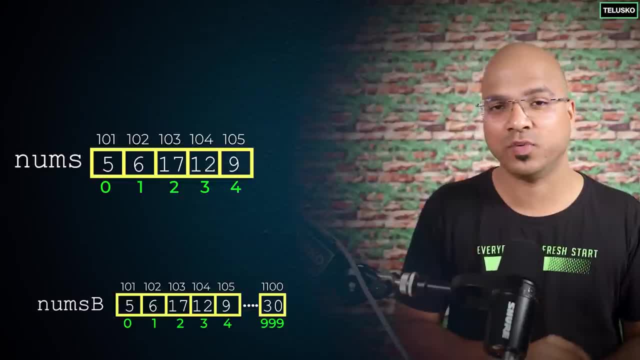 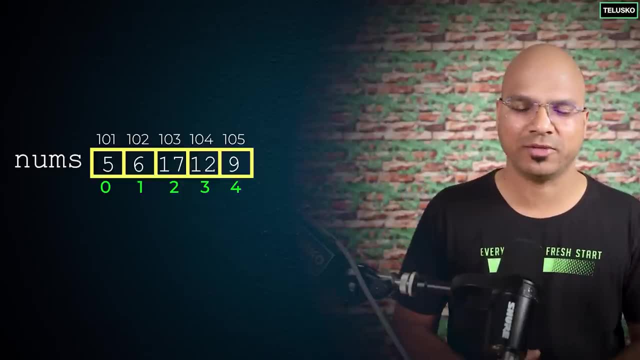 let's say a thousand values. to move between this values It will take some time. What about inserting? Now this will be tricky is because, see, if you want to insert a element, what do you think Will it take a lot of time. 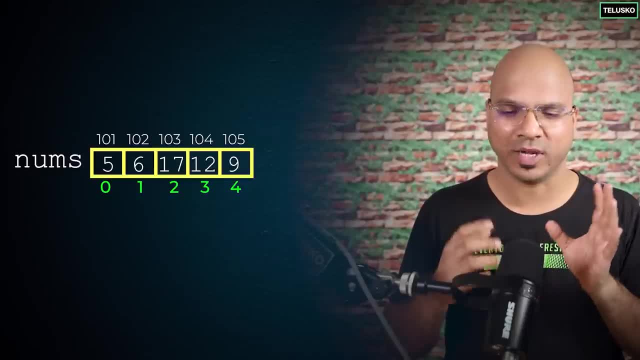 See if you want to insert the element at the end. that's very simple. You can get the size of the array, because we also have to have that option of getting a size of the array right. So let's say you have five values. 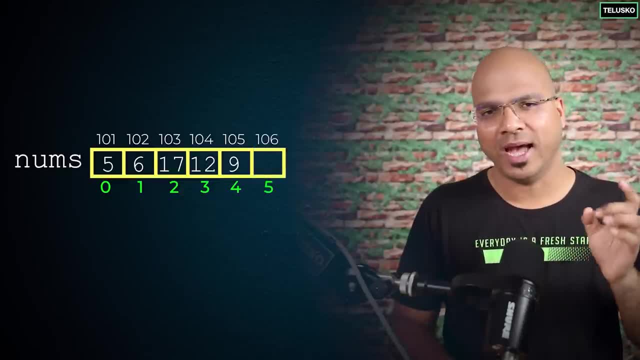 You will. you will simply jump to the sixth location, which is index five, And then you will say: okay, I want to add a value here. Let's say the value value is 21 and you can add the value. it's very fast. 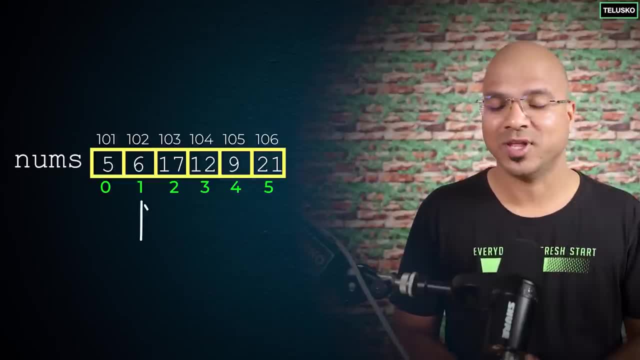 but what if you want to add a value in between? So let's say you want to add that value at the second location. So after the first, you want to add the new value. Now what you will do is you don't have a space there. 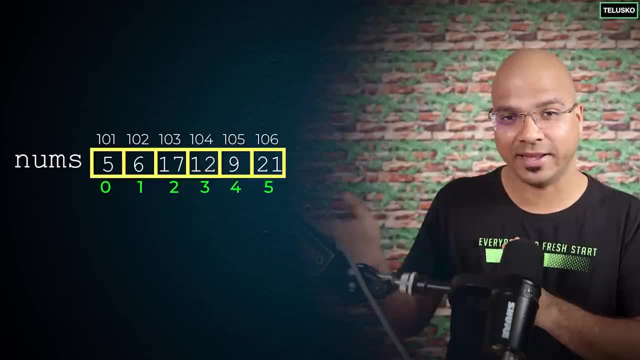 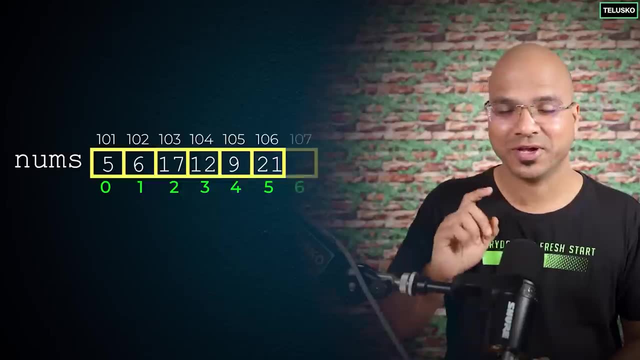 right. You can't simply create a new space. You can create space at the end. So what you do is you basically have to move all the elements and you- it's not like you can simply move the elements- What you do is create a new block. 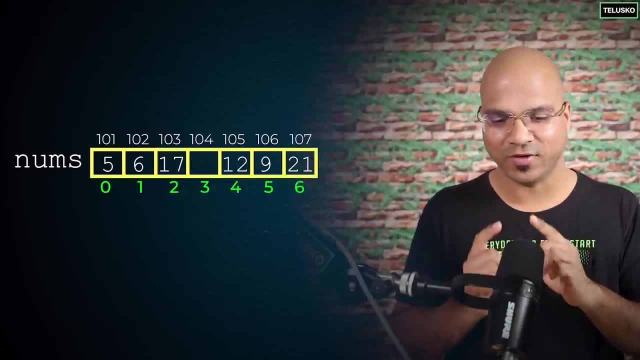 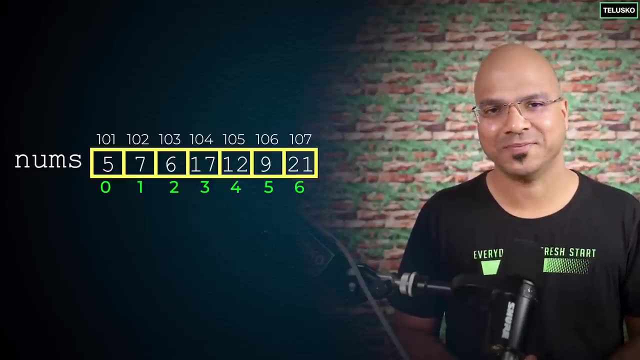 So move the second last element now to the last block. Then again you have to move every element one by one. Then you can add your value to the second location. So if you are inserting at the end, that's fine, But if you're inserting in between, 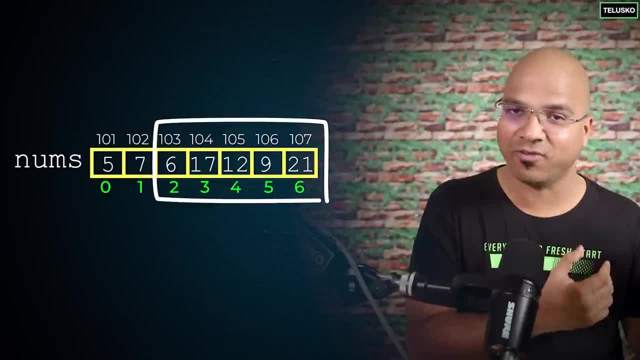 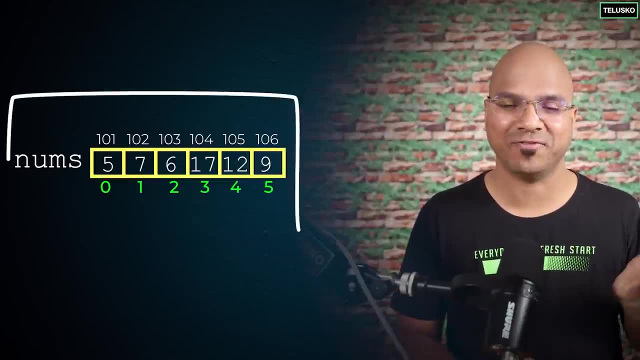 that will take a lot of time And that depends upon the number of elements after the position which which you're adding. What about deleting? See deleting from me from the end is always welcome is because you're not affecting your array in total. 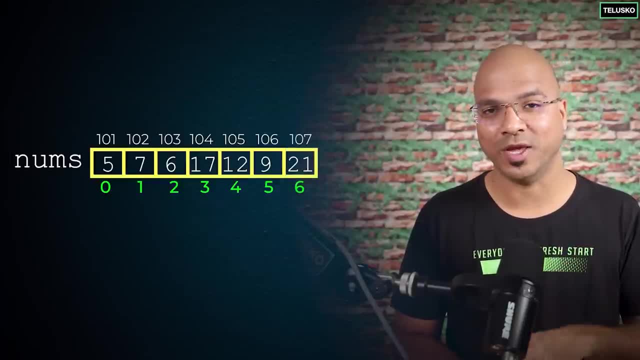 But what if you want to delete a particular element from between? now you can't simply delete from the between right? You've delete the end block, but how will you move So again when you have to do, when you want to delete this? 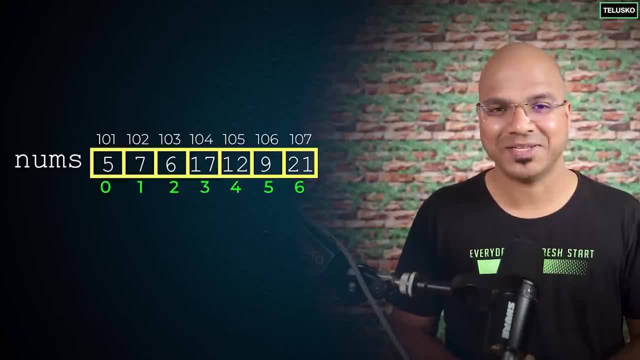 just replace all the values, right? So that's that's tricky, So it will take a lot of time, depending upon how many elements you have after that index value. Now, while we are talking about all this thing- and it was simple- 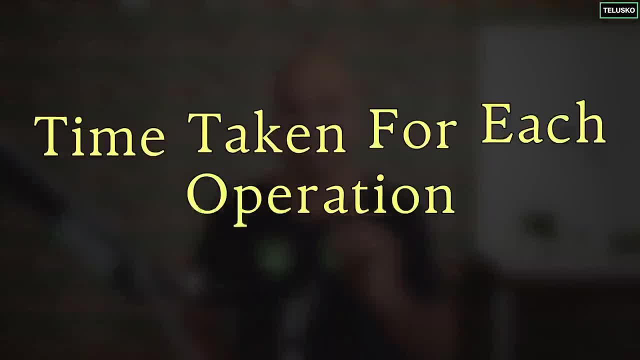 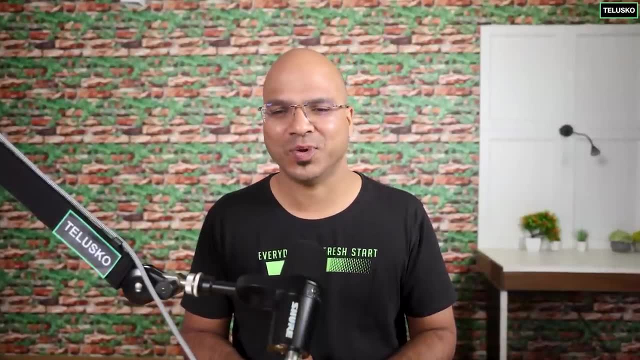 right, We can perform the operations. The important thing here is time taken for each operation, And it's not about CPU time. If you're thinking my computer is super fast, it will be happening very fast there. See, in the world we have different computers and different computer have different CPU power. 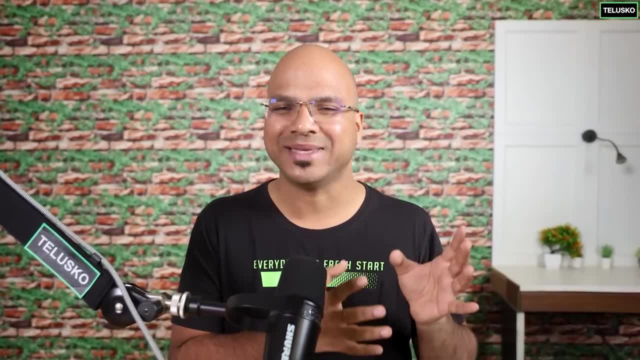 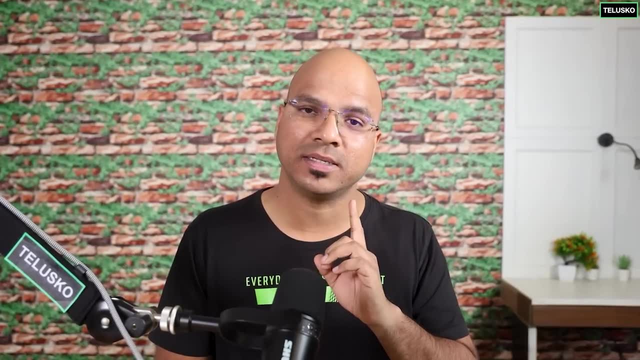 different ramp power, different configuration, And that's why let's not calculate the speed of our speed of a code or the algorithm by the actual runtime. Important is the number of steps it takes. example, Let's say, if you want to insert the element at the end. 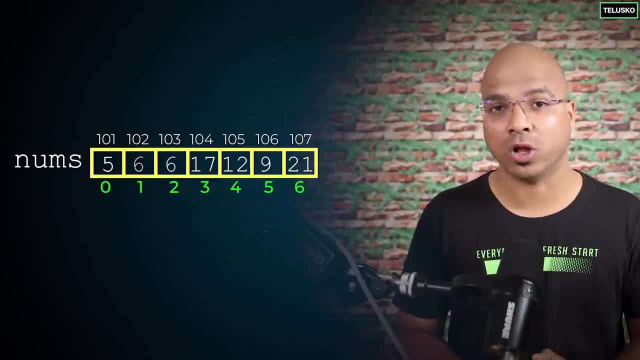 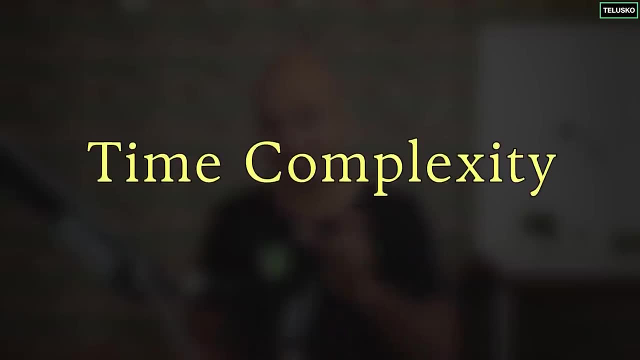 that's good. If you want to insert the element in between, that will take a lot of steps- is because you want to move the elements right now in the upcoming videos, where we haven't also talked about time complexity, which is a very important concept. 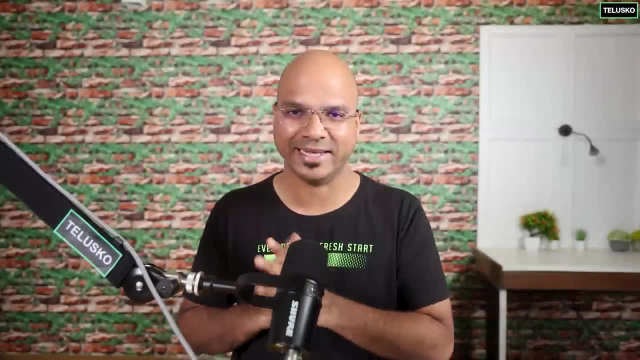 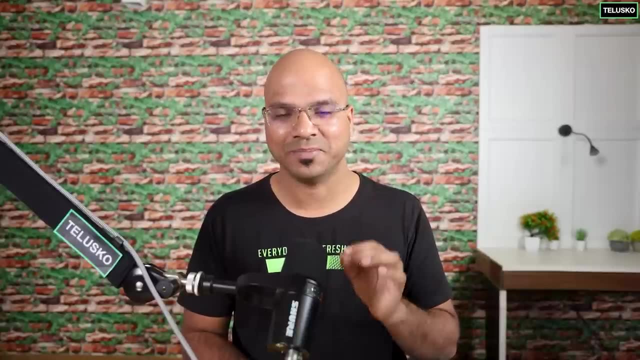 something called a big, big O notation. But yeah, we'll talk about that in detail Later. I know you're excited to hear that. but important thing is, when you write a code, think about the number of steps your code takes. 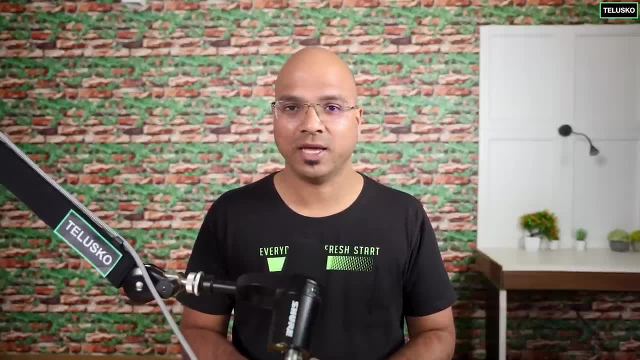 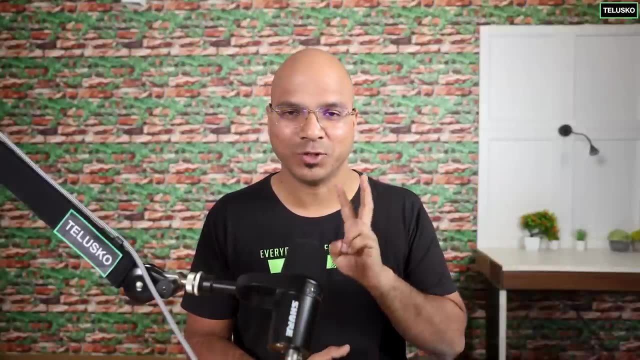 because that defines your time complexity. And if you say my algorithm is good, it should be time efficient. Okay, So for the same particular operation you can write two different codes. Example on the screen: If you want to print, let's say, 10 numbers, from one to 10,. 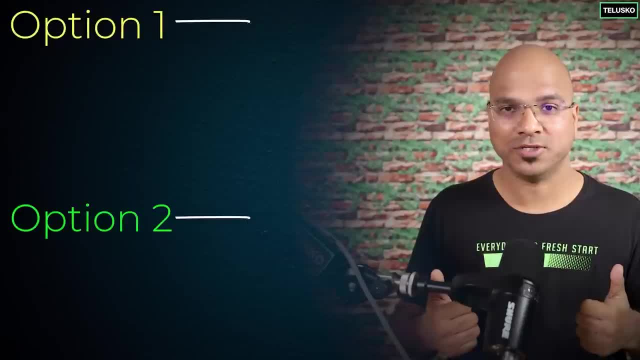 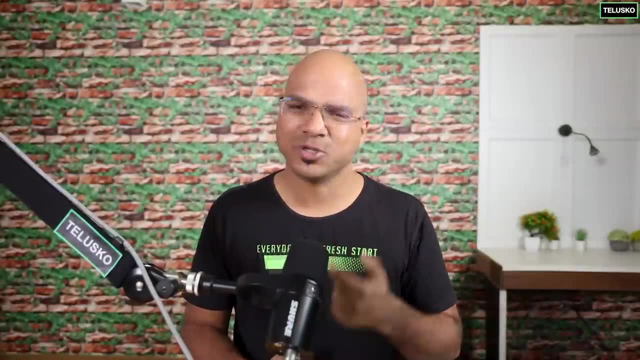 and maybe you just want to print the even numbers. We have two options there. which one is good, Of course, you will let me know in the comment sections, but the code which is not trading between all the values is good, right. 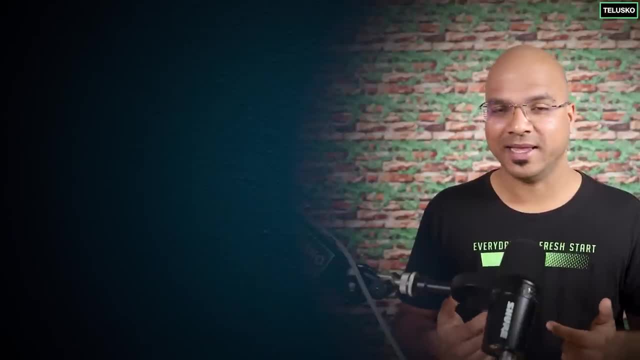 So that's how you define, how your algorithm is good. Now we can also expand the example. Let's say, if you have a sorted array, so let's say you have an array and this is sorted by default. So every time you insert the element, 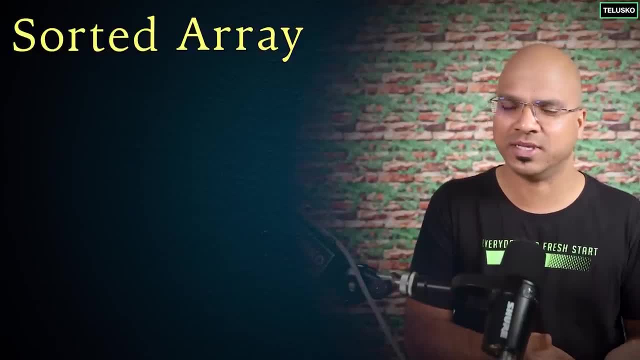 it's gets sorted by default. You don't have to mention where you want to insert this example. Let's say you have a bunch of values here, all are sorted, and now you want to insert the element which is 11.. Now 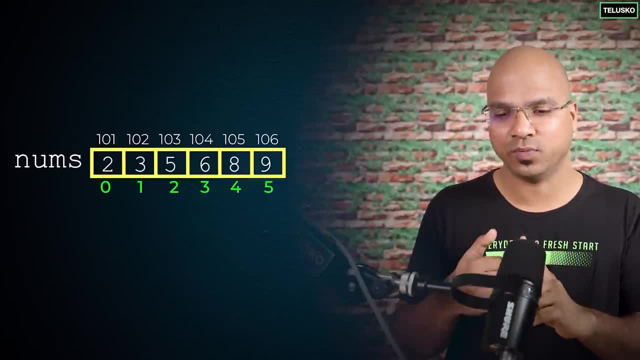 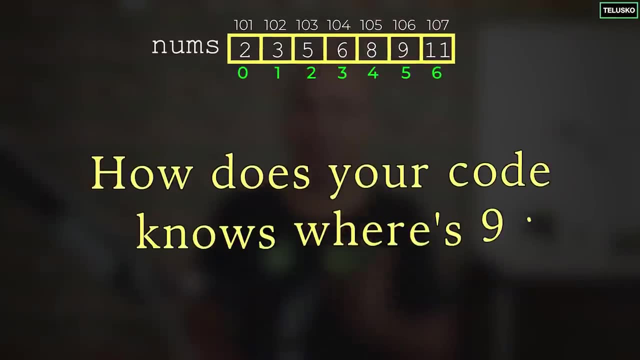 if you want to insert 11 there, where it will get inserted. of course it will search for the location. Let's say we have a number nine, it will get inserted After nine. Now the question is: how do your code knows where is nine? 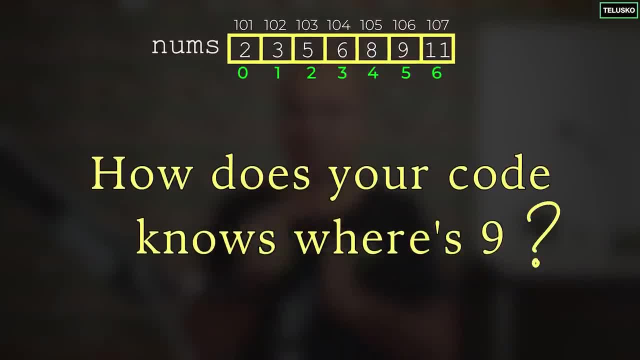 So you have to basically search, you have to match: Is it greater than? is it greater than? is it greater than? and then you have to insert. So that will take a lot of time. but what if you're inserting in between? 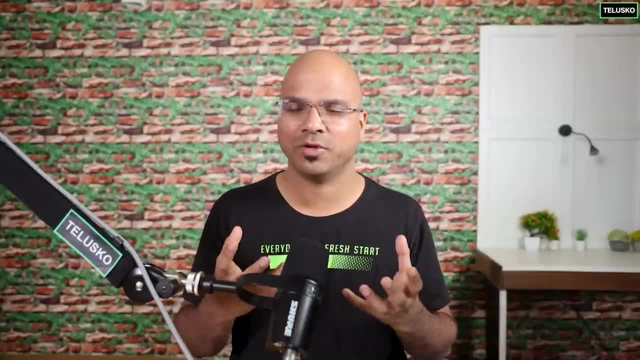 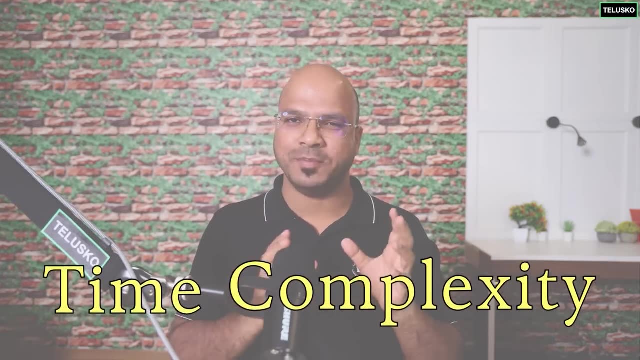 you have to shift all the elements. So that's about the array and a basic introduction of time complexity. We'll discuss that in detail later In this video. we'll talk about time complexity. See, the thing is, in the previous video we have talked about algorithms. 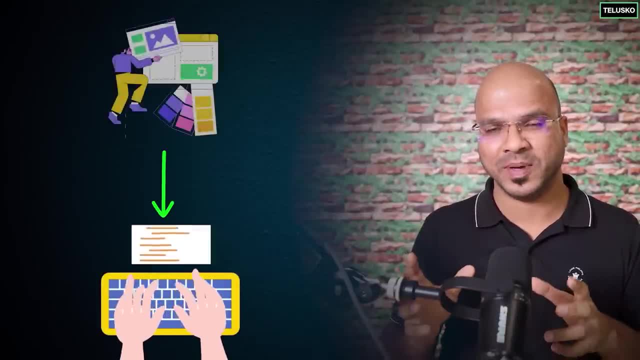 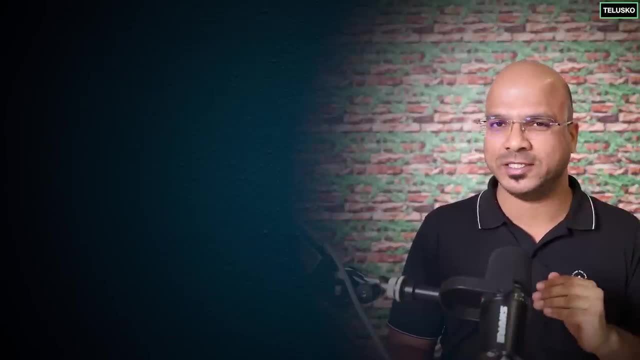 right Now the thing is: if you want to build an application, basically we are trying to solve a problem right, And every problem will have multiple solutions, So the steps which we write to solve that problem, that's what we call algorithm example. 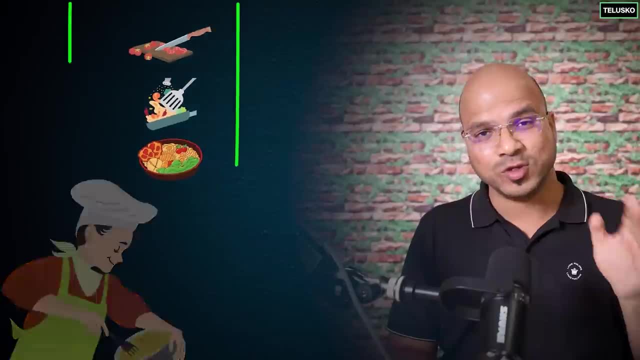 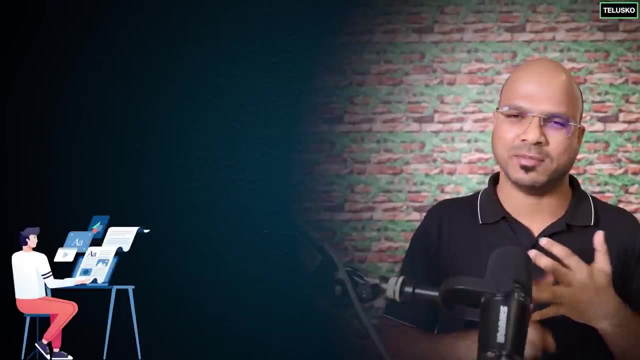 Let's say, if you want to cook something, you follow some steps. right Now, those steps are your algorithm example. If I want to record a video, we do multiple things. We prepare the content, we set up this camera, Mike. 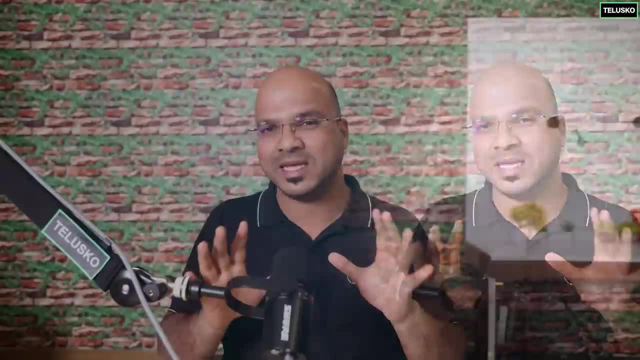 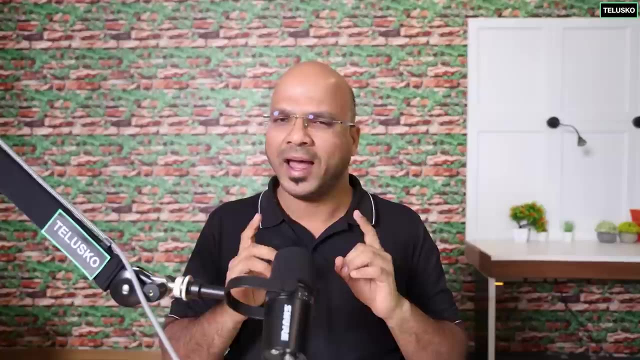 and then we start recording, Then we edit the video. So there are multiple things involved. in the same way, If you want to solve any problem, we have to follow some steps, which we call algorithms, And the thing is for one particular problem. 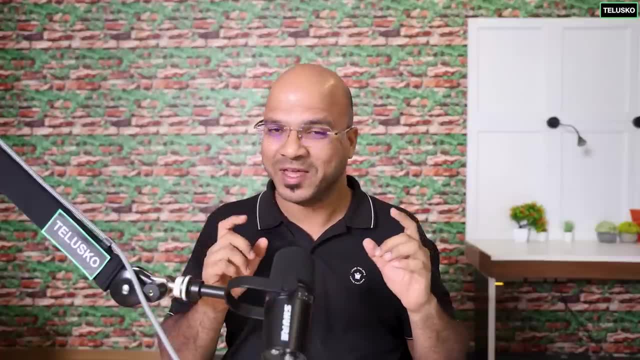 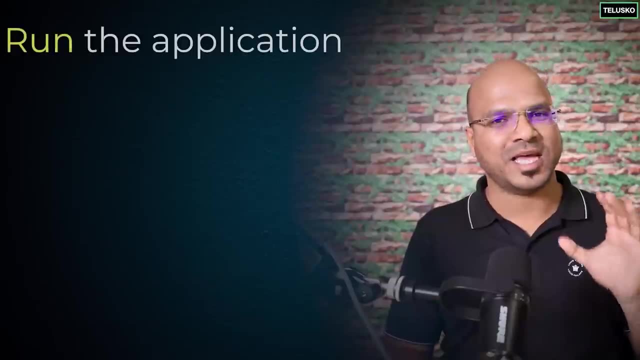 we don't have one solution, We have multiple solutions and we have to pick the best one. Now question arise: how will you choose the best one? So when you say best one, what exactly it means? So let's say, we're on this application. 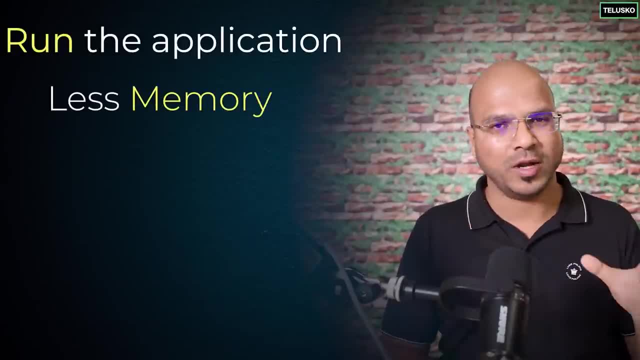 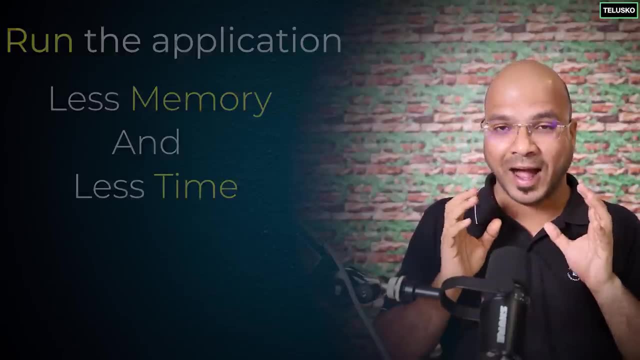 I want my application to use less memory, or maybe I want, when I run this application, I want it should take less time, or maybe both, And that's why we have this term called algorithm analysis. So, basically, you have to analyze your algorithm so that you can make it more efficient. 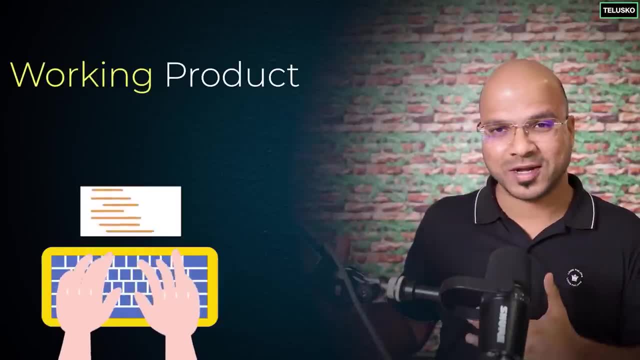 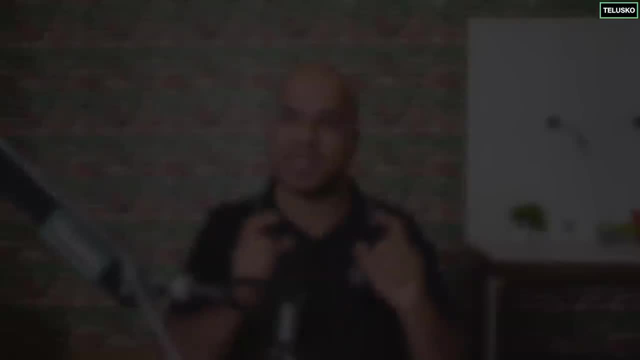 right. Of course, as a developer, first focus is first the production work and then you think about optimizing it. But when you say optimizing, you have to. you can optimize in two ways. One thing about the space- complexity, And second is the time complexity. 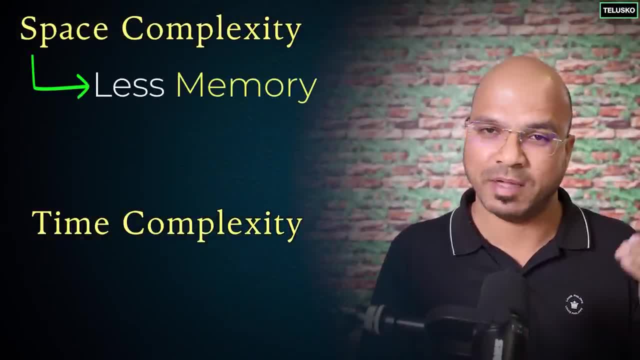 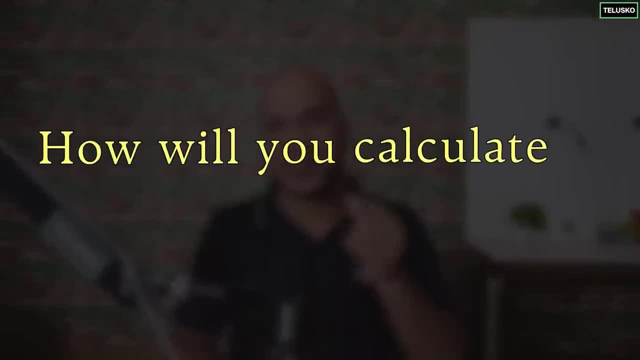 The space? complexity simply means: can we use an algorithm which will take less memory and time. complexity means it will, it should take less time. but there's one more problem here, And the problem is: how will you calculate the time or how do you specify the exact time? 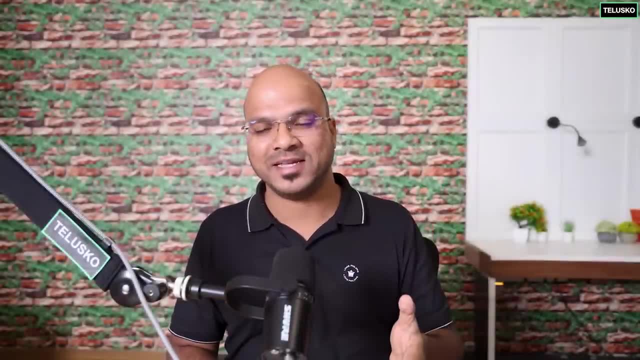 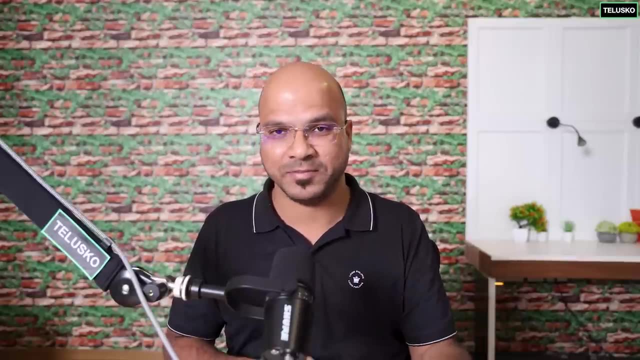 Because every machine will have a different output, right? So if you are testing the algorithm in your machine, it might give you a different time, And then the moment you test this in your office machine, it will give you a different time. So that's not the best thing to calculate the number of seconds it takes. 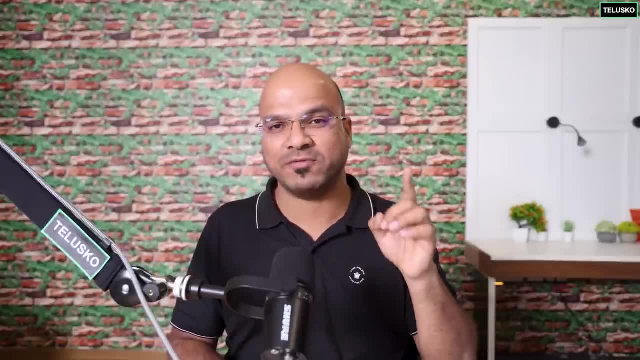 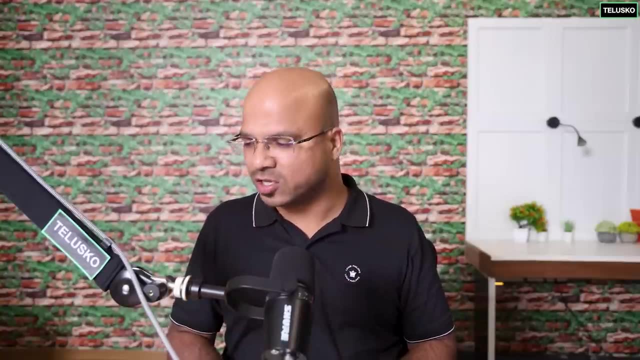 but what you can do is there's a way you can calculate with the help of steps, But before we go there, let's focus on two algorithms here, and then this will make much more sense. So the algorithm which we're talking about now is the searching and 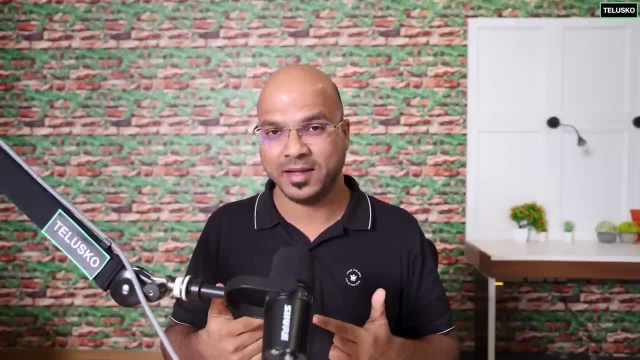 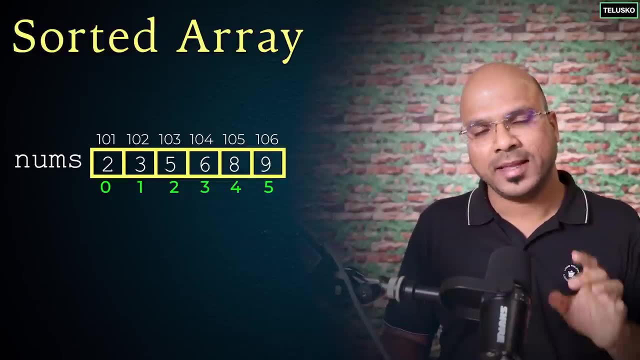 element in a sorted array. So in the previous video we have talked about array and then we also talked about the sorted array. So in sorted array, by default, all the elements will be sorted. right Now. what I would do is I want to search a particular element from 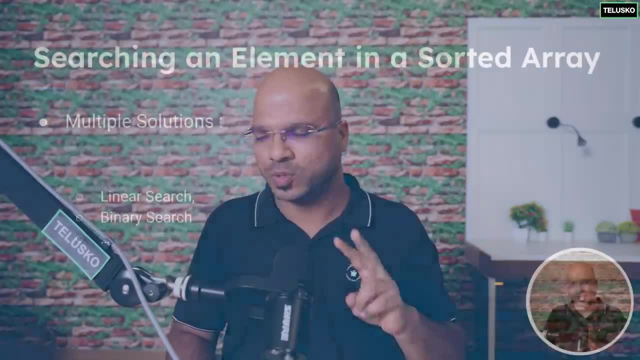 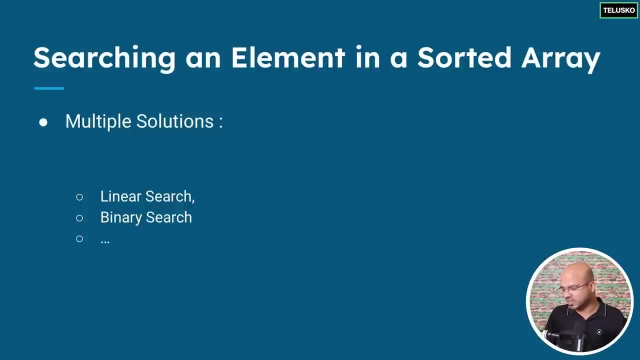 this array. Now there are multiple ways of doing it. Let's talk about the two. So, basically, we have an option of linear search, binary search or many more, but let's focus on this too. So what exactly linear search and binary search is? 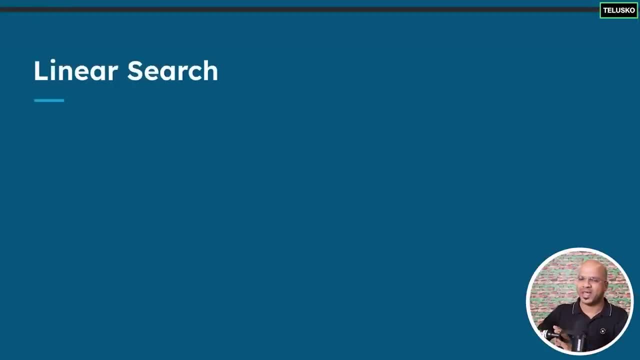 Let's talk about that. So what is linear search? So let's say you have an array with you, Okay, so this is your array And in this you have multiple values. So let's say I'm going with a few values here. 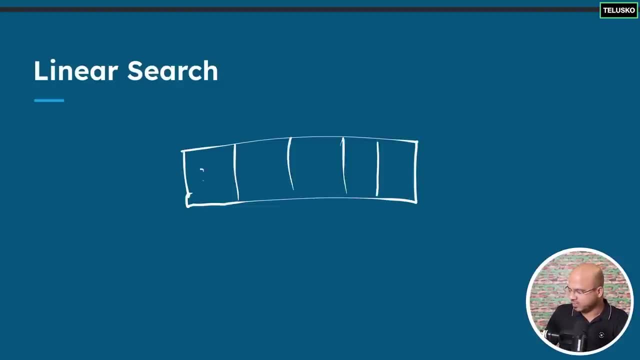 Let's say five values And then I'm going to write: let's say five, seven, nine, 12,, 17.. So we got this five values here, right? And then I want to search a particular element. Now this is sorted array because you can see all the elements. 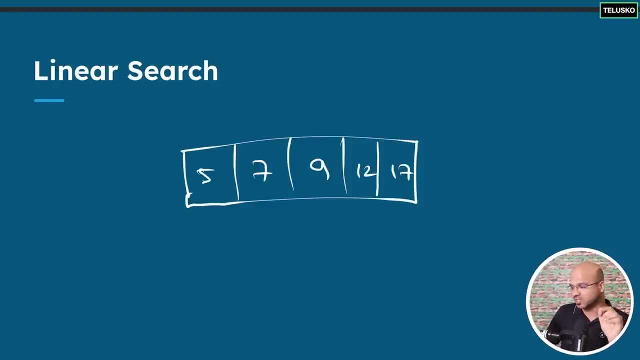 are sorted. We got five, seven, nine, 12,, 17.. And I want to search a particular element. Let's say I want to search 12.. Okay, I want to search this element, So maybe there is a target. 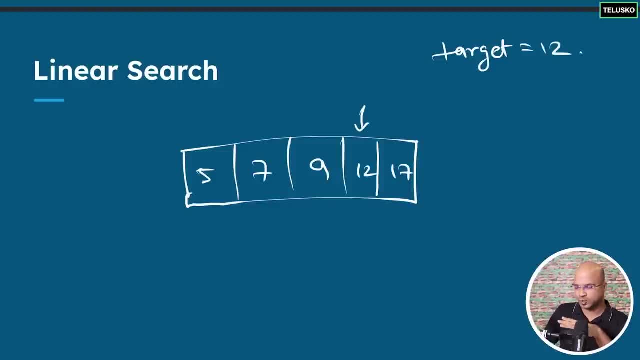 a target value which I want to search, in this case the target values 12.. So I want to search 12,, right, And then this is an array. So what we do in the linear search is you go one by one. 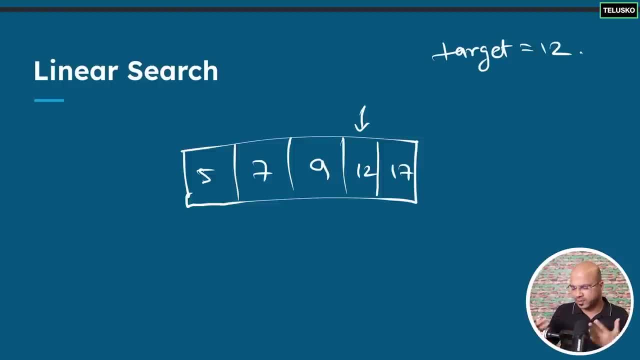 So what you do is in fact, we have talked about this in the previous video as well, So we'll make it a bit faster. So what you do is: whatever your target value is, you will compare that with the first element If it is matching grade. 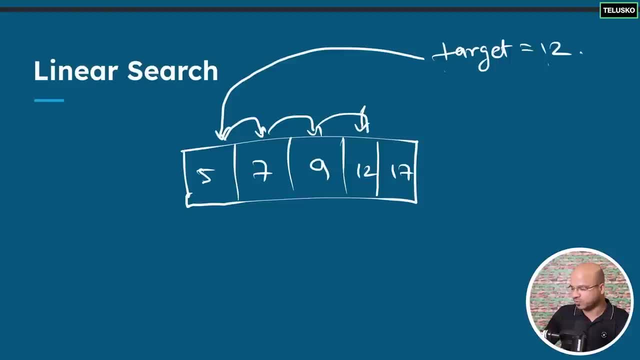 otherwise you will move to the next element, Otherwise you will move to the next element, Otherwise you will move to the next element. And I mean, of course, at this point we don't have to go to the next element. So here we basically. 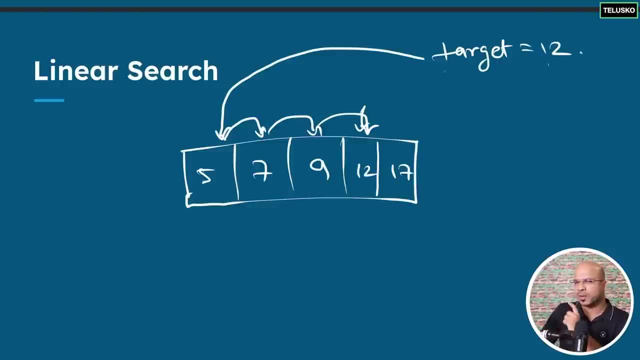 got the value, And once you've got the value, you can return the value right Now. there's a problem here. The problem is what if the element is not there in the array? So of course you have to reach till the end. 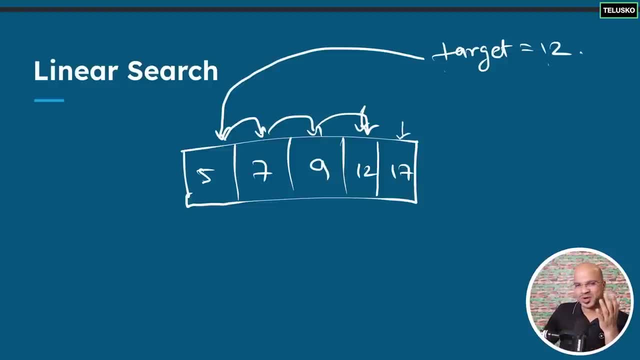 Okay, What could be the best way scenario here? So let's say you're searching for an element. Let's say element is five, And now we know element five at the start itself. So when you have the element at the start, it will take only one step. 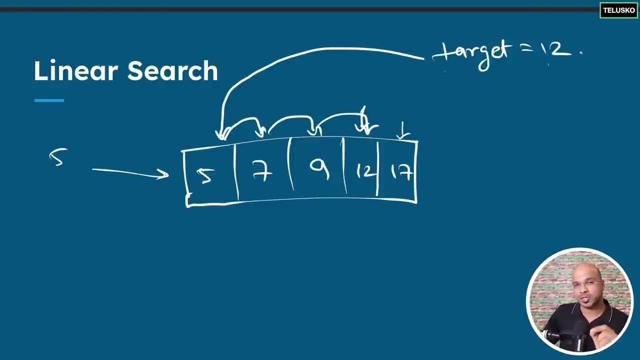 but what if you have element at the end? So it will take. the steps depend upon the length of the array. So let's say, if you have five values, it will take five steps. When you have 10 values, it will take 10 steps. when you have 1 million values. 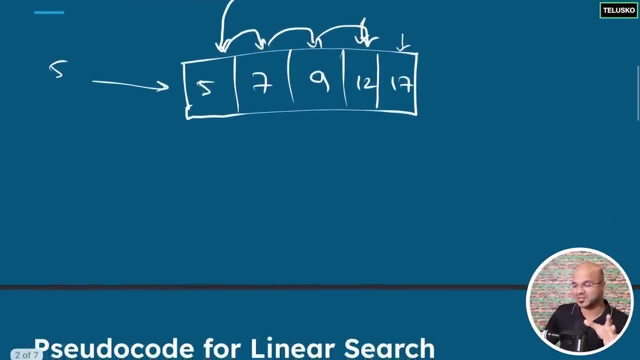 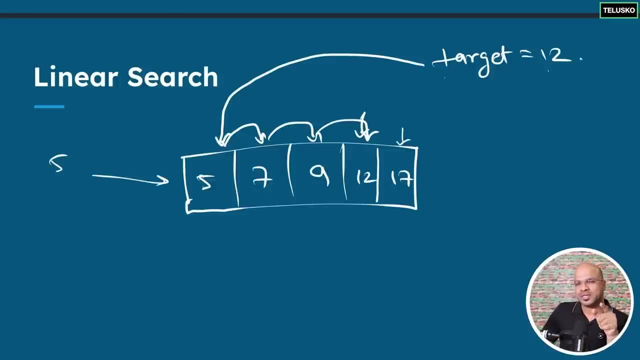 Okay, That's huge. Let's talk about thousands. So let's say: when you have 1000 values, it will take 1000 steps. That's tricky right now. The problem is not, it is taking 1000 step. 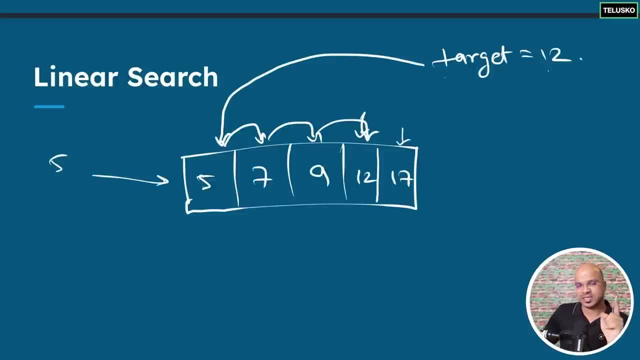 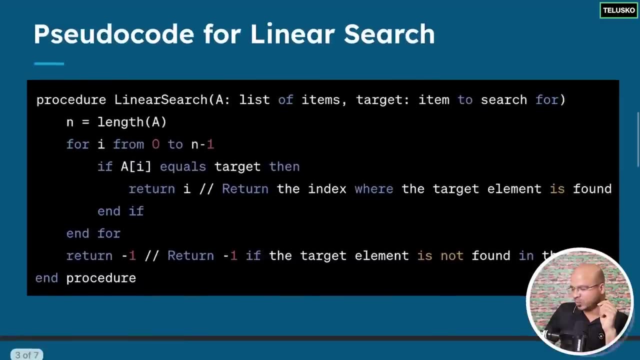 The problem is, as your size increases, it is also increasing the number of steps to search. Okay, That's one parameter you have to remember. So that's a theory. right Now, let's understand that with the help of a pseudo code here. 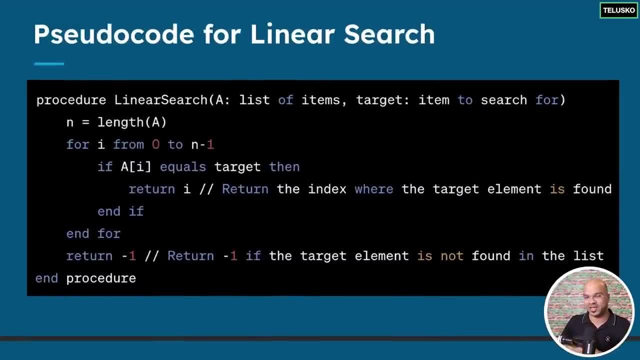 So you can see I'm writing a sort of code. Why sort of code? Why not some programming language syntax here is because we wanted to make a generic so that you can. does it matter in which language you work? Maybe C? 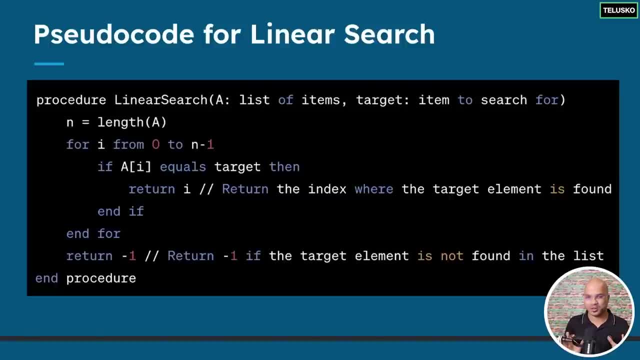 C plus plus Java, JavaScript, Python, maybe Cobol, your choice- that this could sort of call vitamins. It means saying, right now, this can be function, procedure, Does it matter? So what I'm doing is doing doing here is we have a procedure. 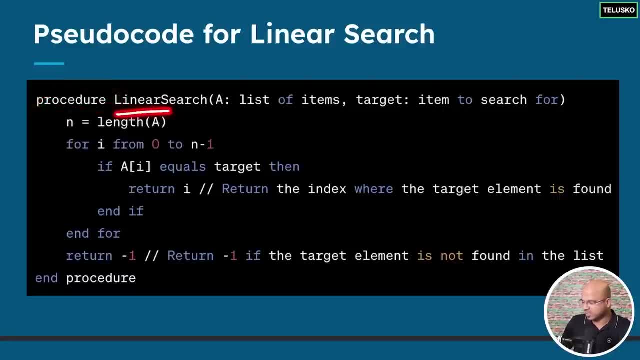 right, It can be a function, And the name of the function here is the linear search. Okay, Now we are accepting a list of items. Now, this is your array. The name of the array is a- okay, And then you are also passing a target, what you're searching? 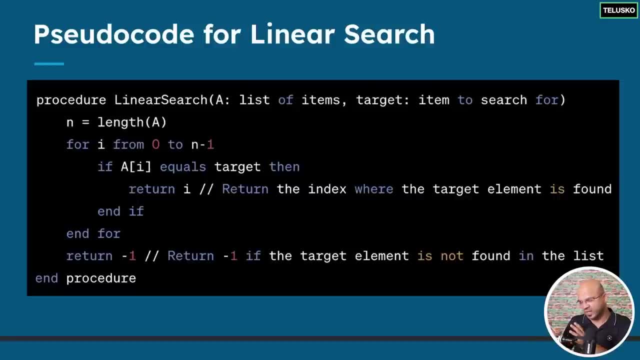 So in this case we were searching for 12, but doesn't matter. So you have an array with multiple values. It can be one value, 10, 10 values, thousand values, doesn't matter. And then you're also passing a target, what you want to search. 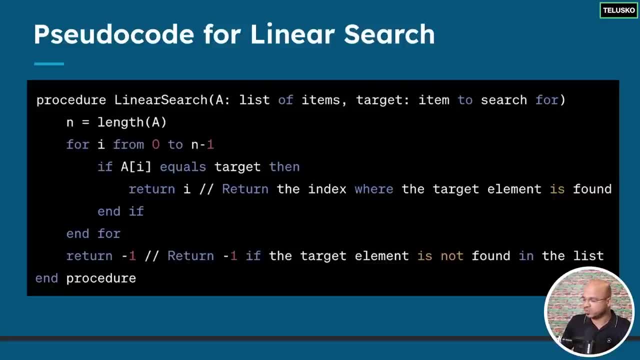 Now you will go inside this and then for the first thing you will do is you will want to find the length of the array, because of course you should know right Till when you have to search. So you've got a length which is stored in the end. 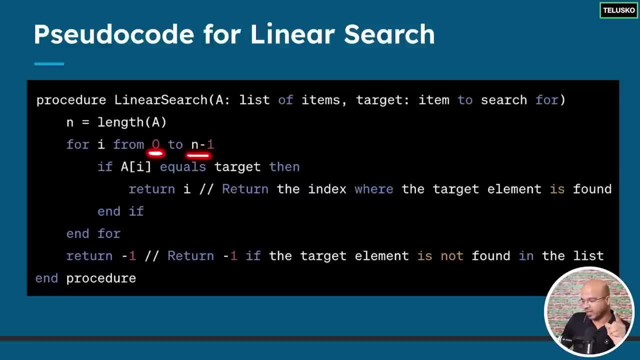 And then we are going to basically going from zero to N minus one, because we, when you start with zero, you have to end with one less right. So if you have 10 values, you will go till zero to nine. So you will go from the first value to the last value and then you will search. 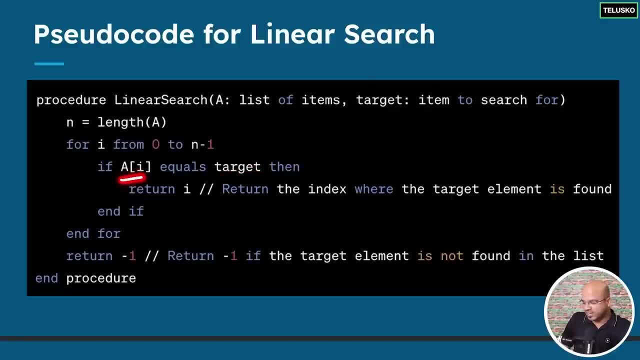 if the target with your searching is equal to the current element where you're searching. So when you're searching for the first element, that's the first element. here, Target is matching. If yes, you're good, You can simply return the value. 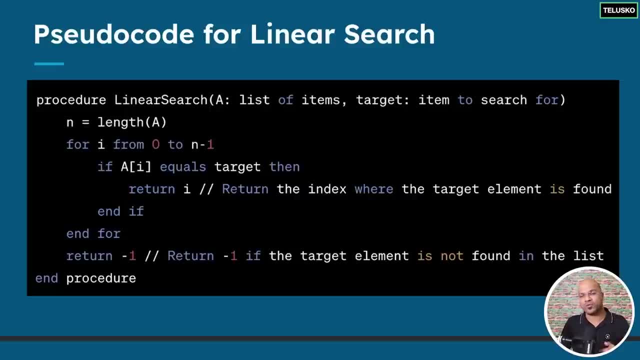 But what if you're not mad? It's not matching, It will go for the next iteration. Next value: is it matching? Yes, Good return. What if it's not matching next value? So basically you have to search each value till you're not finding it. 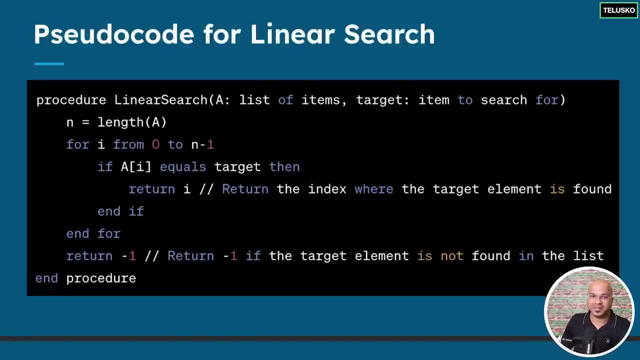 So that's basically a pseudo code here. And what if there's no element? example: you haven't. you have five values and you're searching for the value, which is not there. You can return minus one by specifying: Hey, the value is not there. 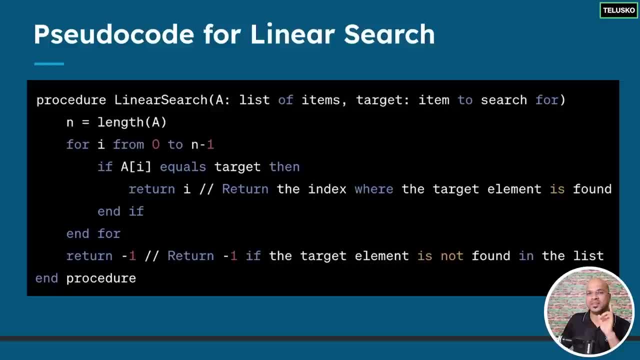 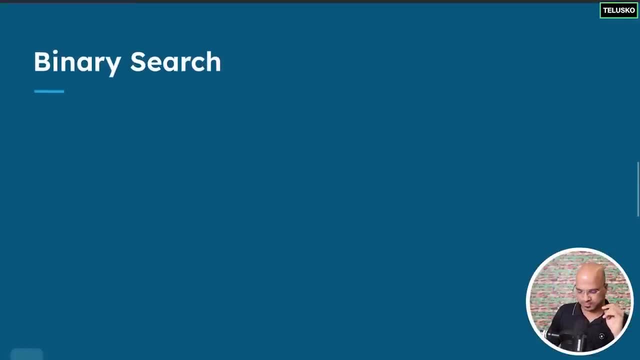 This is simple, linear search. The code is small, but then the time complexity, which is the number amount of of time it takes, is huge. Okay, Now let's go for the second approach, which is your binary search. Now, what happens in binary searches? 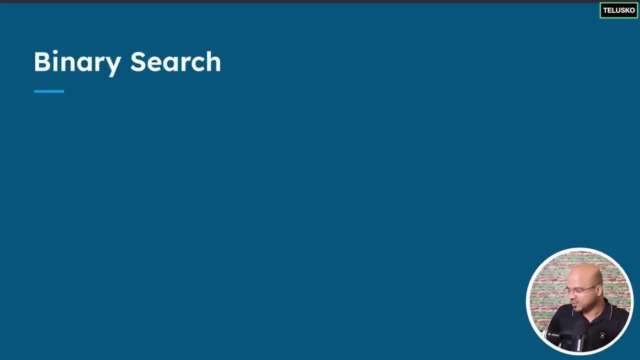 It's very simple. Basically it's not that simple, but let's say so. what you do is you have an array, again a sorted array, and let's say we have multiple values here. I'm not sure how many lines I'm going to draw. 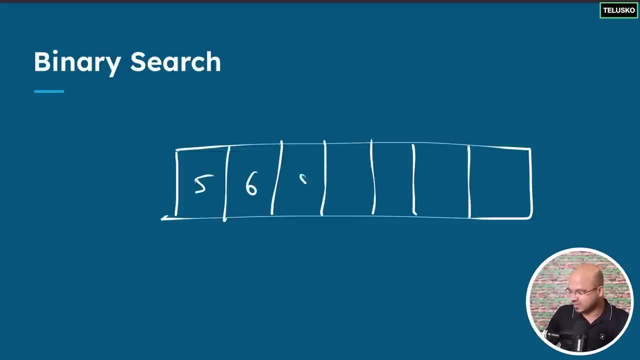 So let's count it later. So let's say we got five year, again six, eight, nine, 11,, 13,, 17.. Okay, So maybe I love odd numbers, So it doesn't matter What values you have there. 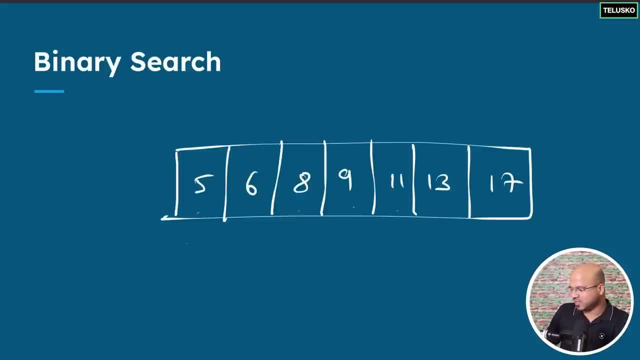 So we got a one, two, three, four, five, six, seven. So we got seven values right Now. what you do is in binary search Now, since this is sorted if you're searching for a particular element. 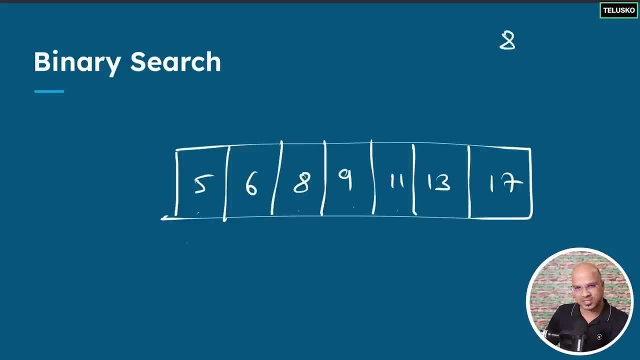 let's say I'm searching for eight here. Okay, And we know eight is here, We know it, but company has no idea. but it is. So how are we, how are we just going to search now in linear search? What we were doing is we were jumping, basically, from value to value searching. 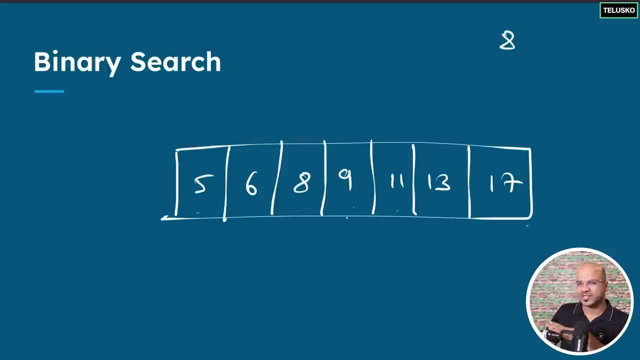 checking this, checking this, and then it goes on. So now, why? why just call it one? is because you, why do you add into two parts? That's the binary is now how you do it. So basically, what you do is you give a starting point and then you give a ending point. 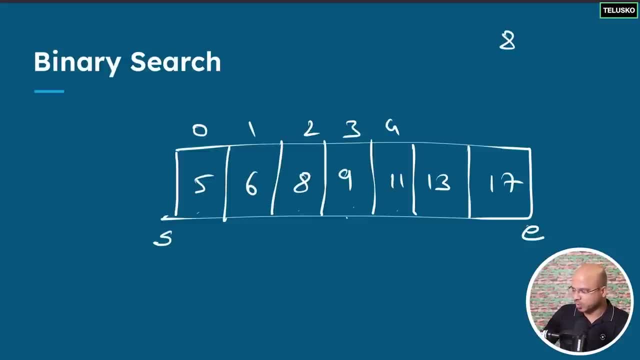 And of course, every element here will have an index value. So in total here we got a seven values right, Which goes from zero to six. Now what you do is you first divide your adding into two parts, And to do that, 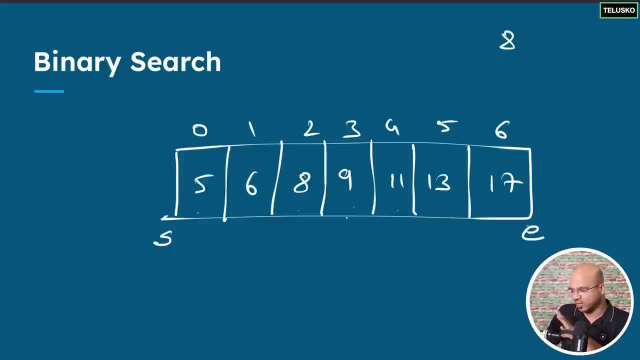 we have to find a mid value. Okay, So even before you divide you, you find a mid value. So how do you find the mid value? So mid value is equal to the starting position plus ending position divided by two. Okay, 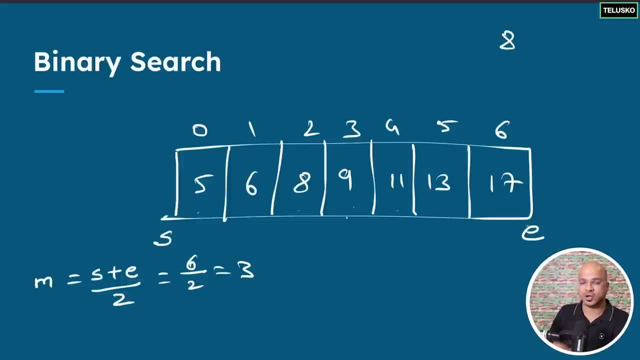 Now, this is six divided by two, which is three. Okay, So your, your mid now is three and this is your middle, Okay, Now, basically, you check with the middle, Okay, So you always check with the middle is the value. 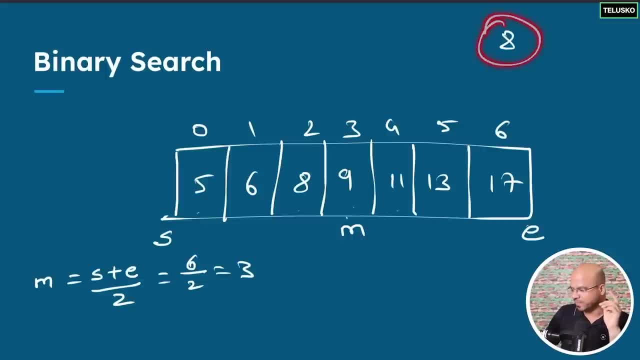 which you are searching for, which is here. Is it matching with the mid value, which is nine? No, it's not matching, but is it less than or greater than? if the value which you're searching for is less than the value, 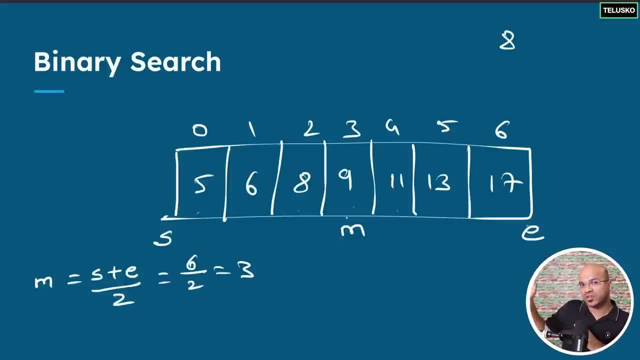 which you've got as a mid value. then the values after the mid value is of no importance, right? So this value is here, has no importance. You can directly skip them. So you can divide your add into two parts. So you've got the first section here. 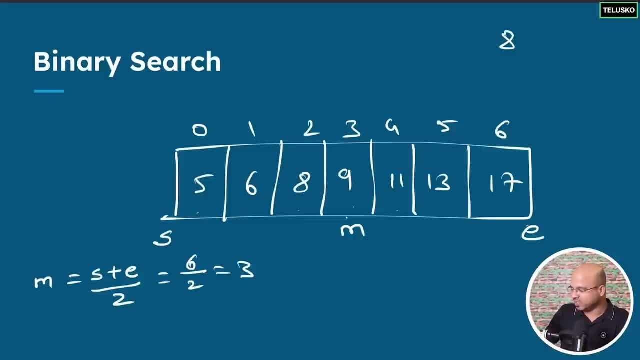 which is five, six, eight, nine, And then you've got the second section here, which is 11,, 13,, 17.. So what you can do is you can basically skip this part, or maybe I will just do that with a color. 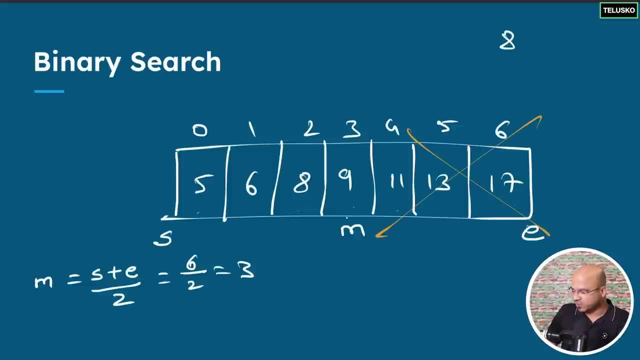 Now we can skip this part. We don't need this value. The value which you want to focus on is five, six, eight, nine. So what you do now is you make your mid as the end. Okay, Because we have shifted to the left part of the adding. 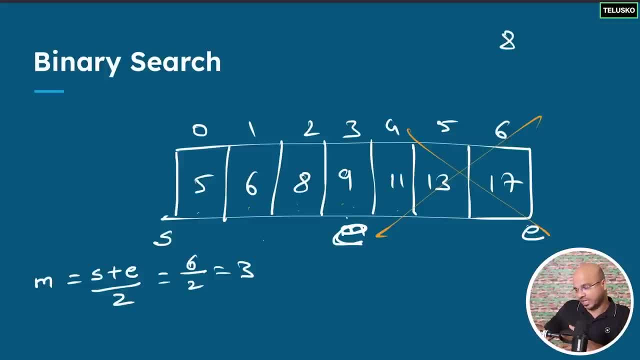 Now, when you after, of course, when you shift to the right part- you thought part of the other in case- then you shift your starting value. Now, here you've got S and E again, And then what you do is you again. 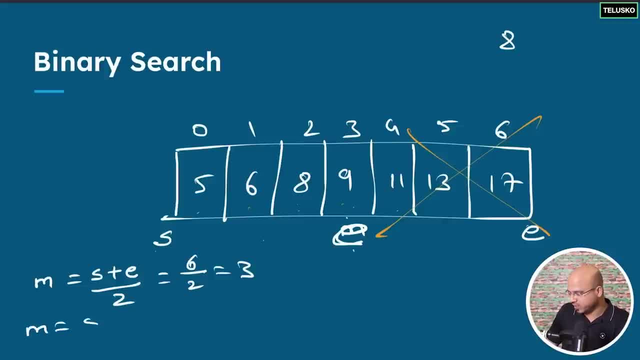 check your ending, You will find your new, new mid value. So again, S plus E divided by two, Now S is a zero. zero plus three is three by two, which is one. Uh, of course you can say 1.5,. 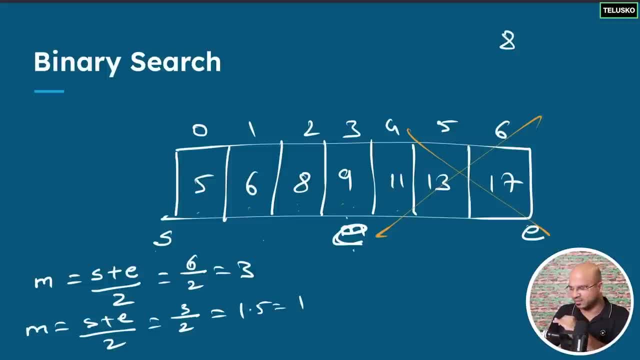 but let's say this is one equal to one. We can apply a float function to get the nearest integer. Okay, So we've got one here, right? So what you do is you check. So this is your mid again, you check. 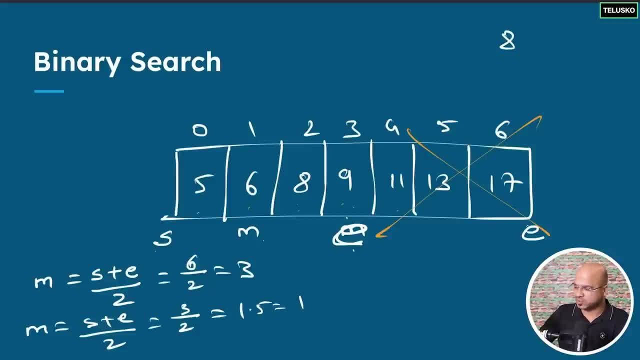 is it matching with the value? No, it's not matching. So eight is not matching with six. Then what you do? then? you again divide your array into two parts. but then which? which one you have to skip now? Now, 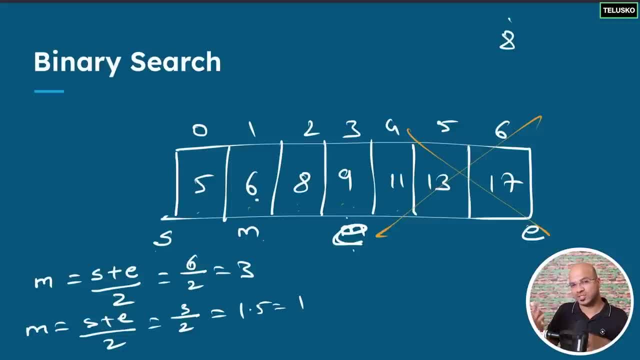 now we know that the mid is six, So we have to jump to the next value. I mean we have to look at the right side value. So six is less than eight, Right? So I have to look at the right side. 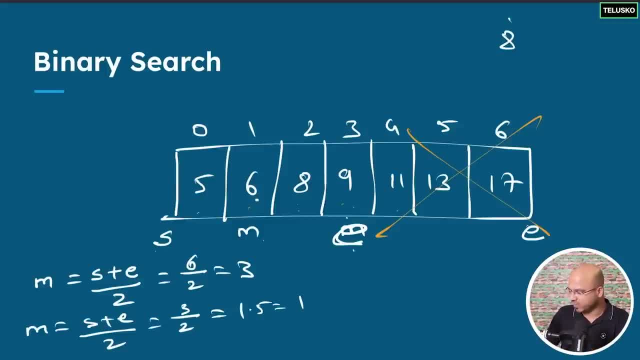 So now what we're going to do is: let's we have divided into two parts, right, So now we can skip this part and focus on the right side now. So your starting position has been moved here Now. now this is your S and you've got E. 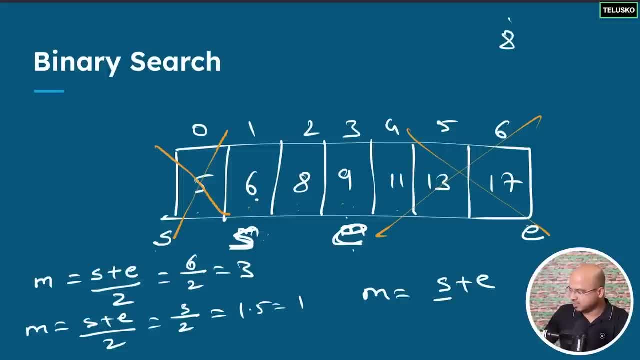 So again you will find a new mid which is S plus E divided by two, which is a one plus three, is four. four divided by two is equal to two. So your mid now is eight. Now is it matching? Yes, 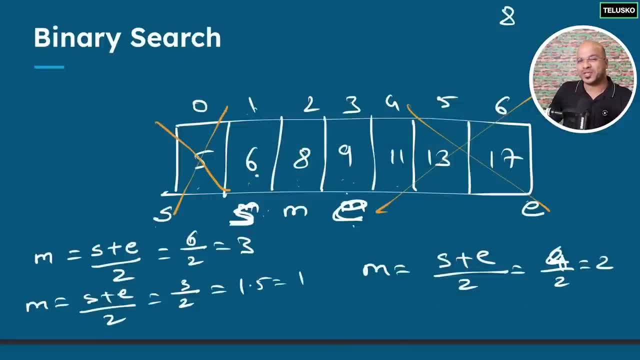 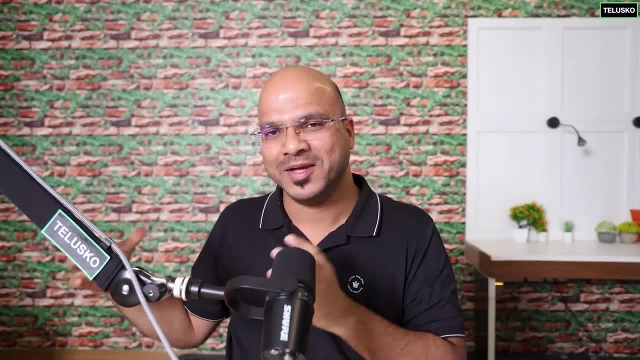 Okay, And that's how you got the value. Now, if you might be thinking, we have done so many steps right, Not exactly Basically, at the start itself, we have removed half of the array and which is very important, right. 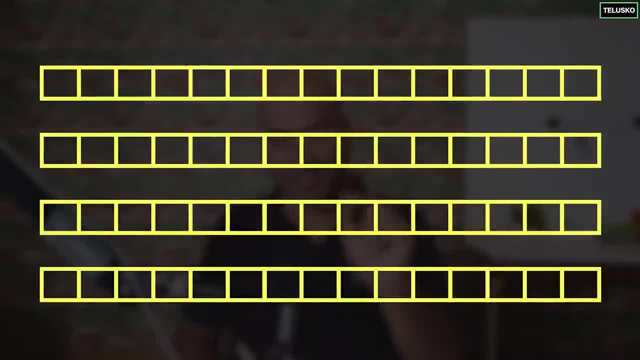 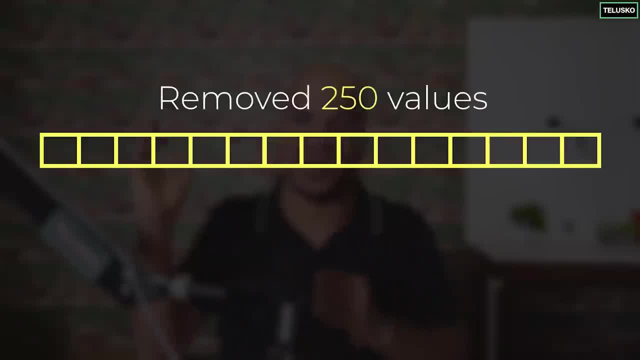 So let's say, if you have a size of 1000 at the start of the first operation, you have removed 500 values for the next operation, When you do it, you remove two, 50 values. So the number of operations which are doing with one is: 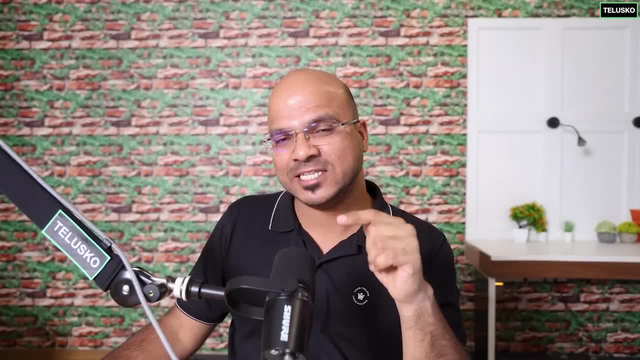 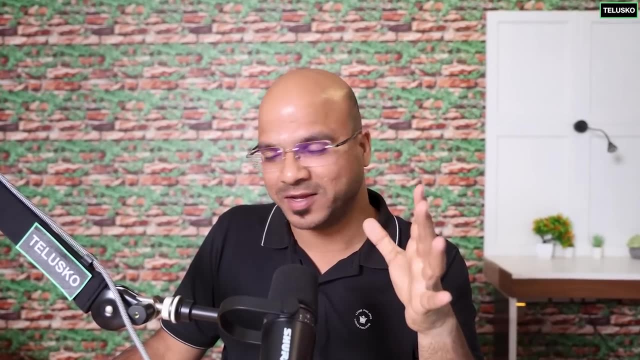 search is less right, And that's how you know that this is better than the linear search. Of course, in linear search, if the value which you're searching for is the first value, it's very fast right. It will take a lot of time for binary search. 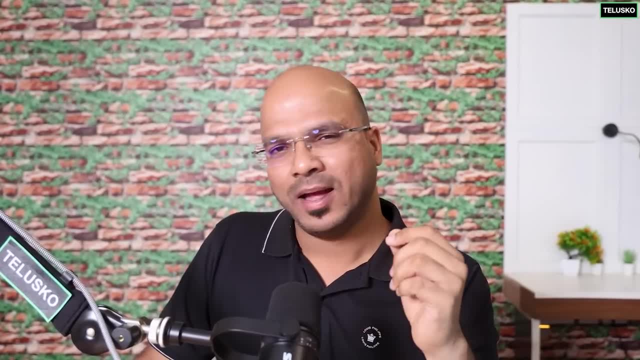 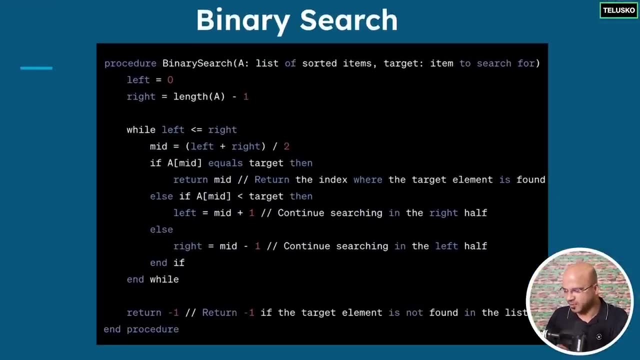 but in general, binary search works faster. But how do you do that? So with this theory, let's talk about the practical implementation here. So let's look at the code here very fast, because we have already done the theory here. So what you do is you basically write a function. 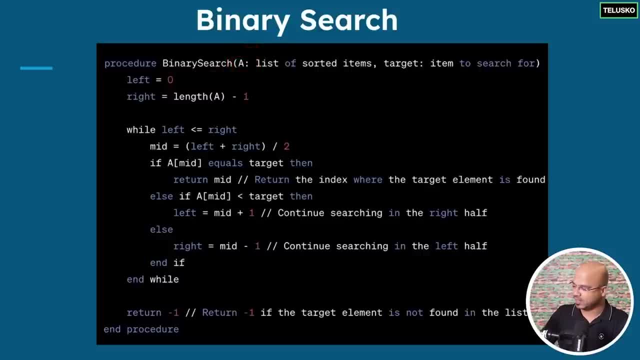 let's say binary search- and then you pass a list of values right, And then you also pass a target- Same thing we have done in the linear search- and here then you go with the left and right. So basically we have mentioned the start and the end here in. 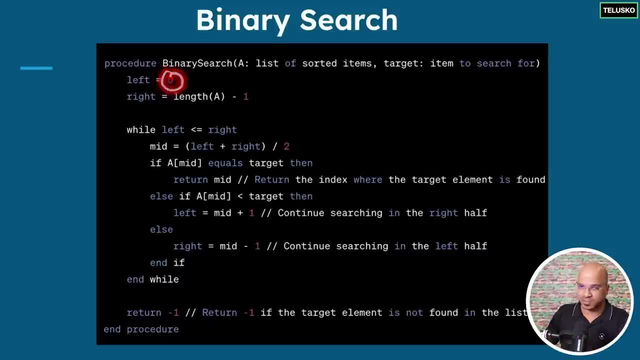 this we are taking left and right. Let's start with zero. As we mentioned, the starting start with zero, ending ends at the last value. Okay, We have done that, And then you run a loop till you find the value, Of course, 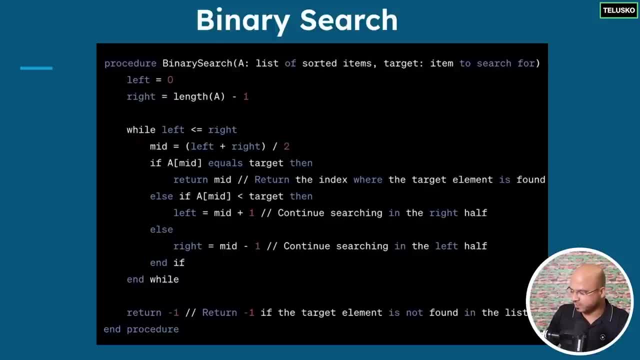 then what you do is you check the mid value. So this is a mid value. We have done that. mid is the starting point, ending point divided by two, And then you check: is the middle matching with the target? If yes, you're done. 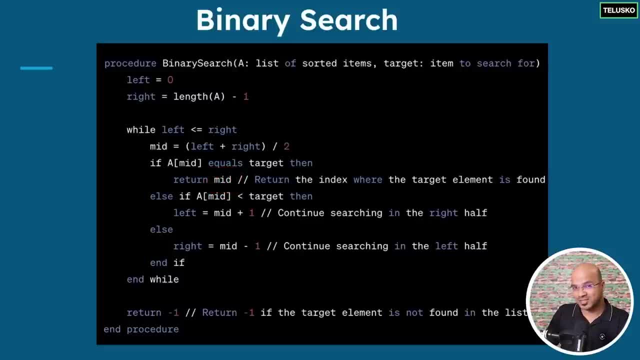 You can simply return the value. Otherwise we have to do something more. Then you would check if the value which you got, which are mid value and the target, if the mid value is less than the target, in this case, you will focus on the right hand side. 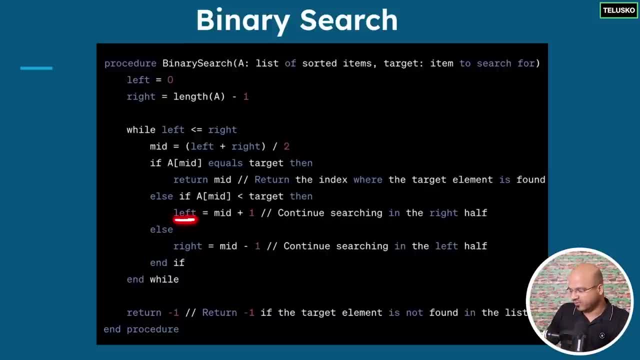 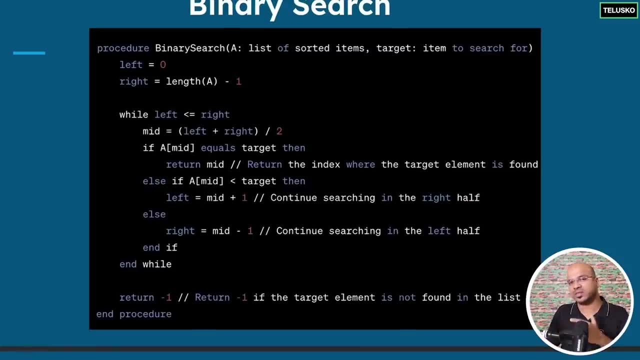 Okay, So basically you have to shift to the right hand side. So your left, your starting point will shift, And we have discussed that here- right, Your starting point will shift. And then what if the mid value is greater than the target value? 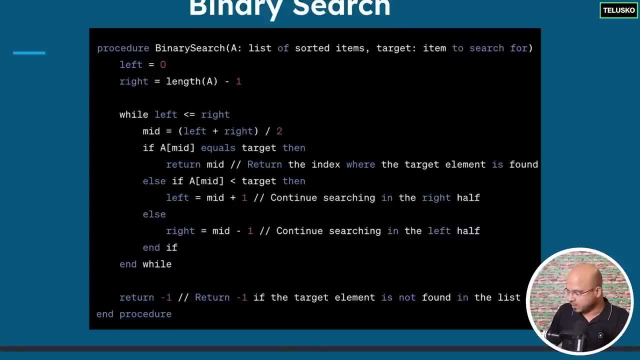 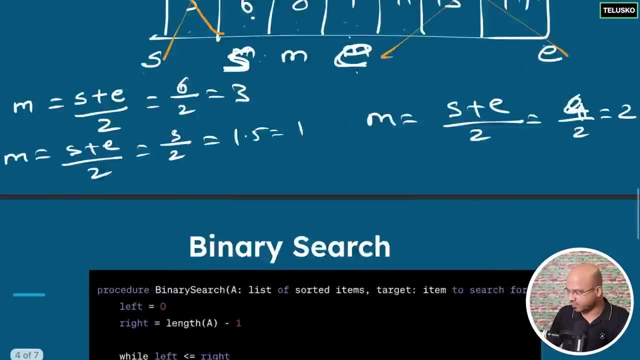 In that case, it will shift to the left position. Okay, So that's what we have doing here. And then, every time you do that, you run the loop again. you find a new mid value, and that's what we have done multiple times. 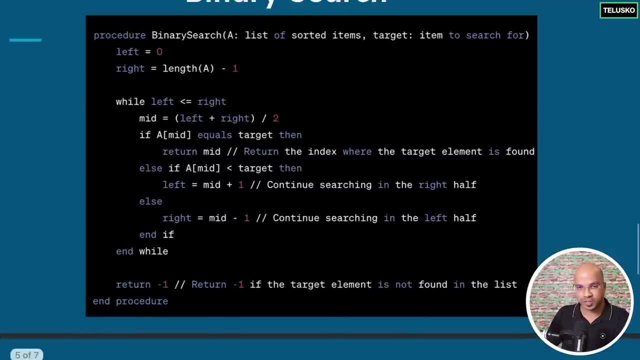 right. We found the mid value three times in the same way you're doing. you're going to do here And then at the end you will get a value. If it is not get, if it is not there, you will simply return minus one, as we have done before. 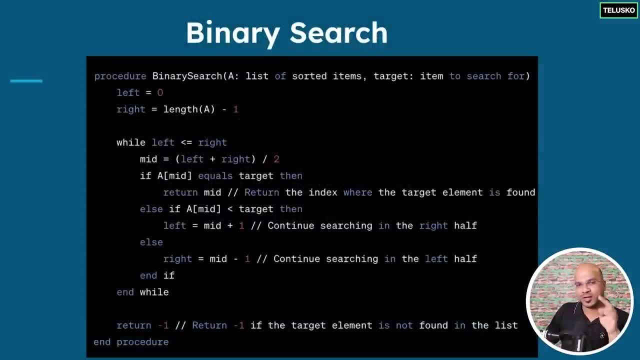 So, basically, by doing this, what we're doing is we have seen two algorithms. right Now we have to find the time complexity. Now, what exactly time complexity is? It's not about number of seconds it takes to run your code. It's all about this. 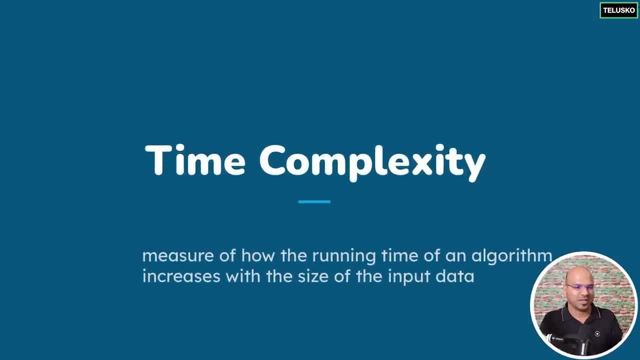 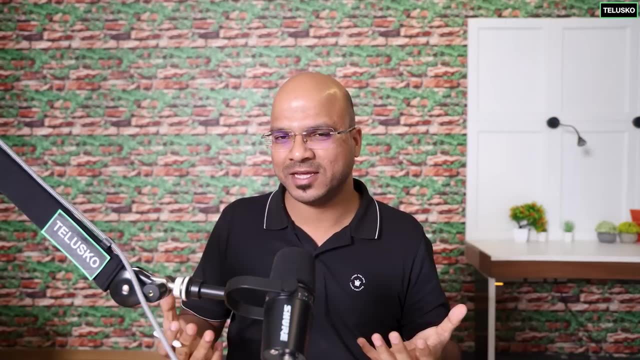 So time complexity simply means the measure of how the running time of an algorithm increases with the size of input data. So basically, let's say when you are testing a particular algorithm you're testing for, let's say, 10 values or 20 values. 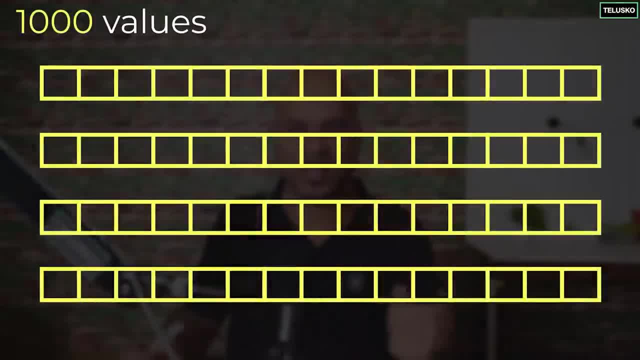 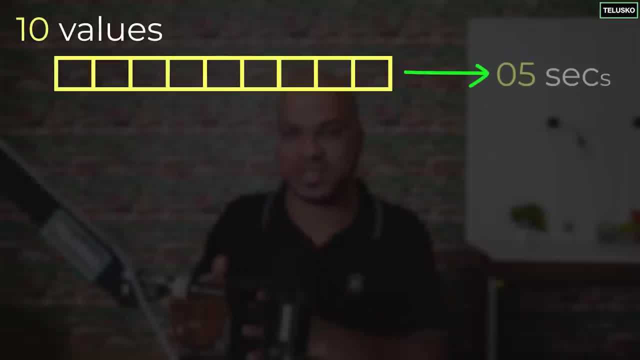 But what if the values goes up? What if you have thousand values? how will it will affect your time? Will it increase the time in linear section? Let's say, if it takes five seconds for 10 values, will it take 10 seconds for 20 values or will it take more? or 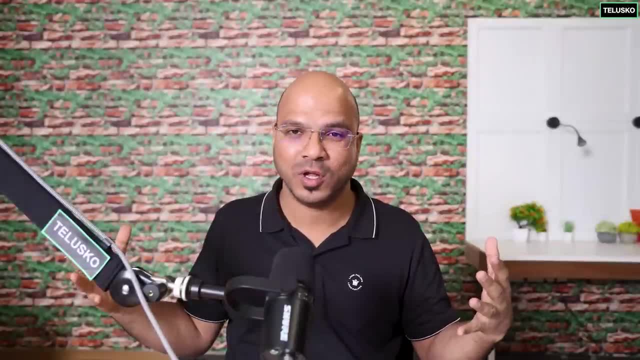 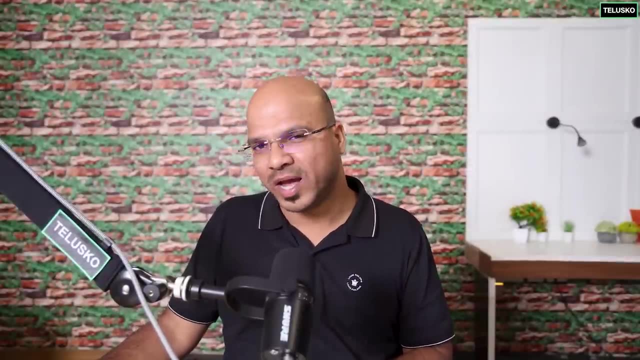 will it take less? Okay? Or let's say, you have 1 million records, Will it take 1 million seconds? That's the question we have to answer. Okay, Now how will you do that? And that's where we have something called big O notation. 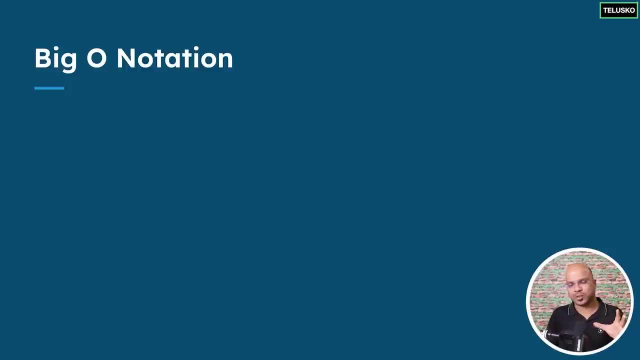 Now, what happens in big O notation is we use this particular concept to understand your time, complexity of your algorithm. If someone says, Hey, your algorithm is not fast enough, You have to first find the big O notation of it. Uh, so why big O? is because it is represented with the help of O, the big O in 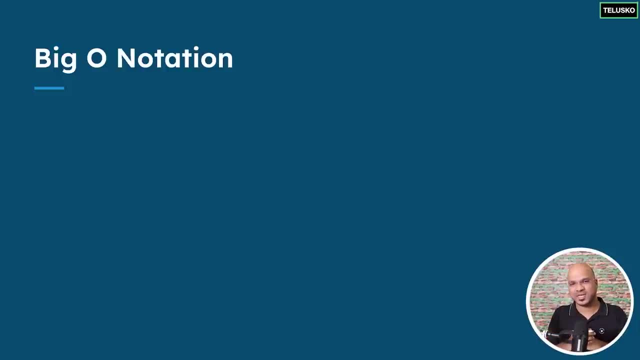 bracket. you mentioned the order of N or something. So basically it is also called order of all big O notation and you anything will do. So how do you represent that? You represent that with something like this: So we have O off and then the value. 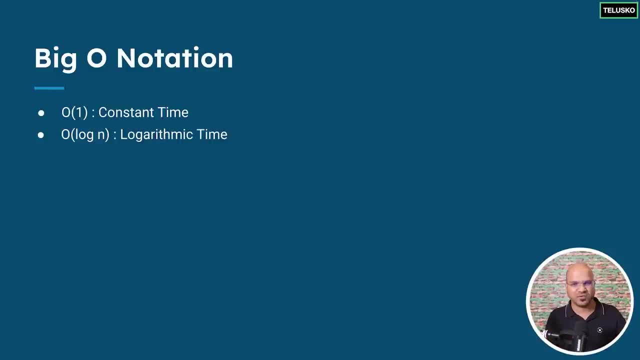 which is one will keep changing. So there are multiple things here. You can say: we have O big O of log N, we got big O of N, We got big O of N log N. We say big O of N square, which is quadratic time. 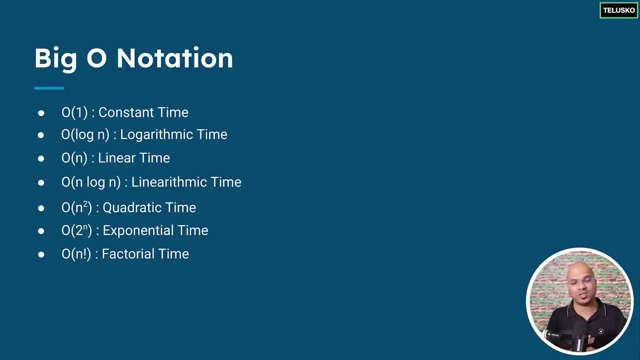 We got to this: to N, We got N- factorial, Okay, So we got all this notation, but how do you find this Okay? Now, this is tricky. So, of course, in this particular video is not, you will not understand everything. 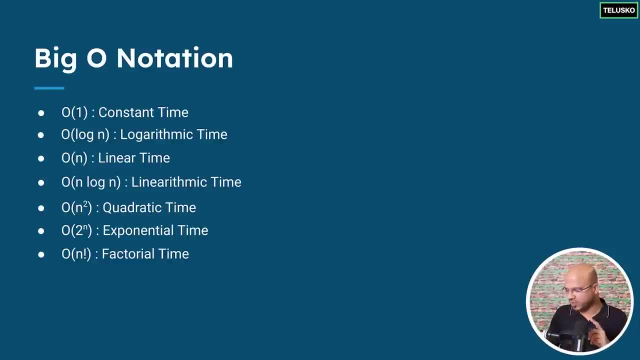 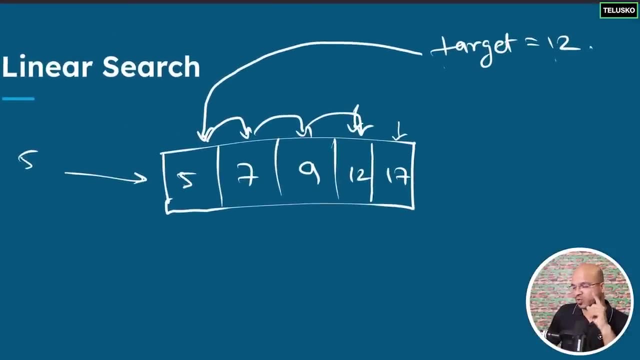 but let's start with the basic. Now let's talk about the linear search. Now, if you go back to linear search, what we were doing there now, in linear search, when you have five values, you take five, five steps. When you have 10 values, 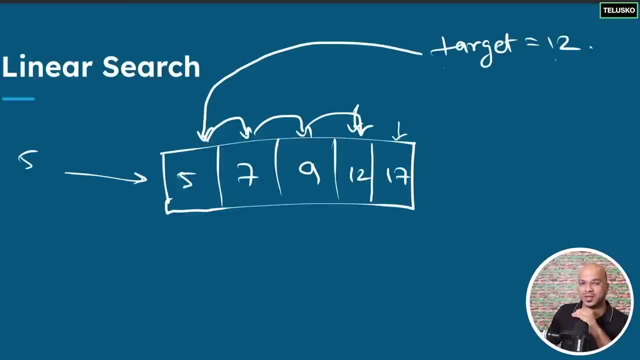 you take 10 steps. You, when you have a hundred values, you take hundred steps. right, But let's say that is for searching, right. What about reading, If you want to read a particular element from the linear search or from the? 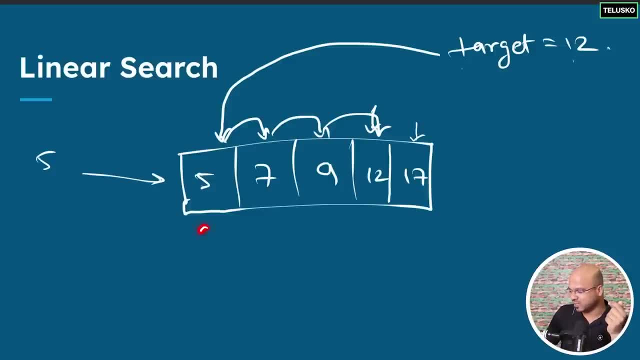 array. it's very easy, right? You specify the index value. Let's say the index value is 0,, 1,, 2,, 3,, 4.. And then you specify: Hey, I want the value at index two. 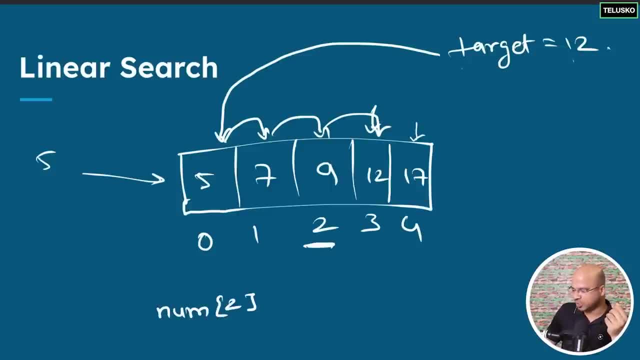 So let's say you say nums, which is the name of the array, And when you say two, basically what you get is nine. It's very fast, So it doesn't matter What is the size of your array: It can be 1 million records. 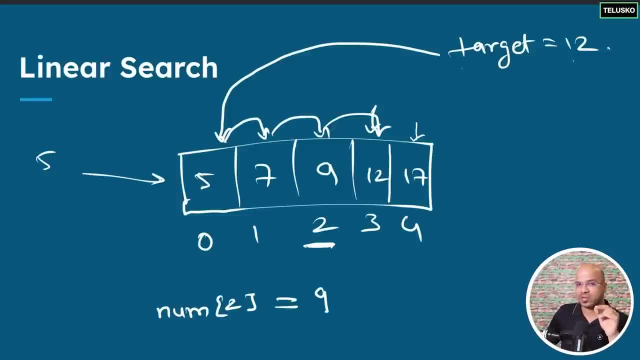 The time taken to get a particular element with the help of index value is constant. right, Because computer knows where that memory is. So in that case I can say the big Oh the time complexity for this is one, because it is constant. 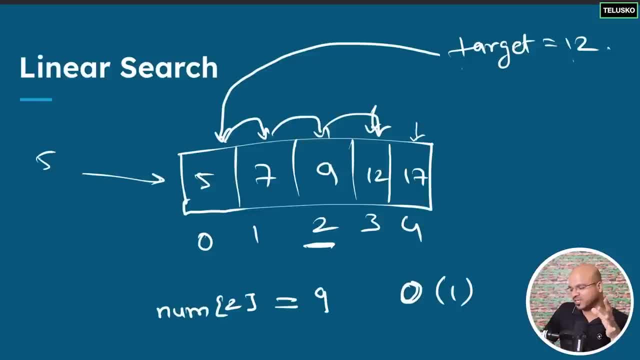 Okay, Now see, it's not about one step. If you're thinking just because I've mentioned that it is only one step, it can be three steps as well. So let's say if you are reading a particular element and maybe behind the scene, 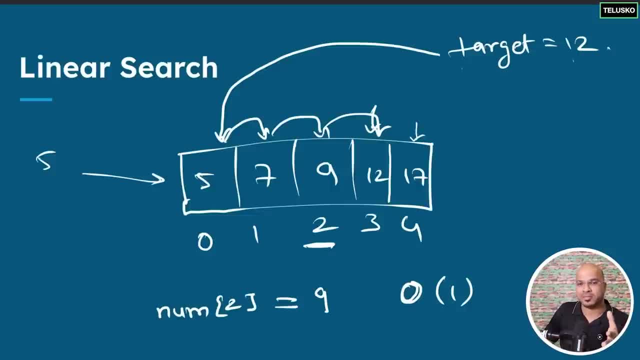 it takes three steps, It doesn't matter, It's constant. right? It can be one step, three step, 10 steps. It should be constant. If it is constant, you can say Oh of one, But what if you are searching element? 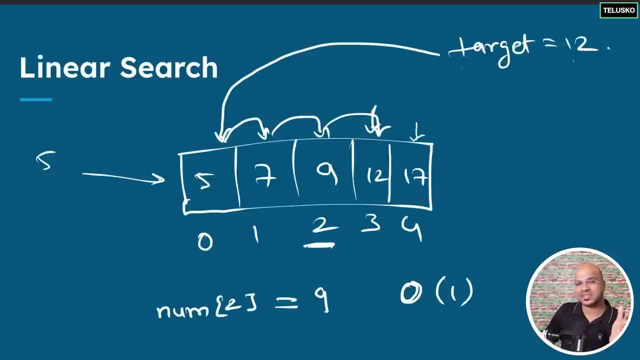 So if you have an array size of, let's say, 10, it takes 10 steps. Now you'll be saying: Hey, you know what, if your element is at the start itself, Of course it will take one step, but we have to go for the worst case scenario here. 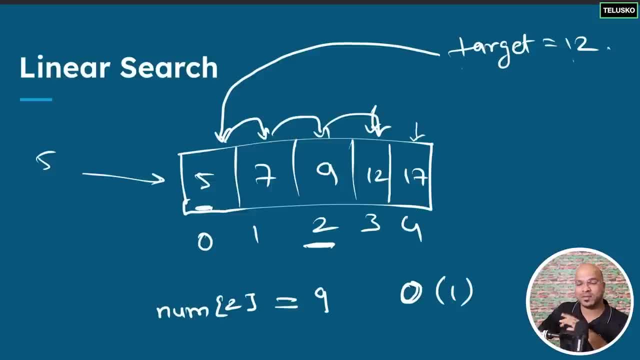 The worst case is: what if the element is at the end? What if the element is not even there? It will take 10 steps and that's why we can say the order. the big O notation here will be n. What is n here? 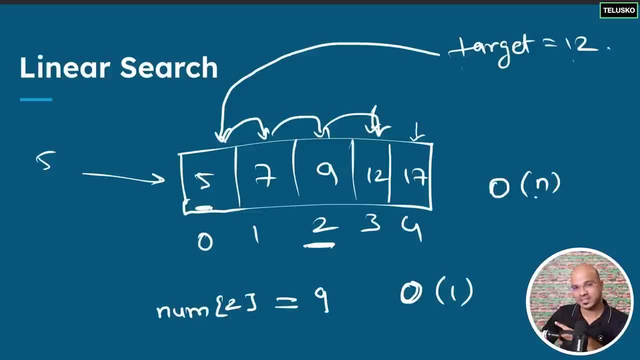 The number of elements in the array. as it increases the time also increases the time complexity. I'm not talking about the actual seconds. Okay, so that's your linear search. Now, coming back to the binary search, what could be the big O notation for binary search? 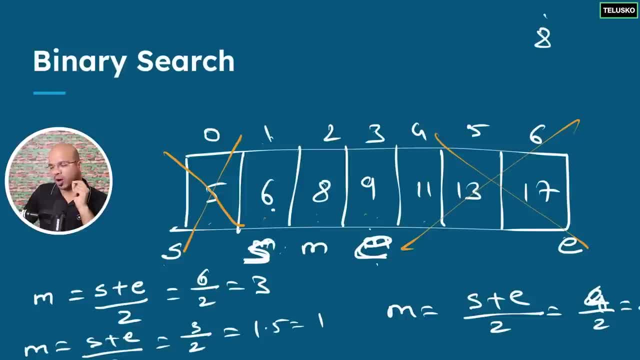 See, the thing is, as the number increases, it will not directly increase the number of steps. Reason for that is: let's say we have we have seven values. How many steps it takes? Let's say three steps, because we have to find the mid value three times. 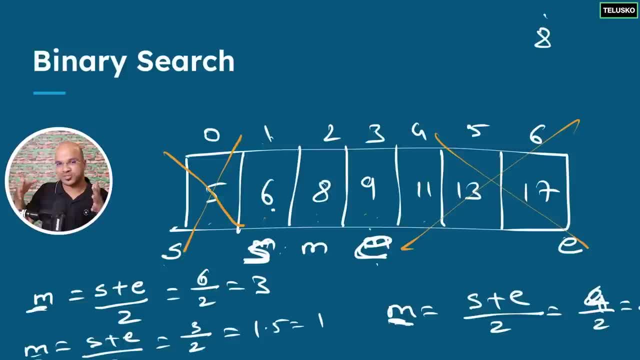 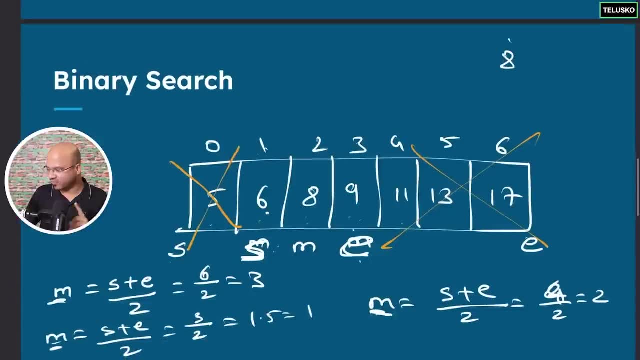 right. What if the size increases to double? So let's say, from seven we got 14.. So what do you think? How many steps will increase? What if I say, only one reason being, even if you have, let's say, 14 values here? 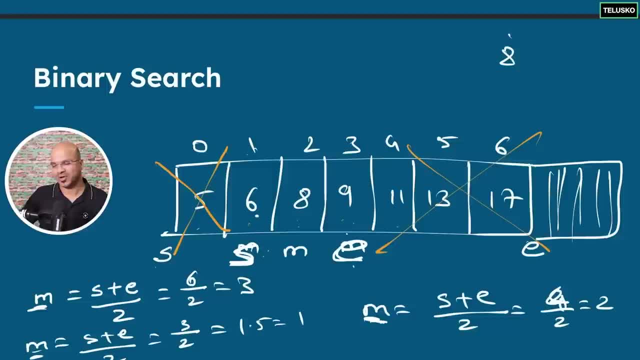 let's say we have so many values at this start itself it will be half. Okay, Right, You will get seven values after one step and then you basically include, increase one more step to find the middle. So that means when your value increases. 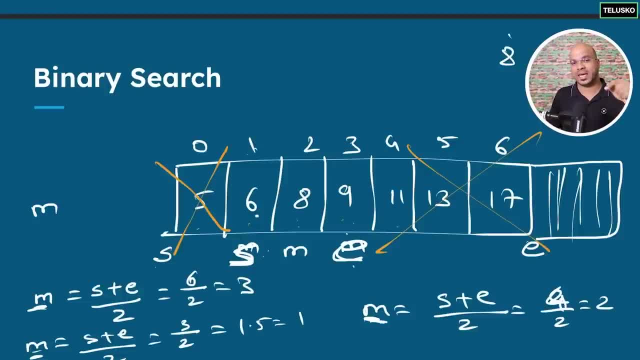 it will also increase the number of steps taken, but not exactly N, because in the linear search if your number of values increases by 10, it will increase 10 steps. here, as the number of value increases, It will not increase the steps in the same sequence. 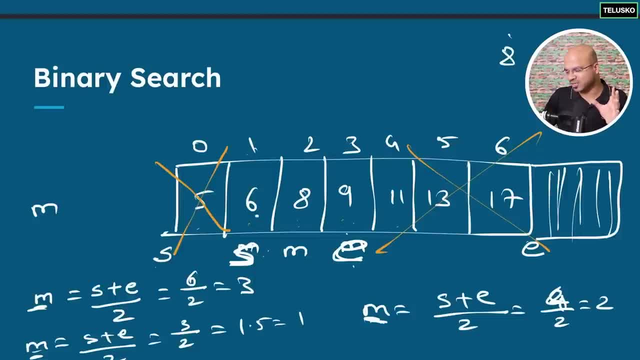 So what we can say is we can say: it is something between constant. It's not exactly constant, but it is Between the O of one and O of N, So it is between this two, And what comes between this two is O of log N. 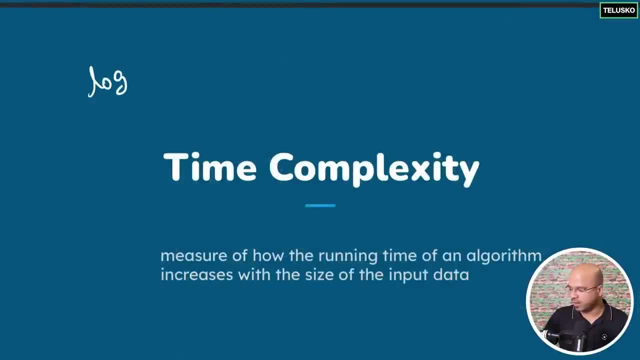 Now what is log N basically? So log N basically means we have a base two here by default, Okay, So number of steps it takes. So what exactly this N here? So let's say we have eight values here. So when you say log two of eight, 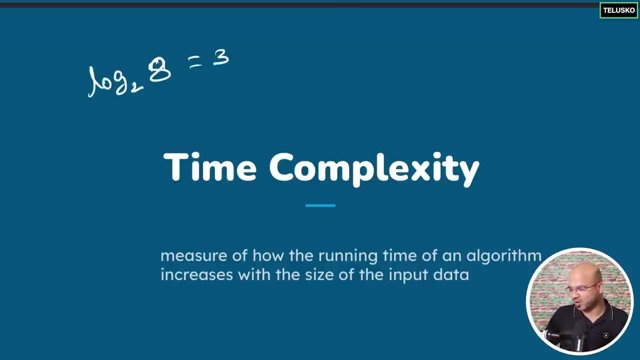 it will give the value, which is three. Okay, Now, why it is three is because a log of eight is simply means it will take to multiply itself three times to get eight. Okay, So as the number increases, let's say now, instead of eight values. 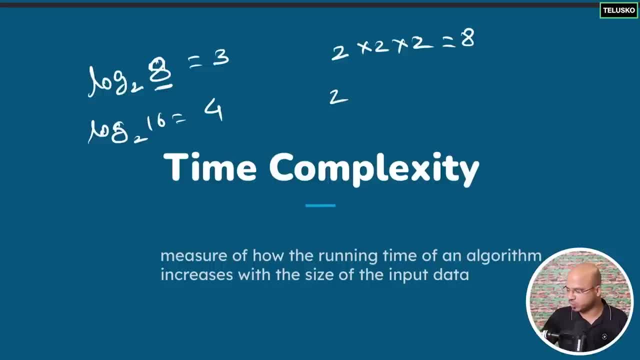 we got 16 values, It will give you four, because it will take two to multiply itself four times to get 16.. Right, So it will give you four. That means, as your number of value increases from eight to 16,, it will only increase one step. 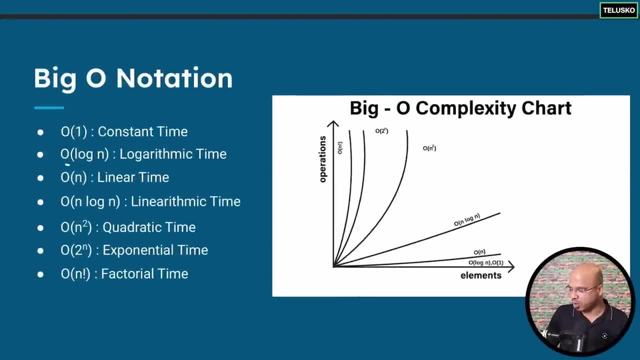 right, And that's why the binary search is log N, So your linear search is O of N and your binary search is O of log N, So, which will take less time. The log of N. Okay, And you can see the graph here as well. 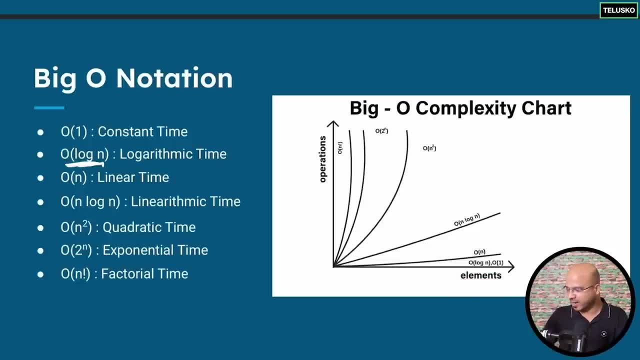 So this is elements, the number of number of elements you have in the array and this is the number of operation it takes. Okay, So number of steps. So if your algorithm is following the constant time, it means it's here. It doesn't matter how many values you increase. 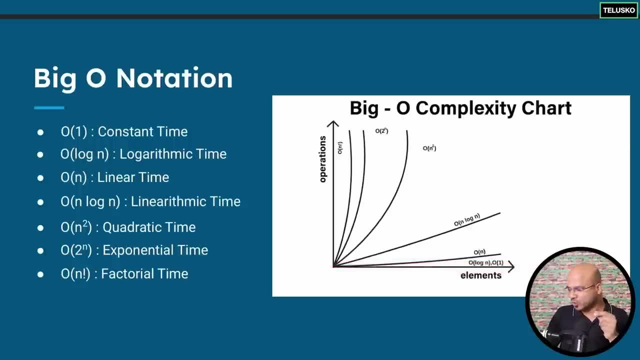 It will be constant time. log N is similar to. it's almost same as constant, not exactly same as constant, but it will take less time. So you can see log N is mentioned here. It's there, The wave is there. You can't see it. 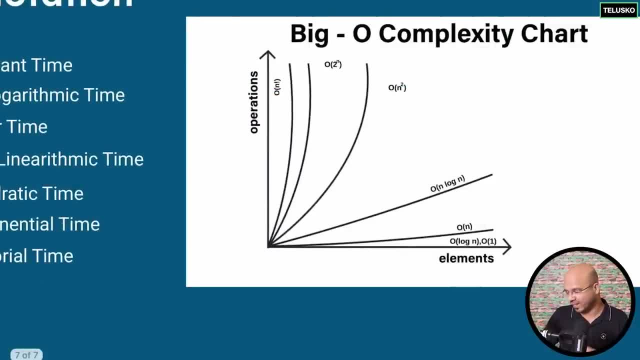 It's there, Uh. so what if you go with big O of N? So as your value increases, your time also increases, right? But there can be some worse scenarios as well. There can be some other algorithms which you implement which might take N log of N. 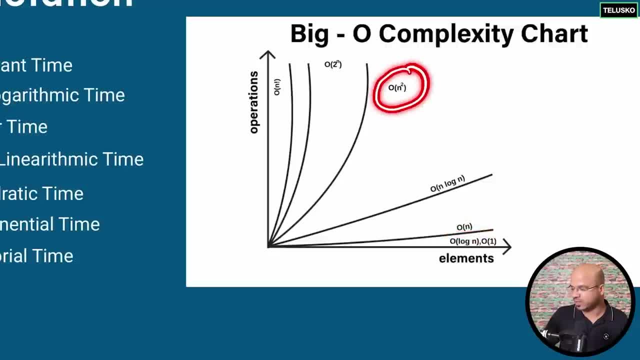 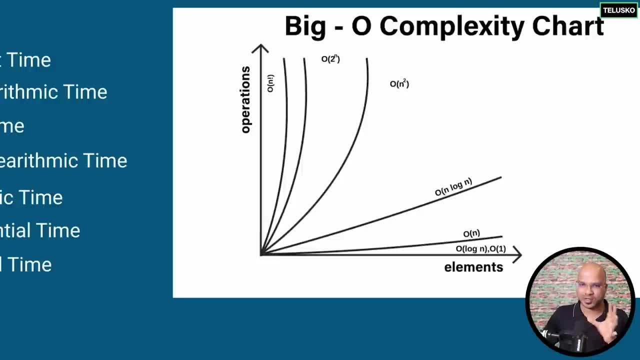 which is worse than O of N. There might be some algorithm which will take O of N squared, which is worse than the O N log N. So, basically, if you want to build an algorithm, try to make sure that you are here. 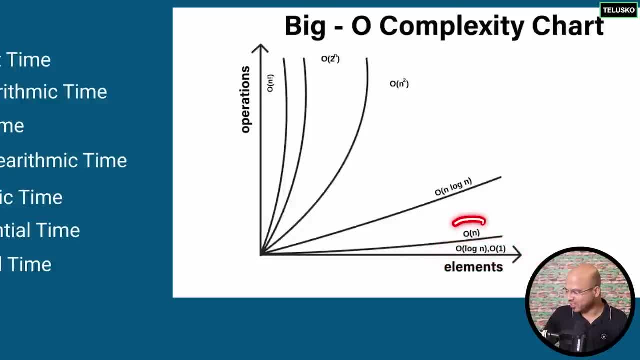 If you are here, you're good. Okay. If you are here, it's okay. If you are here, try to make it better. If you are here, that's the worst scenario. That means you're building an application which is not scalable. 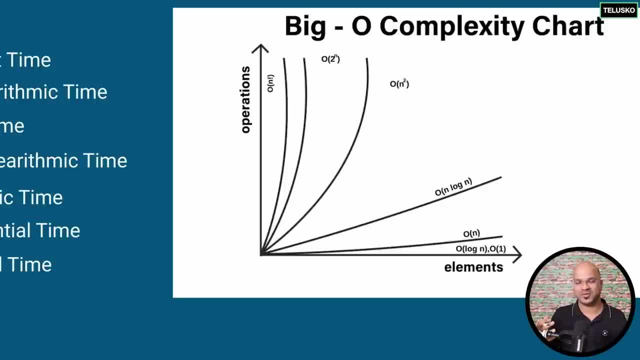 The moment you have five users on your server, your server says: I'm good. The moment you have 1000 users, it will struggle. Okay, So make sure that you, when you- whichever algorithm you write, you follow this. 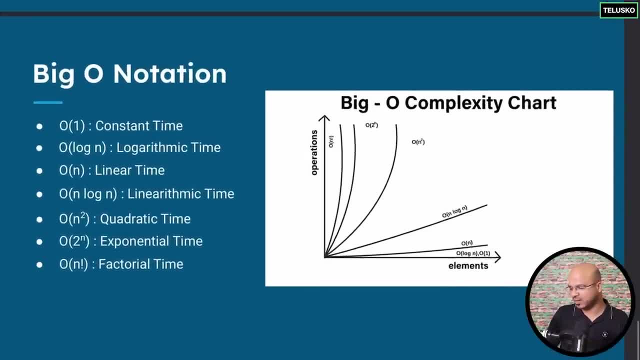 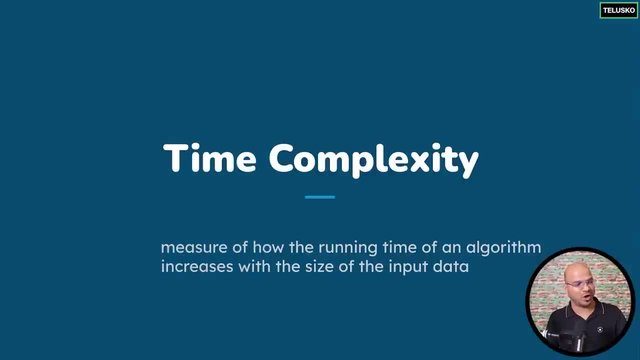 Of course, in the upcoming videos we'll work on some more algorithms. We'll see which one matches there, but you've got the idea right. So the time complexity simply means this definition: the measure of how the runtime of the algorithm increases with the size. 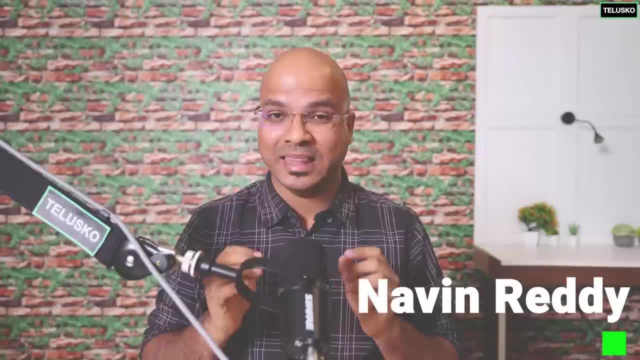 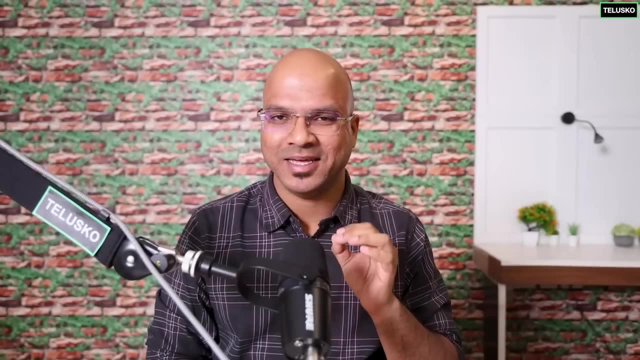 of the input data And to represent that, we use big O notation. In this video we'll talk about the practical implementation of linear search and binary search to understand the time complexity which we can represent with the help of big O notation. 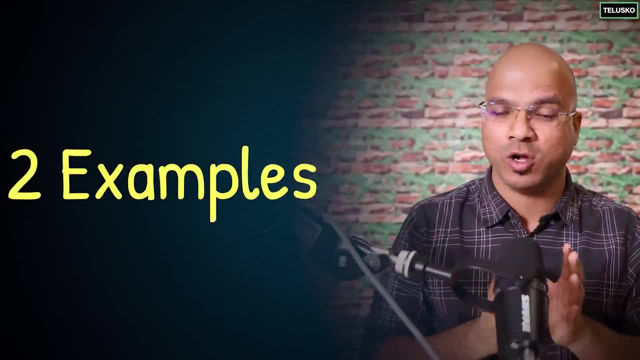 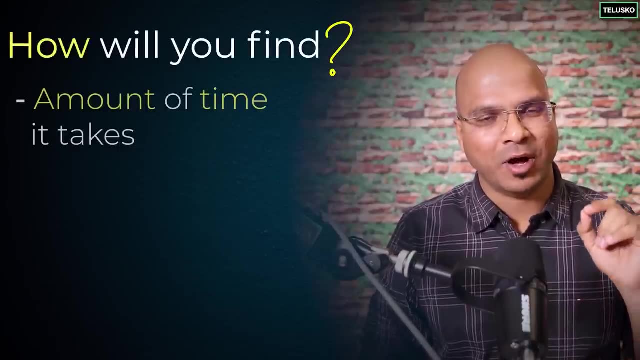 Now, basically, we'll write two examples here. In fact, we will also do binary search in two ways, just to understand how things works. And then how will you find the amount of time it takes, Not in seconds, of course, but the number of steps. 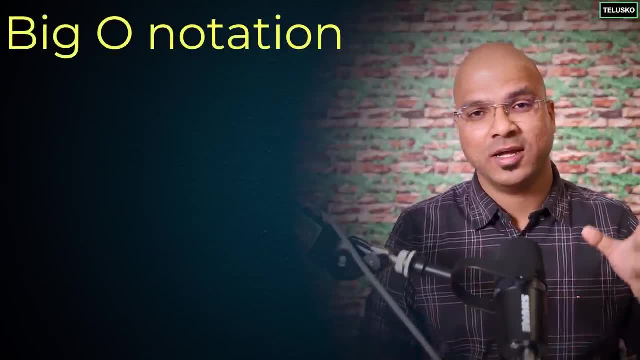 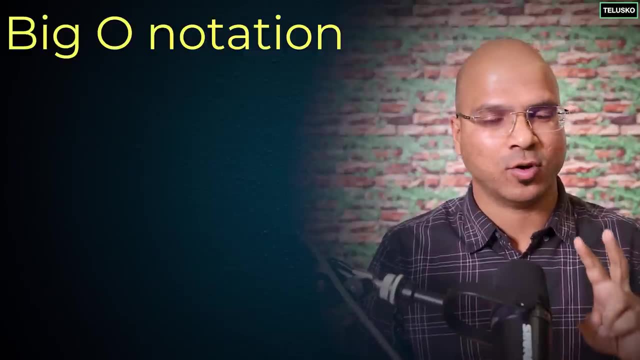 right. So we have discussed about big O notation, which is the big O of one, big O of n, big O of log n, right. But we also have multiple options, but then at this point let's focus only on two, with the help of two algorithms. 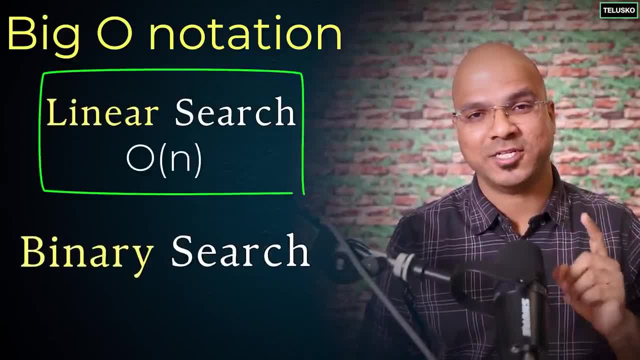 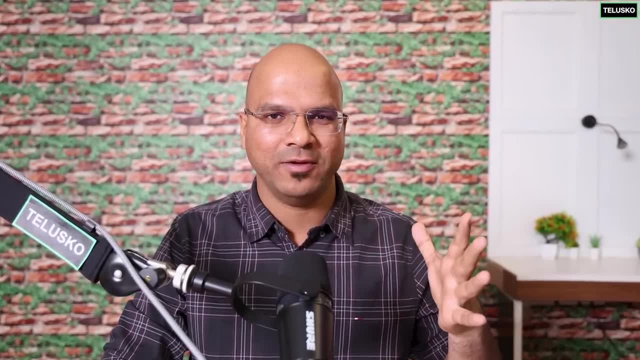 linear search, which is big O of n, and binary search, which is big O of log n. Okay, So what I will do is I will write this code in Java, And of course, we'll not be doing very complex stuff in Java. 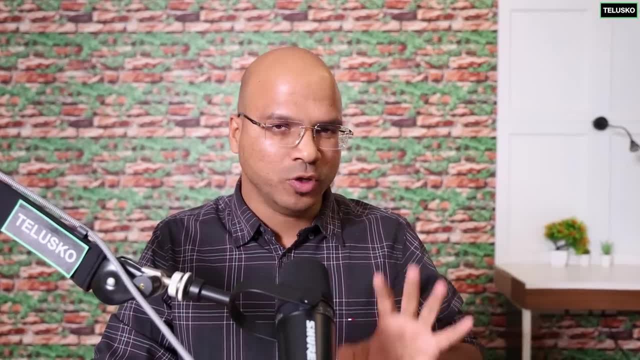 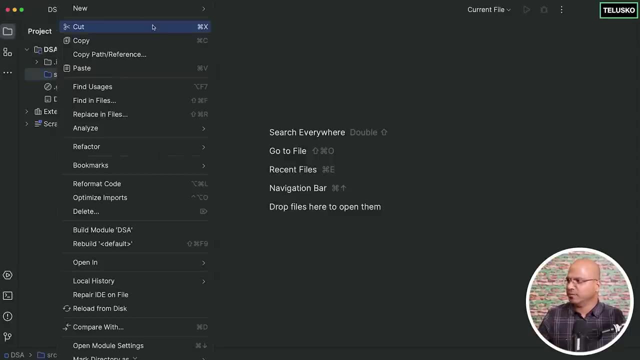 If you know any of the language, you can follow this. So I'm using an IDE And again, you can use any ID. I'm using IntelliJ IDEA. So in this I have a project. I will simply create a file here and we'll name this file as demo. 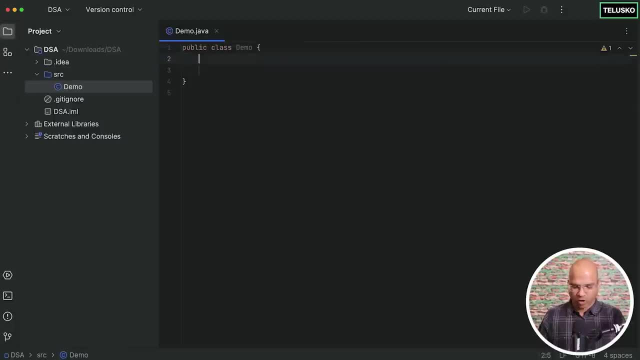 So we got a file called demojava, And this is where, basically, we'll also have our main method. So if you are coming from different languages, you know we also have main there. So we have a main. Now let's start with the actual work. 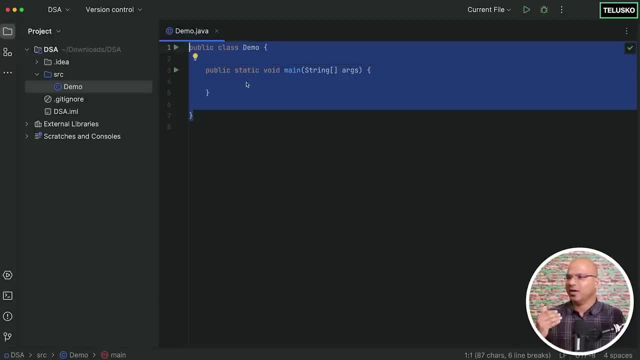 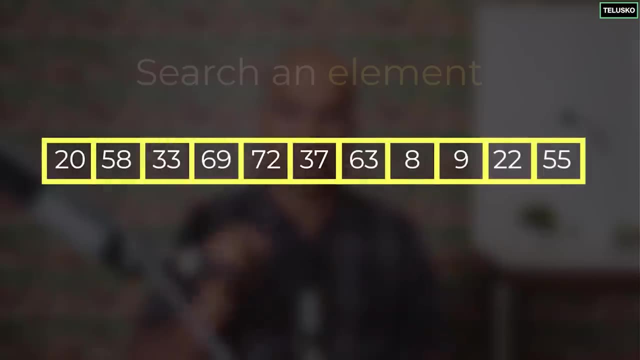 Imagine this as just a template for to run the code. We'll write our code here. Now, what we want to achieve Now? basically, we will be having a list of elements and we want to search a element out of it. Okay, Now, the size can be anything. 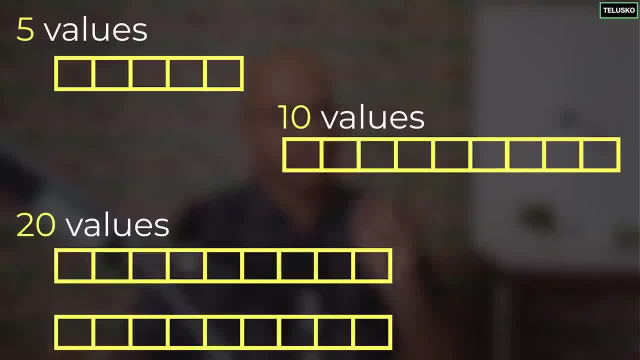 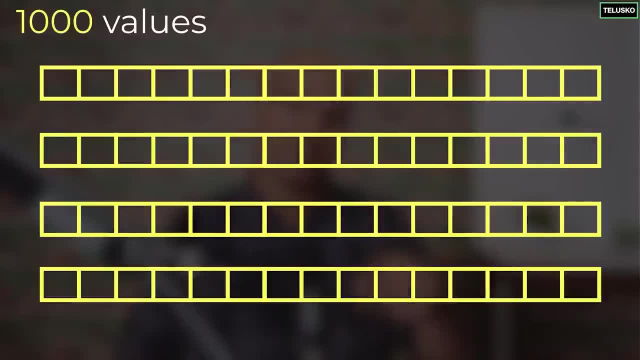 It can be five, It can be 10.. It can be 20,, a hundred doesn't matter. Initially we'll go for less number of values, And then we'll also see how do you work with thousands of values and how do you find element and then how much steps. 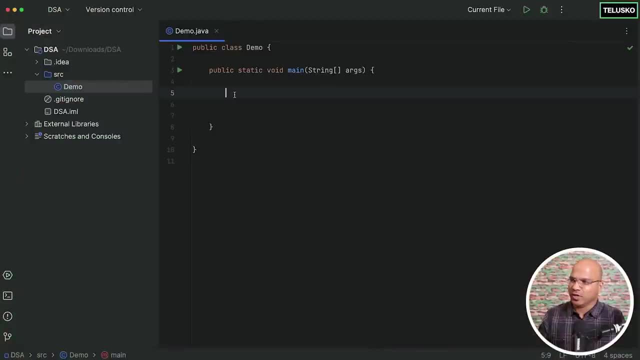 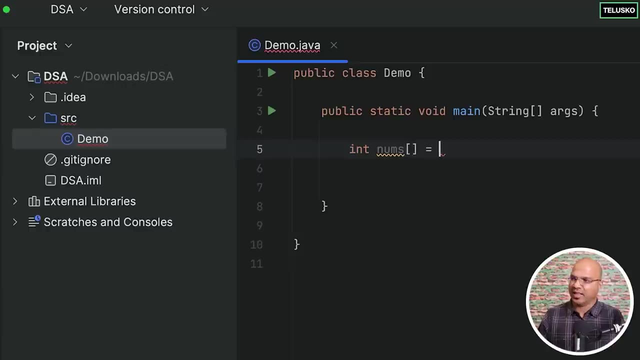 it takes to search a particular element there. So what I will do is first of all I will create a simple array here and we'll say this array name as nums. So let's say we've got an array, and then I will also specify. 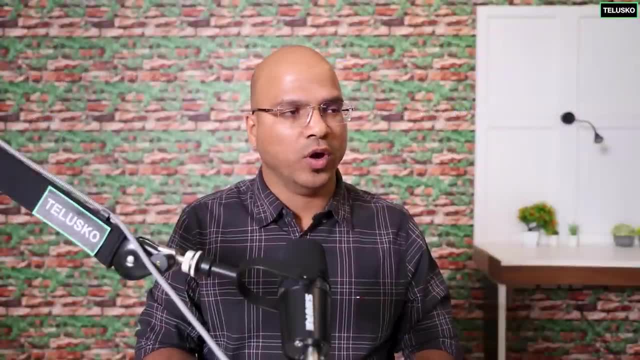 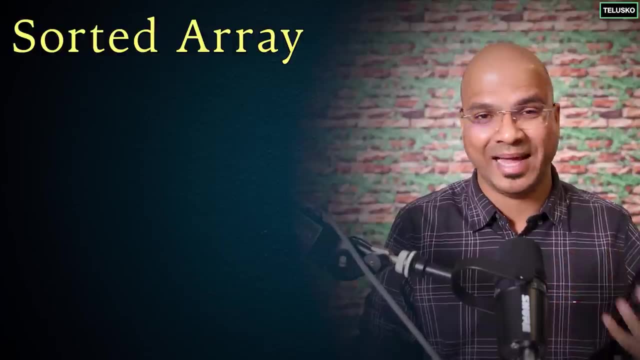 the initial values to it. And since we are going for a sorted array, of course, when you talk about the linear search, we don't have to specify uh sorted array. It can be applicable on any kind of array, but when it comes to the binary search, 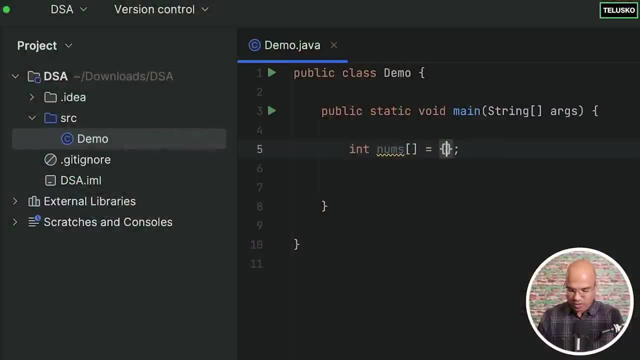 you need to pass a sorted element array or the least you can say. So here I will simply assign some values. Let's say we got five values here, and then I just want to keep it simple with those values. Of course you can have any value. 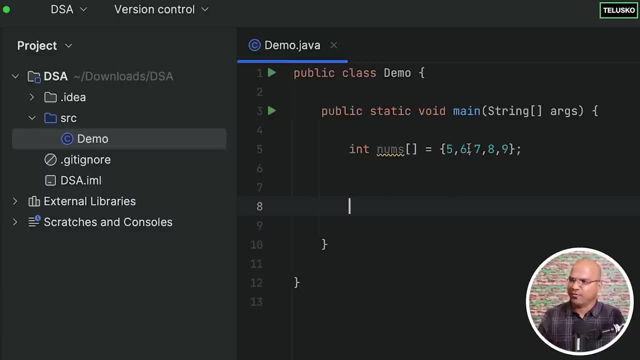 It doesn't matter, I'm just trying to keep it simple. Or maybe, if you want, I can say seven, nine, 11,, 13.. That's my love for odd numbers, Okay, And I want to search a value. 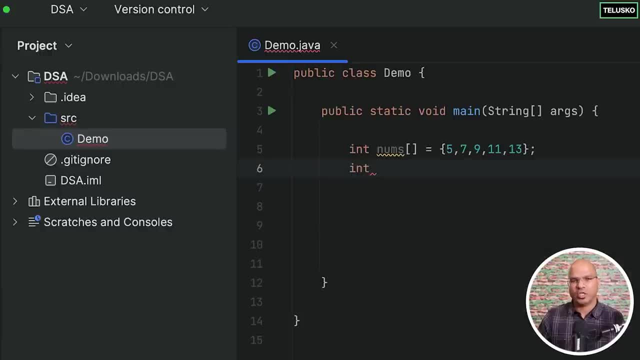 So whatever the value I want to search, we can also specify here. Now we can use any variable name, but we have already used target as a variable right When we were discussing the theory. So we'll say target equal to and we'll mention the target. 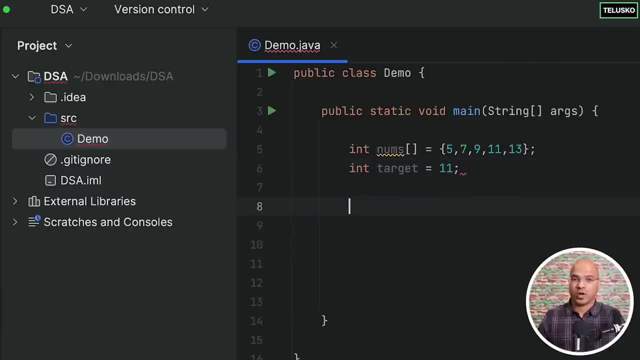 Let's say I want to search our element, which is 11.. Okay, So this is what I want to search from this particular list. We can do this with multiple algorithms. We can use linear search, binary search or whatever you think about. 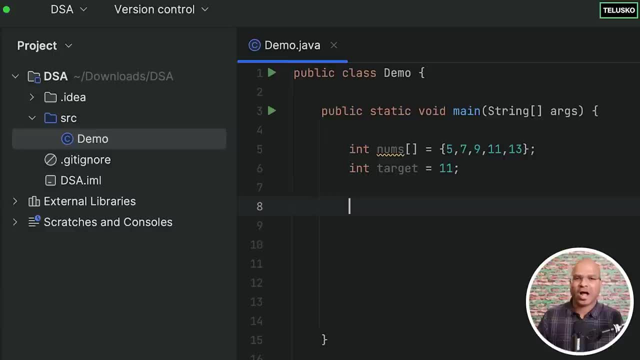 but let's go for linear search initially, And then we'll look at the binary search. Now, how do we do that? So what we can do is we can say: I want to get the result, Okay, Uh, I want to find this 11 in this list and give me the. 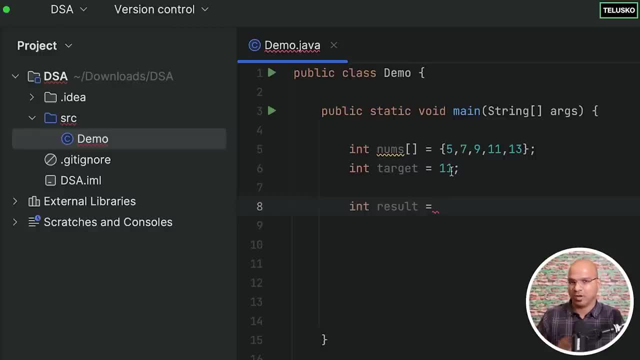 index number. I don't want anything else, just the index number where it belongs to. Okay, So who will give me that? So what I can do is I can assign this to someone else. Let's say linear search. Now this is another method. 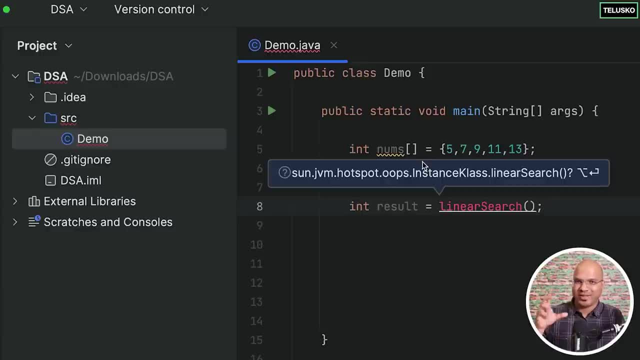 which will give the value to us. So I don't want to populate everything in this particular main Main will simply say: Hey, you know, I got this, two things, I got the list, I got the, the target value. You've tell me which index this value belongs to? 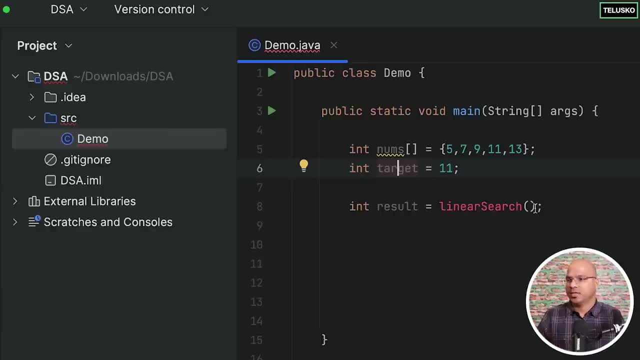 or if you don't have this value in the list, also let me know. So linear search will say: okay, um, accepted the challenge. It will accept two things: First, nums and target. why you have to pass nums, Of course. 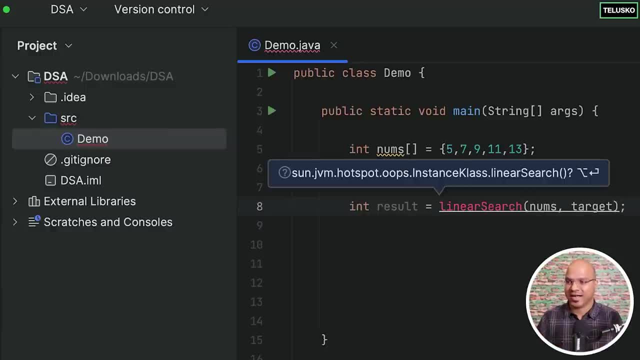 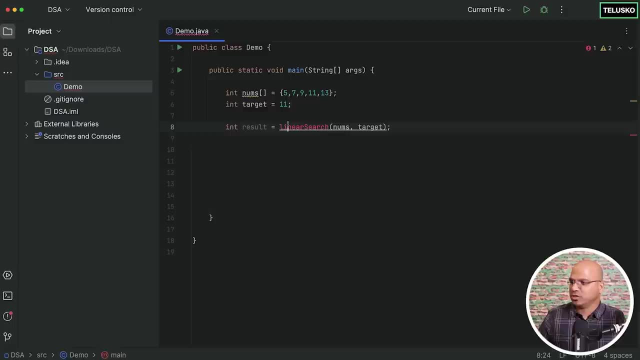 linear search will say: I will search, but tell me where to search and target. We'll say: this is a value you want to search. Now the thing is, we don't have this method yet, So what I will do is I will just use my ID to 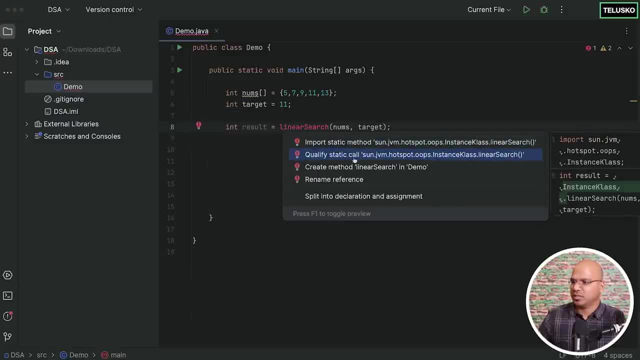 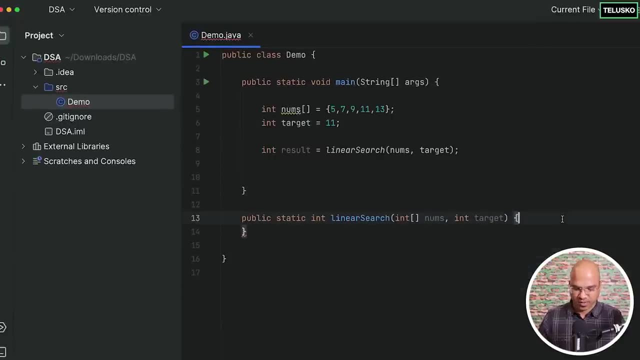 generate. Okay, So I will say more actions. Okay, Let's create this method and you can see. we got this method. I don't want this to be private, I want this to be public, and that's it. What you're doing is you are calling under the method at: 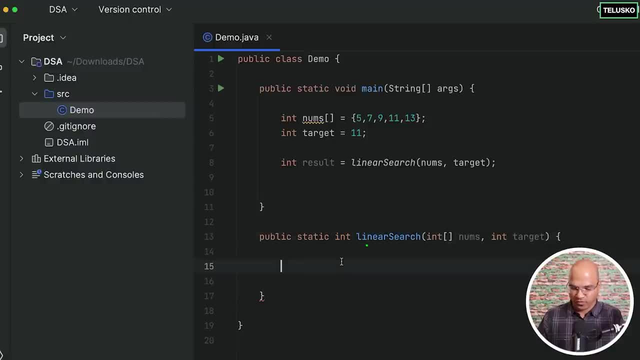 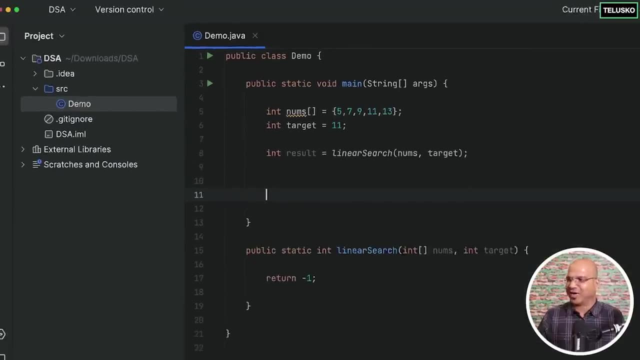 this point: since we are returning a value, what we can say? we can say: return minus one, Okay. Nothing fancy, I just want this to work And that's why I'm returning minus one, Okay. And what if you get the result? 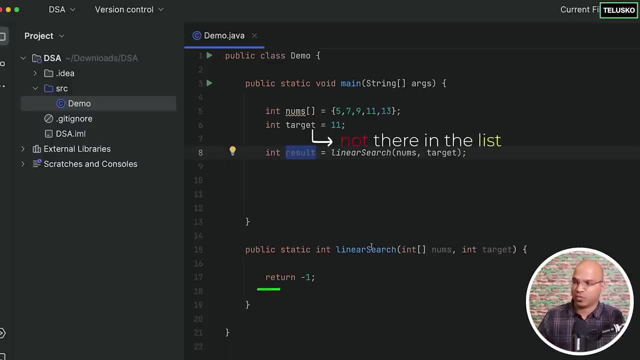 Of course. uh, if there's no, if this value is not there in the list, it will return minus one. Otherwise we can return the index value. So, whatever value you get you can, you can simply print here and you can say: element found at: 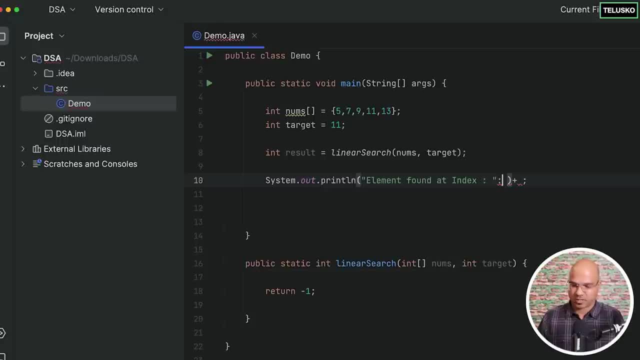 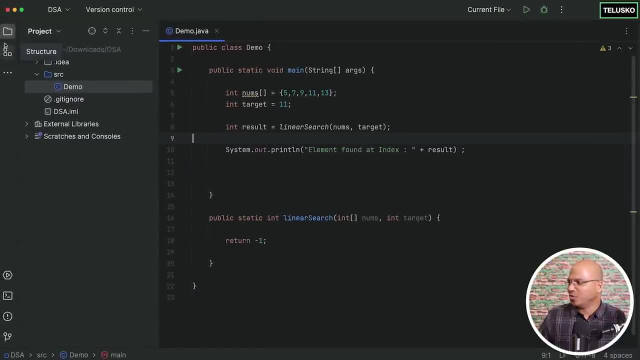 index and then you can specify the next value here. So let me just give a space So I can specify the result here. So whatever index is there, Okay, And let's run this code just to see. I just want to make sure that everything is working. 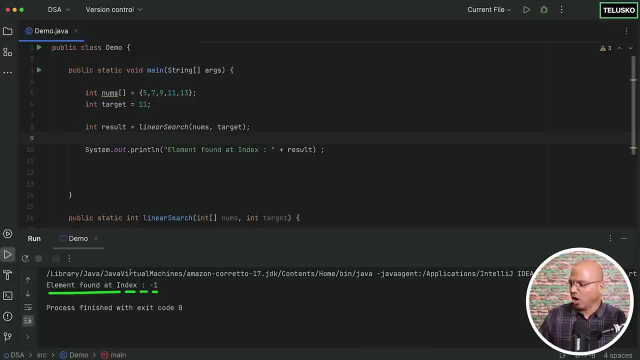 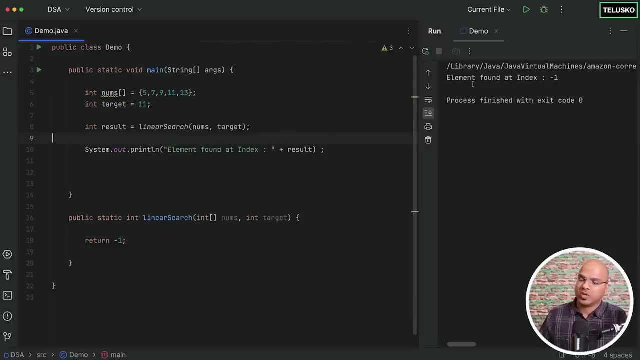 Let me just run this code and you can see. we got the answer. And also I want to move this to the right-hand side. Okay, So it looks good. So you can see the output says: element found at index minus one. That's weird. 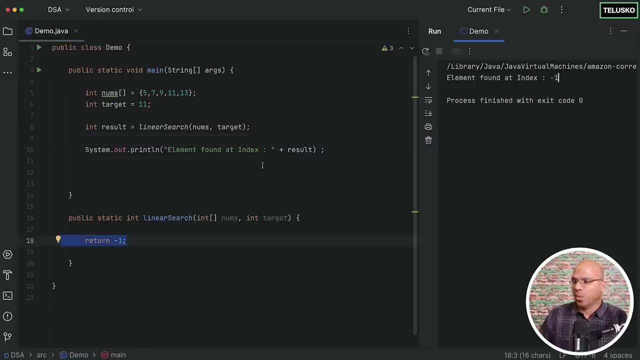 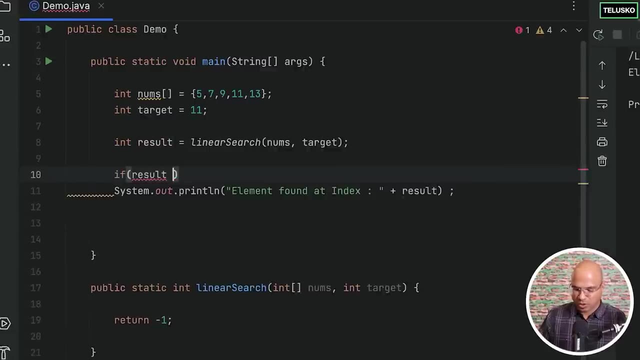 It's just that we are doing minus one. That's what is printing: minus one. What we should be doing is we should be checking if the result is not equal to one or not equal to minus one. So this statement it should print only when the result is not minus one, in case it. 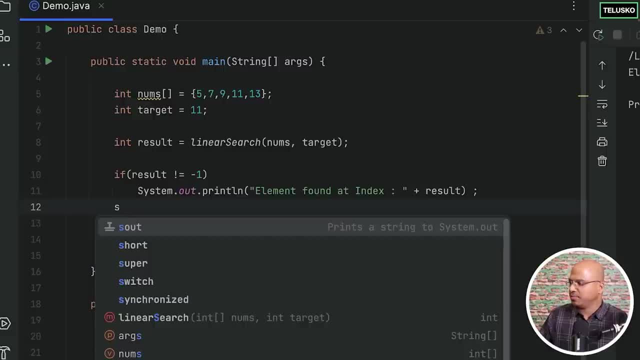 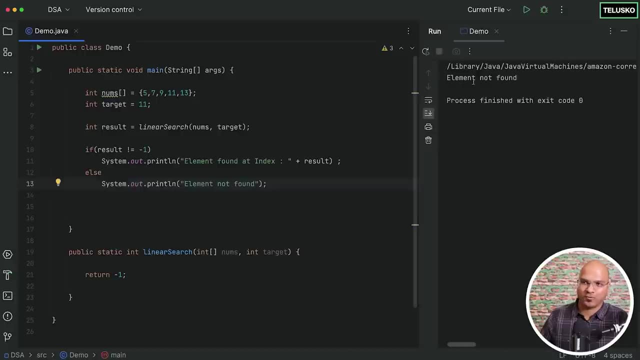 is minus one, That means the element was not there. So I can simply print element not found. Okay, And I feel this, This code, it will print element not found because we are not even searching Right, But we'll search now. 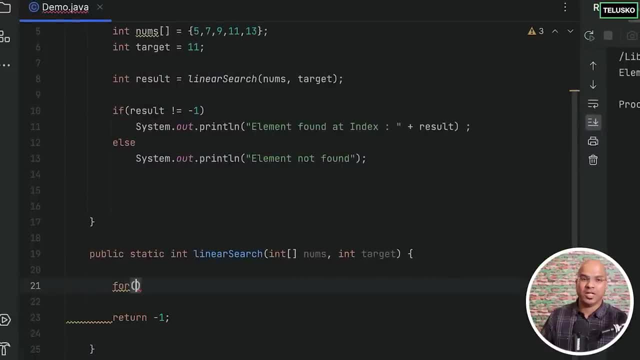 So how do you search? It's very simple. So what you can do is you can use a simple loop here. Okay, Nothing fancy against simple loop, And in this you're going to iterate. So we have seen the linear search. 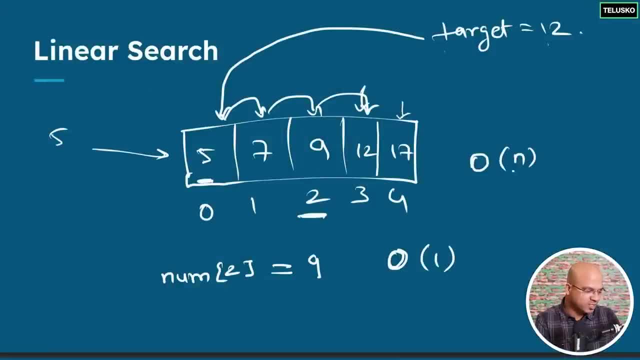 right? So, if you remember the theory, we have talked about this. So, basically, we'll search on the first element, right? So we are going to start from five and then we'll look for: is it matching? Is it matching? Is it matching? 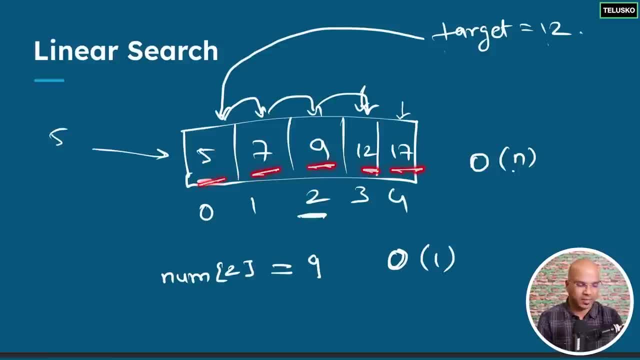 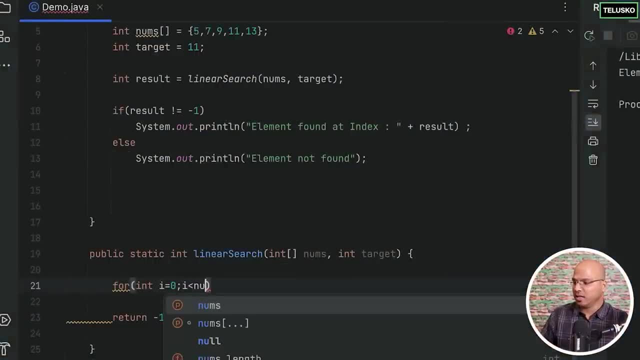 Of course the values are different, but we'll basically search for each element in the same way. in linear Search, If you want to move, you have to use a loop, So it will start from zero and we'll go till the nums of length. 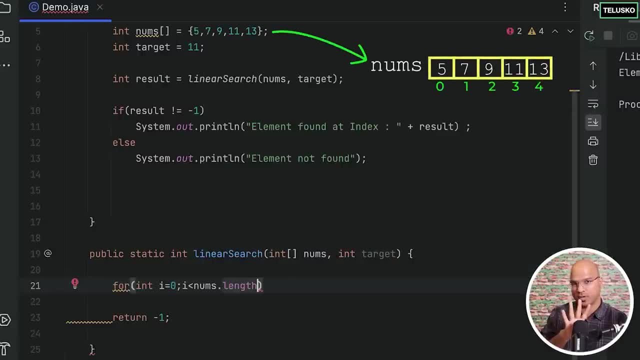 So, basically, if you, if the value, number of values you have, five, you have to reach four. Okay, So that's why we have seen less than, and then I plus, plus, but that's a for loop, right? So in this for loop, 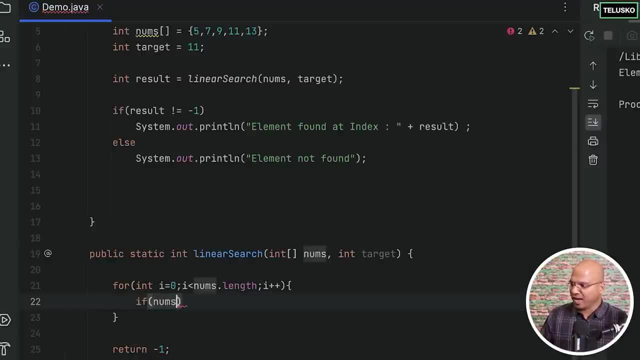 you don't have to do much, You simply have to check. So, whatever element you got- the recent, the current element which you're focusing on. So in the list we have five values. If you're focusing on five, we'll check. if five, 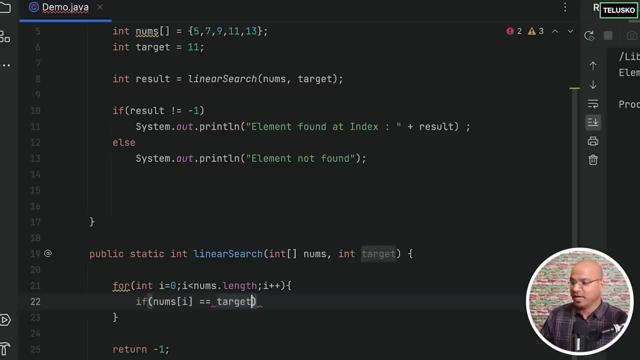 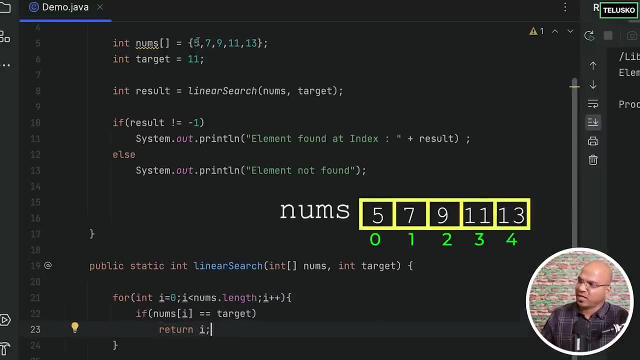 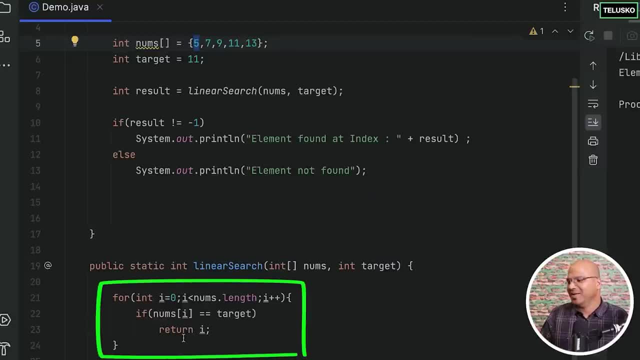 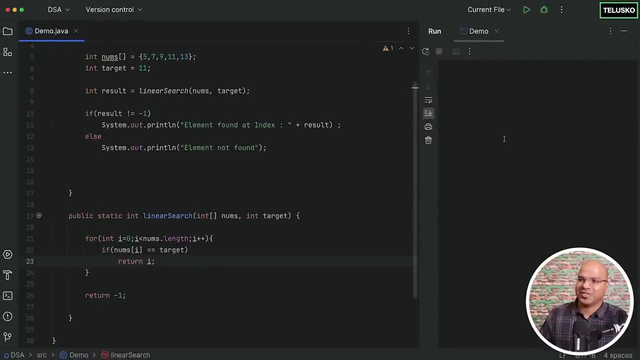 return zero. Your job is done. That's what you're doing here. Okay, And that's it. Okay, It should work. That's what we're expecting. Linear search is so simple. If you run this code, it says the element found at index three. 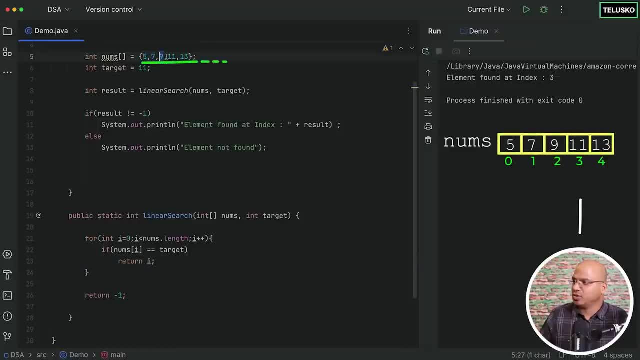 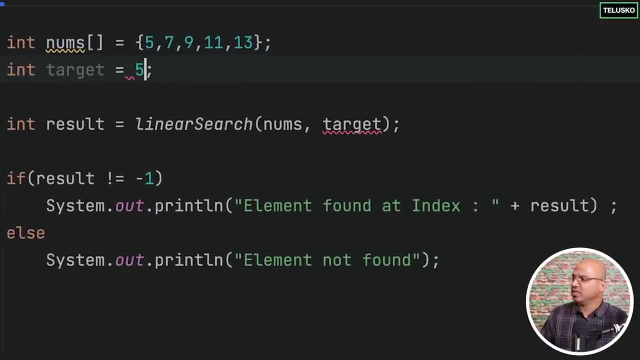 That's right. So this is zero. one, two, three and our job is done, Okay, Uh, what if you are searching for, let's say, five? in this case, it will print at index zero and that's what we got. 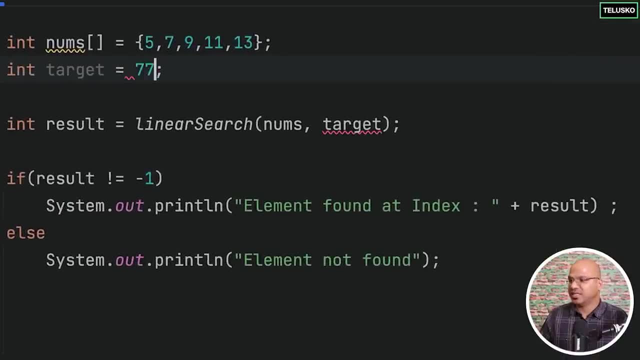 So this is working. But what if you're searching for something, let's say 77,, which is not there but there in the list? if we run this code it will say element not found. So linear search is working right now. 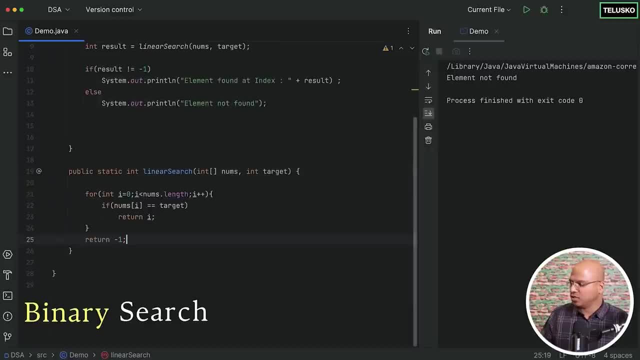 We can do the same thing with the help of binary search. Now let's see how binary search works. So what I will do is I will just write a code here which is public, In fact, I will just copy paste the code. 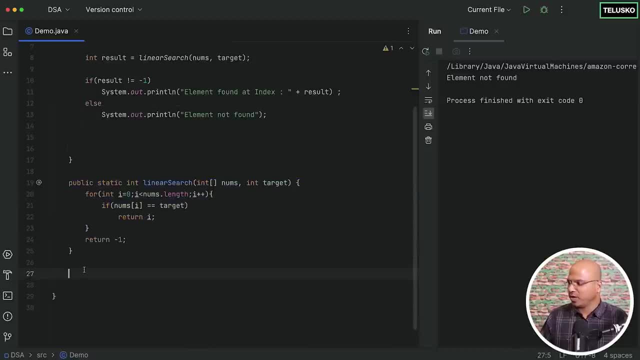 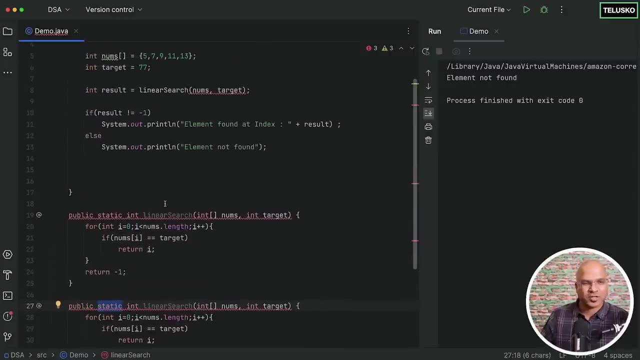 not a copy pasting, but reusing the code. I can simply copy, copy this code and paste it here. Now, if you're coming from Java and if you're getting confused, why I'm putting a starting method, why not non setting methods, is because I don't want to deal. 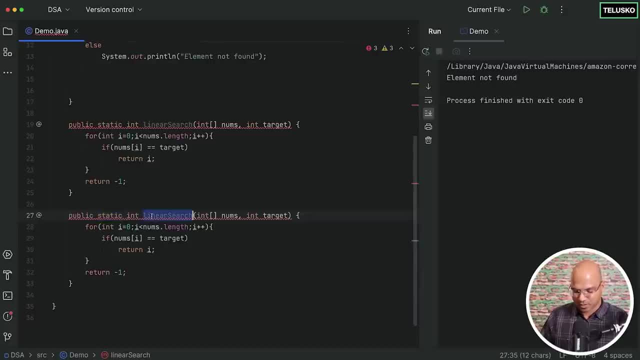 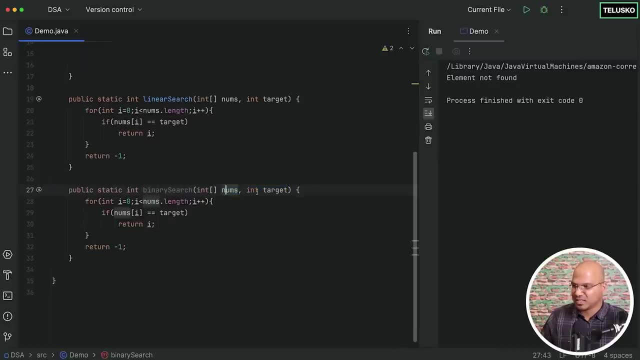 with objects here. Okay, It was one to give it simple. So we got a static method and a binary search. The thing is only method name will change. The parameter will remain same. in binary search Also, you pass a list and you pass the target. 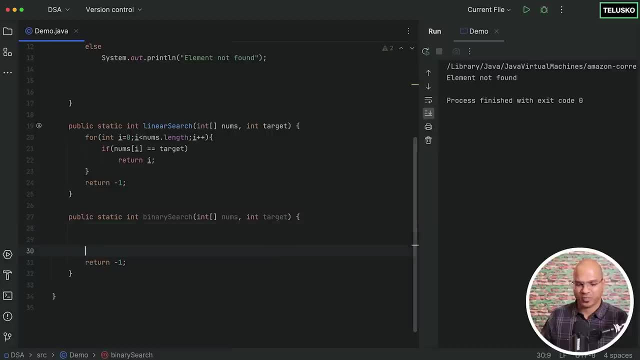 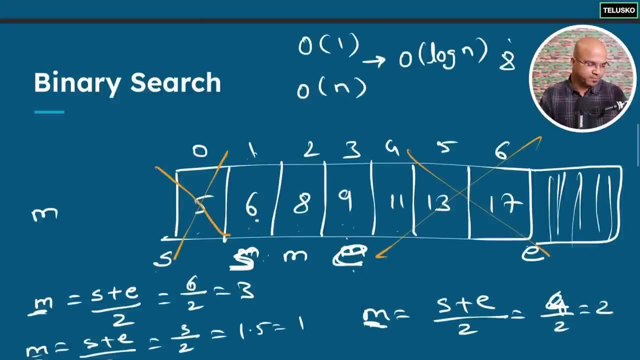 The algorithm will change. Of course, it will do in minus one. That's not. that is not something which is changing, but what we will do inside this. Now, if you go to the board here, what we have done is, if you have a list of values, 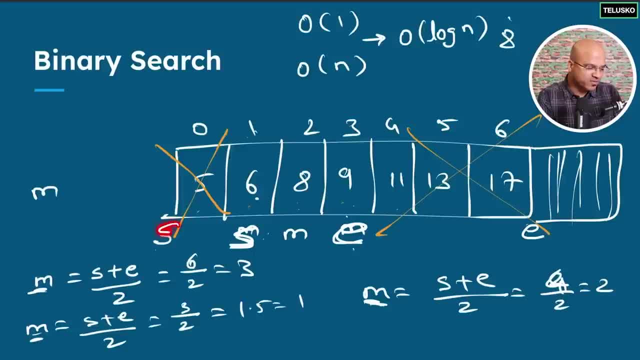 if you can see, we have a list of values here Now. initially you have to specify the starting point and then you have to specify the ending point as well, right? So starting and ending you have to specify. in this example, we'll say left and right. 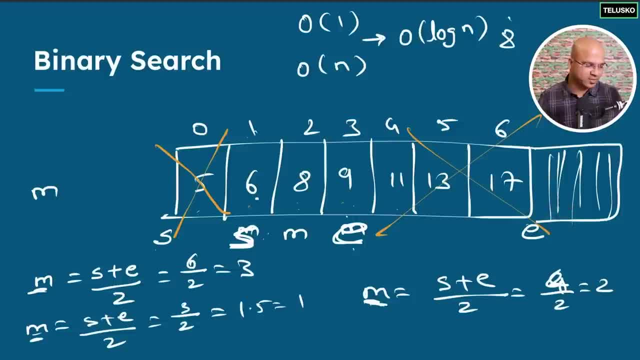 Okay, Because that's how that makes much more sense. right, Left and right. Starting point is left, Ending one is right, And then you will find a mid. every time you find a made. if it is matching, that's great. 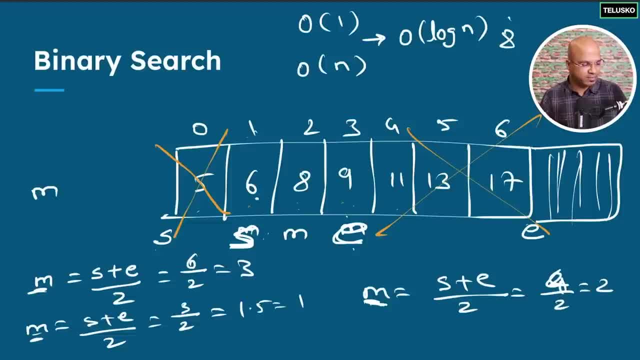 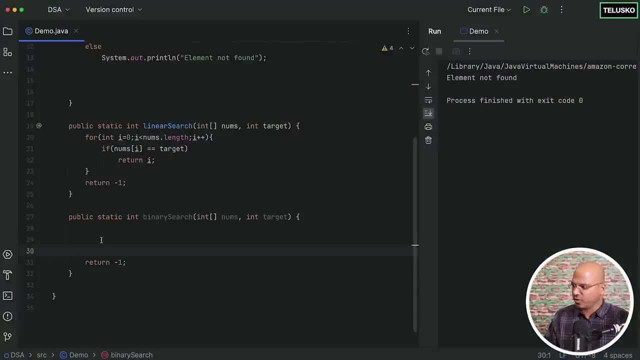 Otherwise you have to basically skip the number of elements which is in the other section. Okay, So how do we do that here? So what I can simply do here is: in fact, I will, just for my reference, I will also have those values here. 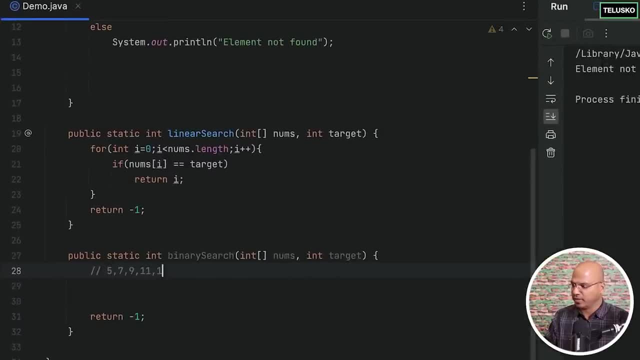 So I will say five, seven, nine, 11 and 13.. Okay, And the value. let's say which I'm searching for. this time let's have the value. So let's say I'm searching for 11.. 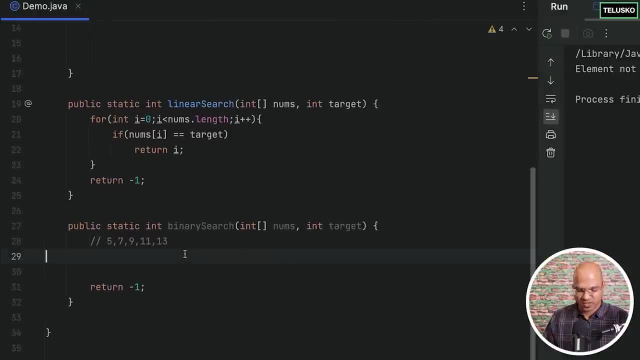 Okay, So what I will do is if you, when you're searching for 11,, first of all, you have to specify the starting point. So I will say: left, In fact, left ain't. left is equal to now, left is a. 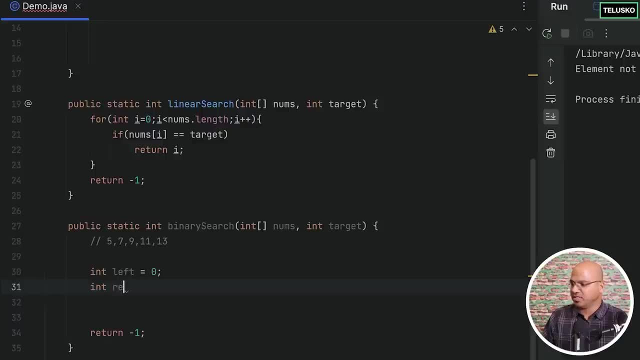 starting point right, Which is zero, then ain't right Which is the ending point, which could be four. but then why to hard code it? What you can do is you can say nums dot length minus one, because nums dot length will give you five. 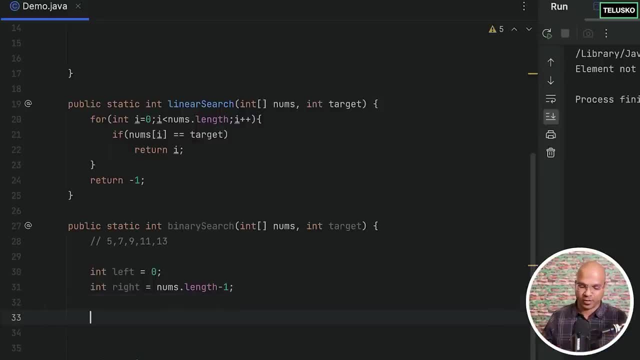 You have to say minus one, which will give you four. So now we've got the starting point, ending point, and then our journey begins, right? So what are we going to do here? So we'll use your while loop here. 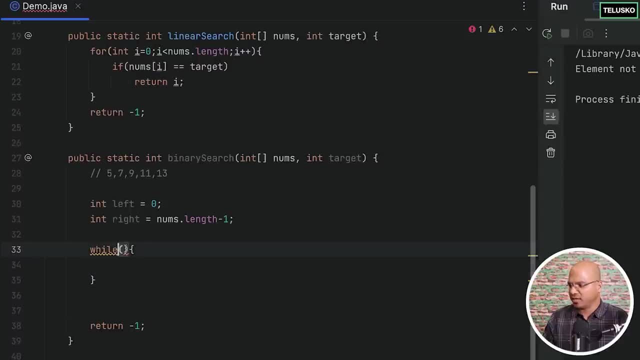 Now, inside this while loop, what I'm going to do is I'm going to check if my left is less than equal to equal to right. We'll check if left is less than right, because that's what we want. right. Left should be on the left hand side. 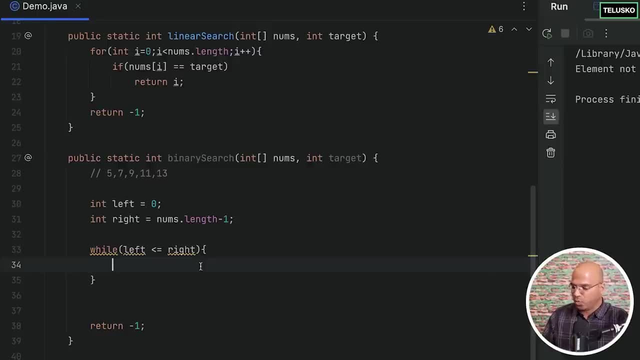 which is the, which is smaller values. And then here, what we'll do is we'll find the mid. Okay, That's the journey we are going to start. So mid is basically your starting point. right, Which is left plus right. 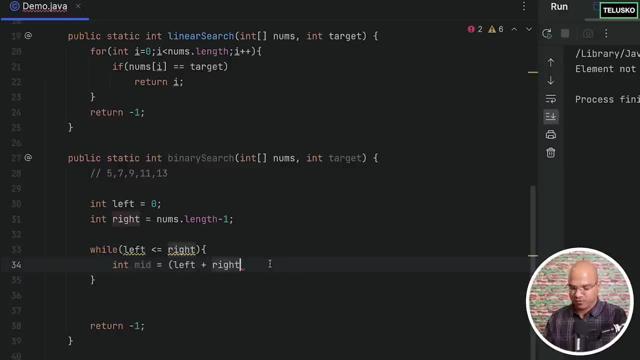 And we want this to be in the bracket so that we can divide. So left plus right divided by two. Okay, That's how you find the mid. right Now, once you've got your mid, you can basically check if the nums of 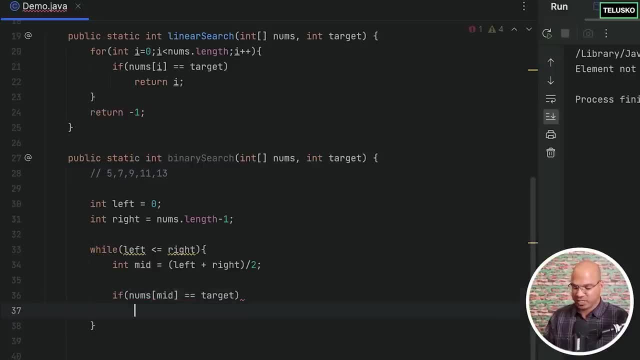 mid. is it matching with target? If it is matching, that's great. We can simply return the index, which is mid. Of course, right Mid is representing, representing our index here. If it is not matching, then we have to change the value of left or 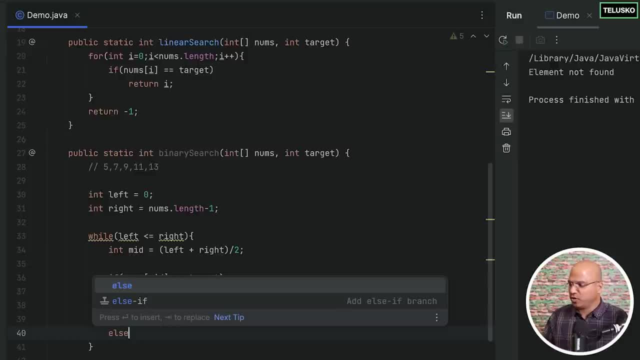 right depend upon what you got in the mid. So what we'll do is we'll say: if else, if now, how do you check? So we can check if nums of mid is less than the target? So let me take this up as well. 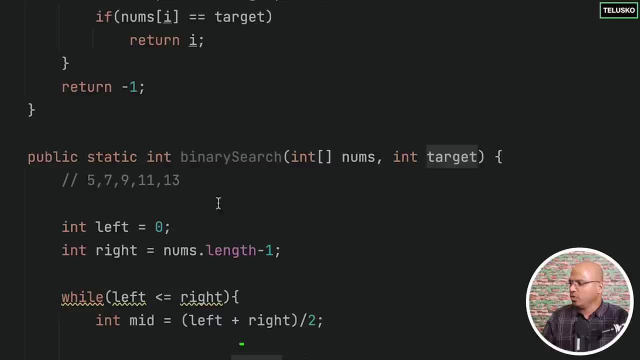 Yeah, So if nums of mid is less than the target. So let's say, when you talk about this, elements, and then we are searching for 11, right, The mid which we got is nine If the nine is less than the 11,. 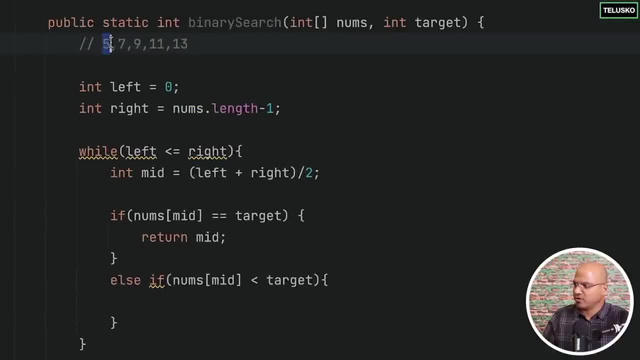 we have to shift our left right. So this left, which was representing five, will shift here now I mean not even nine, We don't have to even consider nine right. So what we can do is we can say left will shift to mid plus one. 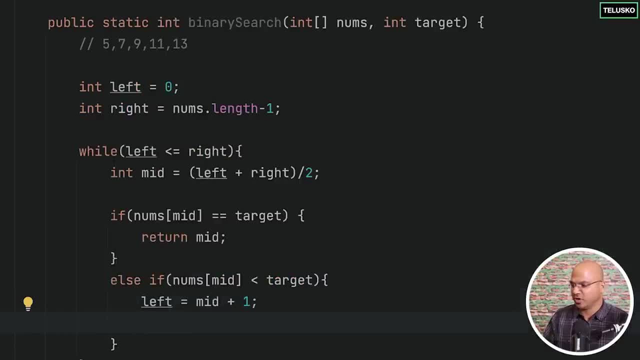 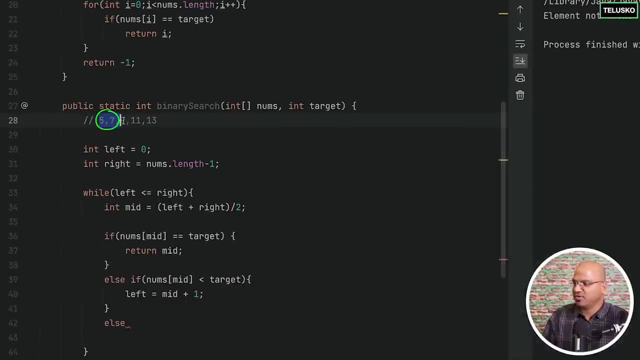 Okay. So basically now we have two values, 11 and 13,, which we are going to focus in the next iteration. But what if you are searching for something else Which is on in this side? let's say we were searching for seven. 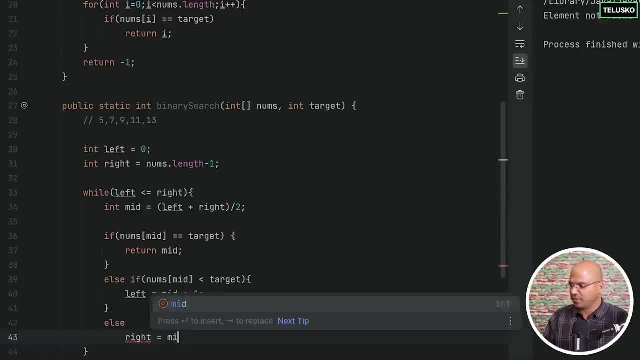 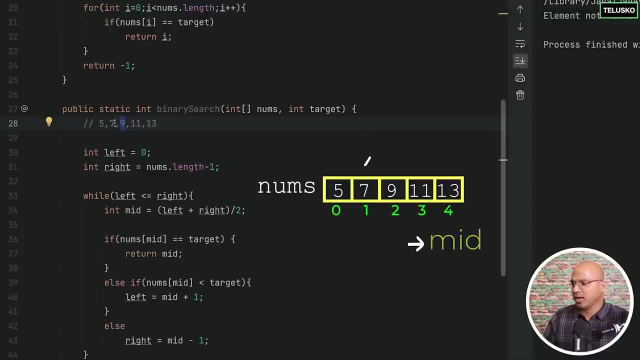 In this case, we have to shift our right. So right is made minus one. So basically, let's say, if you're searching for seven, here we've got a mid as nine. What you will do is you will say: okay, so the value is less than the mid. 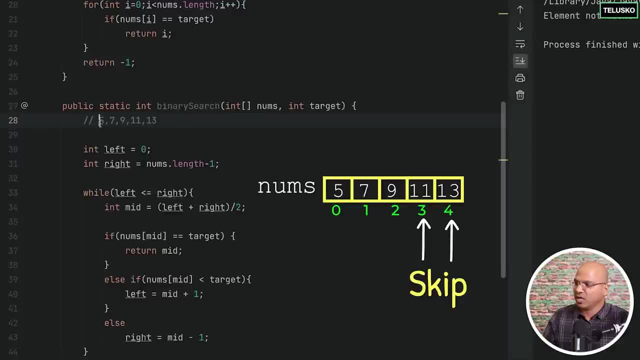 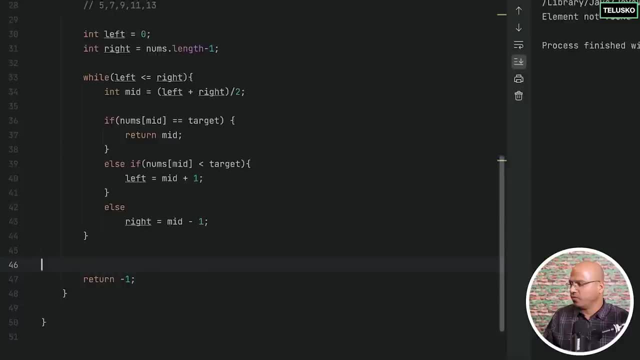 So we have to. we have to skip this too. The focus will be only on five and seven. That's what we have done here. If you're searching for seven, Okay, I think this looks cool. We, our job is done. 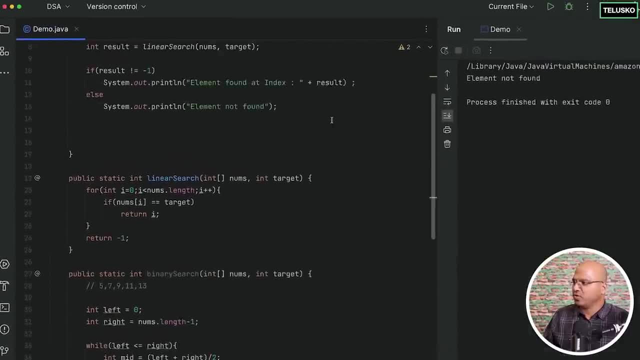 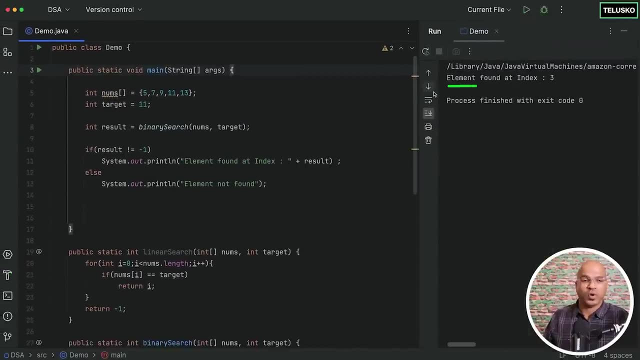 Let's verify If, if things are working out, the only thing that we do is, instead of searching for a linear search, this time we'll go for a binary search. Let's run it works. You can see. it says found index at three. 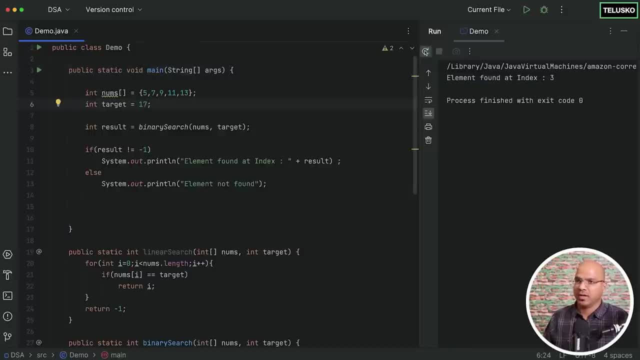 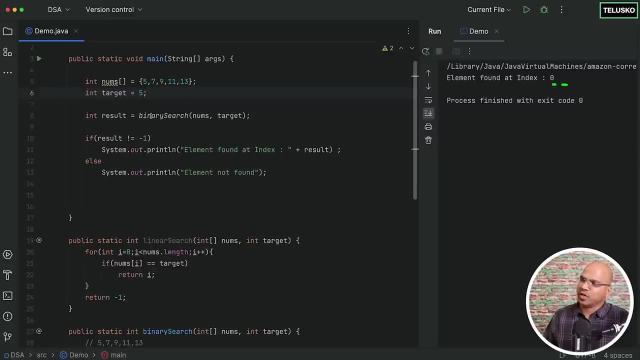 And what if you are searching for, let's say, 17, which is not there run, It says not found. let's search for five, and it says it works. You can say index zero. So that means you can use linear search or binary search. 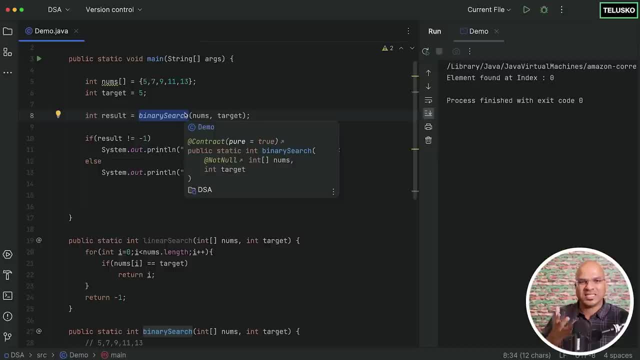 Both works, but what if you want to really see how many steps it is getting? So what I will do is let me just say this is result two, which is binary search, And let me also say result one. Of course, I'm not going to use both the things. 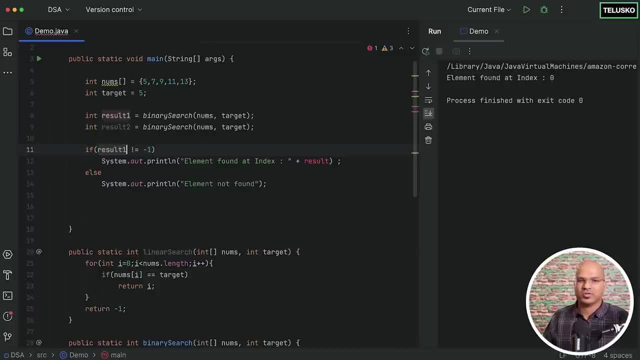 I'm just. I just want to call both the methods. Okay, I'm just going to use result one, because if linear search is able to find it, binary search will also able to find it. Okay, Let's bring result one here. 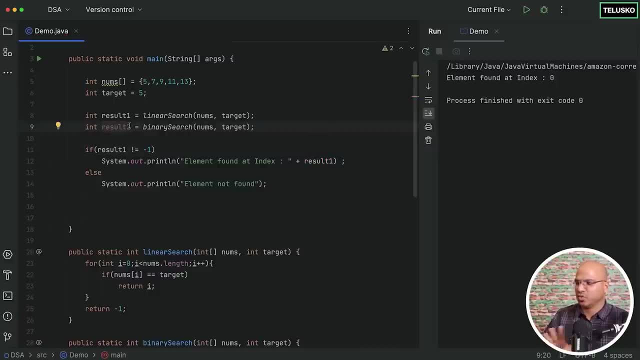 So I just want to call both the methods. That's the reason I'm using result two. but result two, we are not using it anywhere else. Okay, So let's do this with both the algorithms and you can see both will print the same thing. 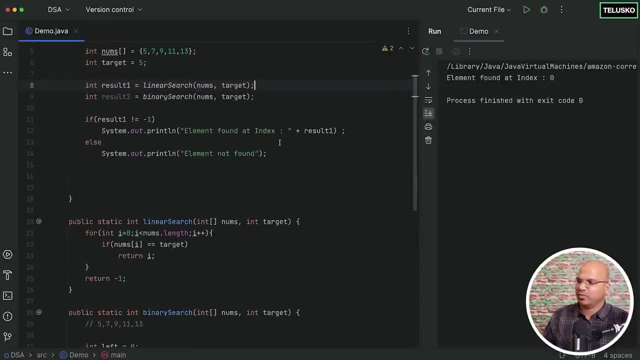 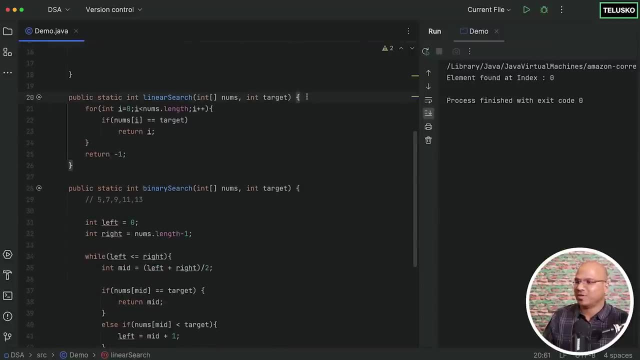 Oh, we are not printing The second part. Okay, Doesn't matter, Both will give the same result. but what I'm really concerned about is the number of steps. So what I'm going to do here is: let's calculate the number of steps it takes. 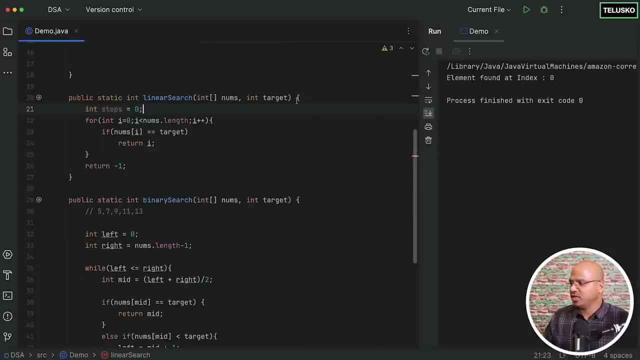 So I will say, for linear search, steps is equal to zero initially, And every time the loop it treats okay, I will simply say steps, number of steps taken. So steps plus, plus, and then I'm going to print, just so, just before return. 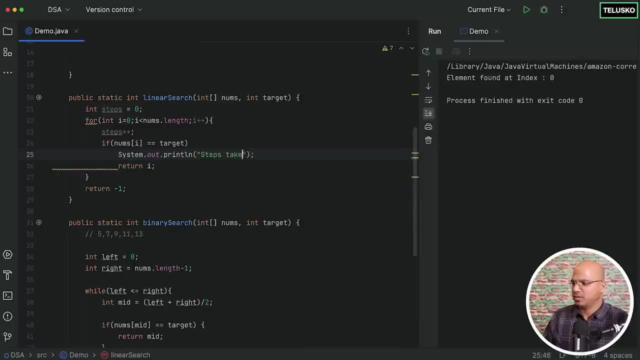 I'm going to print steps taken by linear colon and I will print steps. The same thing I want to print here as well. What if there's no element found? So this will not never be executed, right? Okay, We have to put this into a curly bag. 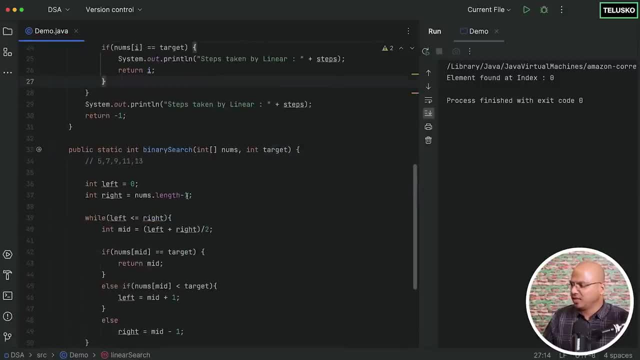 It's cool. So we are printing the steps here. The same thing I think we should do for bunny search as well. So here I will say: ain't steps is equal to zero. And every time you iterate in this loop you will say steps. 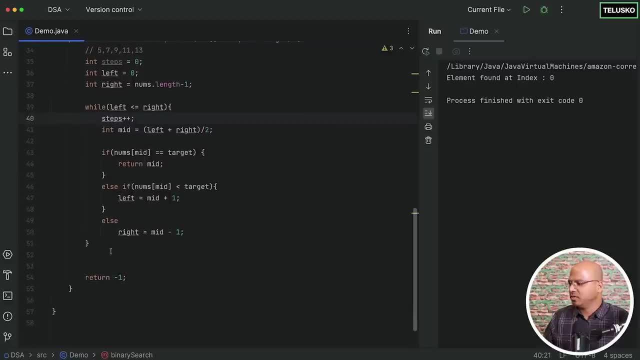 plus, plus, and then basically here you will print the same statement. So I will just copy this, So we'll print before returning the value, but here we'll say binary And we also print this before returning, just to cover all the cases. 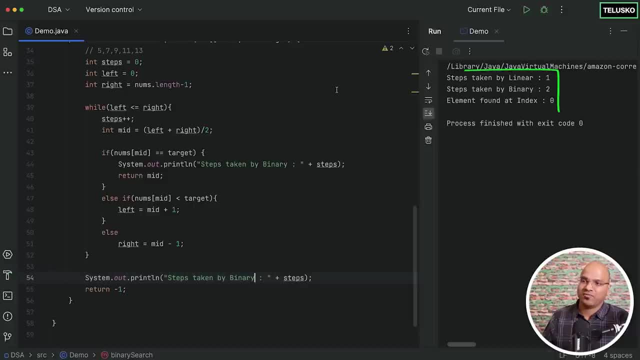 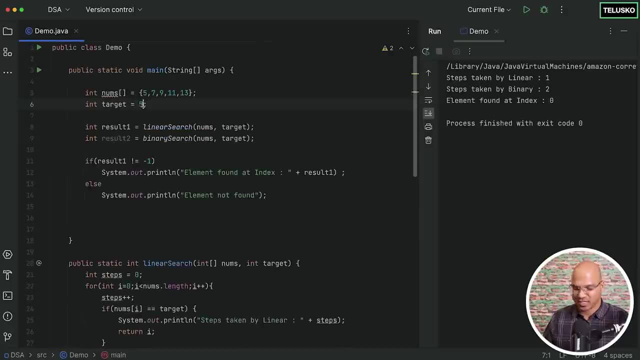 Okay, Let's see what it does. Run this code and you can see for five elements. linear search is searching in one. Okay, This isn't been. we are searching for five. right, I think they're searching for five. Let's search for. 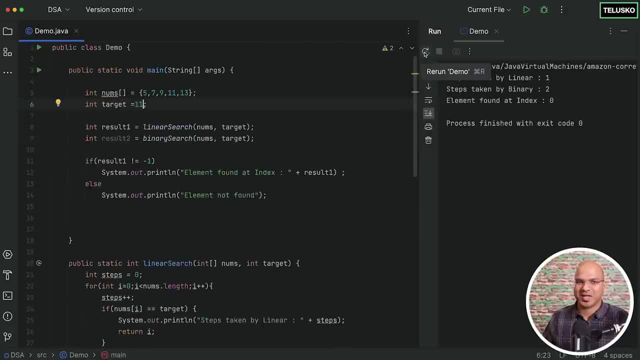 11.. Okay, In some cases linear search works well. run and you can see. the linear search takes four steps. The binary search takes two steps. That's crazy. Run again, Of course, you will get the same output. but what if the values are higher? 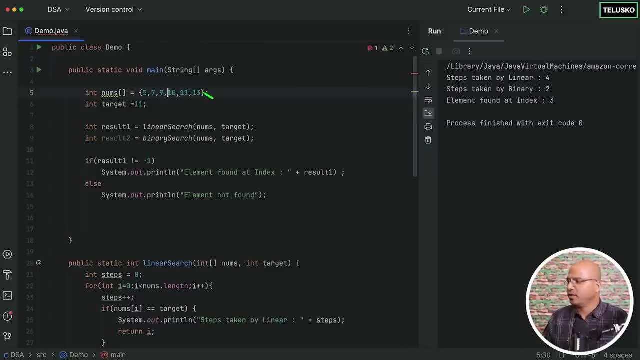 Let's say I have more values here. Let me add 10 me at one, two, three. So now we have more values, right? I don't know how many values we have, but let's say for them this code: 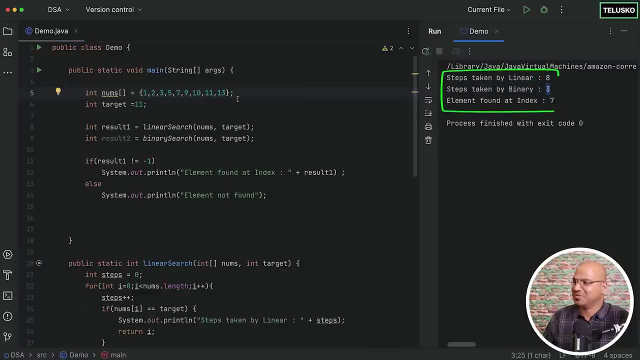 the linear search takes eight steps. Bunny search takes three steps. Okay, But what if you have thousand values? Now, how do you check thousand values? Now, that will be tricky. So what I'm going to do is: let's add some random values here. 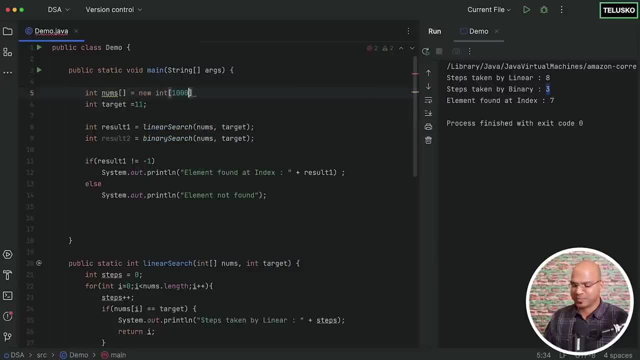 Let me create a array of size: thousand- I don't want to specify my own values- Let's say thousand, And the value of which are searching for is, let's say, 500.. Okay, It's somewhere between, or maybe I will say 900. 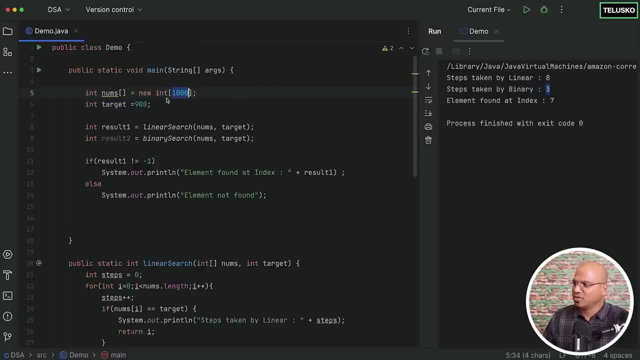 Let's see what happens. So I have a value which is one to thousand I'm searching for- I mean, I have thousand values in the area and I'm searching for 900, but by default the value will be zero. 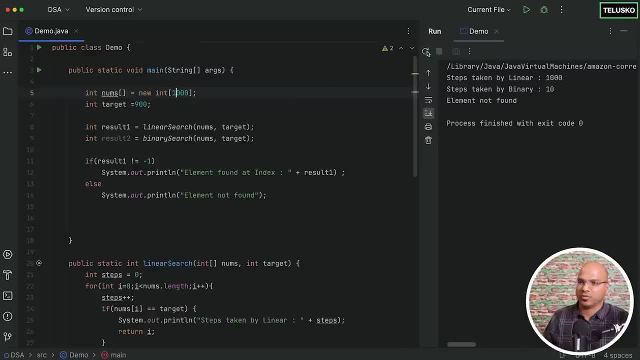 Okay, Uh, example: if you search this it will say not found. but look at the number of steps. Linear search takes thousand, bunny takes 10.. And what if you have more values here? run linear search takes 10,000, bunny takes four. and look at the size. 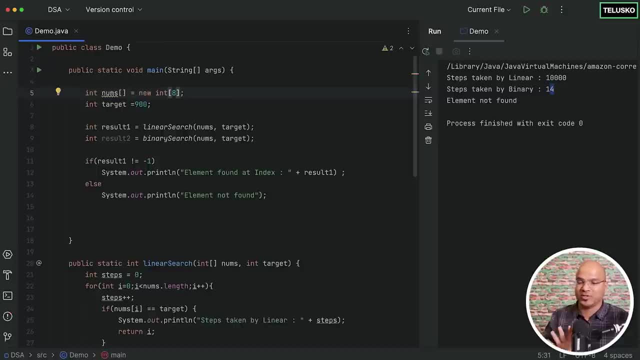 Example. let's say if the size is eight and by default all the values in the area is zero. So anyway it is sorted by default. And you can see if I run this code, uh, which says eight for linear, four for binary. 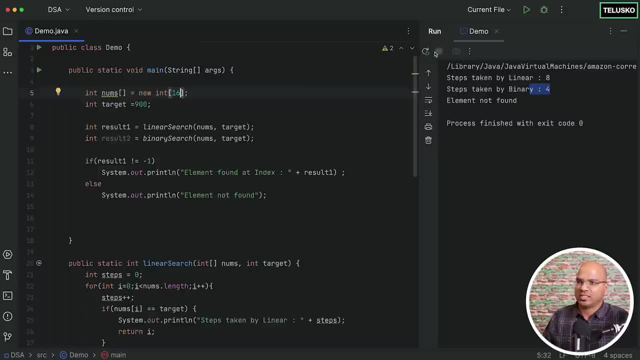 but the moment, uh, I double the values- look at these steps taken by binary is only one extra linear on this double If I double the value again 32.. So every time you double the value, binary search will take only one extra step. 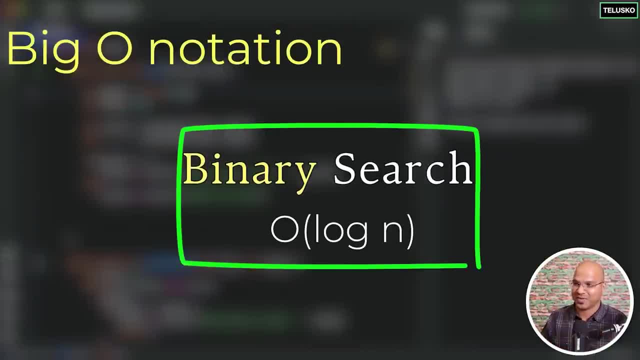 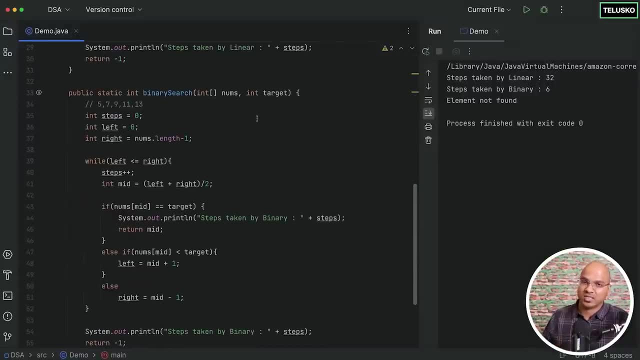 And that's why we say it's a big one. notation for this is log N. Okay, So in this case the binary search works better than the linear search. Now the same code you can write with the help of binary search as well. 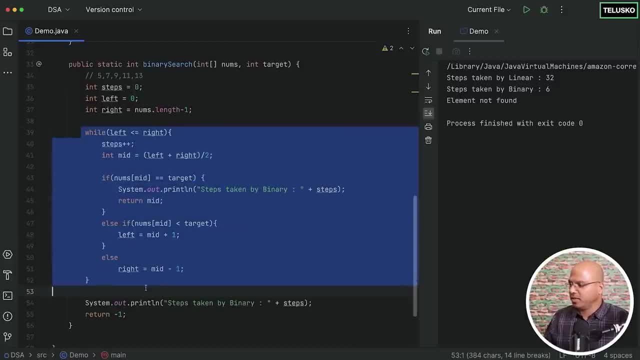 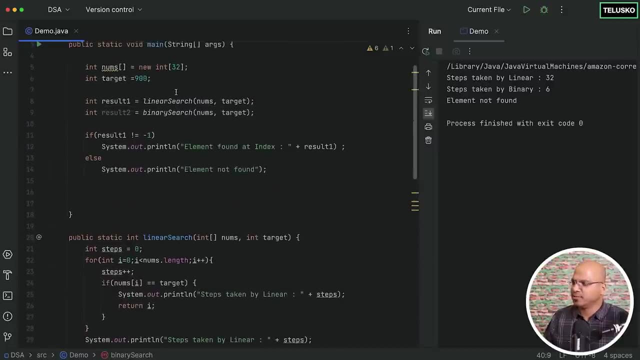 Example: ensure of using a loop. here I can simply come in the entire section and we can replace this with a recursive function. The only thing is in recursive that the changes you will be doing is in recursive. You're going to call the same function again. 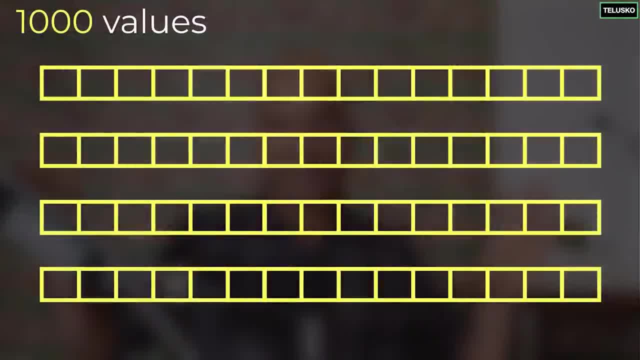 again by changing the values. Let's say, you have this big array and then you're done your first search. You find you found them made. Now, the moment you found this section, let's say this part or this part which was matching. 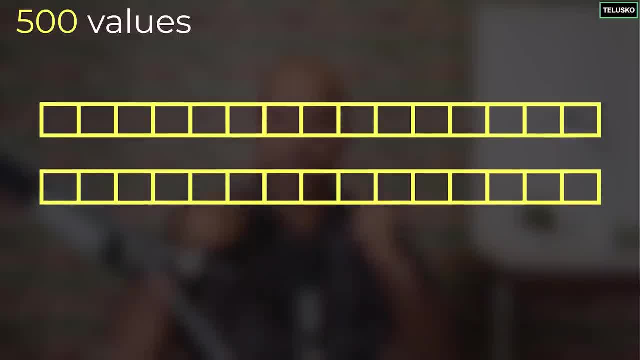 you will remove the other half And again you will run the same when I search on this list, And then again you will break it down into two parts. You will remove one and you will run the binary search on the other one. 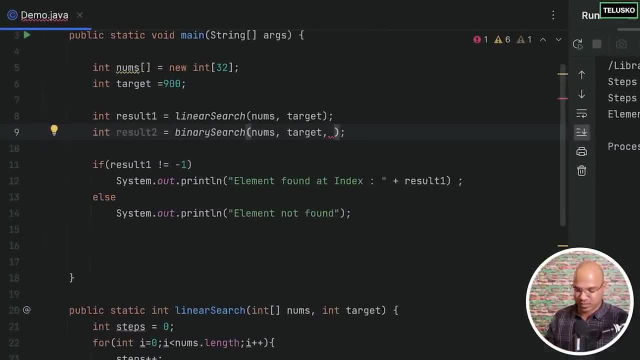 So in binary search, basically if you want to make it recursive, you have to pass two more things: which is int left and okay, not int left. You just specify the left and right. So I will say zero and nums dot length minus one. 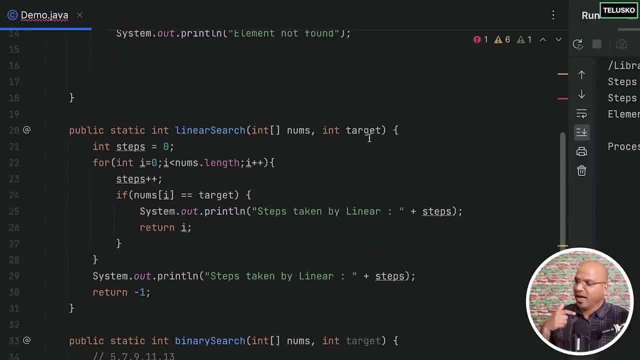 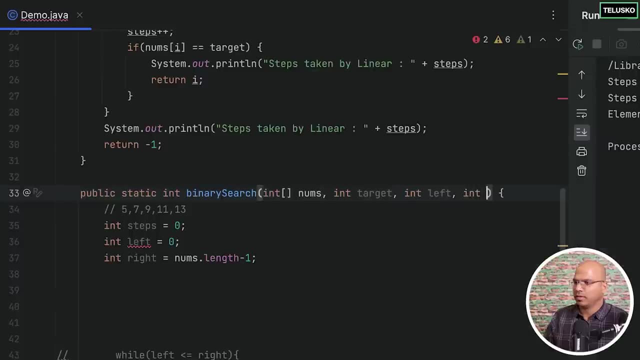 So, basically, you have to specify the start and the end, And every time you call binary, you will simply accept those two things. Yes, You will say left and right, so that you don't have to specify them here. In fact, you know. 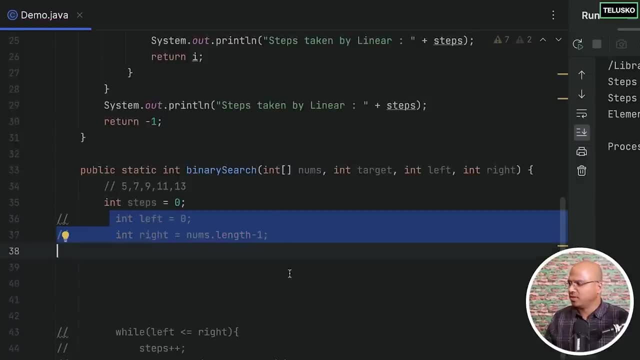 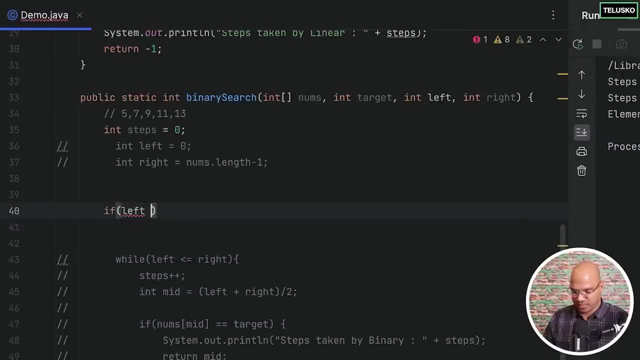 instead of removing it. maybe you want to refer this later. I'll just come in this section Now. since this is a recursive, you don't need a loop here, right? What you can do is you can check if the same step left is less than equal to right. 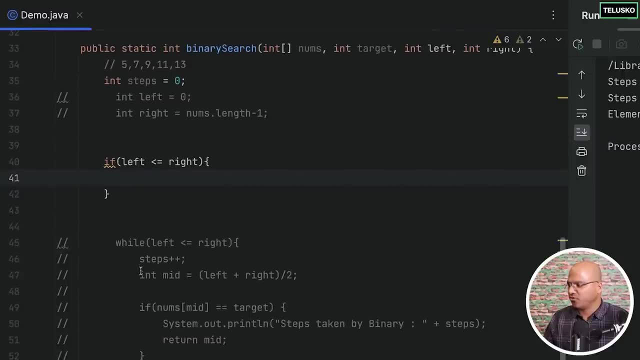 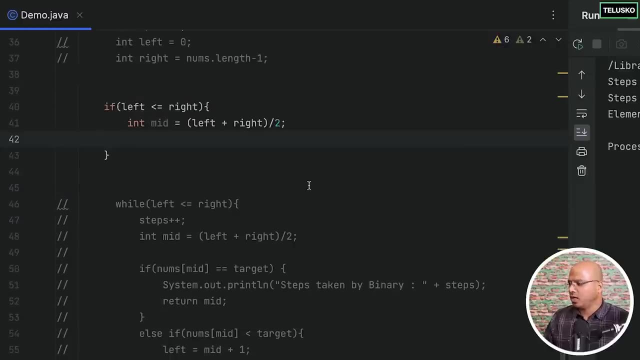 If this is a scenario, what you will do is, of course, you have to find the mid. I will just copy this code: This is where you're finding made, And after finding the made, you can basically also- uh, check the same logic. 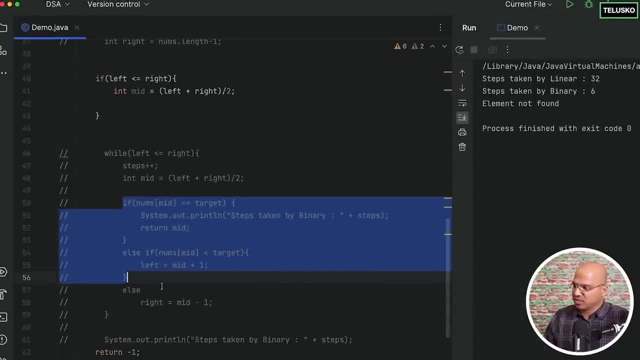 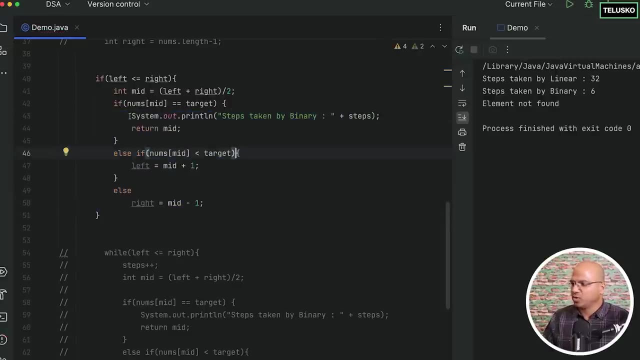 This is a logic you're going to use. The changes is we are. we are going to change in the else part. I'm in the if else part. let me uncomment the entire section, the changes you're going to do. Let's. 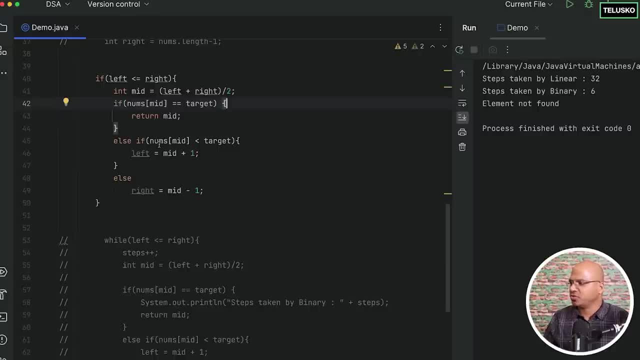 let's not bring the steps Now. we know the steps right, How many steps it takes, but I'm just trying to convert that into a recursive function, So it will. you will return mid here, There's no problem with this. 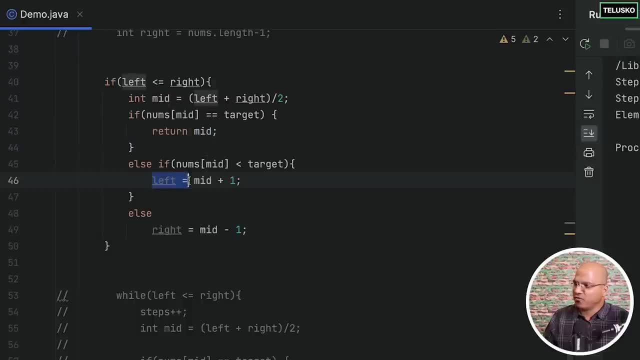 The changes happens in the else. if So, in the else. if, instead of doing this, we are going to basically call the binary search once again by passing the same nums, and then you will change the target value now, So you will pass target value. 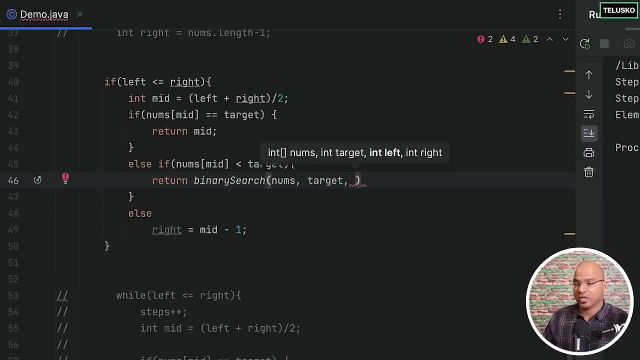 So you have to pass nums and target value, Then you have to pass the left value. Now what is left? So in this case we had to change the left right. Left will become mid plus one and right will remain same, Right will remain right. 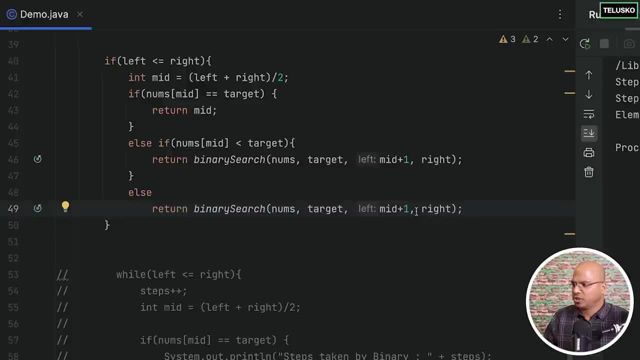 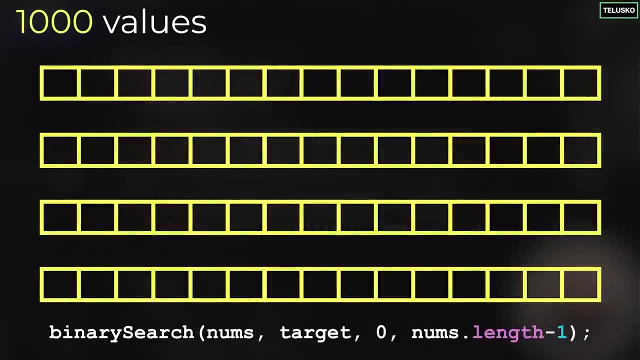 But here again we have to make the changes. else part instead of this, left will remain left and right becomes mid minus one. So basically, what you're doing is you are changing the values like this: If you have this list of values, you break it down into parts again after checking, and then your chain. 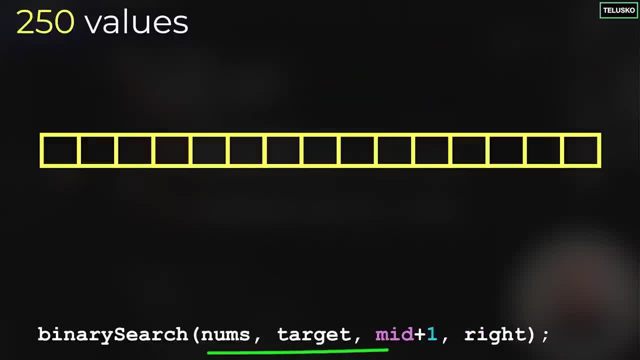 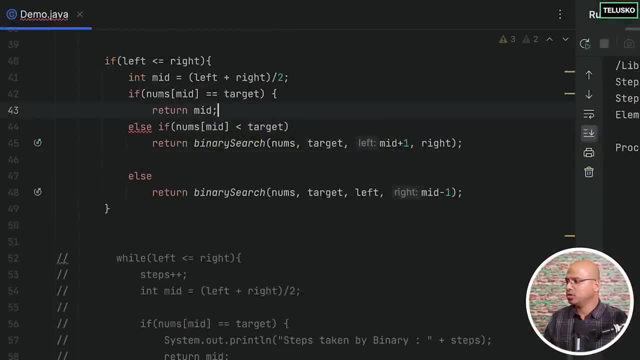 you're again calling the same binary search with the new values. Okay, that's what we're doing here. So remove the extra curly brackets just to make the code look good or short, basically, And that's it. This is your binary search. 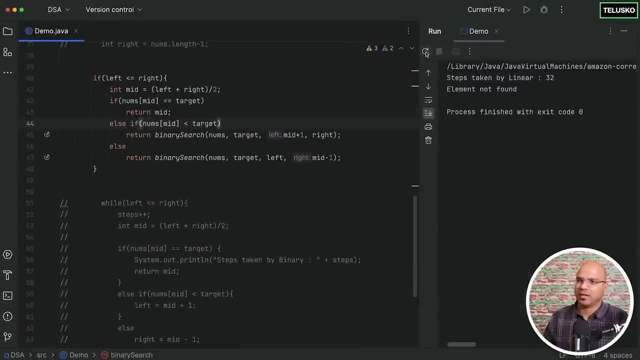 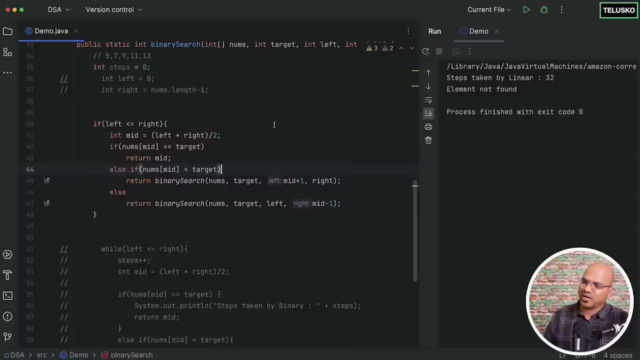 Let's see if this works. Let's restart- I mean rerun- and it says not found because, yeah, of course it's not found, because we don't have that value. But yeah, this is a code for the binary search with the help of recursive. 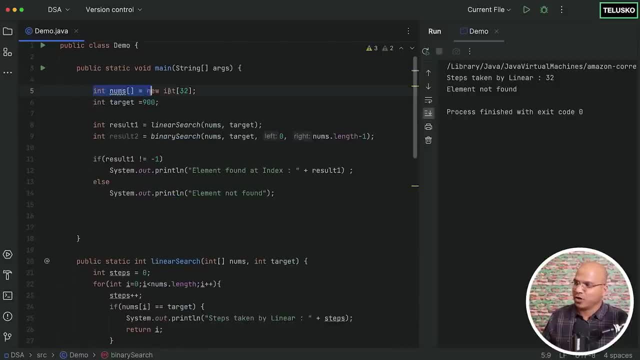 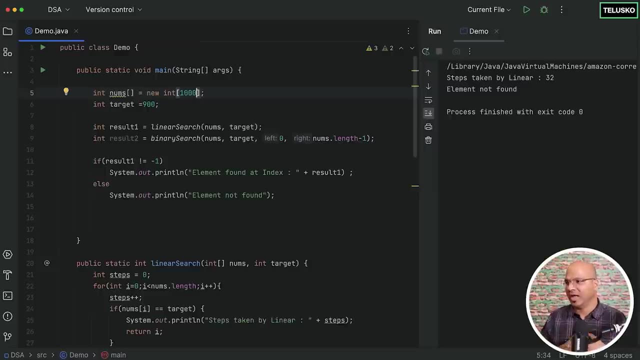 Now there's one more thing you can try with different examples of what you can do is you can take an array of thousand values and add random values. So in Java we have this random class. You can add the values and see how much time it takes. 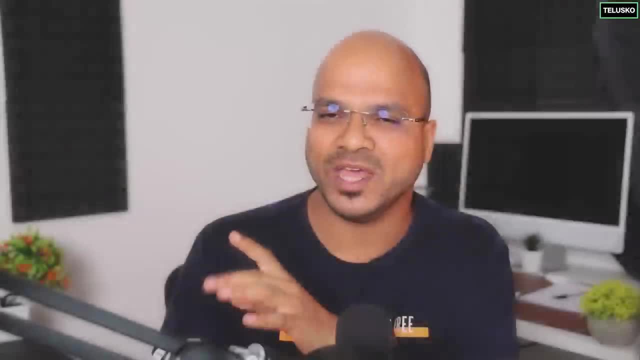 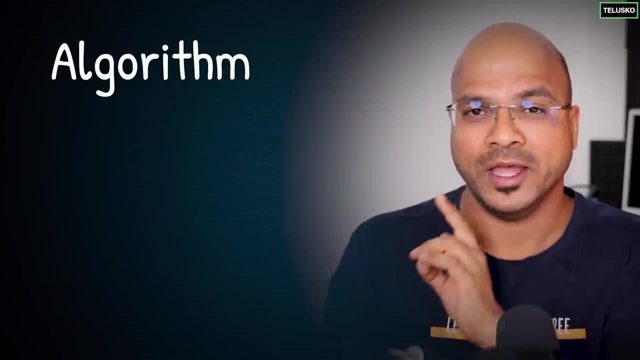 In this video we'll talk about the sorting techniques Now. basically, we have talked about the big O notation, right, And now we know that if you want to judge the algorithm which you are writing, you have to make sure that you are. 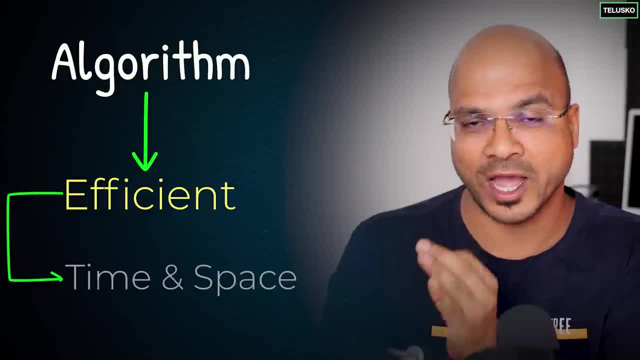 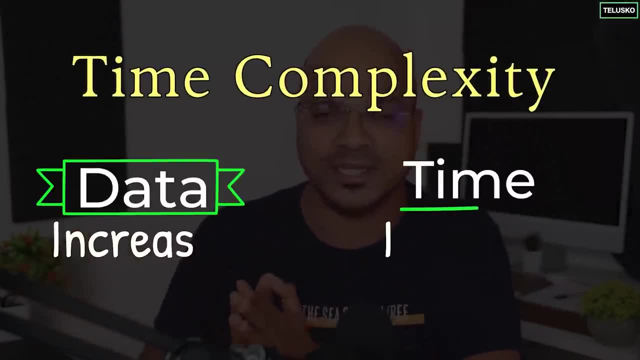 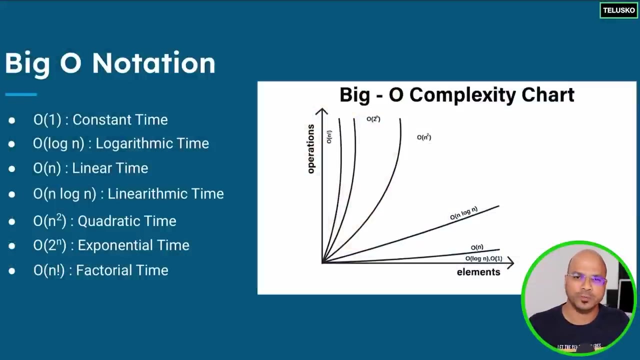 are using an algorithm which is efficient in terms of time and space as well. We are focusing more on the time complexity, where, as your data increases, it should not increase your time exponentially. So we have seen different levels of time complexity and we want to be into that lower zone. 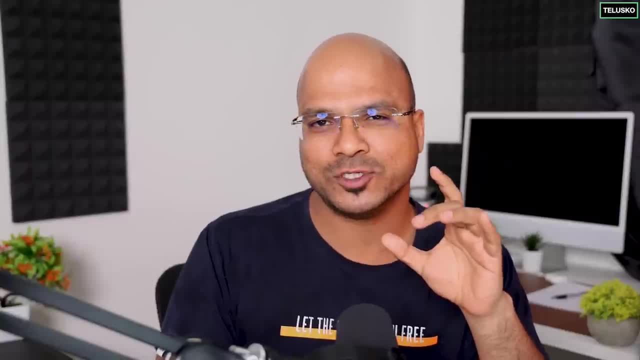 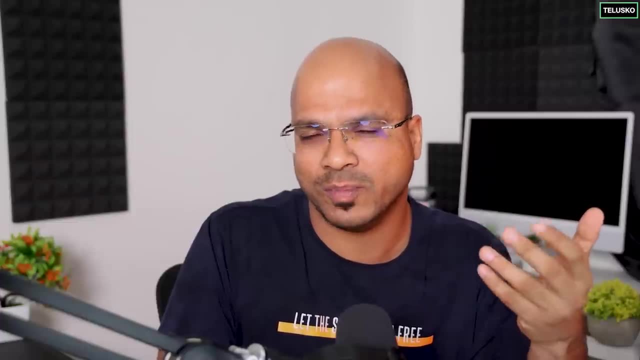 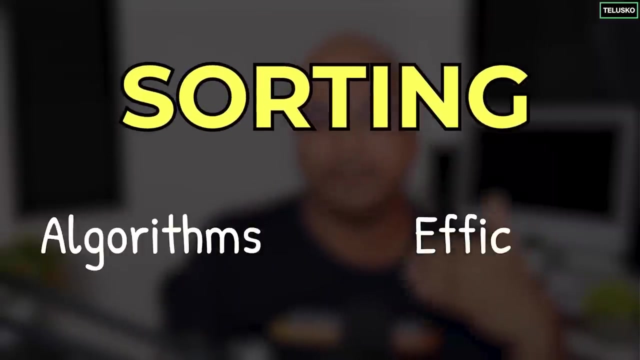 not on the upper zone right Now when it comes to understanding different algorithms. we have to go for some inbuilt algorithms, right? Or some old algorithm which normally we use, so sorting. So we have talked about searching. Sorting is one of the way you can learn more about algorithms and how do you make it more efficient. 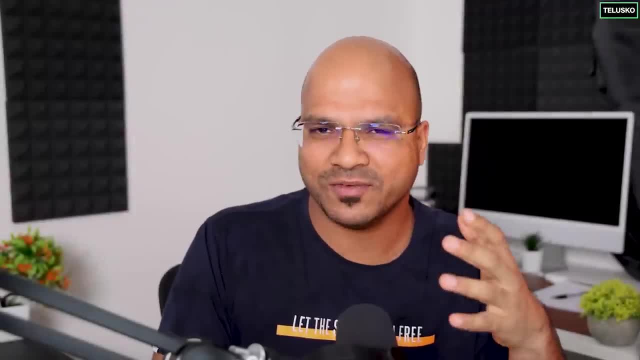 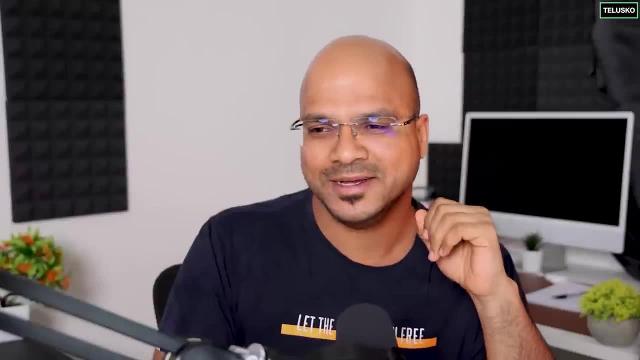 Also in the real world we do use sorting a lot. So let's say, when you, when you say you want to search something on the internet, or maybe you want, you want to buy something on the Amazon, you do that, uh. 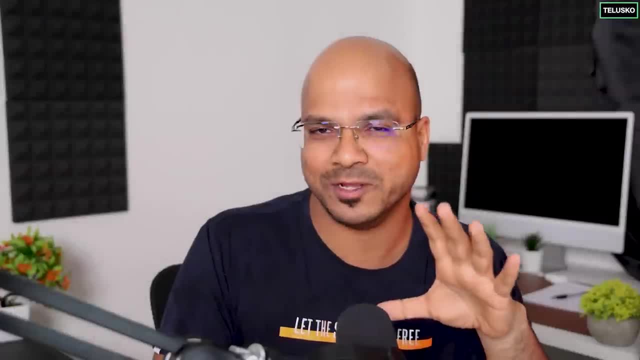 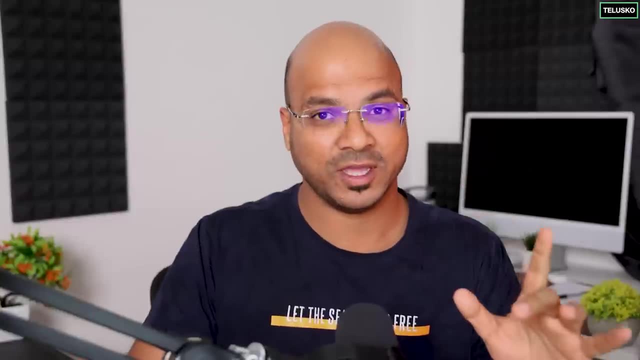 sort by price, sort by reviews- right, So you do that multiple times. So sorting is majorly used. So there are a lot of different sorting techniques available, So we'll try to understand them. Not everything or not every algorithm. 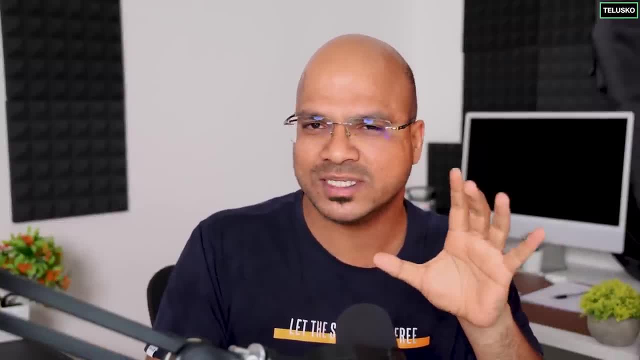 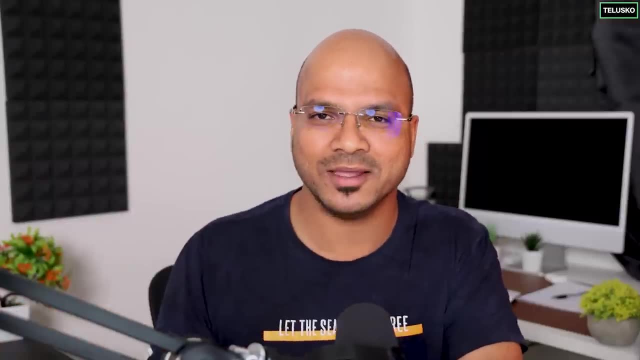 but let's try to understand few of them. Now, if we talk about these algorithms, some algorithms are easy or simple to understand, but they are not time efficient. And then there are some algorithms which are good in terms of time, So they are time efficient. 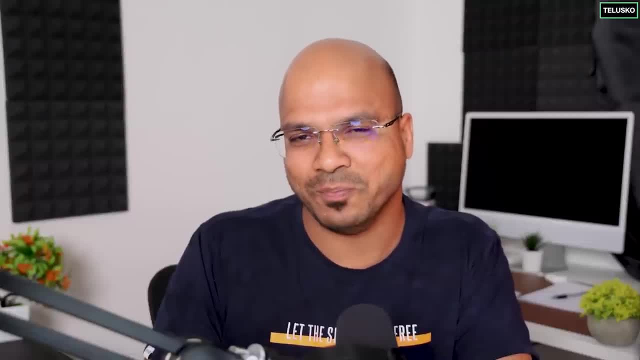 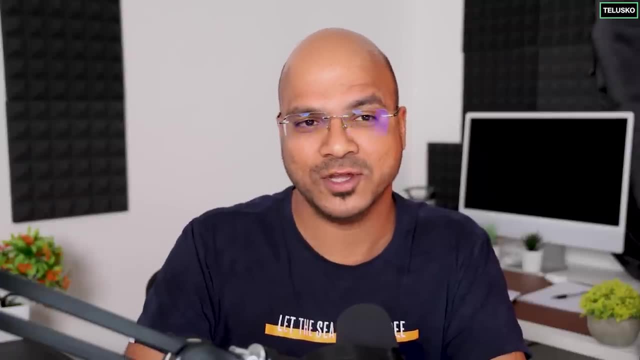 but they're not simple to understand. Okay, Uh, so we have to do a trade off here now which is the best one. that depends if you have less number of elements And if you're learning for the education purpose or to understand how sorting works. 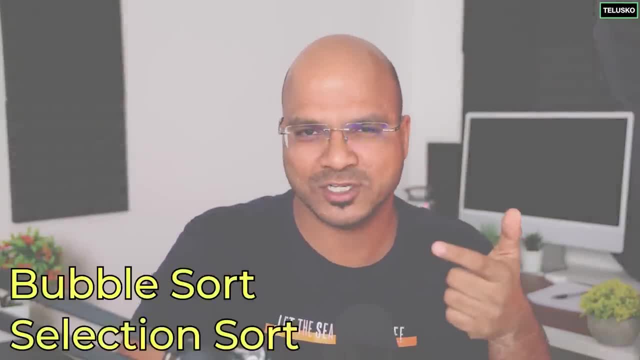 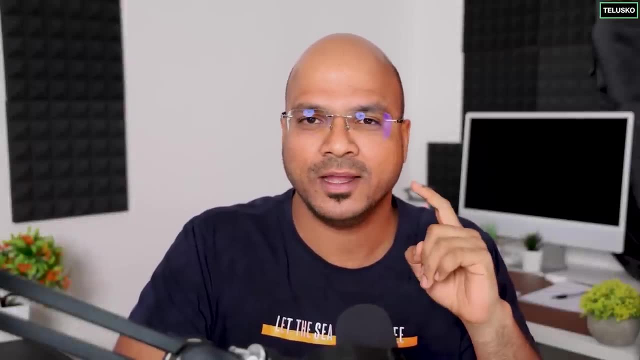 then we can talk about those, those algorithms like bubble, sort, selection, sort. And then there are some algorithms which are bit difficult and they are very efficient when you have huge amount of data, Now what I'm talking about. So, when you talk about sorting, 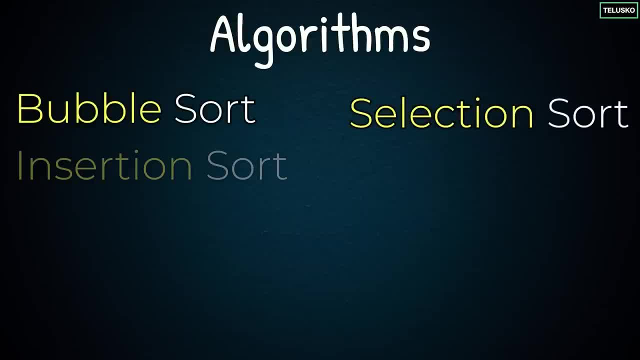 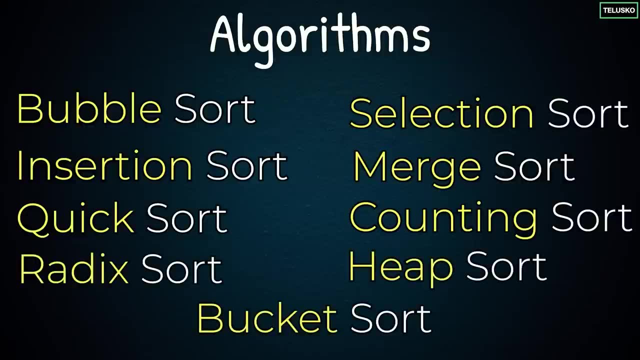 there are different options available. So we have bubble sort, selection sort, interesting sort, a merge sort, quick sort, counting sort, uh relics, uh heap sort, bucket sort, And there are multiple sorting techniques. The famous one are bubble sort. 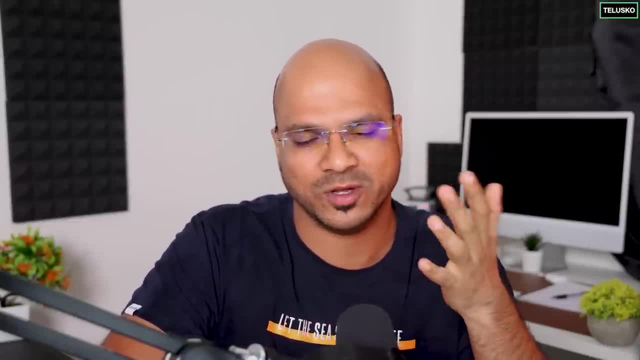 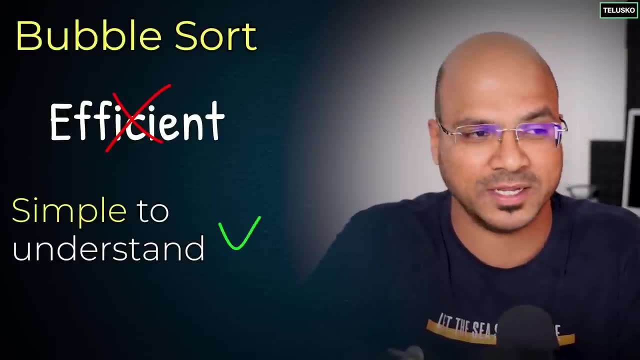 quick sort: selection, sort insertion and then merge sort, If I'm not repeated that multiple times. So let's start with the first one, which is bubble sort. Now, bubble sort is not efficient, but it is simple to understand. So that gives us a starting point. 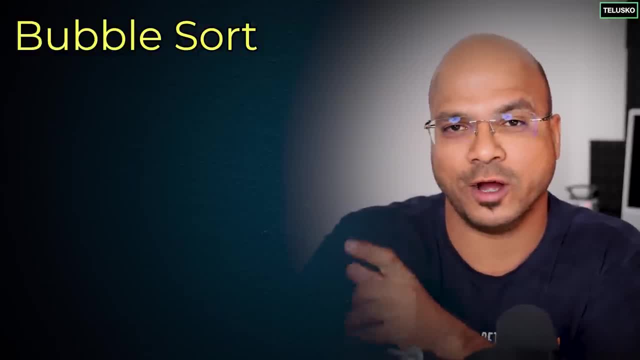 When we talk about the bubble sort, why do we use it? So let's say: if you want to sort different elements, so let's say: we have this list in front of you. The numbers are eight, six, nine, two, four. 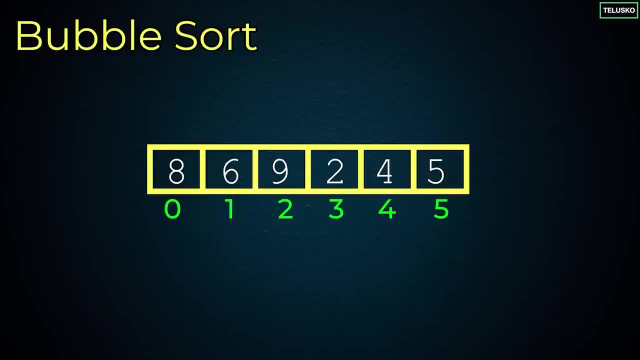 five. Now, if you want to basically sort them, how will you do it? Now, of course, we don't have a magical way where you can find: Hey, this is the first one, This is the second one. So what you do is you basically? 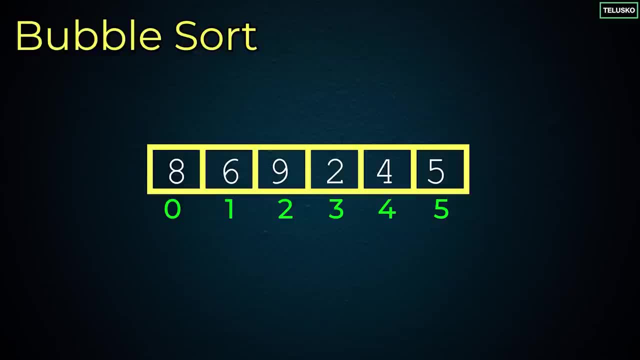 try to use some algorithm like bubble sort to sort it in this. What you do is you basically create a bubble. Now what exactly this bubble is? take one element, put that into bubble and shift it to the end. Okay, Now that sounds weird. 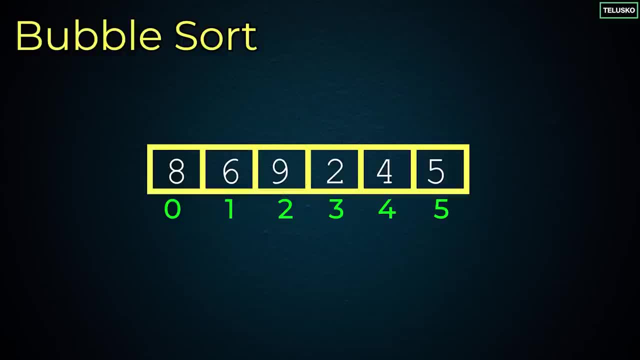 right. So let's, let's do step by step. Now, when you have this value, let's say you have six value in front of you- you can put them in an array like this, and then you have provided the index values. 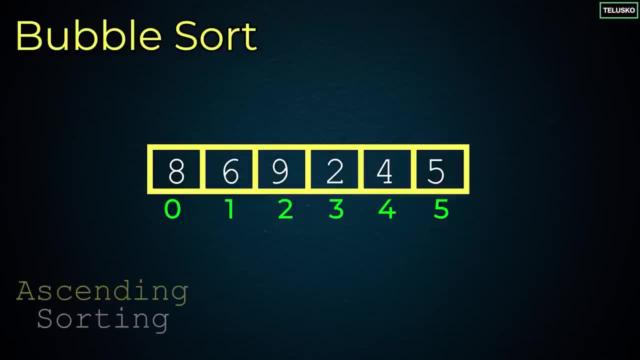 Now, if you want to do this sorting on this, of course we want a ascending sorting here. So basically we want to at the start, then four, then five, then six, then eight and then nine. That's a sequence we want. 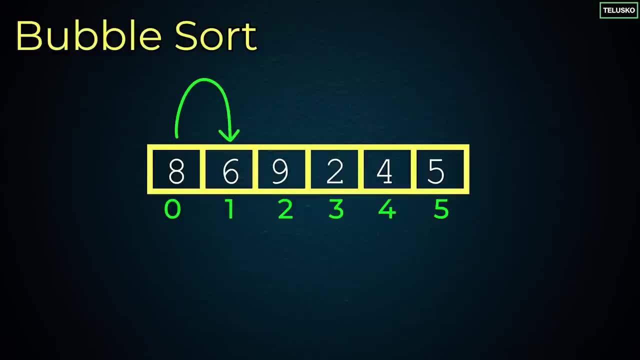 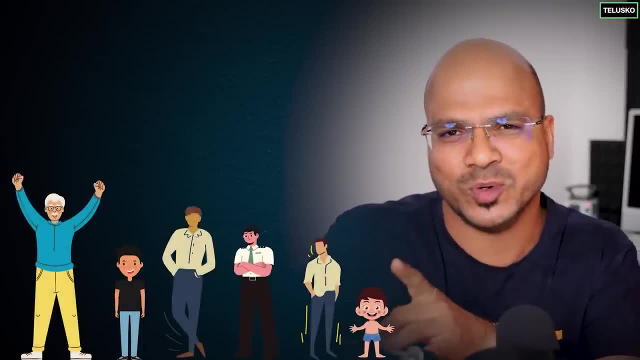 but how will you get it? So what you do is you compare two values at a time. So let's say, if you put six people in front of you and they want to sort them according to their height, So what you do, of course you will come back to people at a time. 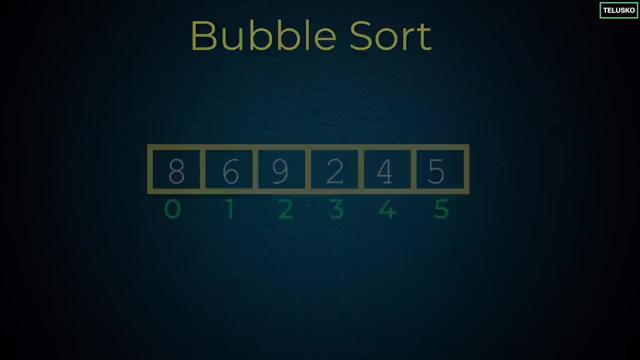 right, That's how you saw it, And then you will try to swap them. So how exactly it works. So let's say we have this: two values here, eight and six, And then what you do is you want to make sure that. 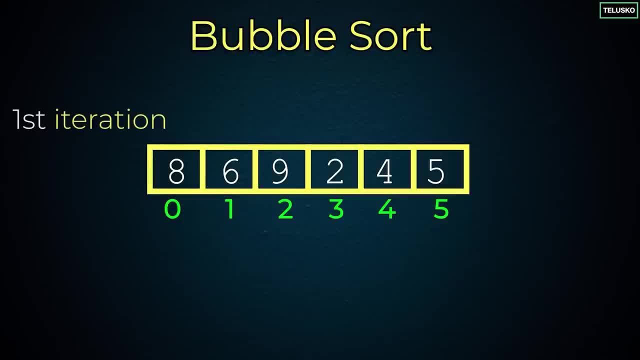 the biggest element from this particular or add a in the first iteration goes to the end. Okay, So the way you do that is: first you compare the first two values. Now, these are the first two values When you're comparing it. 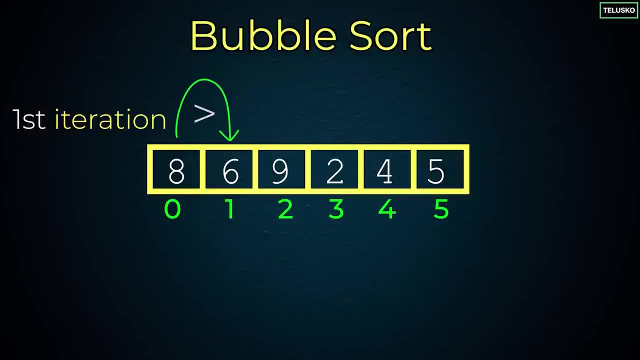 if the first value is greater than the second value, you basically need to swap. Okay, Swapping is very important here, So you have to first compare the first two values. If the first value is greater than the second value, then you have to swap. 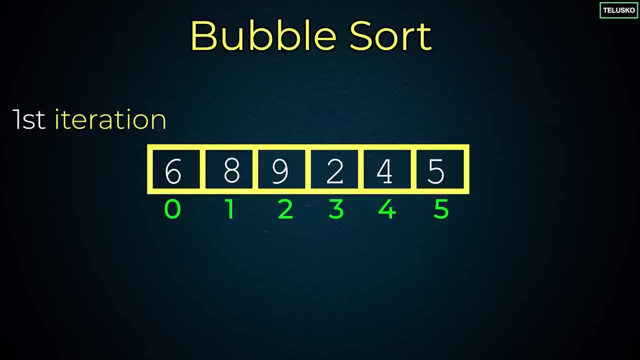 And then you basically shift your pointer to the next two values. Okay, Done, We are done with the six. Now let's go for the next two. The next two is eight and nine If the First value is greater than the second value. 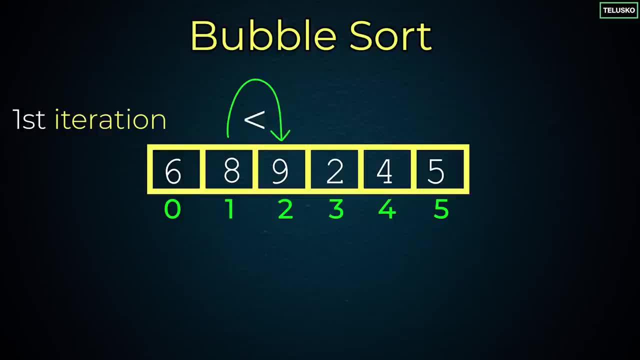 You have to swap. in this case They are not. they are. So the first value is less than the second value. So what you do is you simply say skip, because there's no swapping needed. Then you go for the next two values. 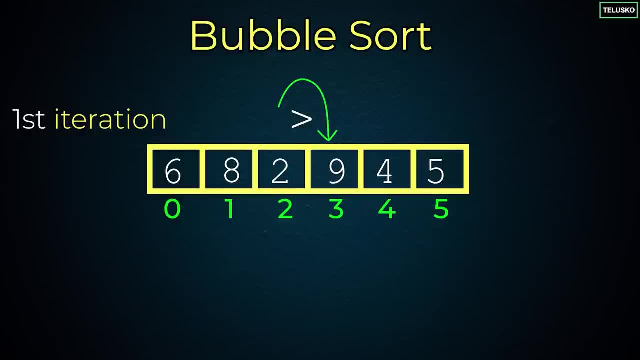 The first value is written, the second value. So of course we have to swap. And then again you shift your values next to values. Again you will compare: the first one is greater than second. swap. Then again you will compare the next two value. 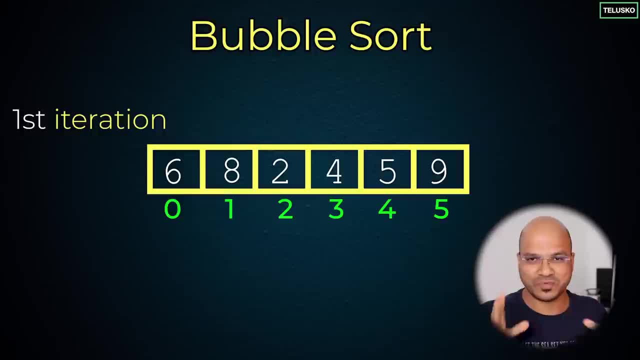 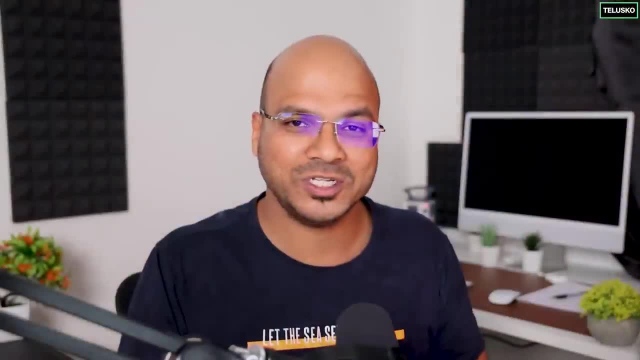 The first value is written, the second swap. So basically, after the first iteration, you got the biggest value at the end, but is it sorted? Unfortunately not. You have to do this operation one more time, Actually, not one more time, multiple times till you get this sorted. 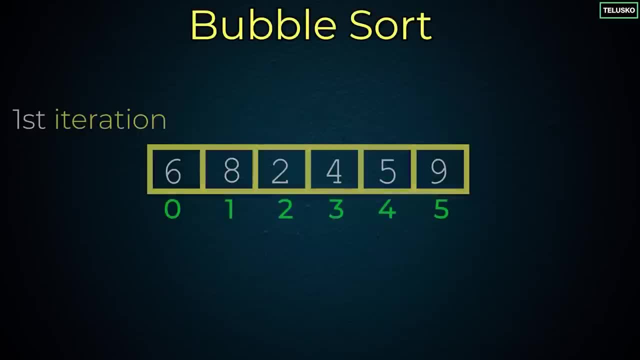 Now, this also depends upon the size of your elements or array. Now, in this case, uh, the first five values are still unsorted. The last one is done, So we don't have to touch the last element. So in the first iteration, 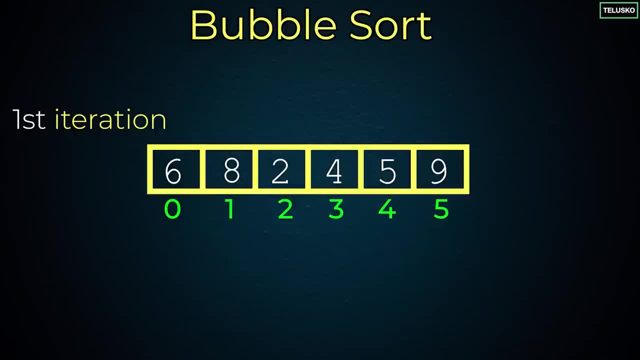 if you're going for six times the second iteration, you can go for five times The third iteration: you can go for five times The third iteration: you can go for five times. You can go for four times. So let's see how that works. 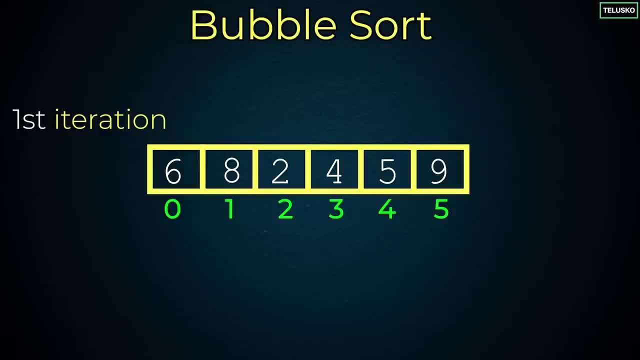 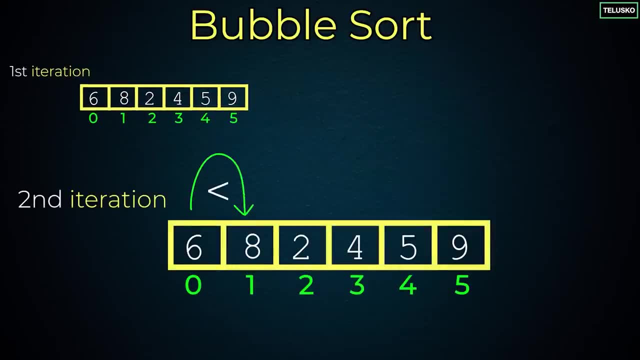 Now, after the first iteration, we got the nine value at the end. Now what you do is again: you repeat the same steps. Compare the first two values. Is it required to swap In this case? No, we can skip it. 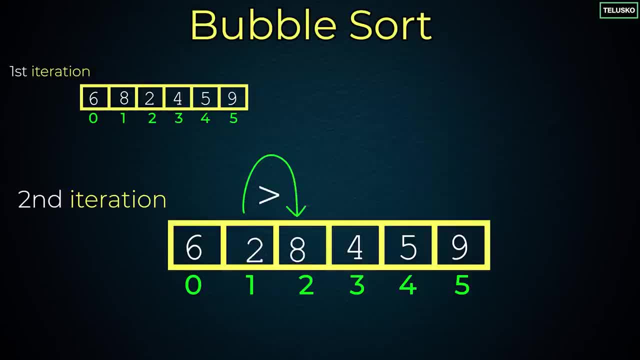 Next two values: is the first value greater than the second value? Yes, Swap it Then again. you go for this. next two values is get eight greater than four. Yes, Swap it. is then again next two values: eight greater than five. 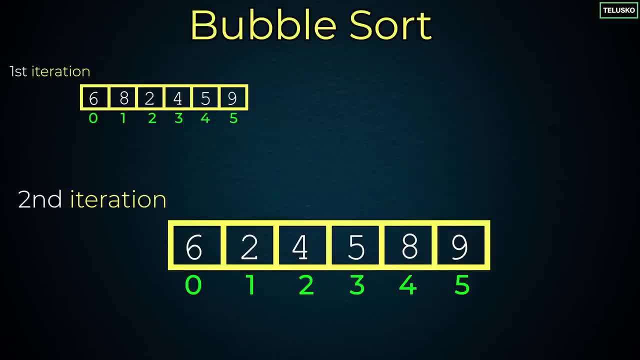 Yes, Swap it. Now, in this case, what happened is, after the two iterations, you got the two biggest values, which is eight and nine. at the end. Now we know that those two values are sorted, but what about other values? Those are not sorted. 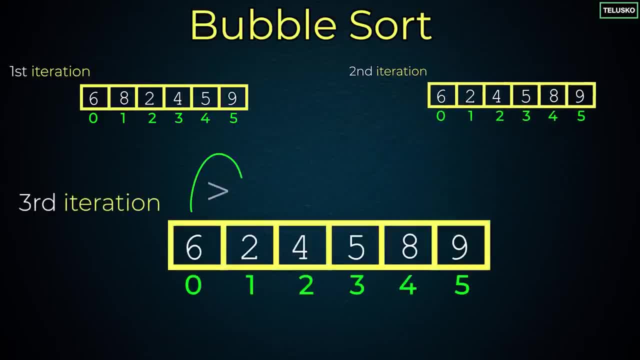 So let's sort them again. You have to repeat the same steps. So you have to say six, two, which is six, is written into again. we have to swap it six and four. greater than six is getting in for swap it six and five again. 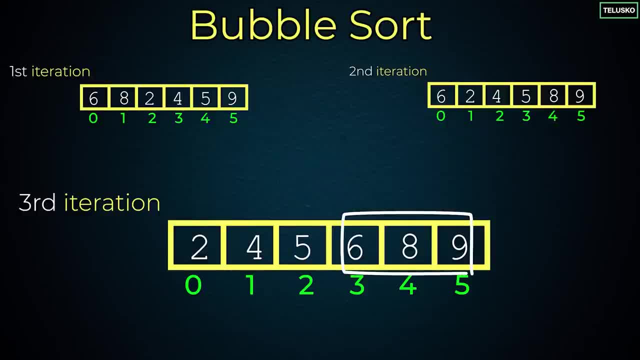 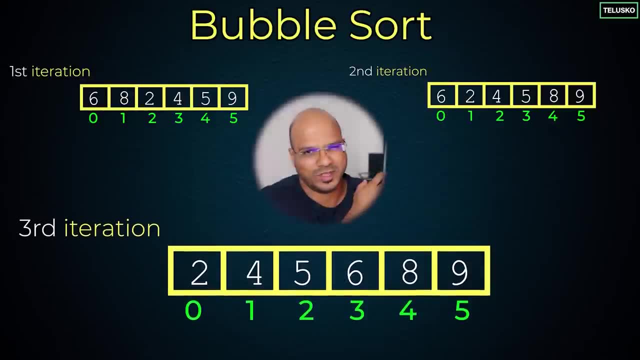 swap it. So now, after the situation, you've got three values: six, eight, nine, which is sorted, But what about the other values? They're still unsorted. I mean, we know they're sorted now, but your algorithm has no idea if they're sorted. 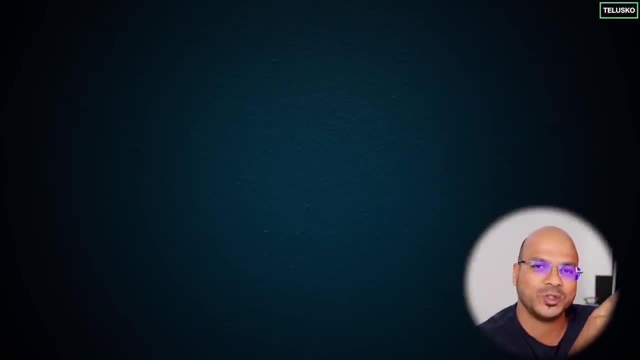 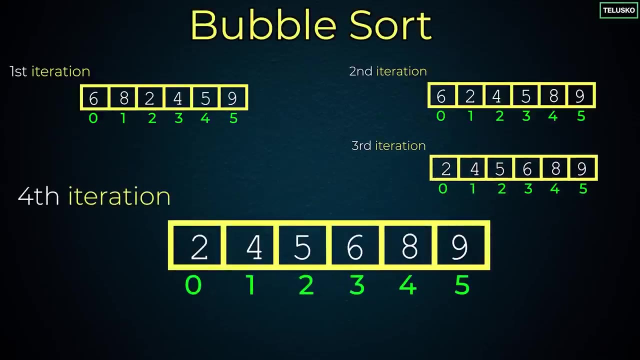 Okay. Now this is tricky is because your algorithm goes from start to end. Okay, It will not check for do the other values are sorted or not? So it will keep doing that. So it will compare the first two values, not swap. 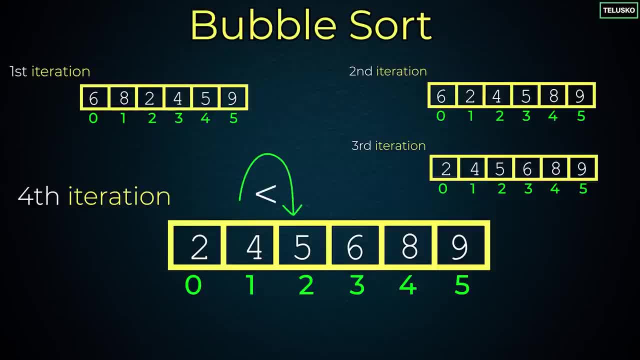 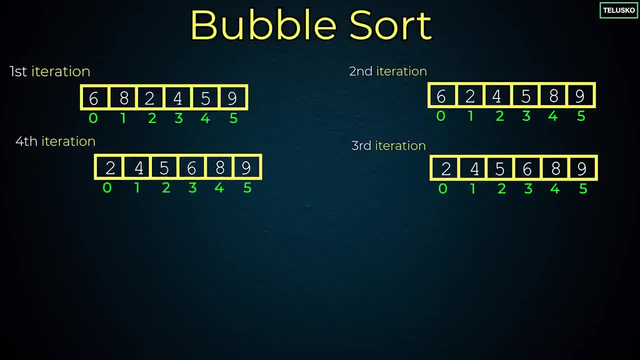 not needed. next to values swap not needed done. We are also confirmed. five: Still there's a confusion for two and four. Your algorithm has no idea. Those two are already sorted, but still it will try to sort them. It will compare the two values. 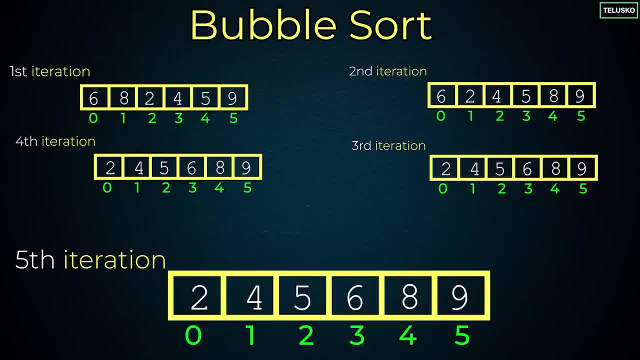 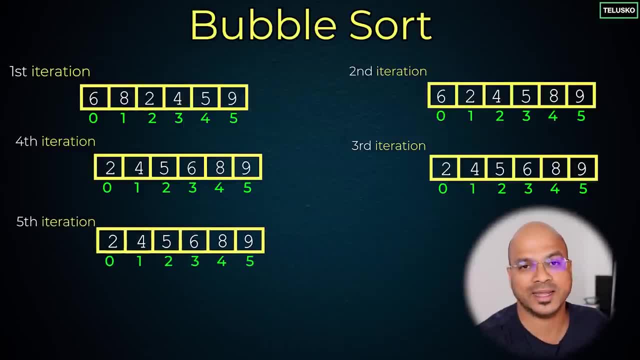 They are compared, swapping not needed. So by doing that, four is confirmed And you, since you only have one element, now that itself is sorted, And by doing this you got the entire solid daddy. So, yes, even if you, it is sorted. 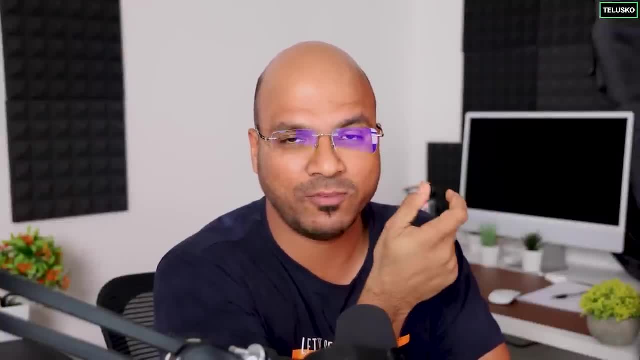 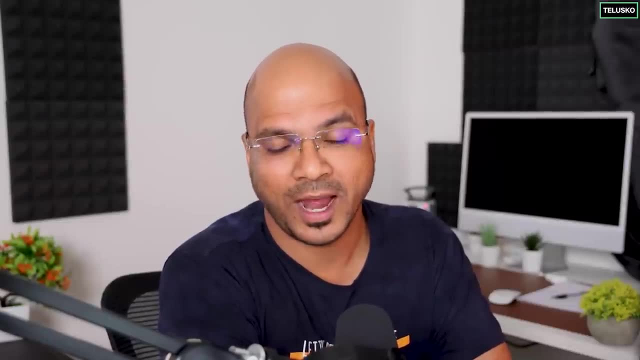 it will still check. We are reducing one step, which is swapping, but still you are checking, And that's why bubble sort is not an efficient algorithm, And the problem is the the time complexity for this is all off and square, because you have to use two loops. 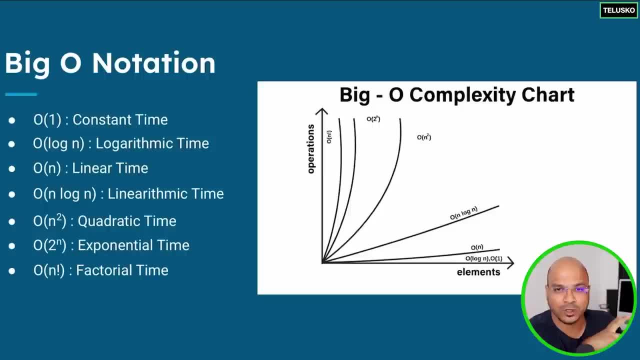 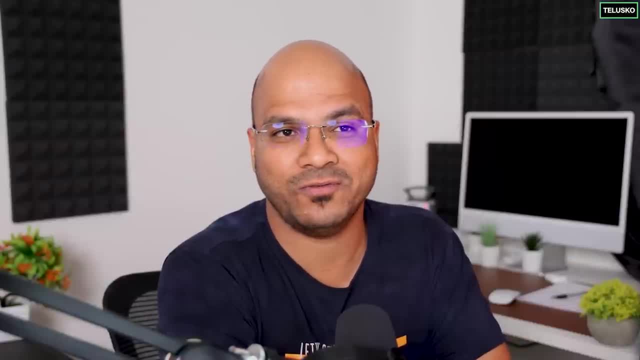 one for the iterations and the inner loop. for each iteration you have to compare the values. So that's your N square. not a good way of sorting the elements. Now think about six elements. So that's good. Six square is not a big number. 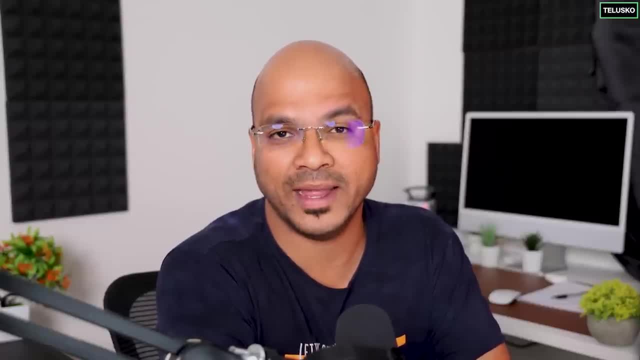 It is actually. but what about if you have a very big array or very big list? let's say 20 values, 30 values. imagine the number of steps it will take. So not an efficient algorithm, but easy to understand. Now it's time to convert this into a code. 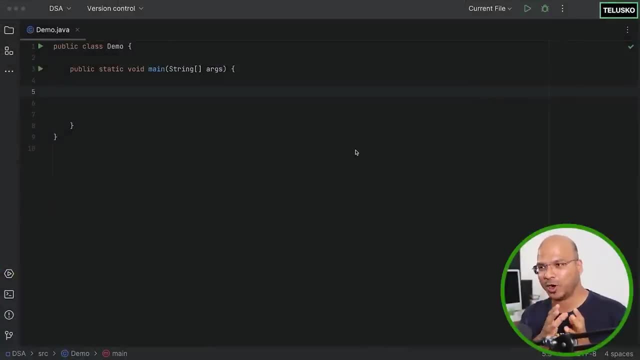 Okay, Now let's try to implement the concept of bubble sort in the code. So we are going to use Java as a language. So if you, if you want to sort, of course you have to store the value somewhere first. So what I will do is I will create an array of integers. 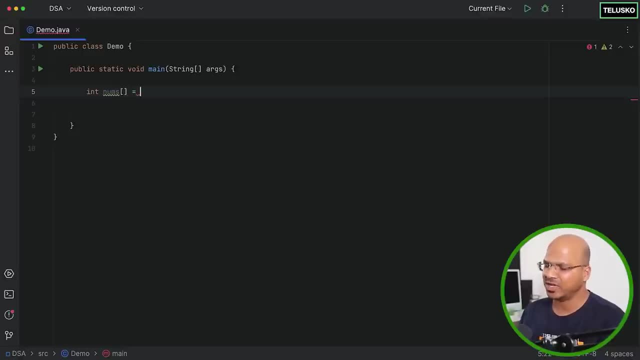 and let me just name this as nums, And then I will assign some values. Of course I can go for this new array and then assign the value one by one, or we can give them the static values. So here, let's say we go with values. 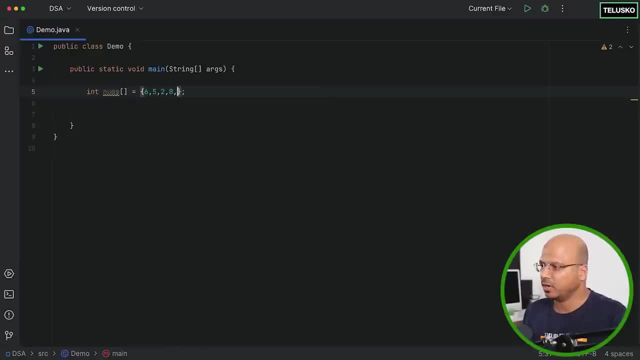 six comma five comma two comma eight comma nine comma four- I don't remember the sequence in the previous video which we talked about, a theory, but let's go with this. values and I want to sort them, Okay. So what I will do is, even before sorting: 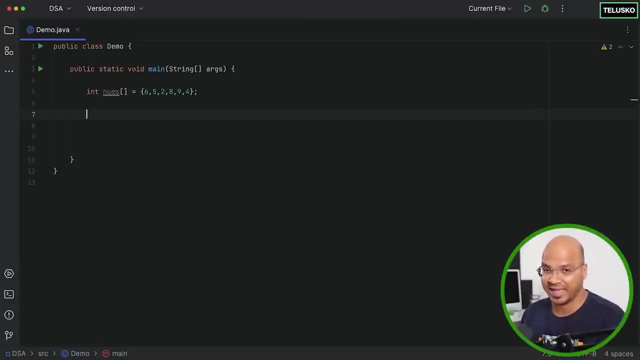 let me print all the values. The way you can print the values of an array in Java is you. of course you can use a normal loop or we can use enhance for loop. So let me just use an answer for loop here. So I will say: for ain't num in nums. 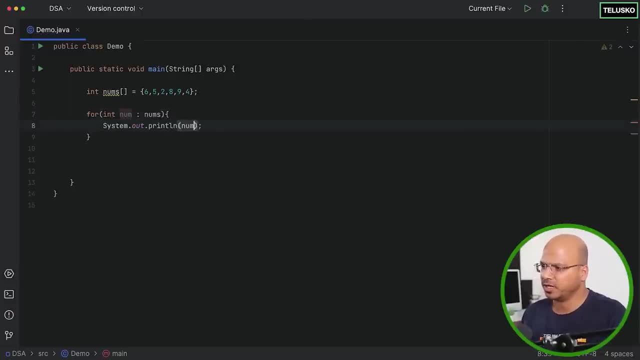 and then you can print the values right. So I'm printing num here. So I will say this is before sorting and then I will. I will do the same thing, I will execute the same code, but after sorting here. So let's say this is after sorting. 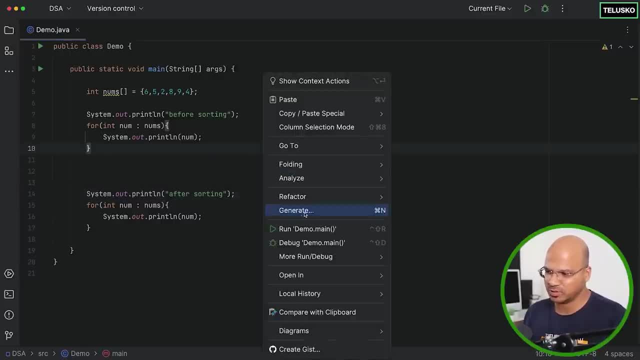 Okay, Now, if I run this code, of course you will get the same value two times. So if I- and one more thing, I will not be- I want to print this on the same line, because Ellen will print on a new line. 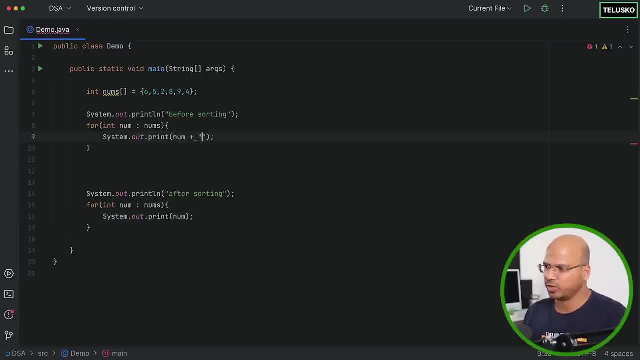 I don't want it And maybe, maybe, after every printing I want to give some space as well to differentiate the values, And let me do that here as well, so that it will. it will print on the same line with spaces right, Like here, and said one. 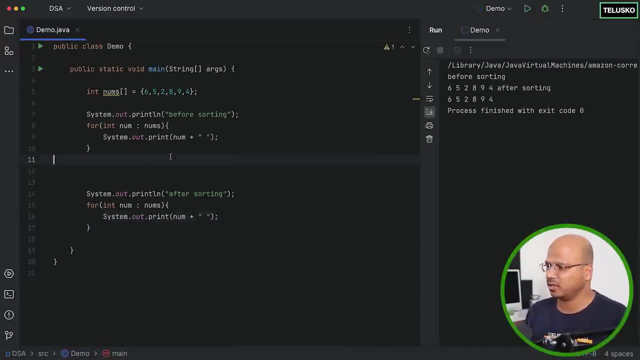 And you can see we got before sorting, after sorting. I think this should be printed on a new line, So what I can do is, just before this I would say it's out and run. Okay, So this is before sorting and this is after sorting. 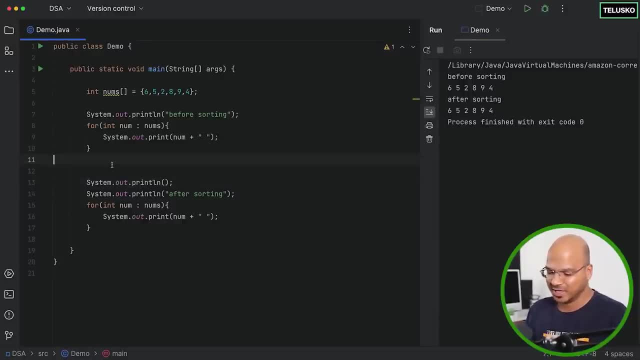 at this point is not getting sorted, Of course. right, We have not written any logic. Yeah, Now this is where, in between, you have to write the logic for sorting. Now in bubble sort. what you do is you compare the values to value at. 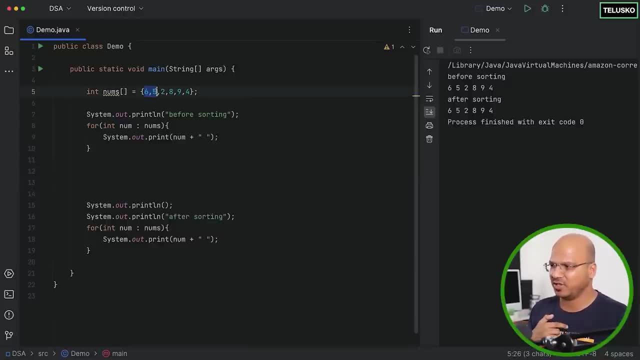 a time and then you swap. So you compare this to values. If the first one is greater than second one, just swap. And then likewise you will do for all the elements. Now for sure, if you want to move to the iterations. 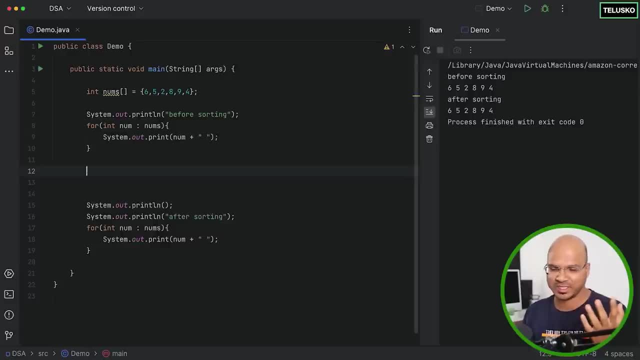 now we have to do two loops here. The nested loop, basically the outer loop, is responsible for the number of iterations or the number of passes, And the inner loop is actually responsible for swapping. So what I mean by that is: I need a first. 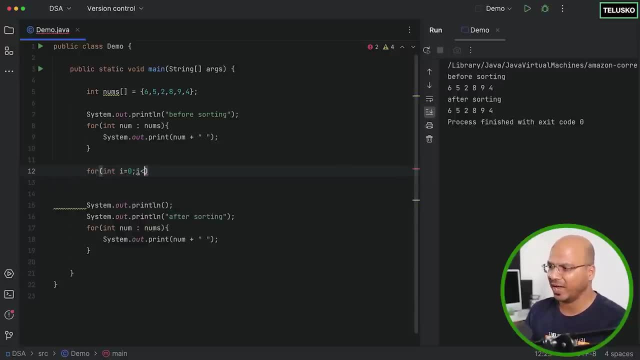 variable. I will start from zero. and where are we going to end it? So of course I can end it at less than six. So you can say six or you can say nums dot length. Okay, So basically we can use the added length. 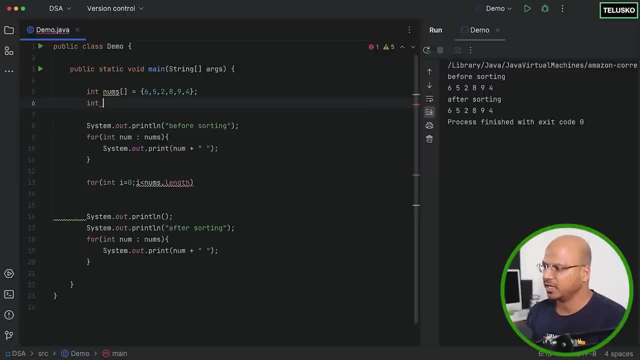 You know, the better way would be to store this value somewhere So I can say size, nums, dot, length. So I'm just storing that value in a variable called size. It will be easier to work with. So I will simply say: say size. 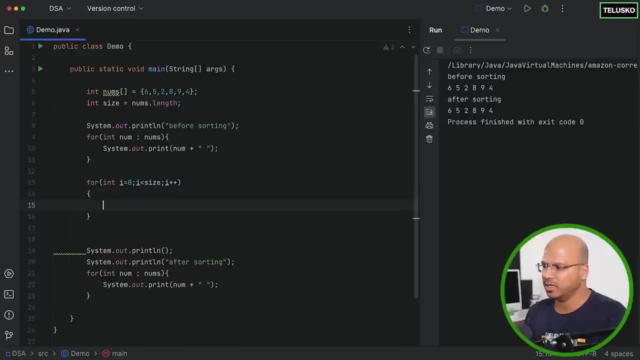 and then I will say I plus plus. So it will go from a start to end. So this is only for passing right. We have to do this multiple times. You have seen that in the animations. but now let's do the inner loop. 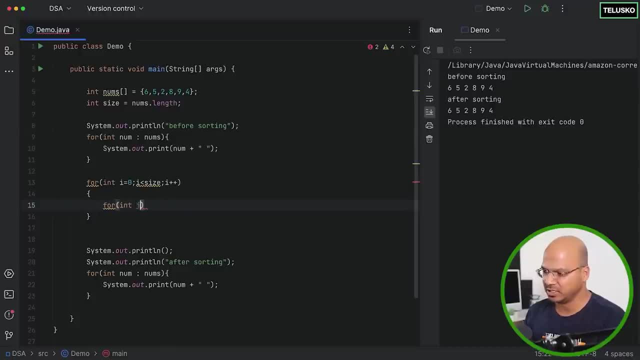 which will do the actual swapping. So here I will say: int J is equal to zero, because I'm going to start from zero. The real question is: where are we going to end it? at this point I will say size and let's see what happens if we do. 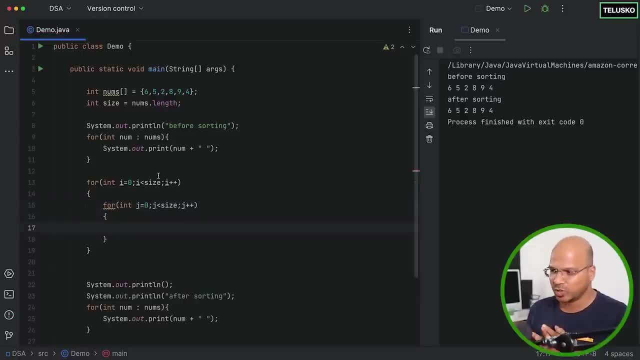 the do with size. Okay, So both the loop, the outer loop and the inner loop, are starting from zero And ending at size, the size of the array, And now we have to basically compare two values. Now, how will you compare two values and how do we? 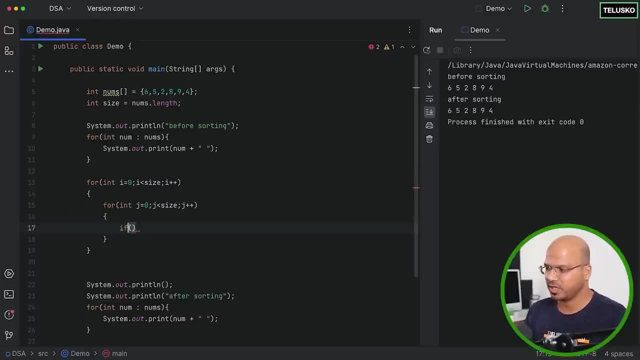 even swap them. So it will check if the first value- Now how do you know the first value? So nums of six or nums of zero? basically, six is nums of zero, So nums of zero compared with nums of one. That's how you compare. 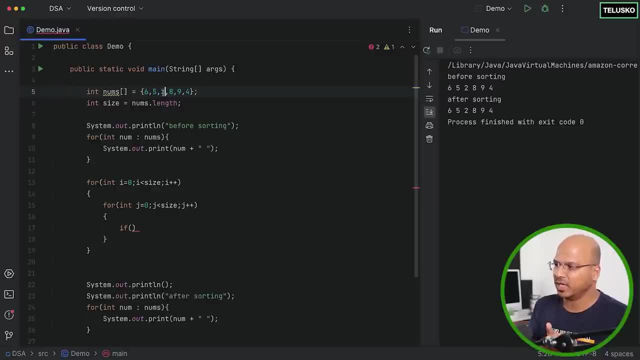 Again, you can compare nums of one with nums of two, then nums of two with nums of three, then nums of three with nums of two, Then nums of three with nums of four. That means the current number when you say zero one. 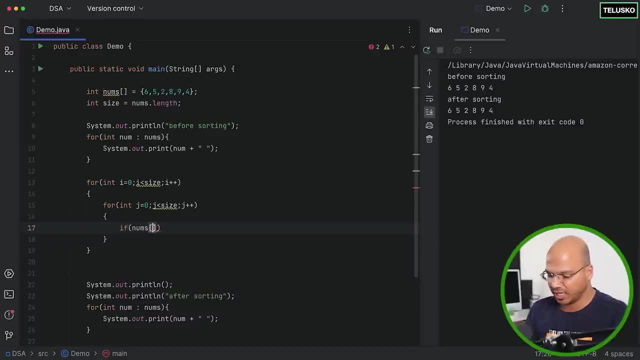 two: it is represented by J, So I can say nums of J, but this will be compared with the next value. And how do I know the next value, which is your nums of J plus one? as simple as that. So we are comparing two values. 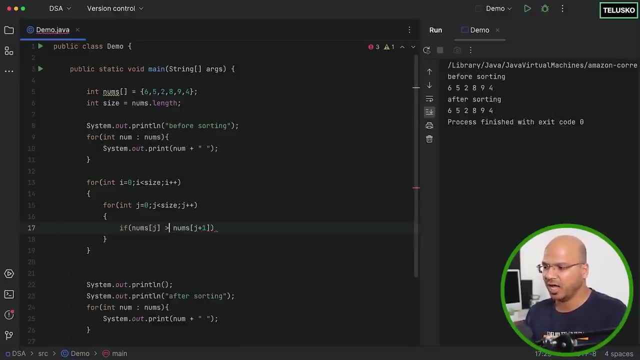 Now how we are comparing them, which operator we are going to use here. So we are going to use greater than. if the first value is greater than the second value, then you have to swap. simple technique right Now. how do you? 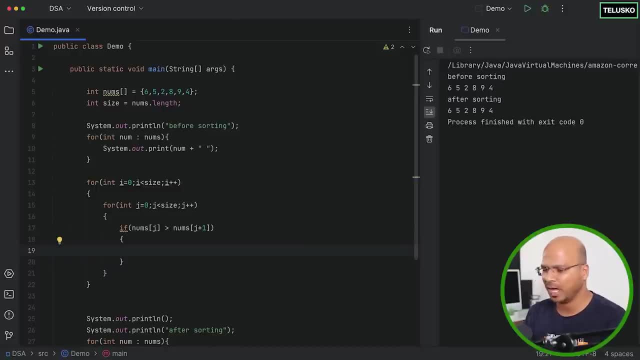 Swap that different ways of which you can swap the values. I'm going to use a traditional way. Let me use a temp variable. In fact, you can also declare a template temp variable here, So I can say int, and it's better to have all the 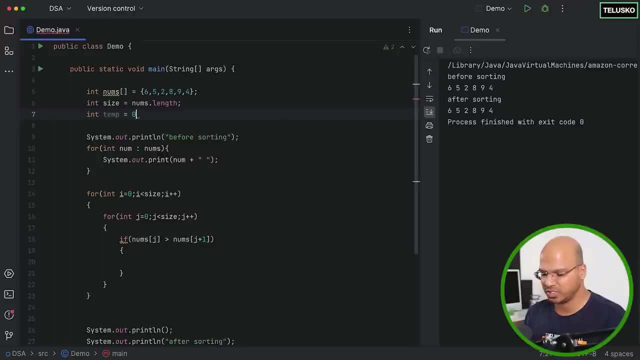 variables on top. So we'll say int temp equal to zero initially, and then, using the third variable, I can simply swap them So I can say temp is equal to nums of J And then nums of J is equal to nums of. 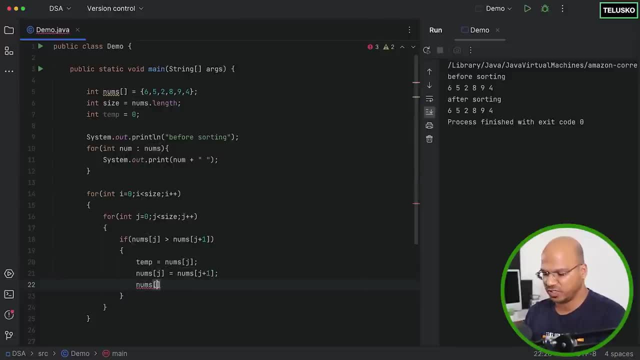 J plus one, And then nums of J plus one is equal to temp. So, basically, what we're doing is, with this, three lines, we are just swapping them. nothing complex, just swapping the two values. Okay, And that's what we have done here. 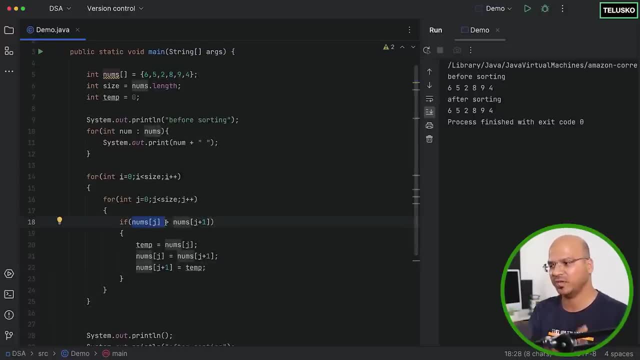 So every time you find this- the first value greater than the second value- just swap them, And you do this multiple times because we are keeping this in a loop and that's it. The sorting is done. Uh, since it will be happening multiple times, 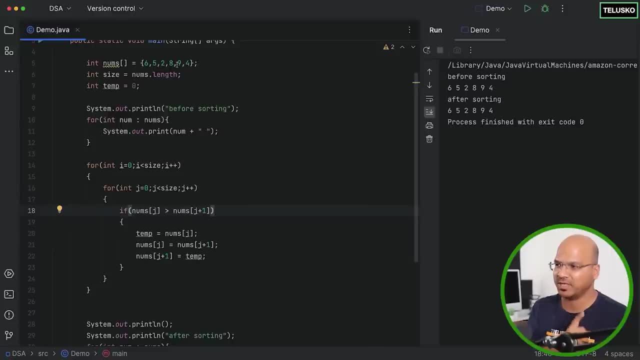 it will make sure that You keep the values at the end, the bigger value at the end after each iteration. So if you run this, okay, we got an error. It says out of bound. Now there's one problem here. 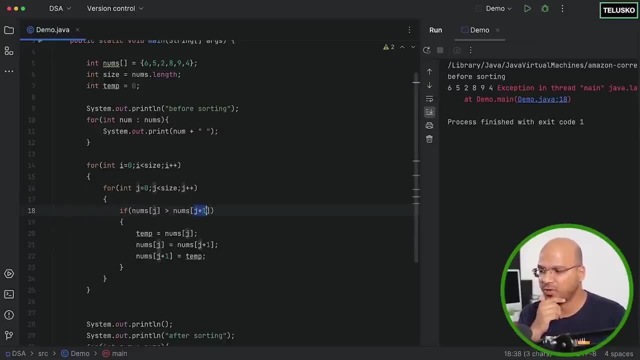 Don't you think, when we are going for J plus one, what about the last value? So we need to make sure that we don't go to the last value. So it should end minus one, right? Uh, because when you're comparing the last two values, 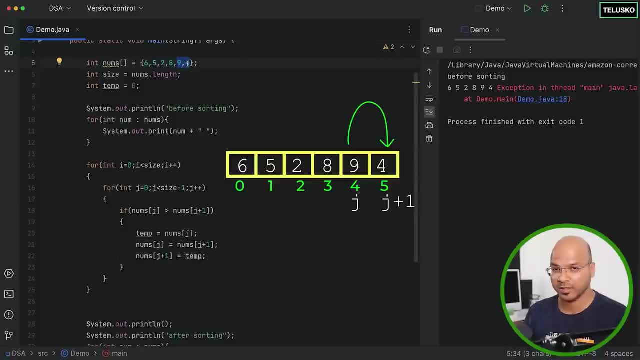 the value for J will be here and this will be J plus one, So we have to make sure that Your J ends before the last value. That was the error and run And you can see sorting done and you've got the sorted values. 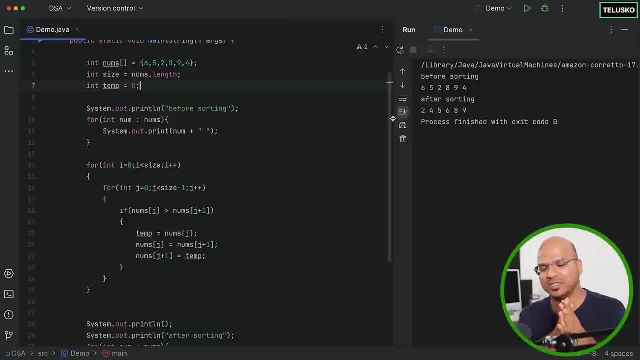 This is, this is how, basically, you sort them. again, We have seen this explanation, the theory, how things are working out, but here we just try to sort it with the help of this logic. Now, there's one problem here. Uh, every time you do this in the animation. 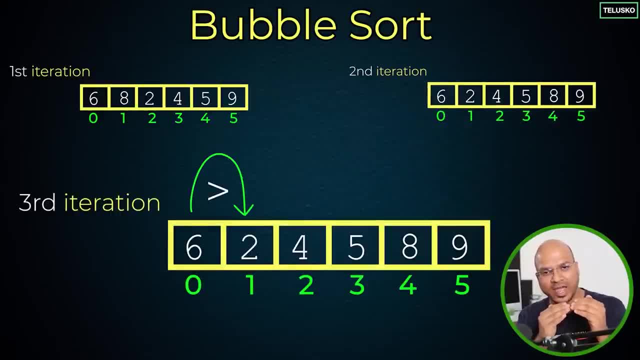 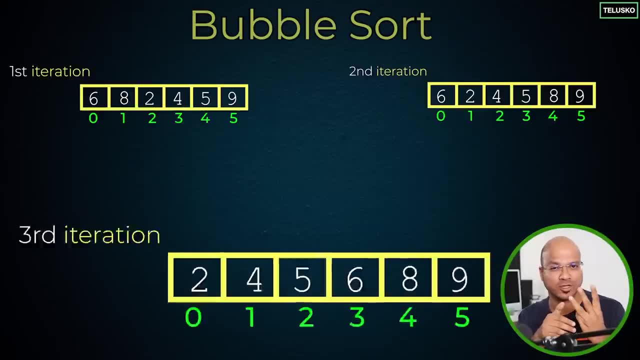 if you remember every after every pass, we don't have to go for all the values, because the last value is sorted In the next Pass. two values are sorted in the next pass. Three values are sorted, so we don't have to sort them again or even check. 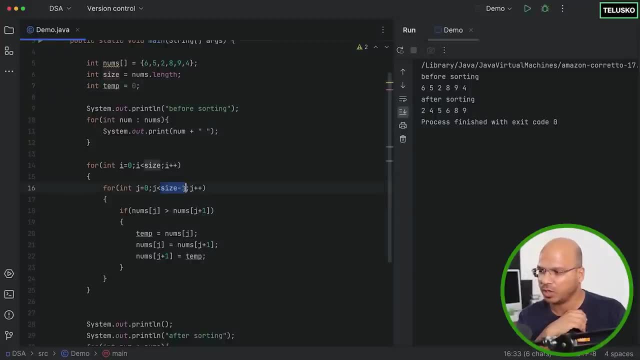 them again. So here J should be not going to size minus one. In fact it should go size minus I minus one is because after every iteration- So let's say we have the first situation where I is zero- it will go to the second. 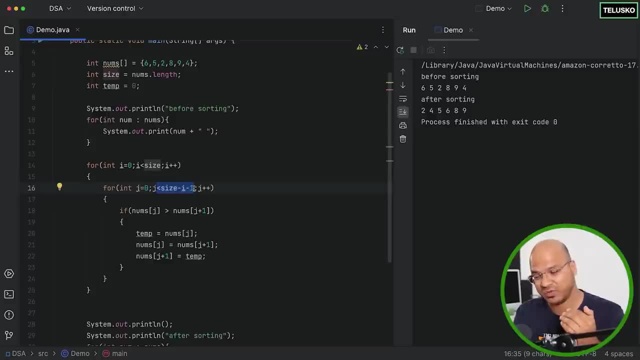 well, second last value, because we are saying minus one in the second iteration, where the I value will be one, it will go till the second last position or third last position, because the last one is sorted. You don't have to check that again. 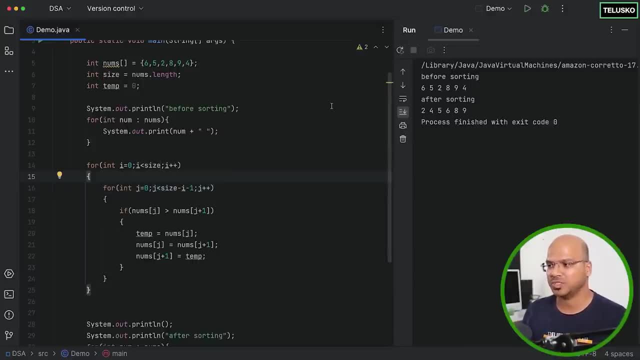 It will not affect the output, but it will affect the speed, because we are saving some time by not checking the same sorted value again and again. Okay, That's how you basically you do it. In fact, if you want, what we can also do is we can print this in: 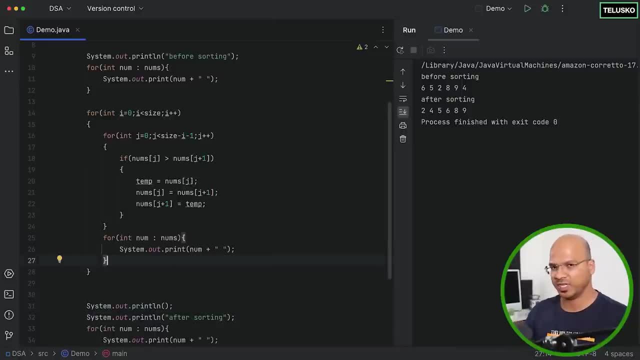 every iteration. So I can just copy this And after every iteration of the outer loop we can print the values and see what is happening there, right? So in fact I will also print a new line here so that it will come on. 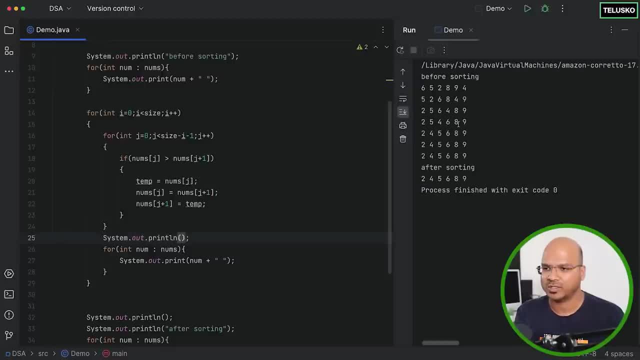 New line. Let's run this. So this, this is what basically is happening. Initially you have this value and then this is where the sorting starts. If you can see, after the first iteration, the biggest value nine just went till the end. 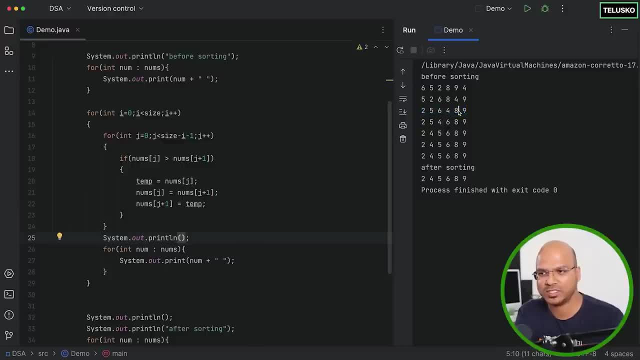 Then after the next, for the next iteration the biggest value, which is eight, is at the end or second biggest value. third iteration: we got three values sorted. for the iteration We got four values sorted. fifth iteration: We got four values sorted or five values sorted. 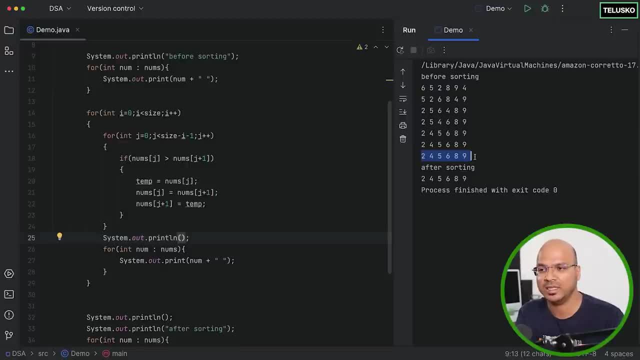 And last last iteration, we got all the value sorted. So that's how, basically, it does. Of course, here too, we got at the start itself. We don't have to sort them again, but that's how the algorithm works, right. 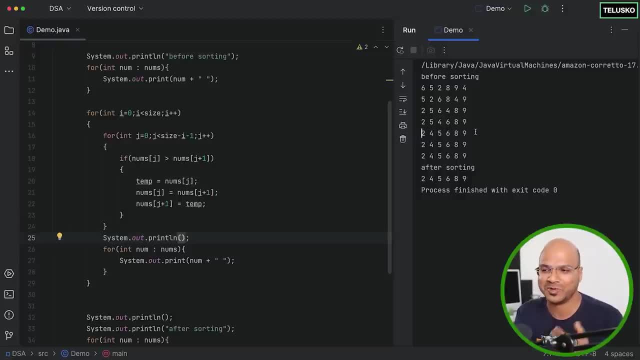 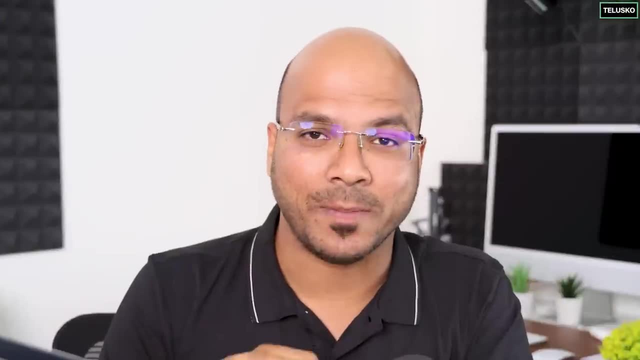 How will you even check if the array is sorted, even before you compare all the values? So that's the thing about the bubble sort, where you compare the values, swap them and you're done. in this video we'll talk about selection sort. So basically we'll talk about the theory in this. 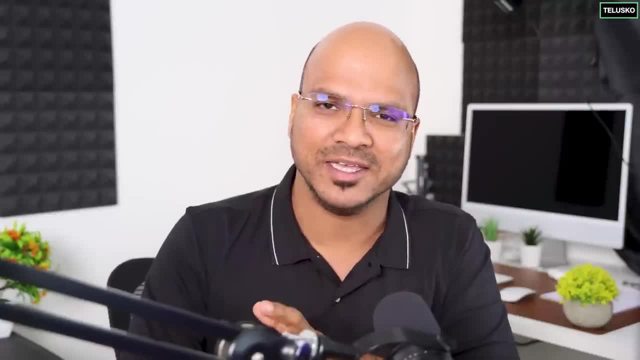 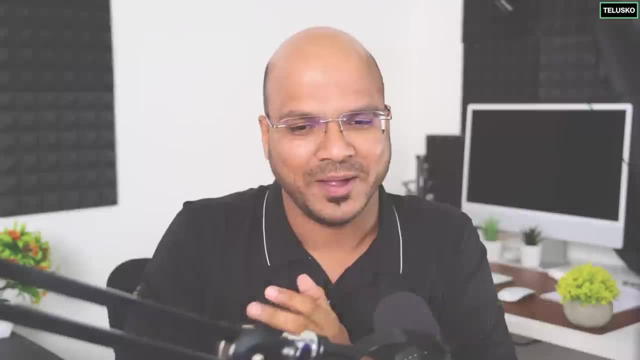 And then in the next video we'll talk about the practical of it. The thing is, when you talk about sorting, we have different techniques Available. in the previous video we have talked about bubble sort and it was working right, But also the amount of time it takes, basically the time. 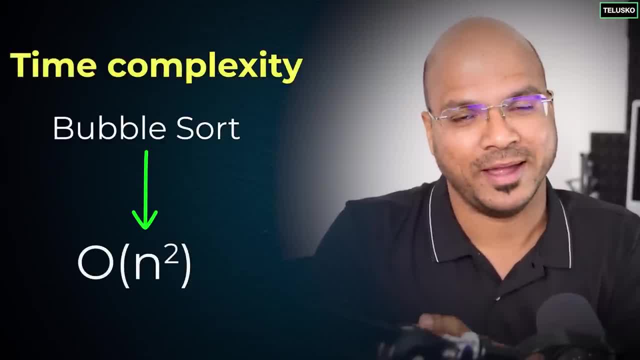 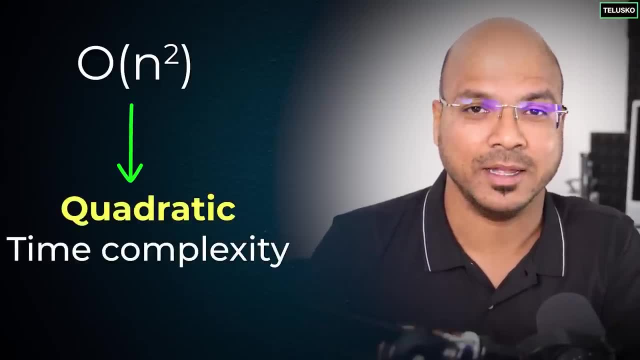 complexity of the bubble sort is N square. Now, that's not the main issue, Of course that's the main issue. But then in this video we are not going to solve that quadratic time complexity, but at least we can reduce the number of steps. 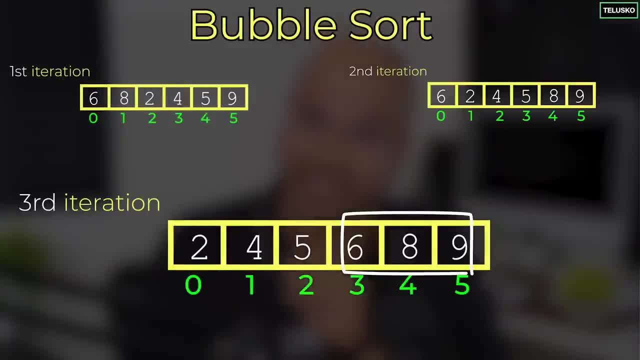 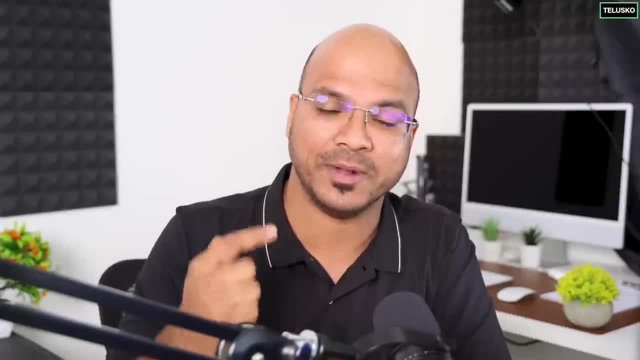 Now in bubble sort, we are going from start to end multiple times. That's not the big issue. The big issue is swapping, because every time in the inner loop we were doing this swapping multiple times and it's consumes a lot of time and memory. 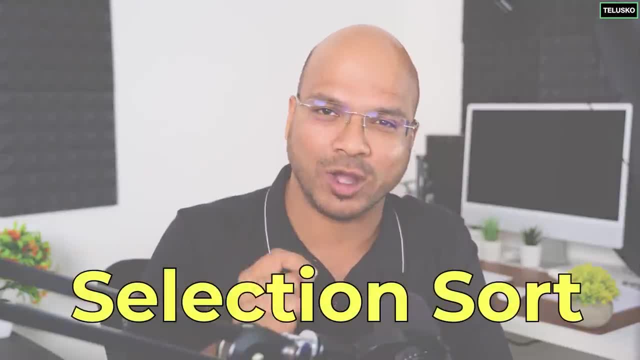 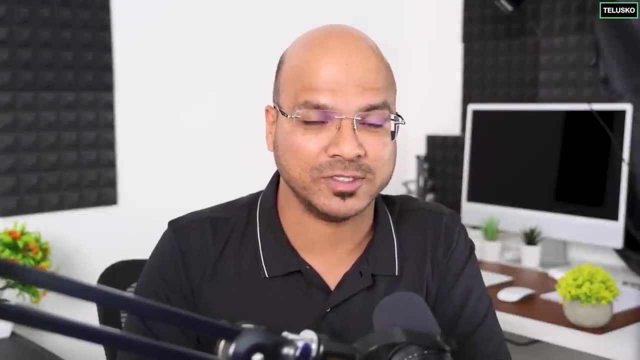 So what if we can reduce that? And that's where selection sort comes into picture. Now, what we do in selection sort is we don't actually swap every time when you compare two values, but what you do is from the entire array, or at least you'll find the minimum or the maximum value. 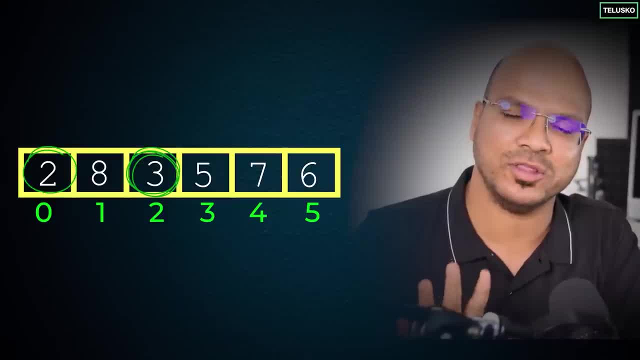 depending upon how you want to implement it. So let's say: we got, we are going for the minimum value. So what you do is, from the entire array, you, you find the minimum value and then you make sure that the minimum value stays at the start. 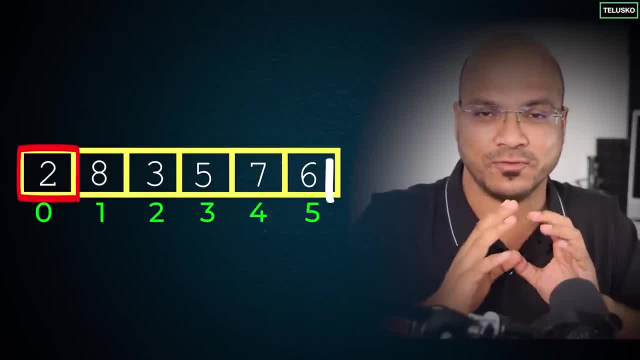 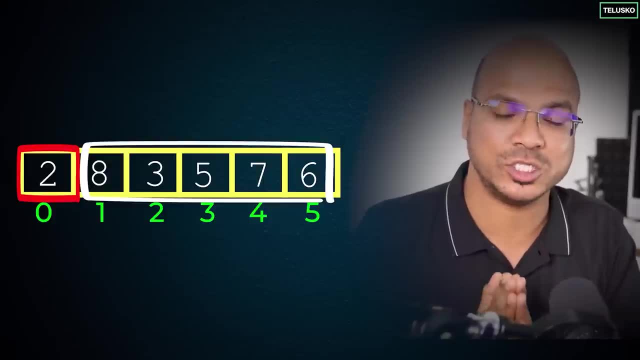 Now, once that is done, now that is your sorted part. So from the entire list you create two sections: the sorted section and the unsorted section. So once you find two, that goes into the sorted section, which is at the start. 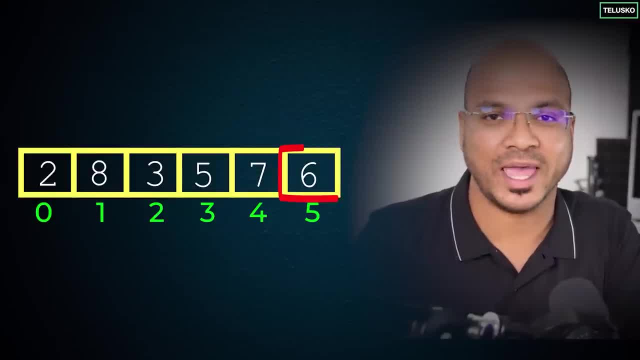 and then you scan more values. Now, let's say, when you scan you find Hey, the, we have three, which is the minimum value in the unsorted data. Then what you do is you pick up that three and replace it with the second location. 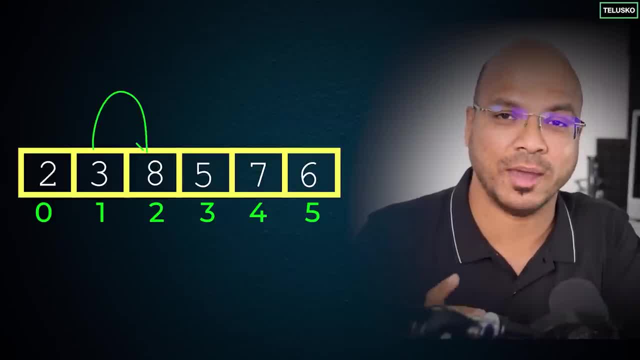 Now what happens to the value of the second location? Now, that will be swapped where the value of three was. So what you're doing here is you are swapping by selecting the minimum value. So when you say selecting, that's your selection sort Now. 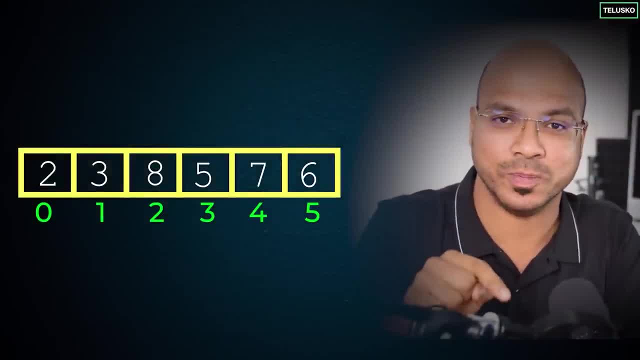 what it does is you're not basically swapping value inside the inner loop. You are doing that in the outer loop, which means the number of swapping in a code will reduce. Now to understand this more, let's look at an example. So let's say we have six values here. 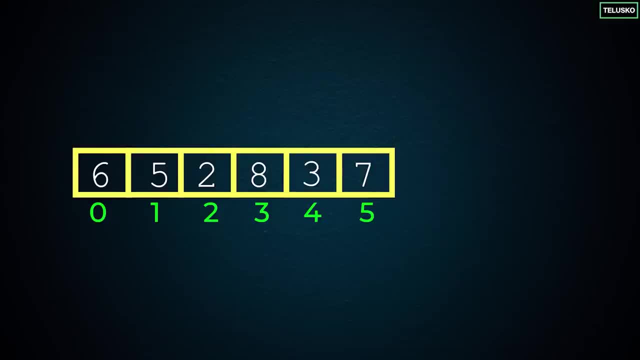 which is six, five, two, eight, three, seven, and we want to sort them. So how would you do it? First of all, going from all the values. now, of course, as I mentioned before, you can go for the minimum value, or you can go. 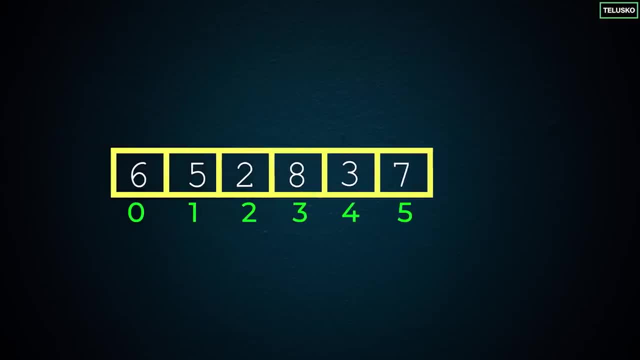 for the maximum value. So let's go for maximum value, Okay, So ultimately you will get the same output, but the way you do do the code will be different. So let's say we are going for the maximum value Now from all these values. 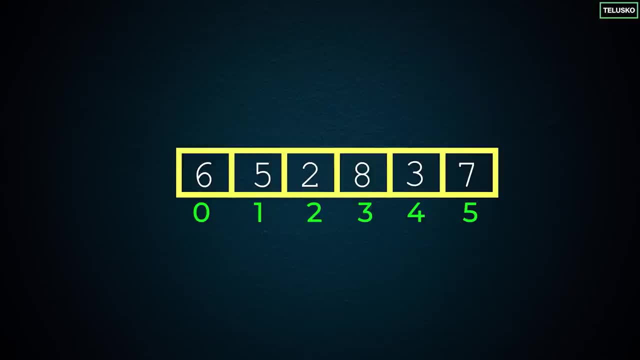 we have to find the maximum value. Now, of course, at the start we don't have any idea which values are maximum. So let's say you make six as the maximum value, Because at this point we don't know right. 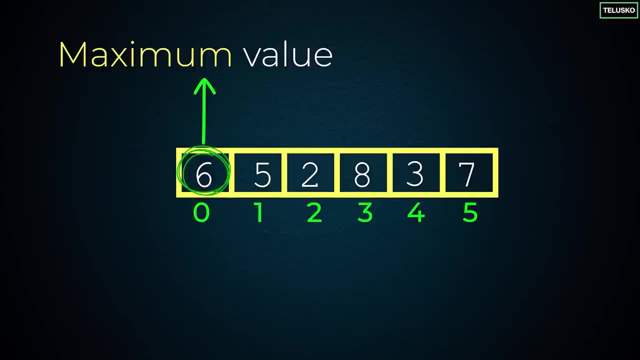 So let's assume that six is the biggest value from the, from all these values, And then you start comparing six with all the other values. So you will compare six with five. If six is still bigger, no issue go with. the next value is six is still bigger. 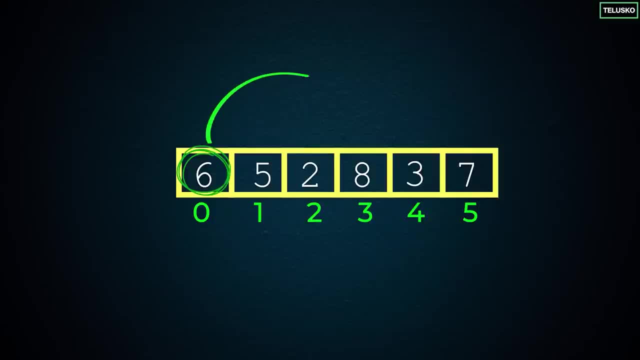 No issue, Go with the next value. Now, at this point, we are comparing six with eight and we know now eight is the biggest value. So now what you do is you change your variable or your change You. you change your biggest value from six to eight. 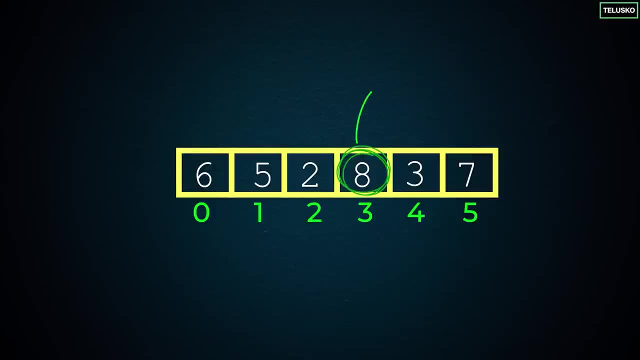 and then you start comparing eight with the other remaining value, which is three and seven. So you compare with three: eight is still the biggest. You compare it with seven, seven, eight is still the biggest. Now, once you go through all the values, 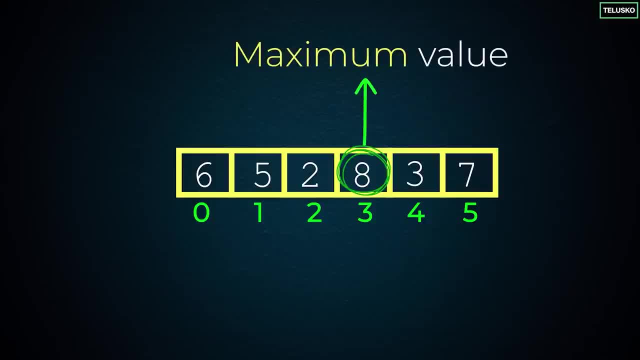 now you know the eight is the biggest value. So what you do is you make sure that eight goes at the end. Now, if you're doing this with for the minimum value, what you do is you take the value two. 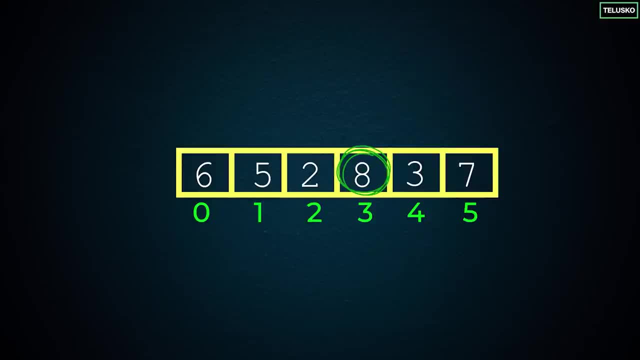 which is a minimum value, and you put that at the start. But since we are going for a different approach, where you're finding the biggest value, you will make sure that eight goes at the end. Now, when you move eight to the end, 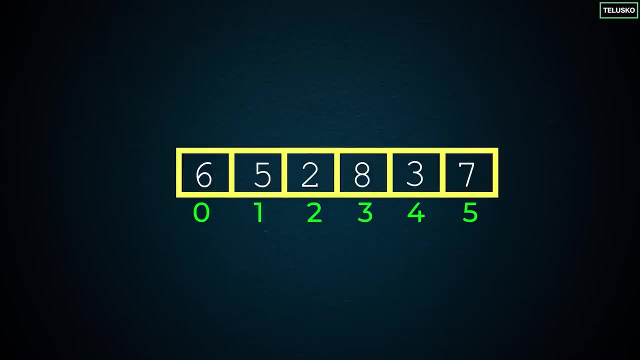 what happens to seven? Now, seven will say, okay, I don't have a place. So eight will say: don't worry, I will come to your place, You come to my place. That is swapping of the values. But if you remember, 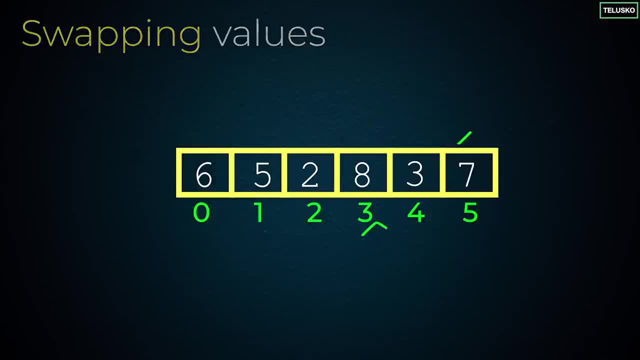 we are not doing it in every iteration of the inner loop, We are doing that in the outer loop. So once you complete one pass, that's where you do the swapping. So only once for the entire iteration. Okay Now, by doing this: 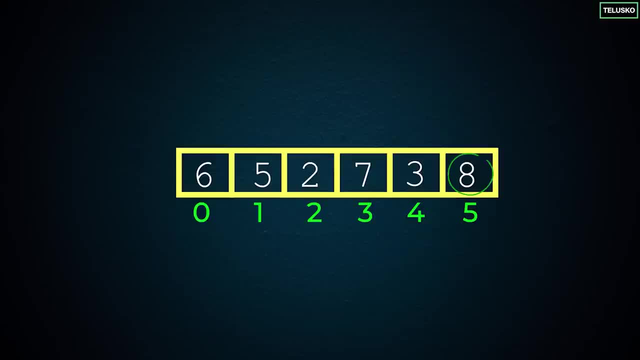 we have made sure that you have the biggest value at the end and you got a sorted at the end, which is the eight, And then the first five values are still unsorted. So what you do is you repeat the steps Again. 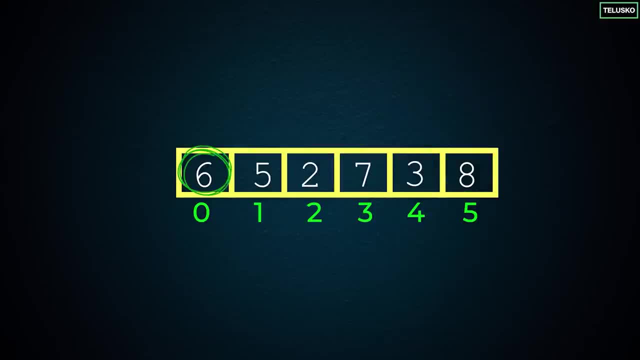 start with six. Now we'll say, okay, six is the biggest value, Let's assume that. And then you start comparing six with five. If it is the biggest value, six is still bigger. knowing to change the value of biggest value. 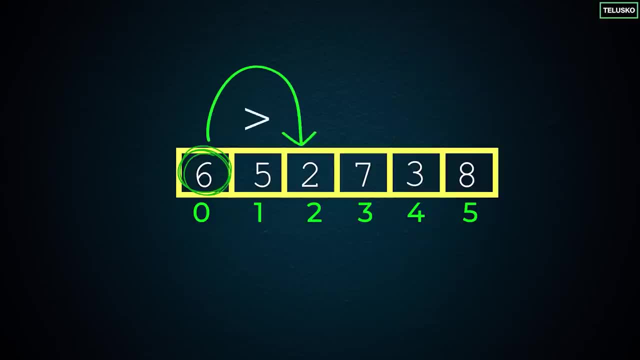 Then you compare it with two knowing to change. But then when you, when seven comes, you know, you know seven. seven comes to the picture. Seven says: Hey, you know, I'm the big, I'm bigger than you. 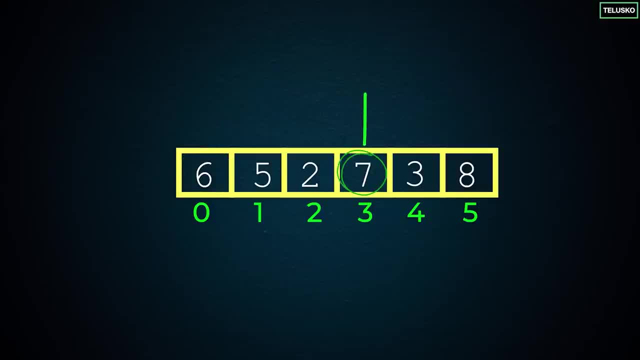 So six says: okay, you're the biggest value. So now the current value will be seven. The biggest value is seven. Now again we have to compare seven with three. Now seven is still the biggest. So we have to make sure that after all the situation. 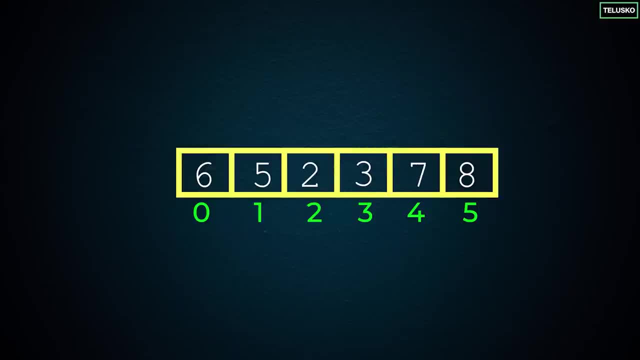 we move seven at the place of three, And that's what we are going to do now by doing the second iteration. So we have completed the second iteration, in which you got two values- seven and eight- at the end- And the first four values are same. 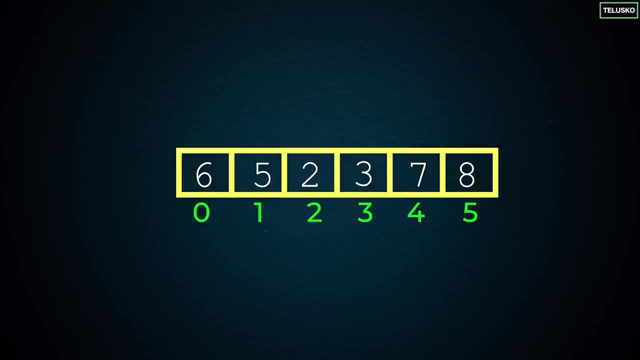 So again you do the same thing, next iteration. So you have to do this till the you, till you complete all the sorting. So you again go with six and say, Hey, you know I'm the biggest. now let's compare six with five. 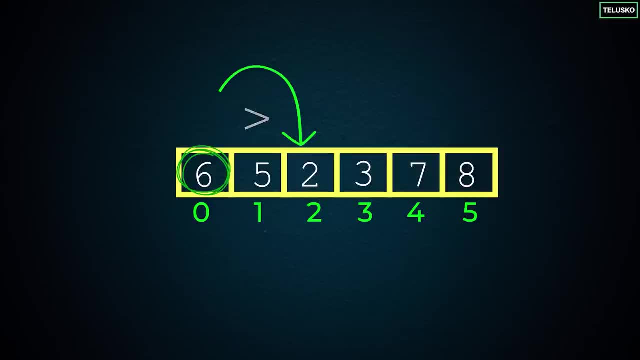 So still the biggest compared with two, still the biggest compared with three. still the biggest. Now, once you complete that unsorted iteration, you will make sure that you move your six to the location of three, because that's what the six should be. 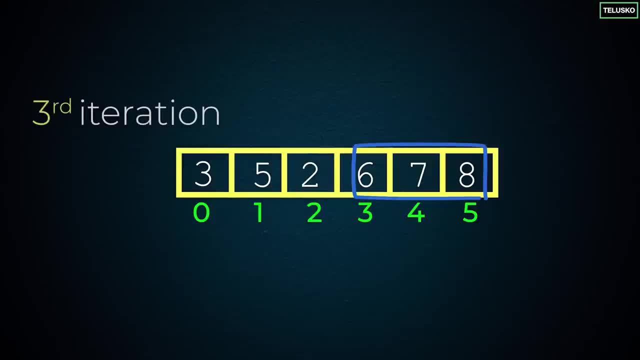 So it will swap with three And then if the first three values- six, seven, eight- are sorted, the first three values are not sorted. So again, if you observe, what we are doing is we are making sure that you got two different sections of sorted values and unsorted. 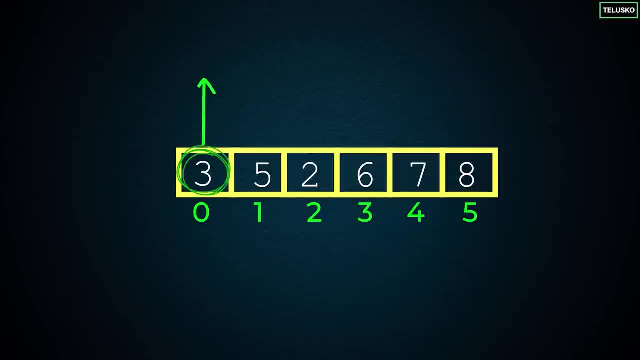 values. Now goes for the first three values. So three, let's assume three is the biggest and then compared with five. Now we know that five is the biggest of all, or at least bigger than three, And then you compare you. 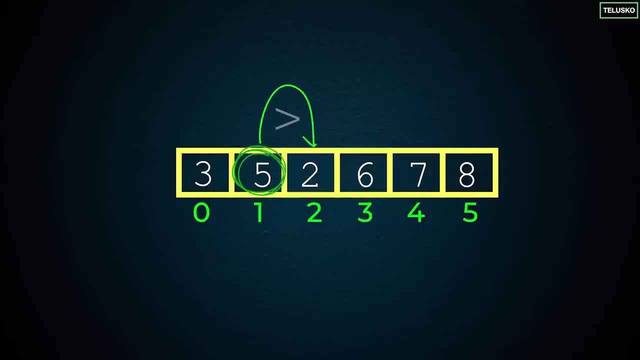 you make the bigger value as five. Now three is gone. Then you compare five with two. still five is biggest. And now we know that five need to go at the location of two, So you have to swap it. Now comes the first two values. 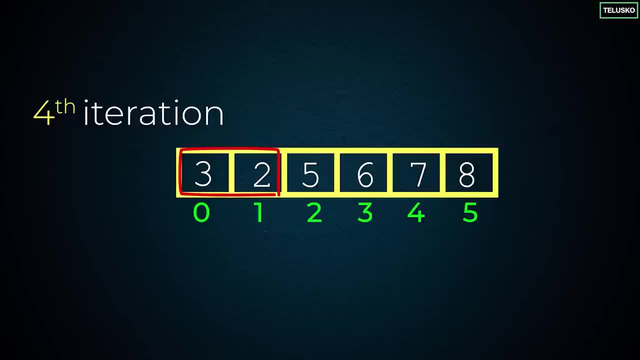 Again the same thing. You will keep doing this till you reach to the end of your array And you move to three. And since we only have one value, don't need to sort it. That's already sorted. And by doing this, 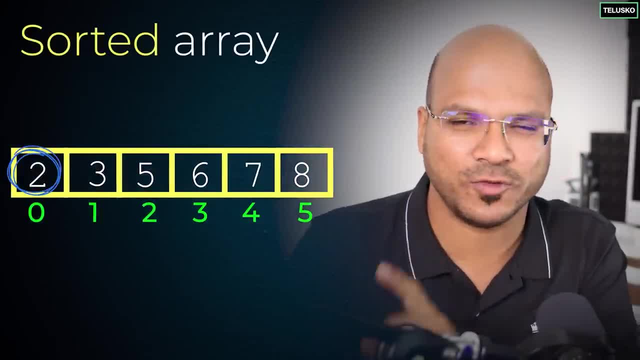 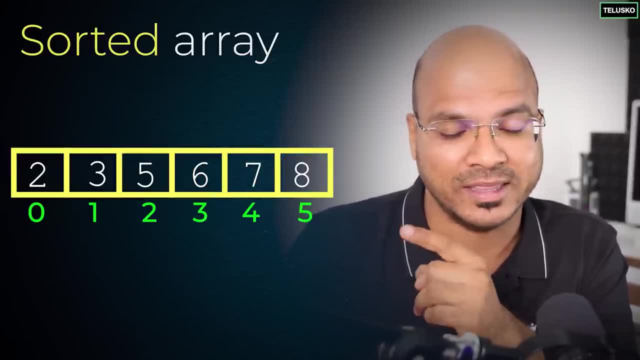 you basically got a sorted array. Now again, compared to the bubble sort, we are still going from start to end. You have an outer loop, you have an inner loop, but we are doing swapping only once in every big iteration or it in every. 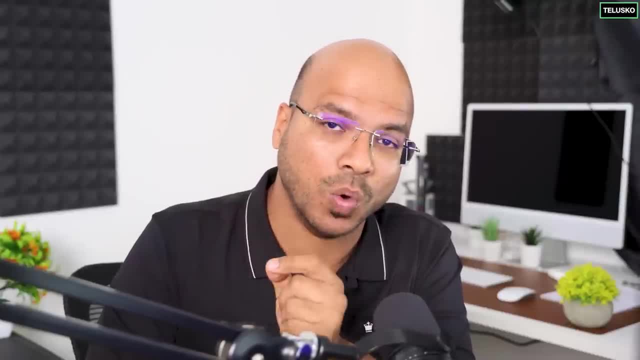 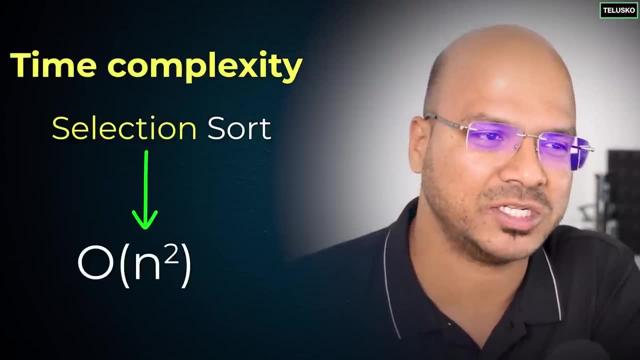 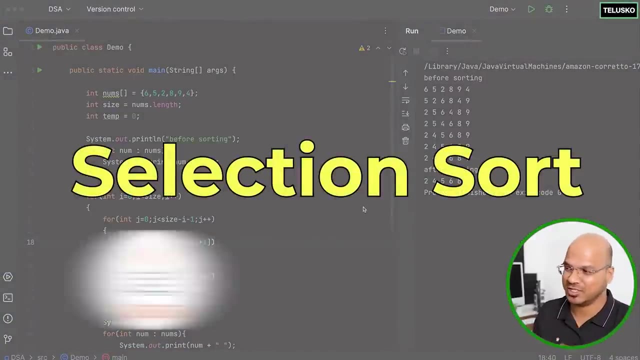 pass. So that's the advantage of using selection sort over the bubble sort. about the overall comp, the time complexity is still O of N square, but at least it is better than the bubble sort in terms of swapping. Now it's time to implement selection sort in Java. 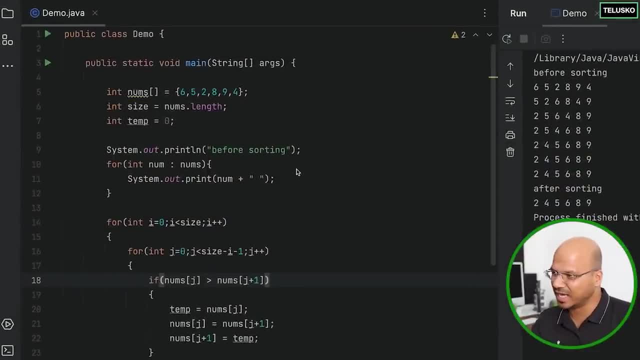 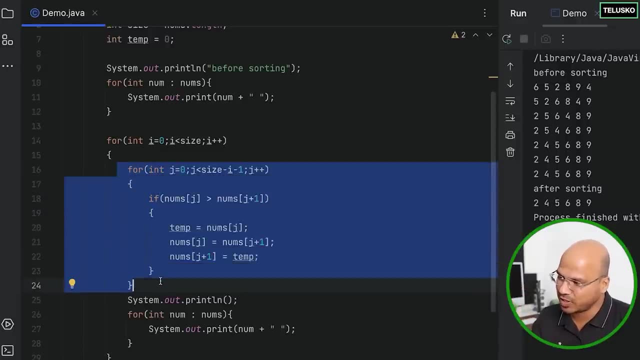 So in the previous video we have talked about the bubble. sort right, And this is how it works. Now one thing to remember: in the inner loop- and you see this loop, in this loop, we are basically doing this swapping, So it increases the time as well. 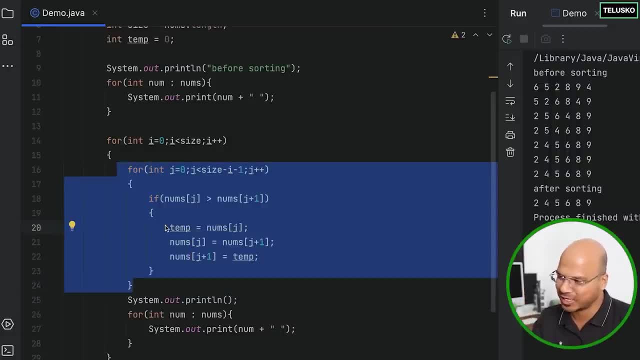 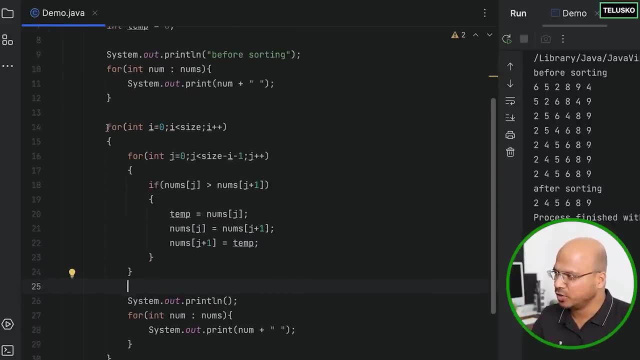 So in selection, what you do is you basically swap this. Of course you do that swapping, but outside the inner loop somewhere here, So it reduces the number of swaps you're doing probably do it. So what I will do is I will just remove the entire code. 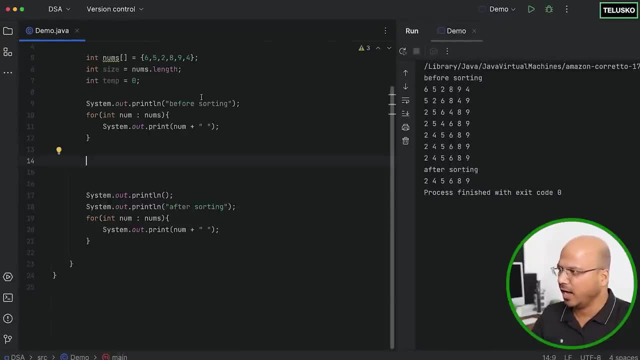 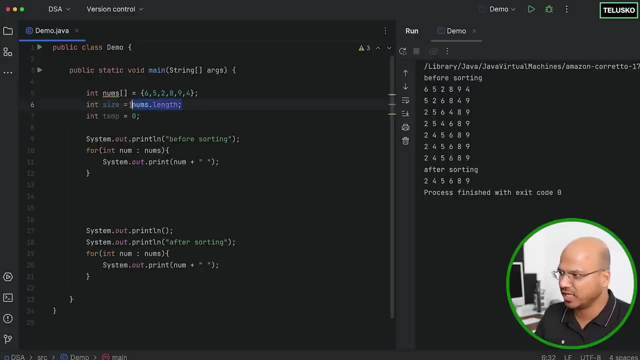 from here, because this is the bubble sort. I don't need this, And what we have here is we have the array, which is, which has six elements. We've got a size variable where we are storing the length of an array, And then we also have a temp variable for swapping. 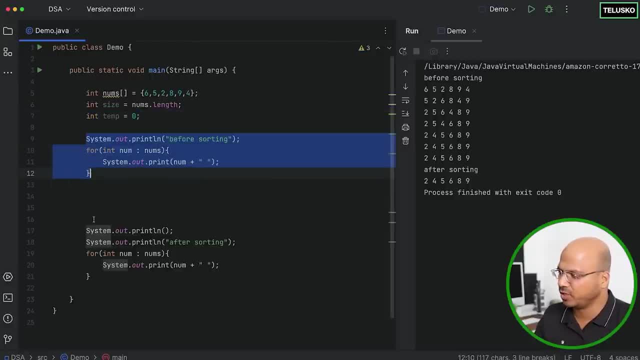 Then we are printing the array before sorting and we are printing the array after sorting. okay, So if you run this, you will get the values before sorting, after sorting, but at this point they are same. It's because the main logic of sorting is missing here. 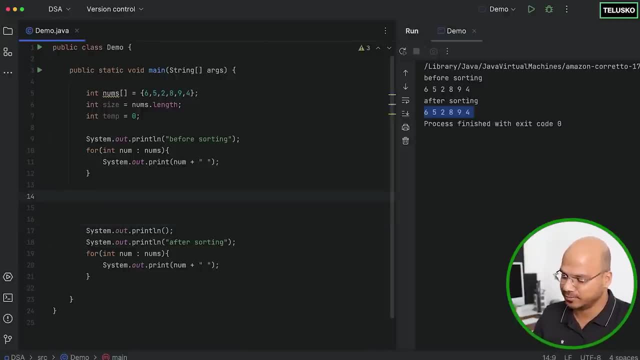 So let's write the logic for selection sort here. The thing is in the theory. we have said that we'll go for the maximum value, the biggest value to swap, or we'll put the biggest value at the end. Let's say in the practical. 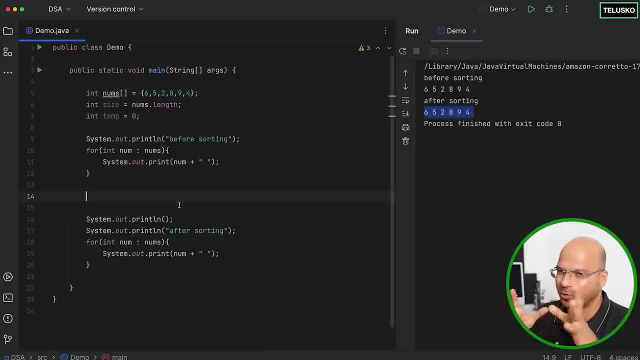 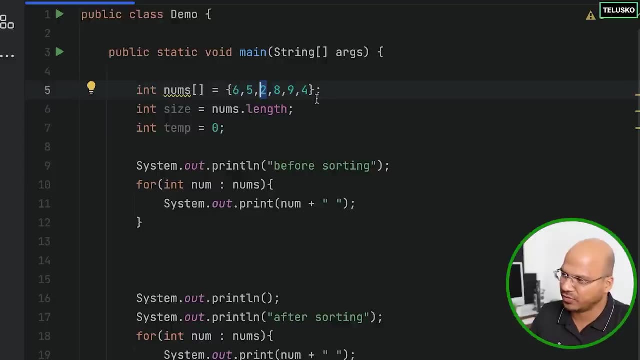 let's try to implement with the smallest value- and we have seen both the approach then. So what we are going to do is we'll look at the entire array and then we'll find the smallest value, which is two. Of course, you have to iterate between all the values. 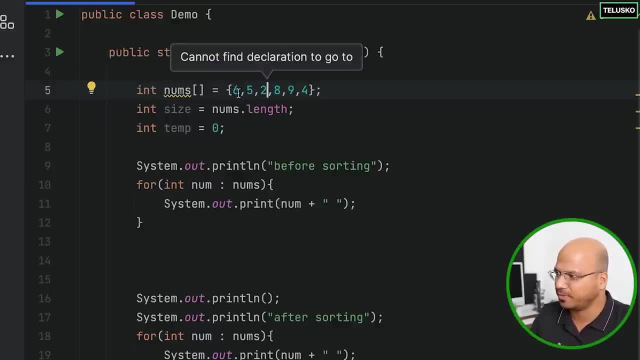 And then, once you've got the smallest value, you will swap the six with two, because two should be the first value, and that's how we can start. And for doing that we have to use two loops: the outer loop and inner loop. 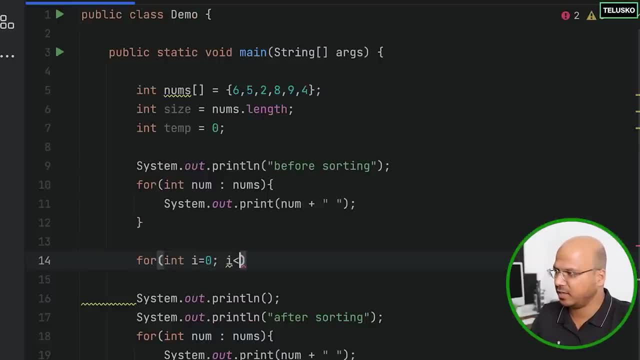 We'll start outer loop with zero and then we'll say i less than size, right, Okay? so we'll say i plus, plus. But also we can make it more efficient by saying that size minus one. It's because, if you remember, 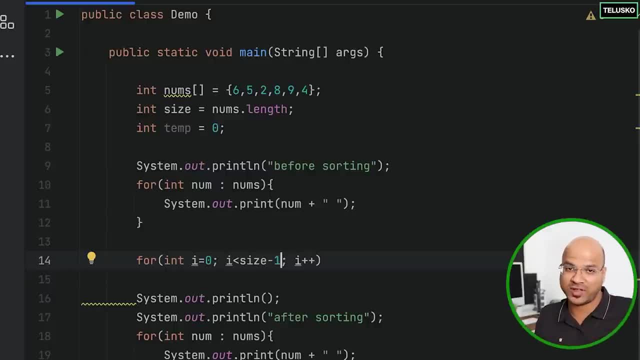 when we were doing the sorting. and once you got all the values sorted except the first value or the last value, you don't basically sort the one value right. So you can reduce the number of iterations you go for. So we can say size minus one. 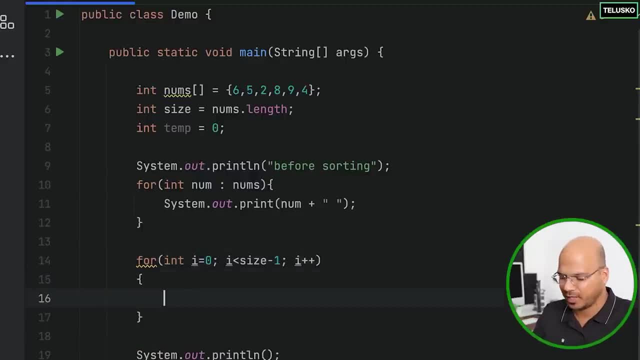 and we'll see if that works or not. And if it works, then we are happy. We'll also go for the inner loop. Now for the inner loop, we'll go for j equal to Now. where do we are going to start j? 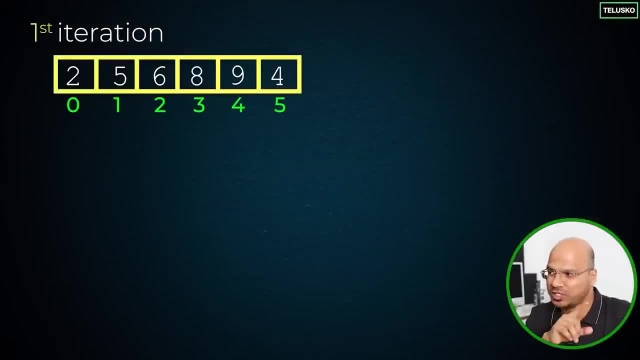 So basically, if you're putting the starting, the biggest value or the smallest value at the start, what it means is after, for every iteration, the inner loop, we can skip the first value right. So for the second iteration, we can skip the first value. 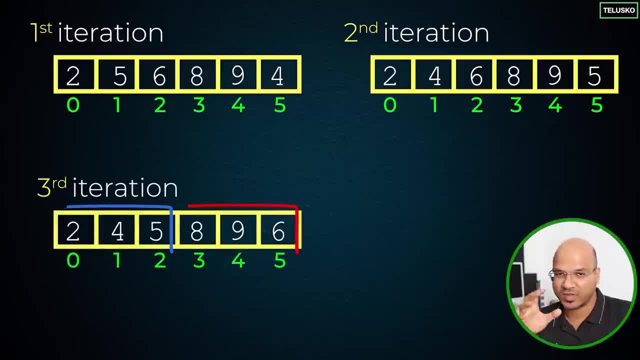 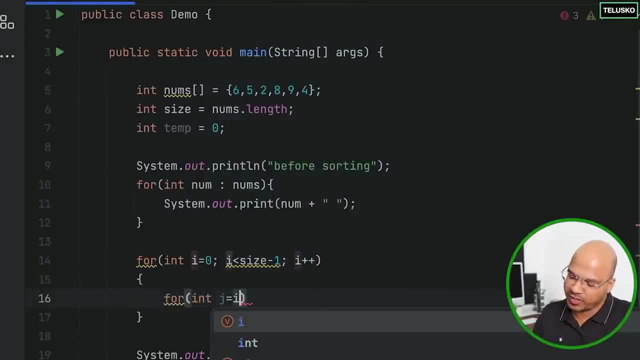 For the third iteration. we can skip the first two values because they are sorted right. So we have two sections: right Sorted array and unsorted array. So here we can start with j equal to i. Yeah, in fact, when your i value is zero, 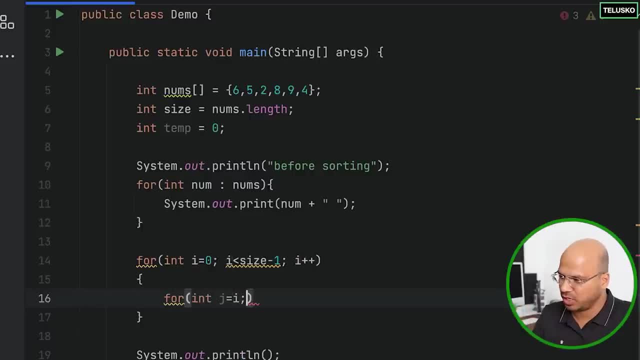 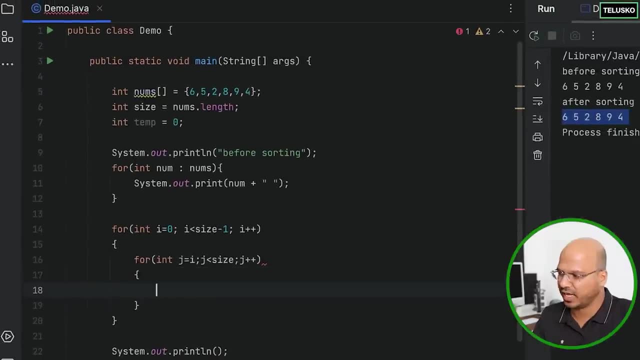 j should start from zero, So we can say j equal to i and j less than size and j plus plus. So basically, we have to go to the end. Okay, so that's the for loop. we have Now what you do inside this. 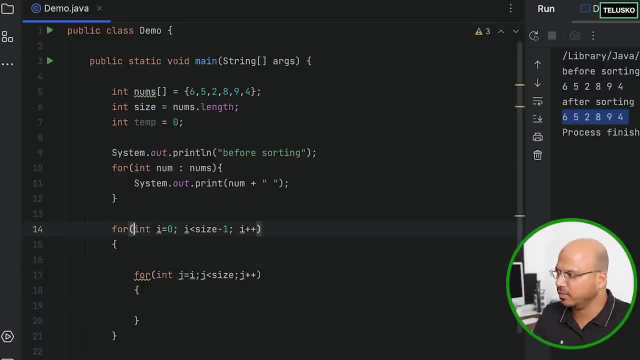 So we have to find the minimum value To start with. we can take min value variable here. So I can say int min is equal to zero. In fact we want the min index, not the min value, because we have to work with the index, right? 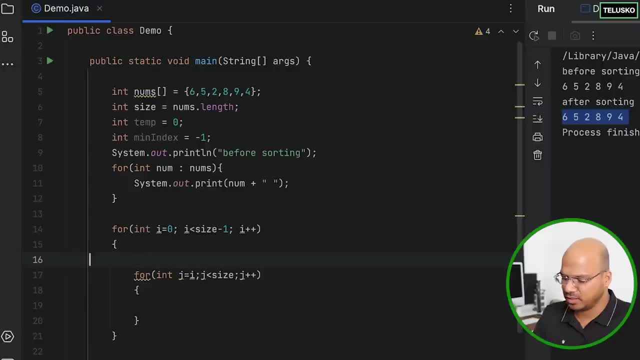 And we'll say: the index is, by the way, by default minus one. And here, to start with, we'll start with min index equal to i. And then what you do? you basically check if the array which is nums of min index. 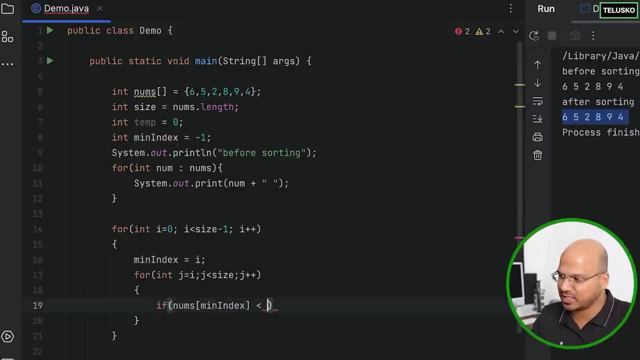 Now we want this to be smallest value, right? So I assume that this is the smallest, but what if this is not the smallest compared to the value which we are considering? The value which is considering here is nums of j. So, example, if this six is the smallest, 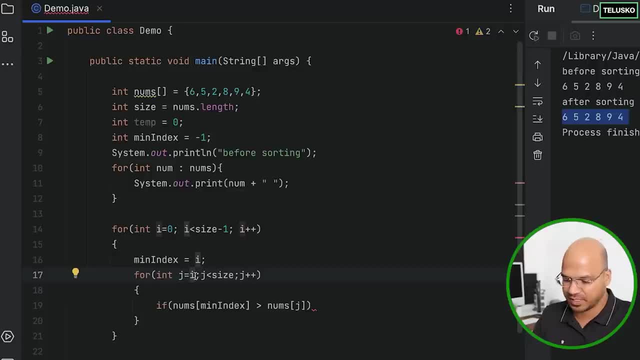 which we are thinking. in fact, you know we should be say i plus one, The reason being, when you are saying that six is the minimum value, we are assuming that, and then we are comparing with five. Now you will get five. when you say j starts with i plus one. 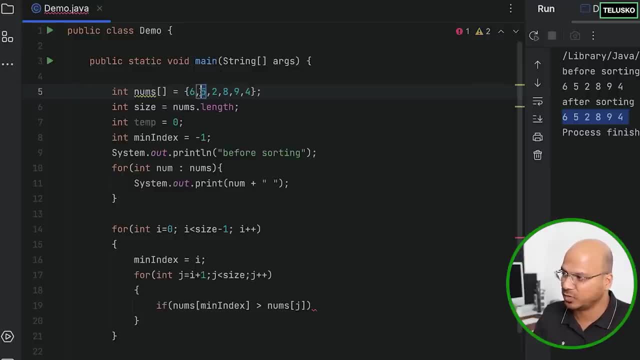 because in the first iteration the value of i will be zero and this five is one right. So we'll compare these two values. If six is smaller than five, then everything works. but what if six is greater than five? In that case we have to swap. 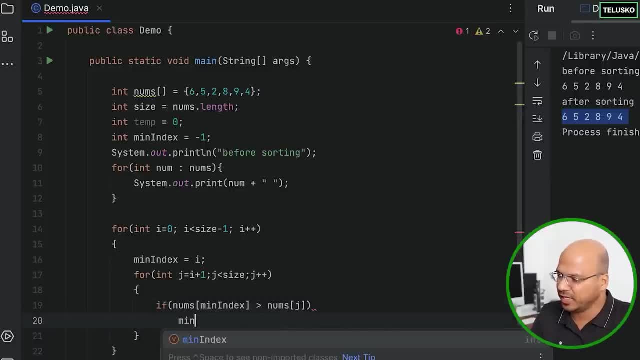 Now, okay, we don't have to swap. We basically have to change the min index to j, because the new index we will get is j, So the new index here is one. okay, So that's the min index. So what we are doing by doing this is: 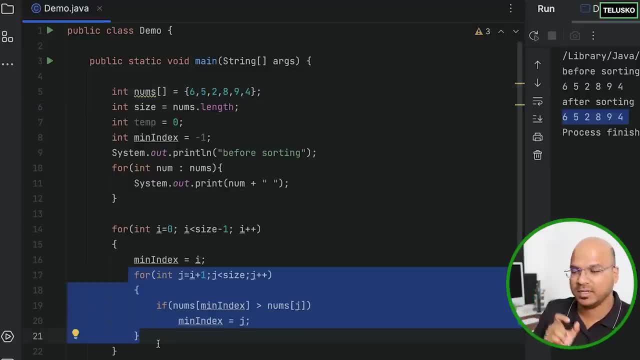 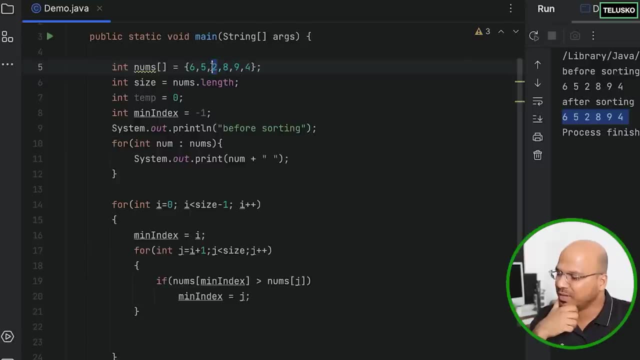 after the entire iteration, you will get the minimum value from this adding okay. So that means after this iteration you will know that two is the minimum value. Now, once you know the minimum value, what you do is you swap two with six. 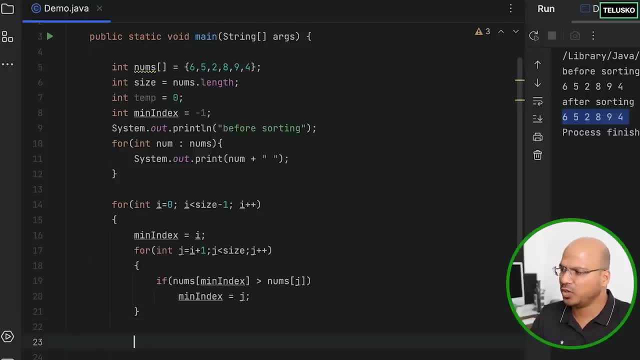 It's that simple. How do you swap two and six? How do you know we have to swap six? Because i is referring to six and the min index is referring to two. So we can simply swap them. So we can use a temp variable here. 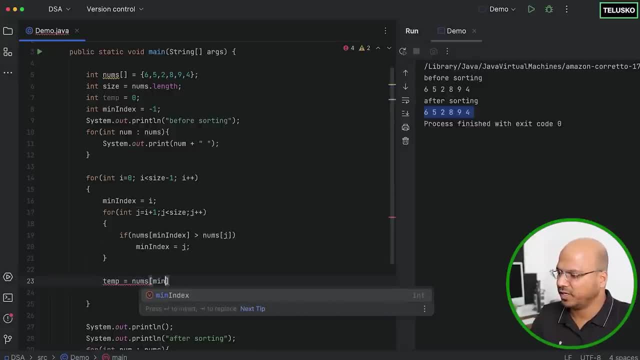 and we can put nums of min index and we can say nums of min index is equal to nums of i and nums of i is equal to temp. So basically we just have to swap them. So what we are doing is in the inner loop. 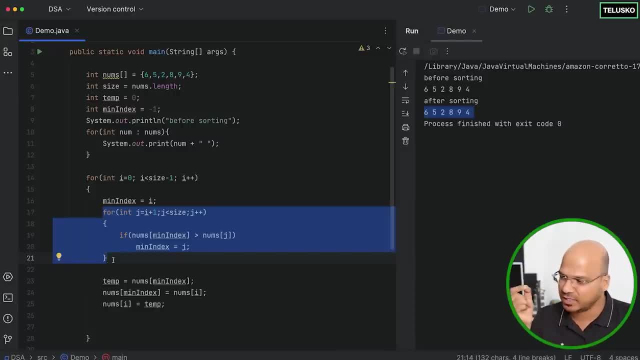 we are just finding the minimum value and then, once you find it, you simply swap it with the min value which you're considering, which is the first value, And as the i value goes up, first you will compare with this, then you compare with the five. 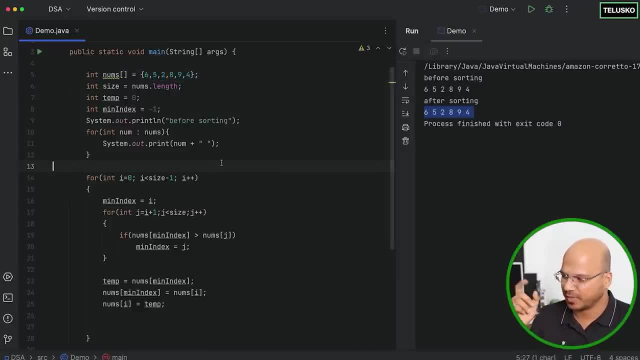 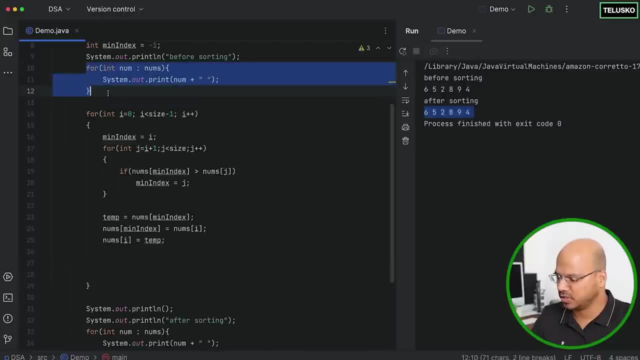 then you make two as a minimum after, of course, after the swapping. And what I will do is I will also print this values after each iteration, So I can just copy this and paste it here and we also print a new line to get it on the new line. 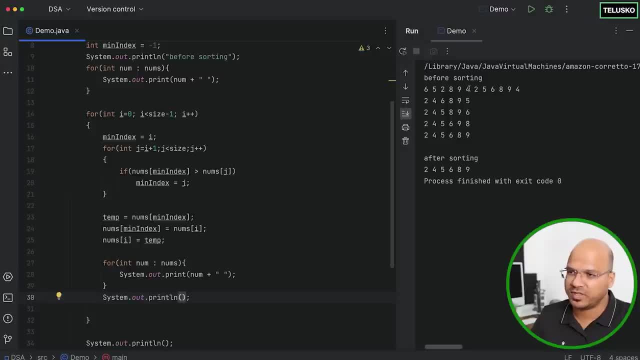 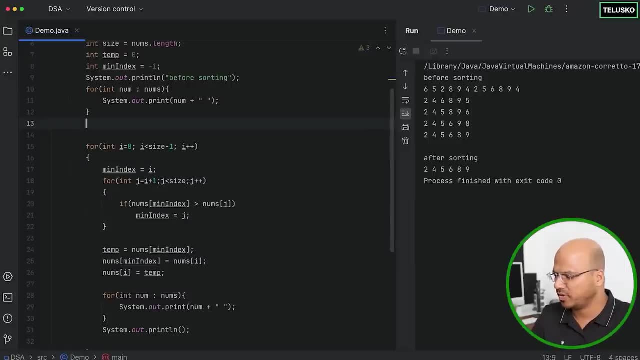 So now, if you run this, let's see what happens. So you can see, this is okay, I will after printing this also, I will just say new line, or maybe I will just skip this new line before the for loop printing. 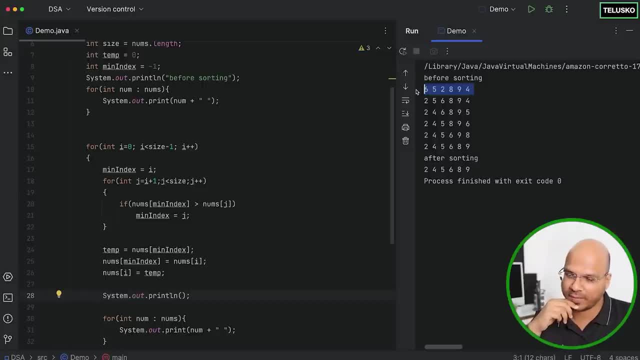 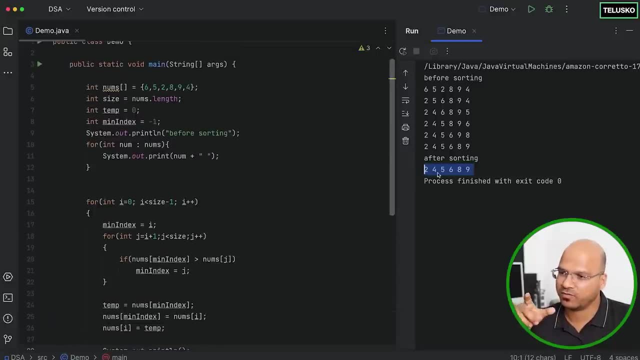 okay, let's run and you can see: this is before swapping and this is after swapping. So let's compare the value. Is it properly sorted? Yes, two, four, five, six, eight, nine. Those are the values we have. 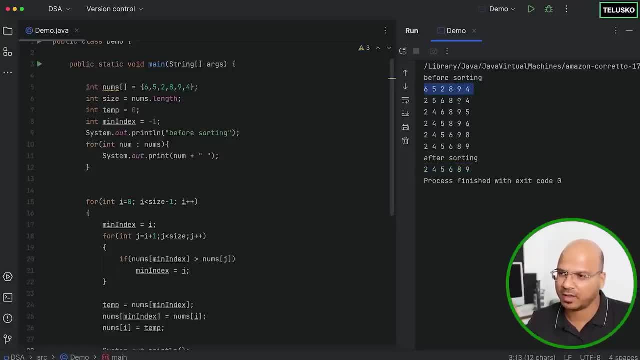 And then see the steps In the first iteration before swapping. So this is the first iteration. What you do is you know that 2 is the minimum value, So you swap 6 with 2 and that's done. Then in the second iteration, 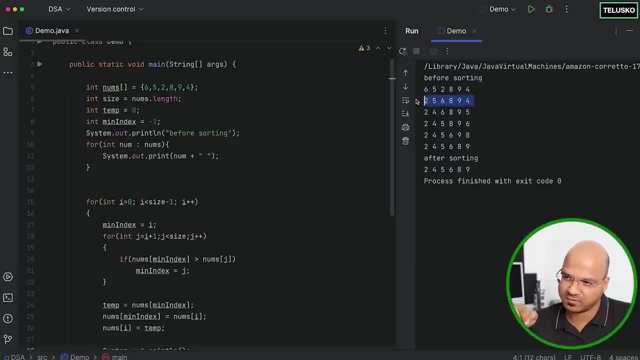 You find the minimum value. So the minimum value from this is 4. So you swap 4 with 5 and that is done here. Then you consider 6. Then you say you find the minimum value from this, which is 5. you will swap 5 with 6. 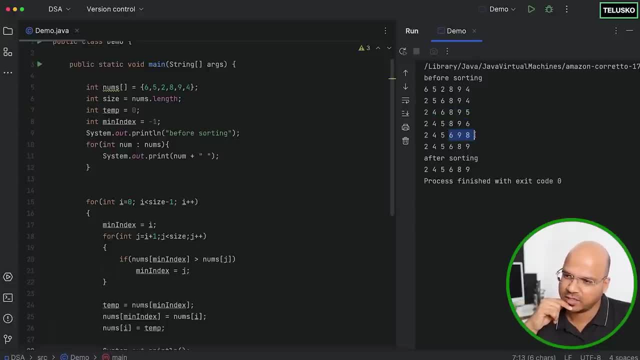 So in this you will say 6 is the minimum, so you will swap it with 8. Comparing this: 2, this is 8 and 9, so you will swap 8 with 9. and in the last one You don't have to even sort it because it's already sorted. and that's what we are doing here. 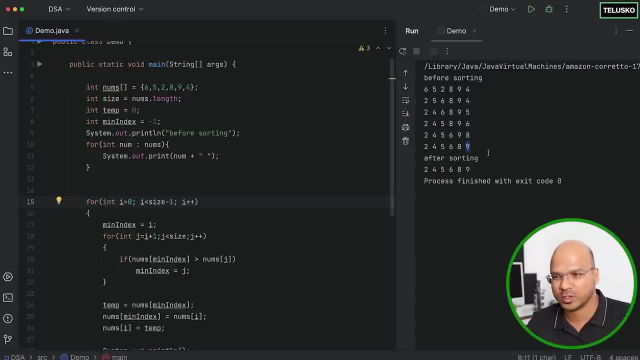 And that's why we say it's size minus 1.. We don't even sort here. In fact, if you don't put this minus 1, what will happen is, if you run this code, You will get one more iteration and there is no change there. It doesn't matter how many values you have. 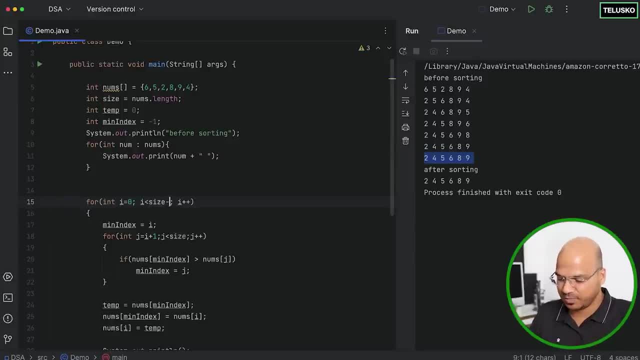 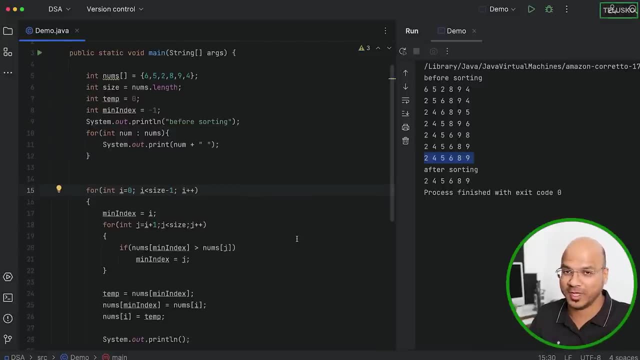 You're not going to have any change in the last iteration, So you simply save it by saying minus 1 here. So that's how we use selection sort Basically: You find the minimum value and swap it with the location where it should be. So we have talked about different sorting techniques. 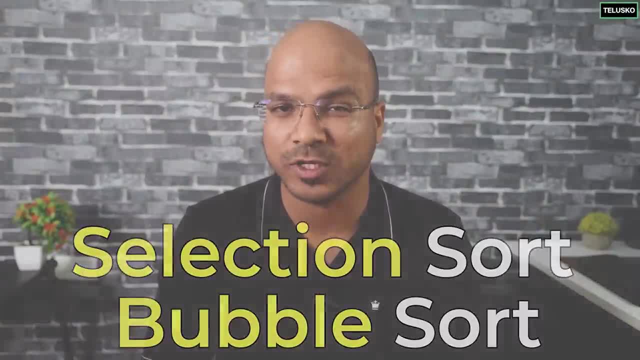 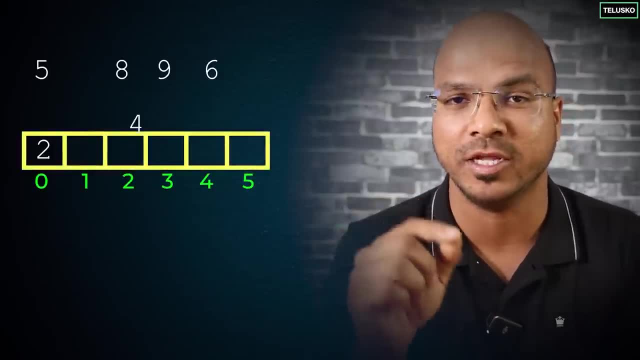 We have talked about bubble sort and selection sort. In this video we'll talk about insertion sort. So what you do in this technique is basically you take the elements and then you put the elements at the right position. That is your insertion. So you have to put at the right location. 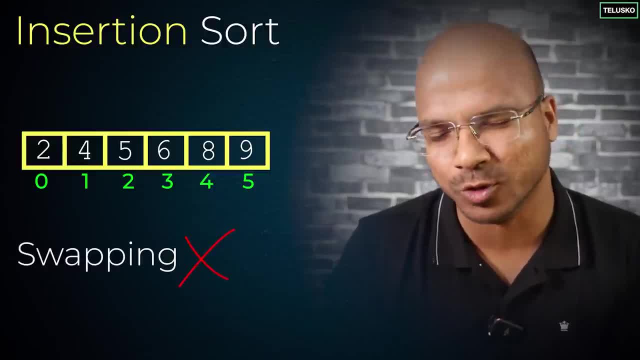 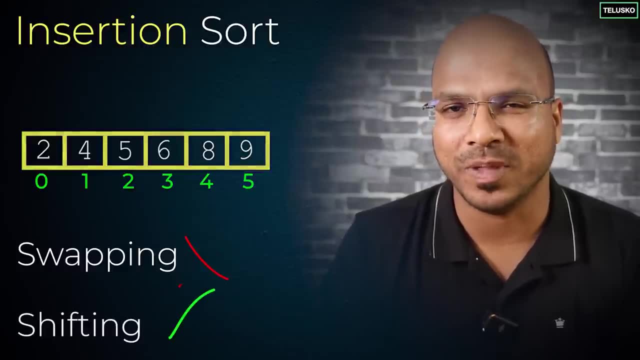 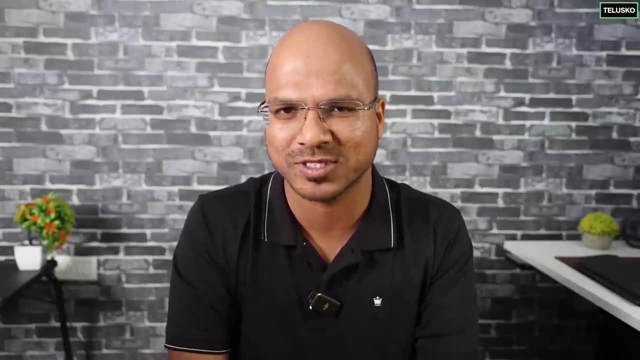 Now, in this you don't normally do swapping. Yes, we do swapping, but we don't use word swapping. What you use is something called shifting Okay. so example: if you are playing, if you are playing cards, So if you, if you have a random cards on your table, so basically, in this example, you're not going to use cards. 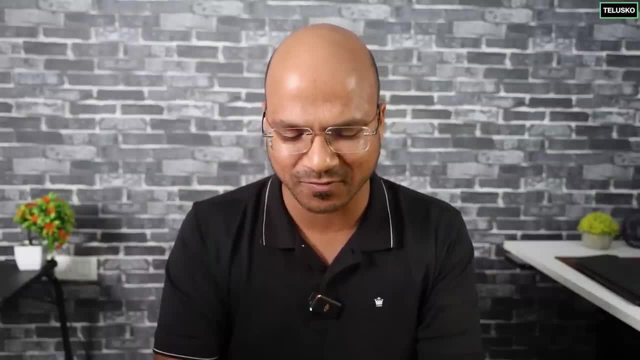 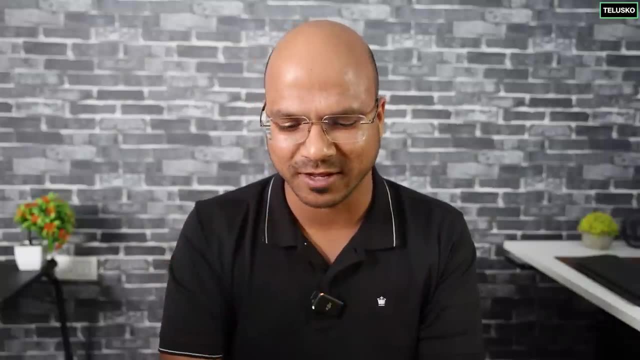 We are going to use this characters. I found these characters in my In my drawer. I think I got it for my kid's birthday, but doesn't matter. So I got this and we'll try to sort this values here. So let's say, if you randomly get these values and if you want to sort them, 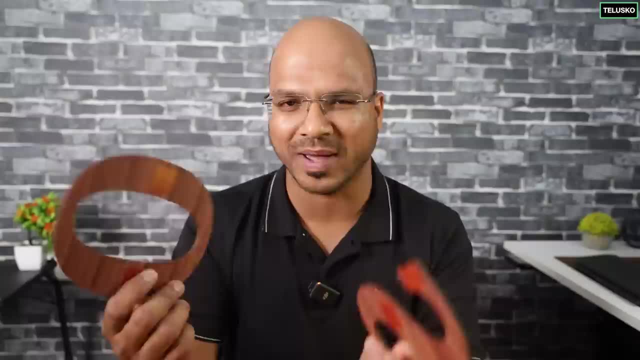 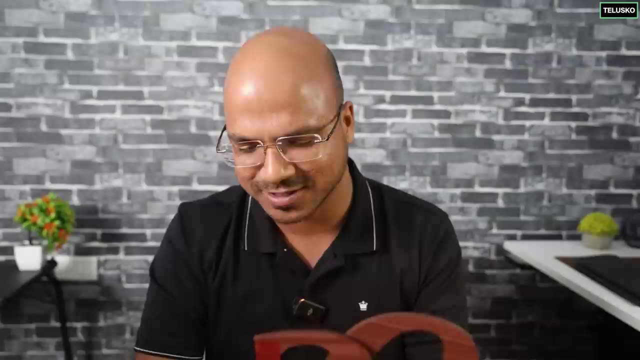 What you do is you pick up the value and then you- you know, imagine these are cards- playing cards. So what you do is you take the first value, you take the second value and then you keep it like this. I don't know if how many of you played cards. I used to love them, not for money. 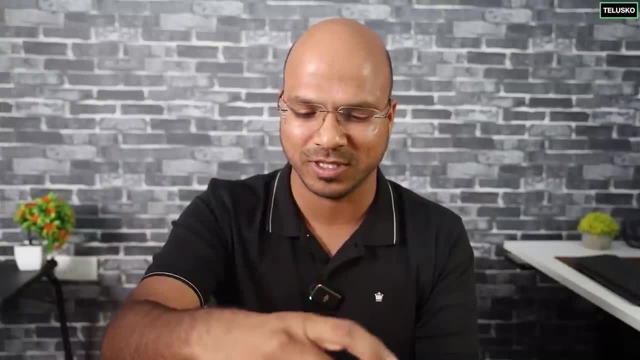 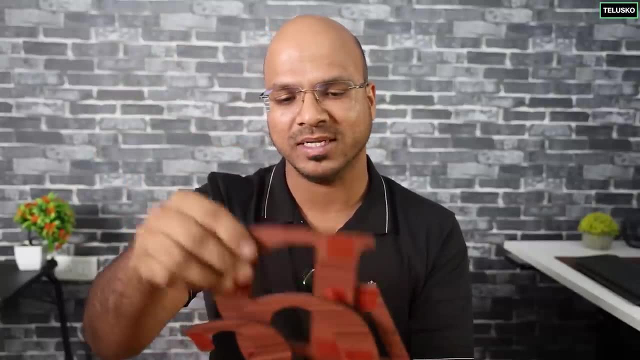 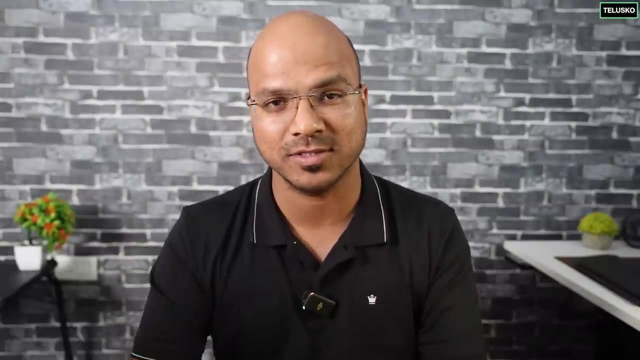 But I used to love them. then you take a next card and then you put it before this. Then you take a card, then you know that this card goes between A and O. you put it here. So this is called insertion. but how exactly you're going to do that, that we'll see, with example, on this table and with this, with this cards. 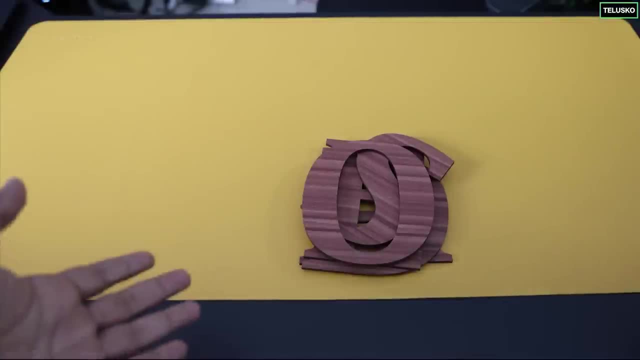 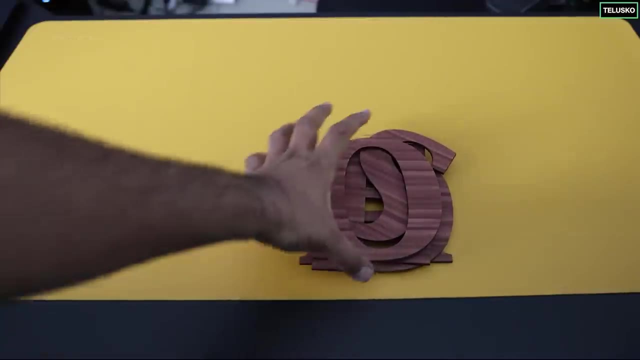 So now let's sort this. values now, These are not values, but characters, So let's try. so what we have here is: we'll start with the first location. as you can see on the screen, We have different values here, and I'll pull this down a bit so that we can have some place to clip this. 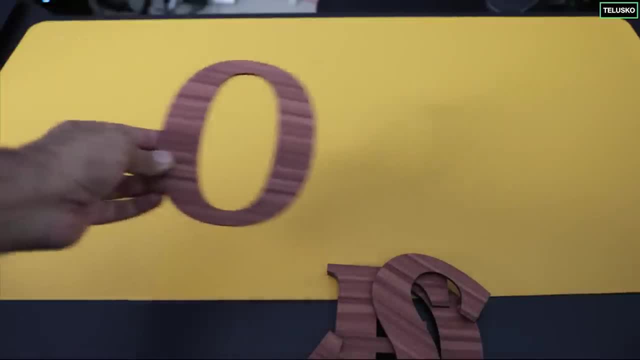 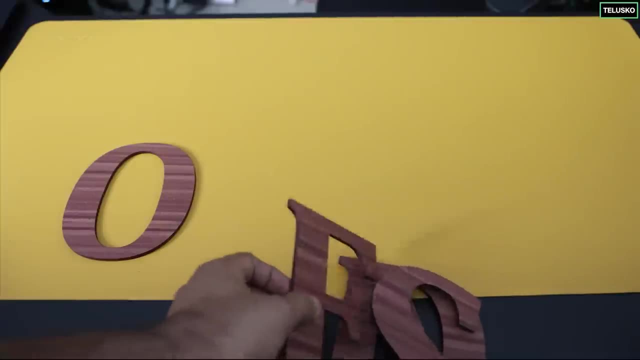 So the first value is O. now I'm assuming that the O goes here, the first location, because it's always sorted- and then you take The next value, which is E. Let's say, now We know that E comes before O, so what we need to do is: 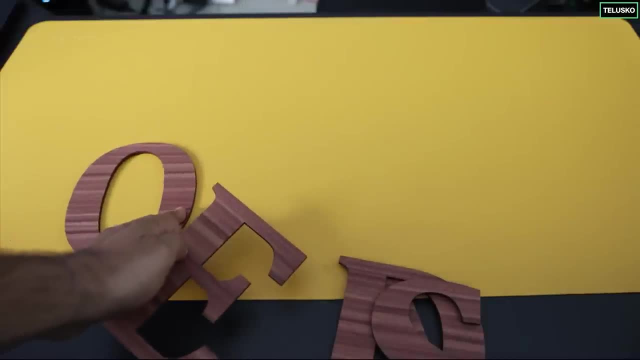 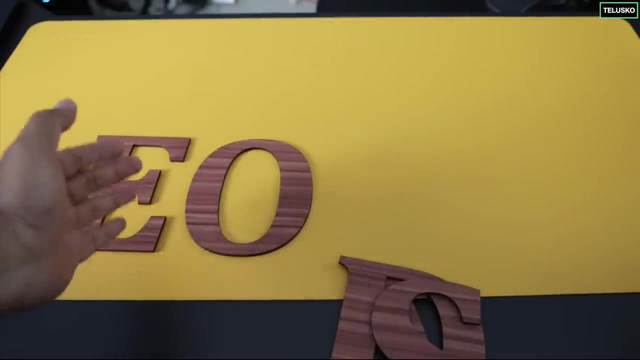 This need to go at the start, So you have to move this to the next location so that you will have some space for E. Now the point to remember here is: it's all about shifting, okay, So we don't use a word swapping here, or you'll understand that in some time. Why don't we say swapping? 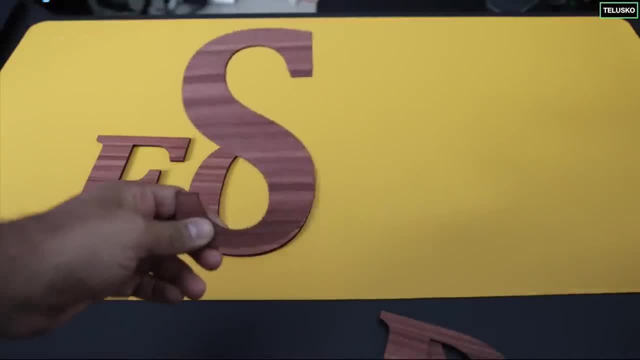 Let's go for the next one, which is S. Now we know that S is greater than so we'll compare S with all the values. so we'll compare S with E. Okay, it goes after that, it goes after O. so S goes here. Okay, I'm not promoting any camera model here. 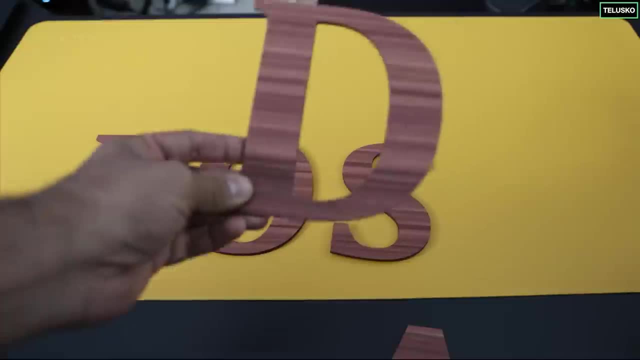 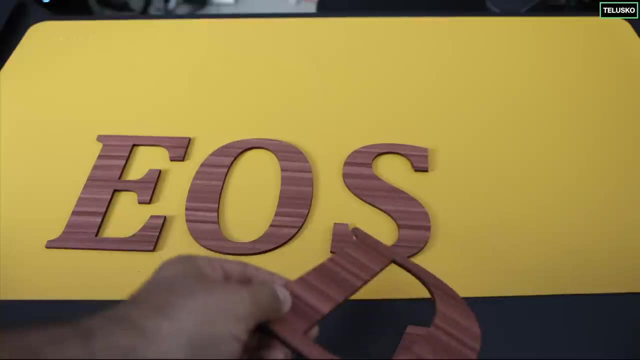 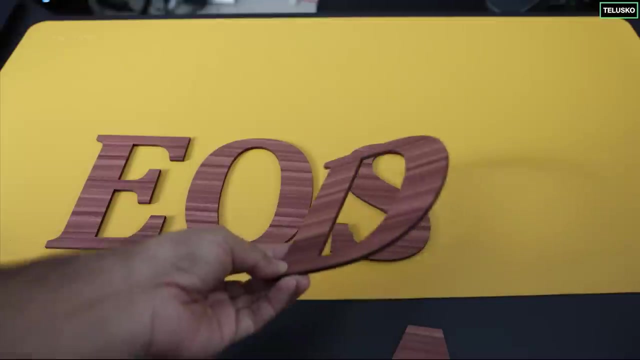 But that's a sequence. then you go for the next one, which is D. now D goes at the start. So what you do is you basically have to move all the elements, right? So if you compare with S here, D is Less than S. so you compare, so you have to shift S. 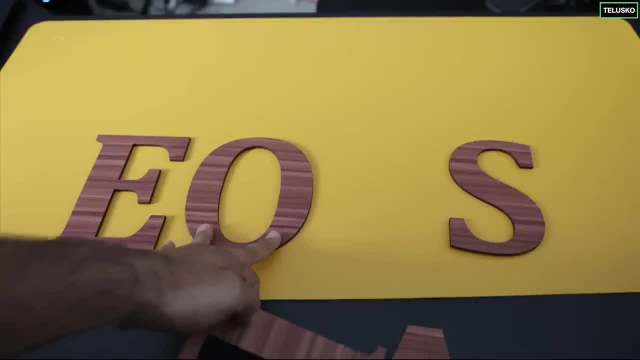 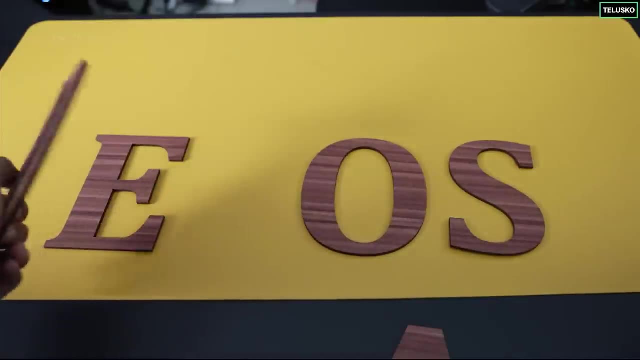 You have to make some space for D. Then you take O and you move O here so that you can make some space for D. Then you compare D with E And you have to make some space. of course you have to swap, you have to move this. You will make some space for D and D goes here. 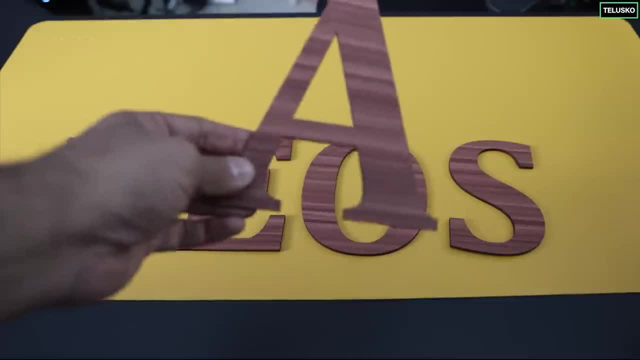 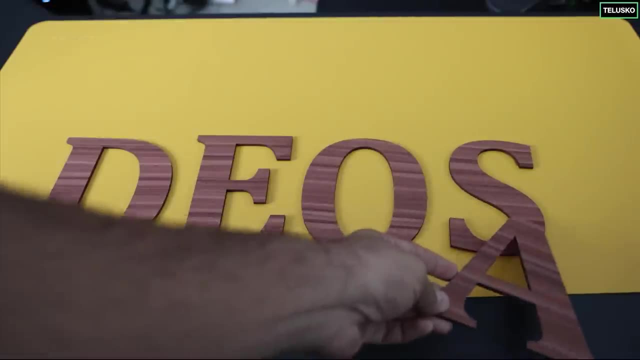 Right, so now it is in sequence. then what about the last value, which is A? Now A? we all know we have to. I mean it. of course it goes at the start, But we have to compare from start or last. so this goes here, Which is S? if it is less than that, we'll shift this to make space for A. 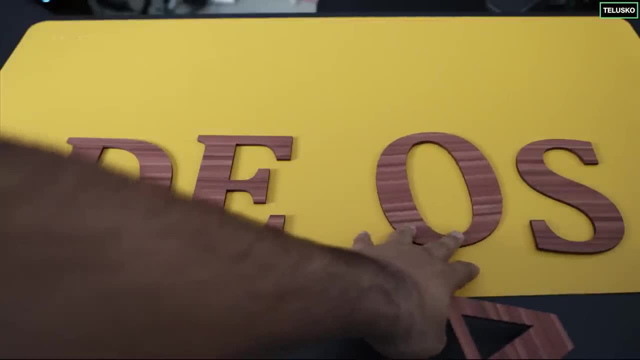 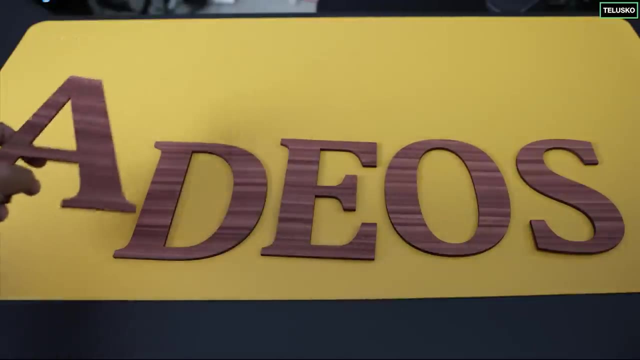 But then we have to also check with O- This I also have to shift. we check with E- This also Have to check shift. we compare with D- This also has to shift, and then A goes at the start. by doing this, what you're doing is you're basically 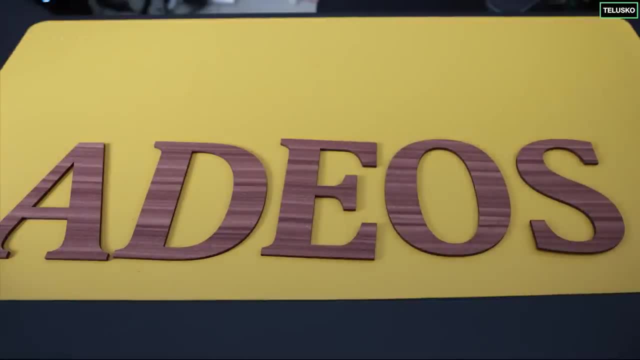 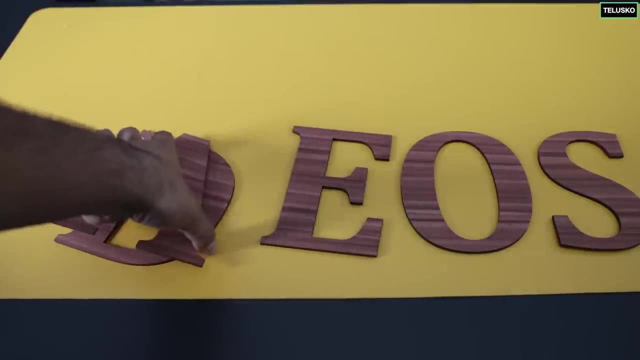 Inserting value at their location. so this is how you do the insertion sort. now Let's say this was the randomly we were picking values, right, but what if you have things already in the array? So what we'll do is we'll keep it here. 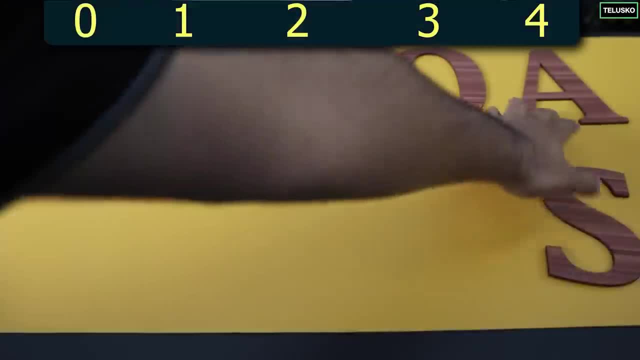 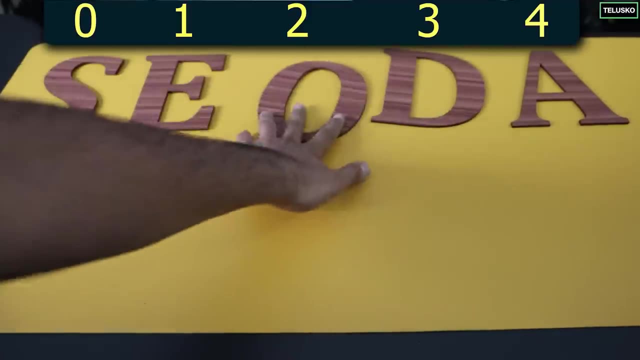 We'll keep this here, We'll keep this here, this goes here and let's say, this goes here. in fact, I will also move this. Okay, I'm not trying to make any city name, but let's say: we have this sequence, We have these five values and now you want to sort them. 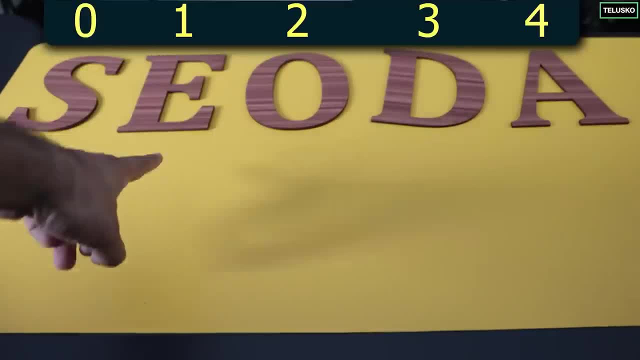 so what you do is you don't start from the first value, you start with the second value and Then- because we are assuming that the first one is already sorted- okay. so what you do in this technique is basically you divide your List, or array into two segments: this sorted and unsorted. at this point, all are unsorted. 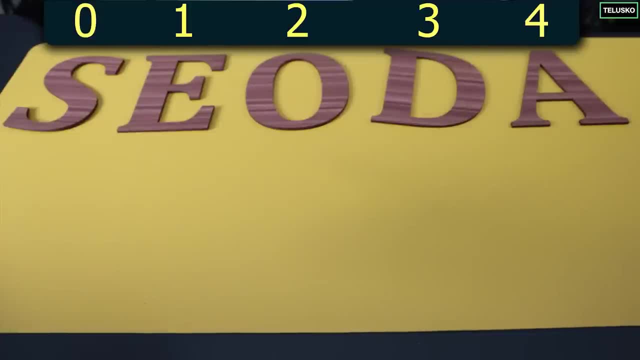 So this is unsorted array, but when you start you have to assume That your s is already sorted. then you start with e when you see, hey, Do we have e at right position? the way you do that is you compare e with s And this and you say, hey, you know e is not the right position, so you will take out. 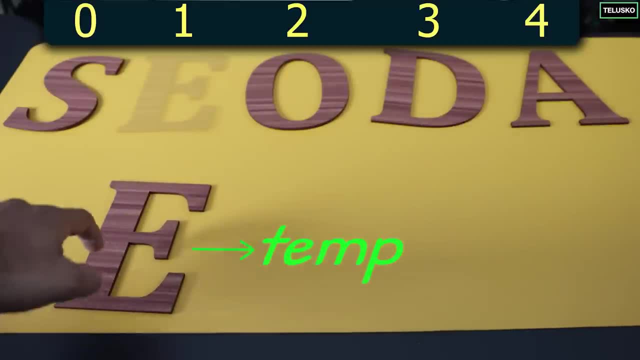 In programming, what you do is you save the value of e in the temporary location. Okay, so exactly. you're not moving e, You're just making a copy of it. Maybe there will be a copy of e here as well, but you have an extra copy with you saved a temporary variable. 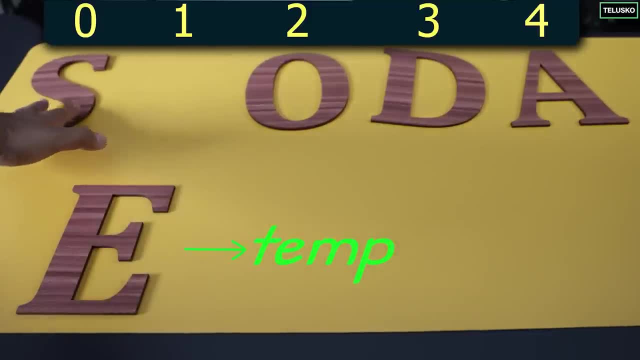 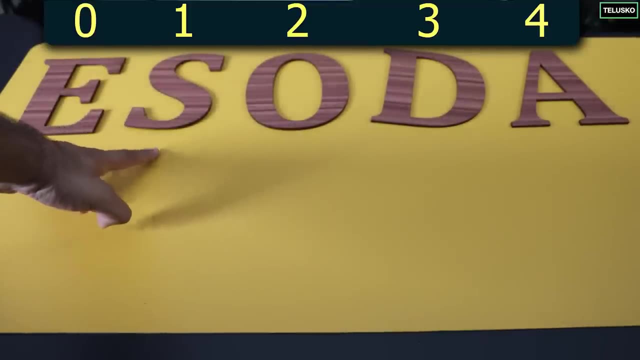 So let's say this is a temporary space. Then you move your s here so that you can make space for e and that's sorted now. now, if you see This two, it looks sorted. Now, what you do is you check e Before. do we have any value? 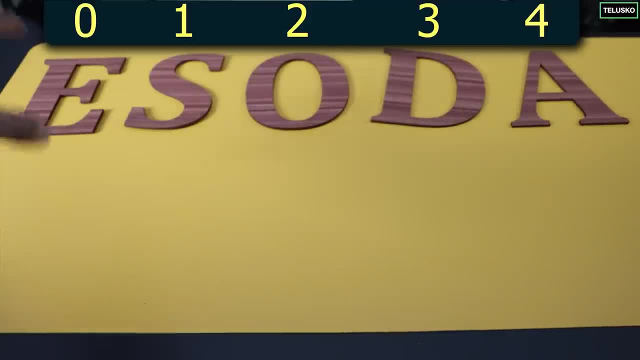 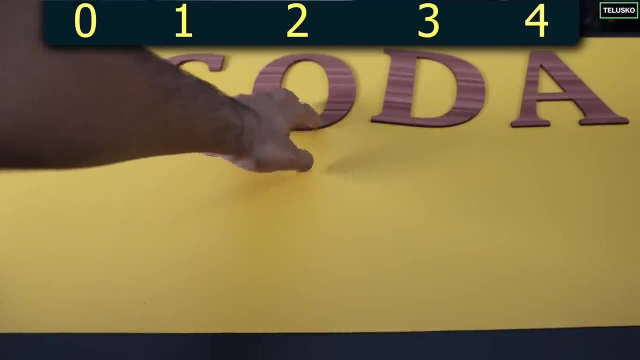 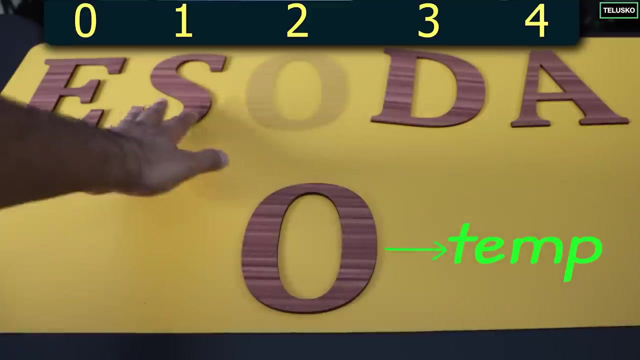 So of course we don't have any value before e. now that is sorted. then you go for the next value, So we started here. in the next iteration You basically start with o. now o will compare with the previous value, so which is s? now? is it the right position? no, so we have to copy o in the temporary variable and 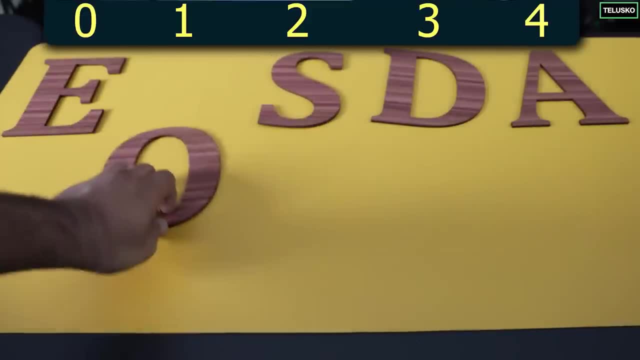 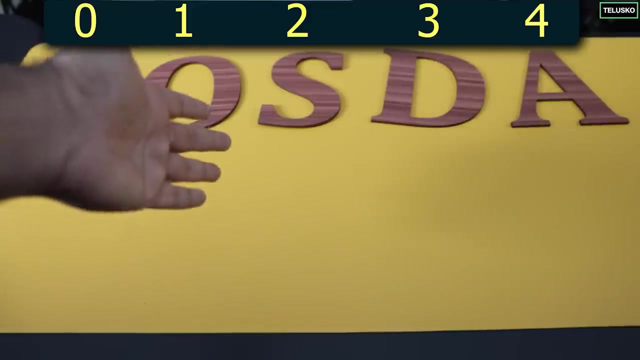 Move your s so that you can make some space for o and o. of course you can move o here. you have to also check if o really goes here. you have to compare o with the previous value, which is e, and We know that o is greater than e, so you can keep o here. So that's how you basically sorted the third element. 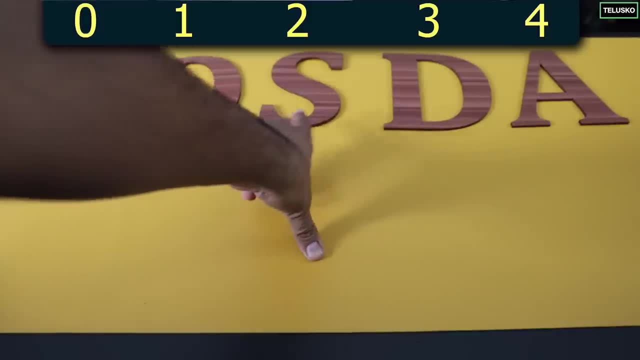 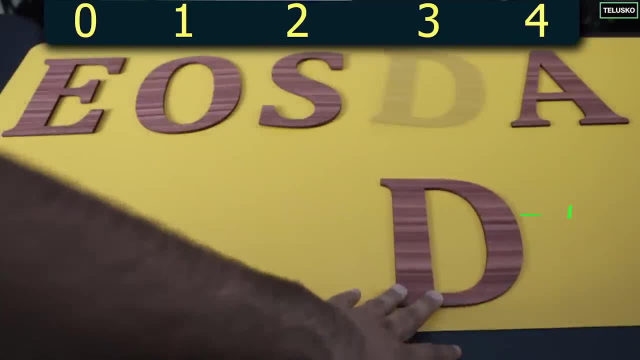 Then you go for the next element, which is d. So what you do is you compare d with s here and then you know that D is smaller than s or s is greater than d. So what you do is you have to move. So you take into temporary variable, move s here. Of course you don't move d directly there. 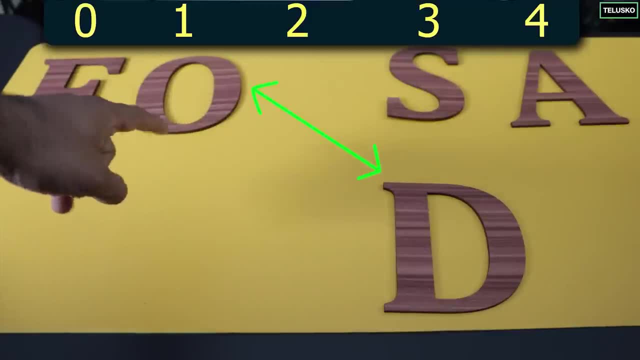 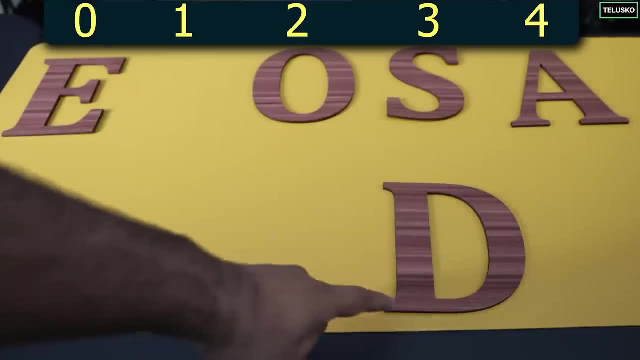 You have to compare d with the other other elements. which is o: is it smaller than that? Yes, We have to move this here. We have to make space for d right again. before that also, We have one more element, which is e, so you move e here. 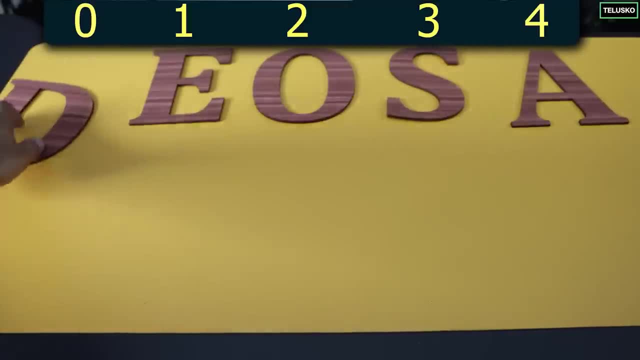 It's all about shifting values. and then your d goes here and if you compare It looks Sorted right compared to the other other values. so it looks sorted. But then you have to complete one more iteration. So you take a, you compare a with s. now a here is compared with s, so again we have to shift. 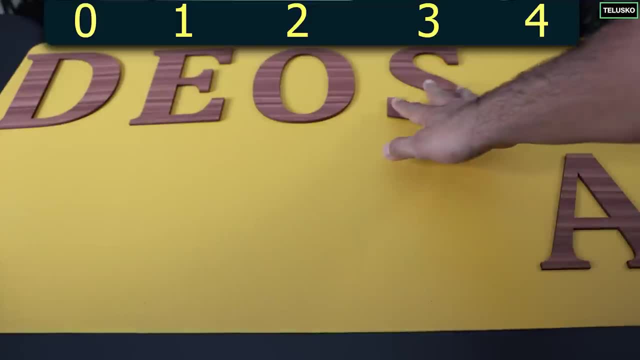 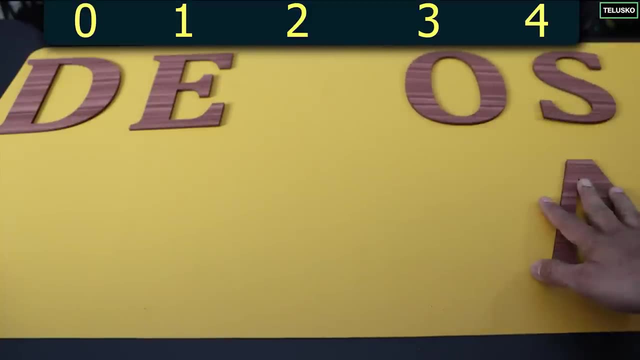 So what you do is you take a in the temporary location, then you move your s. You will check a with o again. You have to move o. then you check a with e again, you have to move e. so Remember, we have to only move When you know that a will. 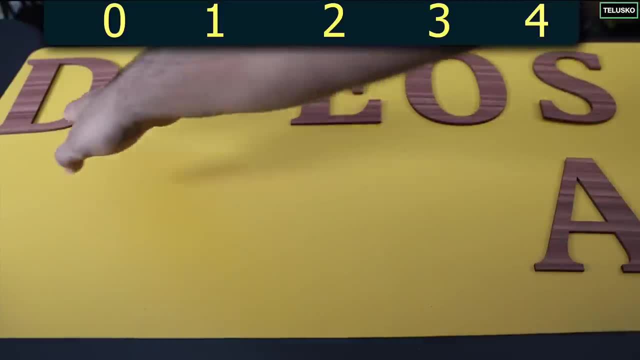 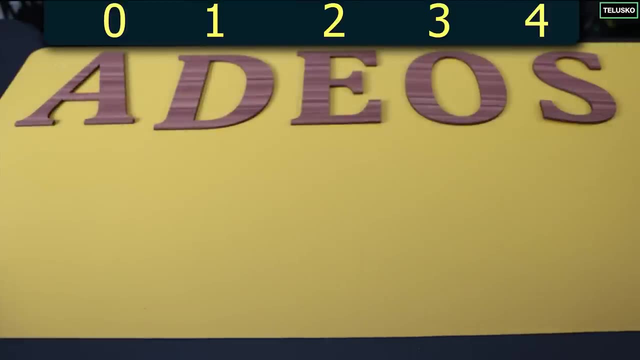 Not be the right position. and then you compare a with d again. d has to move so that you can make some space with For a. so this is how, basically, you do this sorting technique. now question arise: How will you do in programming? So what you need is you need two loops, one for the number of passes you are doing right, moving from different element. 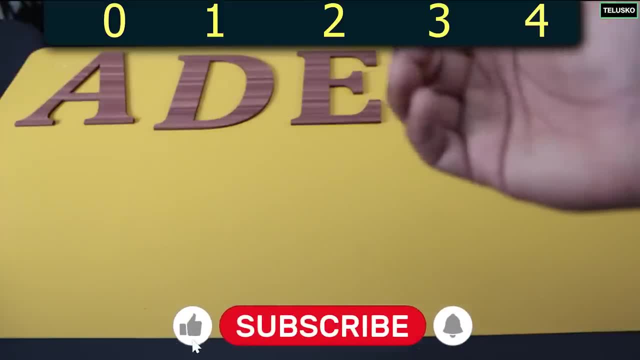 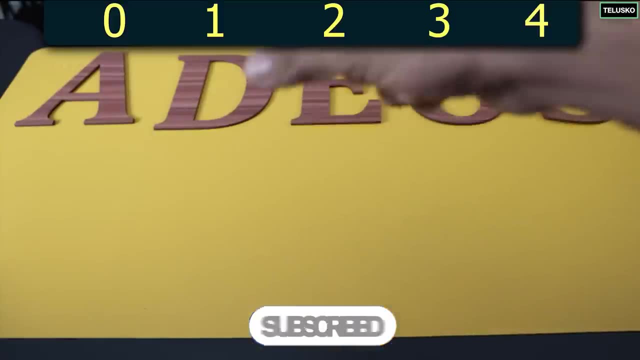 and you need a inner loop which will responsible to find the key and Shift the values, and also you need a temporary variable so that you can store it somewhere. So you have to. you need a key which will go into a Variable on something. now How do we do this that implement in the code? 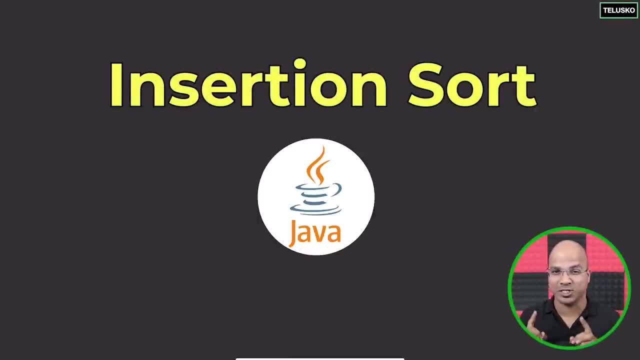 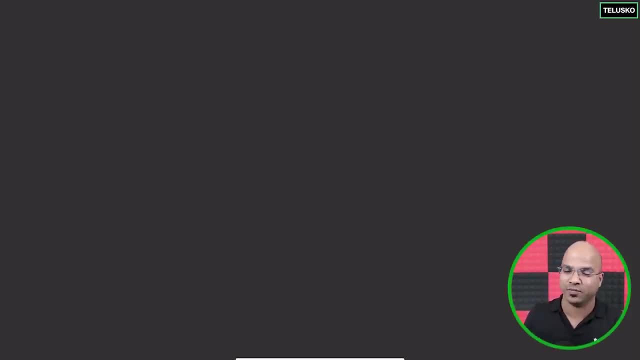 So let's try to implement insertion sort using java now. basically, even before we implement that, before write the code, Let's write the algorithm on the board and then we'll try to convert that into code. So what we'll do is, first of all, let's create some, let's get some values. okay, 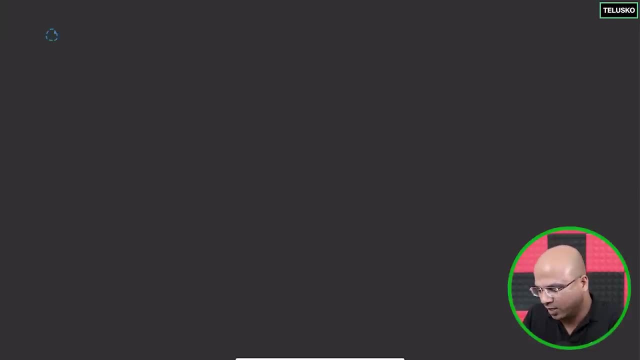 So we also need a array. so let's say I will name this as Array itself, arr, and then it will have some values. So let's let me create an array here and we'll take Few values. let's say we got Five values. of course you can go for more values here- and then let me just say this: values are three. 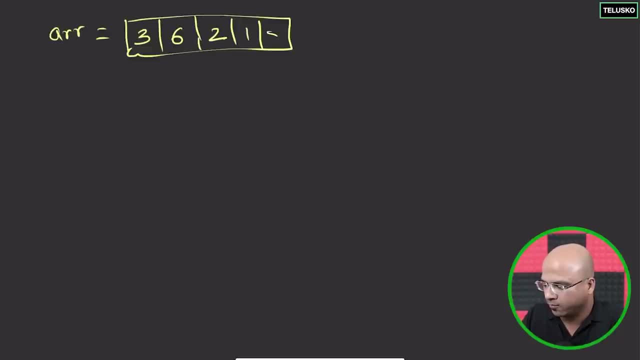 six, two, one, Five. okay, so we got this: five values. now I want some variables as well. so, as I mentioned before, we don't swap here Right, we do shifting of the values. so of course, to achieve that we need inner loop and the outer loop. 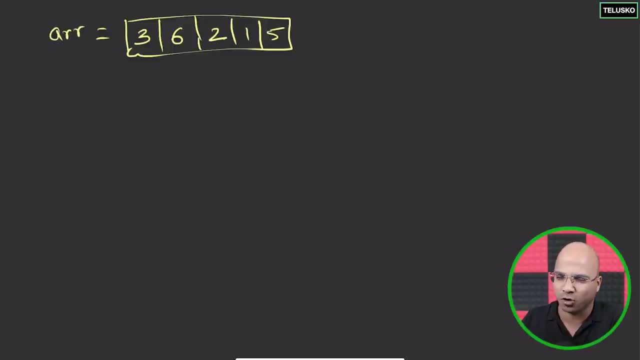 So let's say we got the outer loop, which will go for for loop. so let's say we have a for loop here And then we have to take a variable, which is I, for the outer loop counter, And then inside this we are going to have a while loop which will have, let's say, some condition of course. 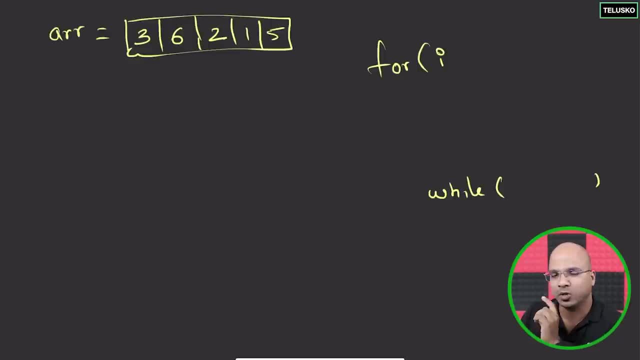 You can also go for, for and for, but then, when you talk about Insertion, using while loop inside makes much more sense, because we want to be, we want to run this based on the condition, Not on the number of iterations. okay, so this is your outer loop. Let's finish it here. 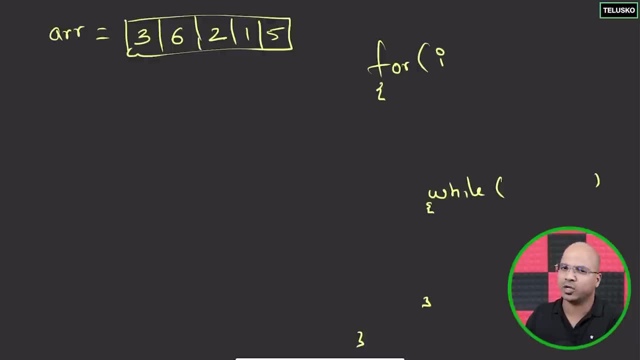 This is your inner loop. Let's finish it here and let's write the code there. now We need two variables, as I mentioned, of course, in the while loop. We are not going to create a variable, We are going to use one variable, but let's also go for J, So we need our I variable. 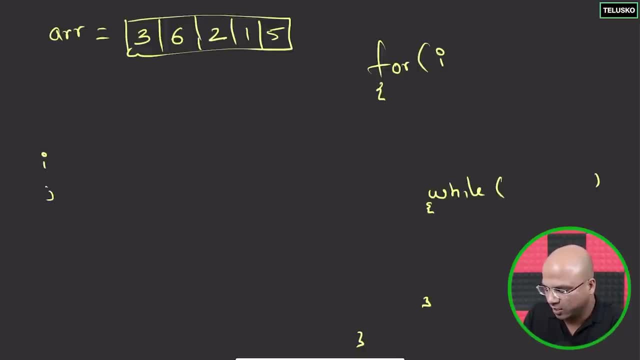 Let me just write: I here We need a J variable and we need a key as well so that you can store this value somewhere. So at one point you will compare and you will save it. now, from where we are going to start this? now, if you Want to understand what what we're going to do is where it's very simple. so initially, you will take your six as a key. 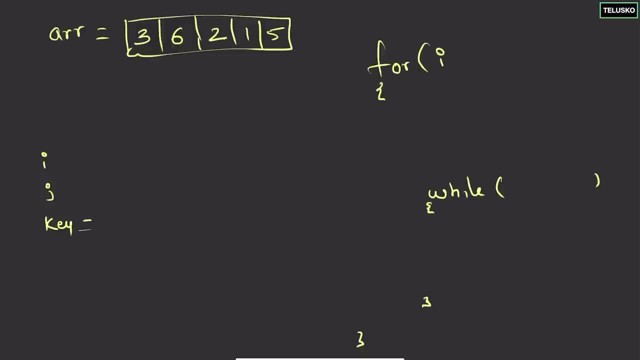 so When you write this variable will say: key is initially six. okay, now how you're going to get six? So let's say we take a variable I here and then we'll keep the J here. okay, So we're not going to start I from the first one. 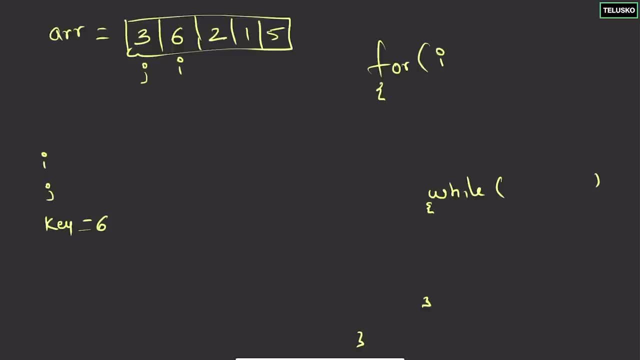 We are going to start I from the second one and then J will be the first value. now I will represent the outer loop and J will change in the inner loop as well. okay, So that's why we are going for I and J. We could have gone for different variable name, but we got used to I and J for the outer loop and inner loop, okay. 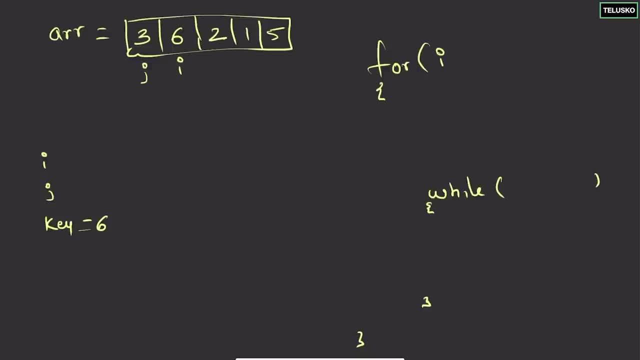 so now What you're going to do. so the idea is very simple: once you've got a key, which is six in this case, now How you got six, maybe we can do something like this: We'll say: ARR of I, whatever I represents, will save that in the variable K. 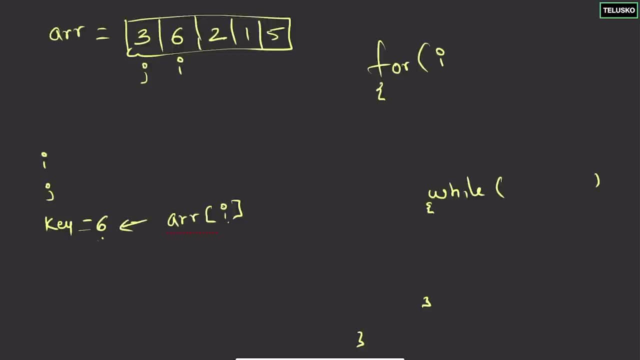 Okay, and then we are going to start J by saying J is equal to I minus 1, so I is starting from 1. So J is I minus 1. that means the value for J initially will be 0 and I is 1 now. 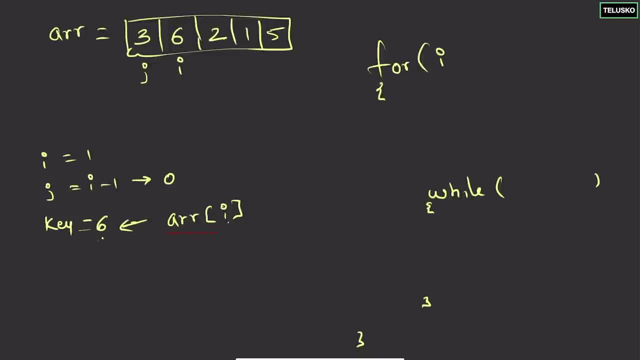 What you're going to do with this. It's very simple. you will Simply compare the value of J, which is this the first value. So we'll compare J with the key. if this value is greater than the key, Then you will do the shifting part at this point. 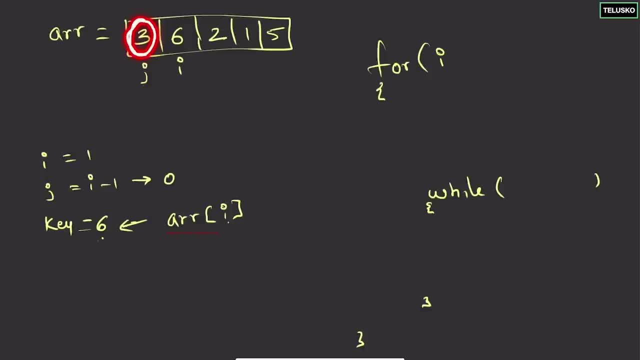 We don't need that right, because the value of J, where the J represents, is less than the key. Then you don't have to do any shifting part. So this is already sorted. Okay, but let's go for the next iteration now when you send it? next iteration? It's very simple. 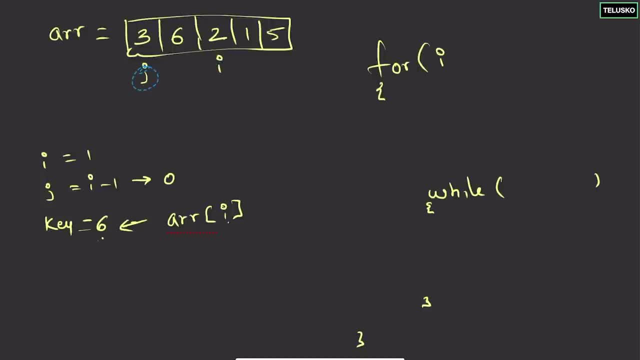 What you simply do is so you shift your value of I here and you shift Your value of J here, because we know that the 3 & 6- if you compare this to they- are sorted. Let's go for the next one. now in this, what you will do is you will check again. 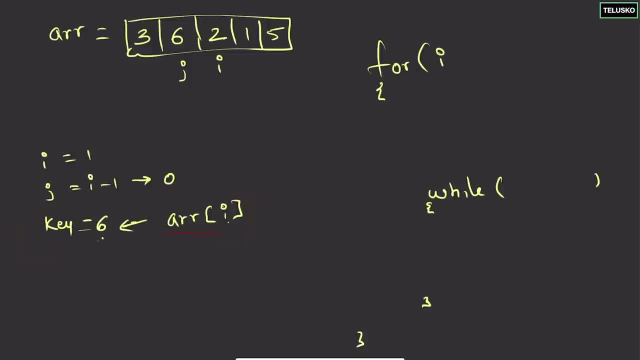 You will change certain things, right, if you can see. this will change, because now ARR of I is not 6, ARR of I is Basically 2. okay, so key is 2. now What about the value of I? even I is changed. I is now 2, so index is 2, so let me also write index so that it will make much more sense, right? 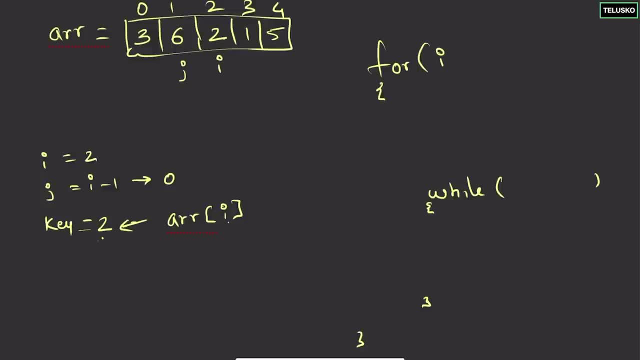 So that those are the index value. So I values 2. now what about J? so J is I minus 1, so J will start from 1. that's done. And now you will apply a condition. So what basically condition we are checking for? so, of course, if you write the code here, 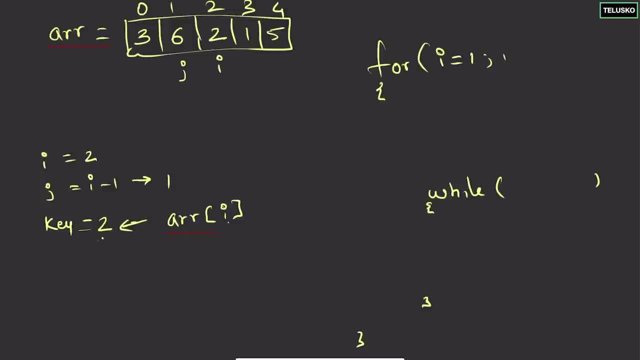 So I is initially starting with 1, We are now starting with 0, and then we'll go till I less than n, if the value, if the length of this array is n, And then we'll say I plus plus, Okay, and then we'll assign the value, Okay. Well, let's not write the actual code, Let's write some dummy code. 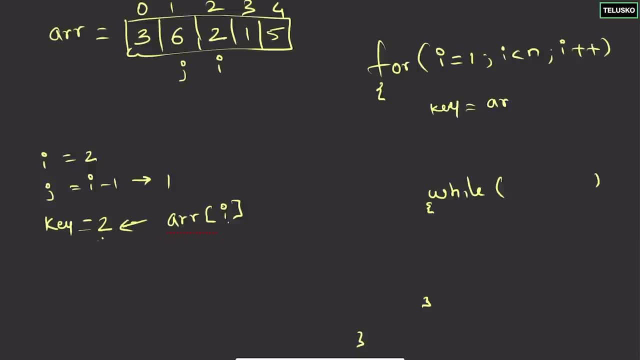 So let's say we got a key variable. The value for key is basically ARR, which is the array of I, and that's what we are doing here. That's one thing. next, We also need J variable. So we'll say J is equal to I minus 1. 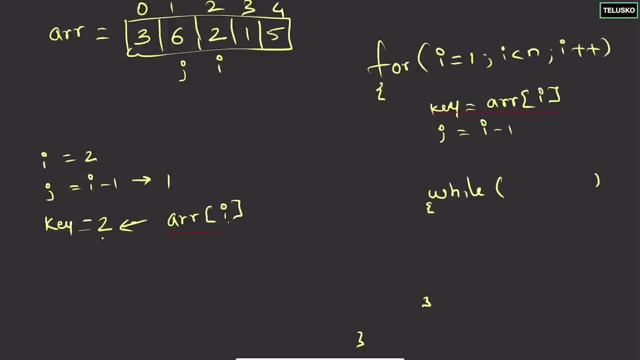 Okay, that's how we're going to start now, what you're going to compare in the while loop. So in the while loop, it's very simple: You will check for the ARR, So ARR of J, Let me just say, complete this here. So this: if this is greater than the key, because the shifting 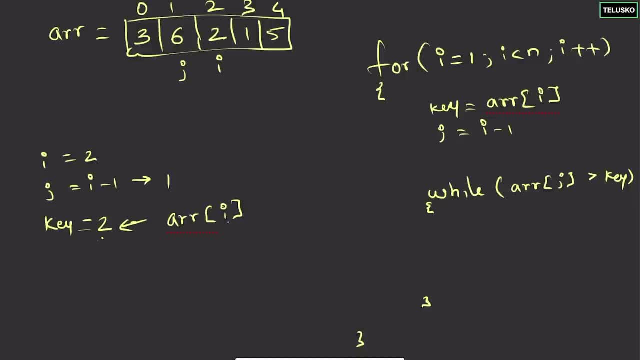 Part will come only when whatever is represented by J is greater than the key. So, if you can see, the key is 2 here and in this case, yes, it is greater, So 6 is greater than 2.. So what you do is you basically perform some operation. now, what I'm going to perform, 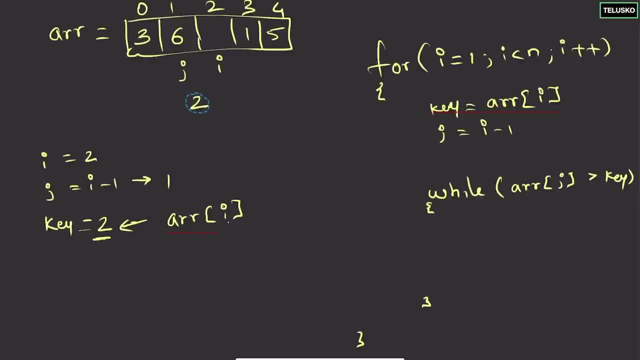 So basically, first of all I will take this key somewhere- Of course we are storing that key 2 in the key variable- and then you do the shifting. shifting of what? So you will first compare this 2 with 6, and now we know that we have to shift 6. 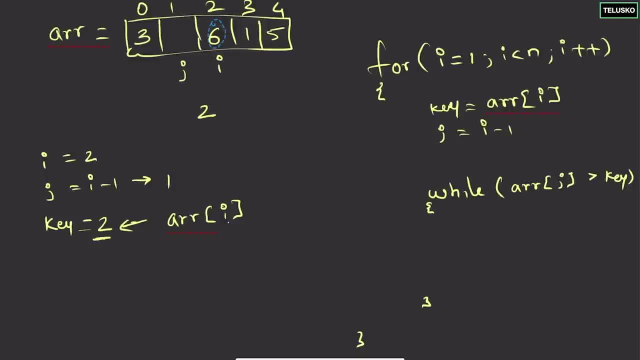 So you will shift 6 here, then That's one done, right, Can you put 2 here? We can, actually we can put 2 here, But the problem is we also know that we have to compare 2 with the previous value, which is 3 in this case. 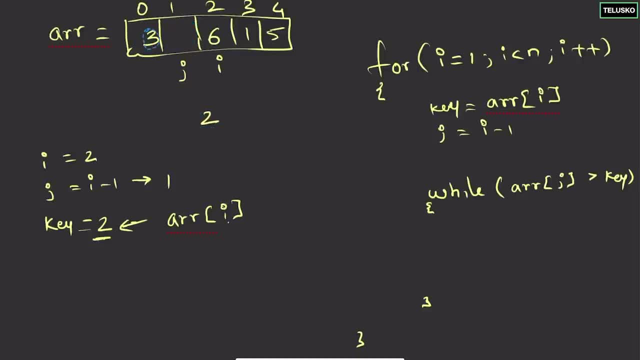 So you will not shift 2 there, but we'll shift 3 here. But then to shift 3 here, what we have to also do is we have to first shift our J here on the first location. That means we are also going to perform J minus minus, right? 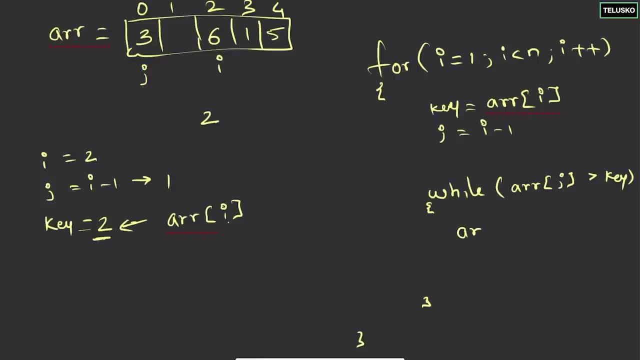 So what I'm saying is the first option you're going to perform is shifting the values, right? So how do you shift? you simply take the next one, Or you can take the next value. So initially J was here, right, So this value 6 is going here. 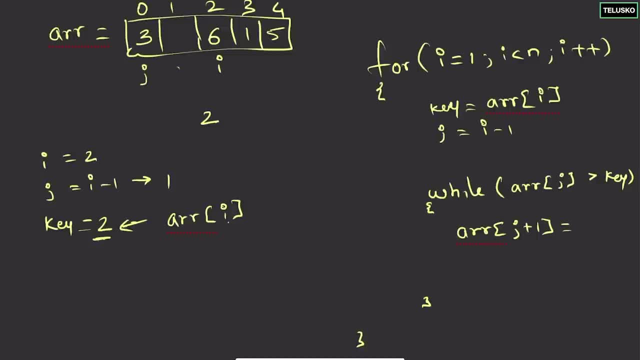 So that means what we can do is we can say: aRR of j plus 1, which is, in this case, 2, Is xRR. clear joke. By doing this, what you're doing is you're shifting J initially was here, which is 1, so index of J was 1 or the value of J was one. 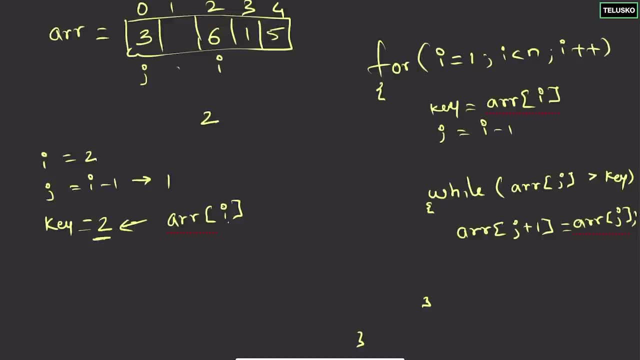 Then you're saying J of 2, I mean J becomes 2. then what you're saying is we are saying J plus 1, which is 2, so the value of 6, which was here, will move here on this line. that's a shifting part. and then you will say j minus minus, so you can say j minus. 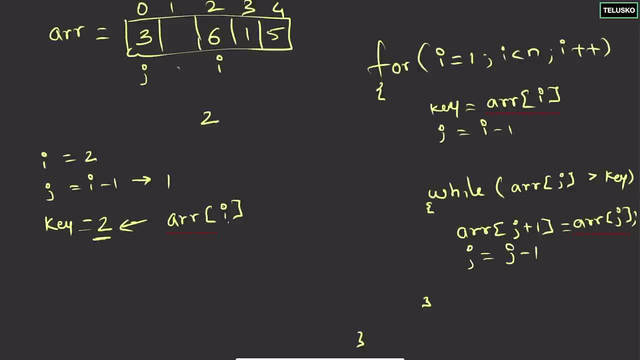 minus. or you can say j minus 1. it will both works. so this is the entire logic. you have right. but this loop will repeat right now. when it will repeat? look at the condition here. the condition is: whatever j, so we are shifting j backwards, right, j is now here, so we'll check if arr of j. 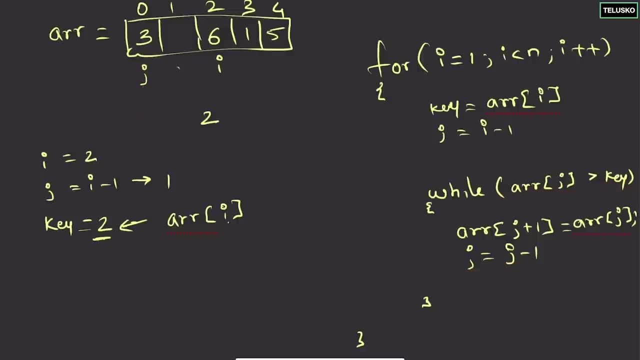 is greater than key. in this case, yes, you can see, the key is 2, arr of j is 3, so it is greater. so we'll shift. so how do you shift? basically, you do the same operation which is inside the while loop. so if you compare this operation, this is what it is doing, the shifting part, right. and then we know: 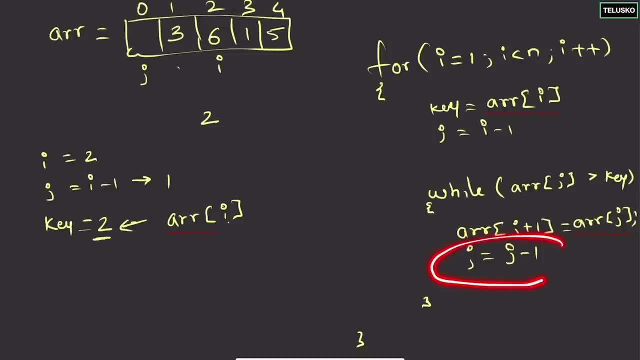 that, of course, if you can see, here we have one more step. you will do j minus 1, which means your j basically moves 1 here, because when you reduce the value of j, it becomes- it became 0, right, and then again you're doing it, so it will become j, j becomes minus 1, so we have to stop it here once. 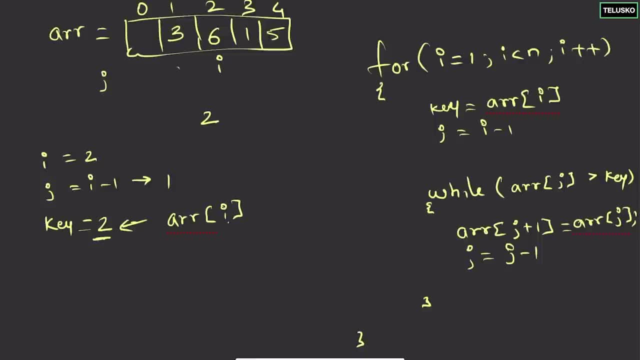 the j becomes less than 0, we have to stop. but don't you think we have to also add that condition in the while loop? so we'll do that. we'll say: and j should be greater than equal to 0. okay, this is one condition we have to add. if this is false, 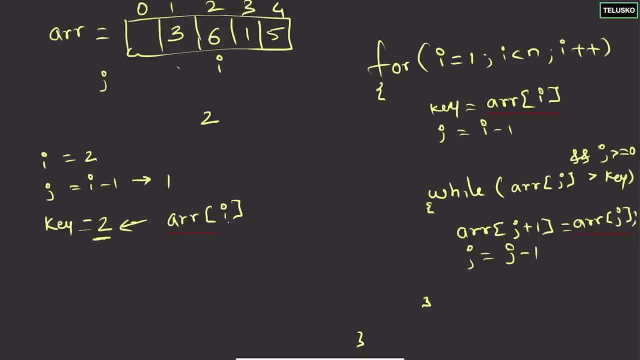 if j is not less than or equal to 0, then you will do the last, last step. the last step is very simple: you move your 2 here, and the way you can do that is by saying arr of j plus 1, because j became minus 1. we don't want minus 1, we want 0 is equal to k is equal to key. so, basically, this is where. 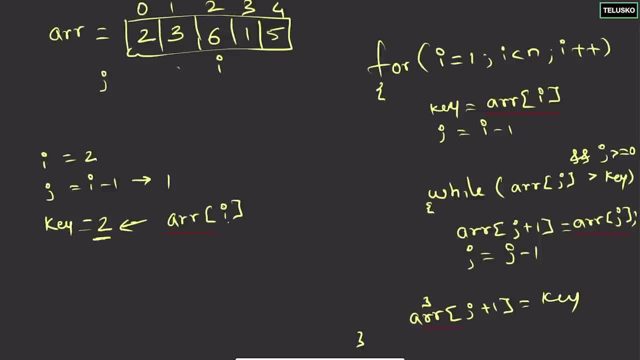 the value goes first. now, by doing this we were able to sort the first three values. now what next? of course you will increment the value of i. so when you say increment, that means the value of the i variable goes here and again. for the next situation: j goes i minus 1 right. 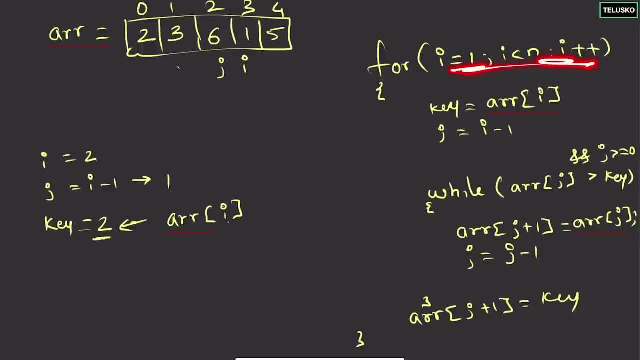 because of this, basically for the outer loop, the i value is incrementing, but the j value is just before. i and again you, just you do the same things. what are the same things? you first check: if the key okay, we have to update the key as well. now, how do you update the key? now? the key value is arr of. 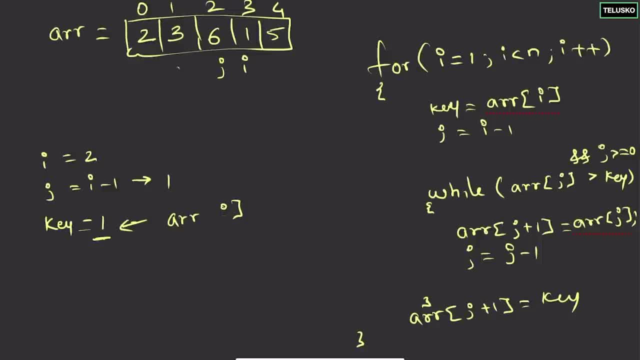 j. so the new key is 1 and j i is what, i is 3 and j is 2. okay, new key value is 1. you will compare if the arr of j- this is the condition we're checking now- if arr of j, which is in this case is 6, is. 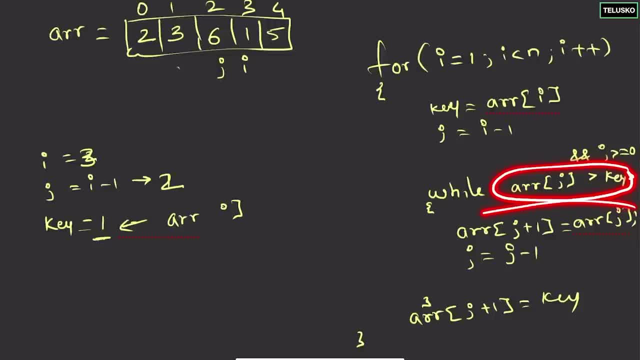 greater than the key in this case. yes, you perform this operation. what is the operation? it's very simple. let's keep this value somewhere. you start shifting 6 here, 6 goes there, and then your j comes back, j comes here, and then you start shifting 6 here, and then you start shifting 6 here, and then 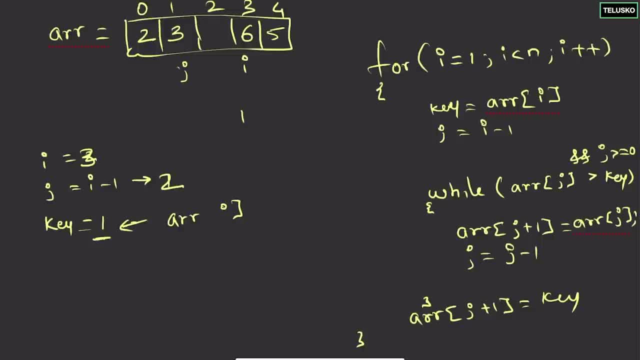 you start shifting 6 here, right, because of this step here, right. and then you, you again check if arr of j is greater than key. yes, 3 is greater than 1. again, you will shift 3 here, then you shift j here. then again you shift 2 here, then you shift j here, and then now j becomes minus 1. let's stop. 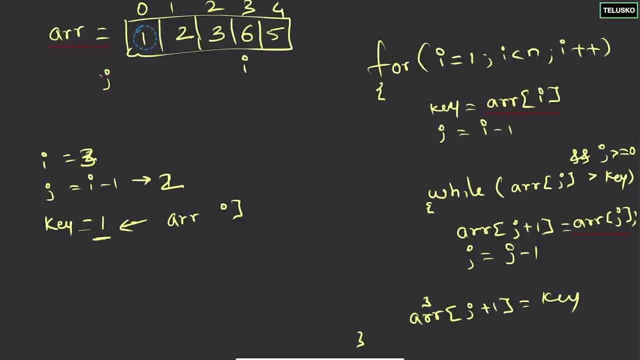 the loop and shift 1 here. you can just do the same thing for 5. let's do that quickly. so what you will do is you will shift the value of i here, which means certain things are going to change. now this i becomes 4, this j becomes 3. the key value now is 5. right again, you do the same things. you keep your j here. 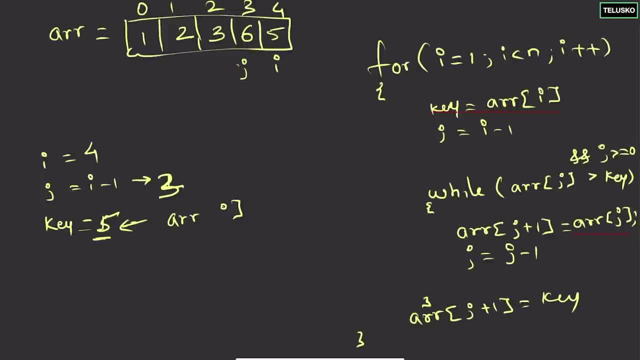 because j is just i minus 1. then you compare if the arr of j, which is 6 in this case, is greater than the key. yes, let's do the shifting. now, how do we do that? let's move that here. and then we have to shift 6 here. j goes here. now again you check: is the arr of j is greater than key? no, it's not. 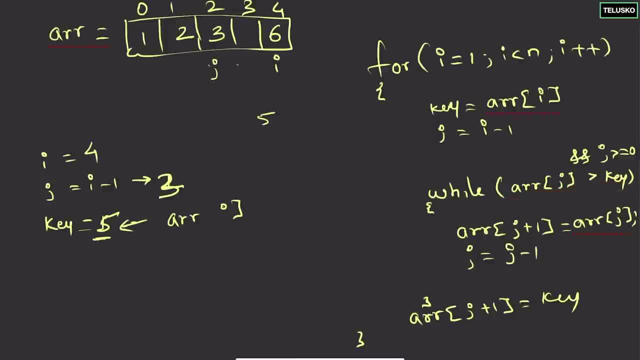 there. so you will just simply do the same thing again, you do the same thing again, you do the same thing again, you do the same thing again, and then you will shift your j. we move this j particle that we have, and then we will do, becomes 4 here to join j, so we can. 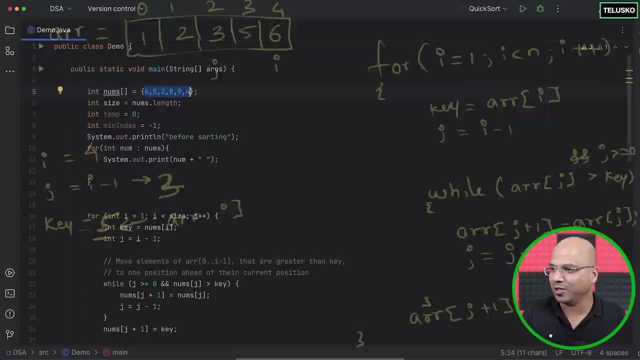 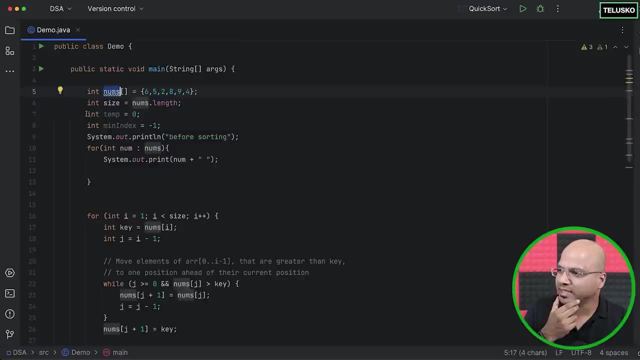 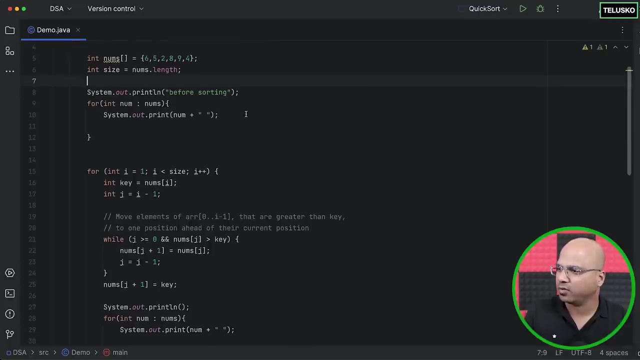 бEN. Missing j is a Joind in the loop we need. we will remove the exp of the two j's. now we will do the same thing again. this is basically the older code which we had for selection sort, if i'm not wrong, and this is the before sorting elements. this logic is going to change for sure. 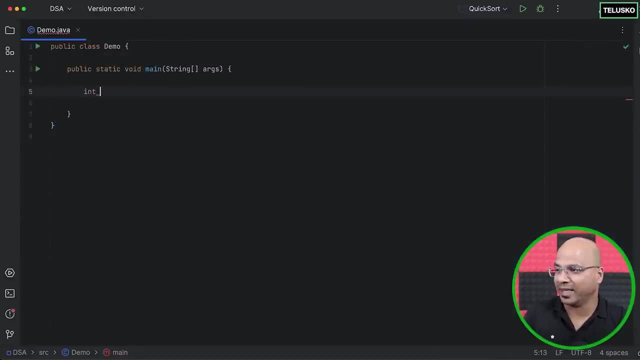 okay, so let's write the logic. it's very simple. you create a array. so let's say this array is arr, is equal to. let's have some default values to it. let's say five, six, two, three, one. this time we are going for only five values and this is an array. okay, what next now? basically, as we have, 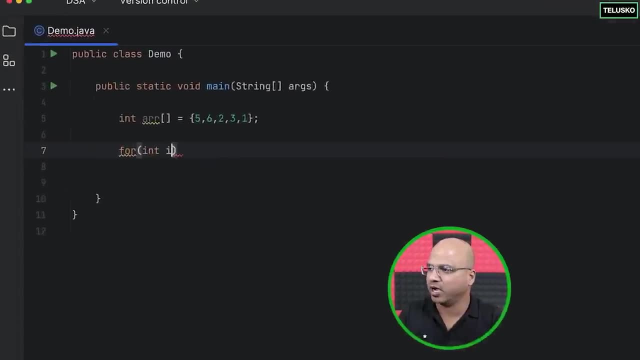 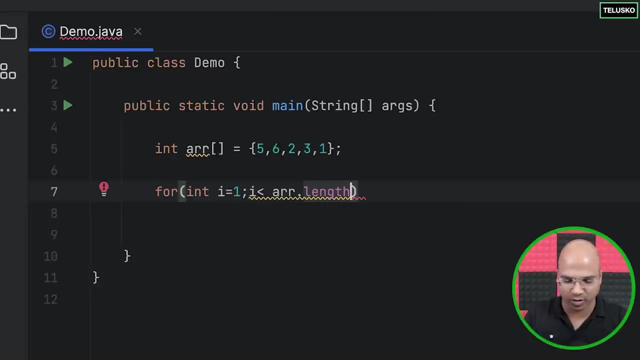 written in the board. let's take a for loop now. the for loop is going to start with i. i is equal to one, and we can do that quickly now. it will finish at n, but we don't know what n is, so we can say arraylength and we can say i++. right, that's one done, and now okay, let me just remove. 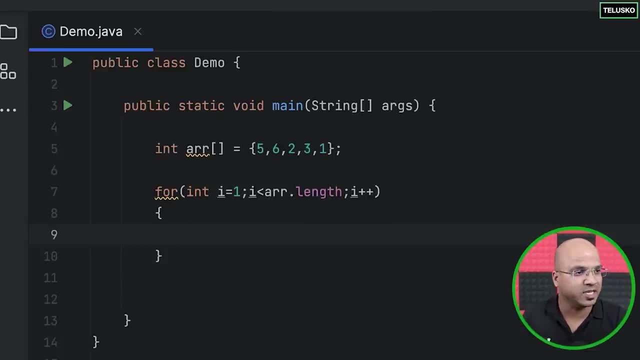 some space in between. okay, now, what are the extra variables we need? basically, we need two variables. we need key- the value for key will be arr of i, which we have done earlier. and then we also need j, and we know j is j minus one. you know this. this is what happens when you know the algorithm on the on. 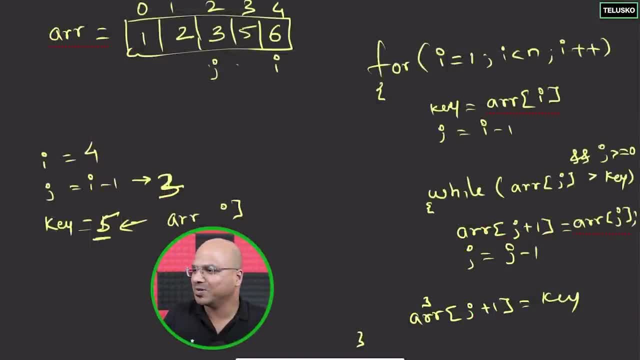 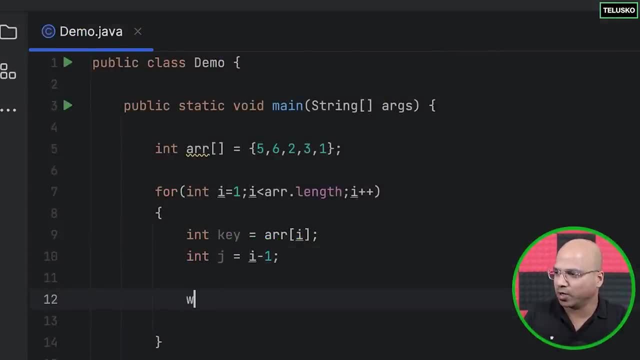 the board. right, i have a, i have a board with me. so, okay, those are the things we need. okay, not j minus one, it should be i minus one, and then you do a while loop, because this is where you do the iteration. we have to make sure that j is greater than zero. that's one thing, and we need to also. 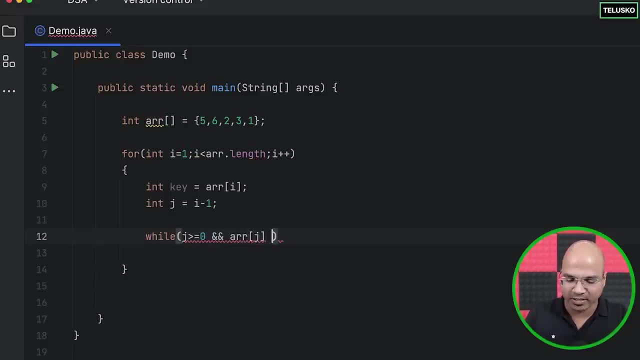 check if arr of j is greater than key. in that case you will execute the while loop. so you will do certain things here now what you are going to do inside this while loop. so basically, you have to do the shifting right. if it goes inside, you will say arr if j plus one is equal to arr of j, right. 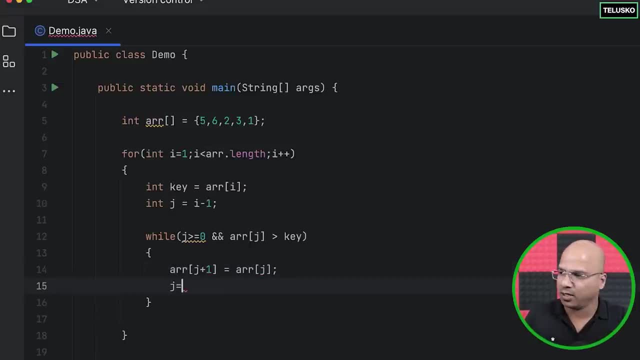 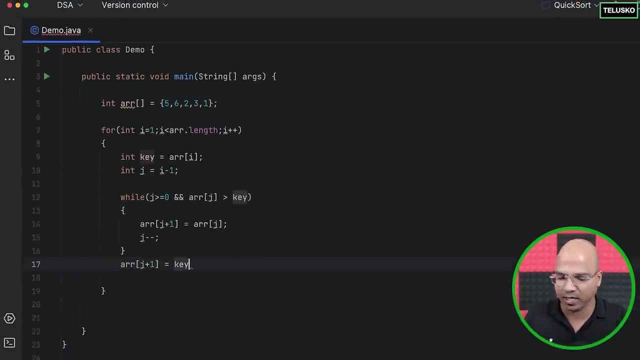 and also you have to reduce the value of j, so you will say j. we can even say j minus minus. syntactically that works. and for the outer loop you will assign the value for key for that particular empty location, and the empty location is defined by j itself. so j plus one is equal to key and i 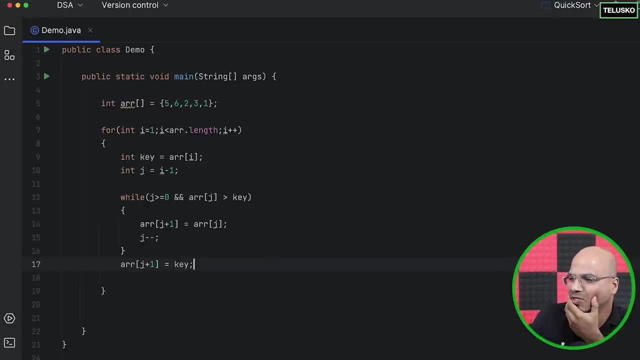 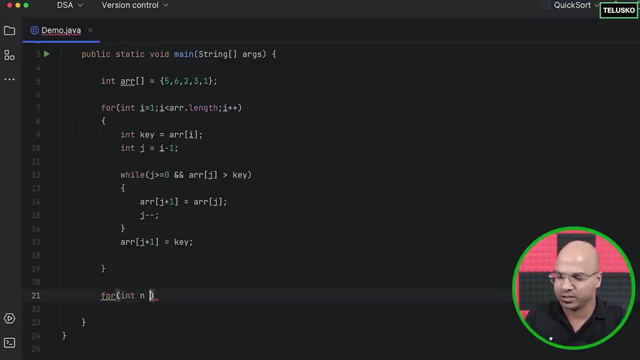 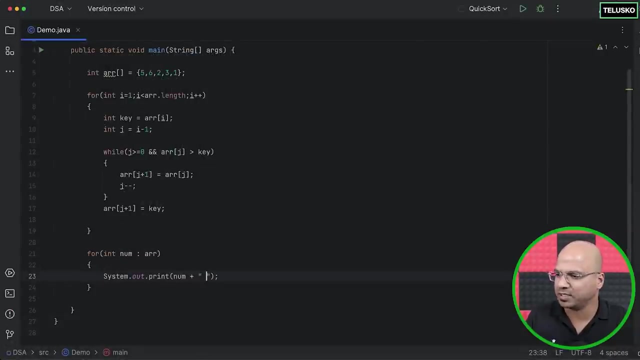 think we are done. so the code is so short, let me check if that works. what i will do is i will just print the values here. so i will take a for loop and i will say int, num from array and let's print the values. let's print num. i don't want the new line, i would just want a space here and let's see if that works. 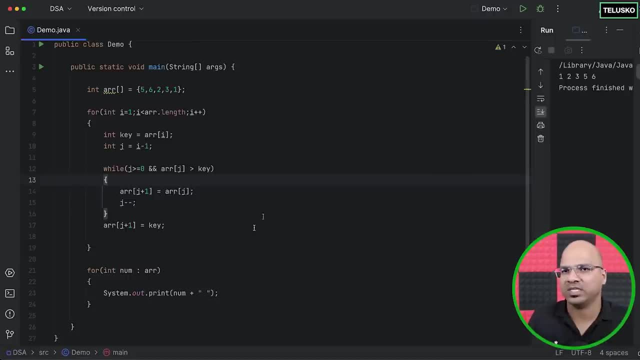 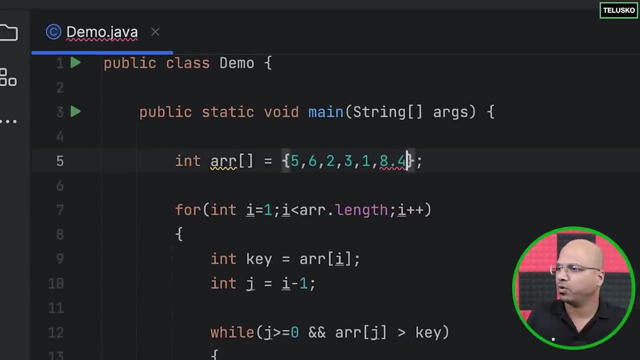 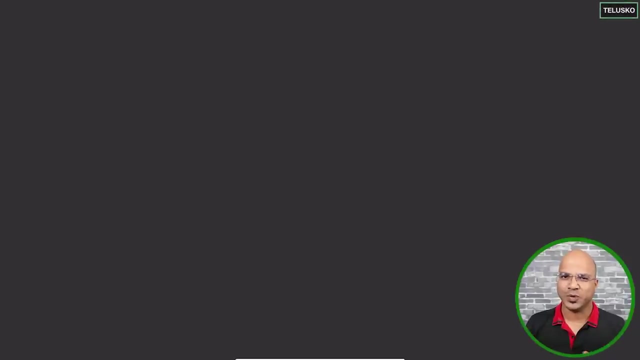 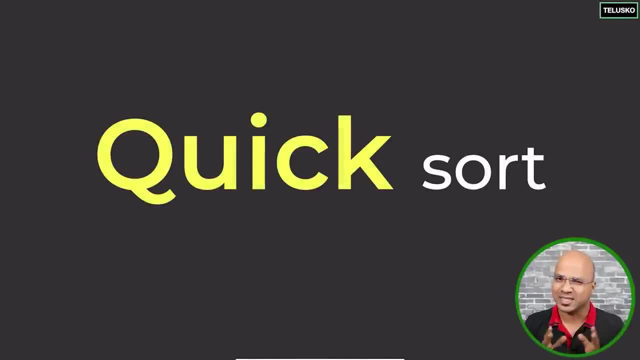 another sorting algorithm, which is called a quick sort. so the thing is, when you talk about sorting algorithms, the idea here is to explore different algorithm and we'll see how efficient it is. now, when we talked about the other algorithms which we talked about till now- bubble sort selection. 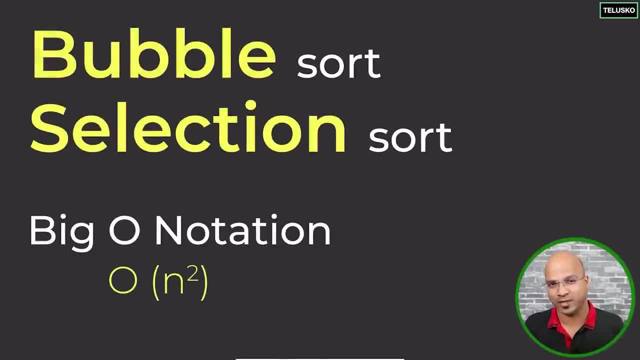 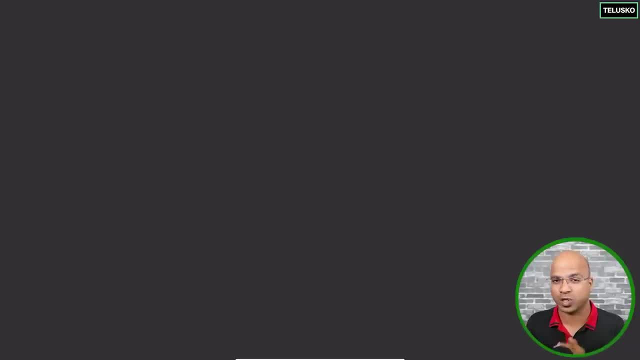 sort, they have a big o notation of n? square, which we don't want right. we want to make it faster or efficient. now, in that case, we have to explore some other algorithms and one of them is quick sort. now, in the best case, the quick sort goes for n? log n, which is much better compared to the n? n square. 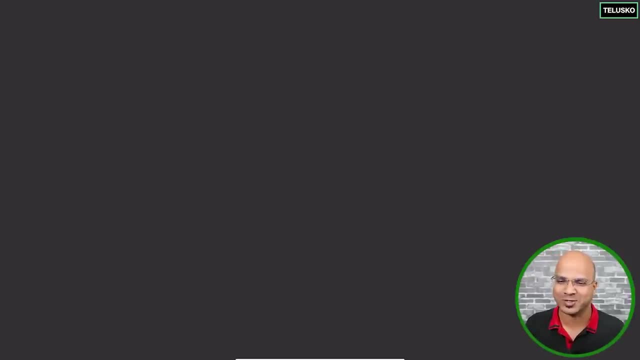 but in the worst case also, it goes for n square. so in the worst case, yes, it is almost there, but on average it is n log n, or you can say the best case. so at least we are happy in the best case and in the average case. now let's say what is the best case and what is the worst case and what is the. 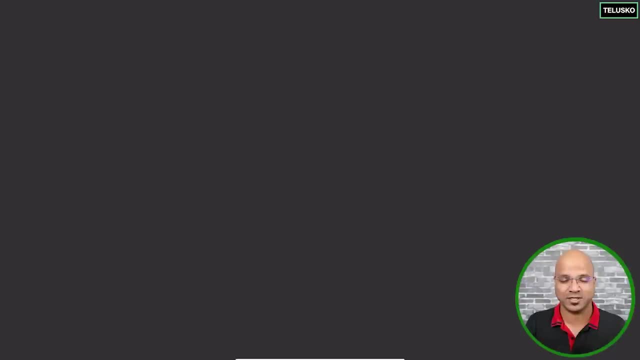 best case is quick sort. so actually it uses multiple things, so let's talk about that first. the first thing is divide and conquer. so basically, till this point, when we talked about bubble sort or selection sort, we were doing the algorithm on the entire collection. so let's say: if you have a 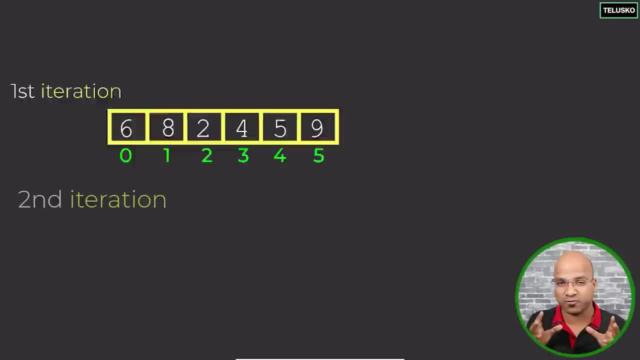 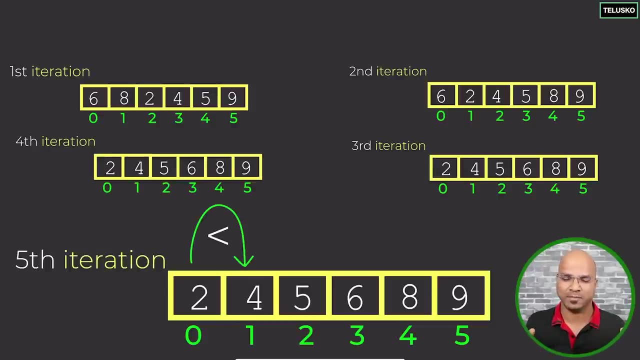 list of values, which is six values. so what you do is you perform the operation of bubble sort and all the sorting techniques which we have done before applied on the entire list. but what quick sort says, let's do divide and conquer, which simply means divide your problem into multiple things. 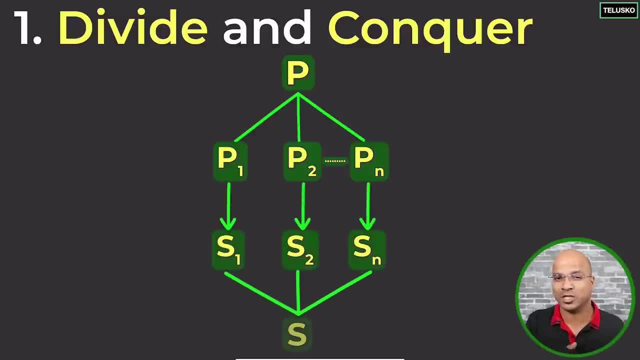 and solve the problem or sub problems individually. so what you're doing is you're dividing it, you're solving it and at the end you will combine it. so that's your divide and conquer. so in this case, if you have six values, let's divide the values into multiple sub problems and then sort it and then 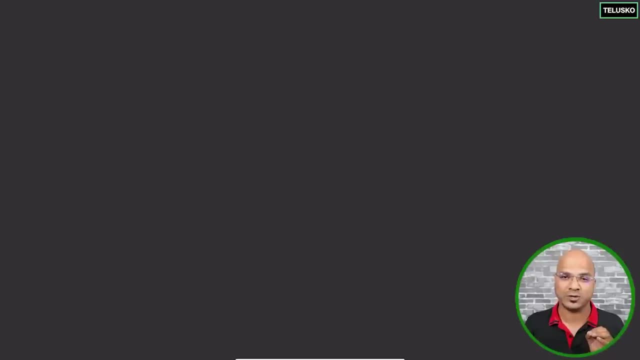 combine it. so that is your divide and conquer. next it you. it uses something called a recursion. of course you can also use recursion in the other other algorithms, but here it works with recursion. now, basically, what is recursion? so when you call the same function by a different function, 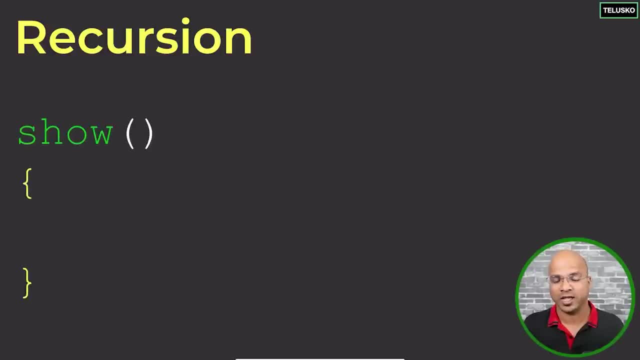 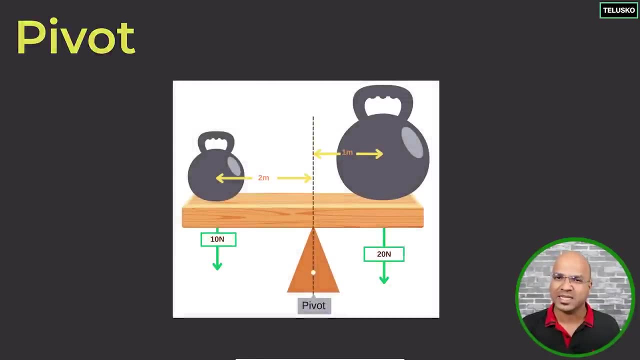 itself. so example: let's say the function name or the method name is show and if you're calling show inside show, that's your recursion right. and next we have to understand the concept of pivot. now, basically, pivot is something called a central point of a problem. okay, so let's say you have 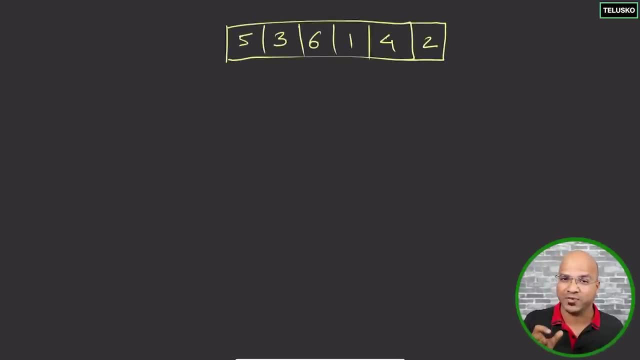 this entire list here, or the array. now you have to find a pivot and then, based on that, you will perform the operation. of course, it will make much more sense when we start, but remember we have to work with the pivot. so those are the things you have to remember: divide, conquer, recursion. 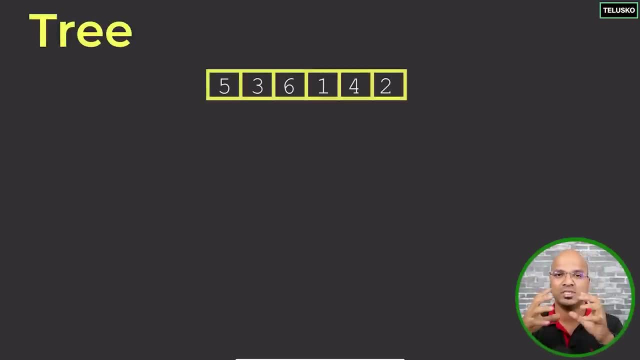 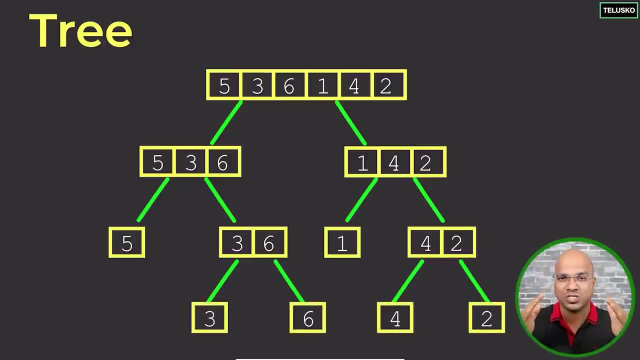 and pivot. there is one more thing, which is the tree. now, basically, when you say you are dividing your entire list into subsections or sub problems, what you're doing is you are creating a tree structure. okay, so once we start with the diagrams you will make, it will make much more sense. but 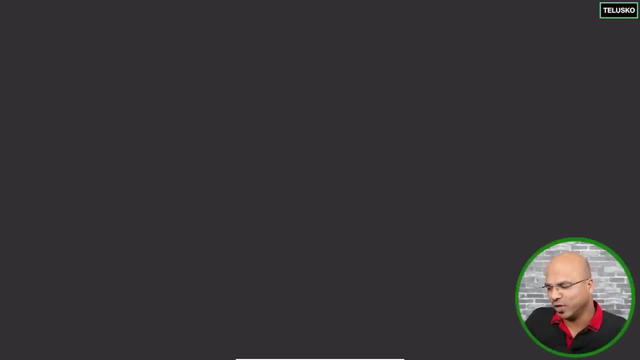 these are the things we have to remember. so let's see how your quick sort works, and then we'll try to convert that into algorithm and then we'll see how to write a code for it. now, the basic idea here is: let's say you have a list of values, so we are discussing about quick sort, so let's say we have 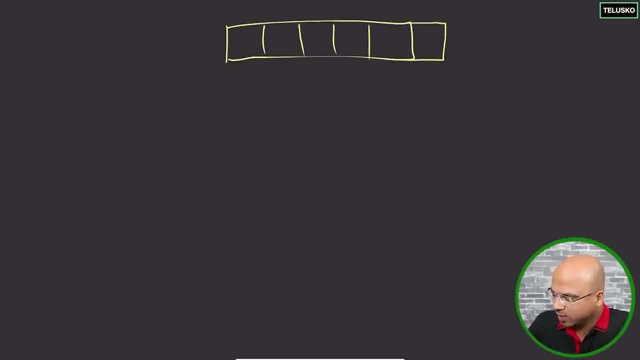 a list of values. so let's go for six values here and i will say: this is five, this is three, six, one, four and two. so let's say we have the six values. i'm not sure will it really make sense to use this example, but let's get started now with this six values. what you normally do is you do divide and 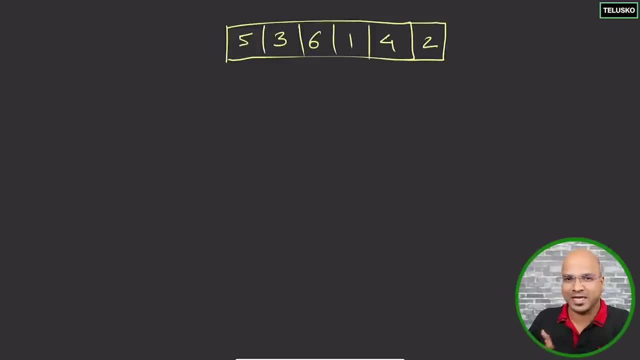 conquer here. so the basic idea is break the entire list into sub problems. okay, something like this: maybe we can. we can create uh, two, diff, two different arrays. here we'll be having three, uh, i mean five, three, six. here you can have one, four, two, and then you can again divide this maybe. 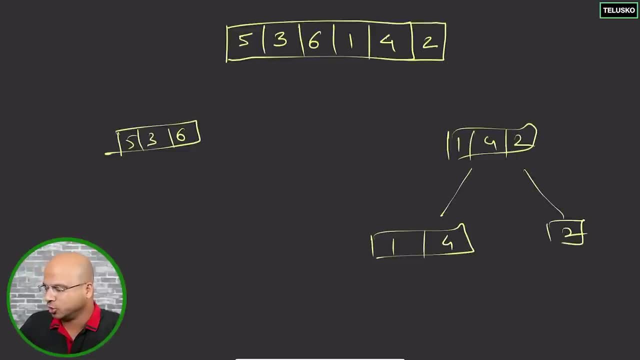 you can have one and four here and divide this into two. here also we can have five, and then we can have another array which is three and six. so we got these two arrays from the big array and then you create the shorter format of it. so at the end, what you're doing is you're creating the 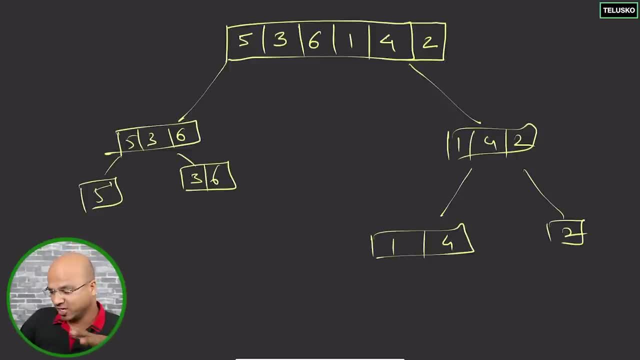 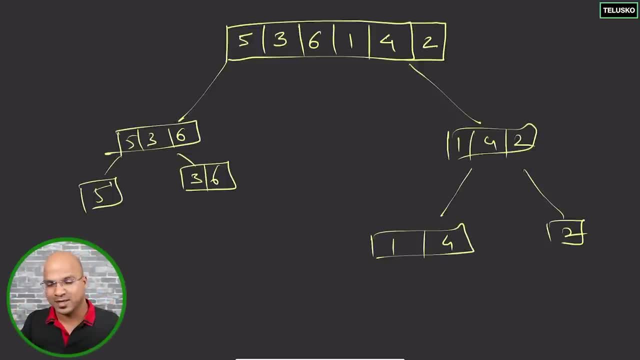 performing the sorting on each section in sub problem. that is your recursion, but is it the real thing? no, so basically, we talked about the idea, but how do you divide the array? randomly? i just divided the array, but that's not the main idea. but we have to divide, but not this way. so how we 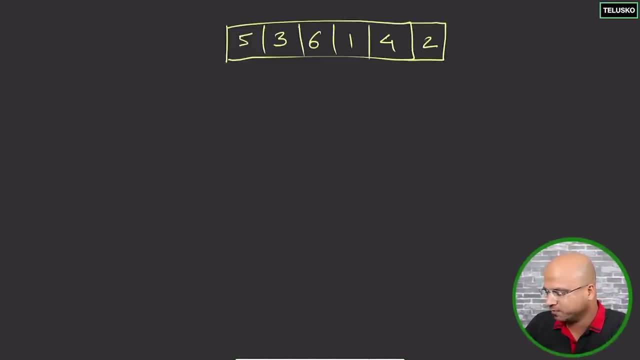 are going to divide this. that's the question. let's remove this and let's go with the values here. the idea is: you want to divide- for sure you will divide this into two, and then you divide this into two parts- but you need to find a point from where you will divide this, and that point is: 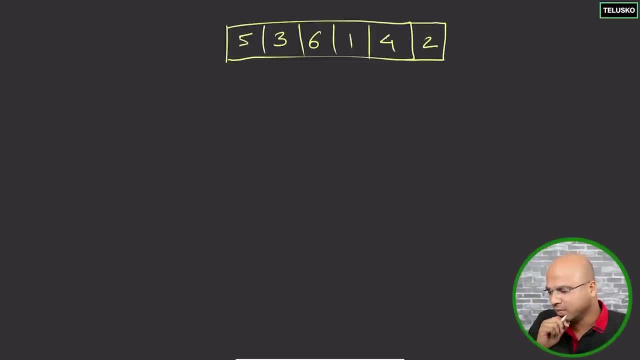 basically your pivot. now, how do you find a pivot now? basically the reason: we get this partition or pivot to do the partitions of the array right now. should we pick up one now? that depends. so even before you divide, you have to do one more thing. so i'm saying pivot, but then that pivot should be a. 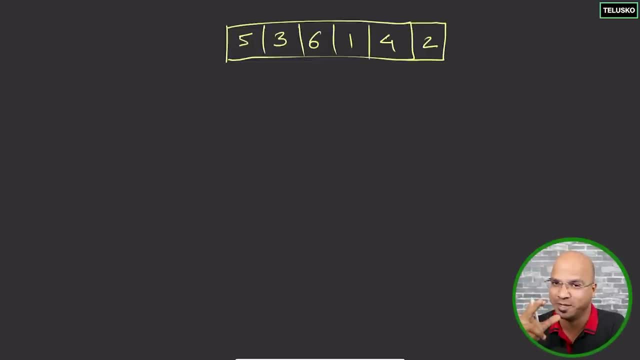 point which is at the right position. let me repeat: the pivot is a point in this array which is at the right location. now, if you see this, after this sorting what the values you will get. so you will get values like, let's say, i will just write it in shorter format now, so you will get one, two, three. 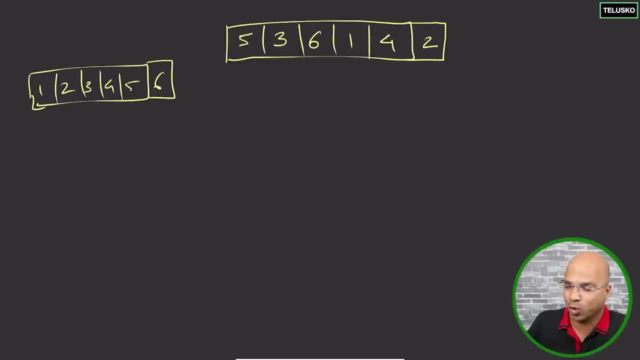 four, five, six. this is the output i want. okay, just went for the sequence of numbers here, but this is the output. so this is the output which we want from this input, which which we have the bigger array here or the big size which i mentioned. okay, so if you talk about the value one, two, three, four, 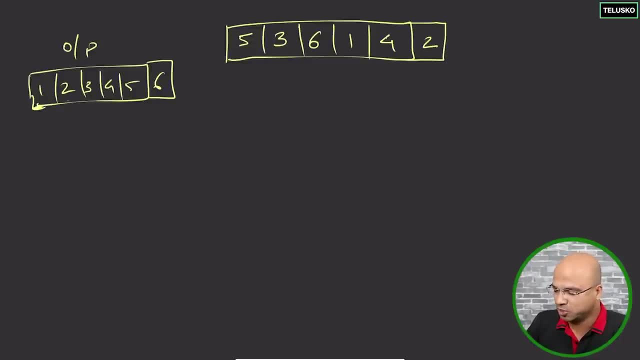 one here, so one should be at the first position, two should be the second position, three on the third position, fourth, fourth position, fifth, fifth and sixth right. so they should be at that position now, since we have taken those values, and that's why it might be confusing. but you got the point. 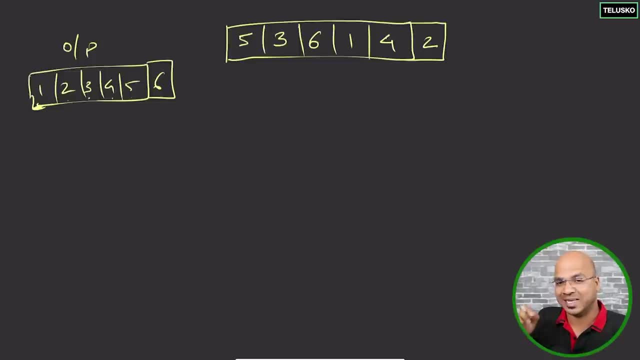 right. uh, it doesn't matter what your values you have, it should be in the ascending order. so the first value, the smallest value, should be first, and then at least goes on. okay, now we have to make sure that at least you will you find one point from here, or one value which is at the right. 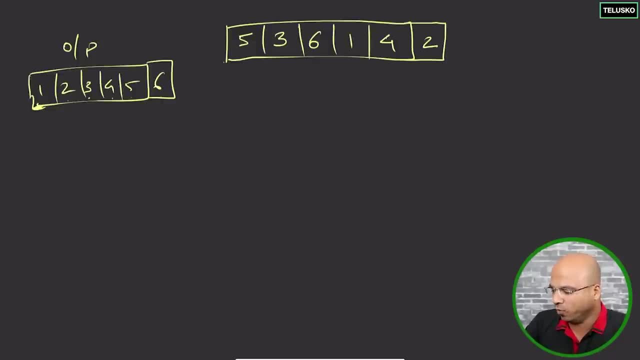 position example. let's say: uh, let me, let me take four. now four is it at the right position? the answer is no. four should be here right. so instead of one it should be four. then we can say four as at the right position. now, if you want to understand this with an example, so let's say you're in a classroom and 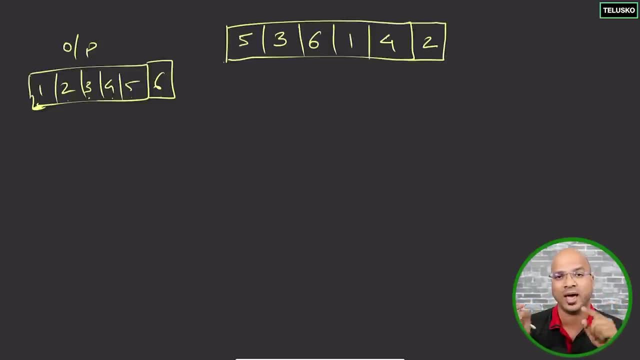 then you have multiple students there, okay, and then you want to sort them based on their height. there is one way: as a trainer, i can be there and i can say: okay, you go there, you go there, and that's what we have done in the bubble: sort. right, i was controlling it. but what if student can sort? 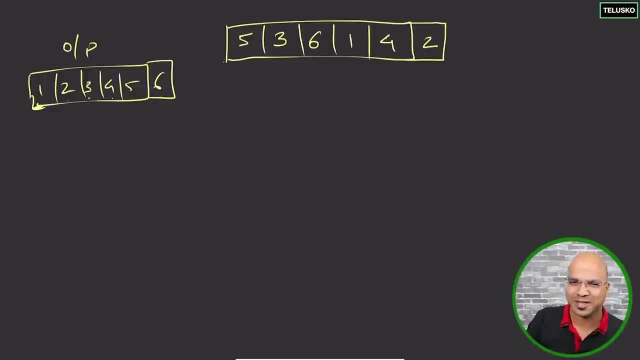 themselves so they can compare each other and they say, okay, i should be here, or i should be here, and they will move. now one way is one person can sort them, but then we don't want it. so what we want is what if the students themselves can get into the right position, that that will solve the problem right. 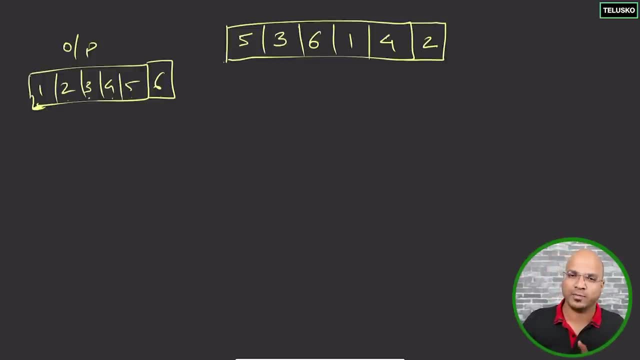 okay, but how we are going to do here, how they will reach to our right position. now what you do is initially we don't know the position right, so you can take any value, normally we can. we can find the pivot. so for the first iteration we what we are trying to do is we want to make sure at least one value is at the right position. 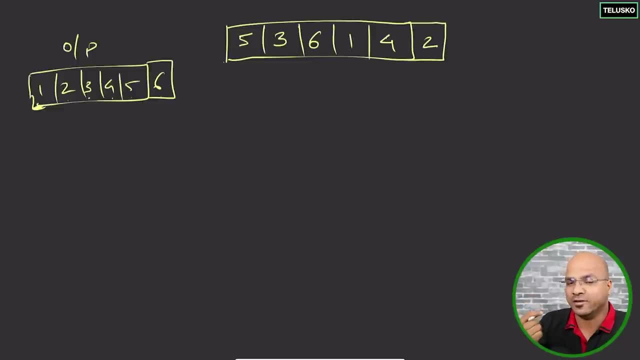 so that we can divide the array. now, which value should we take? technically, if you take the average value, or if you take the middle value example, if you, if you go from one to six, the mid value is three or four. right, so if i can take three as my pivot, it will be much easier for me to divide the array. 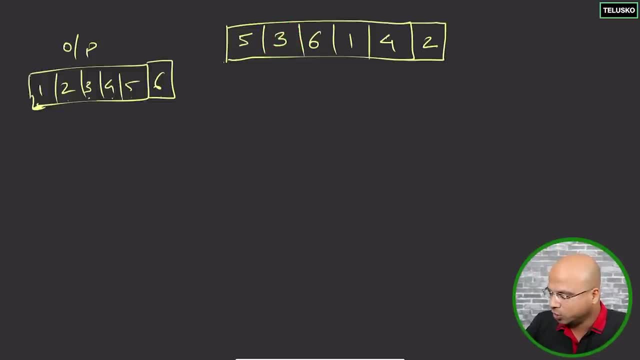 so what will happen is, if i take three as my pivot, then three should be coming here, right. so three is the right position for three. right, but it's not. if you start with the area, this is not at the right position. but if you get to the right position, we can divide into two parts, right? okay, so that's the. 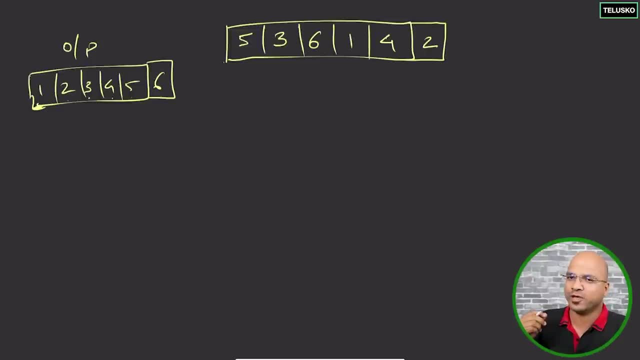 main idea: how will you get that there? so normally what you do is if you can find a good pivot, and that's very difficult to find, because how do you know the mid value? since we know the values here, i can find the mid value, but as a program or the software, they don't. they don't have any idea what. 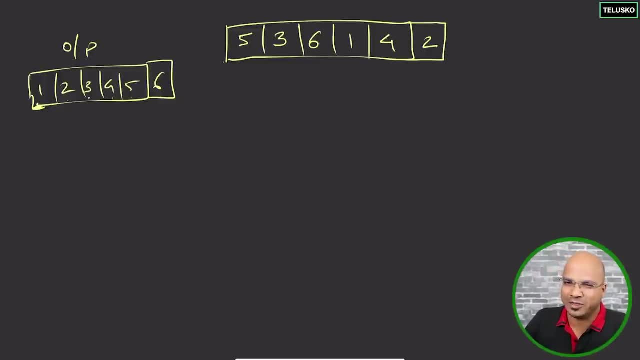 are those values are. so what we do is we randomly pick the pivot. maybe you can pick up the pivot, let's say, between somewhere, anywhere if you want. so you can pick up this one, you can pick up the six, or you can pick up the first value, or you can pick up the last value, or what you can do is you can. 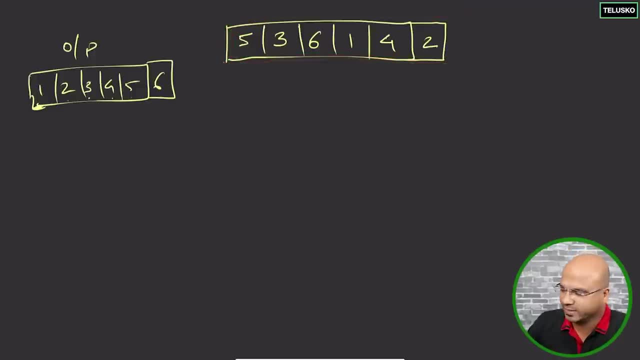 you can just add all these values and divide by six whatever value you will get. so try to find the average of it. that's what we can do, but again, that's a lengthy process. normally- which i have seen- is they go for the big, the last value, not the biggest, one last value, because we don't have any. 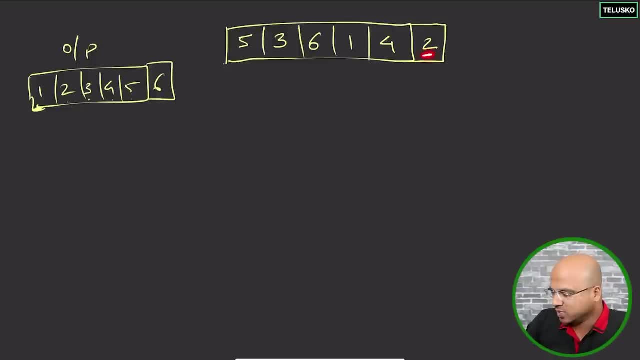 idea what's the biggest value is, so we'll go for the last value. okay, so this is: this becomes your pivot. that's the first one, and then the second one, and then the third one, and then the fourth one, and that means we need multiple variables here. now what variables we need, so i will just write: 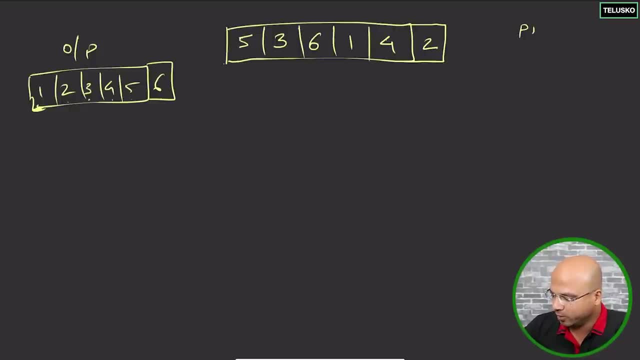 variables here. so the first variable we need is a pivot variable. so we'll say pi, okay. and then you need few more variables. you need a variable i for the positioning- again, we'll discuss what this positioning is. uh, then we'll need a j which will track, which will go through each element, and we 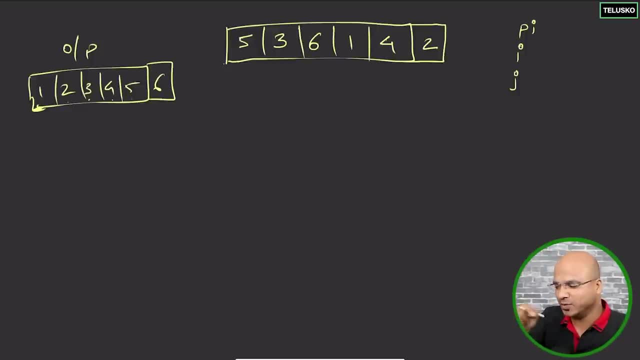 have done that in the sorting right. so when, when you jump from each value, that will be done by j. and then, of course, we also need array here. so let's say: this is arr, this is your array, okay. and let's have the index value, so we'll say: this is zero. one, two, three, four, five. those are the. 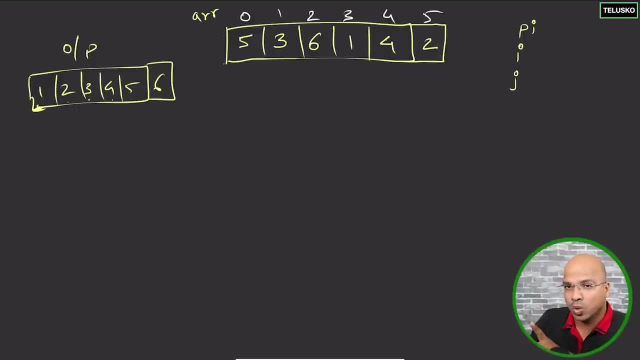 index values we have. apart from this, we also need a low and a high variable. okay, so we'll say l and h. so let's say this is l and this is h. now normally we can say h is the last value, or we can say it's. 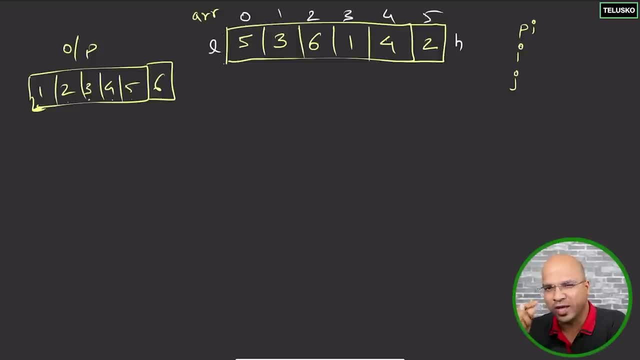 a length minus one. so we can say that. so we have a low and we have a high. so low starts from the first and h is the last value. now how do you perform the operation? it's very simple. first you find the pivot. now we know that we are going for pivot, which is two in this case. so what you? 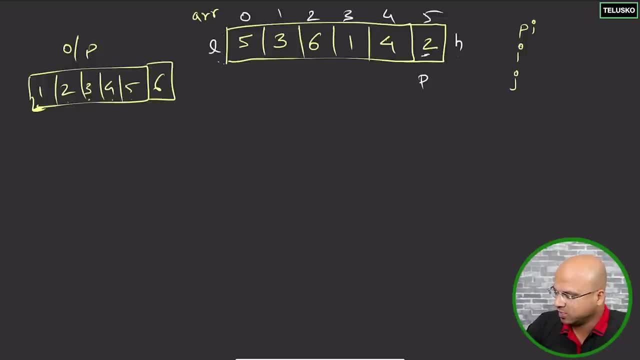 will do is: let's take this two as the pivot. so i will say: this is p, so this is referencing. this is referring this two. so pi variable at this point is referring two. so i will say: this is two in this case. and then we need two variables. so let's take variable i now by default the value for i will be. 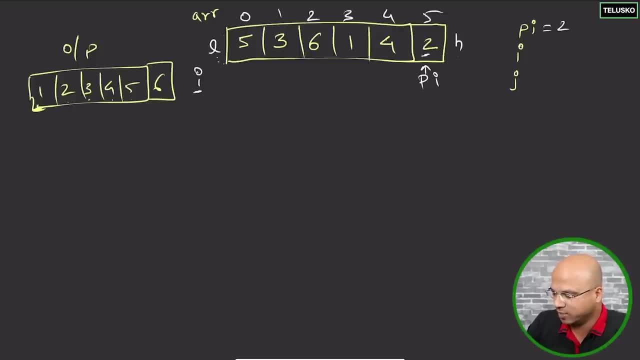 lowest value minus one. so let's say the i value is here at this point. you know what i will do. let me just remove this portion at this point because let's keep this slate clean. so we need an i variable, and then we need a j variable. so j will be here to start with. so i will be here. 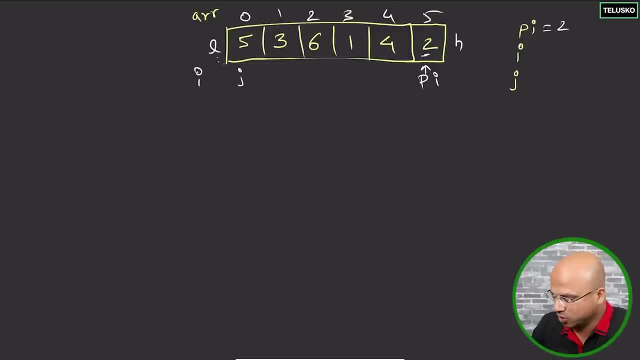 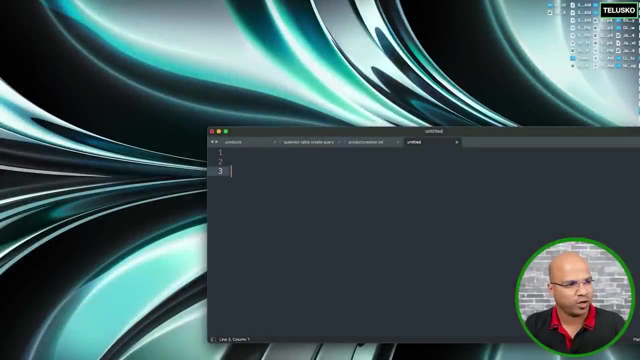 at the minus one position. j will be here at the zeroth position, and then what you do is you basically run a loop where, of course, the i will also increment. but the main loop here we want is for j. okay, so we'll take a for loop for j. okay, so let me write the code here. so what we want is, of course, 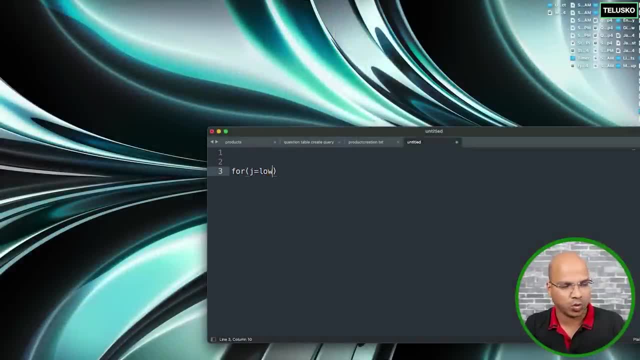 the rough code. so i will say: for j will be starting with low. okay, that's what we are doing here, and then j should go till n, but then we are not using n variable, right, we are using variable high. so let's say j less than high and j plus plus. now what you are going to do in this, inside this loop. 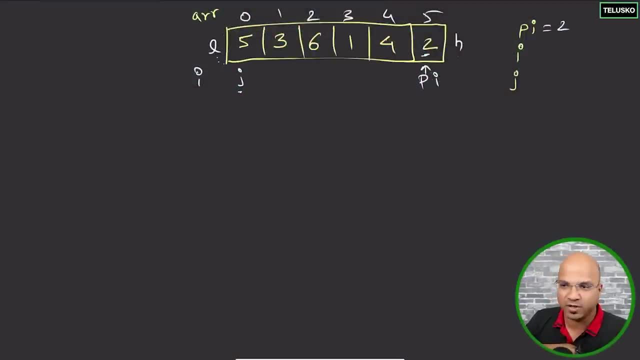 so, basically, you will first make sure that you get the pivot value right. so you will- i mean, of course, you have a pivot value here which is two, and then you also have a pivot value which is two, and then you also got i- i is still minus one. now, inside this loop, what you will do is you will 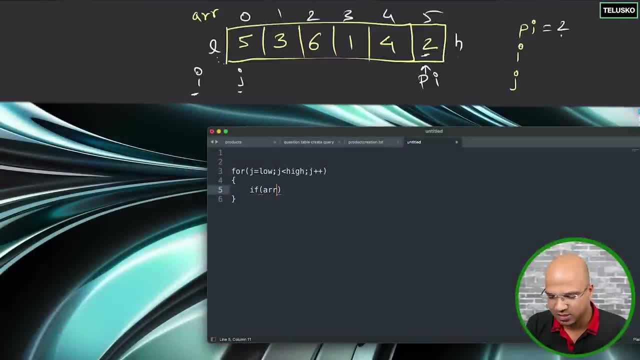 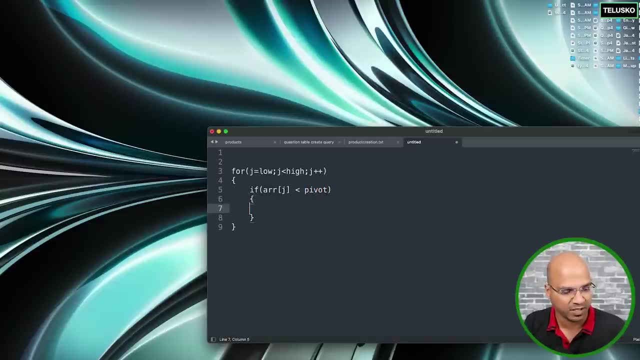 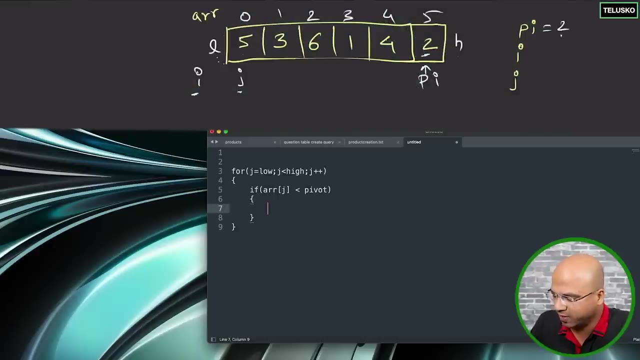 check if the arr, which is in this case, we have an array- if arr of j, if it is less than the pivot, so pivot, we have a variable here. if it is less than pivot, you will perform some operation. now, if you compare the values here, do you think the arr of j, which is five in this case, is it less than the? 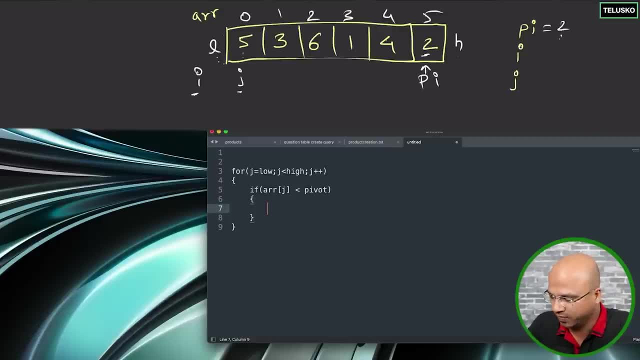 pivot, because pivot value is two. no, it is not less than pivot, so we'll not do anything, but we have to find the value which is less than two right. so if the value phi is less than two, you will perform some operation. it is, since it is not true, we are not going to perform any operation. 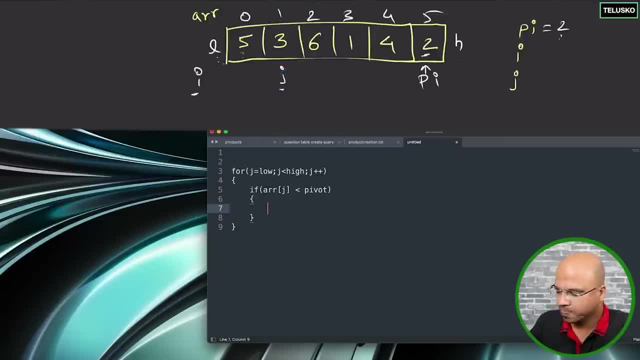 here. so basically, you are going to shift your j here. okay, now how? why we are doing it? of course we are running a loop, right. so j starts with low and then we have to increment. so j goes there. it will compare itself with the pivot. is it small? no, so again, you will shift your j, then you compare. 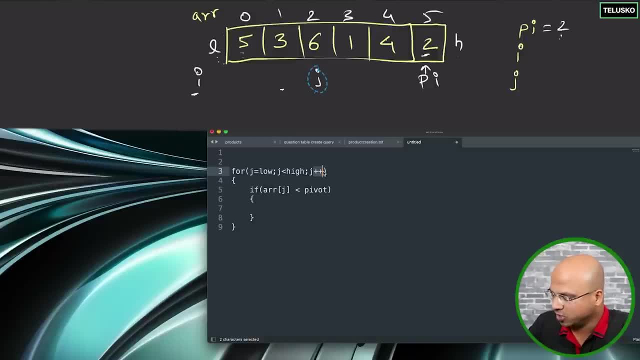 six with two, then is it smaller? no, then you shift your j here. then you check: is it smaller? yes, what if it is smaller? then what you will do in this case? if it is smaller, you perform some operation. first thing you do is you increment the value of i basically. 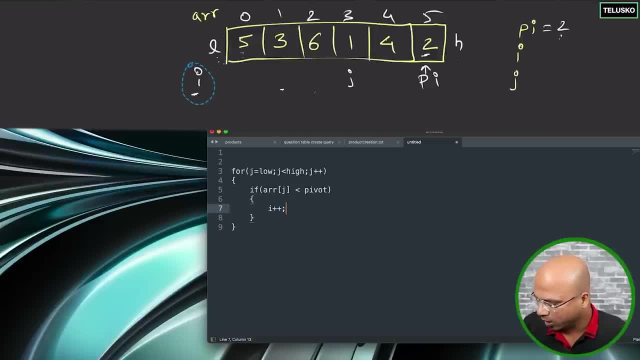 what you're doing is you are shifting your i here. okay, that's done. next, we have to make sure that you swap the value of i and j. okay, so whatever value you have with i and j, you basically swap them. so what i'm saying is: take this value here. 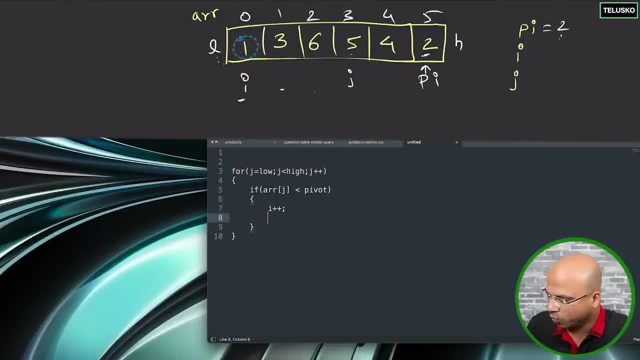 move this value five here and move this one here. okay, now, how do we do that? of course we have used it before, so we can use a temp variable, or maybe at this point i will simply say swap and then we'll write the logic later. so i want to swap basically the value of arr of i with arr of j, okay, so 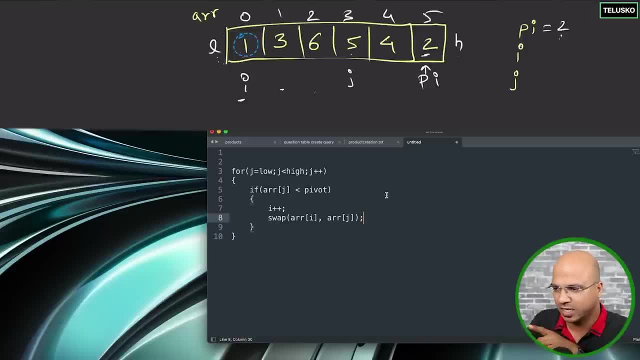 we need to do the swapping, that's it. these are the thing we are doing inside the if condition. now, once that is done, of course, you have to move your j again because we are in a loop. so j will go here now again. you will compare if the four is less than two. no, and that's it. 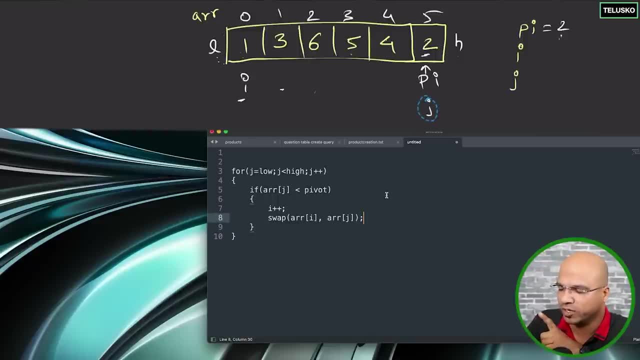 j will move here, because if it is not less, then we are not doing any operation. then your j goes to the last value because your j ends at high right. so j, reaches, reaches here, and of course the pi and j is same. then you don't, you don't have to. i mean, of course it is false. the condition this: 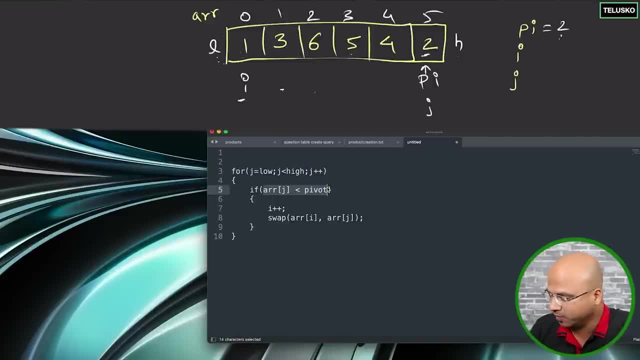 condition will be false, which is: arr of j is not less than pivot, so in this case it will not swap. but what happens after that? even if you complete the entire loop, do you think two is it the right position? no, two should be here, right? so this three need to go there. so what you do is you perform one. 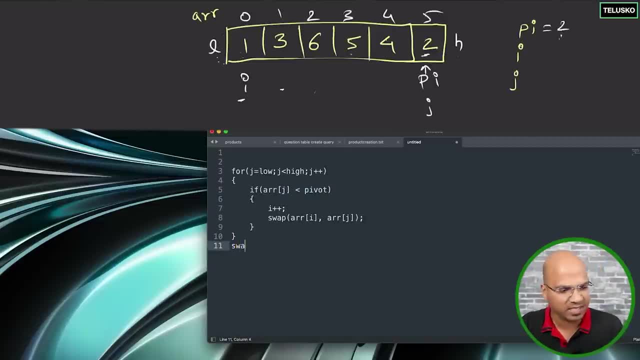 more operation after the loop. so, after the loop, you, what you will do is you will basically swap the arr of i plus one with the arr of high. okay, now, this is the option you have to perform. now what will be happening here? so what is the value of i? value of i is zero, which is index. you're. 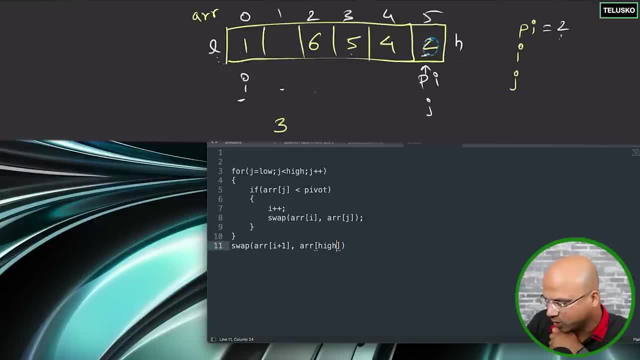 going to swap the next value, which is three. so you have to swap this three with this two, because that's what your arr of high is. so you will move here and you will move this side. now, by doing this, we made sure that the pivot value which you choose is at the right position. can you confirm? is it the? 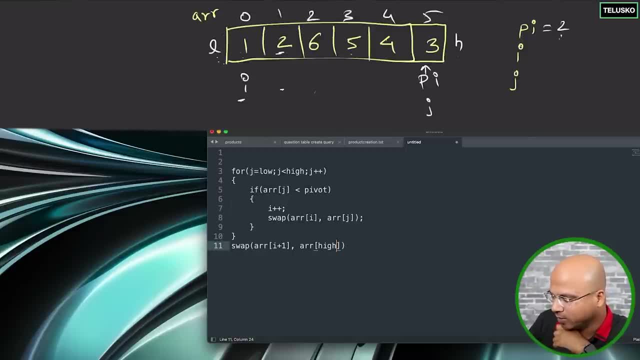 right position. yes, it's the right position. now, what you do is you divide. i mean, if you, if you observe the array, if you look at the pi, which is pivot here now, if you see the left hand side of it, this is always lower than two and this value is always greater than the two. so, yes, two is the right position. now what's the next? 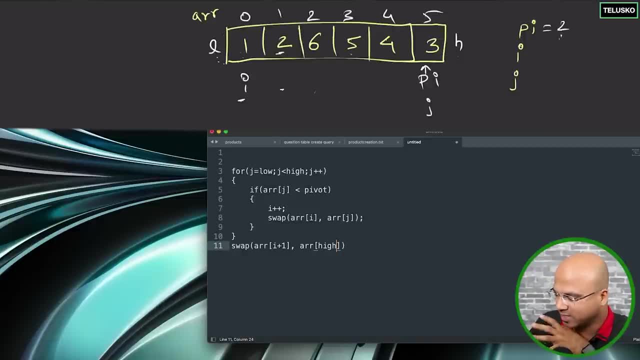 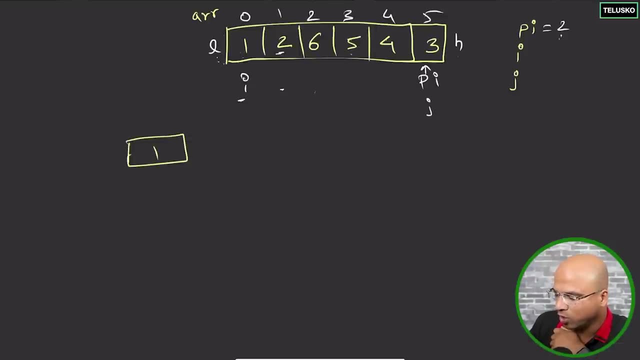 step. the next step is very simple. you divide this array based on the pivot value. so what you do is you create another array here and in this you will be having only one value, which is coming from here. right, in fact, we can also draw an arrow there. so this is coming here. two will remain there. 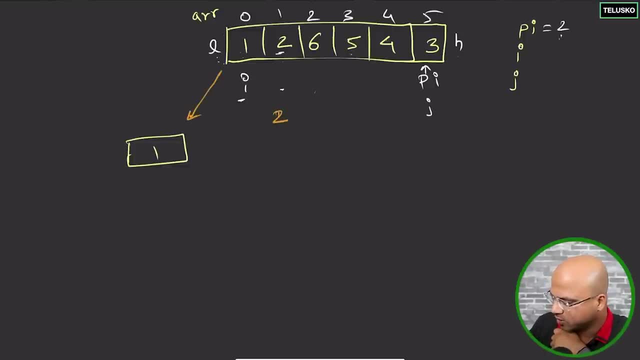 itself. we can write two here. we don't have to work with two because it's already sorted- and then you can add another value to this particular section into another array, not another, but let's say logical partition we are doing here, so we'll get another array here. so we are doing divide and 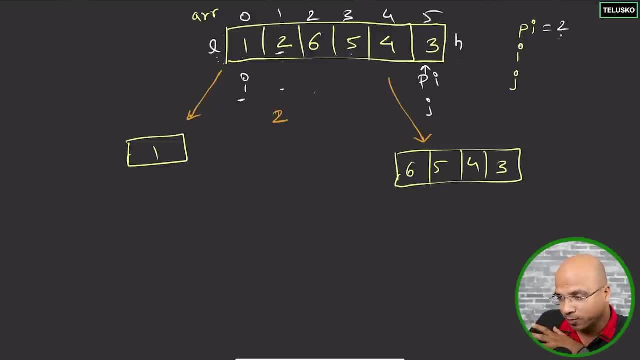 conquer. so here you're going to have six, five, four, three, if you observe, they're not sorted, but at least we got the partition right now. what you do is you again perform the same operation which we have done here in the first example. now you help me. should we start with this? yes, we can start, but you 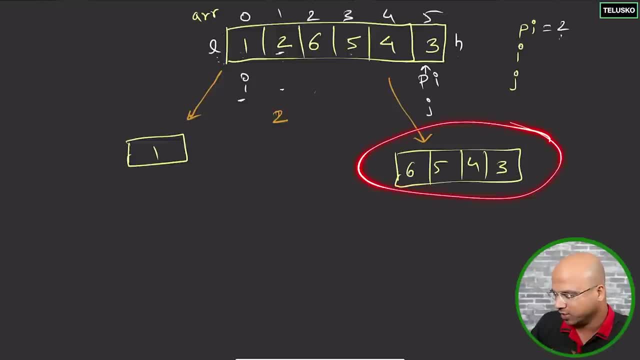 can also do the same thing. you can take the value, and whenever you have one value, it is already sorted. let's work with this. so what you do is you again take the same thing, so you take the low, you take the high, and then you, of course, you again have this p of all these values here. so all these, 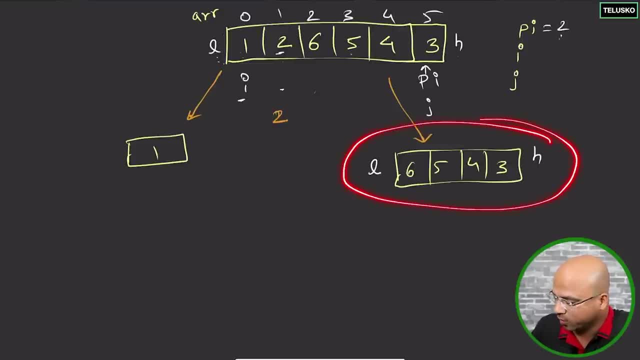 variables are still exit because you are going to apply quick sort again on this particular values. so let's get started. let's take pivot. which pivot we are choosing? of course, we are choosing always the last value. so this is your pi pivot. then you got i here, you got j here. then you have the other. 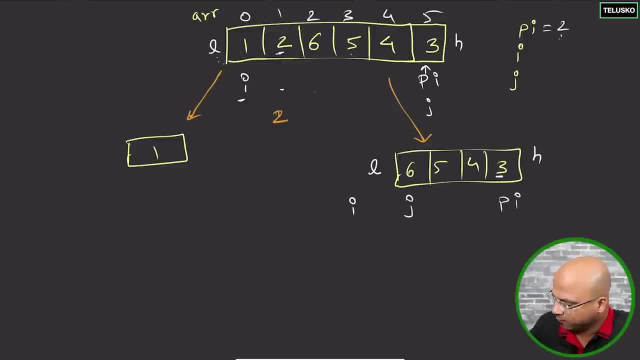 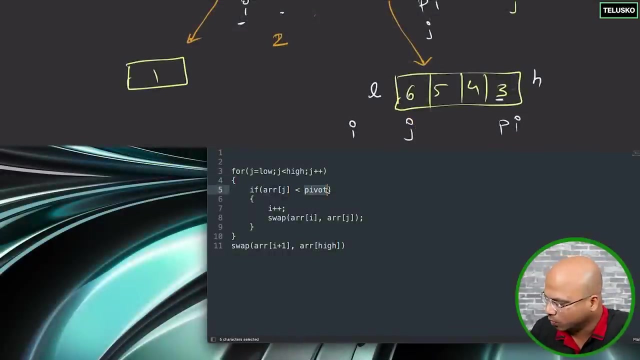 value, and then what you do is you start running your algorithm, which is: first, you compare the value of j, which is 6 in this case. is 6 smaller than 3? look at the algorithm which we have done: is 6 smaller than the pivot? the answer is no, so you will simply so, you will simply move your j. 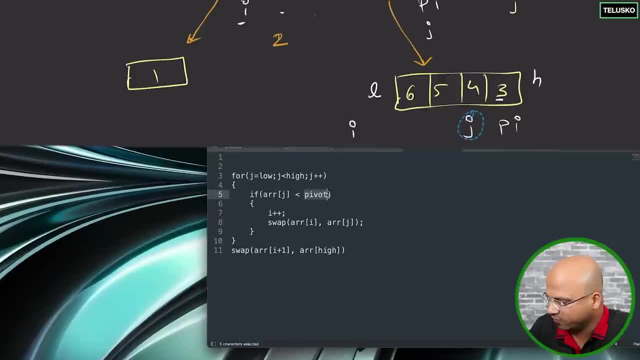 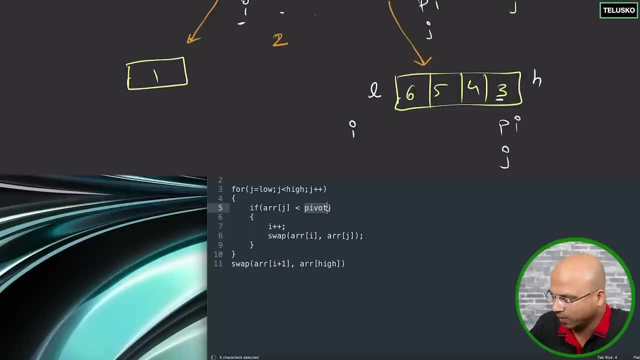 here again check: is it uh small, no, shift. is it small, no. is it? then again goes here: is it small, no. so what you do is: you have not. you have not done any swapping, but at the end we got one more logic right. so once you complete this for loop, you will do something with this, which is swapping. 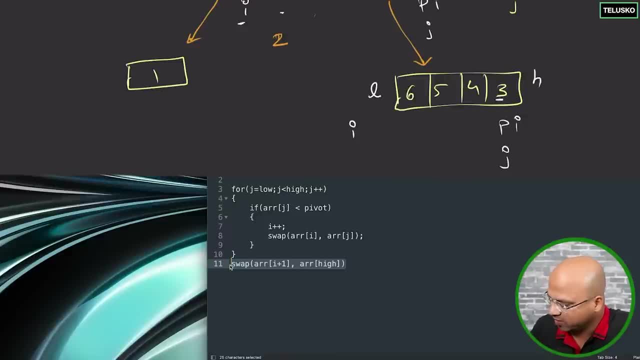 the i plus 1. so i is at minus 1. so you have to basically swap the 6 with the area of high, which is 3. so this goes here and this goes here now, if you look at the pivot, this is sorted right. so now what you do is you write 3 here, which is your pivot value. 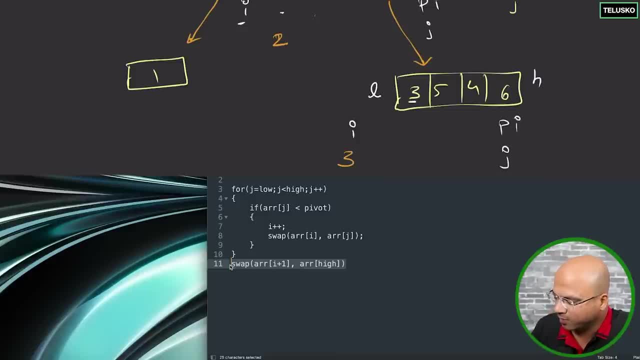 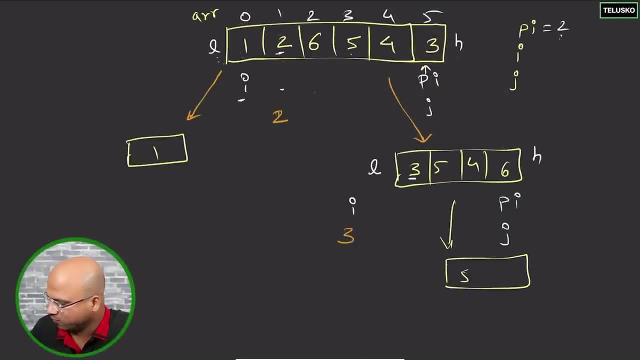 and then you divide your array into two parts, but since the pivot was the first value, what you will do is you will get the new array now from this, which is 5, 4, 6, and then you start performing operation here. now, what operation? the same operation which we have done. 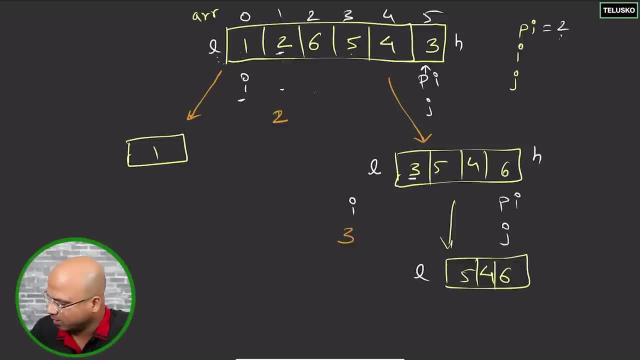 again, you will apply quick sort. so this is l, this is h, so pi is referring 6 here. and then you start: so you got i, here, you got j. then you start comparing: is the first value the value of j? is it smaller than the pivot? yes, now, when you say yes, what you will simply do is you will increment. 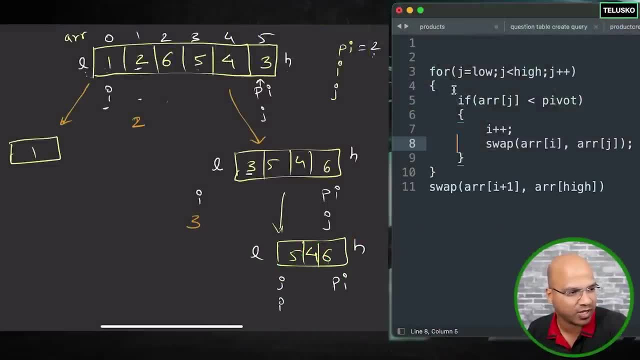 the value of i first. if you look at the code, that's, that's what the logic we have, and then you swap the value of i and j. now, in this case, i and j are referring to the same value, so swapping doesn't make sense. of course they will get the same value. then you increment the value of j. 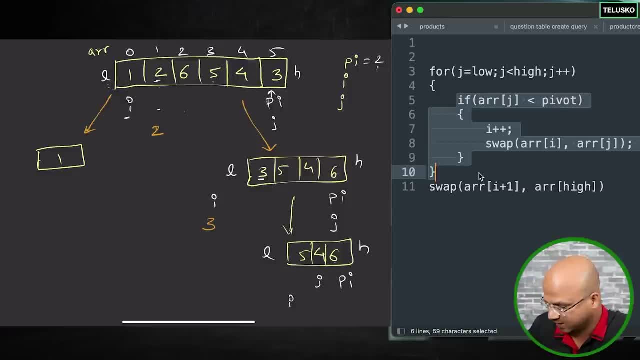 j goes here. check is 4 less than 6. yes, in that case you will move i here and then you will swap the value of i and j again. it remains same, so nothing to do here. then you shift your j here. of course the array of j is not less than pivot because they're the same value. then this loops end. 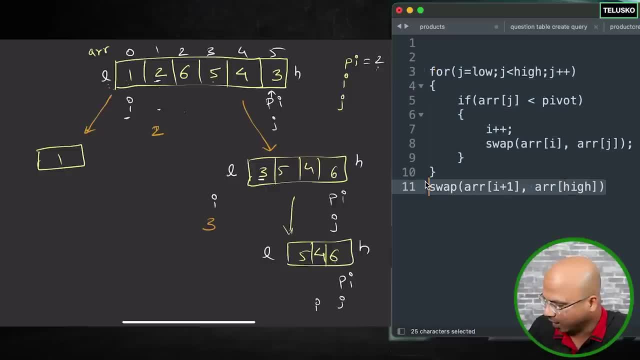 the for loop ends, then you perform this operation, which is arr, which is plus one. this will be replaced by high and that remains same right. so there's no swapping. i know it all depend upon the value, type of values you're getting. so at this point there's no swapping happened, so this remain. 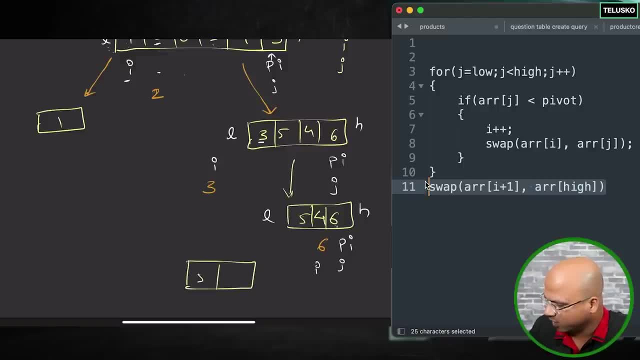 but then you will get a new array here which only has five and four, and then you start applying the same operation. let's get started. in fact, i will just write this bit up so that i will have some space, and this is coming from this particular section. then what you do is you will take the 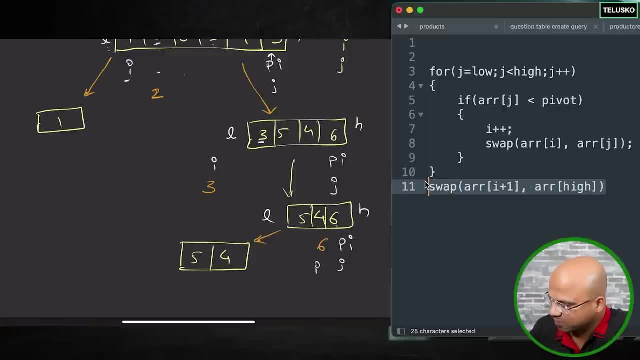 same value. you say, and if you observe we are doing recursion right, the same steps we are repeating multiple times. so l? h, we got p i. here we got the variable i referring to minus one position, or in this case it is one less than the low. so in this case, the low is this position. right now, what is? 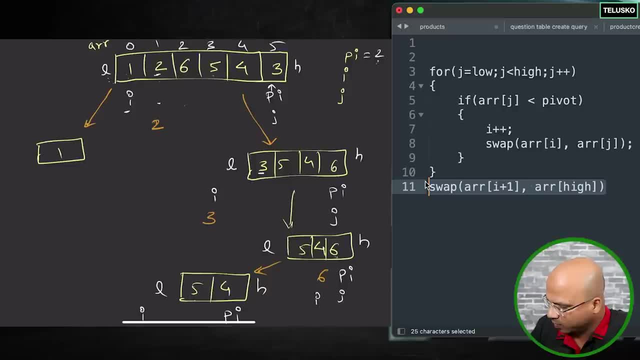 this position. this is, in fact. we should have maintained the index value, right? so this is zero. this is one. this is two, three, four, five. then we got three here, which is this one. this is three, four, five. what we got here is three, four. so these are the index values for them. okay, so we got i. 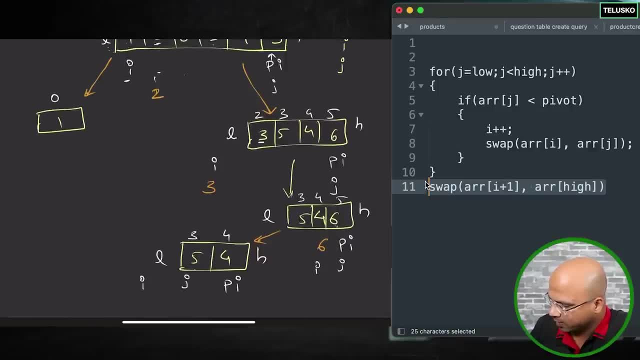 referring to the index, value two and j is here. then what you do is you simply compare the same steps we have, which we have done. so the area of j: is it less than four? no, so all this operation, this swapping, is not needed. you will simply move your j here again. 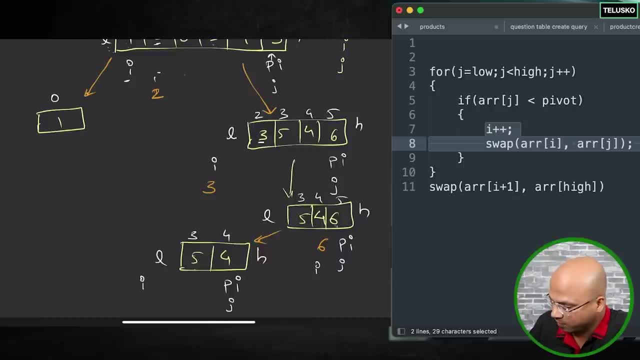 do we need to swap? of course not, because the array of j is not less than pivot, so it will remain same. but then you will perform the last option, which is this one: what it says? it says: swap this value with the high value. so this will be swapped. so five goes here, this goes here and this goes here. 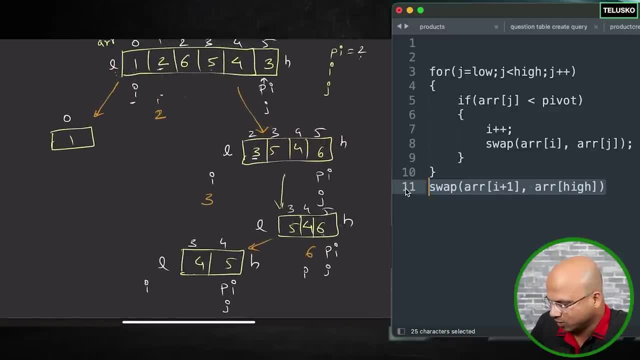 now, if you observe, we divide it and we concurred. so if you merge this, in fact we are not merging physically, we are merging logically. right, because nowhere we have we were breaking the array. but if you see, if you try to merge logically, what you will get. so you will get this one first, which 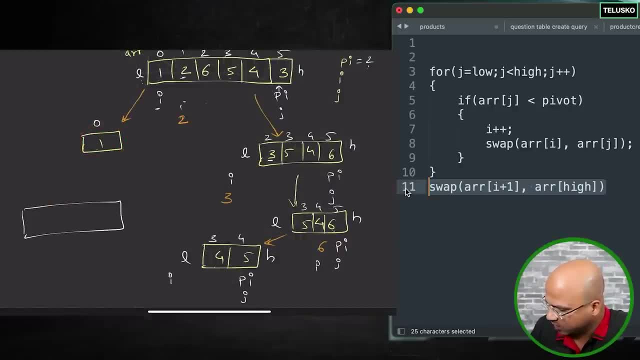 is: one goes here, then two goes here, then by sequence, three goes here, then by sequence, this four to five goes here, and then this six goes at the end. so if i want to write this, this will go. so let me write one. then this goes here, that's two, then three goes here, that's three. then if 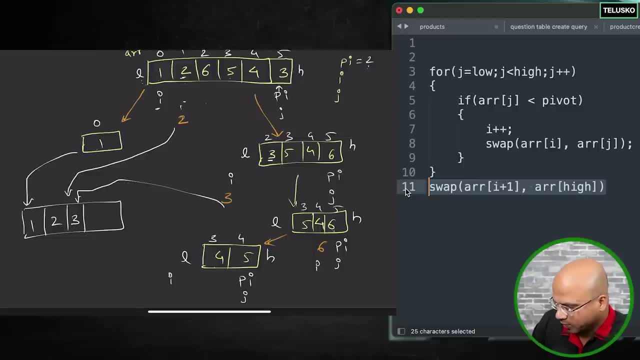 you can see, in the binary tree, we always goes from the left to right. so if you see the left, because six is there on the right hand side, you will say four and five and at the end you will get six. now this is sorted. so, after all this explanation, this is how, basically, you 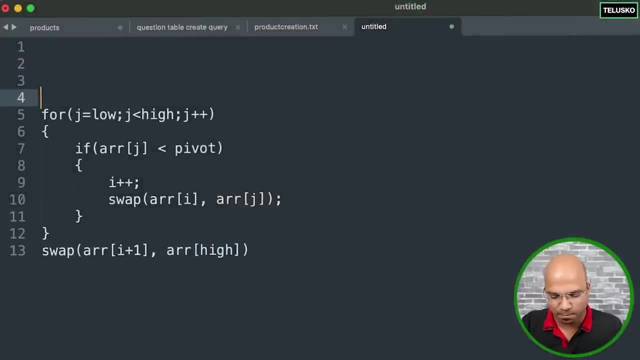 sort them. now. this logic which we have written here is actually a part of a partition method, so this is a partition method, so the entire thing goes there. but we also need to return the pivot value, right? so which is the pivot value? so we'll return, i plus one. 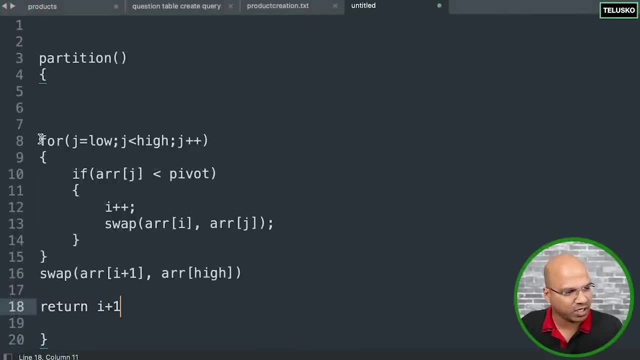 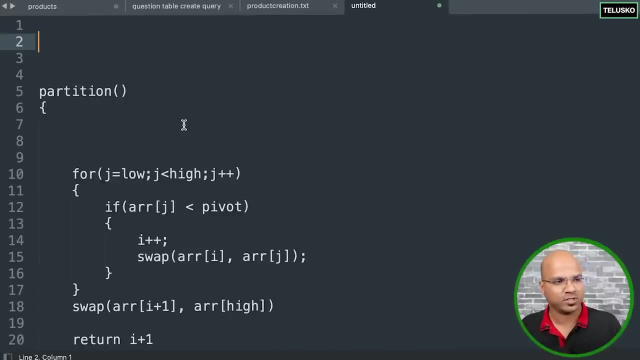 because that's what the pivot is. but this particular function will be called by whom? so we have a concept of quick sort here. so quick sort is going to call this partition how. that we're going to say in the code itself. so you got the idea. basically you divide, sort, each values. 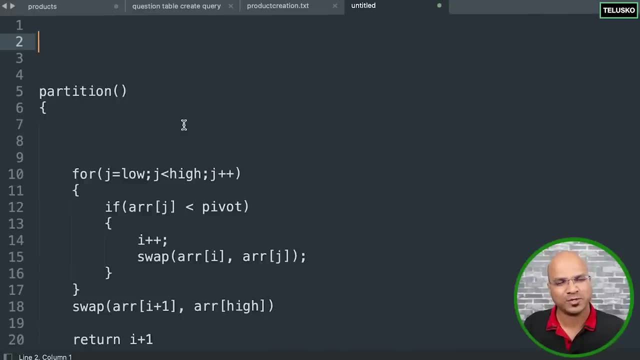 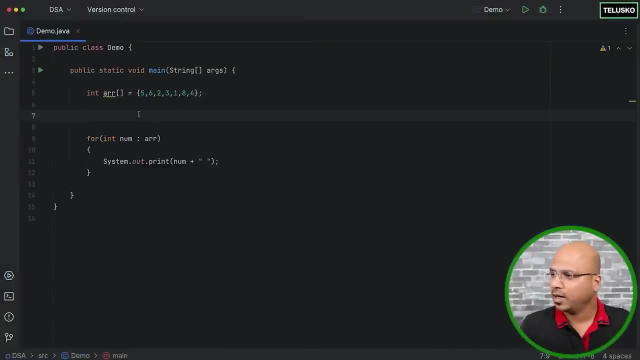 and you will get the output now. this will make much more sense once you start coding, and i hope it will get clear. so what i will do is i will just remove the entire part here. we got this array and we are going to perform the operation now. of course, you can write the. 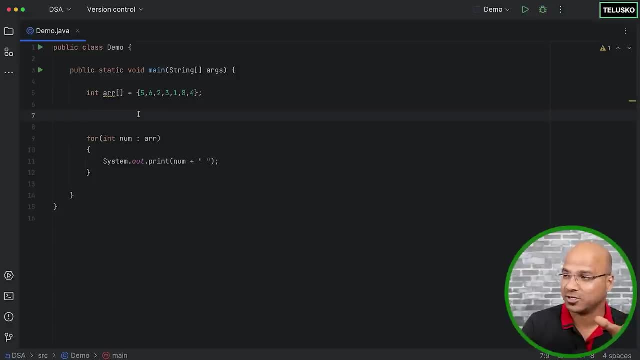 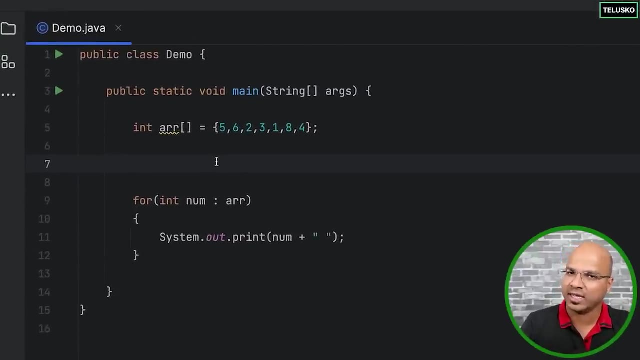 entire logic here. but then remember, quick sort goes for recursion. so when you say recursion you have to create a function or a method which will get called. so what i will do is i will create a function here and let's call them- so we'll say a quick sort as a function name or the method name. 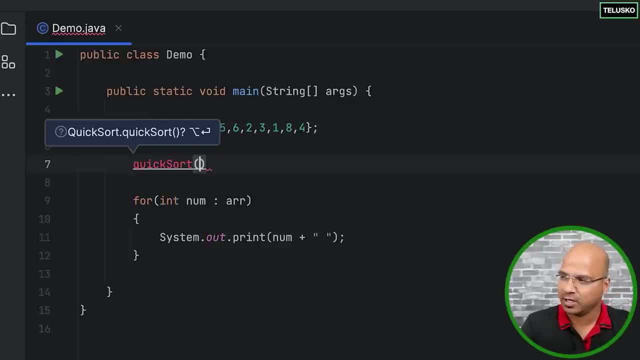 which will take three parameters. now, what are the three parameters? the first one is the array itself. you want to perform the operation. next is the starting point and the ending point of each section. example: if you start, it will be the entire array, but remember when we have to break it down. 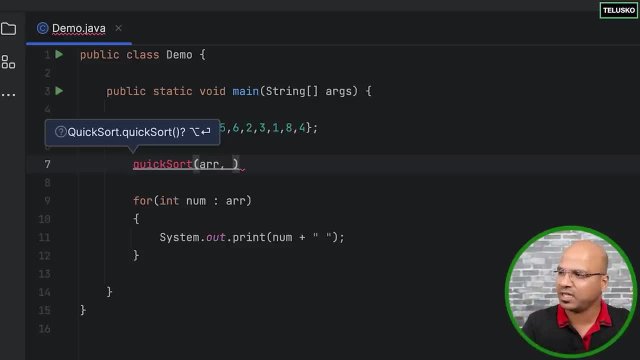 so that is your each section. okay, so we have to specify the low and then you have to specify the high. now, in this case, what is low? so low is zero and the high is basically the array dot length minus one. right, that's the value you have to send now. basically, we don't have this function, so we 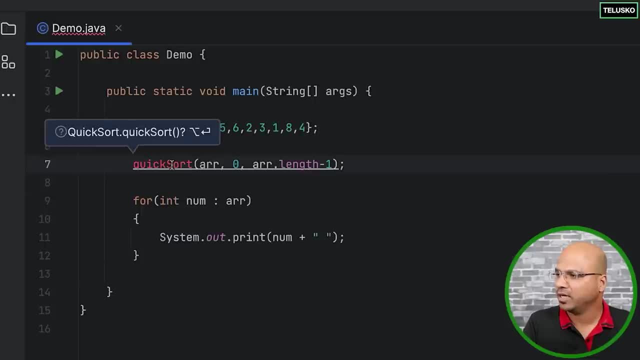 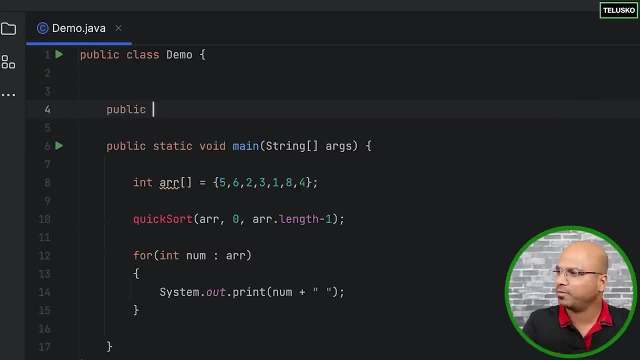 just right click here and say, okay, i want the ide to create this method for me, which is using some inbuilt methods. okay, let's create our own. so what i will do here is i will create a method called public. i don't want to get the object, so it's a static void, quick sort, and it will take these: 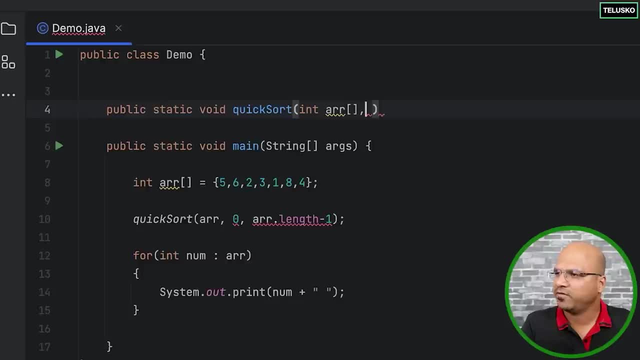 three values. so first it will take a int array, in fact one of the syntax of array. you can write it on this side, because it will make much more sense. you got array and then you got int low, then you got int high. so these are the variables you need. 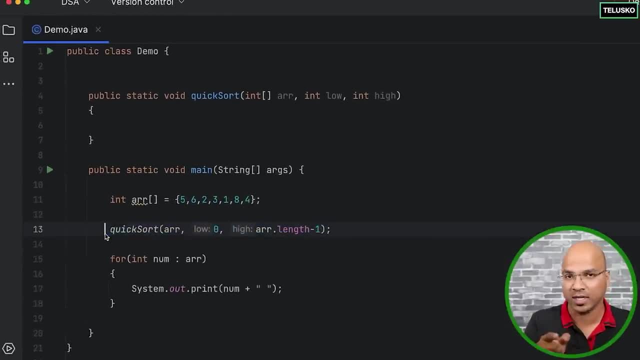 you can start performing the operation. so basically, from the main, you're calling quick sort only once, but quick sort will be calling itself. okay, but based on what? now? basically, i want quick sort to call itself only till when your low is less than high. we don't want it right. so 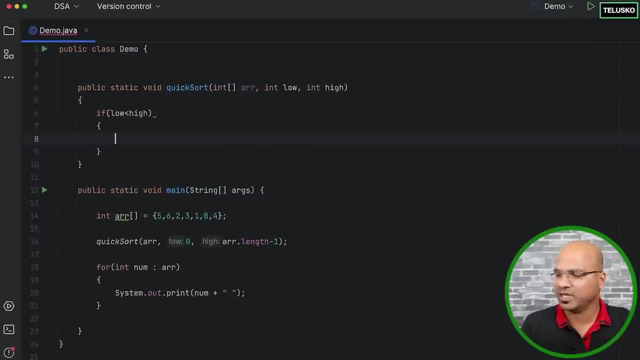 that's what it makes sense, right. low should be low, high should be high, and if it is true, then keep calling the quick sort. so i will keep calling the quick sort, but the question is what values have to pass? now think about this: if you have one big array and then you're saying that we'll be breaking this, 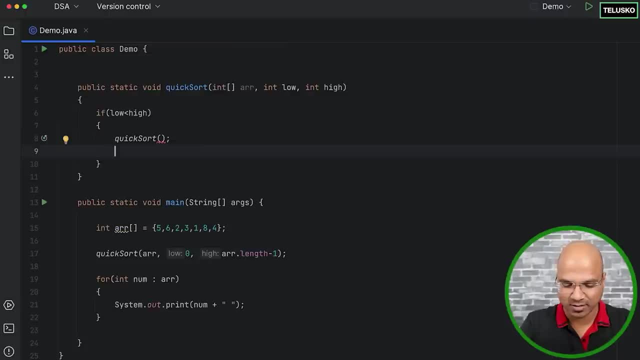 don't you think you have to call quick sort two times for two different arrays? that's right, so you have to call it two times. but the question is: what are the values? for sure, the first variable will be array, because that's what we are sending right. we have to sort the array. the question is: 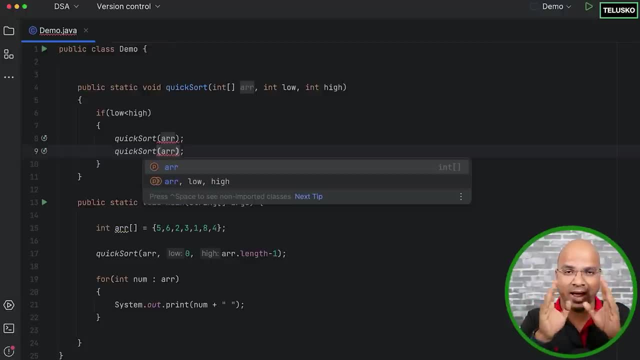 what will be the low, what will be the high? because when you divide your array into two parts, what should be the starting point of the second array and the ending point of the second array? that's what you have to mention, but how will you know the starting point? it is easy, actually. here the 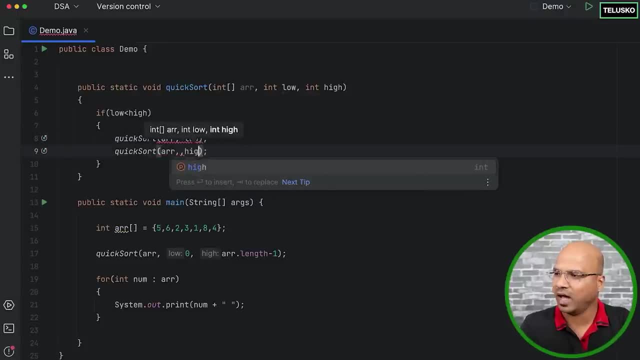 starting is always low for the first array and the ending is always high for the second array. okay, even that is solved. the problem is with the ending of the first array and the starting of the second array. that's what we need to find now. how do you find this? for this, we have to run. 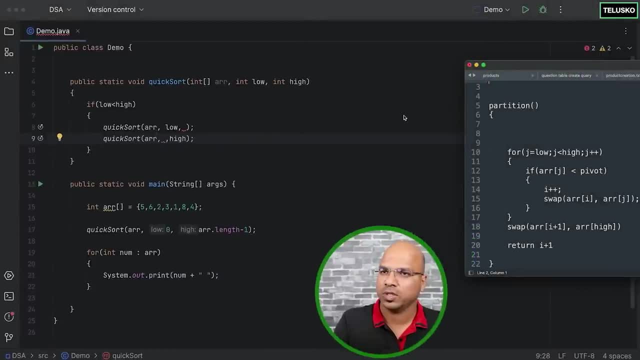 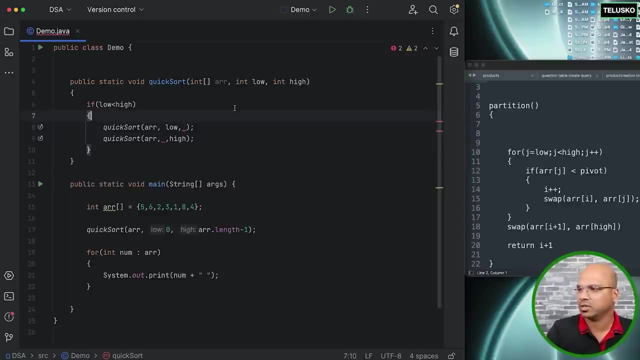 a partition. okay, so this is the logic which we have to refer to. so what i will do is i will just reduce the id size so that i can see those values. i mean this logic, so this is what we have to implement in the partition. so, basically, to get this value, the pivot value, what you will do is: 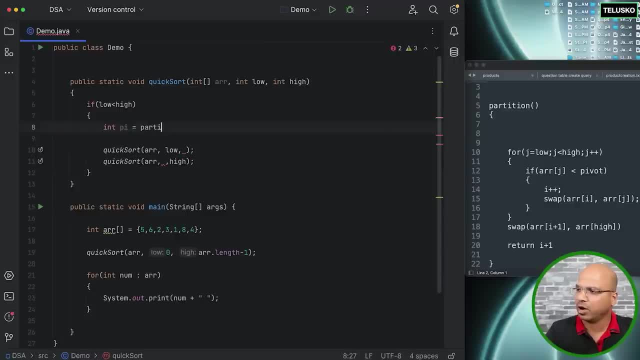 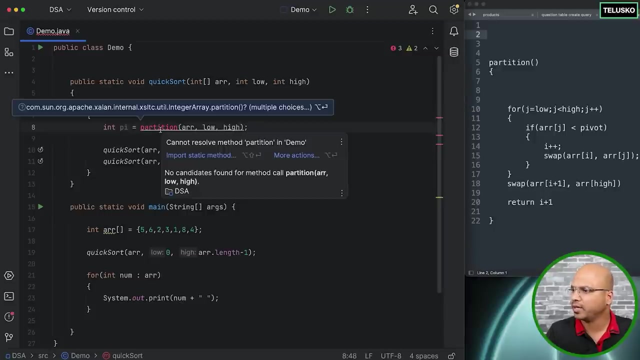 you will say int, pi equal to, and you will create a method called partition, in which you will pass three values, the same three values: array, low and high. so basically the logic. i have not mentioned it, but we want this value as well. okay, so we need to create this method. so what i will do is i will just go back here. more actions. 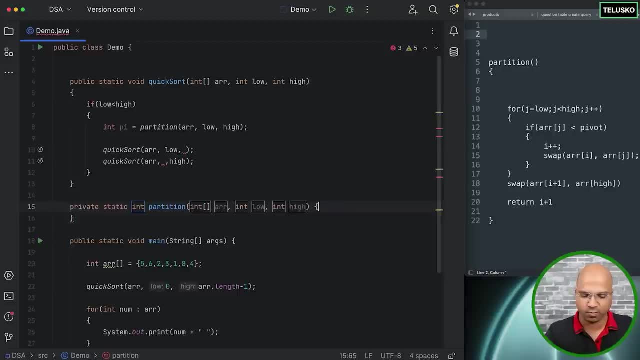 create a method. okay, so we got the method. let's perform operation on this method. we can make it private because we're not going to use partition outside this class, so private works. but what should be the logic here? and we have to return something. remember, we have to return the pi value. 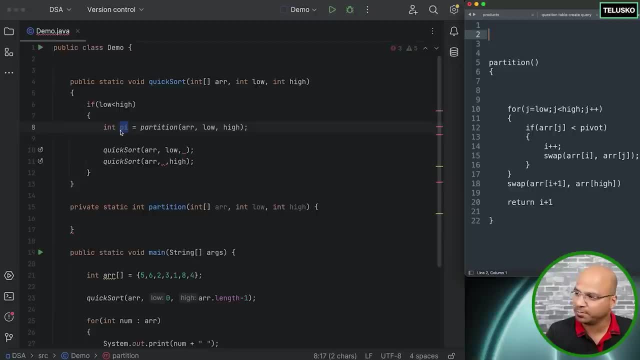 okay, so we can write the same logic which we have written here and once you get this pi, you can basically pass the pi. and we don't want to include the pi, so we can say pi minus 1 and here we have to pass pi plus 1 because every partition when you create, you don't consider the 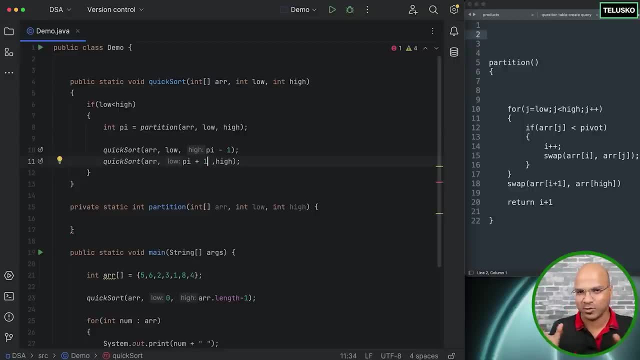 pi right, pi stays there, you create two parts and then those are your two partitions. but we have to find this pi. that's the main task and for that we have to write this logic which is mentioned here. so we need some variables. the first one is temporary pivot variable and we have to assume 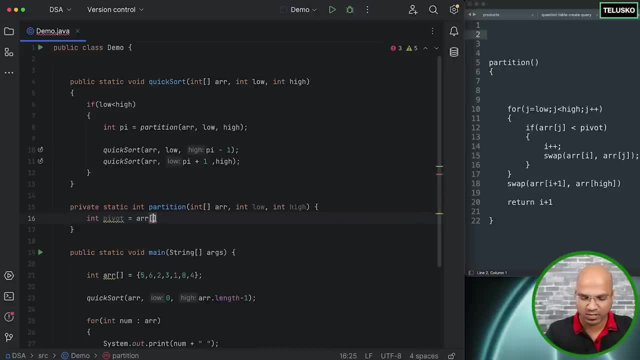 pivot for the first time, so the pivot here is always high. so that's the algorithm we are using, but we can pick up the starting value or randomly pick any value that works. so let's say we got pivot high. and then we also need one more variable, which is: i remember we have to use this i, which will return. so i is basically your. 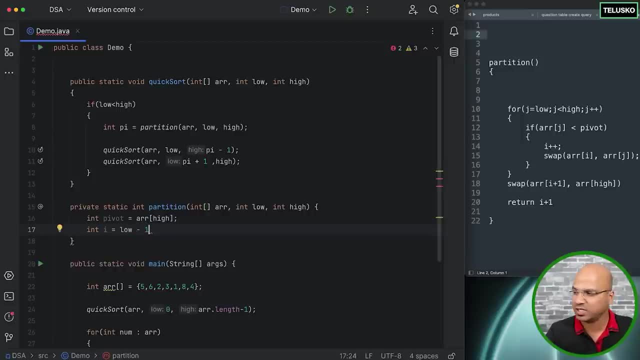 low minus one. remember, if the, if the array starts with zero, the i will be at minus one. next we need a loop so we can get the entire loop from here. or maybe you can type so we can say: for int j is equal to zero. in fact, not zero, right? it should be always low, because when you create different partitions, 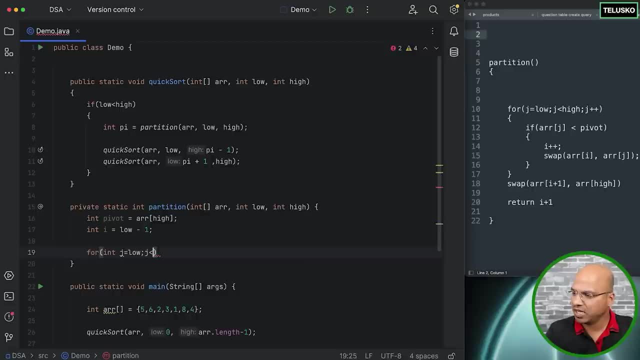 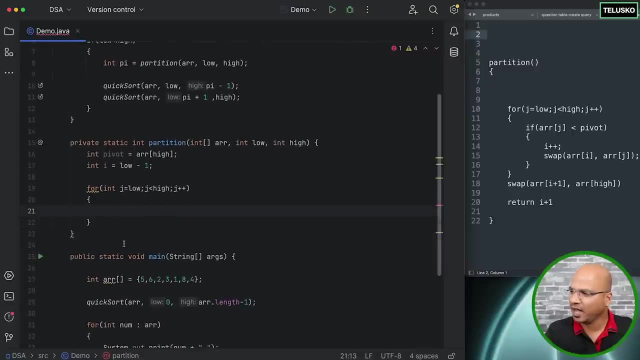 not every partition will start with zero, but they will start with low. so j less than equal to high and j plus plus. i'm just referring to my algorithm, which i mentioned here. and then the logic we have to write is: if arr of j, if it is less than pivot, then you start doing some operation. 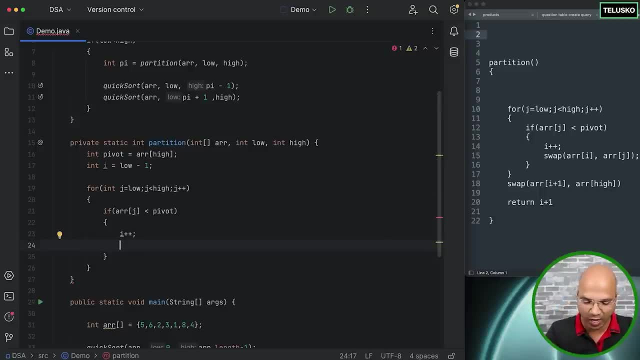 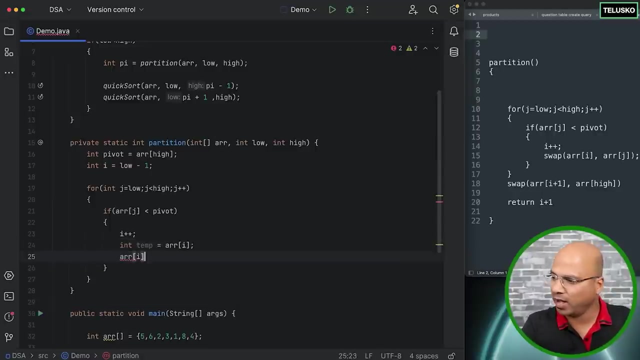 what operation. first you increment the value of i and then you swap. but how will you swap? we don't have a cell function. actually, we can create one, but instead of that, what we can also do is we can write the logic so i can say: int temp is equal to arr of i, then arr of i will be replaced by arr of j. 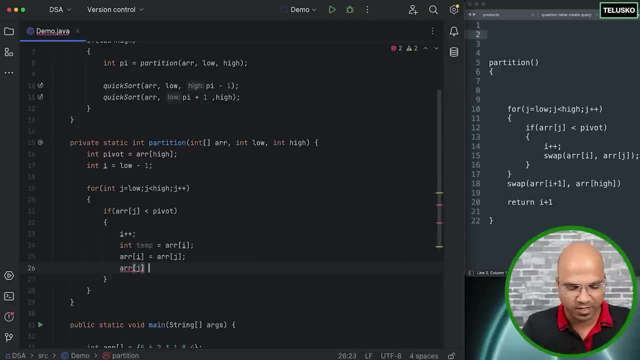 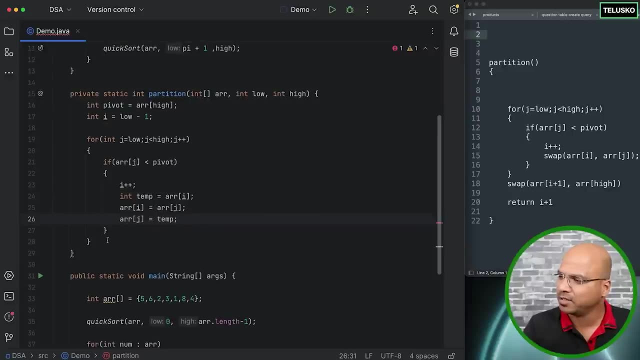 and then arr of j will be replaced by the temp. okay, that's the values we have to swap, and that's it. this will run and you will do the partitioning part. but once you complete the for loop again, we we have to swap the value of i plus 1 with high, so you can actually use the same logic here. 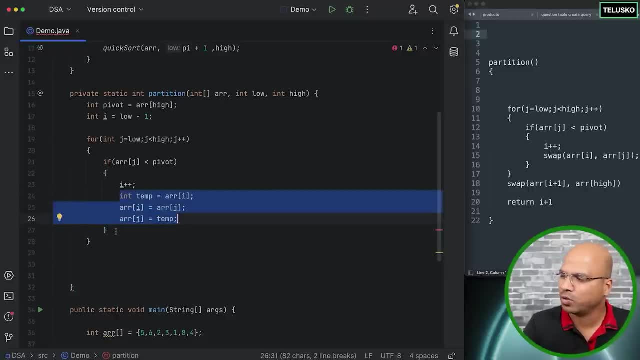 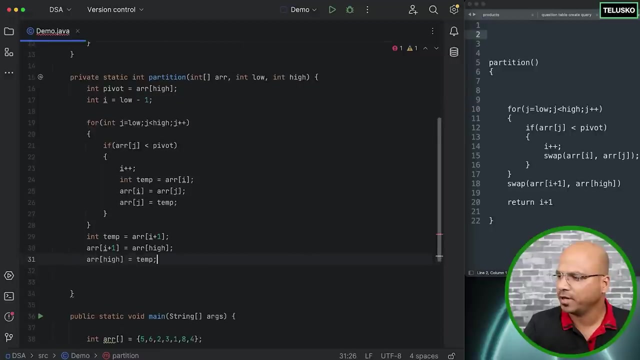 or same statements. so i'm not copy pasting, i'm just reusing the code. sounds better, right? so here we can say: this will be replaced by i plus 1, and i plus 1 will be replaced by high, and this high is going to replace by temp. so i've been done, and at the end we need to return i plus 1 because 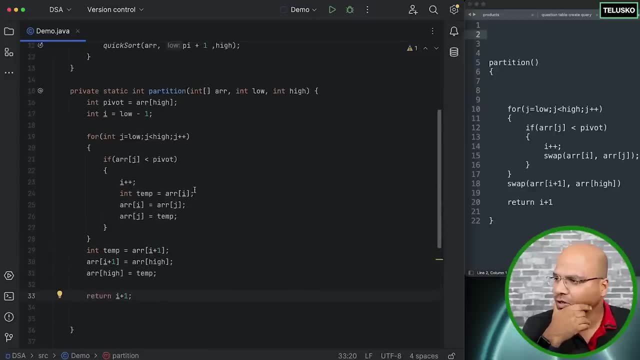 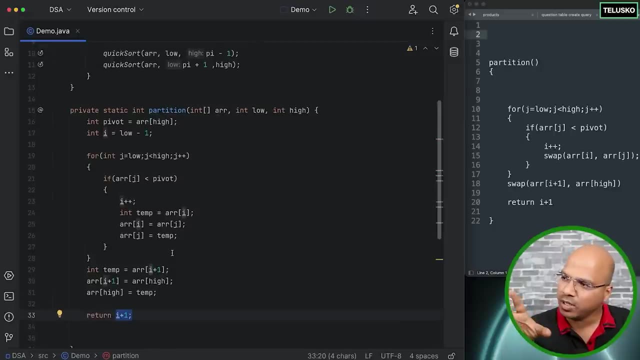 that's what is referring to the pivot. okay, uh, looks like a right logic. we just converted that into here. so by doing the partition, we are saying replace one. in fact, once you get this algorithm, also try out the same thing, which i've done on the board. okay, then it will make much more sense. 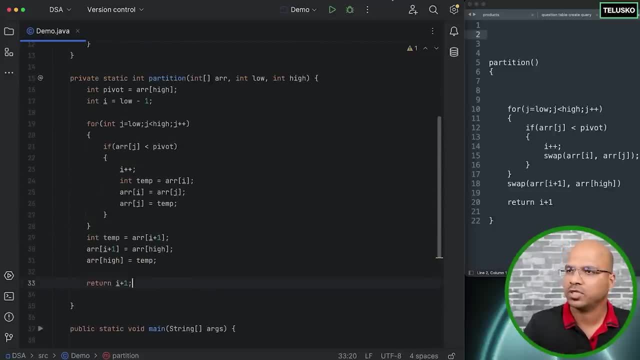 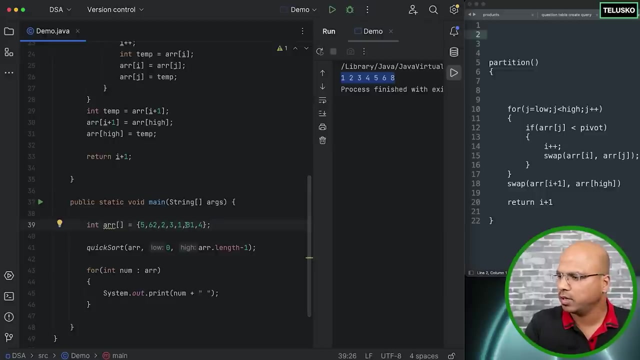 okay, i hope this will work. what do you think? let's run and let's see. run and, yes, looks like sorted. one, two, three, four, five, six, eight. let's change some values. let's say this is 81, 81, this is 62 and this is 111. let's try with these values and let's see if they're sorted. 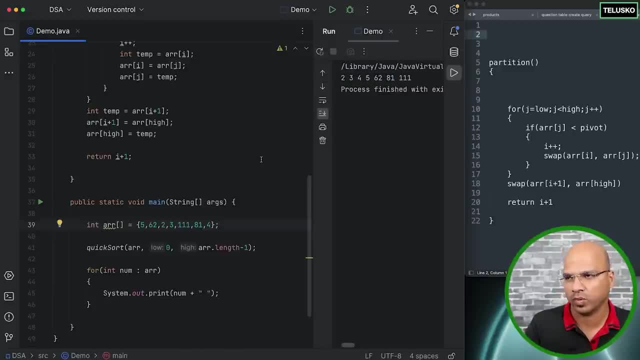 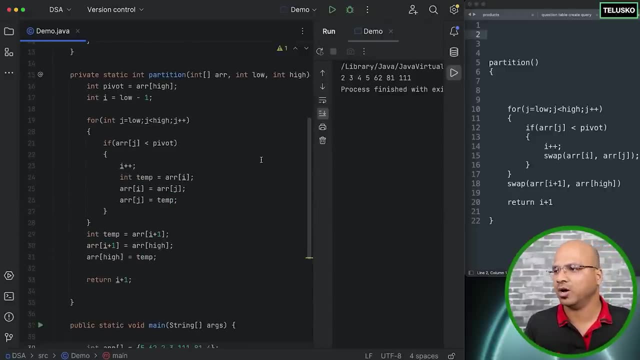 so 2, 3, 4, 5, 62, 81, 111, so it works. so those, this is your quick sort. now, why we are saying this is n log of n is because we only have one loop here, which is for loop, plus we are doing the partitions. 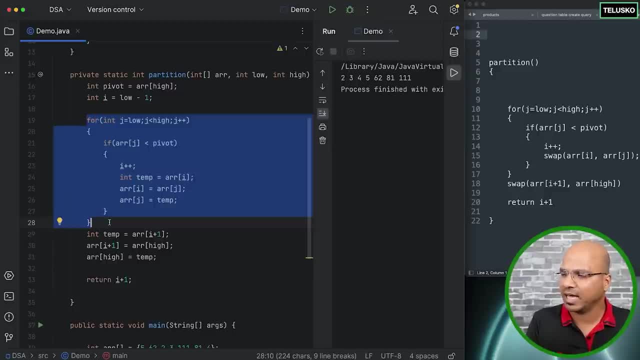 of it right, so they can run parallelly. yeah, so this is n log n, but in the worst case it can go for n square, but better than the other sorting techniques. so yeah, that's it from quick sort. we have written the code in java. in this video we'll talk about merge sort. now, basically, let's talk. 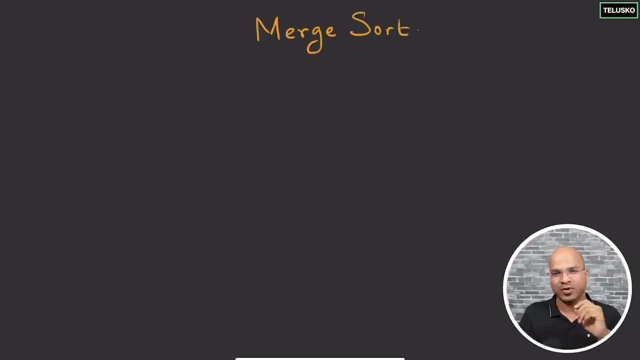 about the theory first and then we'll focus on the implementation. now, when we talk about sorting techniques, we have worked with multiple sorting technique, and when we talked about the quick sort which was going for the time, complexity of n log n- now we have one more there which is called. 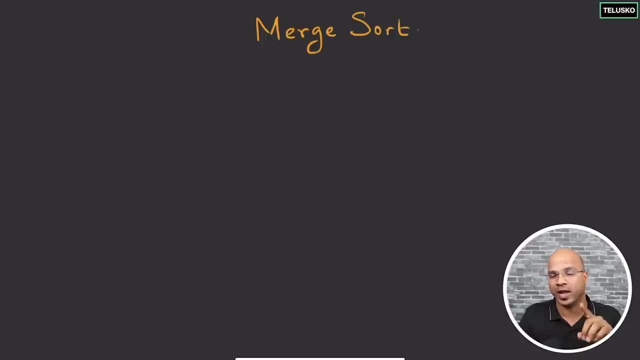 a merge sort which also has a time complexity of n log n. now, both quick sort and merge sort follows a technique called divide and conquer. so basically, what you do is you break down the problem into sub problems and apply the algorithm on those particular sub problems and 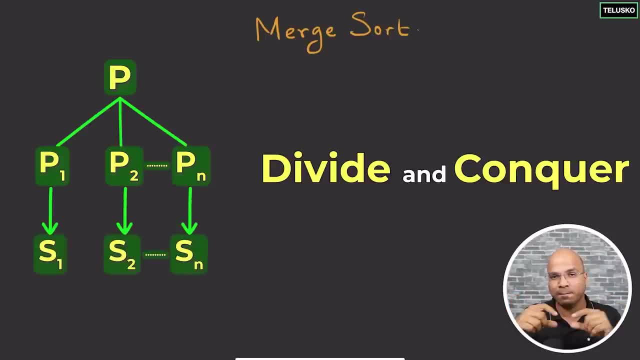 once you get the solution for each sub problem, then you combine the solutions or sub solutions to get a final solution. that's what we are going to do here, which is divide and conquer. okay, so how we are going to do this now, basically, it is actually easier to understand. so, if you can be with me, it. 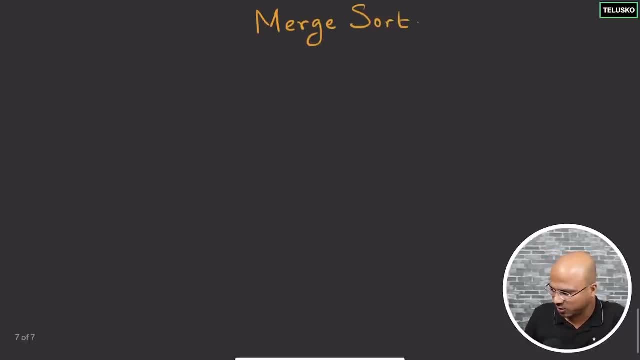 will make much more sense. so what we're going to do is we'll take a array initially, okay. so let's say i'm taking a list of values here, so let's say we are going for six values here. and what are these six values? so let's say i have a value which is eight, five, nine, one, six, seven. let's say so, we got these values. 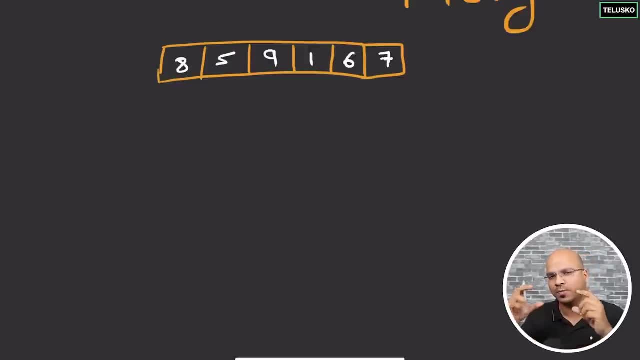 here and then i want to sort them. so what you do is you will apply a merge sort now. basically, here, as i mentioned before, you will do two things. you will, in fact, three things. first, you will divide this problem into sub problems, and then you will conquer them, and then you will simply merge them. now, since it is called a merge sort, the important- 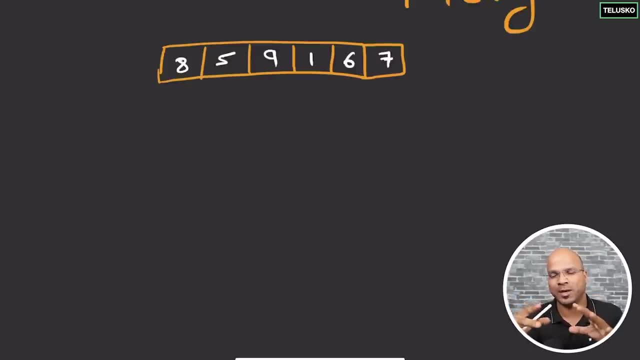 step here is merging. so when i say important, i'm also, i'm also saying it is complex part. the easier part is to break down this into small parts. merging will be time consuming, so let's understand this. so when you have these values here, what you will do is, first of all, you will break down into two. 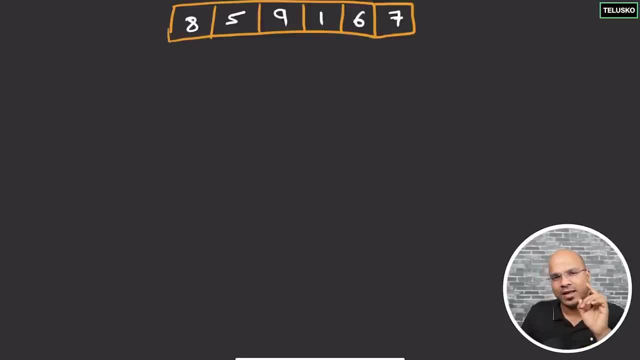 parts. now the question is: how will you break it down? in different sorting algorithm we have a different way of breaking the entire list. in fact, in quicksort we use a pivot, but here- let's make it very simple- we use something called a median. now what is a median? or maybe a midpoint? so here, what we can do is, as we know, that if you 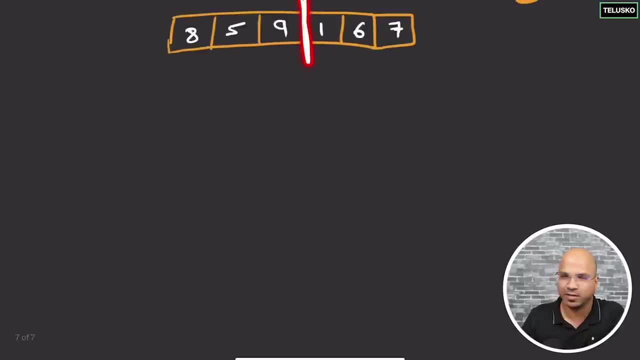 talk about this particular array here. the mid is here, right, we can see and we can tell that. but how an algorithm will know that this is a mid? and that's why we will do some calculation. now, what kind of calculation? it's very easy. so what we can do is, let's say, this is your left and this is your. 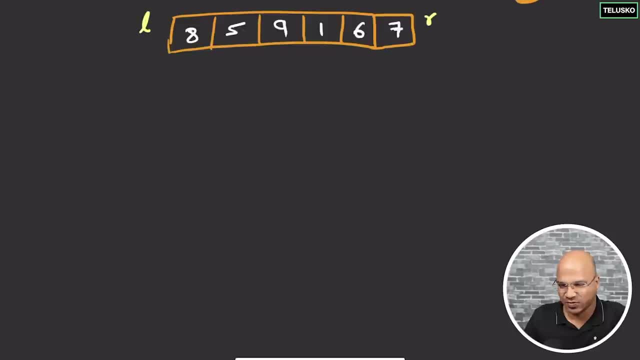 right. so what we will do is we'll do a mid point, and then we'll do a mid point, and then we'll do a mid point. so what we will do is we'll simply use index values. so this, the index values for this, is zero, one, two, three, four, five. so that depends upon the values you have. and then, if you want to, 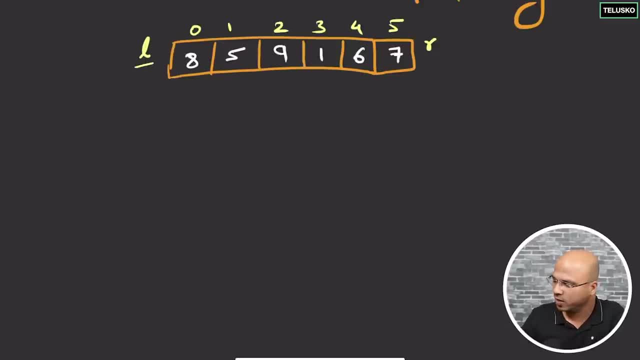 find a median. so basically, l represents the first index value and r represents the last index value. so you have to find a median, and the formula for media is very simple. so what you will simply do is you will say: median is equal to left plus right divide by two. that's how you get the median right. 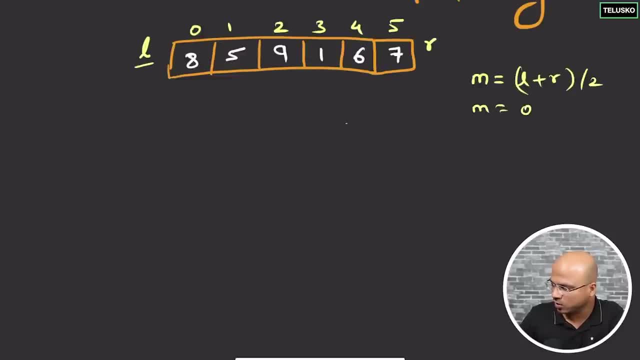 now, in this case, the is what is l, l is 0, r is 5 and this, divided by 2, is equal to 5 by 2. now, since we're in different languages, we get different outputs, so let's say this is 2 in this case, because in most of the 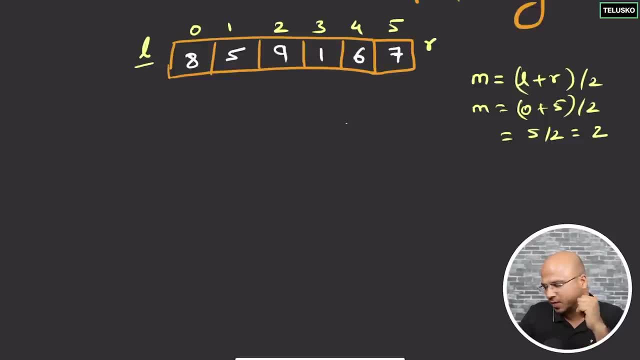 languages, we go for the floor value. so we got 2 here. now. 2 is your median, so this is your median. so whatever is there on this side will go into a different array, and whatever is there in this side will go into different array. so when i say array, i'm talking about the least, so what we can. 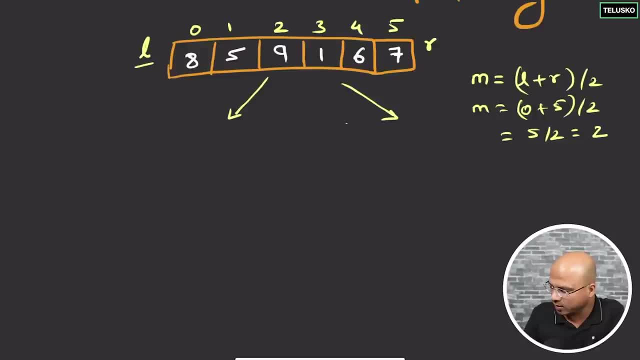 do is we can divide into two parts and then we can create a different section. so we got a section here which has three values. we got a section here which get three values, and then the values will be 8, 5, 9 here and 1, 6, 7 here. okay, and again the job is not done. again you have to divide into two. 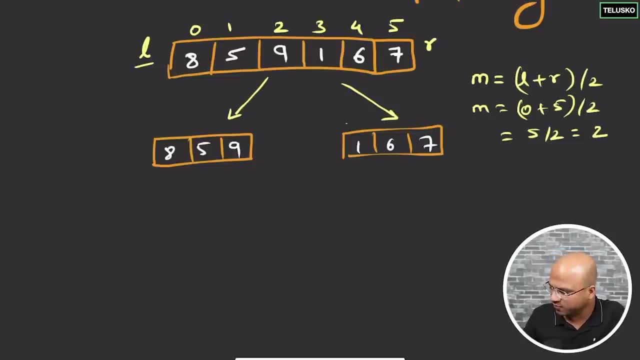 parts now how we're going to do that. it's very simple. the same steps which you have followed again. you will take l and r here, l and r here. you will take l and r here and you will take l and r here, and you will take l and r here and you. 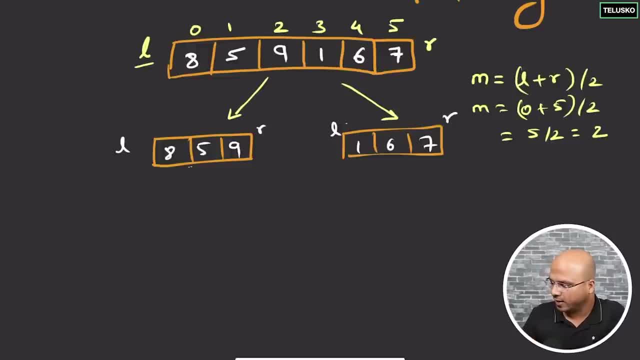 let's find the median of the first point here, or the first array. now how do you get the median? again, you will say: m is equal to l plus r divided by 2. so now we can do it quickly. so what is l in this case? so if you go with the index value, index value is 0, 1, 2 in this case, and 3, 4, 5 now, if you 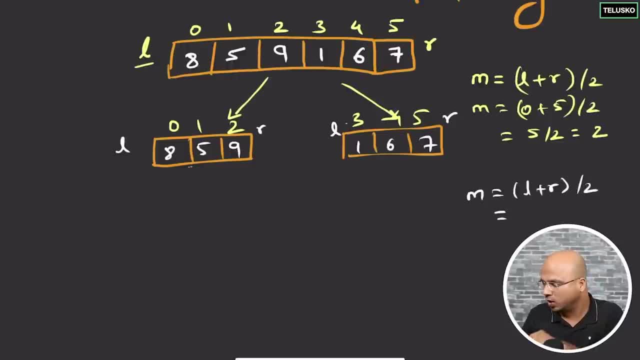 talk about the first array. the l is 0, r is 2, so you will say 0 plus 2 is 2, and 2 divided by 2 is 1, so m for this is 1, so m is here. now if you want to calculate for the next array, you will have to. 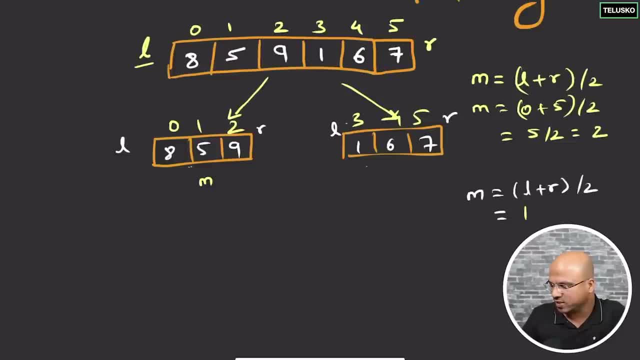 calculate for the next array or the next values. so again the same value. so what is l? l is 3, r is 5, so 3 plus 5 is 8. 8 divided by 2 is 4, so 4 is here, so median is here, of course, when you look at the 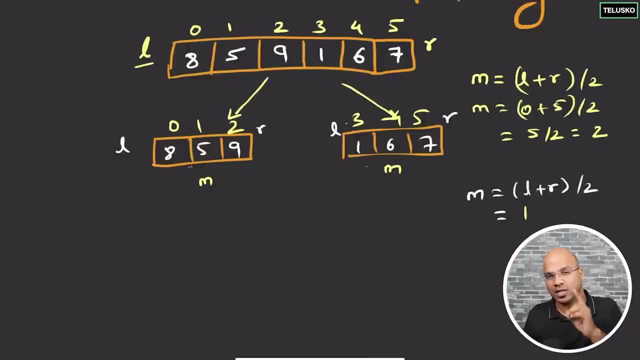 values. you will find the median just by looking at it. but let's talk about the algorithm and we don't have a limited set of values. what if you have 500 values? you will not simply search for the median right. so that's how we can get the median again. you will divide into two parts, so 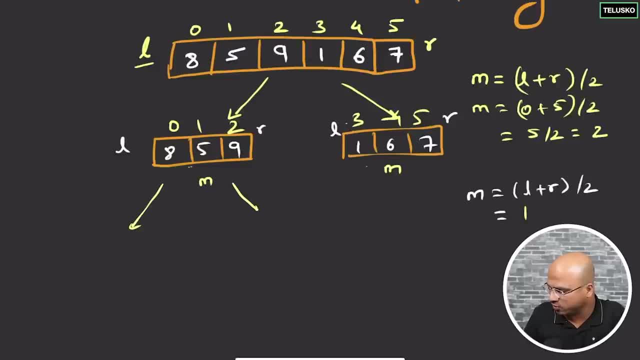 we can divide something like this: you will get two sections here for this and two sections here for and two sections for this. we can say: the first section will have two values, which is 8 and 5. the second section will have a value which is 9. here the first section, since we only have 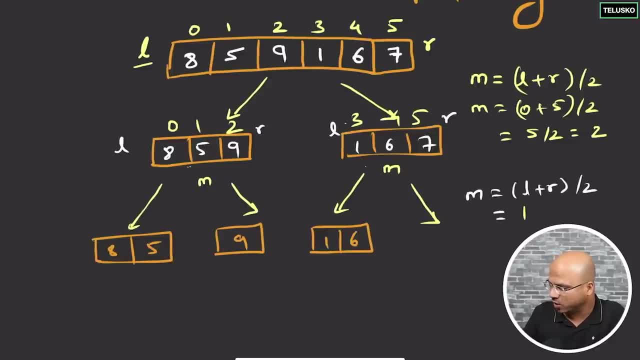 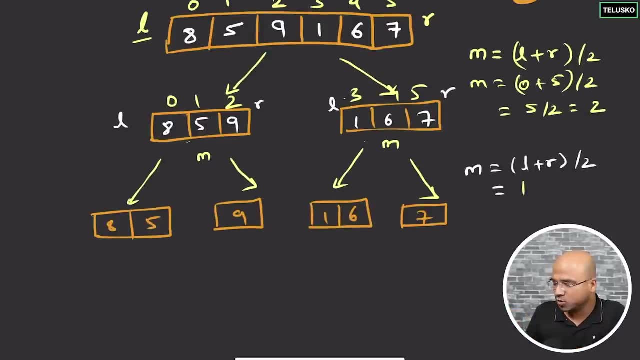 one value, here 9, we got 9. but let's say, here we got 1 and 6 and here we got 7. so basically, that's how you divide. again, the job is not done, so you have to go till the end. so what you're going to do? 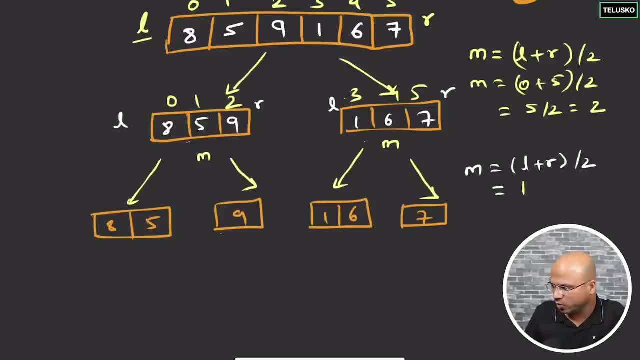 again, you will divide the first one. so can we divide the second one, the 9? we don't. we don't need to divide this part right, because when you get one value, you cannot, you cannot divide it. so let's divide the first part here. so if you divide this, you will get again two values, which 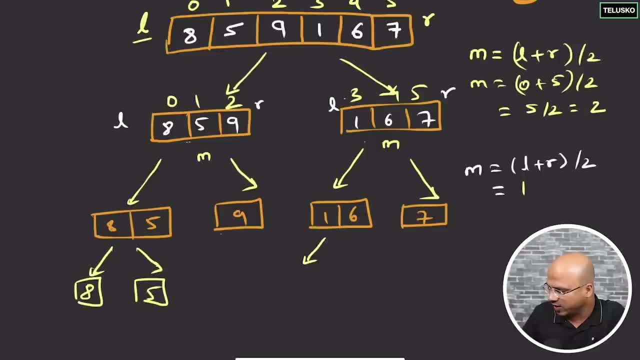 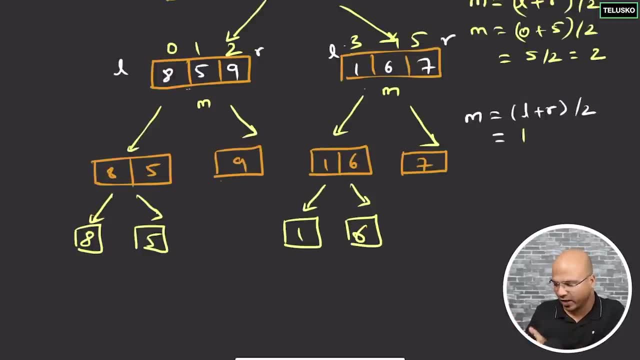 is 8 and 5, and again you will divide this, you will get two values, which is 1 and 6. so that's how you can divide and at the end you will get the individual values. now, still, we can persist the index value because we are not physically dividing them, we are just virtually dividing it. 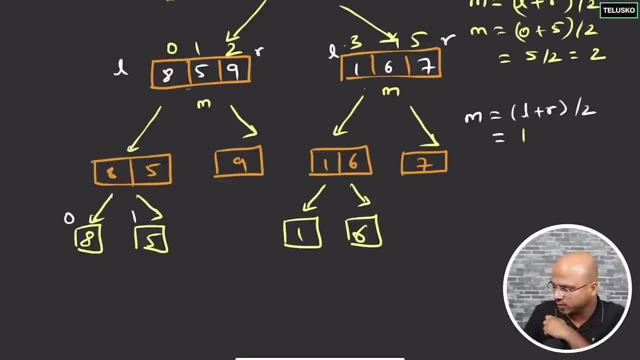 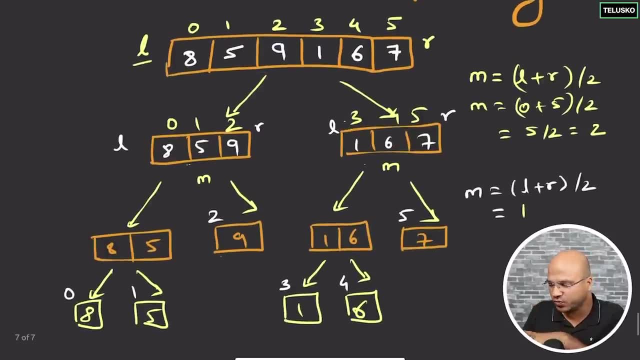 right. so index value for this is 0, 1, 2, 3, 4, 5. the index number remain same and if you compare the actual list, we got the index value and the values are same, right. so till this point we have not done any sorting part, we just did the divide part and now it's time for the conquer. now when 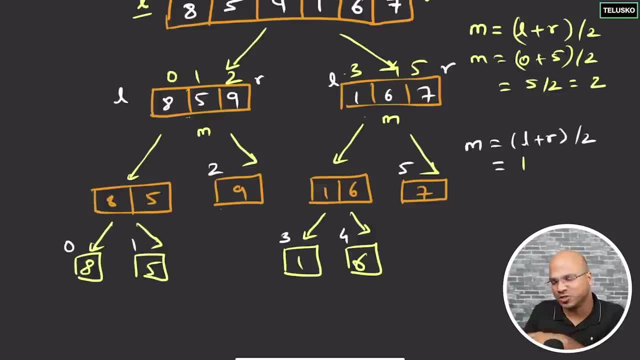 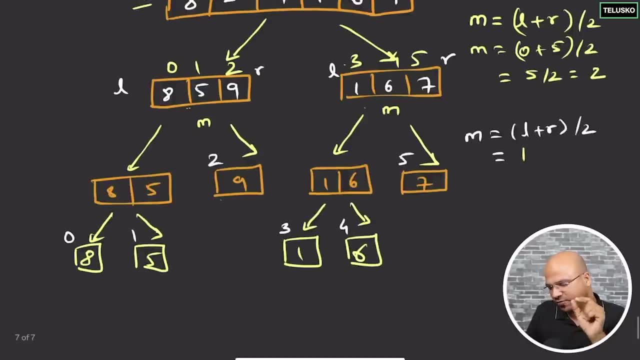 you say conquer, it simply means that you need to sort this value. so whatever value you got at the end, sort them. but if you observe, they are already sorted because each element, if you compare, if you say 8, this list is sorted. when you have only one value, it is by default sorted. okay. so sorting is. 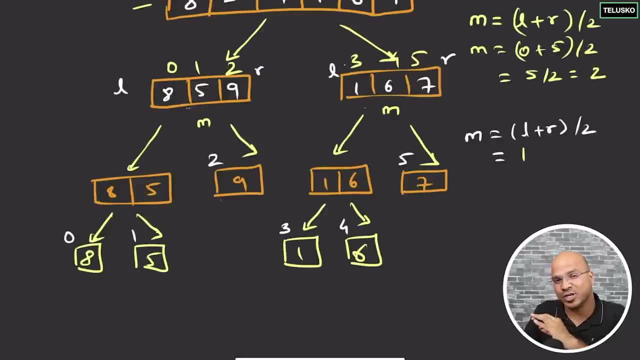 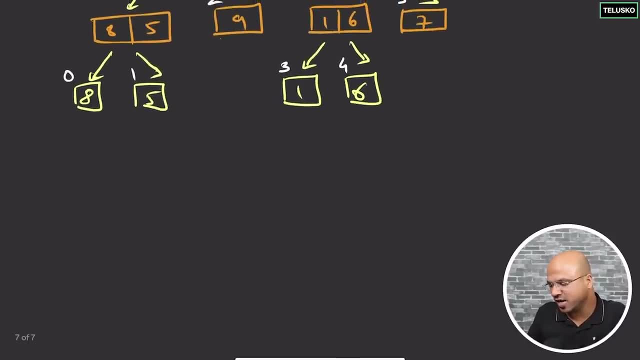 done, so conquering is done. basically, the next step is actually is to merge them, and the actual fun starts here. now, when you, when you say merge, what it means? so basically what you do is you start with the first two values and then you merge them. now, merging is important. so when you say we, 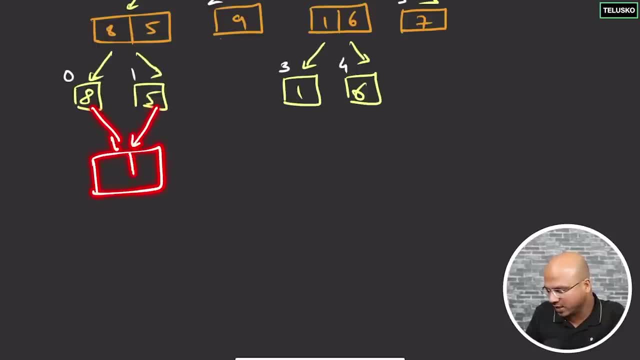 are merging 8 and 5, of course you will get a list and you can again say 8 and 5, but no, this is not how you will merge it. so the way you will merge it is this: so you will take these two values and 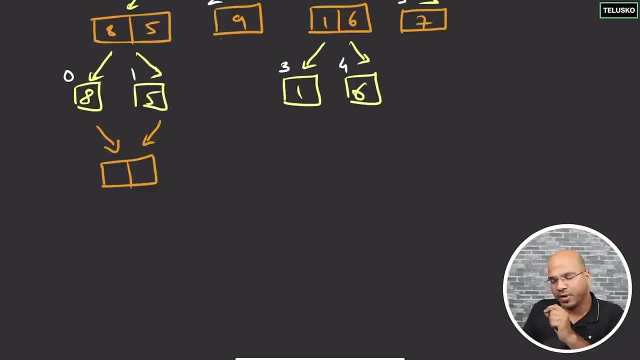 merge them into another block. you will get two values, but when you are merging it you will compare these two values. so which is less here? so if 5 is less, you will put 5 here and then you will put 8 here, because that's the only. 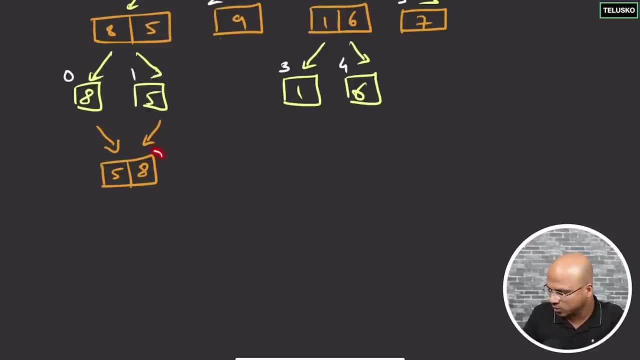 remaining element, then you, you think about merging, so you will. you will merge this two. now, when you are merging this two, of course you will get three values right, so you will take it take three values here, and this is coming from here. so these two values and this one value, now how will you merge? 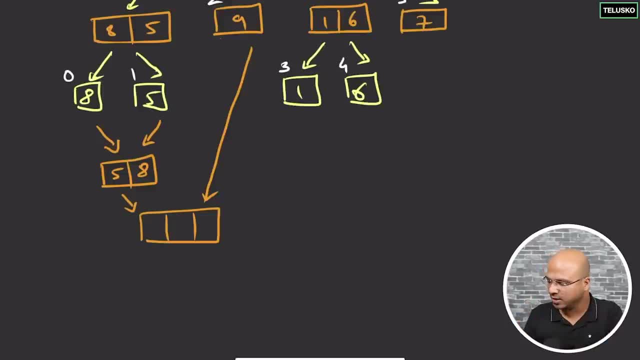 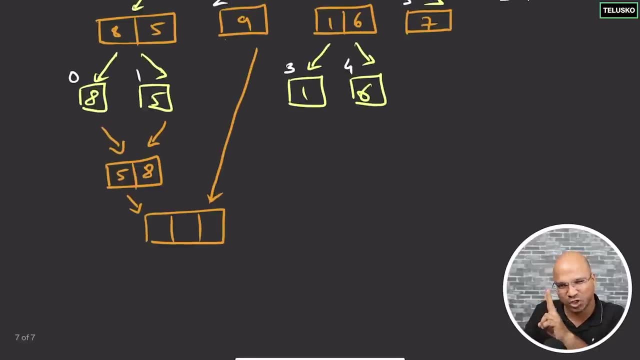 now, since we have two different lists, or two different values here, or two different areas, we can say: when you want to merge, that's where the actual algorithm starts, because when you, when you are merging two values, you can simply compare smaller or get greater, but now we have three. 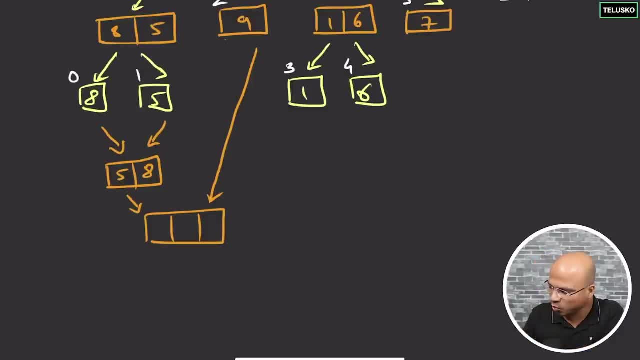 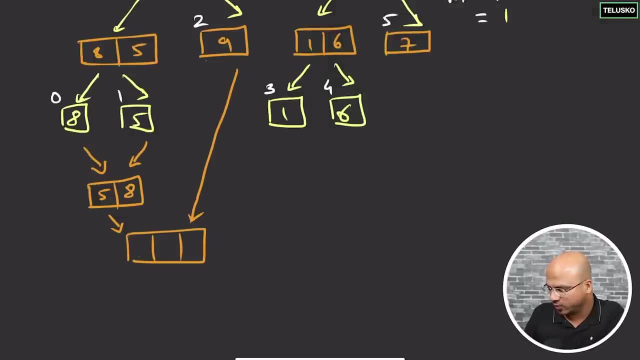 values. in first we have two, in second, we have only one. so what you do here is you basically compare these values before adding them. so what should be the first value? now we know that the previous array is sorted right and then, in fact, both the values are sorted, both the arrays are sorted when 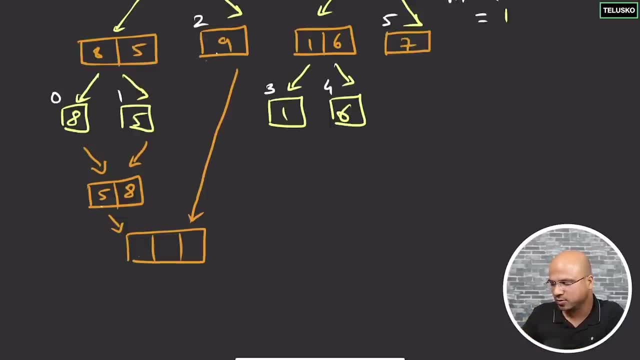 you combine them. what you can do is you can compare the first two values, only the first two values, not eight, only five and nine. so which is smaller? five, so you will put five here. now, since five is done, you can simply say: okay, i'm done with five, now let me focus on eight and nine. so which? 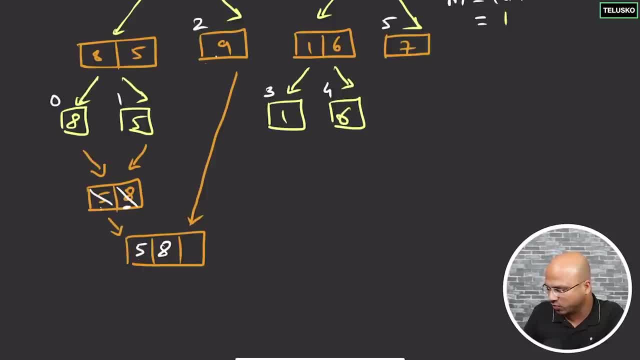 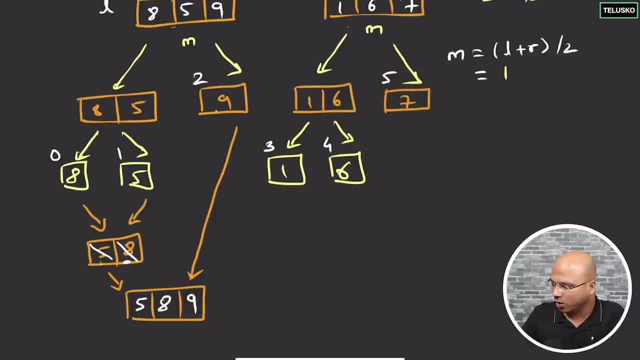 is smaller, eight, and then the only thing remaining here is nine. so we'll put nine here now. that's done. now let's combine this three, which is a one, six and seven. now, first you have to combine this two, so you will get another box here, which is one and six. so we will compare. so it is one and six because they are sorted. so now we will. 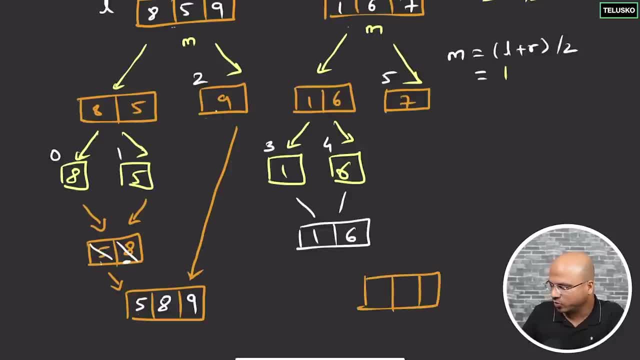 combine the next part. you will get three values here. now, when you get three values, what we are doing is we are basically combining this section and this section, same steps. you will compare the first two values, so one compared with seven. so one will come here. this is done. then compare six and 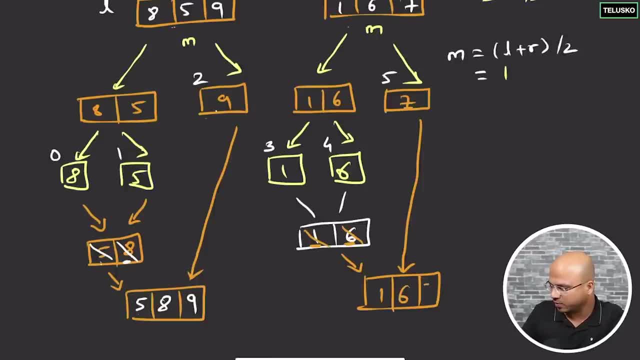 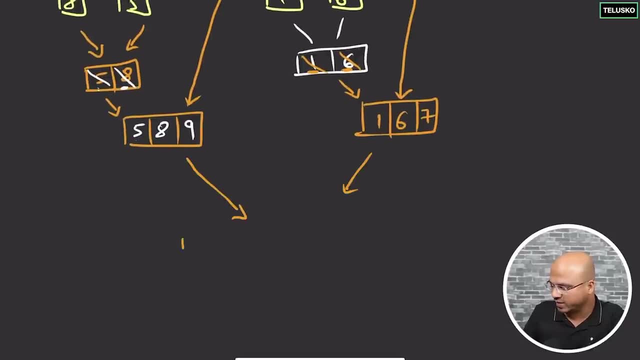 seven, six will come here. this is done, then seven will come here. okay, and then now the major work starts. we have to combine this two. now, when you're combining these two, you will get a bigger array of six elements. so one, two, three, four, five, six. so we got six box. now what you will do is you, you have, you got two areas, and we know that. 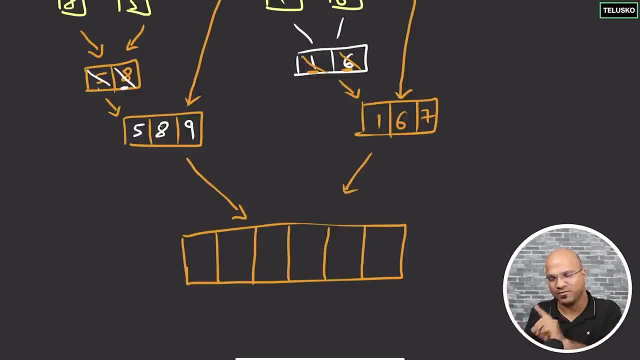 those two areas are actually sorted. when you combine them again, you will start with the first two values. so when i say, first two values, let's come, let's compare five and one, so what you will do is we'll compare, okay, five and one, which will come here, so it is one. so this is done. 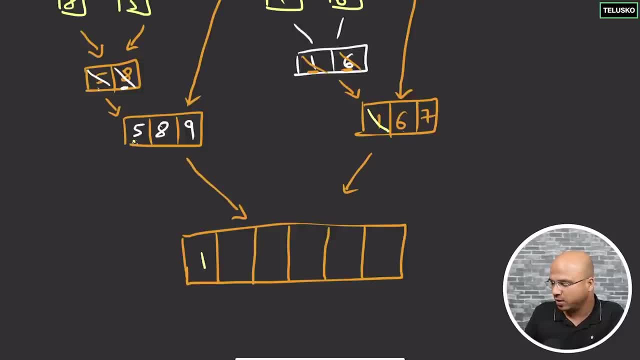 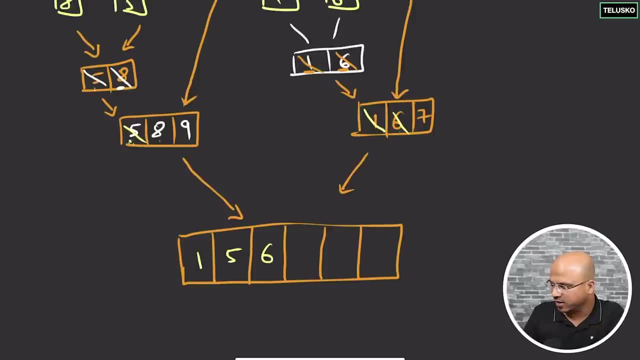 then you compare six and five because, far still remaining right, so five and six, it is five, then eight and six, which is six, so five done, six done, then eight and seven, so which is seven, so seven done, then eight again. now we don't have anything compared to compare from the next array, so you can simply take these two values as it is. 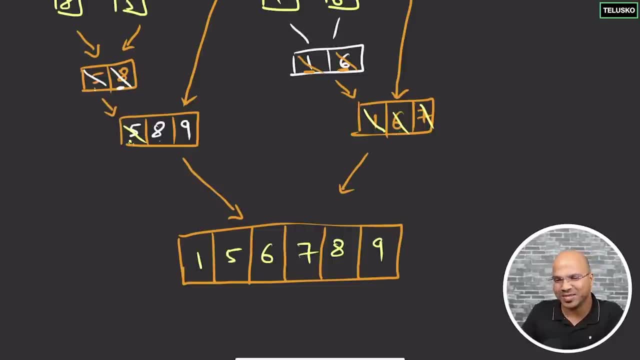 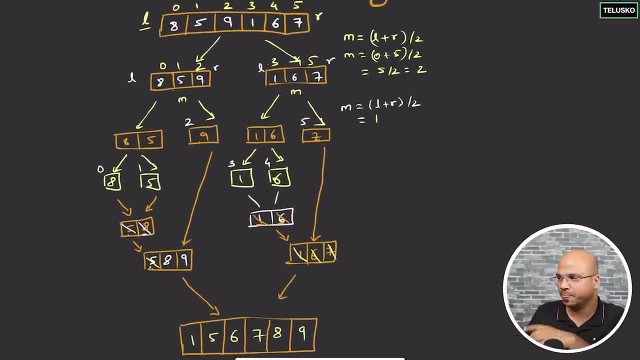 here. this is merge sort. okay, so you get this audit value. i hope, yeah, you got sort of value. so this is how basically the merge sort works. that's how you basically divide and you combine. but if you want to do this in programming, how will you do it? and we'll keep this as a reference. 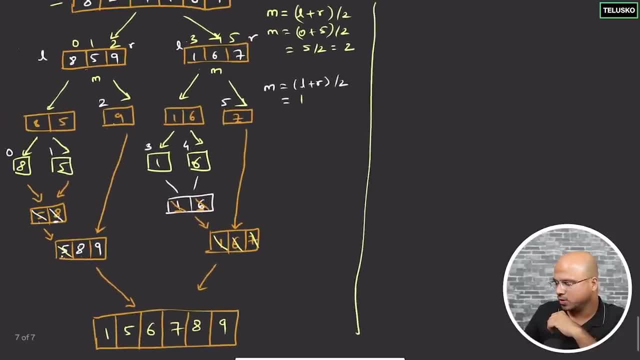 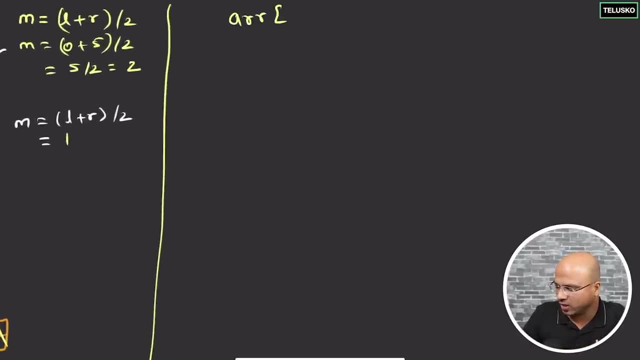 so we can divide. we can write this section here so we can compare with this. now, if you want to write an algorithm for this, first of all you will get an array. of course. now in this array you will have some values and we can take the same values which we have here, right? so let's say we have an. 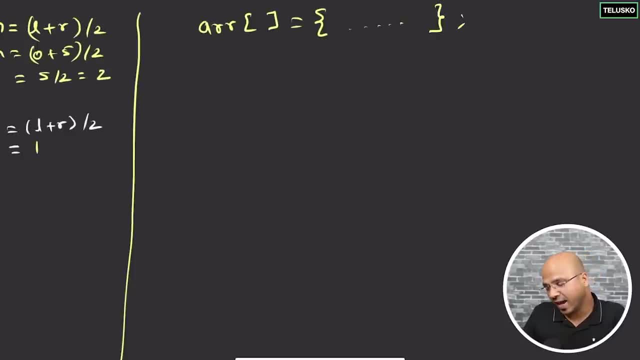 array with some values here, the same values which we have, and then the next step is you basically need to create a function, let's say merge sort, and this is where you can divide the value of the array. so this is where you will do this sorting part. so when i say merge sort, the first 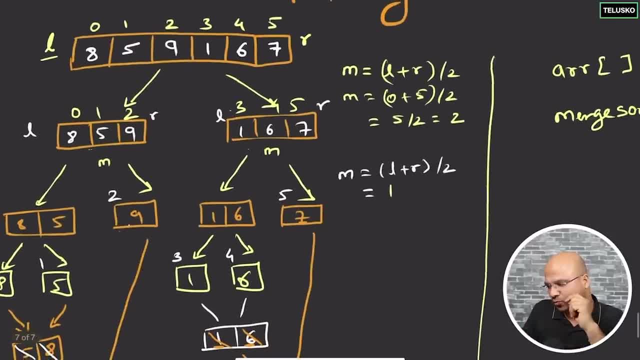 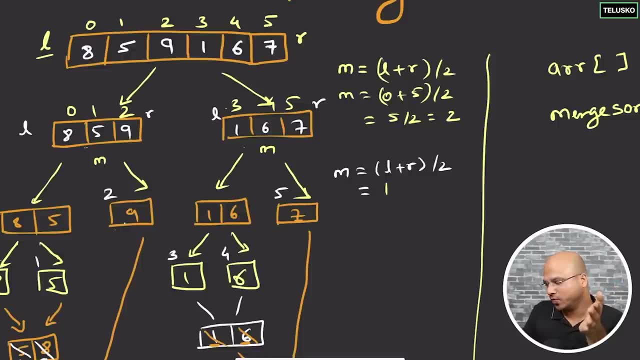 thing you will do is you will say divide. now, when you say divide, you have to pass two, three things: first you have to pass the array, then you have to pass the l value, r value, right, and then if you observe, we are dividing again, you're dividing, again, you're dividing. so don't you think this is? 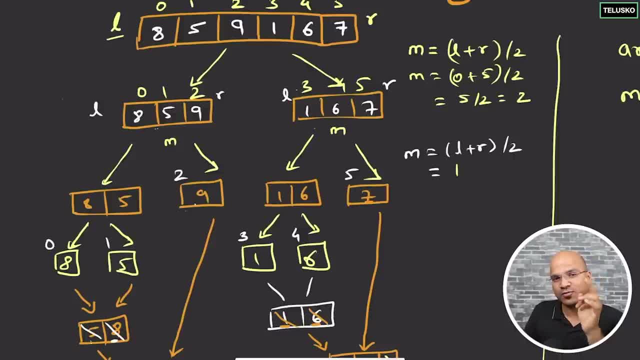 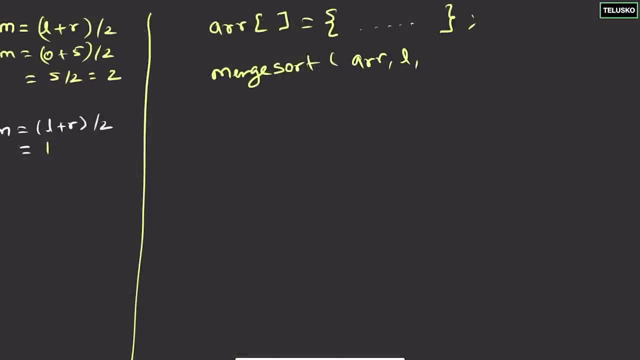 a concept of recursion when you do the same thing multiple times. so we have to do recursion here. so basically, here we have to pass three values, right, so you will pass an array. you will pass a left and right value for each array. now, as this will be called multiple times in recursion, every. 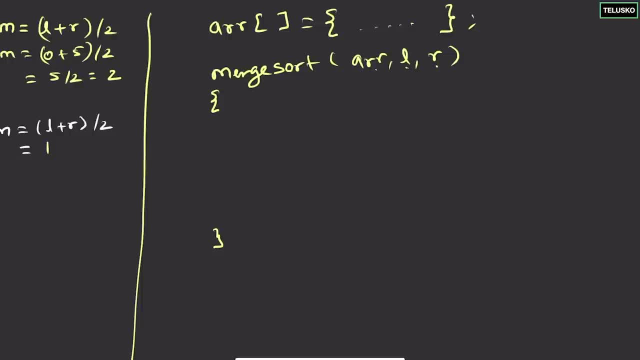 time you have to pass the array, the left and the right. remember one thing: we are not dividing the array physically, we are dividing it logically. so even if you divide this array, ultimately the values will remain same. okay now, when i say divide what it means. the first thing you 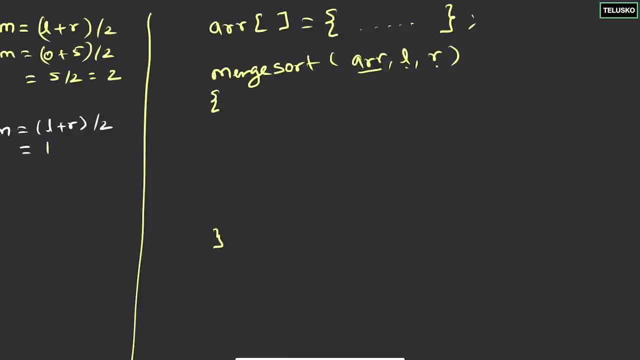 will do is you have to find the median or the mid value so i can say mid. but then since this, okay, so let's find mid here. so we got mid is equal to. we know the formula r, l, p. this is the middle one plus R divided by two. 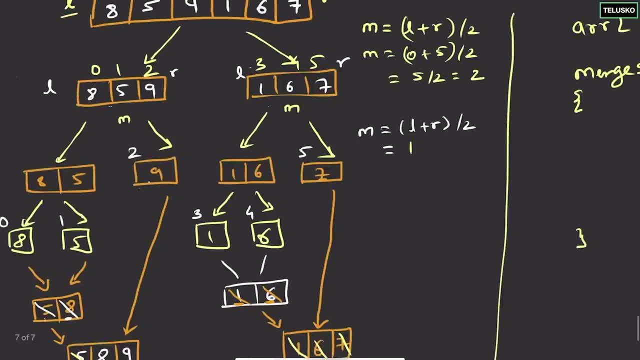 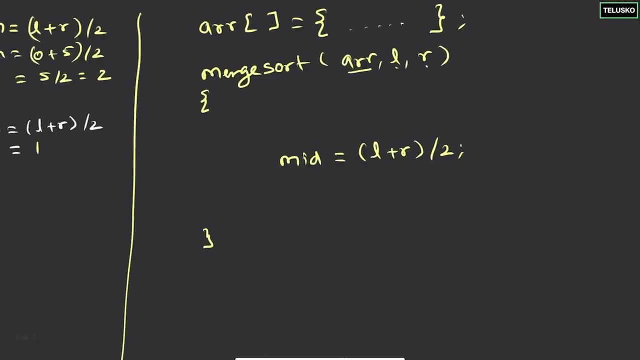 Now, once we got the median, what we're gonna do is, once you've got the median, you will break down into two parts and you will apply the merge sort in each section. So what I'm saying is, when I'm calling this for the first time, 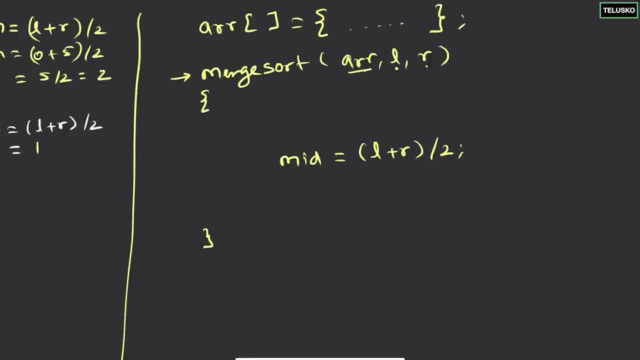 I'm passing the entire array with the L value as zero and R value as five, which is the last index. But again I'm going to call the merge sort by passing different values. So I'm going to pass ARR. Next I need to pass the first array index value. 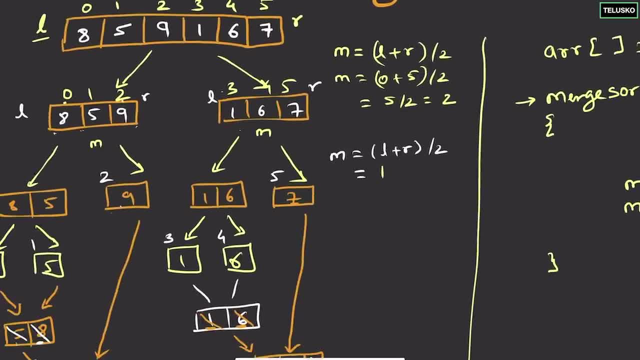 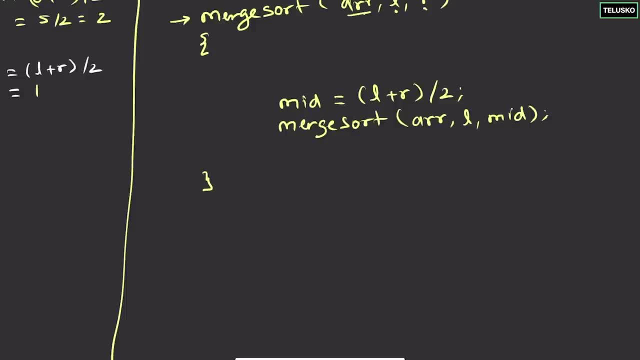 So the first array here starts from zero to two, which is the median. So starting is L, ending is median, or middle value or mid value. we can say Again I will call merge sort. for this second array, Again I have to pass ARR. 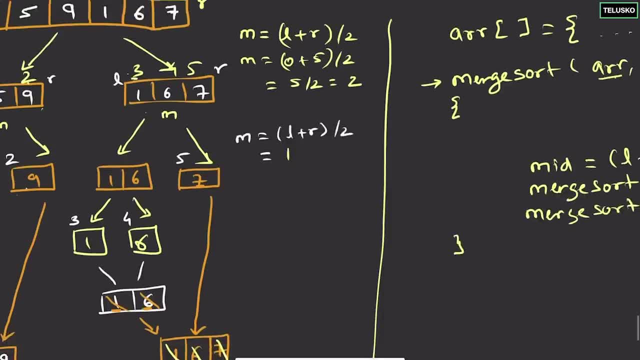 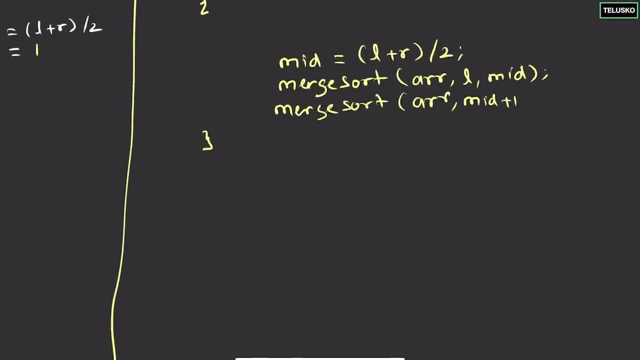 but this time you have to pass. if you look at the values, you have to pass three and five. Now where do we have three? We don't have three anywhere. so we can say: mid plus one, So mid is two. so mid plus one is three. 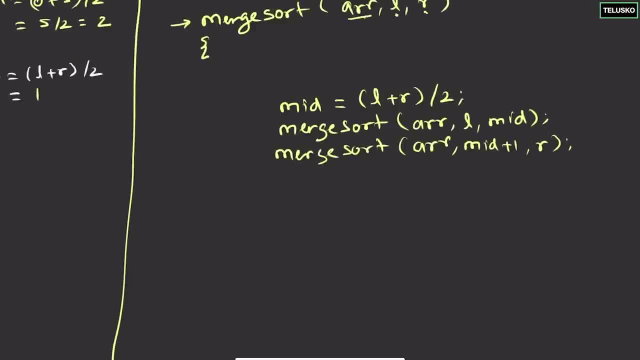 and the ending is right. Okay, so that's how you call the merge sort. We have to remember one more thing: After doing merge sort, which will break it, we have to merge them as well. So when you say merge, you have to pass four things here. 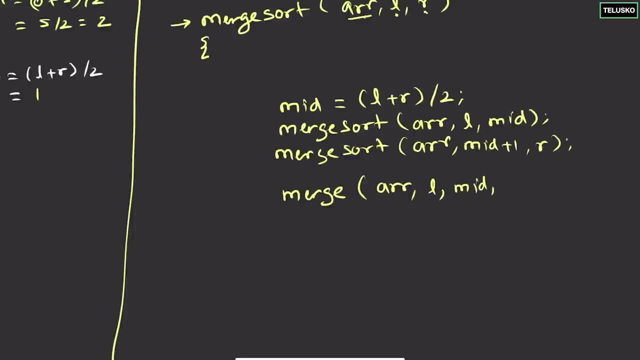 First the array, the left value, the mid value, and you have to also pass the right value. Again, we'll see the logic later. but this is the merge you have to pass. But if you call the function by itself, 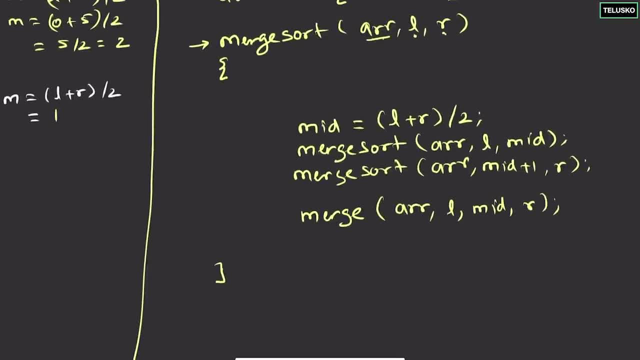 you can see, merge, sort, merge, sort is calling itself, but don't you think there should be a limit when it should end? So of course there should be a condition as well. When your left is less than right, then only you do this, otherwise stop. 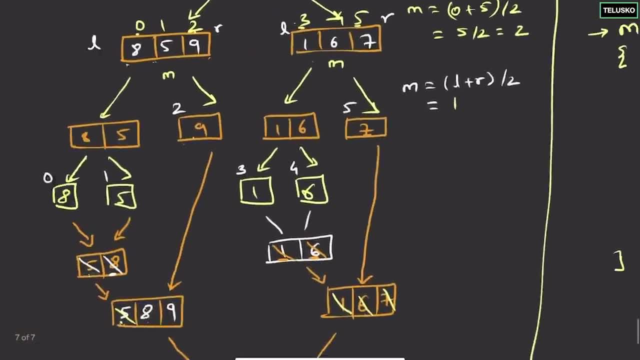 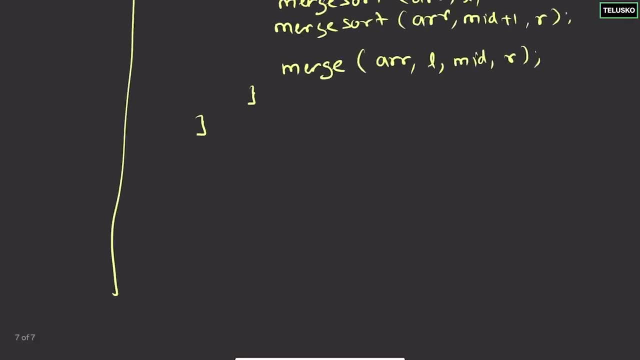 Okay, this is your merge sort. So by doing this, what you will get is you will get the values divided, But where's the concept of merge? We are calling merge, but we are not defined the merge function yet. Now this is where things gets complicated. 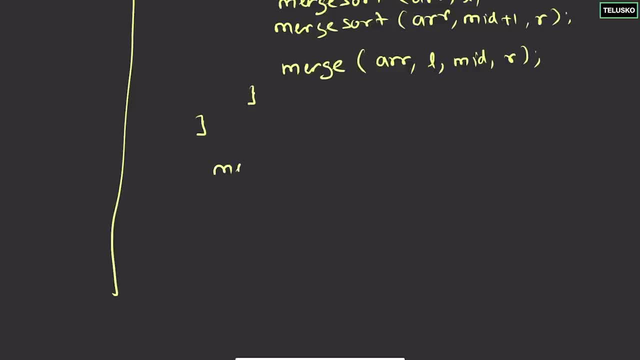 Not exactly complicated, but it's a lengthy process. So what we need to do is, when you say merge, of course you have to pass all these values here Now in this merge. what we are going to do Now, basically the first thing here, is: 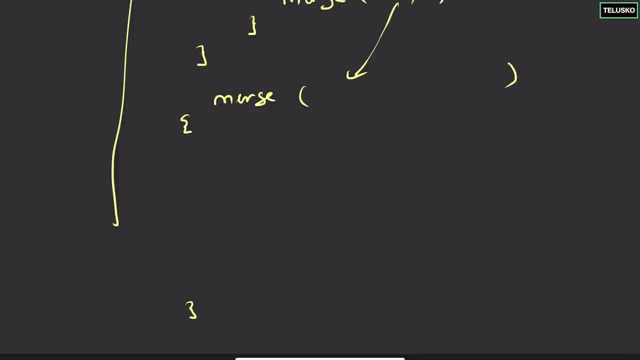 you need to create two arrays. So I will not write the logic- exact logic- here, but let me just draw something. What we need is we basically need two arrays here. When you say merge at one time, you need two arrays. 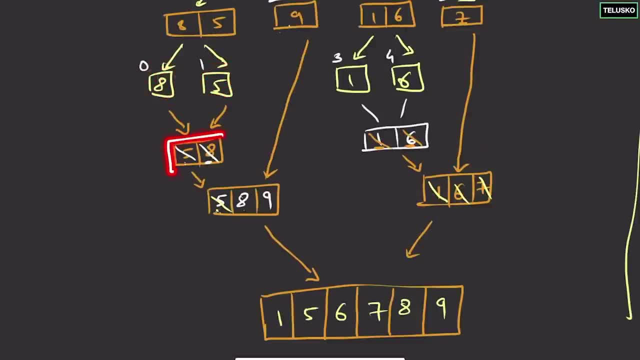 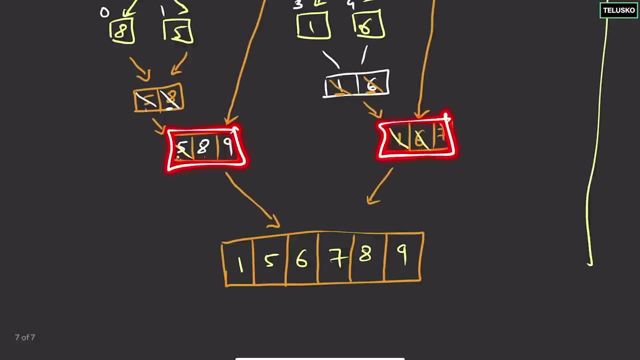 Example. so when we were combining this two, we got one array. So at one point you need two arrays to combine so that you will get one big array. Same goes here. When you got two arrays here, we need to combine them to get a big array. 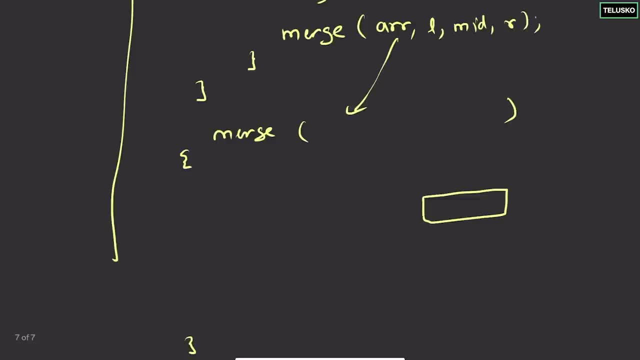 So that means every time I call merge, I need two arrays. We'll call them, let's say, left array and right array. Okay, so we got two arrays here. The next thing we need to do is we need to copy the elements of the left array and the right array. 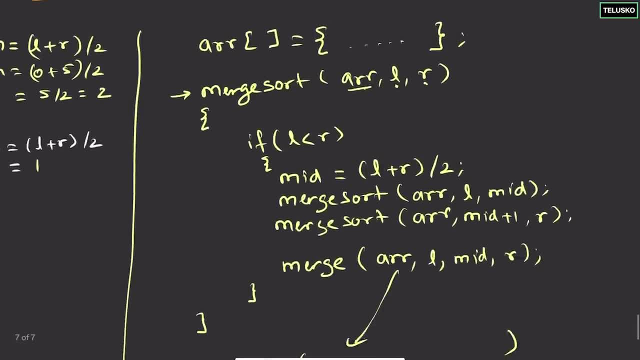 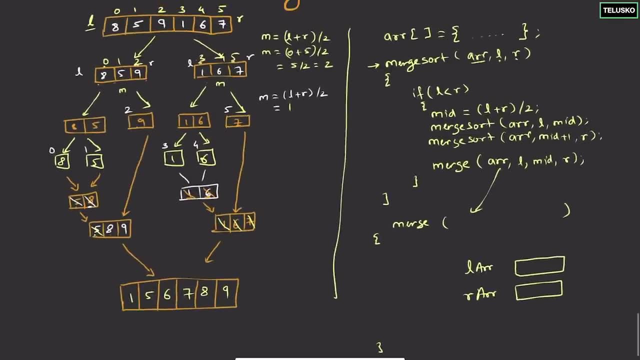 This is empty at this point, So we need to copy these values from the actual array. okay Now. so we need to write a for loop which will copy data from the array. So, basically, it will copy data from the array and put them in this list. okay, 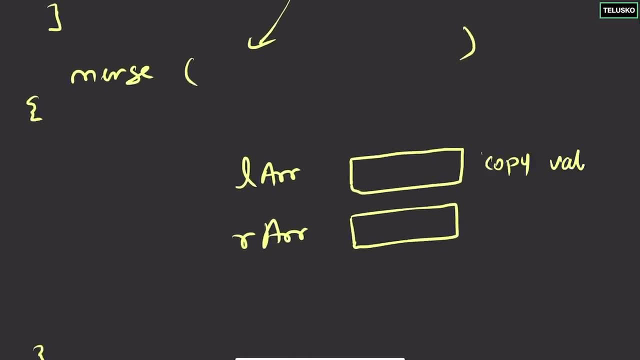 So maybe I will just write copy values Again. we'll see the actual logic in the code itself. Okay, next thing we have to do is, once we have done with the copying part, you will simply use these two arrays to combine to get a bigger array. 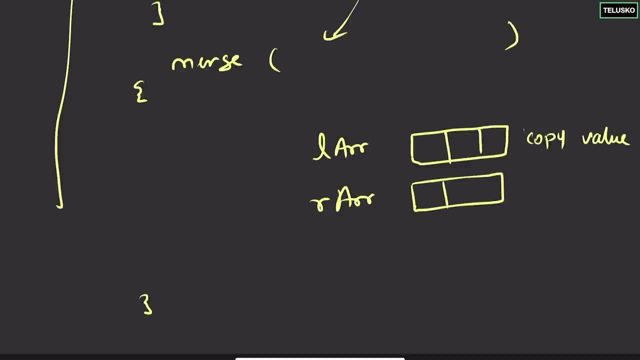 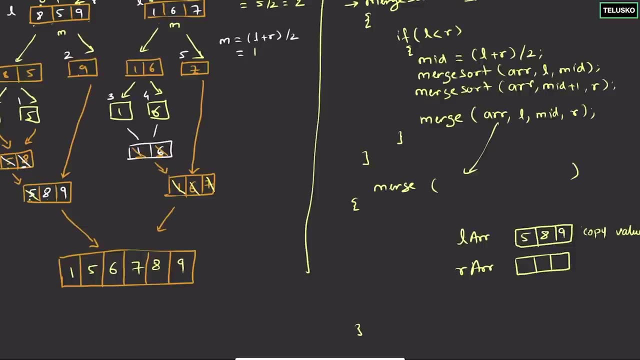 Now, how will you do this? So, of course, there should be partition here. There should be some values. So what we will do is: let's compare, let's work with the last values here. So we got the last value as five, eight, nine. 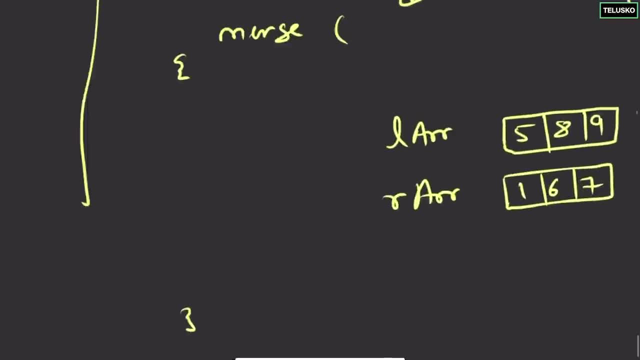 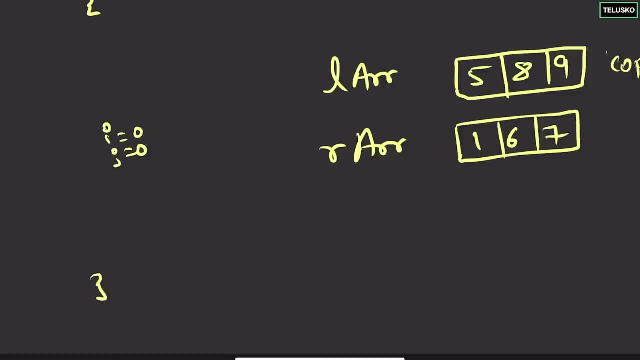 and one six seven. So the logic of combining this is: you will need multiple variables here. You need a variable array, you need a variable j. Now why we need these two variables? one to represent this particular array and one to represent this particular array. to iterate: 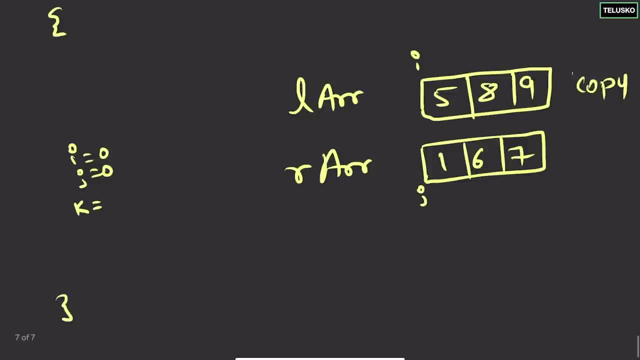 Then we also need a k, which will be used for the big array which you're going to create. So from these three values, or three three values, you're going to create an array of six right. So k will be handling this part. 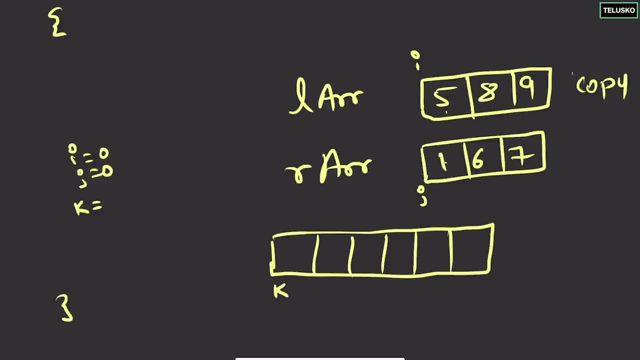 Now, every time you copy one element, so let's say, when you compare five and one, and you know that you're going to copy one here. so basically the j value will shift here. right, Because this is done. The same thing goes here: 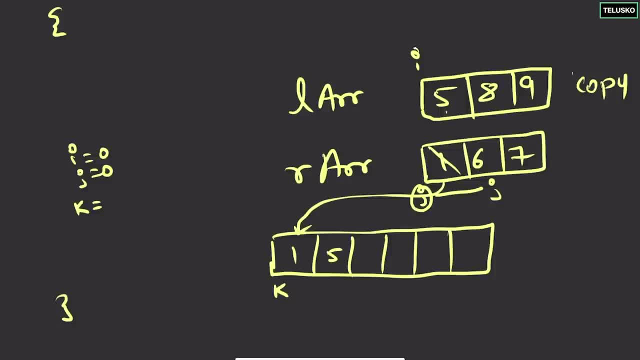 So once you've got one, next time you will get five here. then you have to increment this here. So i goes here. And of course, every time you copy element in the bigger array you will increment the value of k. That's the logic, okay. 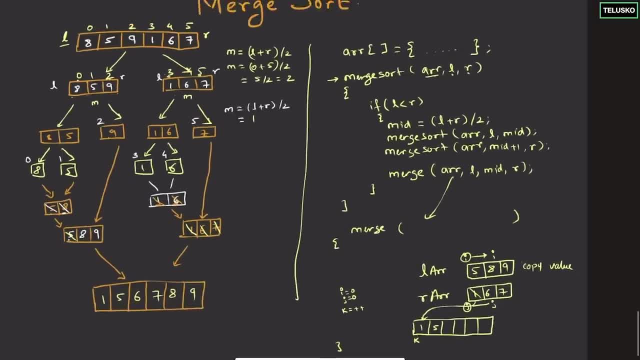 So this is how you are going to complete the merge sort. Now how exactly you have to write the code that we'll see in the practical video. So I hope merge sort makes sense, where you basically break down the entire, you know. 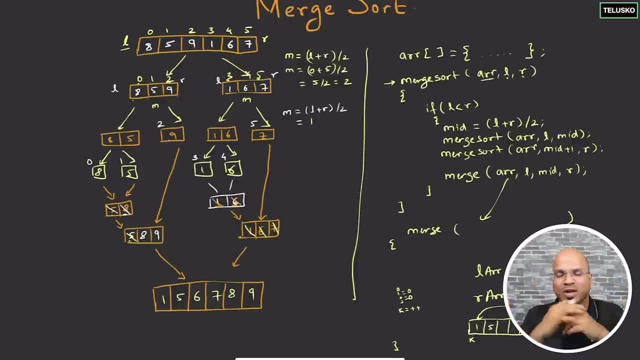 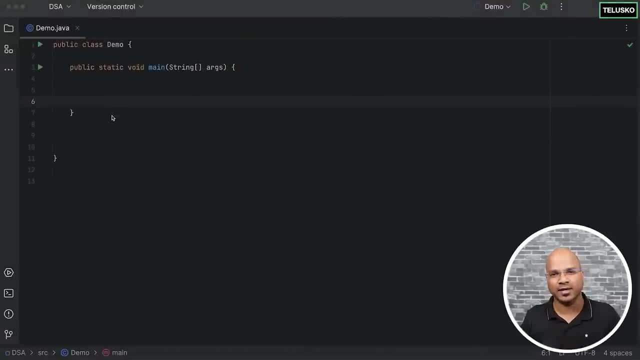 the array into small chunks, and then you combine them to get the sorted values. So now let's implement this logic with the help of Java. Now the thing is: first we need an array, right, So let's create an array here. 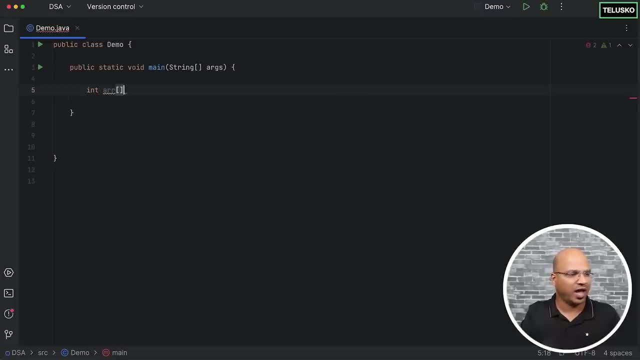 So we'll say int, arr, and this will have certain values. So let's have some values here. We'll say three, five, one, four, six, two. So we've got these values here And let's apply the sorting techniques on this. 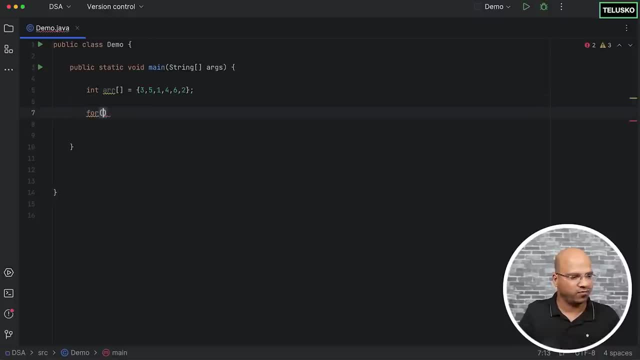 So before sorting I will print some values. I'll say for in n in array and let's print this values. So I will say print n, but I will also make sure that I will put a space. I will not print on new line. 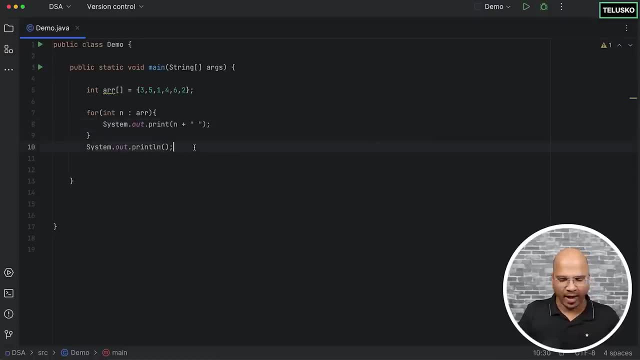 And once it is done, I'll print a new line And then after sorting also. so I will say this: I will just write it here after sorting. So here let's do the same thing And let's say after sorting, it should print some value. 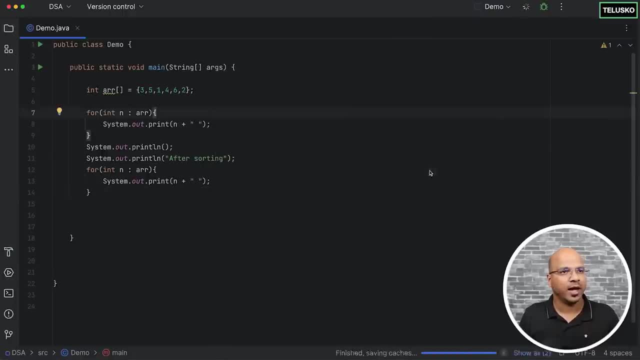 But at this point, if you run this code, let's say, after sorting it should print some value. Let's run this And you can see in the output they both are unsorted. So because that's why we have to do some sorting here, right? 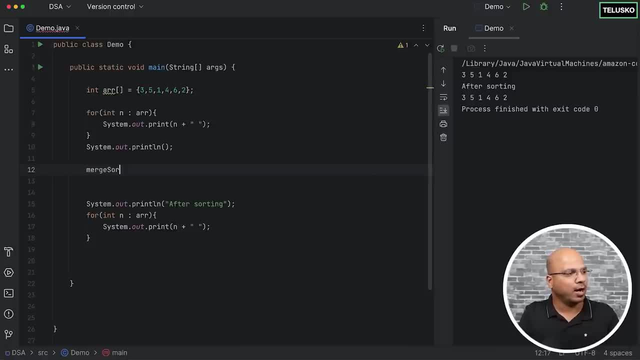 So let's apply the sorting logic. So what I will do is I will simply call a merge sort method, which will basically accept three values: the a, r, r, the l. now l here is zero. And then you have to also pass the arraylength minus one. 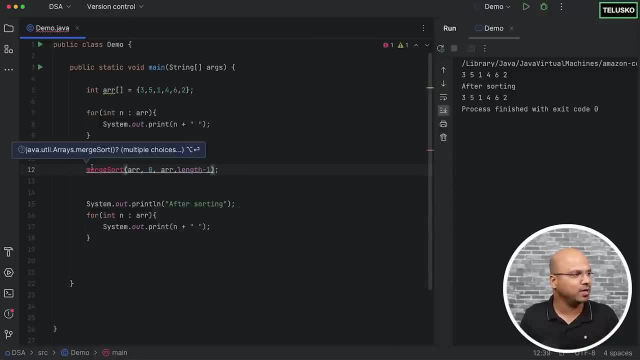 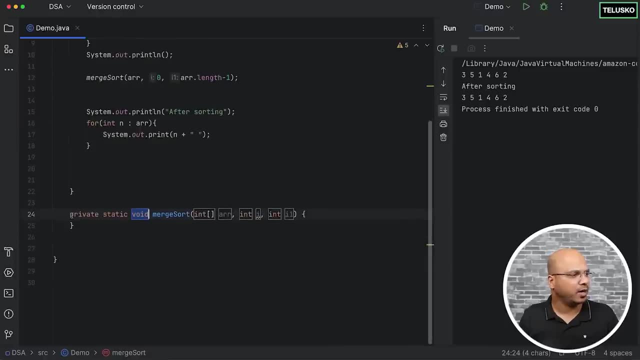 Basically, you have to pass the r value as well. Remember, we have to pass three variables. Now, since we don't have this method, I will simply say: more action. create this method and you can see. we got this method here. 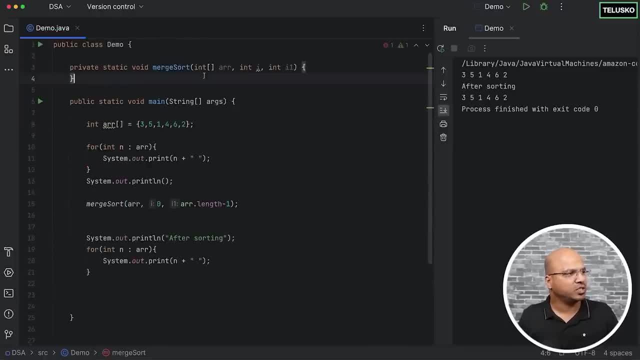 And let me just put this method, not here, but on top. Now this is where the actual logic is going to happen. So you can see we got two variables: This should be l and this should be r. So left and right. 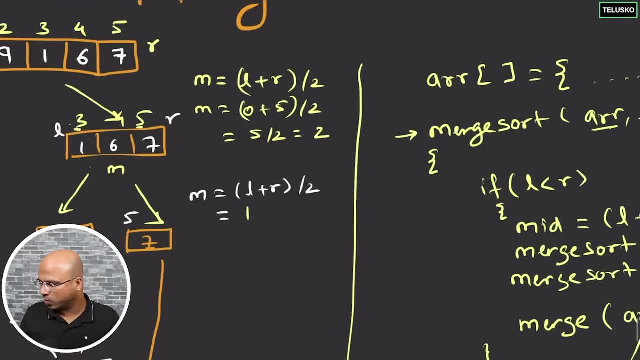 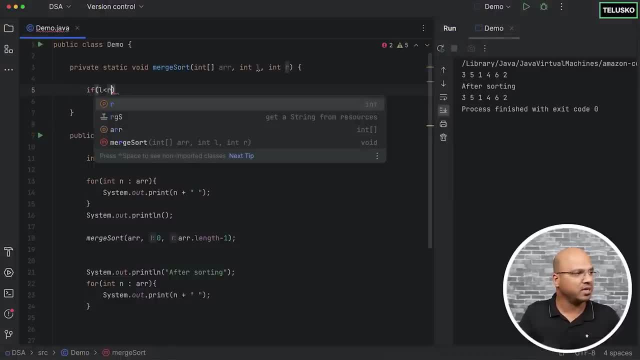 Okay, Now as for the logic, if you can see, in our logic we have already mentioned this logic. So basically what we do is we have to first check if the l value is less than r, then only you do certain things. 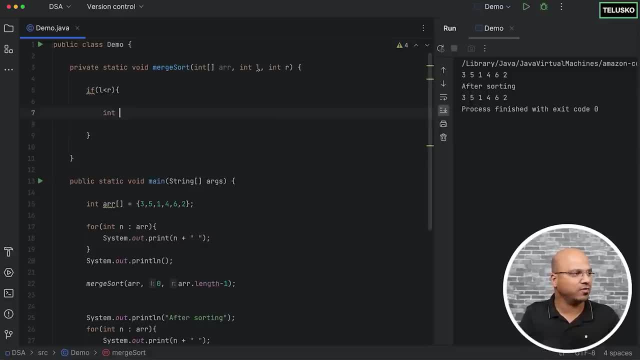 And what are the things you have to do? Basically, you have to find the middle value. So I will say int mid is equal to l plus r divided by two. And then you have to call merge sort two times Again. I'm just going with the logic which I've written. 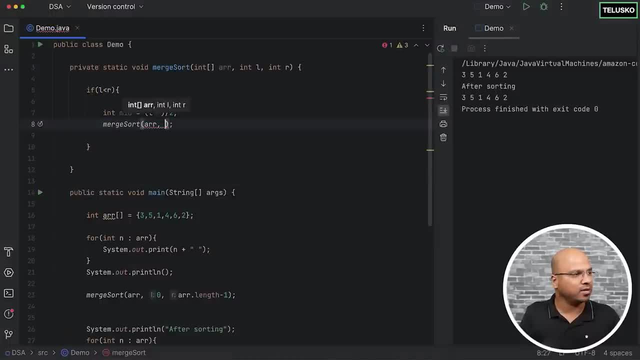 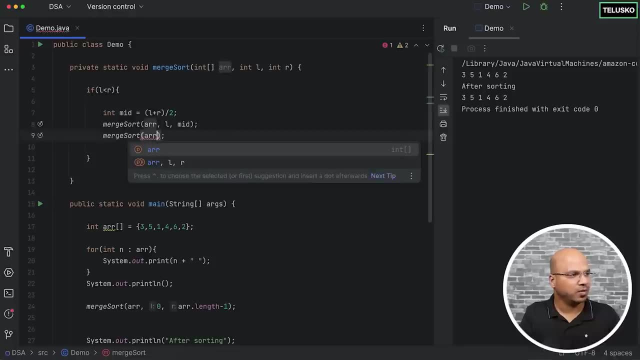 in the code or in the board here. So you have to pass arr, and then you have to pass the l, and then you have to pass mid. That's how you create two different arrays, So mid plus one and r. Okay, and then you will simply say merge. 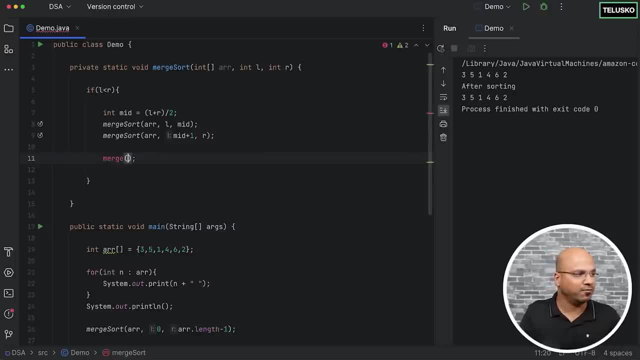 Of course, right after doing the sorting, after breaking it down, you have to also merge. So, while doing merge, you have to pass three values: arr, you have to pass the left, mid and right. You have to pass the three values. 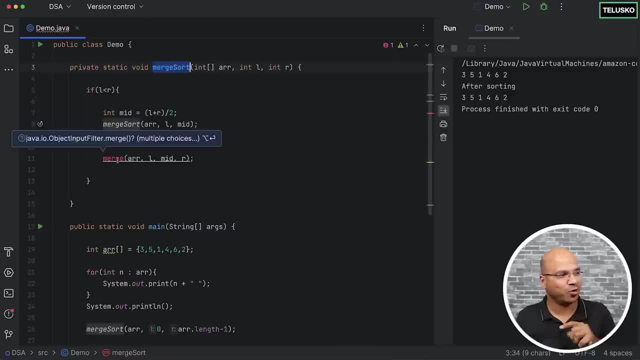 So this is the only logic you have to write inside merge sort method. But then we have to also complete merging, because dividing is very easy. This is how, basically, you are dividing the values. The difficult part is merging them. So let's implement merge here. 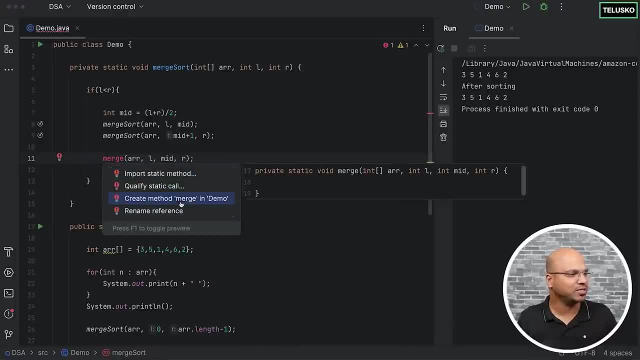 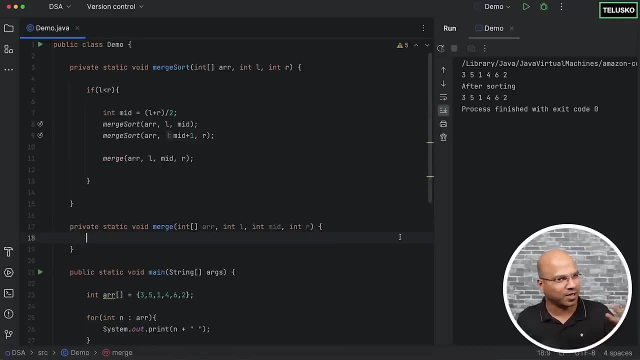 So I will just go back here. More actions: create a method, merge. yes, At this point there are private methods, just because I'm going to call from the same class, But depending upon your requirement, you can just change them. And now the actual logic goes here: the merge. 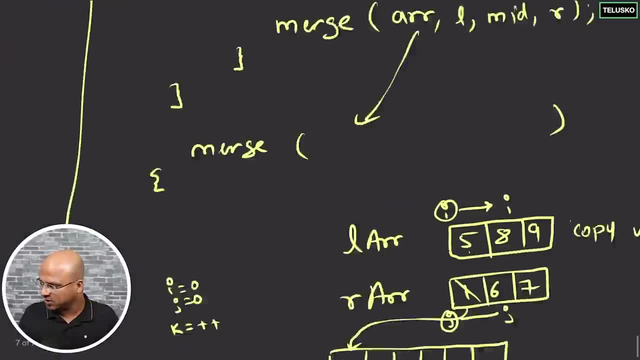 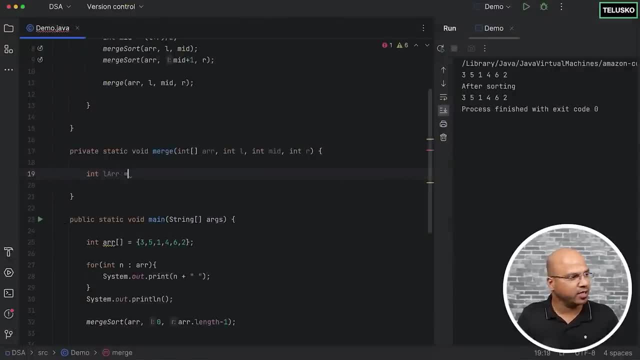 Okay now, as I mentioned, you need to create two arrays here, right? So, if you can see the logic, we need two arrays. Let's name this as lrr, which is the left array, And this will be an array. 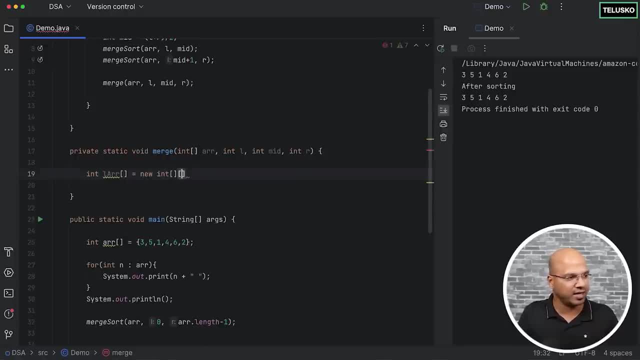 But the question is: what will be size of it? Because when I create this array, I have to mention the size. I don't know what is the size here Now, based on when it is getting called, it will be different size. 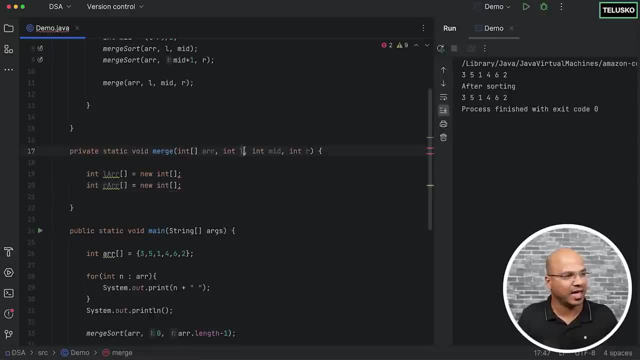 But the question is how we are going to know the size, And that's where this l, m, all this thing comes, or l? r comes into picture. So let's use that and let's get the size. So if you want the size of the first array, 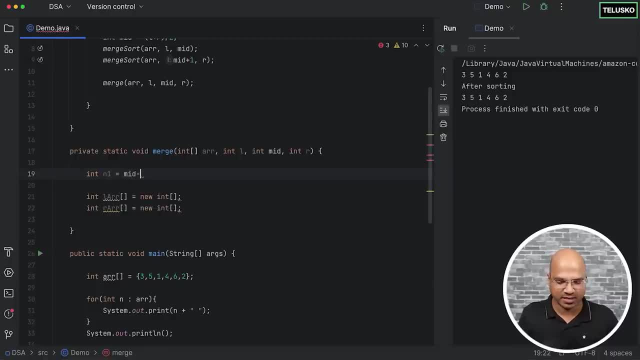 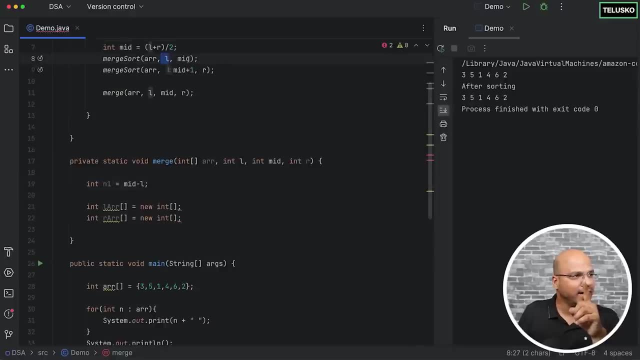 the first section. basically, you can simply say mid minus l, because for the first array it starts with l. If you can see here it starts with l and ends with mid. So if you say mid minus l you will get the length right. 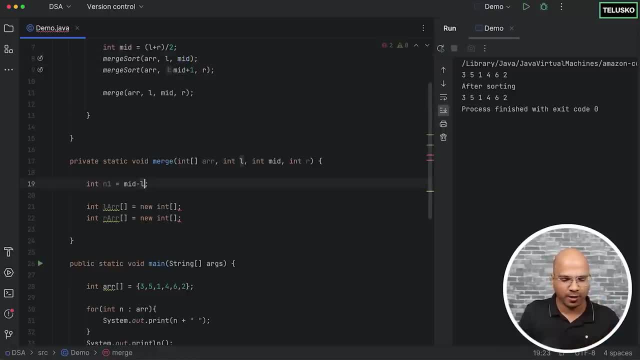 But the problem is, since this is zero indexing, we have to also add a plus one, because mid is not representing the size of the array, It represents the index value. So you have to say plus one, Then you will get the second array length. 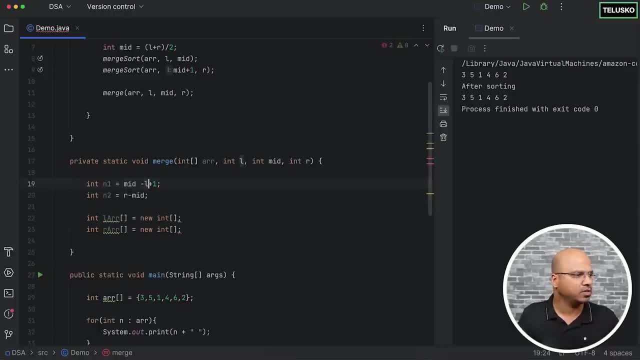 with the help of r minus mid. So we'll just put some space here so that it will be much more visible. Okay, so you can see, we got these two values and this is the size you have to mention here. The first array will be of size n1,. 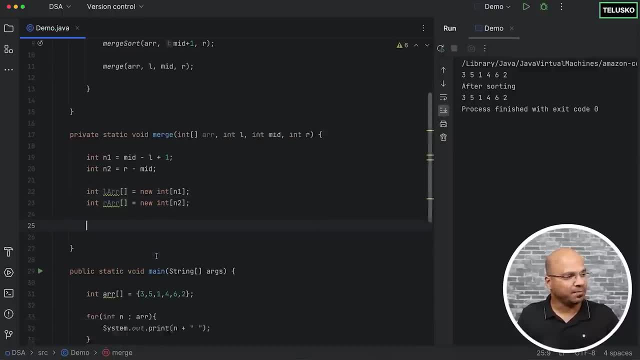 the second array will be of size n2.. That's done. The next step is actually to copy the values. If you can see, we are mentioning the copy values here, right in the nodes. Now, how do you copy value? 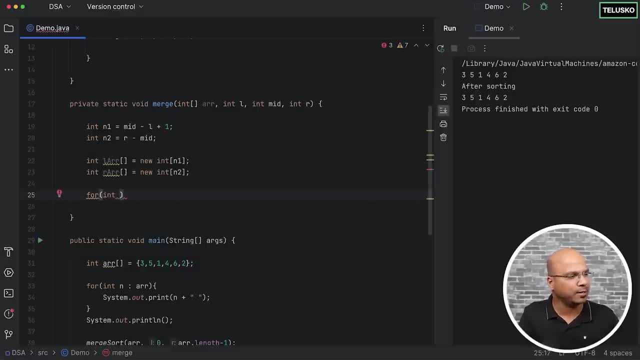 We can use a for loop and let's use two different variables. I will say x and y. this time X is equal to zero and depending on the size of the array. So for the first array the size is n1 and x++. 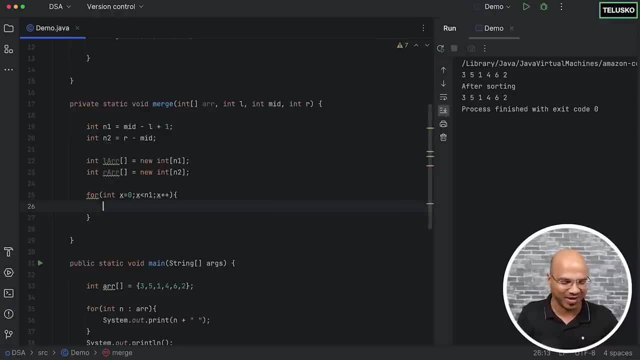 Not used to using x and y instead of for loop, but let's try So. how do you copy So arr, this values, which is x? now how will you get the values So from arr, from the main array? we have to start on the left. 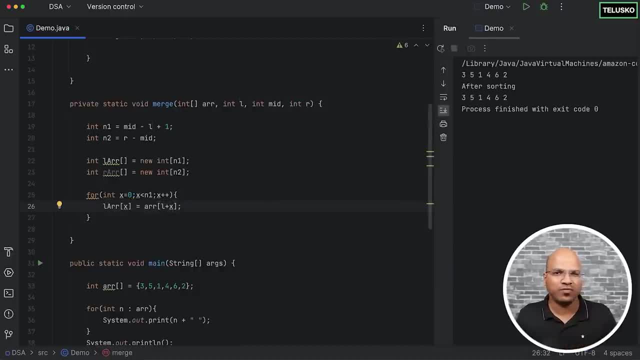 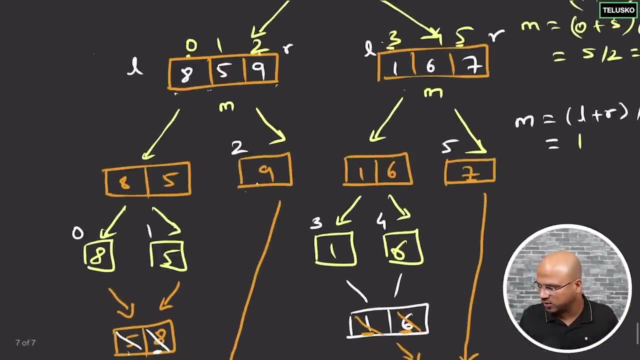 So we have to say left plus x. That's how you get the values. So whatever value of the l is example, if you look at here, for the first array the index is 0, 1, 2.. But let's say, if you're merging the second array, this one. 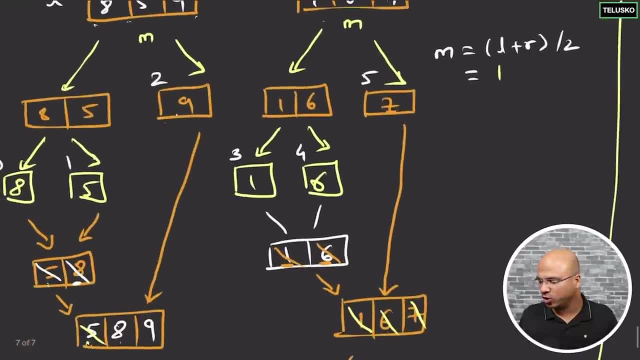 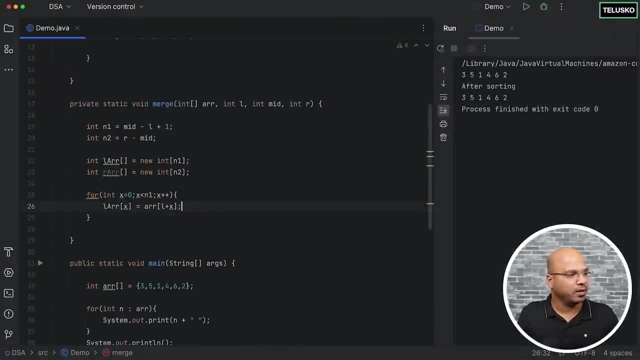 the index value is 3, 4,, 5, right. So whatever value of l is, which is the left, which is three, in this case it is three plus x. That's how you will copy And none. So this is for the first one. 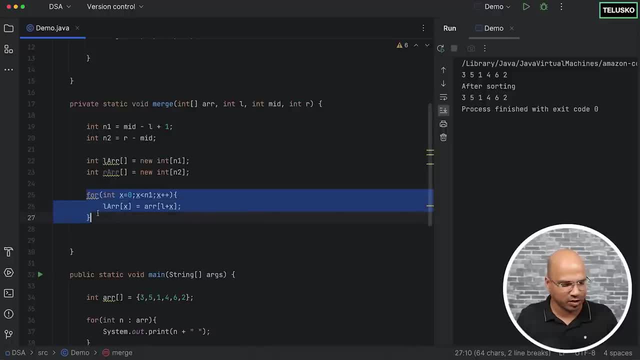 Let's do the same thing but a different value. So I will just copy this for the second array: Okay, we can also use x here, no problem, We can say n2.. And this will go into the right array. But the question is, what will be the value here? 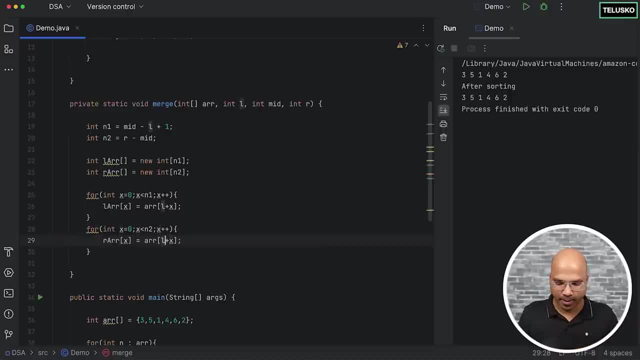 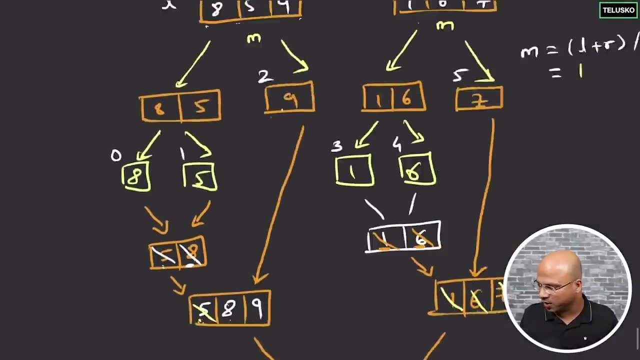 Now any guess. So when you say on the right-hand side, it is your mid plus one, because we are not considering the mid value for the next array Example. if you go up, the mid here was two, but we started with three. 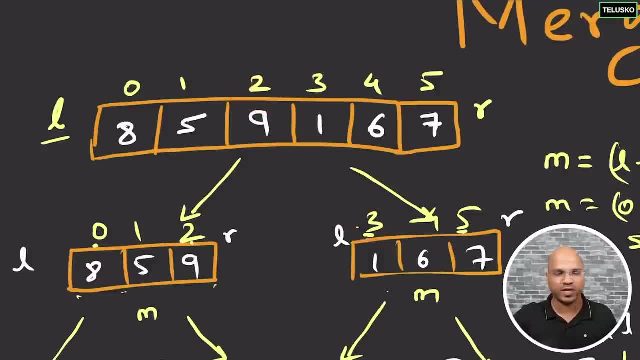 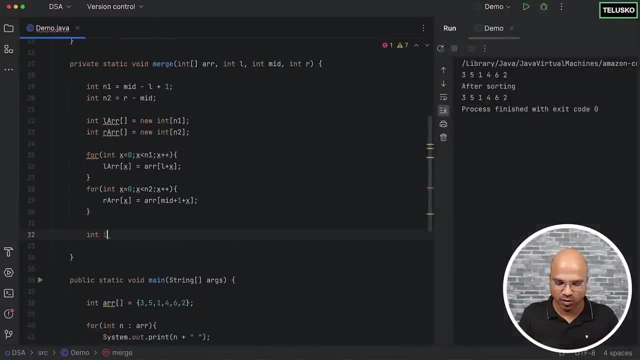 So you have to say two plus one, Mid plus one, so that you will get three. Okay, so we copied. What's the next step? And now the actual work starts of merging And, already mentioned, we need two variables. One: is i equal to zero? 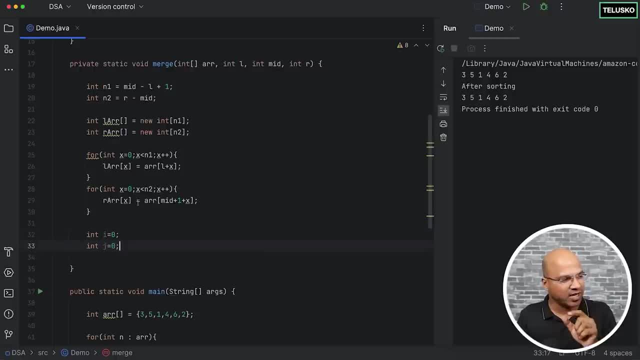 We also need j for the second array. So first array will be counted with i and second array will be handled by j. But we also need one more counter which will represent the main array right, And this value will start with l. 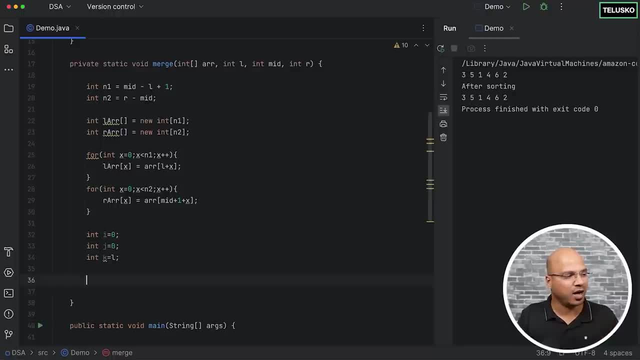 because we have to start from the left-hand side. Now, once we get these three values, let's say, let's start merging them. So we have to do multiple times right, When you say merge, you have to take my value from here. 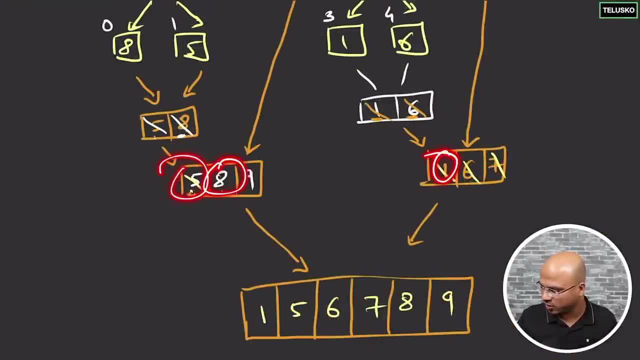 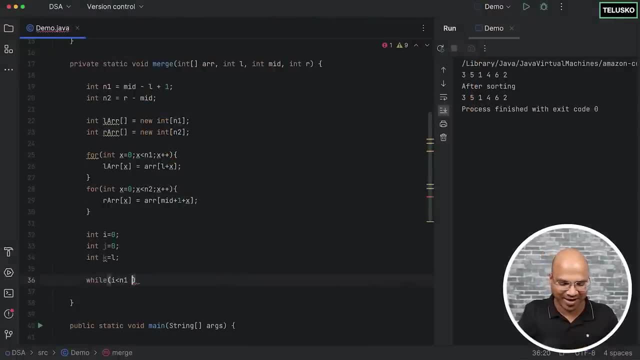 Example. when we were doing this, we would compare the first two values, compare the next two values. That's how we were doing it right? So when to end this, If your i value is less than n1, and not this, and: 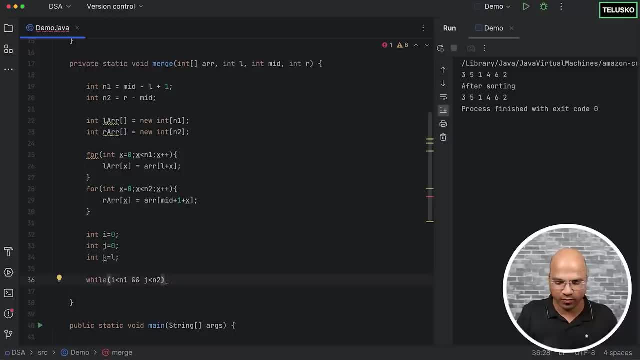 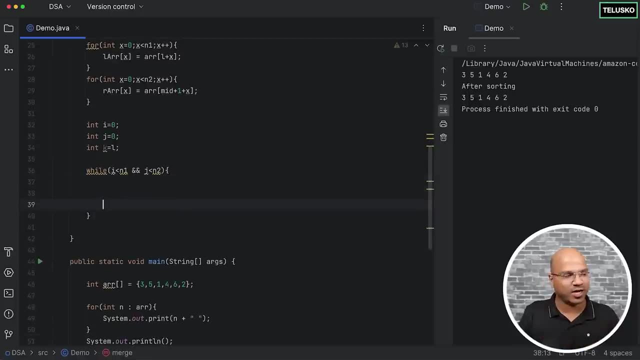 and j value is less than n2,, we'll continue till this point. If they are not true, then we'll have to stop, because that means we have to reach the end. But now question arise: how will you merge? And that's where you have. 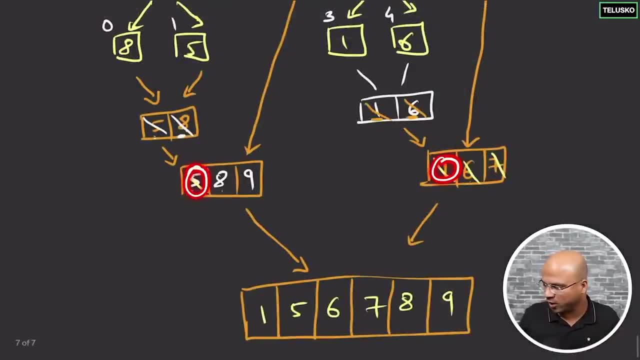 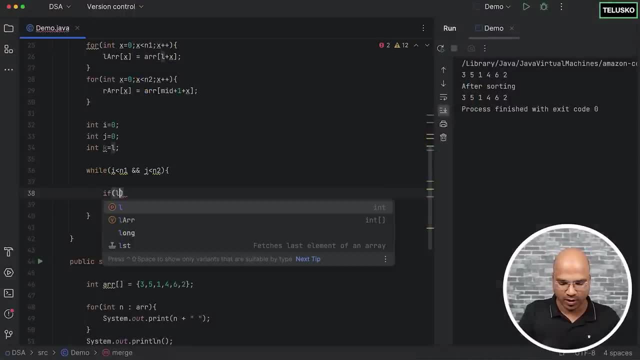 to start comparing values. Now, when you say compare, what it means? Compare five and one. So basically, the first element of this array and the first element of this array, let's compare them. How will you do that? So, simply check if the l array of i 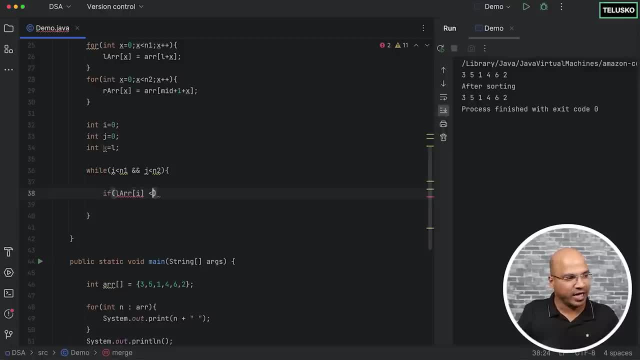 because that's what is representing the l array, which is the i variable. if it is less than- and we can also say: equal to what? if they're equal, Then we have to compare this with the r array of j, If the left one is smaller, in this case. 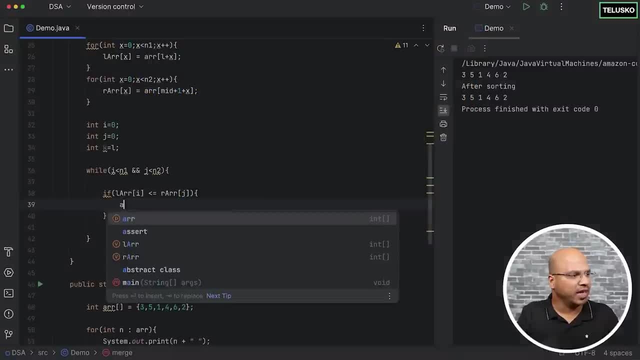 the r one is smaller, not the left one, but let's say the left one is smaller. in that case you will put that into the main array. So array k is equal to l array, not length, l array of i. 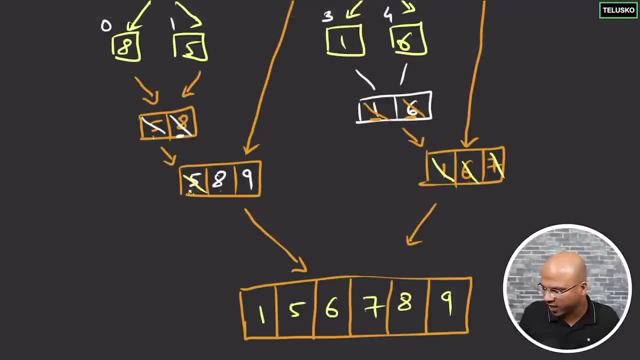 Now, since we have used- so let's say, this was a smaller value- and once we have used this, we have to cancel this, right? I mean, this is done So we can shift our pointer to the next element. How do you shift your not the pointer, but the reference? 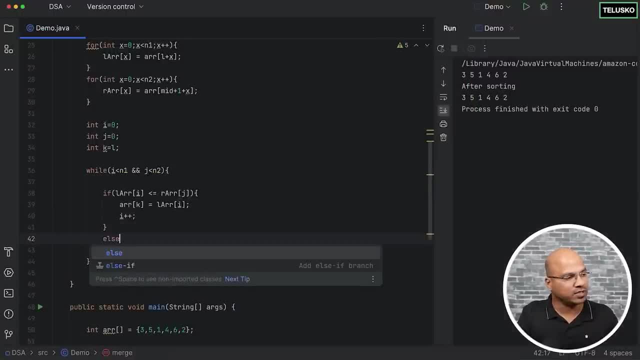 You will simply say: i++ here in this case. But what if it is not same or not? what if it is not the same? But what if it is not same or not? what if it is not the same? But what if it is not the same or not? what if it is not the same? But what if it is not the same or not? what if it is not the same? But what if it is not the same or not? what if it is not the same? In that case, you will go to else part. 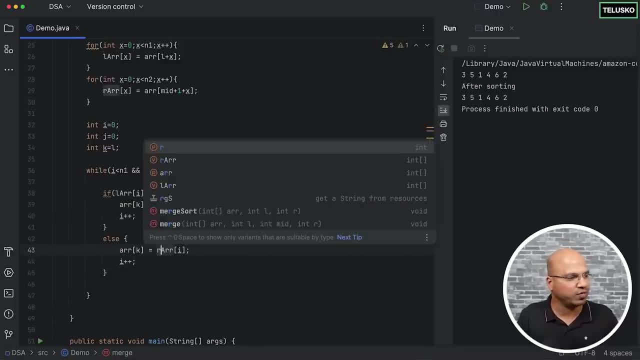 You will do the same thing, but not with the left array. You will. this time you will do with the right array and then the j variable and you will say j++. And every time you run this loop, because, see, after one iteration of this loop. 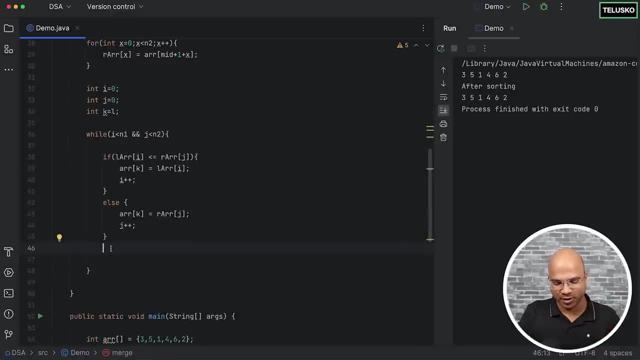 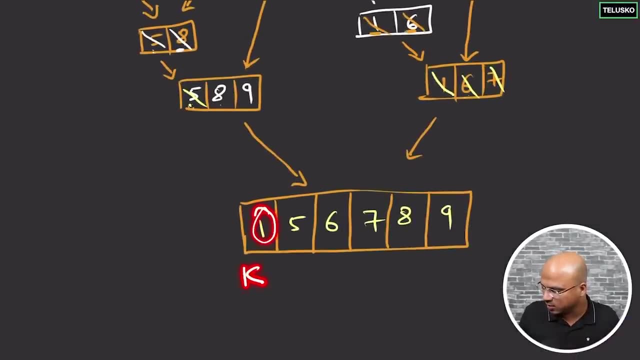 basically, you will get the first value of the array right: Main array. you will simply say k++, Because you have to also increment this. So once i is done, because k is here, once i is done, you have to move k here, okay. 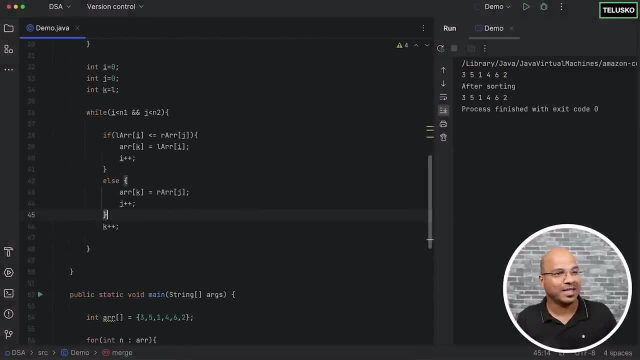 And that's why you're doing k++, And that's it. this is your merge sort. Let's see if that works. Let's refresh this or just rerun. and we got an error. Something went wrong. You can see. everything was going well. 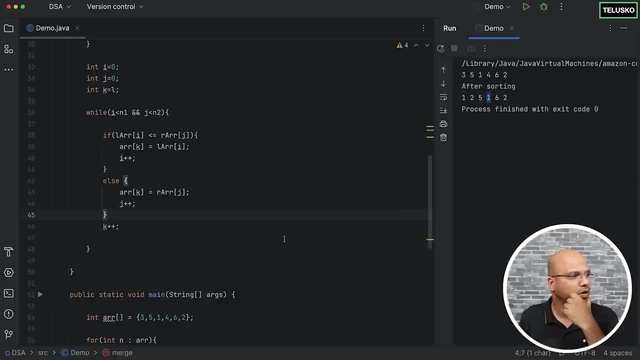 but this four is not at the right place. We got one there Because sometimes what may happen is when you're copying two arrays, what if the values are left in one of the array? Example: if you look at our example when we were copying this: 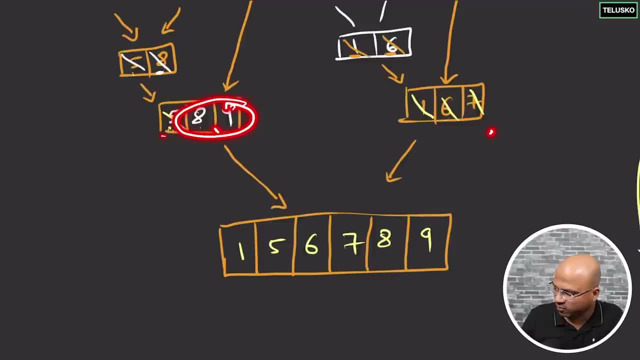 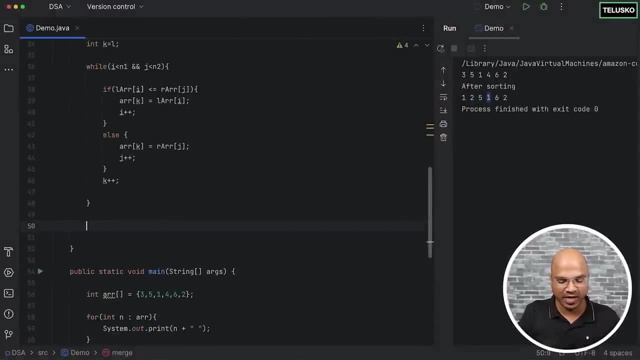 remember, when we were completing the entire task, these two elements were remaining from the first array, Which goes at the end. So that thing is not covered yet. So what you do is for the remaining elements of the particular array. you will again run a while loop here. 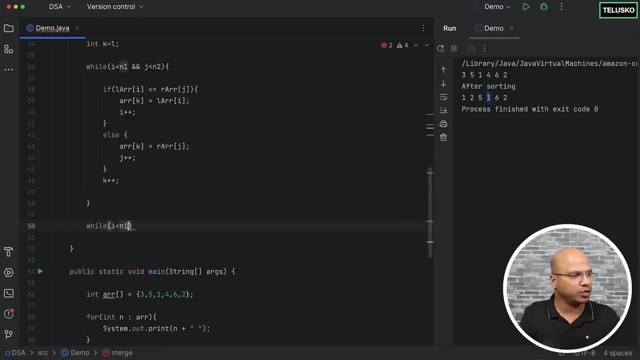 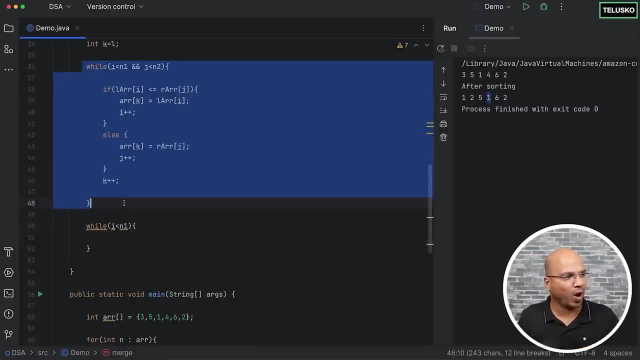 So we'll say: if i is still not less than n1,, you will simply copy the remaining elements, whatever is left, Because after this loop at least one array will be ended. okay, So we have to work for the second. 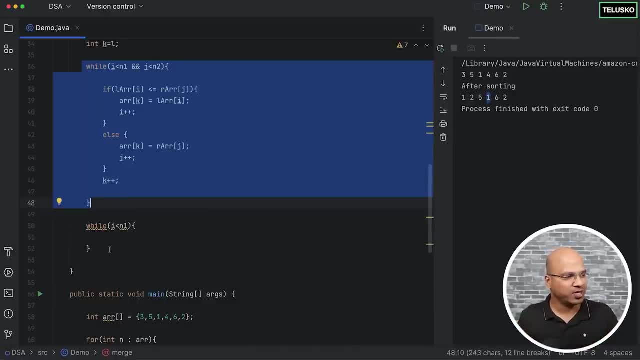 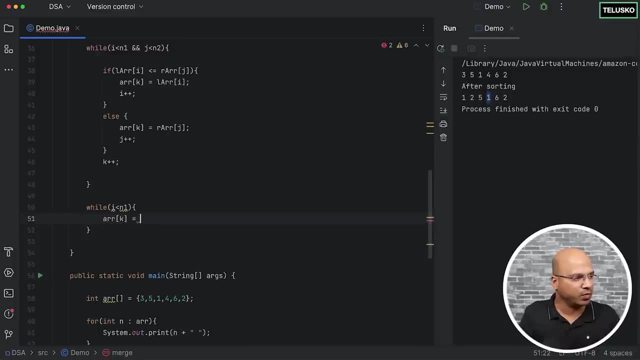 the remaining element of one of the array, maybe left inside or right inside. First we're trying to understand left inside. Let's see what happens on the left inside. Simply copy all the values So you will say arr is equal to. we have to copy from the left array. 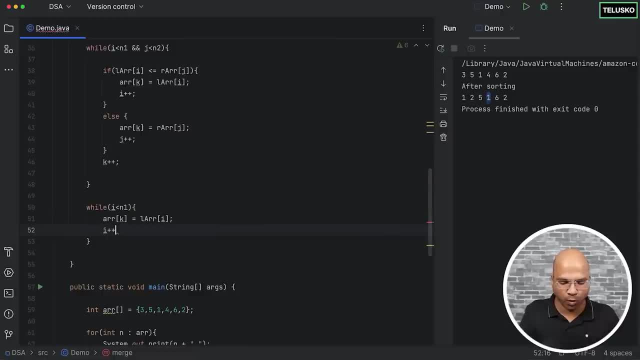 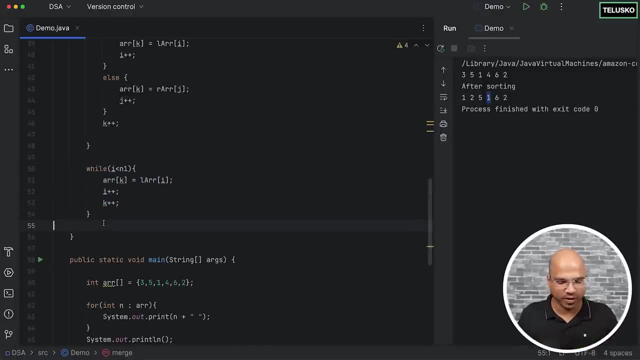 and let's use i here Now. every time you do this, you will increment both the elements i and k both. So this is what the left inside, left out, values. The same thing should be done for the right inside. So this time I will say j is less than n2.. 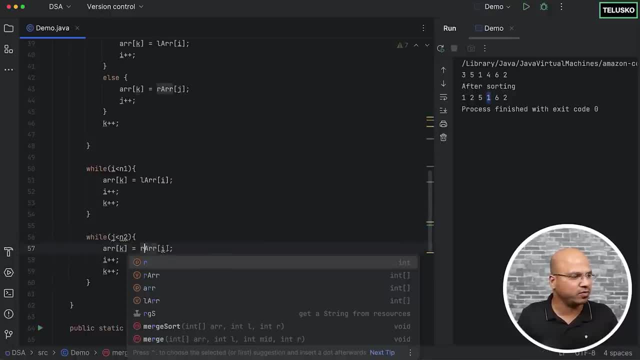 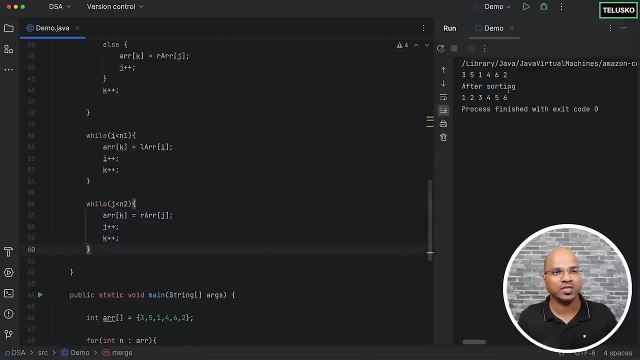 In that case you will copy, but not from the left inside, you will do it from the right inside. The variable is j and the increment you will do for j++. okay, And let's run this and you can see. now it is sorted. 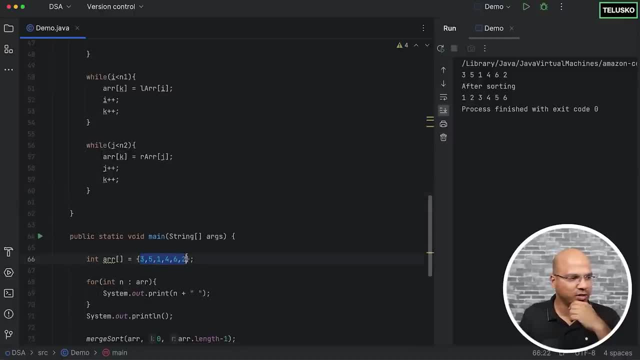 And now it doesn't matter what values you have. Let's say, let's take the values which we have written on the board, which was eight, what was the value? Eight, five, nine, one, six, seven. And if you run this, 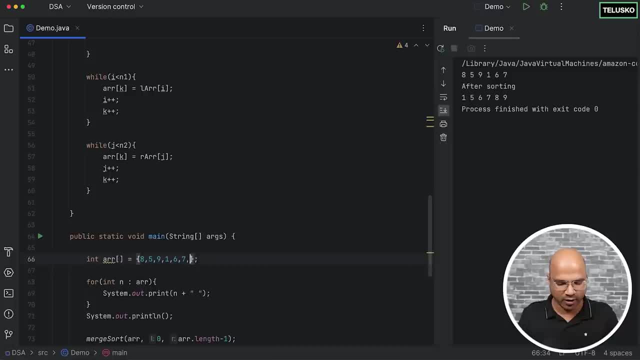 you can see we got sorted values. Let's add some more values here, just to remove the confusion with different values. Let's say one one one. This is 57. And now let's see six, seven, eight, nine, 57,, 75, one one one. 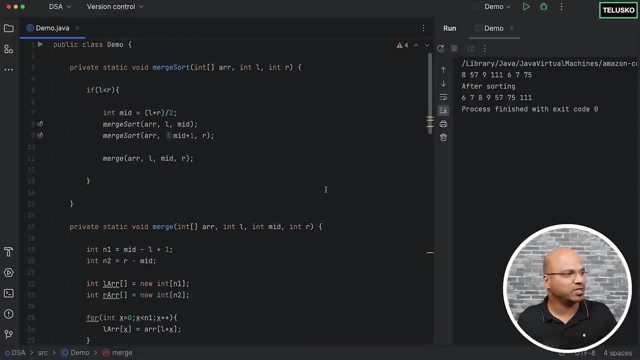 So this is your merge sort. So the steps, basically, you have to first do the breakdown of, you have to break the array down into small chunks and then you have to also merge them. The only thing you have to remember is when we were drawing this. 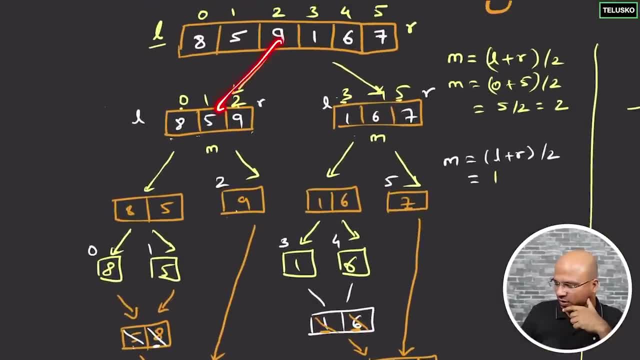 we were going in two sections, right? Something like this: We were saying: okay, we will create two different section and then first section will break into two parts and second section will break into two parts. No, that's not how it is working. 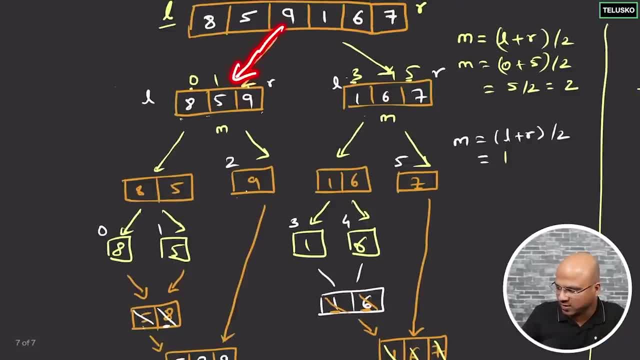 If you observe what it will do is it will break down the entire section into two parts. yes, But then first only you will get the first part. Then you're not going to the second part. okay, You're not looking at here. 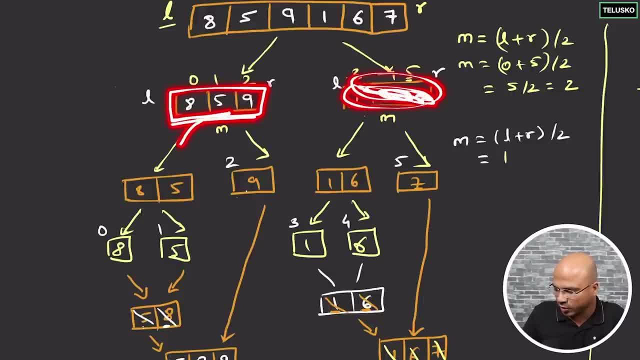 This is not there yet, You're still into the first part. Then this will divide into a section. You will get this eight five. Then you're dividing into two sections, which you will get eight five, And then you will merge them. 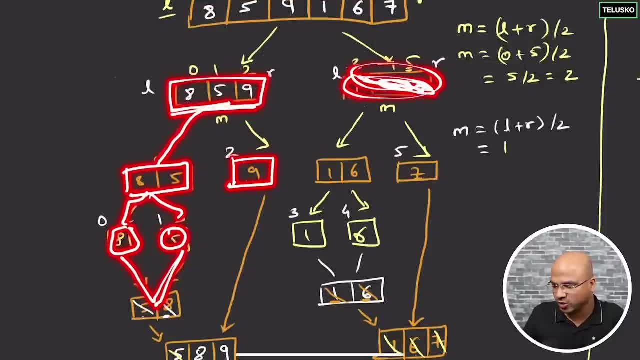 Then you will start breaking down the second part, which is nine. Okay, nine was still not there. Then, once this is also merged, once you get this, it will start working on the next part. Then it will work on this. It will work on this. 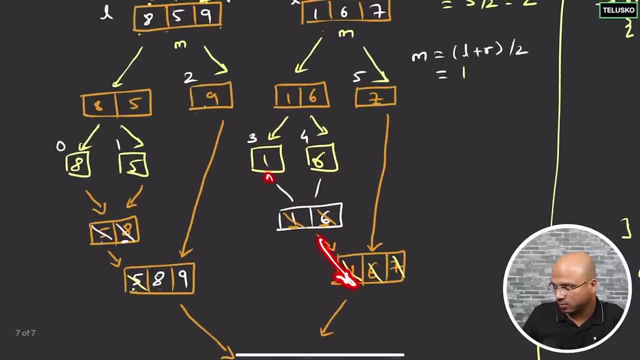 Merge and merge. I mean sorry, Break down, then you get seven, Then you merge this two And then, once you have merged, then it will go for the next two. So it's not exactly breaking down the entire section equally. 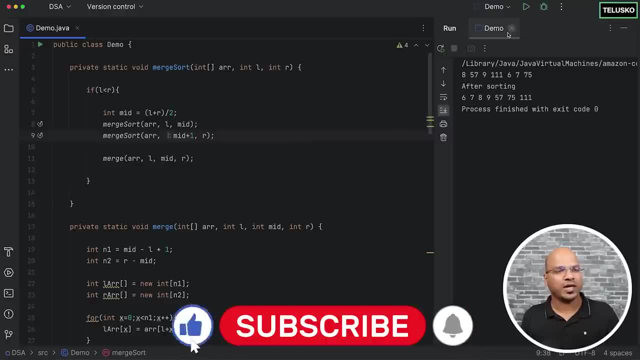 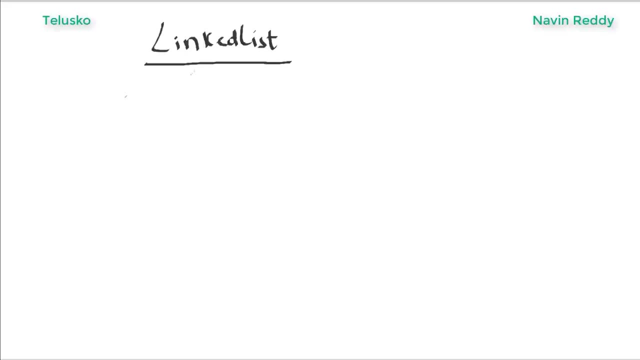 It's basically going from left to right. So yeah, that's how things are working out And this is your merge sort with the help of Java code, And I hope this makes sense. Let me know in the comment section. In this video we'll talk about linked list. 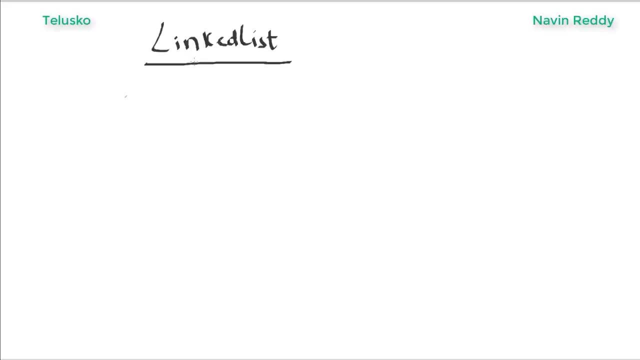 In the last video we have talked about arrays and what are the drawbacks in array? Now, one of the drawbacks which we have seen is, once you define the size of an array, you cannot expand it or you cannot even shrink it. But in case of linked list, we can do that. 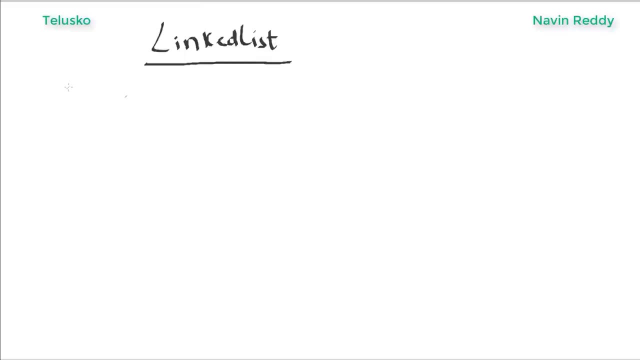 Now, in linked list, what we can do is we can create a collection of elements, and every element will be linked with each other. Okay, so let's make it simple now. So what I will do is: let's take an example here. 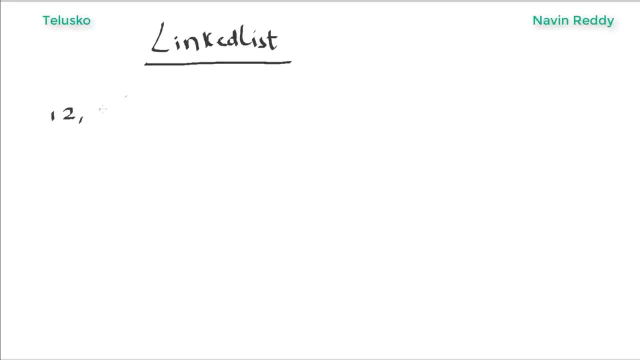 I will take four values. Let's say I want to take values like 12.. The next value is, let's say, six, and then we have eight and then we have three. So I want to store this and then we have four values. 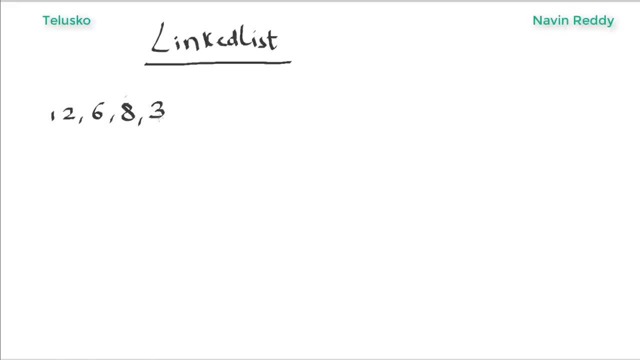 So I want to say 12,, six, eight and three. I want to store it as a collection, not individual, because if you want to work with individual values, you could have created three or four variables and you can assign those values. 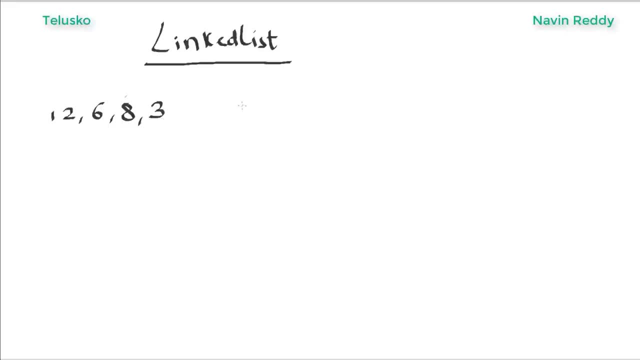 But if you want to keep it as one collection, in normal way we can create an array, but the only problem is you cannot expand it. So in linked list, what we do is we use a concept of a data and a reference. 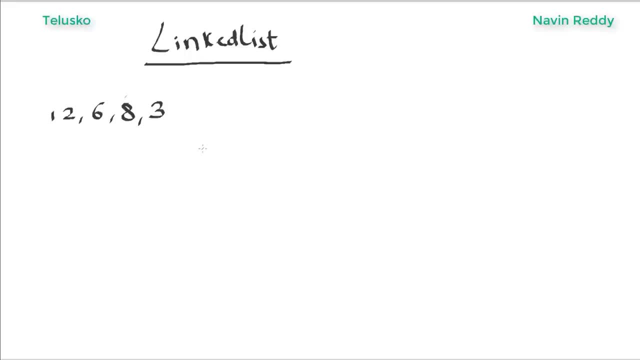 Now what it means. Now, first of all, to store these values. I will not go for any continuous memory. What I will do is I will create this four boxes. So the first box is: will you have a value 12?? 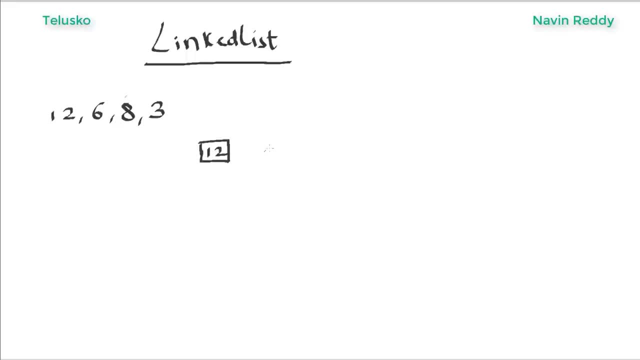 The second box. maybe it's anywhere. So you have a sequential memory right, You can have your data anywhere. But just to make it simple, you know, just to represent in a diagonal format. I'm doing it in the same way. 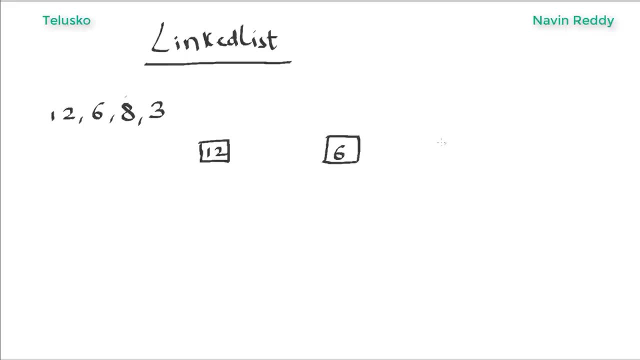 So we have one more value here, which is six, And then let me just draw one more here, which is eight, And the last one, which is three. So we have these four values. We have 12,, six, eight and three. 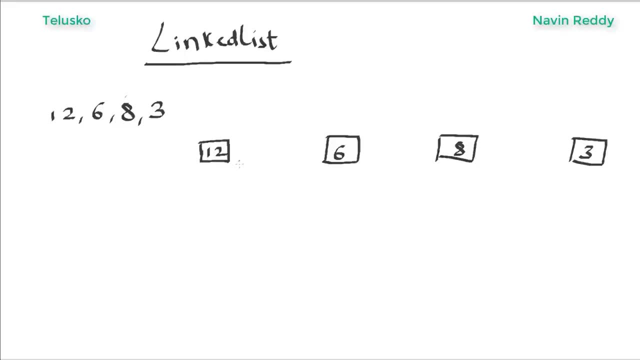 Now what I want to do is I want to say this is a collection, but then it is possible that they are not in a continuous location. There might be some elements in between. So let's say we have 12 here. After that we have some element here, maybe A, B. 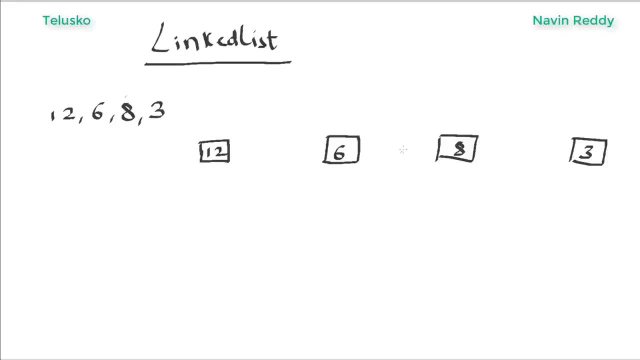 Then you'll be having some more than maybe five to six elements in between, maybe 15, 20 elements in between. So they're not continuous, right? So when I say I have these elements, they're not in sequence. Example: if I want to say 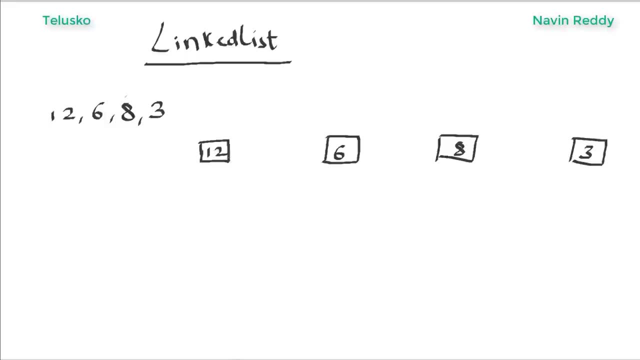 hey, I want to fetch the third value. how can you mention third value? Because you don't have it in sequence. If you want to make them in sequence, what you have to do is, first of all, you have to make the first element as a head. 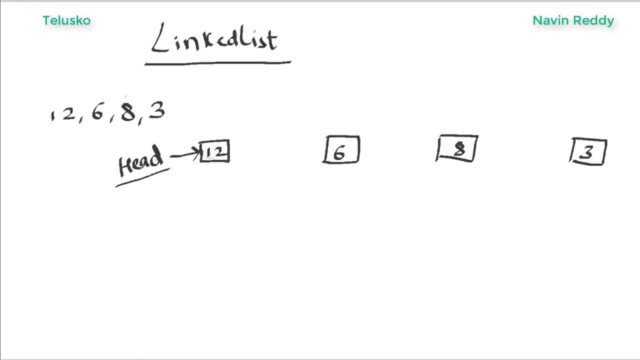 So you have to make this as a head. So once you have made this head, that means this is the first element. So that is simple. But how about the second element? How do you link the first one and the second one Now to make it work? 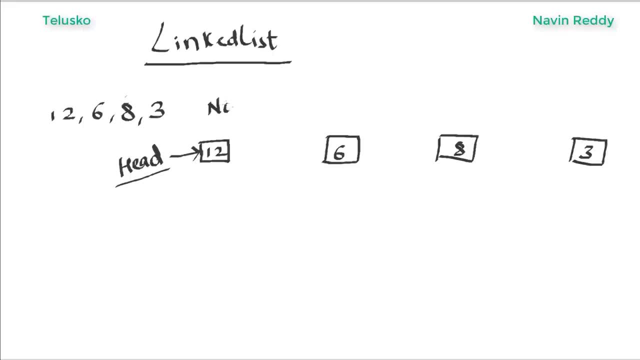 we will call each element here as nodes. So the elements which we are using here are nodes. So this is a node, this is also a node, The eight is also a node, and three is also a node. So all these are elements. 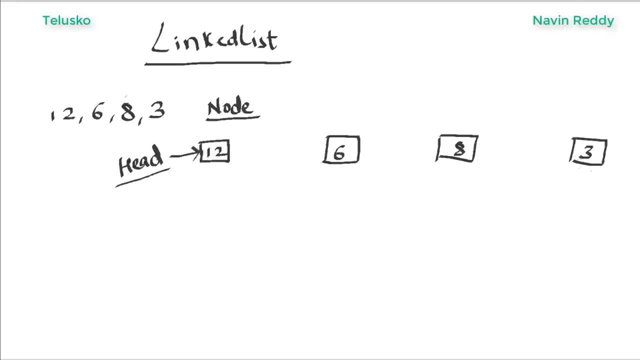 So node value is 12, node value is six, node value is eight and node value is three, Or you can call them as value, you can call them as info. Now how do you link this 12 and six? The way you link is by creating one more memory here. 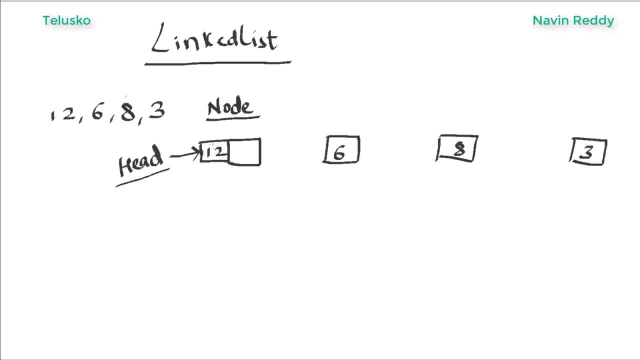 or one more box. Now this node will have two things. The first one is the info, So this 12 here is the info, and the next one will be the address of the next node. Now every node will have an address, of course, right. 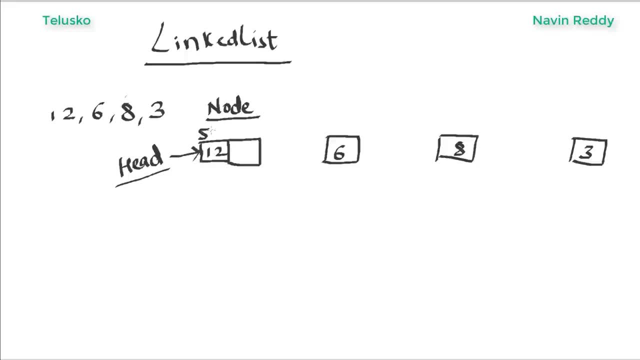 So let's say, the address for this node is 12,. that's the address for this node. The address for this node is, let's say, 326.. The address for this node is, let's say, 101.. And the address for this node is, let's say, 202.. 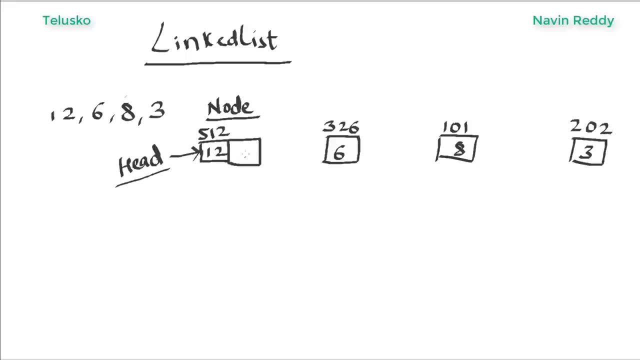 So we have all this address here Now in this box. this will have the address of the next node. So in our example, six is our next node, right? If you want to have eight as a next node, you can write the address of eight here. 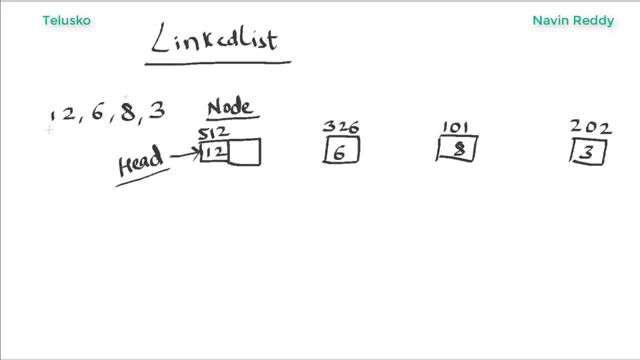 But in this case six is our next node. as you can see the sequence here. I want to maintain the sequence. You can say 326.. So this is the address of the next node. That means we have a line between this. 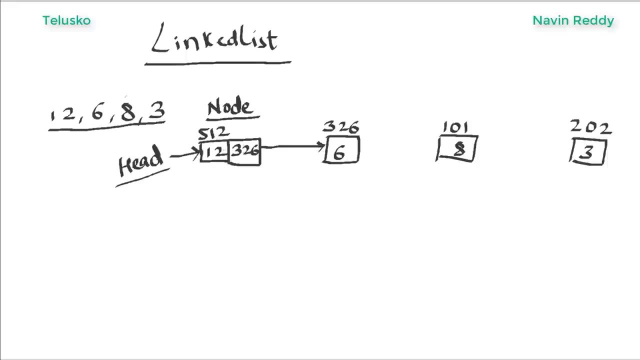 So we have a line between the first node and the second node. So there's node one, there's node two, node three and node four. Now, as you guessed it right, in six you'll be having the address of eight, which is 101, so this is 101 here. 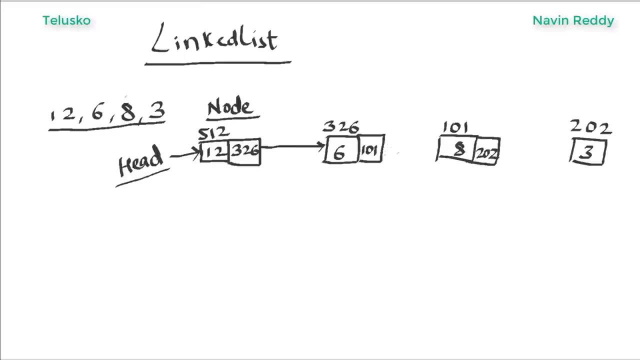 And this one will have 202.. So we have a reference, so this is a link, and even this is a link, And that's quite simple, right. But the problem is, what about the last element? Now, of course, we don't have any element after that. 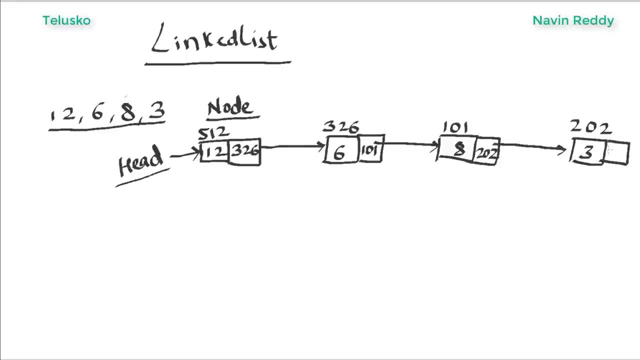 Even there we'll be having an address, but then address of what? So it will be null. Now, since we don't have anything after that, it is null. So we have the first node here, which is 12.. This is the first node. second node, third node: 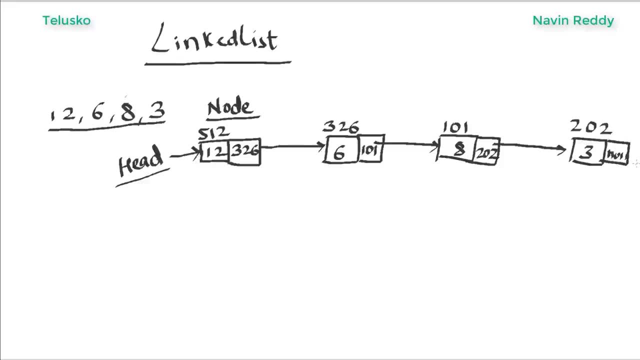 and fourth node, and fourth node will be null, because we don't have anything after that. This is how you create a linked list. So we have a list of values and they all are linked- And that's why they say linked, because they all are linked- and a list. 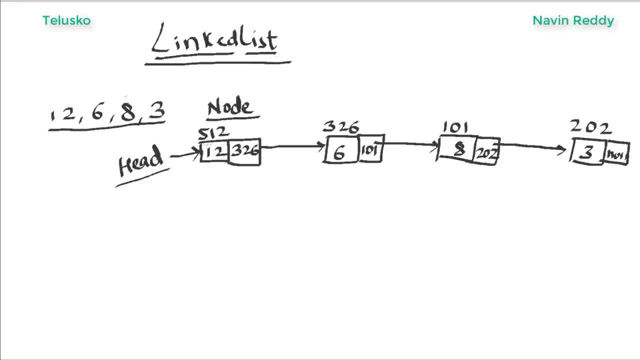 because they are linked. It's a list. So once we have all these values assigned, this is a list. Now, if you remember, in the start of the session we said this is expandable. So when I say it is expandable, 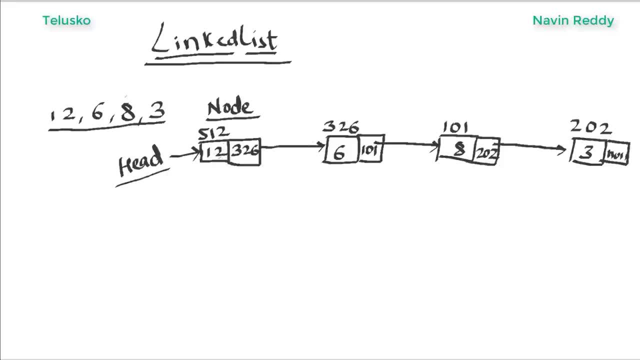 how do I start the first one? I mean, how do I add the element anywhere? So maybe I will start by adding the element at the end. Maybe I want to add the element here after three. So let's say in the list we have one more value here. 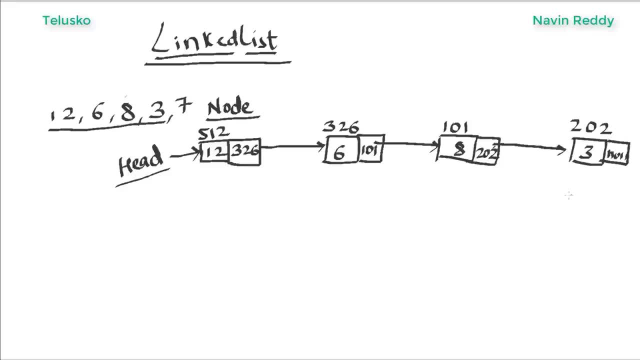 let's say seven, And how do we add seven at the end here? So what you can do is this very simple step: just create a node here, Whatever node you want, And then the value for this node will be seven. So this is the value, right? 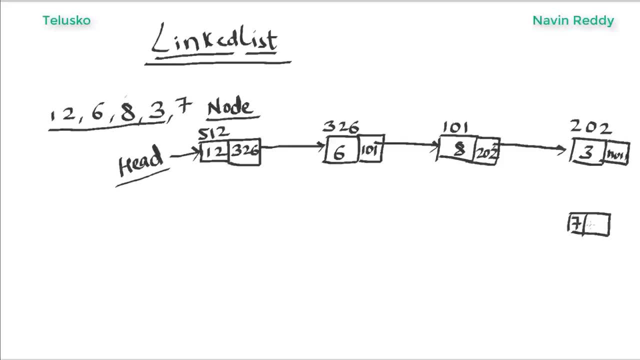 What about the address? Now, as this is the last one, you can simply put here null. So you can say this is null because this is the last one, But then we have mentioned three as null. right, But then now, three is not the last element. 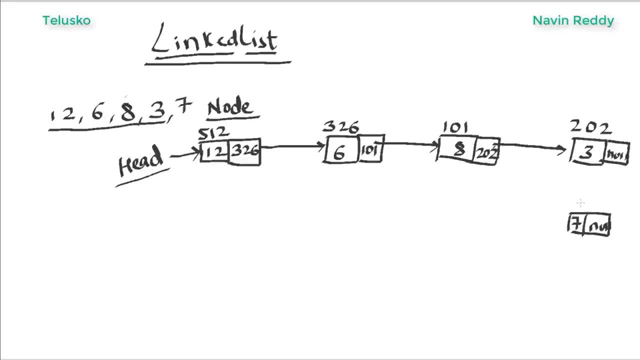 The last element is seven. So after three also we have seven And the seven will also have an address. Let's say the address for this one is one, two, six. This is the address. We want to link this You have to mention. after three we have seven. 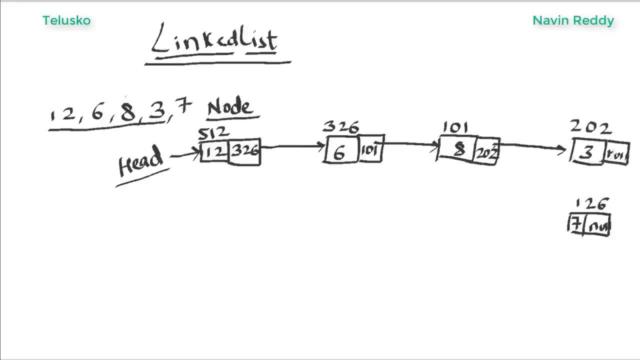 So what you will do is you have to change this value. So now you cannot have null here. Now you have to make it one, two, six. After three we have seven, right, So you have to mention the address here. 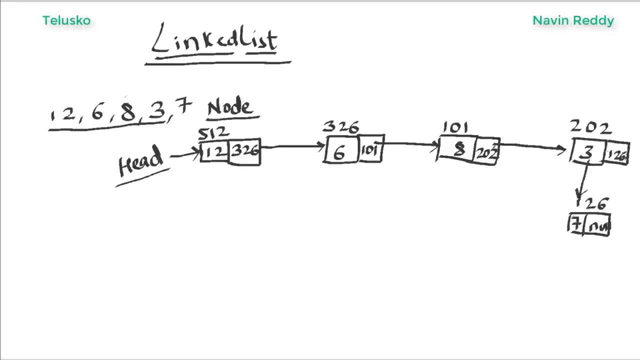 And then we can give an arrow. So this is the seven, is the last element here. After three we have seven. That's how you can simply add the value. It's that simple. Can we add the value at the start? 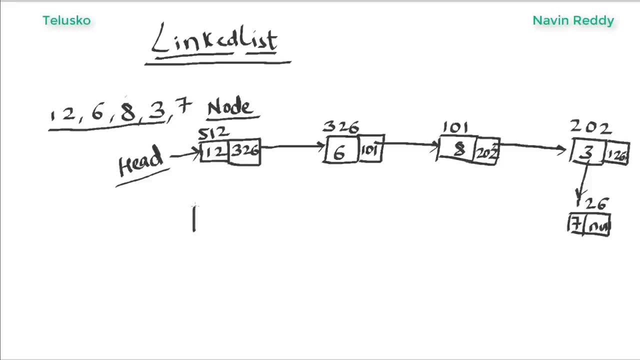 Yeah, it's quite possible. The only thing you have to do is again create a node. So we've got a next node, We've got a next node here, And let's say the value for so after before 12 as well. 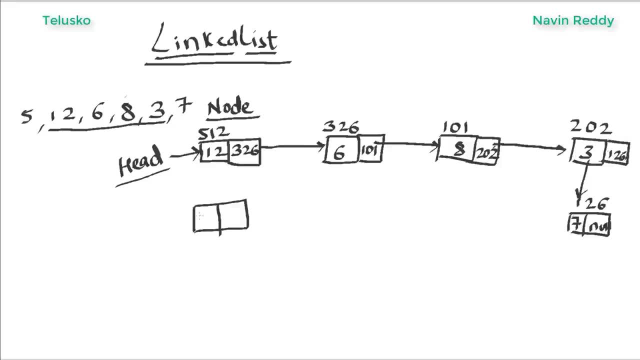 I want to assign a value like five. I want to have a value five here. So what you can do is you can make the value five here, And how do I refer? So now? there is one more change: You cannot refer the 12 as the head element now. 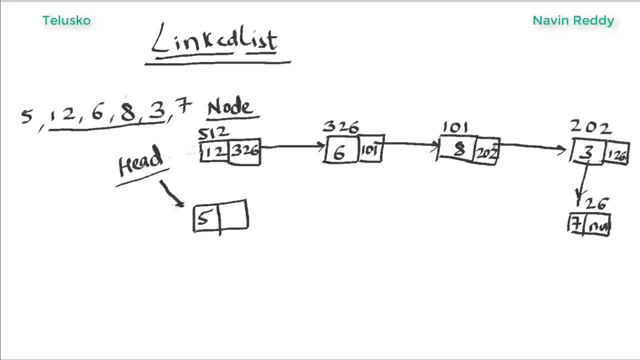 So 12 is no more the head element. Now the head element is five And of course this will have an address. So let's say five is at address three zero six. That's the address. Now, what you will do is: 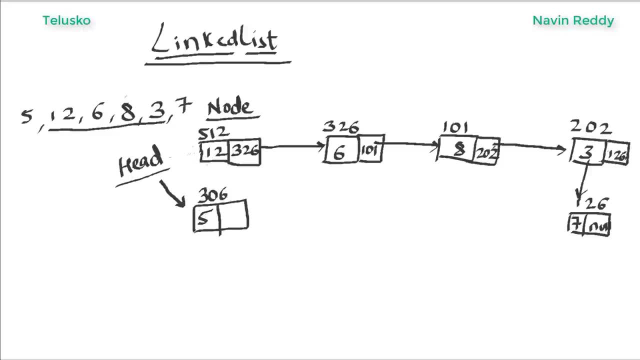 in five after five, the element is 12, right, So we have to mention the address of 12 here, which is five one, two. So five one. So after five we have 12.. So that means we have an arrow. 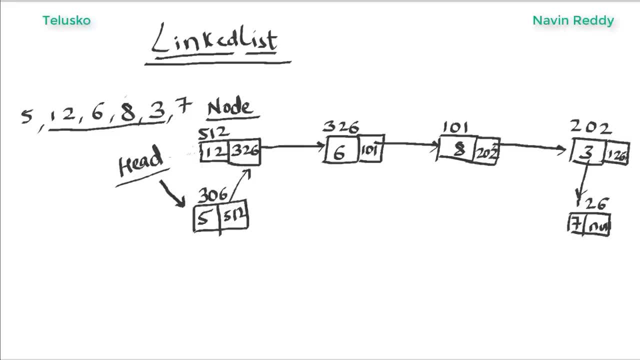 So five is the first element now, because that is head, And then after that we have 12.. After that we have six, After that we have eight. So that's how we can add the value at the start. Now can we add the value somewhere in the middle? 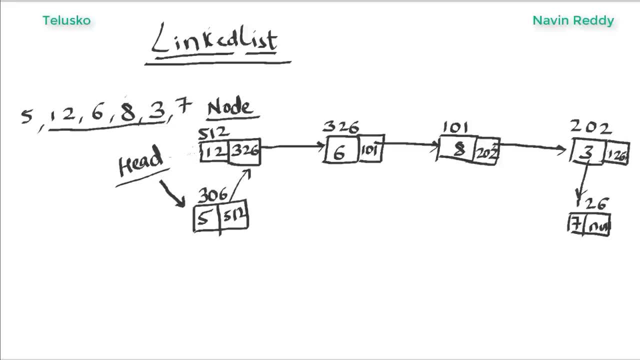 And the answer is yes, it's quite possible. What you can do is you can create one more box. What you can do is you can create one more box. You can create one more box here. Did you make a box, And that box will have a value. 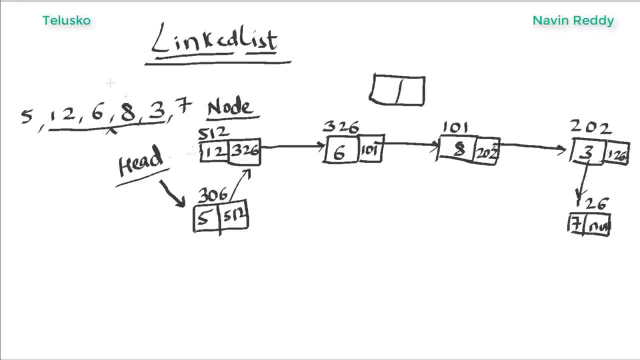 So what I want to add? so between six and eight, I want to add, let's say, nine, So I want to add nine between six and eight, So you can create a nine, You can have a nine value here, And then it will have its own address. 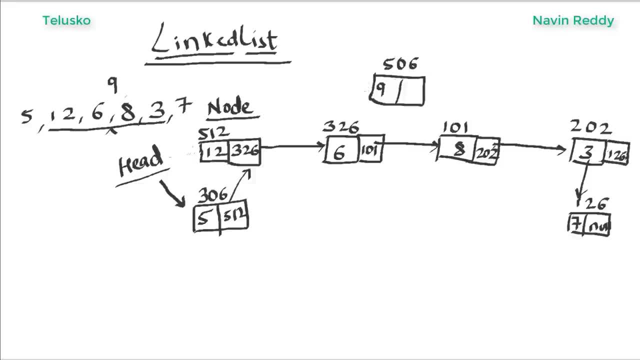 let's say five zero six. I hope that address will not go there, So we have five zero six here. I know if you can observe I'm giving random values or random addresses, because all these values will be stored somewhere else. 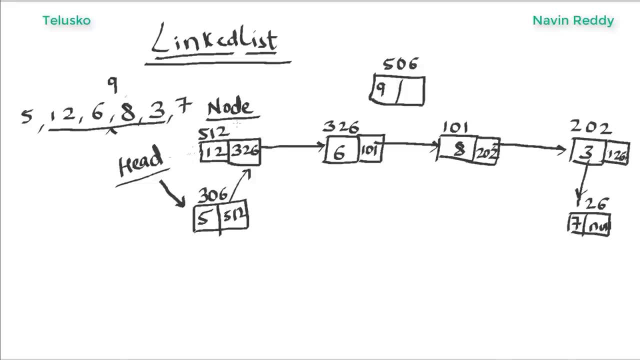 you don't even know right, They're not in sequence. I mean, you will know by the address, but then they're not in sequence. So if you don't have these links, you cannot fetch them in sequence. Okay, so now in nine. 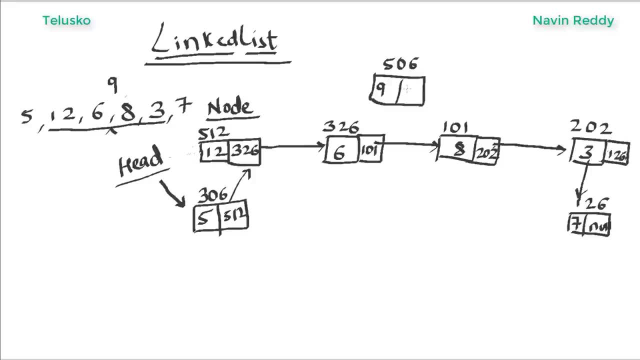 so we have to mention: nine comes before eight, So nine will have an address of eight, which is one zero one. So now nine is linking to eight. That means we have to remove- I mean, we have to of course remove- this link. 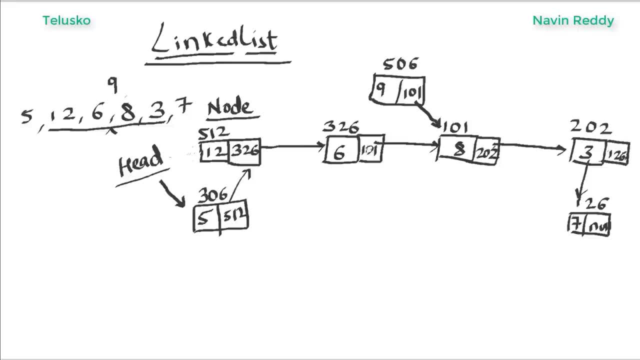 But then if you remove this link, what should I put here? So six, so inside six will be not. so the address will not be of eight now, it will be of nine. So we have to say five zero six. 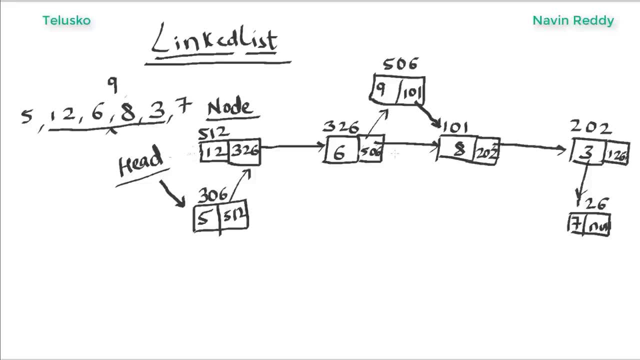 And we have to give an arrow. So of course we are not using this arrow anymore. So after six, we have nine, after nine we have eight. So that's how you can add values in between. So it's that comfortable. 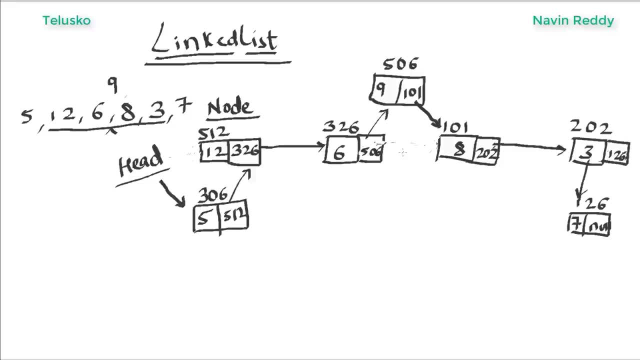 because we are not consuming data in a continuous location, So we can create as many nodes as possible. provided you have enough memory in your system, It will create a number of nodes and all these nodes will be connected with a link list. Now, this type of link list which we have created here, 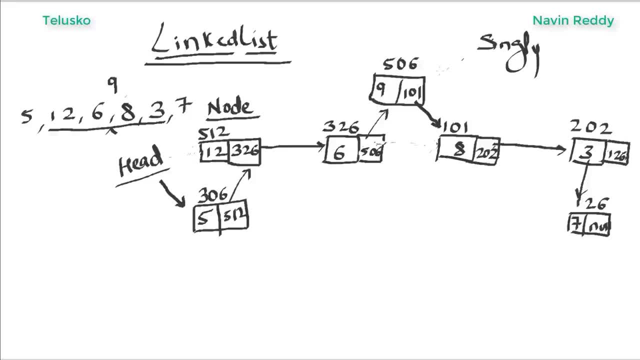 is called as a singly link list because it is single link list. That means we also have a doubly link list or double link list. Yes, we also have a double link list. We'll see that in one of the videos in future. 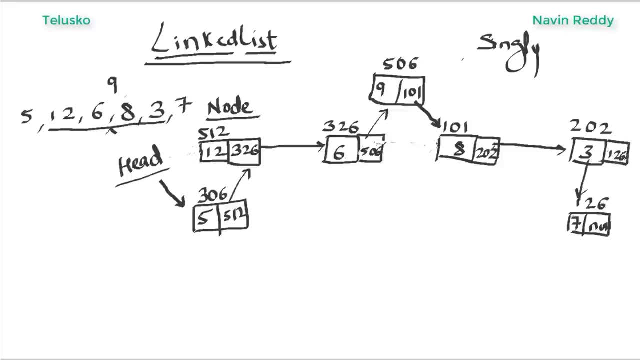 But now this is a single link list, So this is better than arrays, right? So before we have talked about arrays and now we are talking about link list. So now you tell me which is better: Is it array or link list? 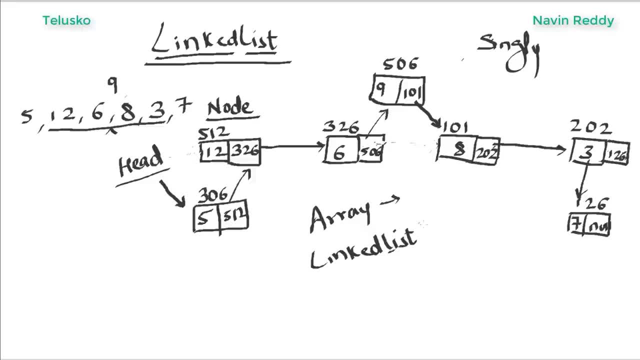 Now, of course, both have their advantage and drawback, But what is the advantage? So the advantage of using link list is it is expandable. You can increase the size of the links. you can reduce the size of the list, right? 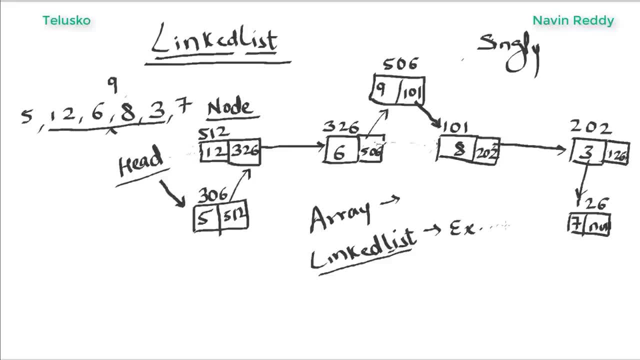 So you can say: the advantage here is expandable. But the problem in link list is it is slow. So when I say drawbacks, it is slow when you compare with array, Because in array it works with index numbers Now, since everything is stored in a sequence. 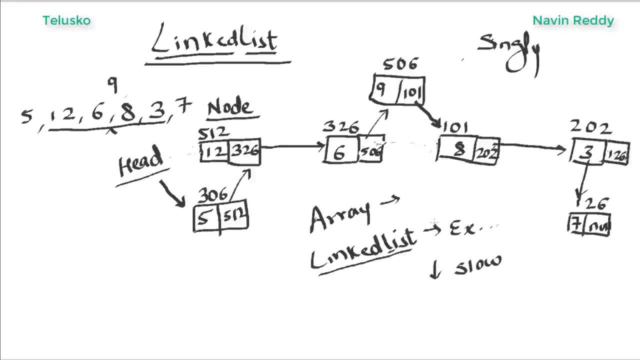 it works with index numbers. you can fetch the value randomly. So the benefit of array is you can fetch the value randomly. Right, so that's the positivity of it. So let's say this is arrow positive value And the so link list drawback is it's slow. 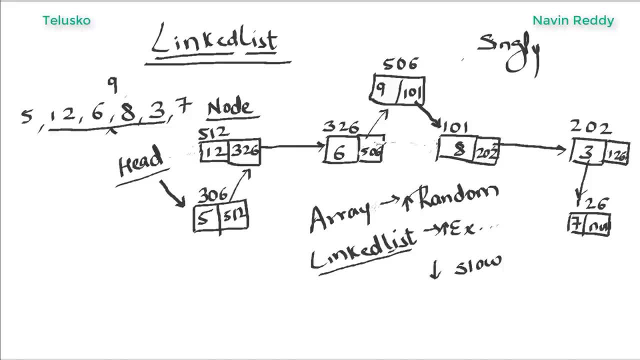 We have to also mention the drawback of array right. In fact we have talked about in the previous video: it's not expandable. So, yes, link list is slow because if you want to fetch a particular value, let's say if you want to fetch eight. 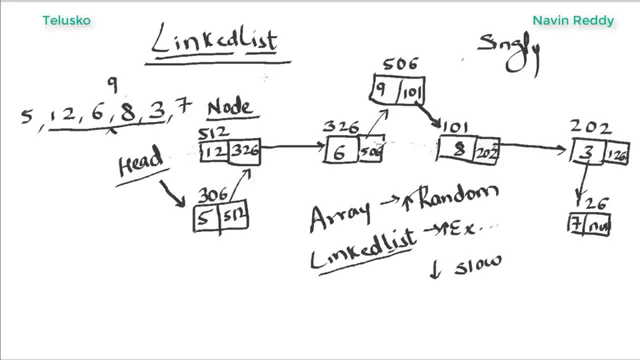 you cannot directly go to eight. You have to go from five. so first you have to go to five, then you can. so you can go. first you have to go to five, then you have to go to 12.. So you have to follow that sequence. 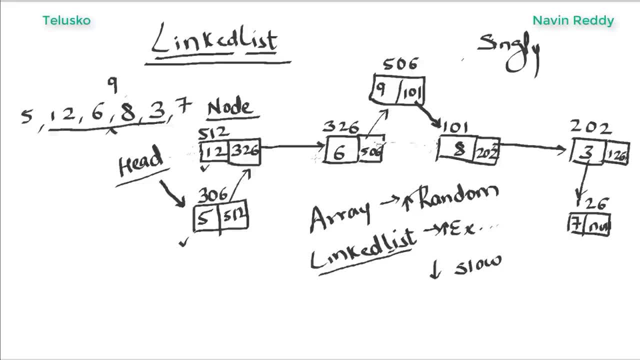 And then you can reach to eight. In fact, we also have a concept of big O notation. Again, we have not discussed that yet. So we'll say big O notation would be big O N. So if you want to search for the value, 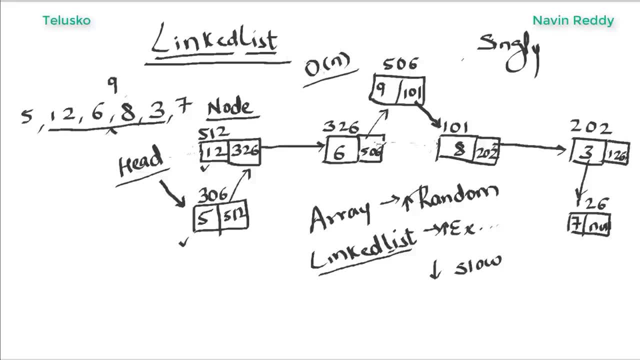 you have to say big O N Again. we'll talk about it later. Remember that link list for search. it uses big O N, So it is time consuming compared to N, So you can add it in terms of searching. But if you want to fetch, if you want to insert value, 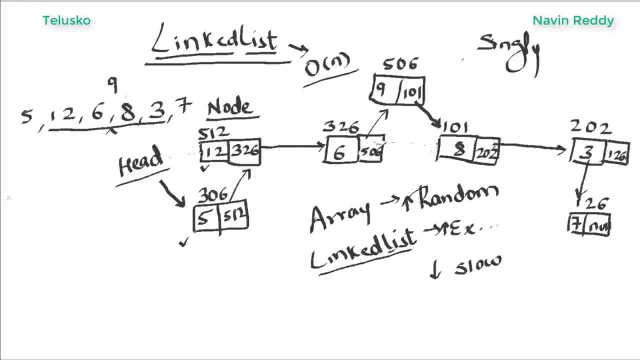 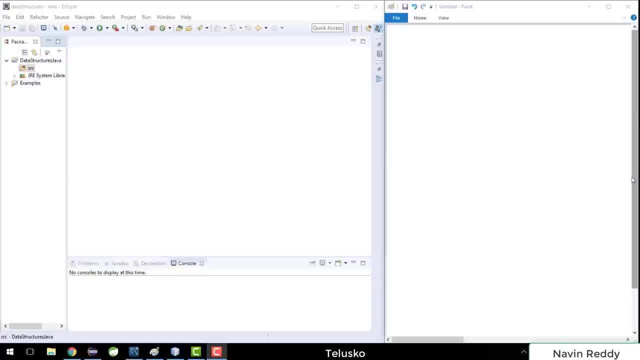 in between. link list is the best one. Now. this can be implemented using any language which you like. You can implement this with C, You can implement that with C++, You can implement it with Java or maybe Python. In this video, we'll see the implementation of link list. 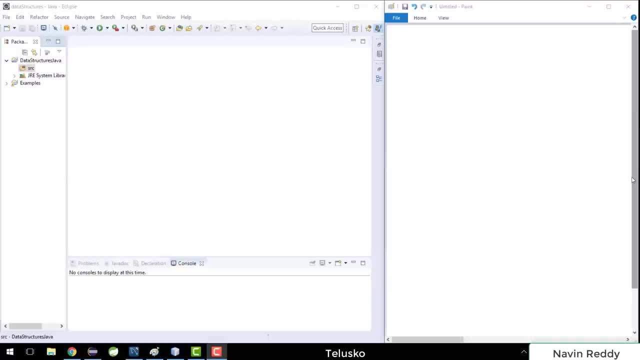 In the earlier videos we have talked about why do we need link list and what is link list? So let's try to implement that with the help of Java language. Again, you can implement that concept with any language which you love. In this video, we'll focus on Java. 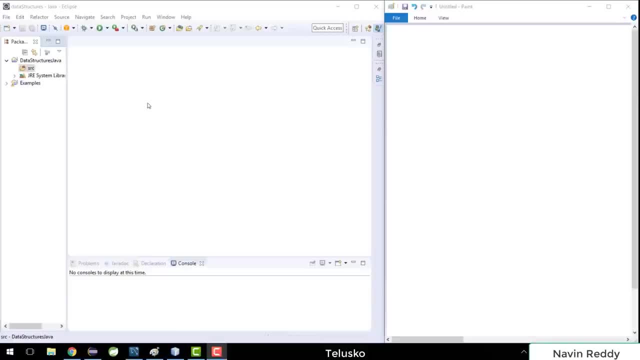 We have two sections on this screen. We have on the left-hand side, we have Eclipse IDE. You can use any IDE which you prefer. You can use IntelliJ, You can use NetBeans. I will be using Eclipse here. On the right-hand side, I have a paint. 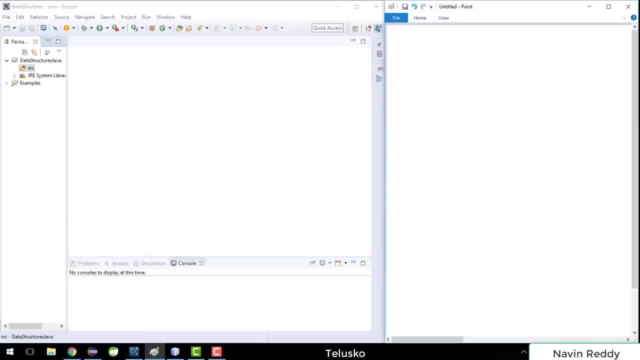 So that if I want to show you anything, any diagram or representation of that, whatever we are doing, you can see on the right-hand side, So what exactly we need. So just to make a quick recap, what we have learned till now is: 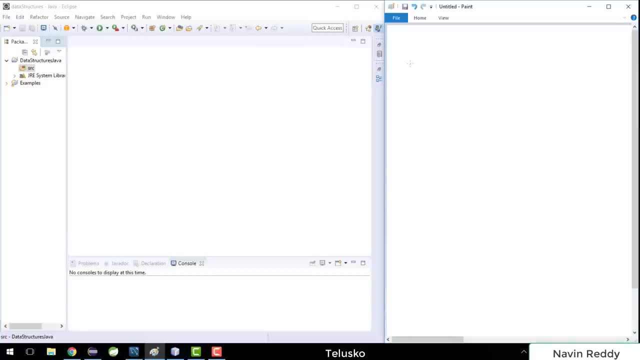 when you talk about link list, we have representation like this. We have node. Now these are our nodes, right? So let's create a first node here. So this is our first node. And let's say: I want to store values like five. 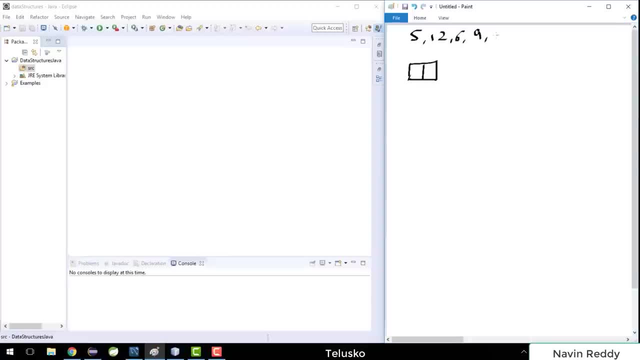 12,, six, nine- I don't know why I love these numbers- And let's say we have eight. So I want to store these five values. That's it. nothing fancy, just five values and a link list. So in link list, what we do is we create individual nodes. 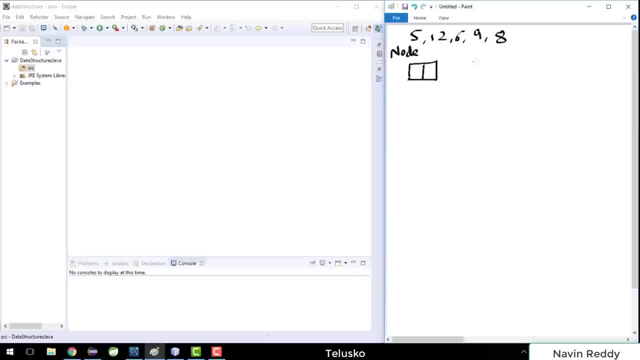 So all these things are called as nodes, right? So this is a node, and then we'll create another node, So this node will have a value which is five, And then we'll be having another node here which is, let's say, value 12.. 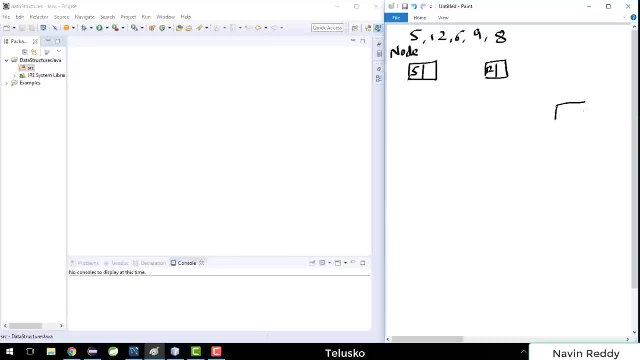 And this node will have some address And we'll be having one more node here. let's say six, So this is six. We have one more node here, which is nine. Again, I'm doing it purposefully, creating the objects anywhere. 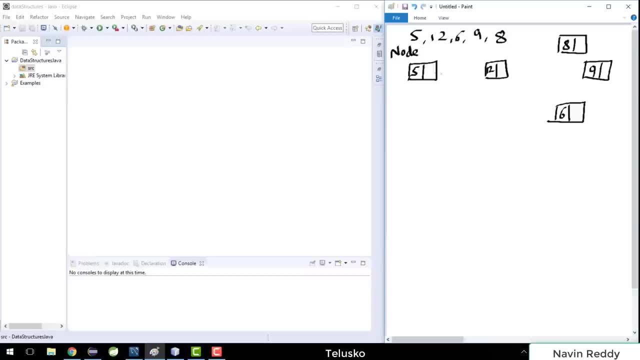 And then let's say we have eight here, So we have all these nodes here. So this node, which is a five, will be linked with 12. We have to find a way to link these two nodes. And then we have to find a way to link these two nodes. 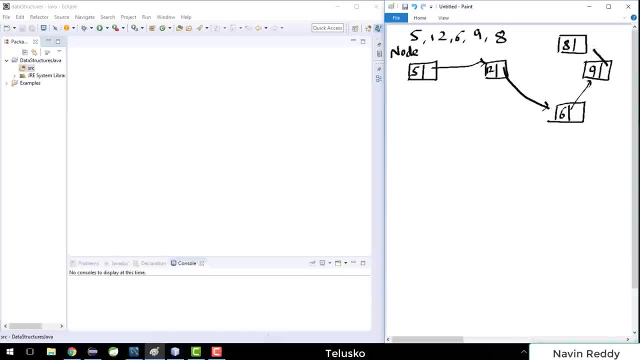 And then and this node and this node. This is what we are going to do. So once we can link this node in future, if you want to add some new elements, you can do that very easily. Every node will have two things. 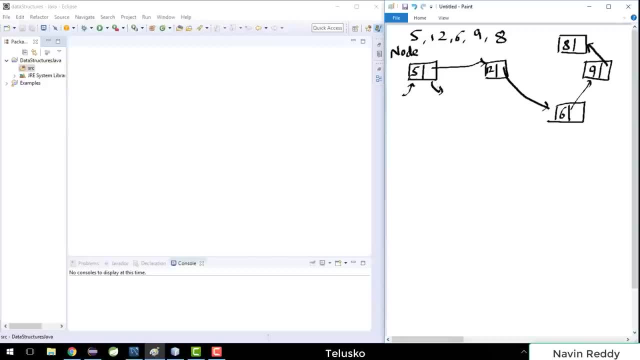 A value. so this is your value And this is your address. Now, this is an address of the next node. Now, in C programming we can use pointers, But in Java what we do is we create a reference of the next object. Java is all about objects, right. 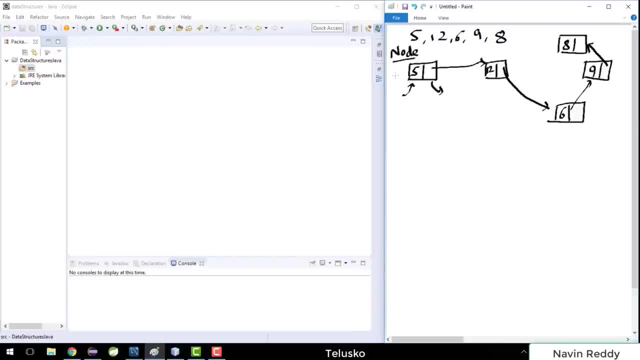 So of course this node is also object. So this is the first object. So you can say: this is the first object, This is the second object. So the first object will have a reference of the second object. The second object will have a reference. 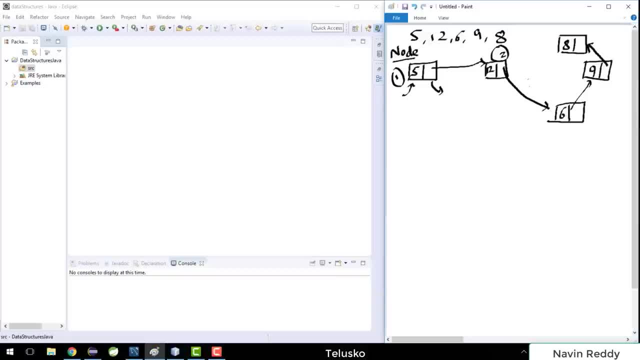 of the third object. Now again, we don't number them, But then every object will have a reference of some other object. The last object here will have nothing, It will have null right. So we don't have any other object after that. 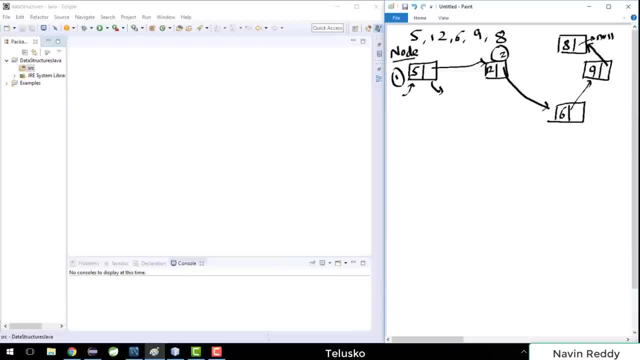 So we'll be having null. Maybe after some time we'll add one more node. The reference of that node will be assigned here. So let's try to implement this. So what are things we need here? So let's see what are things we need in Java perspective. 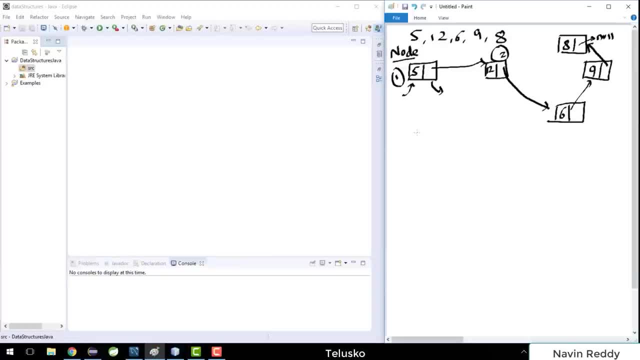 So of course, we need to create objects right. So before creating the object, we need to use a class. So the first class we need is a node class. A node class will have two things: A node class will have a data and a node class will have the next node. 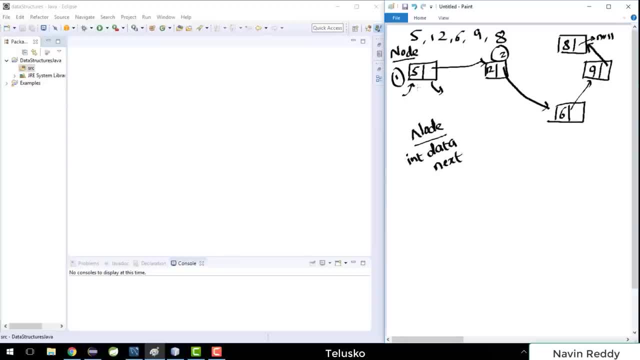 So data will be of type int. Again, you can have any data you want, You can have a string data, You can have any object, Maybe alien object, maybe accounts object, maybe a laptop object, your wish. And then the next node will be of type node itself. 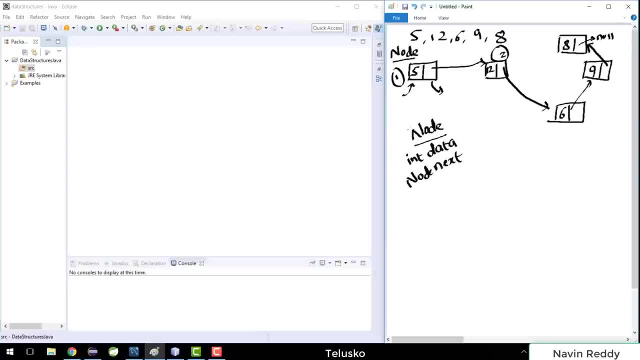 Because this will refer to the next node, A node class. so this is a class which has two things: We have a data and a node. Then what other class we need? We need a linked list class, right? Because linked list class will have certain features. 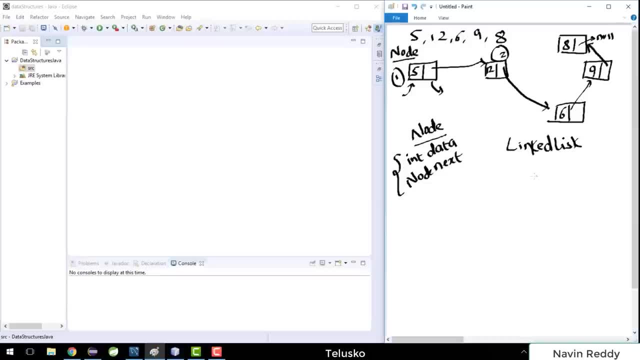 because when you talk about linked list, it has certain methods. Example: we are going to look at insert, So we look at insert. Now, insert will add data at the end. So let's say, if I specify data as five, it will add that at the end of the list. 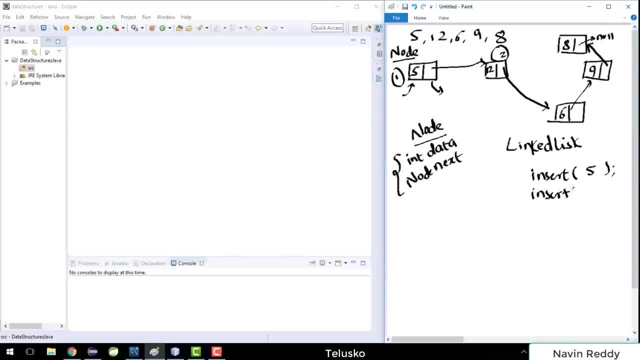 What if you want to add in between? So you will say insert and you will say insert at I want to specify the position, Let's say I want to specify position three, and or the index, the value three and the value is, let's say, 12.. 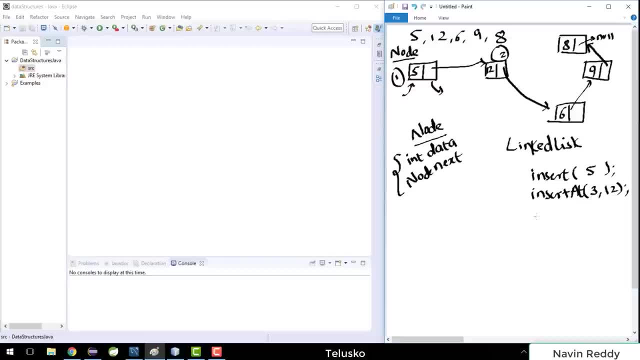 So I want to add 12 at the location three. Maybe I want to add element at the end, So I will say insert. or maybe at the start We are already done with the end, right? So we'll say insert, start. So I want to insert at start. 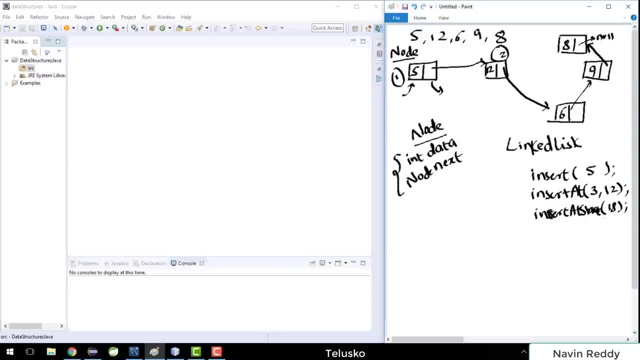 So you can say I want to insert the start, which is 18.. So it will add at the start. So this will add at the end, This will add in between and this will at the start. You maybe want to delete the data as well. 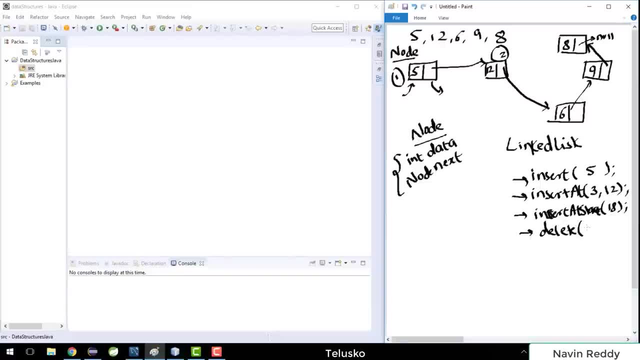 So you can also use a delete method And delete. you have to specify the index. Let's specify the index as two, So it will delete the element at index value two. These are the options I want to perform in my class And then to run this, of course. 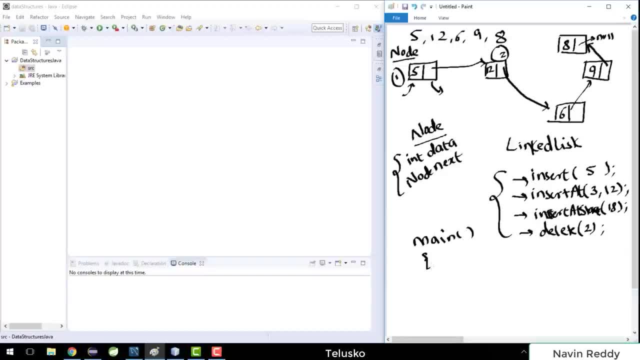 we need a class which has a main method. So we'll have a main method in which you will be doing all these operations. So you'll be having main and then a main will have all the execution. It will have a linked list. object. 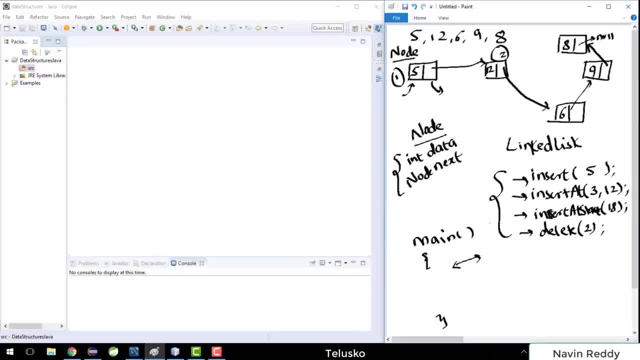 And then, using that linked list object, we can perform all these operations. And then, oh, we also want a show method, right? So show method will display all the elements. So if you want to display all the elements, you can do that. 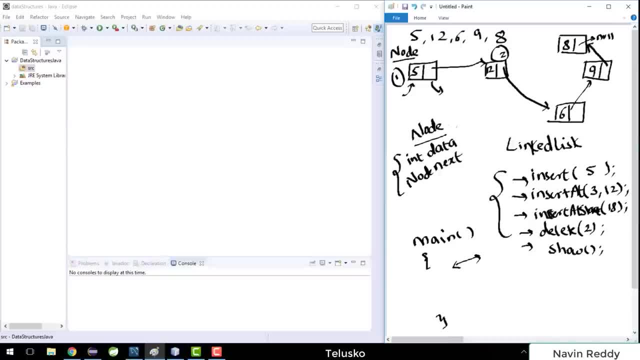 So this is what you'll be doing here. So in total, we need three classes here. So this is the first class we want to work with, the second class we want to work with and the third class. So let's create these three classes in our Java code. 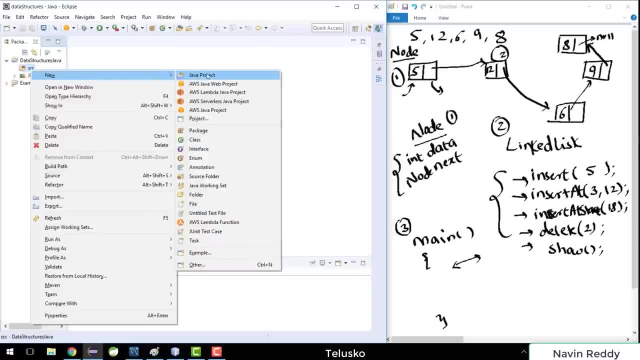 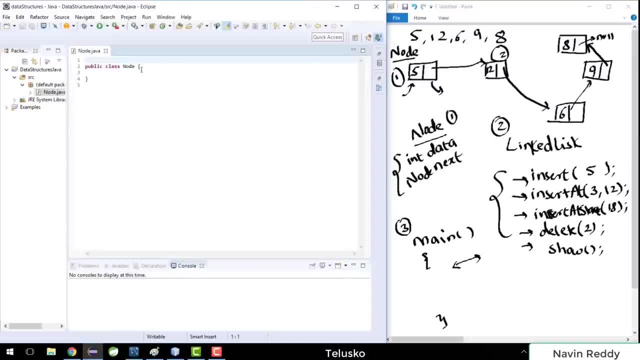 So let's do that. So I will say: right click and let me create a Java class here. I will say this class name as node, because the first thing which we are going to do is node. Now this node will have two things, as we have discussed. 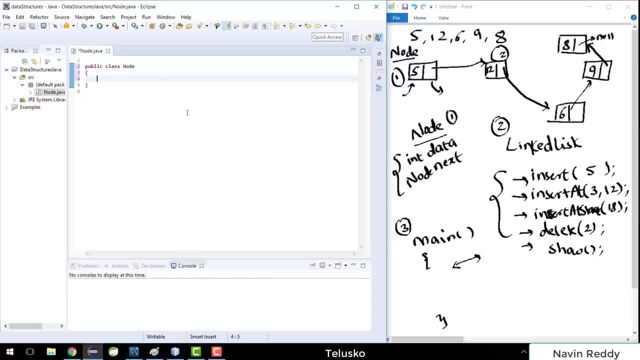 The first thing it will have is the index value. Font is not visible. Let me just do that. So now I would say, this node will have the first thing, which is the int data And, as I mentioned, you can use any data you want. 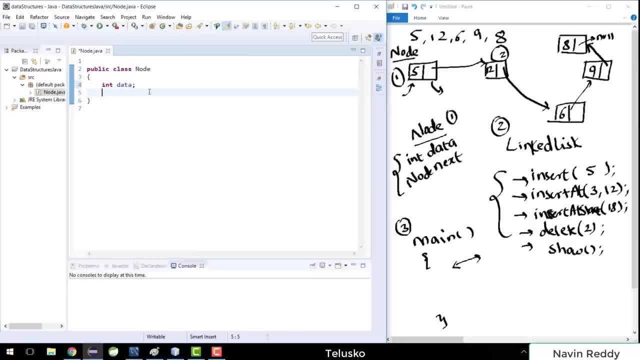 You can go for int, float, double, alien type, any complex type if you want. And the next thing is the node itself, so the node object which is next. So this node is a reference. So this next is a reference for the next node. 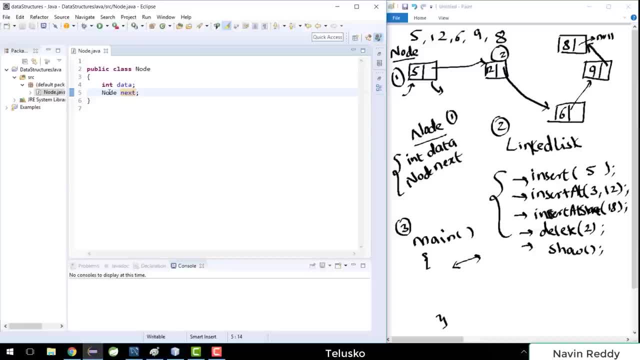 Quite simple, right. So we have public class node and we have just two things. Nothing fancy here, We've got just two things. You can make it more simple, You can make it more efficient, You can make it display with private variables. 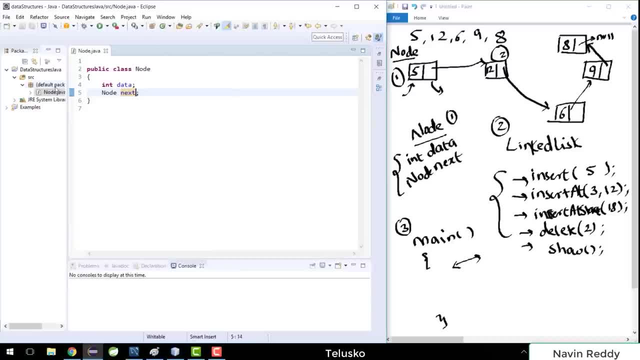 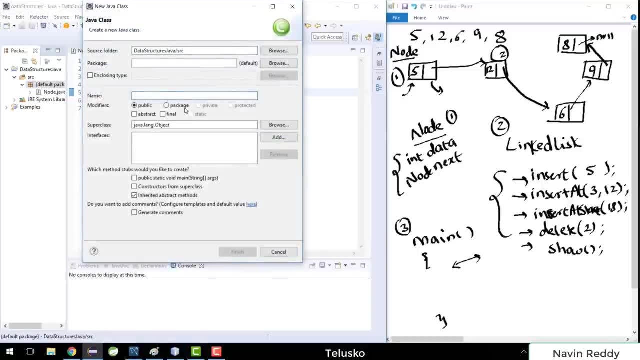 and you can use getters and getters, But then, just to keep it simple, I'm doing this code. The next thing we need is a class which is called as link list. But what if? okay, let's get a main class first. 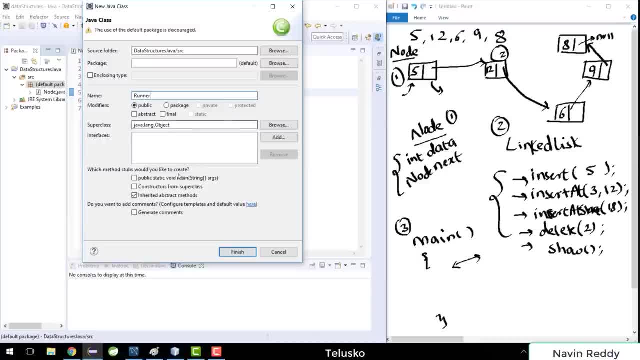 I will say the main class, and the main class name will be runner. Again, you can have any name, It doesn't matter. We have runner class, which has a main method. Now, what if? or maybe? I don't want to create my own list. 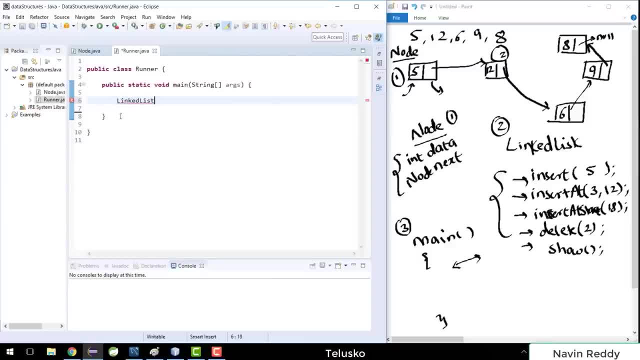 I want to use the inbuilt feature. So in fact in Collection API you do have a link list as a class. So you can say link list. I will say list equal to new link list. In fact you can use the internal one as well. 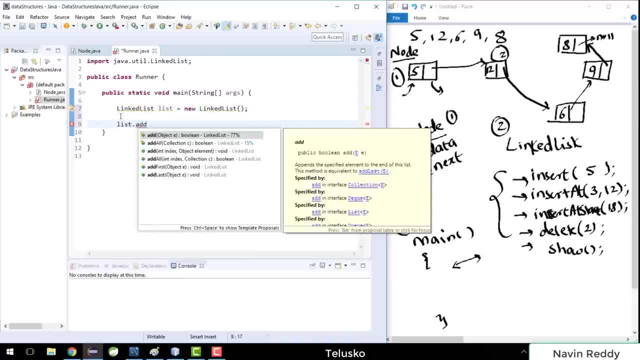 You can simply use this class and you can say list dot. We have an add method. So using add, you can specify which object you want to add. Maybe I want to say I want to add five. So this is same as the thing which we are going to do. 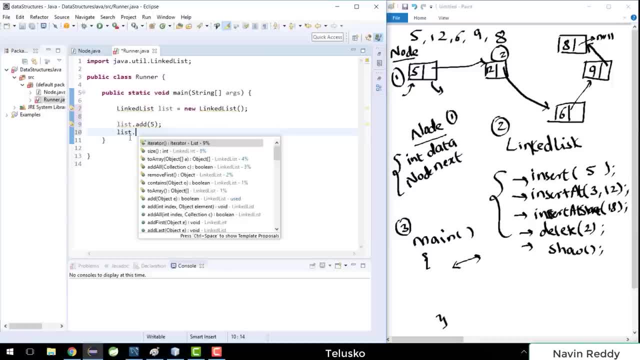 We are going to use insert, yeah, And then we'll be having list dot add. You can specify the index value where you want to add. Let's say, I want to add index at four. add the element as, let's say, 12.. 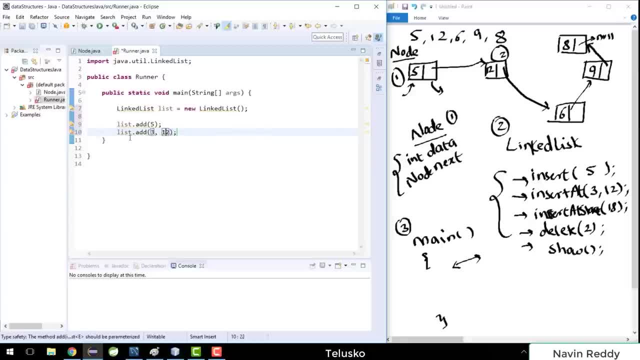 So the same thing which we are doing here, Maybe index value three which we're talking about, And then you can also delete elements, So you can say: list dot, delete, Okay, we have remove, So we have remove, We can specify the index value. 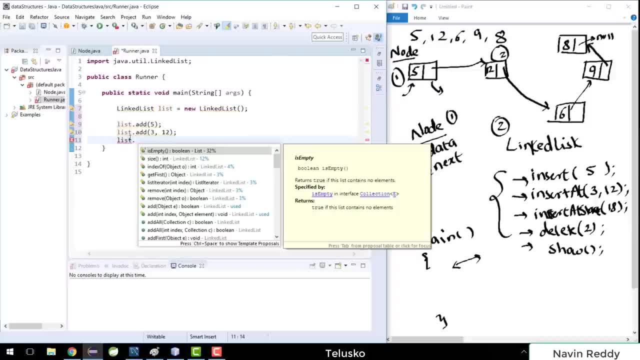 The method which I am going to use is delete. And then do we have a show method? We don't have a show method here, but we have size. Okay, we are missing size there. We'll be doing that later. And okay, we don't have the show method here. 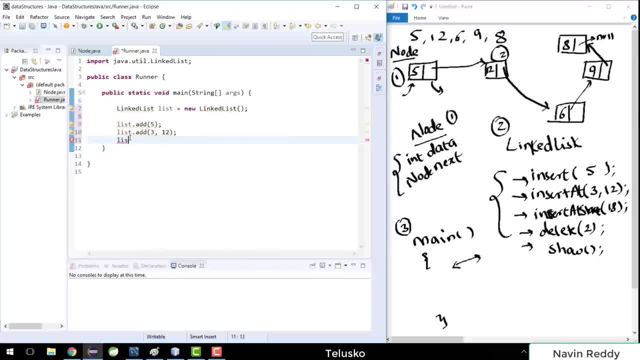 but then we have iterator, using which you can fetch all the values. In fact, you can print the entire list as it is, That will work. This is how you work with list, But then I don't want to use the internal implementation. 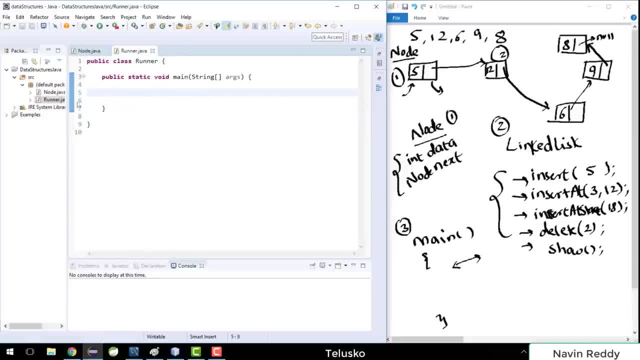 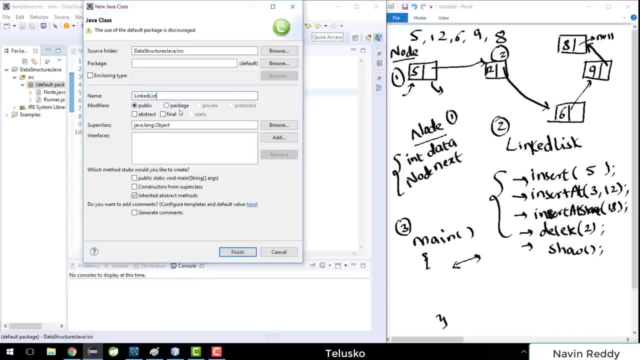 I want to go for my own implementation. So of course we need a class. So I would say the class name is linked list itself. Again, don't get confused with the name which we are using and which is provided by Java. I'm going for the same name. 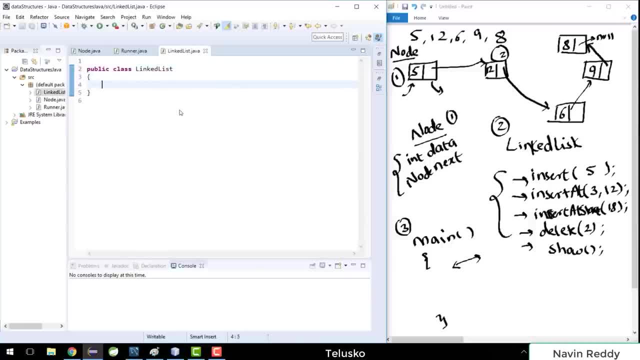 but since they're in different package, we can have our own class names. Now, this class need to have certain methods. right Even before creating a method here, what I'm going to do is every list will have one thing, and that one thing is: 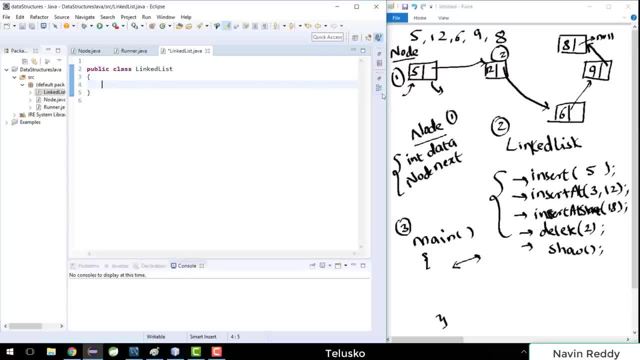 okay, so how do you know that this is a first node? Now, if you remember, we use a concept of a head node, So the first node will be referred as head node. And where do we define it? So in the list itself. 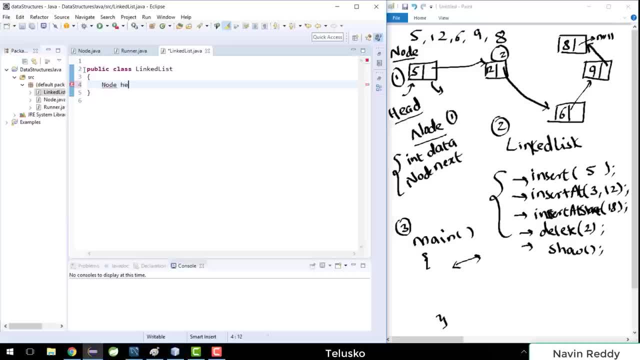 I can say: I have a node which I will call as head node, So this will refer to the first node. Okay, that's it. So we got that node there. Let's implement the functions. First of all, this code is difficult to understand it. 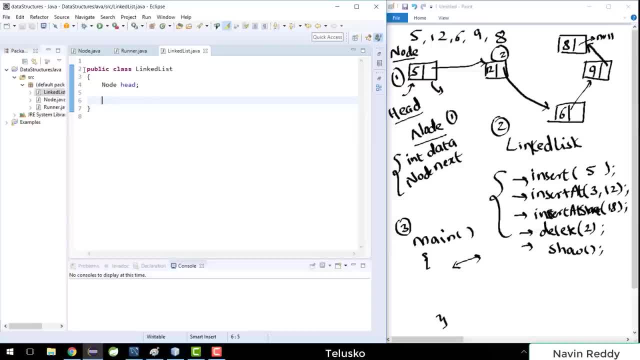 because it's not a good code. So let's go back to the first code. What I would say is watch the entire video and then try it by yourself. So maybe you'll be watching this video two to three times, So make sure that you also practice this. 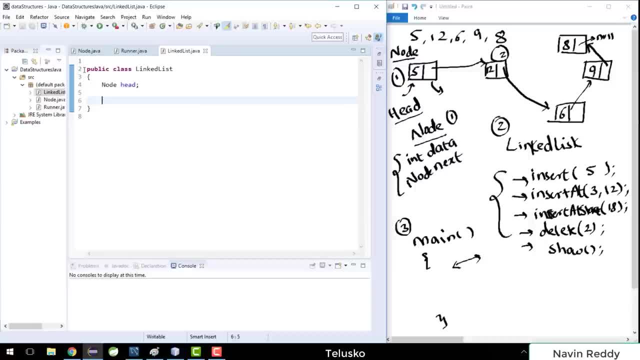 that's where you will get this concept. Okay. so let's start with the first method. So the first method we want to go for is insert. So let's do that. So I would say public void insert. That's the first method I want to go for. 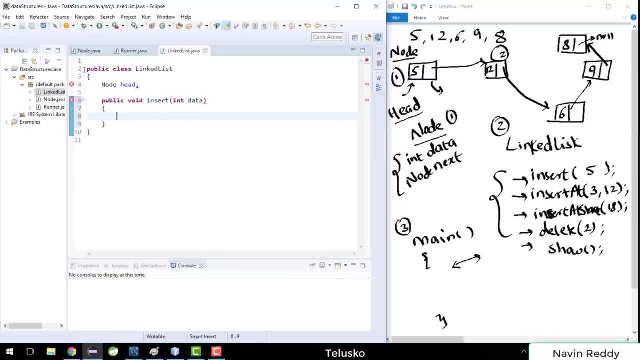 And this will accept an integer value- I would say integer data itself. So this is what I'm expecting from the user. So let's say I want to go for a node. So whenever you call an insert, what we have to do is we have to first create a node. 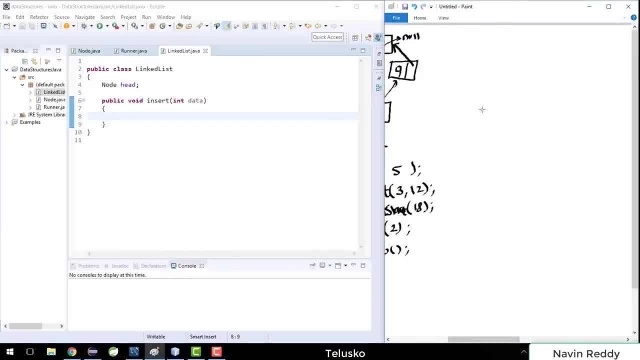 So what I will do is: I will just clear this up. So let's use this area here on this side. So what we are going to do is: every time you say insert, you will be creating a new node. So let's get a node here. 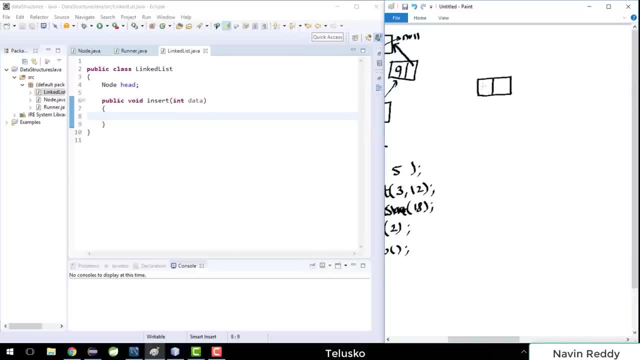 And this node will have a value, which is whatever value you are passing. So what we are going to do here is let's create a new node And then the way you create a new node is by saying node, And let's name that node as insert. 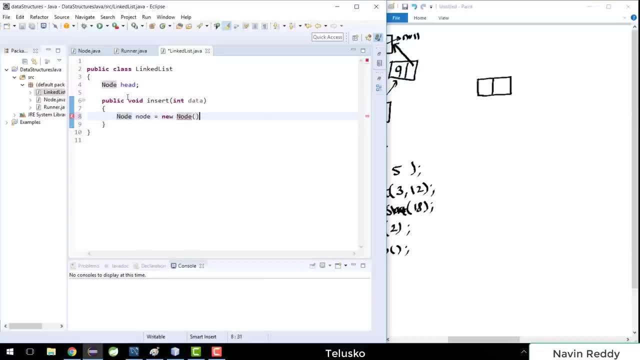 And let's name that node as node itself And we will say new node. This is how you create an object, right? So we got a node there. The moment you say node equal to new node, this is what you will be getting in your memory. 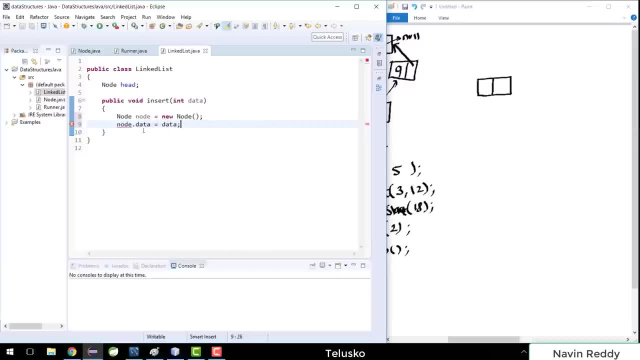 The next thing we have to mention is two values of it. So we will say nodedata, The data which is coming from the user. So whatever user is passing, let's say if user pass 5, the node will get the value 5.. 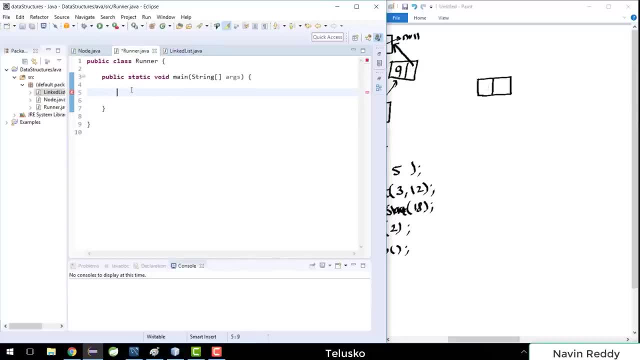 Just to make it more realistic, what I will do is I will also create the object of least, the link list here in the main. So I would say link list As least, itself equal to new link list. And in this link list, 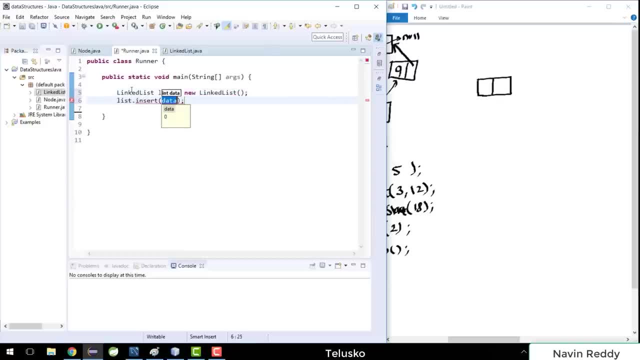 I have only one method right, Which is insert. This insert will take a value. Let's say I am passing 5.. So this method will call 5.. It will pass 5 and that 5 will be assigned to a node. 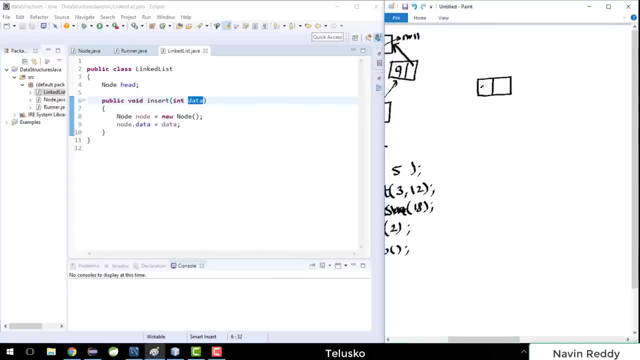 Which means this node. here it will be having a value which is 5. That simple right, And by default the value of this one will be null. So we got our first node. But then it is possible that this is our first node. 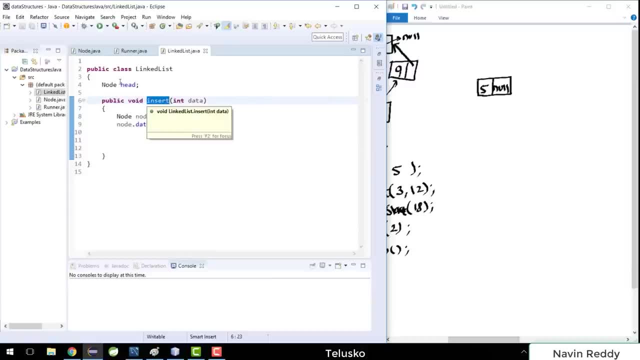 So what we are expecting is, when you say insert, it will add the data at the end. So if you already have a list with you, it will simply add data at the end. But what if you don't have a data itself? I mean, you don't have a list itself. 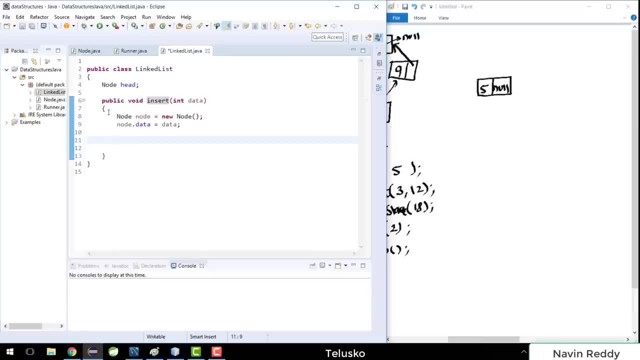 This is your first node In that scenario. you have to check, Because if this is your first node, then the head would be null, right, Because by default the value for this head is null. So if it is your first object. 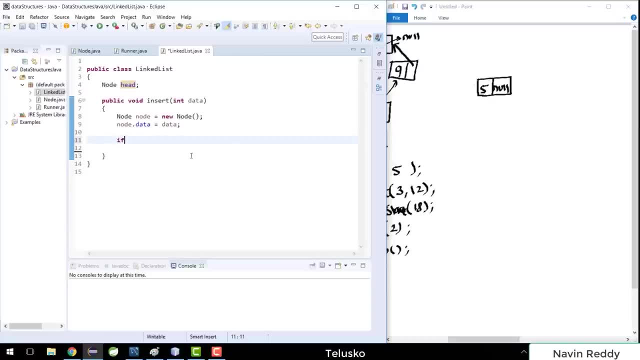 this is the first object we are inserting, so head is null. But if the head is equal to null, in this case, I would say the node itself is a head. So we will say: head equal to node, So the first node itself is a head. 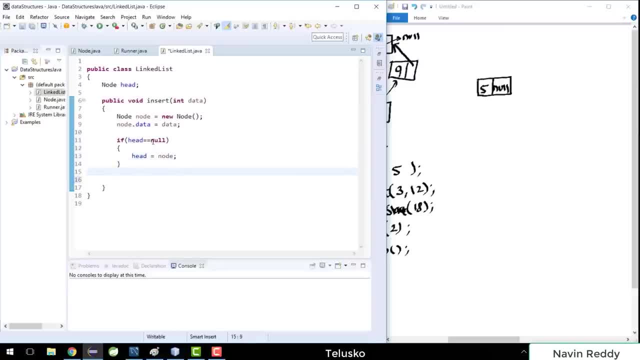 But what if that is not a scenario? What if this is not your first node? We already have some nodes there. In that case, we will go for the else part. So the first case we are checking is: what if your head is null? 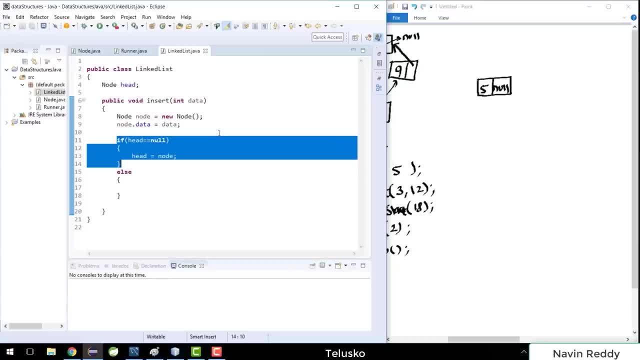 So when you say head is null, it means you don't have any nodes in the list. So whatever node you are adding is the first node. In that case we got the node. The next value is null. In fact, if you want to make it more readable, 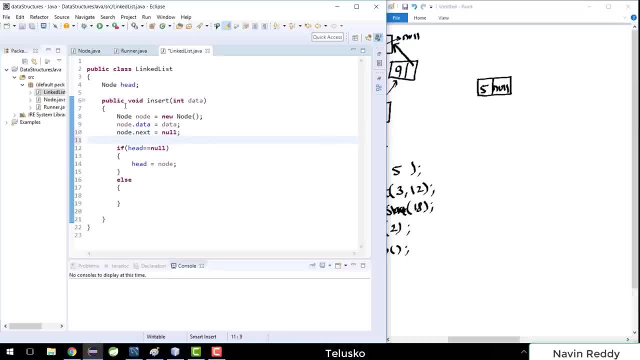 you can assign that to null. Even if you don't do that, that's fine, because by default the value for the object is null. But then this looks more readable, right? So you can do that. So if it is the first object that's become your head. 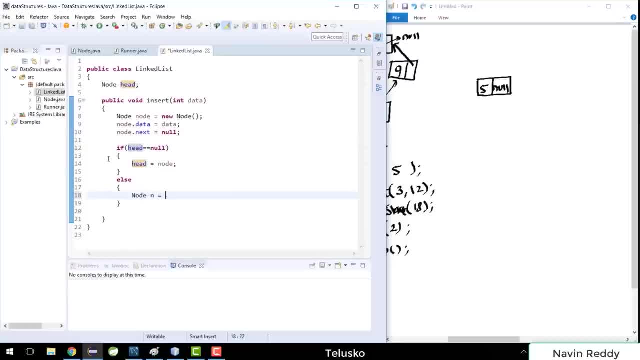 But what if this is not the first object? In that case, you will create a node and you will make it as head. Okay. now why I am doing this? It's because, let's imagine, you already have a list. So let's say, if you have multiple nodes here, 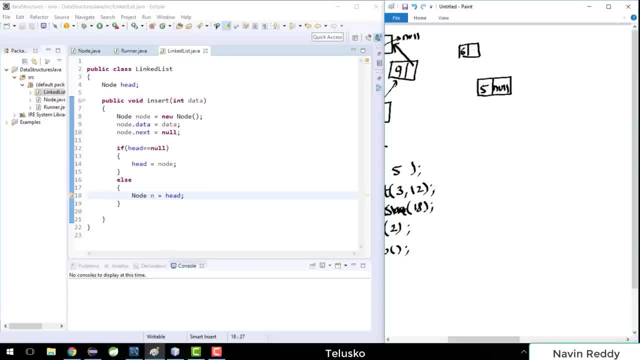 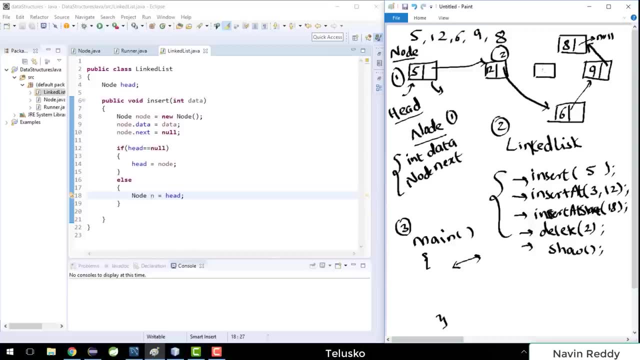 We got 6 and in fact let's go back to the original diagram. Now you can see if I am adding a node in between or somewhere here. So let's say I am adding a new node which is, let's say, the value which I am passing here. 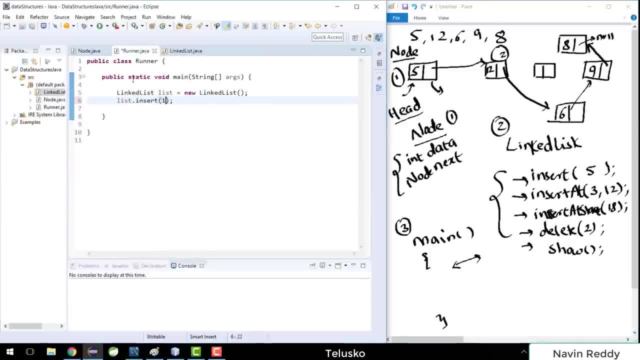 is not, let's say not, 5, it is, let's say, 18.. I am passing 18 now. So we got a new node and of course this is not the first node which we are adding. So head is pointing to 5.. 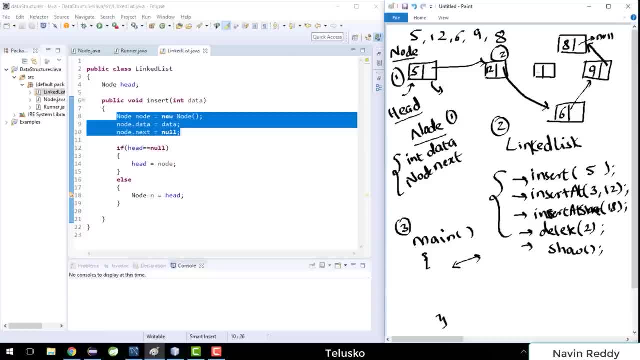 So in this case, what it will do is it will create, it will assign the value here, which is 18.. But then this is getting added at the end, right, That means after 8.. What we have to do is we have to first check, which is the last element. 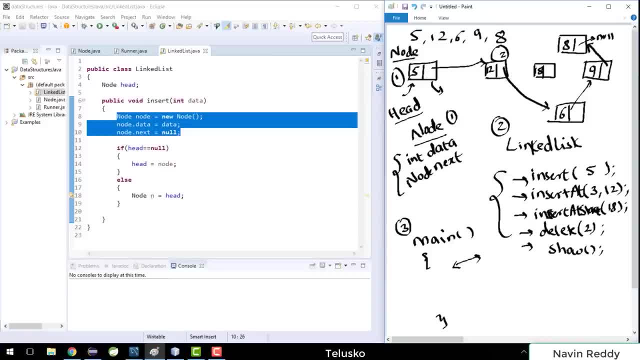 How do I know which is the last element? And that's where you have to start with the first location. So from the first location you will travel from the first location to the last location. Now that is tricky right. How do we travel? 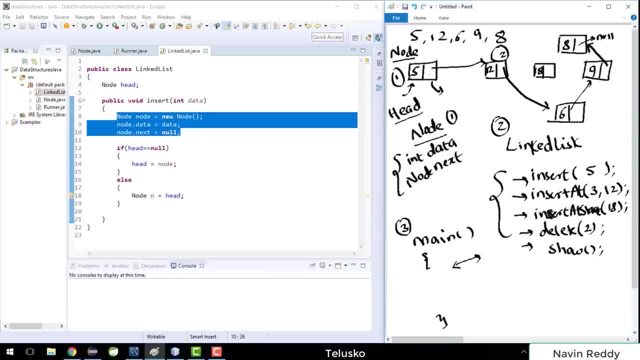 Is it that easy? No, it's not that easy, but just try to understand. So from the first one we will go to head first and, using head, we will jump to the next node. So from the second node you will jump to the third node. 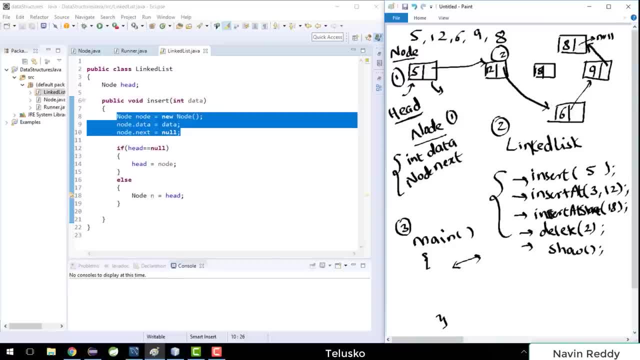 From the third node you can jump to the fourth node and then fifth node, But how do we stop? Where do we stop? So we have to stop the moment you get null as the next value. Now this looks simple. So to traverse we have to use 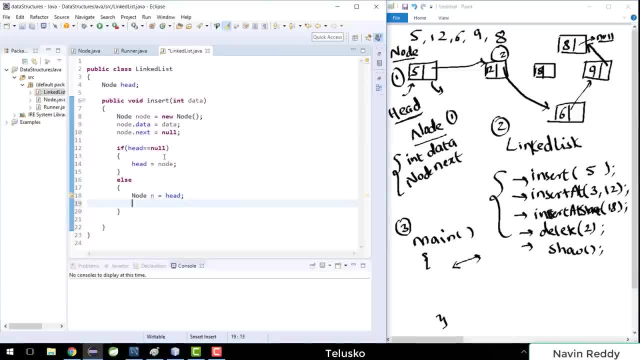 a node, a temporary node, which will hold the data, and that is, let's say, n here. So we will say while nnext. Since we have to traverse between different nodes, so we will use a while loop. So we will travel till you got a null value. The moment you get a null value, 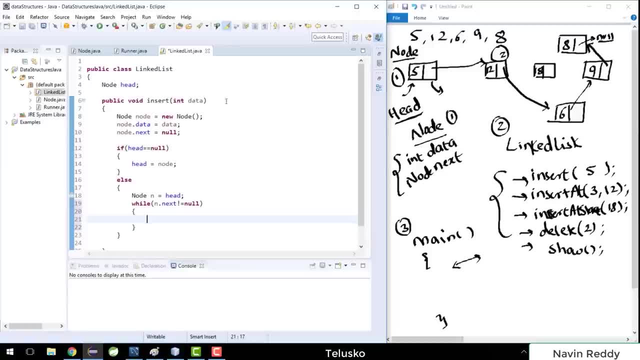 the value will stop. So how do we traverse? So what we are doing is we are saying nnext equal to null. So we have a temporary node here. Let's imagine I am doing that node, I am creating that node here. This is a temporary node. 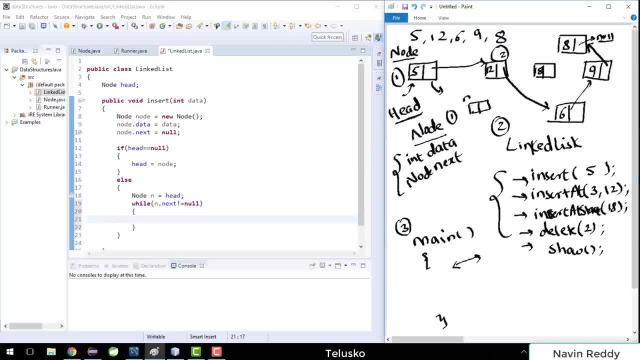 And I will call this node as n. Now this node will first refer to the head node. So it will refer to the head node And then head node will check: Do we have a null value here? No, we don't have a null value, We have the address. 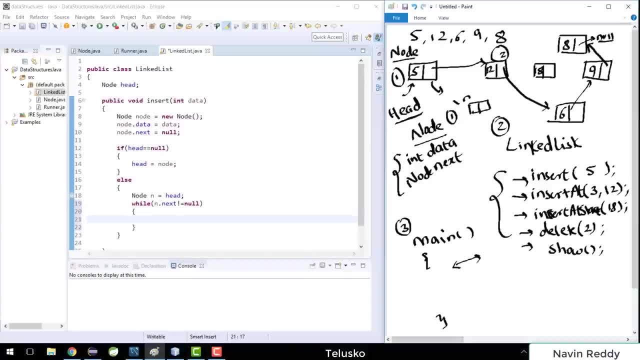 of the second node, In this case a reference of second node, So it is not null. So then we have to jump from here to here. Now, how do we jump? So to jump, what we will do is we will change earlier this was. 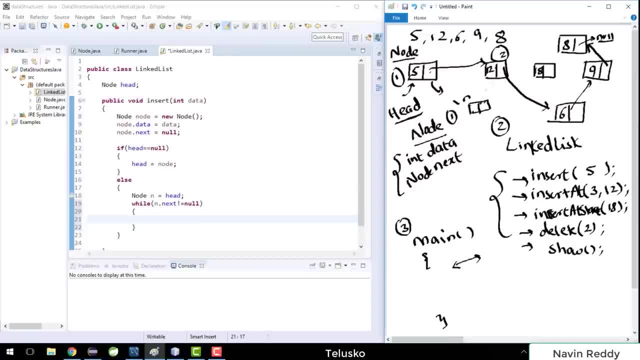 referring to this node. Now, we have to refer to this node. Now, how will you get this node? It's very easy. You will say: n is equal to nnext. So now you are jumping between nodes. So if it is not null, let's jump to second node. 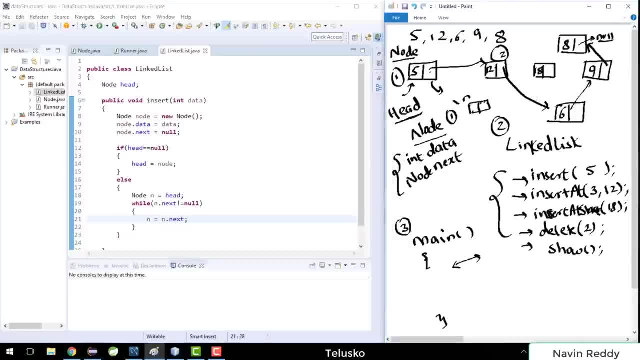 If this is not null, let's jump to third node And using while loop, we can do that Now. this will stop the moment to get null at the end. Now, once you got the null, what you will do is: once you got this null here. 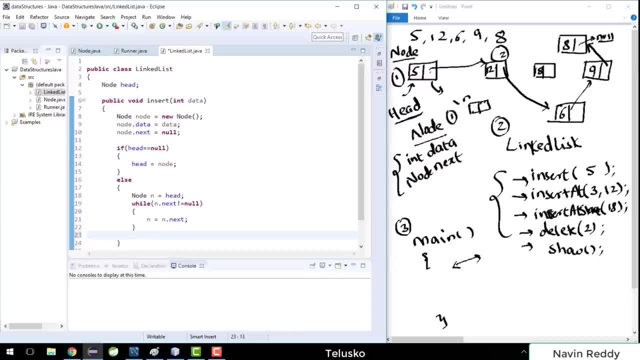 you have to change this value. You have to change from null. here. This is not null anymore, So this will refer to the new node which we have created. Now, how will you do that? So to do that, we have to say nnext. 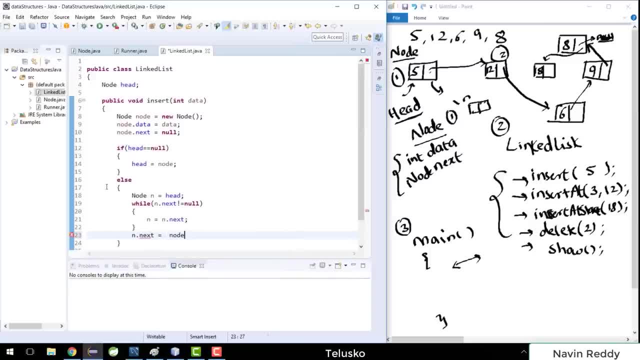 is equal to the new node which we have created. That means the value of this node, because the current n value is referring to this node. Again, this is the tricky part in Java. You have to work with objects. So imagine when the loop gets over. 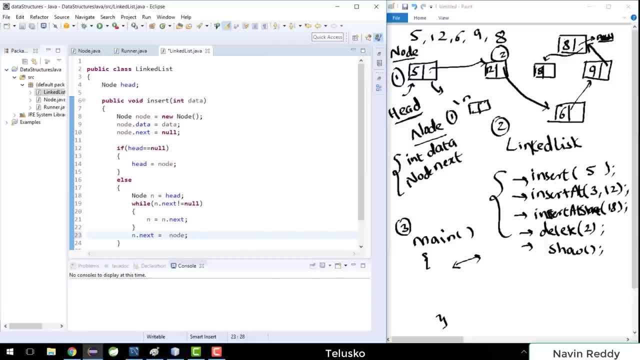 So at this location, when the loop gets over, you are here at this node. You are here at this node. Now what you do is you have to just change this null to the next node. whichever you have, This is a new node, So the value of node will be assigned to. 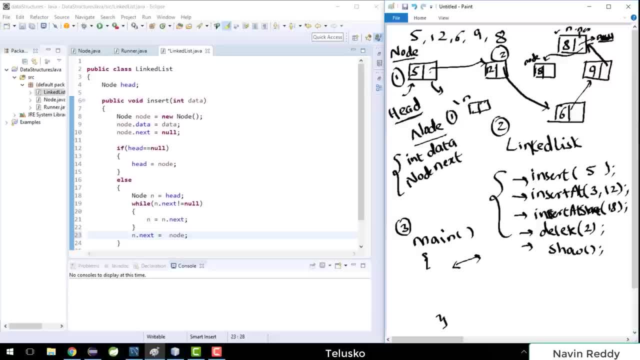 the current node dot next, which is this value, And this will be replaced by the node reference, So you don't have a null anymore And this is null by default. Now, if you can see the code here, We have a null value here. 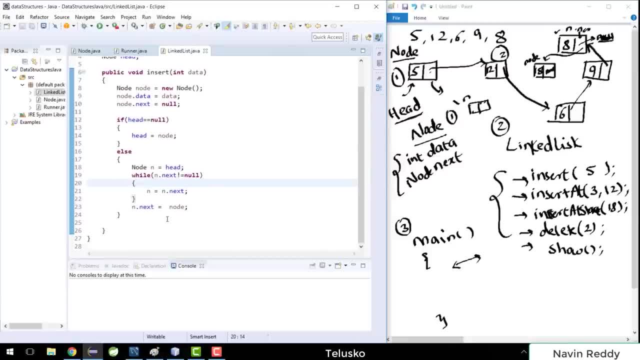 This looks cool. Now, this is how you insert value. Can we verify? Now, even if you can verify, we don't have a way to print all the values. I will insert the data and I will also try to print it. Now, how do we print it? 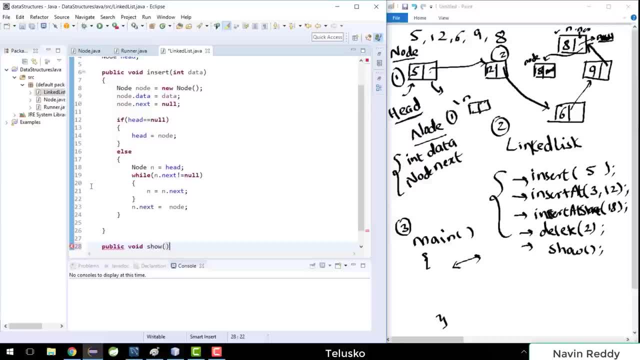 We can use a show method to print all the values. I will say public void show to print all the values. And how do I print the values? We will use some methods, We will use some statements to print here. Now, how do we print the values? 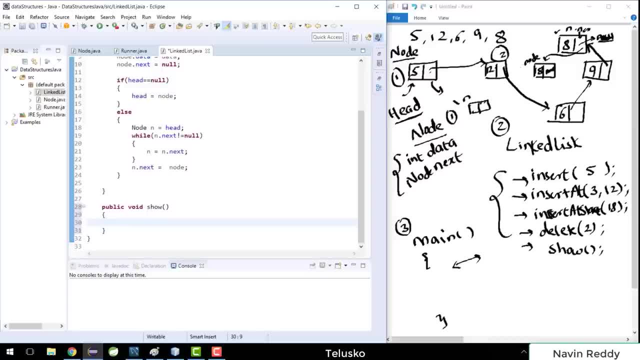 So same steps. You have to traverse from between all these nodes. Now how will you travel between all these nodes? You have to say node n. Again you can say node, node equal to head. So initially you have to start with head, And then we will be using a while loop. 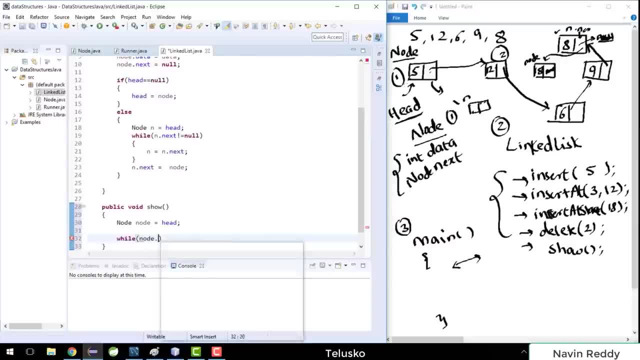 We have to travel right. So when you want to travel you will use a while loop. So we will say n dot node dot next is not equal to null. So while traveling you will print the data of the node. So you will say system dot out, dot println. 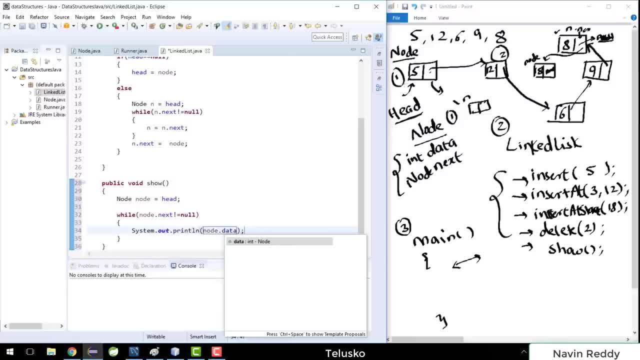 and you will print the data of the node. So you will say: node dot data. That's it. This is what you are going to do, And every time you print it you just have to shift to the next node. And the way you can shift to the next node is by saying: 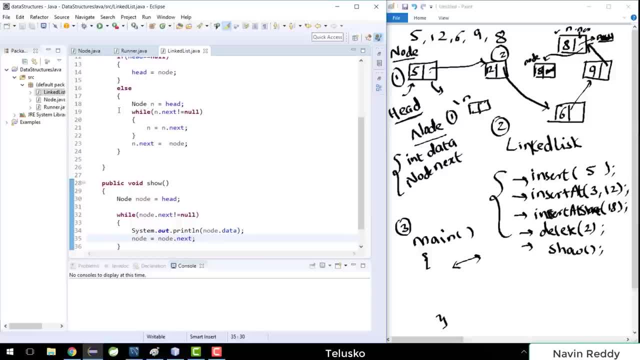 node equal to node dot. next, This is how you shift. Now see this loop, The same loop. The only thing which we are doing here is we are printing it. That's it. I hope this will work, But let's try. 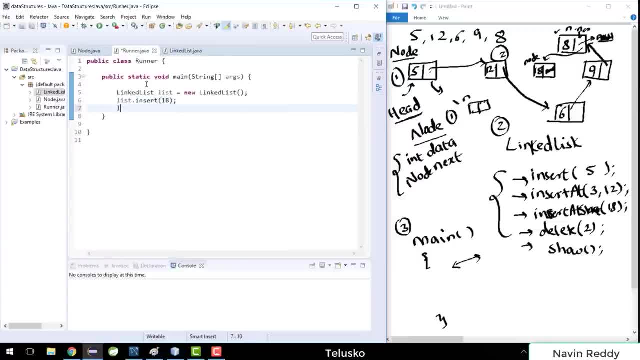 I will insert not one value. I will insert 3 to 4 values. So I will say least dot insert. And I will insert 45 as well And I will say least dot insert, I would say 12.. Let's add 3 values and at the end I will say: 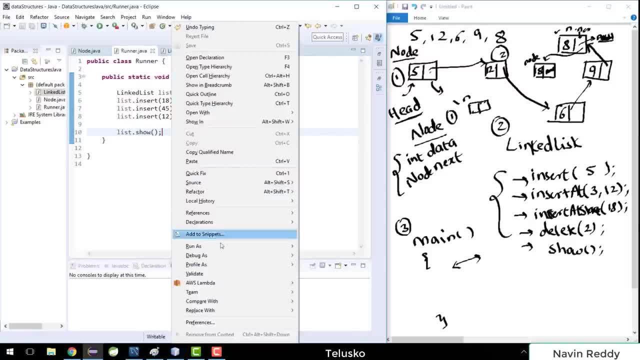 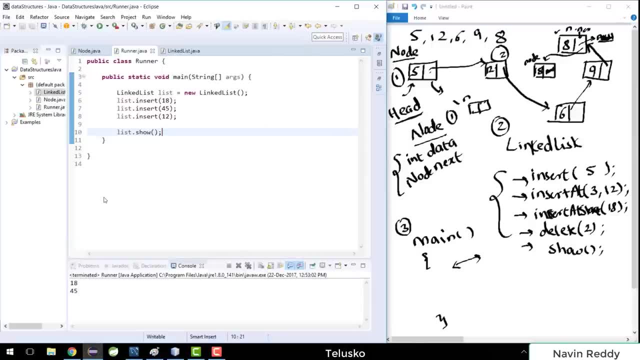 least dot show. I hope this will work now. So let's run this code, Right click and say run as java application, And we got the output. But with one mistake: You are getting 18 and 45. That's perfect. 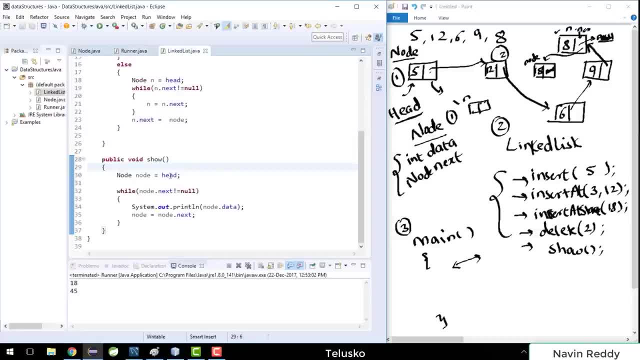 We are not getting 12.. Is it not getting added or is it not getting printed? I think it's not getting printed. It's because you are traversing till null. The moment you get null, you are stopping it. In this case, we only have 3 nodes. 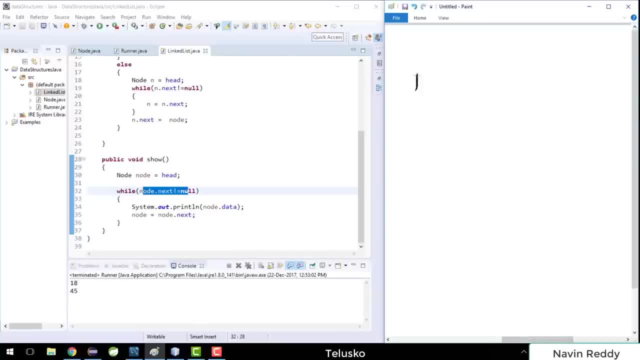 So in this case we only have 3 nodes. Let me just draw that here. So we got the first node as 18.. The second node as 45. And the third node as 12. So you got these 3 nodes. 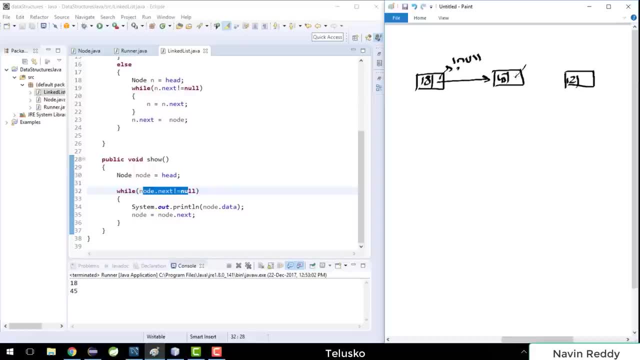 So this node is referring to this node. That means this is not null value. Even this is not null. So this is null, So it will stop as soon as you get null. That's weird. That means we are not printing this one. 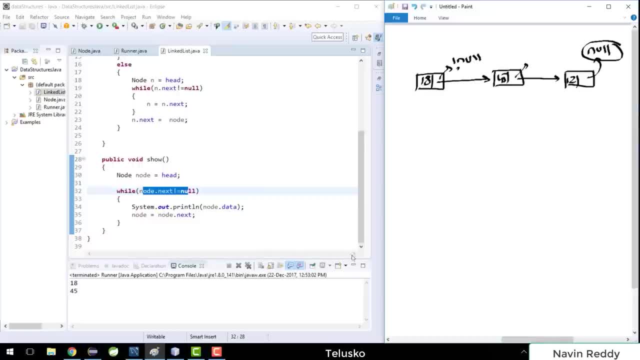 But we are reaching to this point. So when you say it will print data, it will not print data which has an object which is null. In that case let's do it manually. So I will say systemoutprintln and here I will say nodedata. 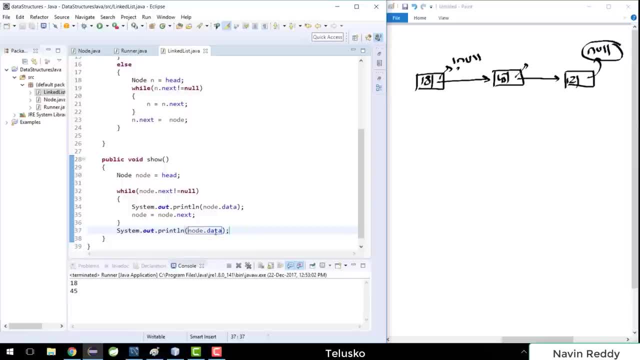 So for the last element, you have to print it outside the loop because it will not get printed in the loop itself. Now let's run the loop And you can see we got those 3 beautiful values. So just to make a quick recap what we have done: 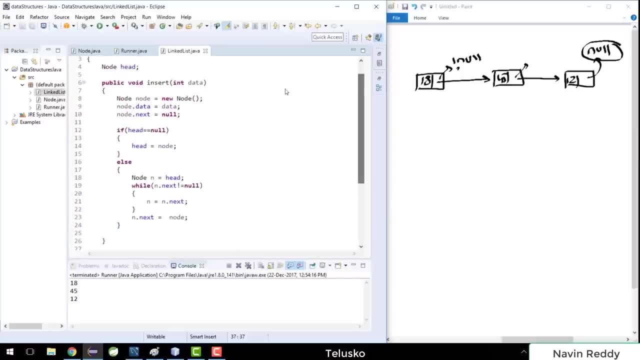 We have created 2 methods here. One is insert and one is show. In insert, what we are doing is we are creating a node, because that's what we do Every time you say insert, it will create a new node And that node will have a value, which is: 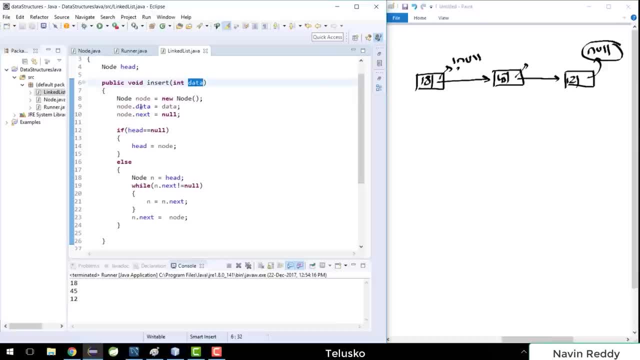 whatever data you are passing will be assigned to that node. Now, if you want me to go for a quick run through of this, we can use a debugger. So what we will do is: we will use a debugger here and let's apply a breakpoint. 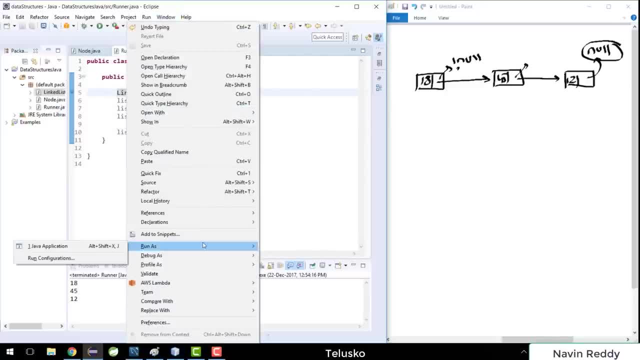 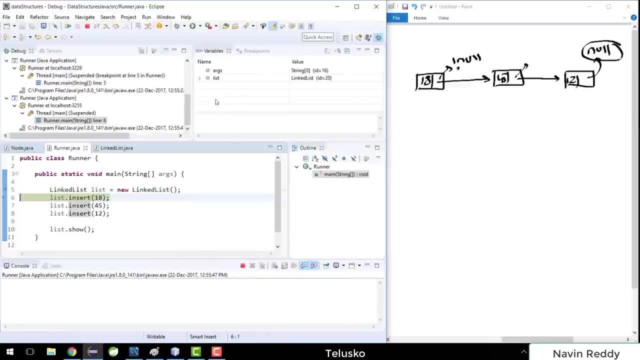 I want to apply a breakpoint And then I will run this in debug mode. I will say: run as Ok. where is the debug mode? It's here And let's jump to the locations. So we will say f5 and f5 will take to the next thing. 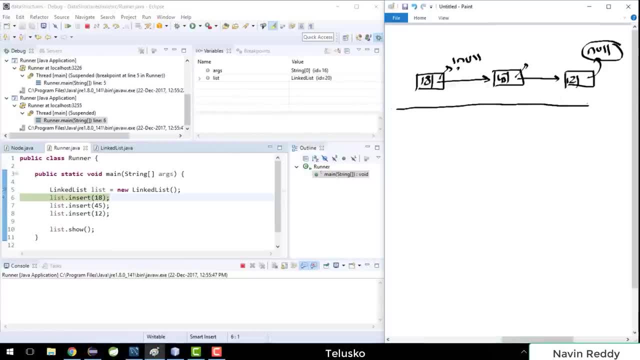 So what we are doing is: the moment you got a link list, So I will just draw it here- So the moment you got a link list, it will create the first element. So when you say insert, So insert, what it is doing is it is saying: 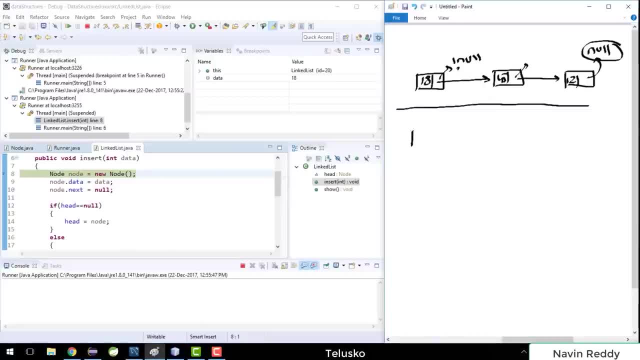 it will create a new node for you. So here it will create a new node. Ok, we got the node there And then we are saying, Ok, it will go to node class. it will take those two values and then it will assign the data. 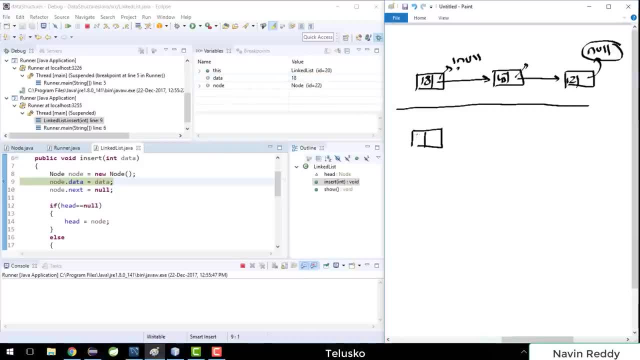 So the data is 18.. Can you see that It's 18 and we got 18.. And the id for this is 22. so let me just write 22 somewhere. So we got 22.. So the value is 18 and the id is 22.. 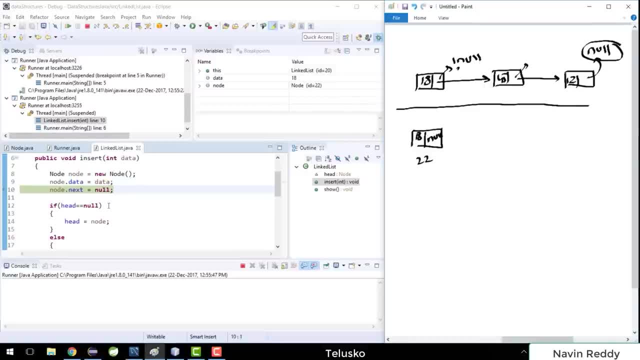 And then it is saying null, So the next one is null here. And then it is saying: if it is null, is the head element null. Yes, by default it is null, So head is null here. In this case, this becomes your head. 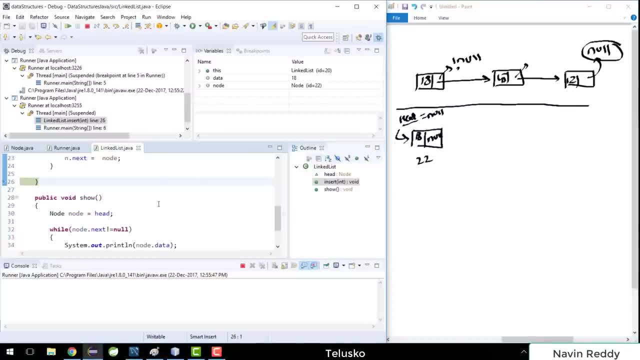 So head will point to this location now And then it will not go to else part because if got executed It will jump back to the second value, which is 45. So in this case it will try to insert 45. So the same step. it will create a node for you. 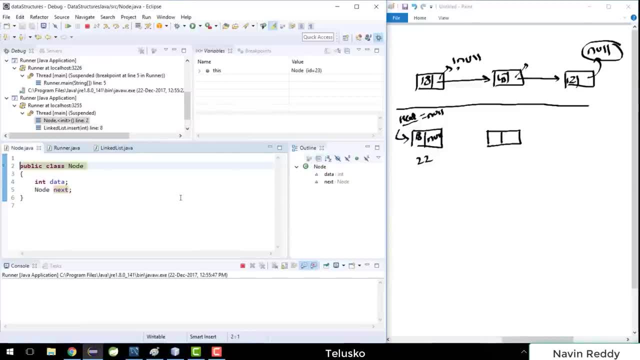 If I jump into this, you can see it is creating a new node and with those two beautiful values, which is data, and next It is the same data, which is 45. So we got 45 here, And then the next value is now when you say null. 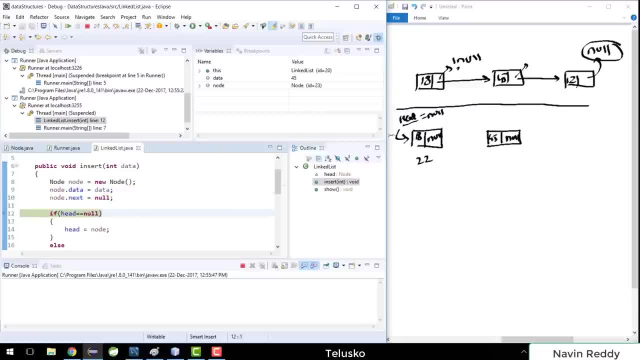 it will jump to the next location. Is it head null? No, it is not null, Because head is pointing to the first node here. So if will not get executed, it will execute the else part, and that is working Now. it will traverse between the elements. 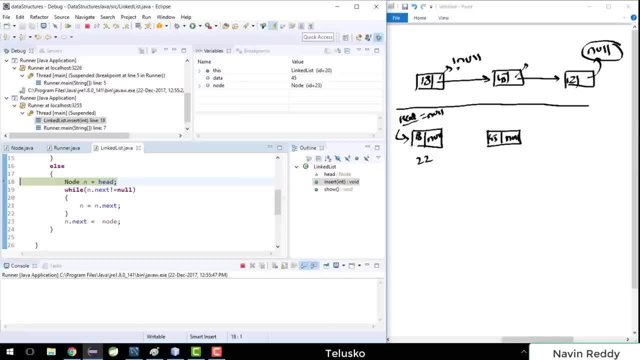 So first it will jump to head and check. if so it will traverse. The first element itself is null, So it will directly jump to the location here and it will say the end, this dot next. So this value will be replaced by the reference of the next element. 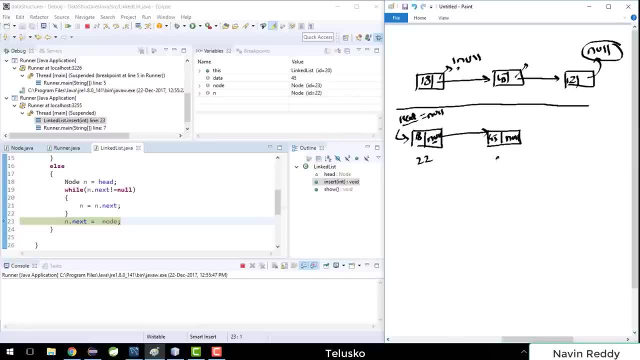 which is 20.. What is the ID for this? This node is 23.. So this will refer 23 now, And then it will jump back to the insert, the third block, and we got the object here with the value 12.. The same steps will happen. 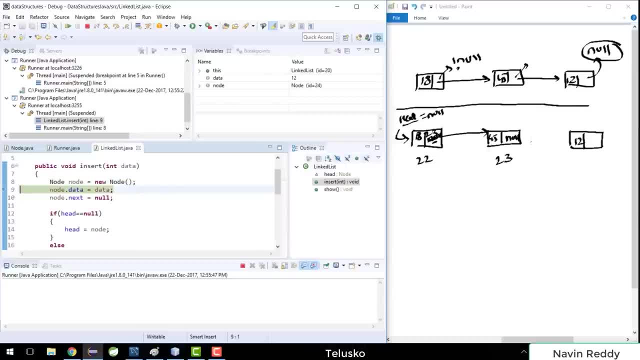 Now it will again go back. It will create the object, assign the data 12 and then this will be null. So the text will be null here And then it will jump to next. It will jump to head. Head is null. No, head is pointing to the 18th location. 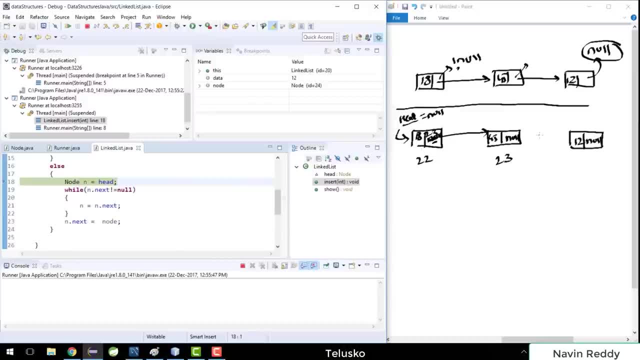 So it will not execute the if block. It will execute the else block In else block. it will traverse from the head block to the end block. So is the first block is null, You can say no, it's not null, So it will execute. 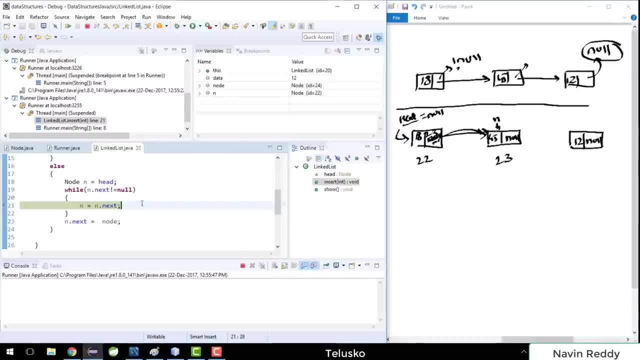 It will say: jump to the next location. So now n is referring here. Now is it null? Yes, it is null. You can see that it is null. The end dot next. Next is this one. So this will be replaced by the id 24.. 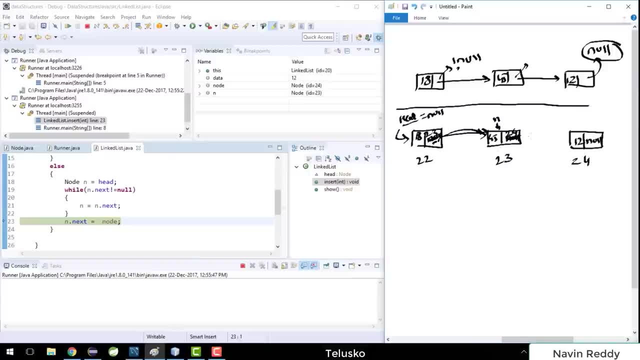 So the id for this object is 24.. This will be 24 here, And then you got a link. It's that simple. The end of the code and then the moment you say show. what we are doing in show is we are jumping from one location to another location. 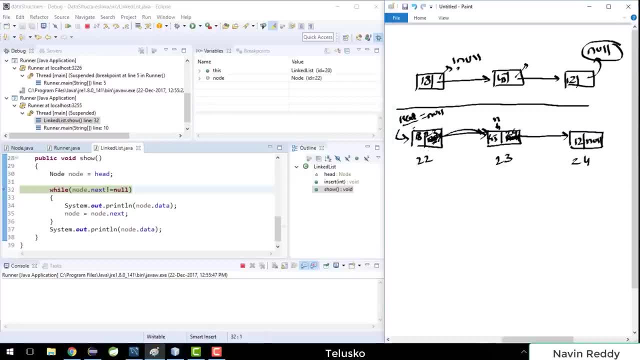 So it will start with the head location and it will check: Is it null? No, it's not null, So let's print the value, Which is 18.. So we got 18 there. You can see the output console window. here we got 18.. 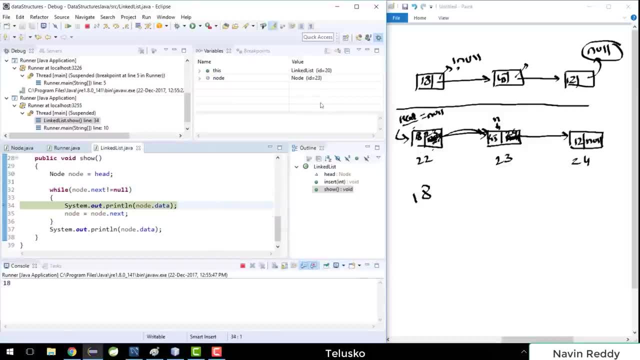 And then, when you say next, you can see it is printing the next node now, So it is referring to the node 23.. Is it So now 23? and then it will print the valid data of that, which is 45. And now, 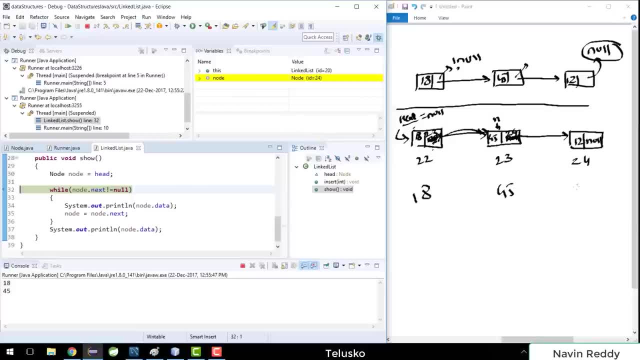 the moment I go back, you can see the node id is 24. now It is referring to 24.. And it will print the data, which is 12.. So this is the beauty of linked list. Now you can add values anywhere. Again, this is a lengthy video, so 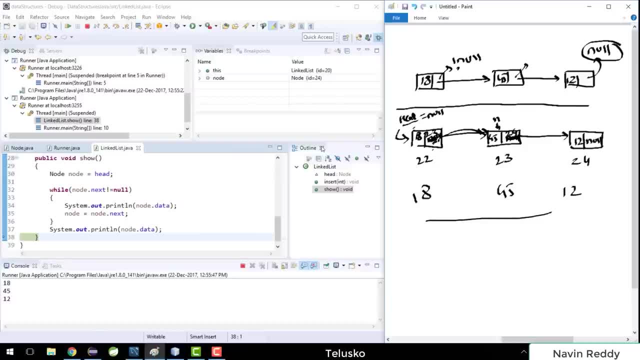 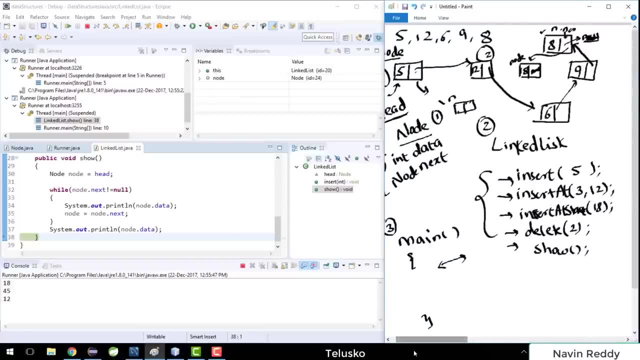 what I will do is the remaining part we will see in the next video, Where we will talk about the other methods which we have discussed. We will talk about insert, add, insert, start, delete and show. So the next will be faster because we have seen the difficult part. 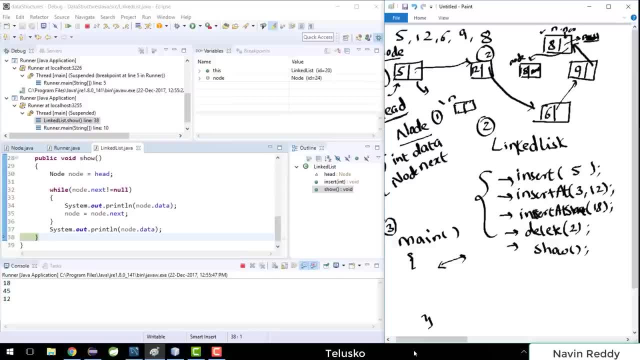 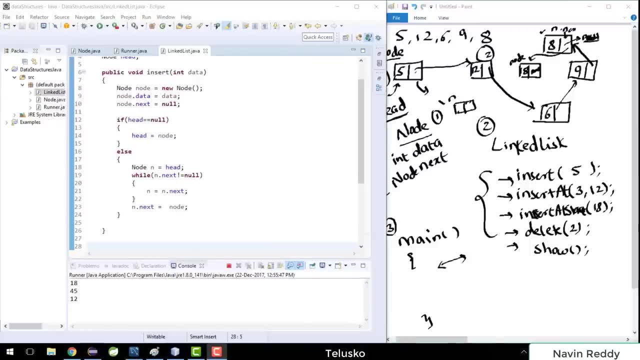 So I hope you understood something about linked list. Again, you may want to rewatch this video again, So let me know in the comment section if it was helpful. So now let's see how do we add element at the start. So we have seen how to insert. 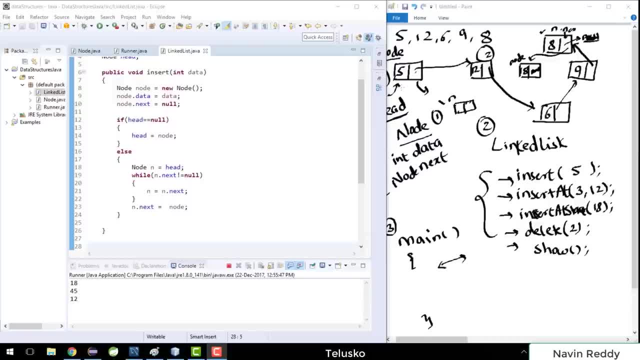 the element at the end. Now we will see how to add the element at the start. So what we are going to do here is: let's create another method and we will name this method as public void insert and then we will say insert at start. 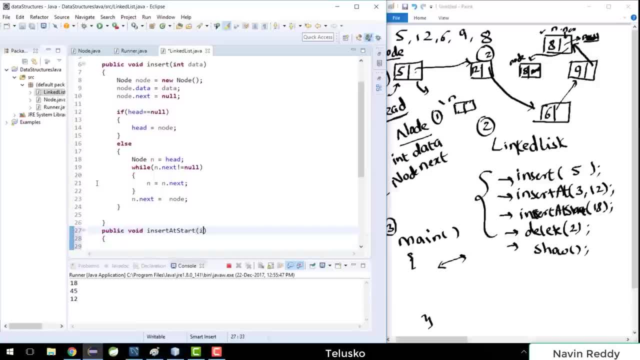 So we just have to pass a value there. So I would say the value would be int data. That's the value we are going to pass Now. let's try to add the value. Now, how do we add the value? So, if you think about this, 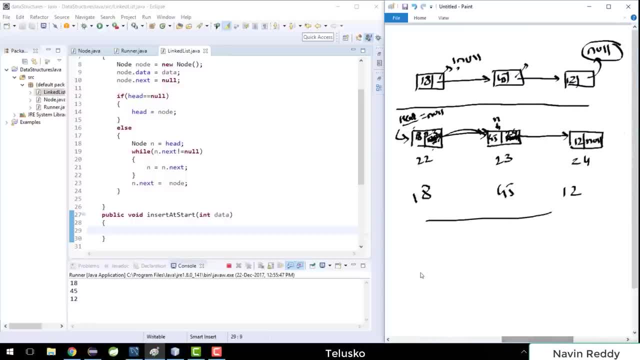 same thing which we have drawn before. Let me just take you there Now, if you remember this image. Now I want to add an element at the start. So I would say a new element, and this element will go at the start. So let's say the element. 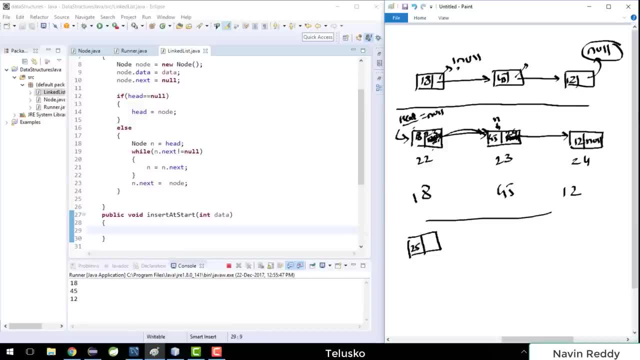 is maybe 25, so I want to add 25, and this will go at the start now. Now, when you say start, it simply means that you just need to change your head location from the current object to a new object. So this is the new head location. 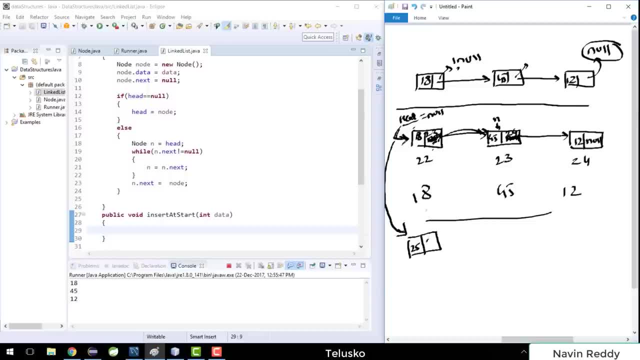 and the value or the address for this one would be the earlier first element, which is 18.. So the ID is 22.. So I want this 22 to be here so that it will refer to this element now. So now the new element is: 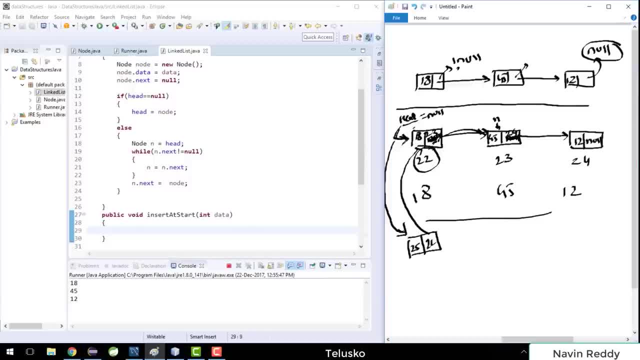 at the start. So the head will become the new element and it will have the address of the previous first element. So let's see how do we implement that? So, same steps, we have to get a node. So I can, you know, I can simply. 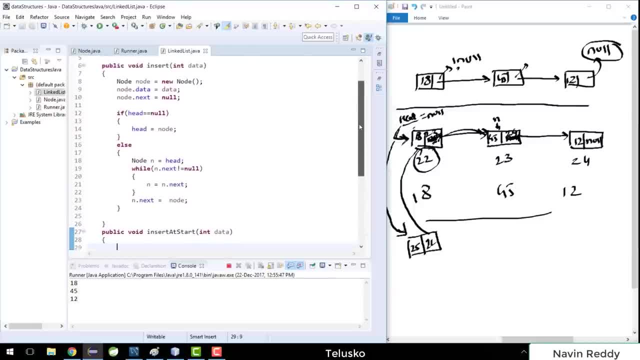 copy paste the code. now What I can do is I can say: okay, the same thing will remain, this thing will remain same, So we will copy and paste it here Again. we cannot say copy paste, I can say code reuse. So I would say: 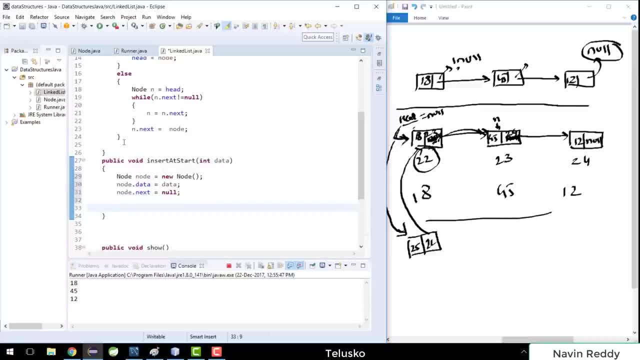 paste here And once I got the value, the only thing we have to do now is the node. So we have to say head node is equal to node The current node. Okay, so when you say, when you say you have to say head equal to, 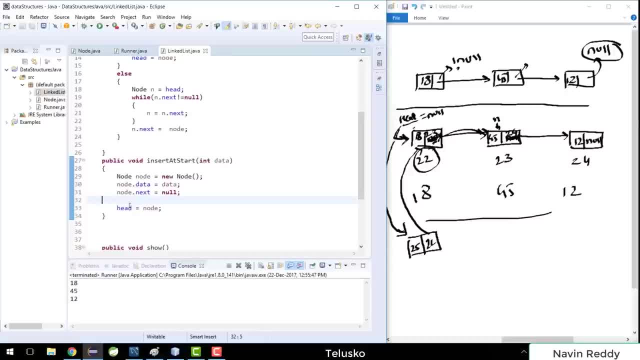 node. So the current node will become the head. But even before doing that, I just need to mention that the next node for this, So this, so the current node next node should be the first node And it is then the head, right, So head is the first node initially. 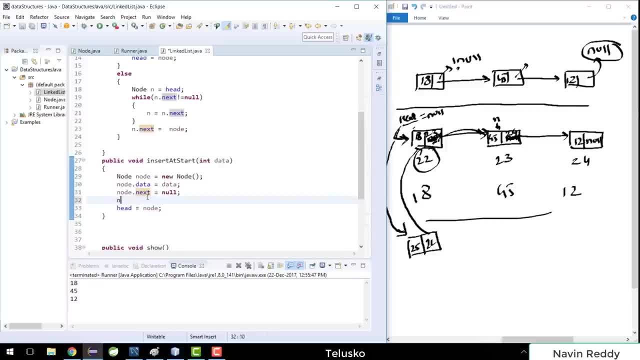 So I would say, before assigning the node to head, you will say nodenext, I want to say head. So whatever value was having with the head will be the next for this one. So let's say this node is maybe let's name it as n6. So this node, 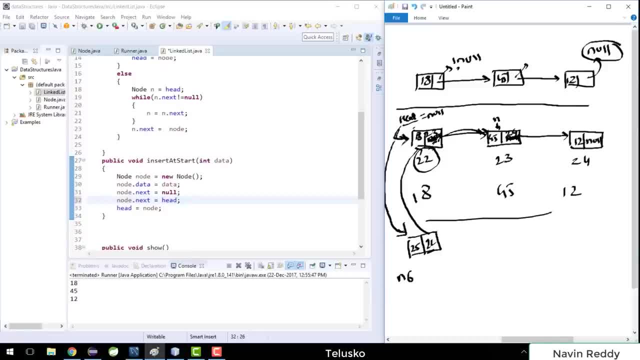 will have an address of this node. Initially this node was head, So we can simply say nodenext is equal to head. Is that simple? Let's verify if it is working. Just to verify that. what I am going to do is Let's go back to runner. 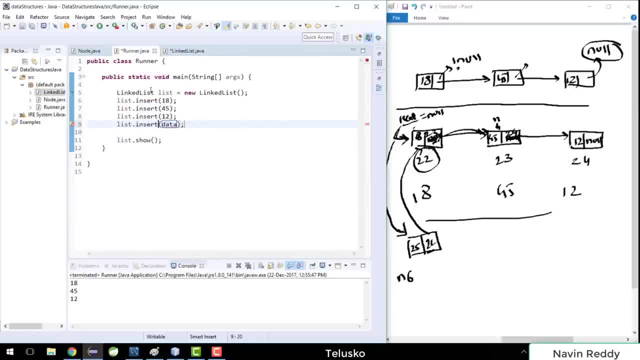 After printing: after adding 12, let's say insert at start. I will say insert at start And the element I want to insert is 25.. So now 25 becomes the first element. Let's run this code And you can see we got 25 at the start. So this is. 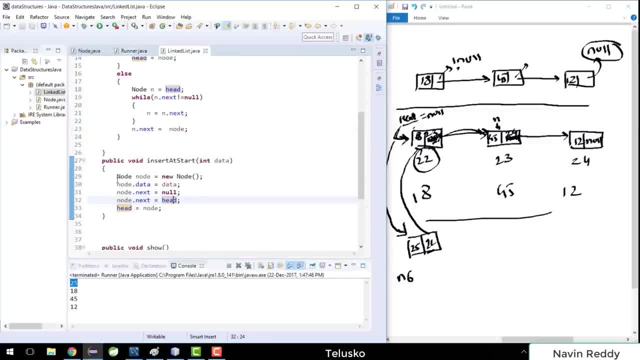 simple Now we can add the element at start itself. At start, what we are doing is we are creating a node and just saying that the node next element would be the previous head node, And now head will be changed to the node, So head will. 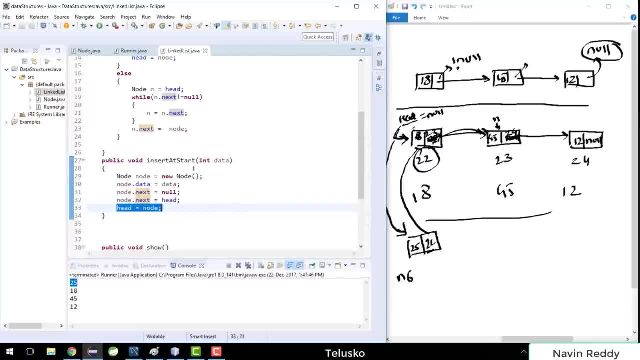 be pointing to the node which we have created just now. That is how you insert at start. The next method we are going to do is insert at any location. So I would say, insert at. And then we have to specify two things. The first thing you have to mention: 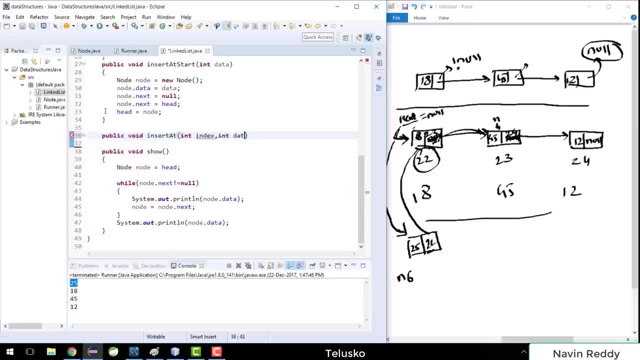 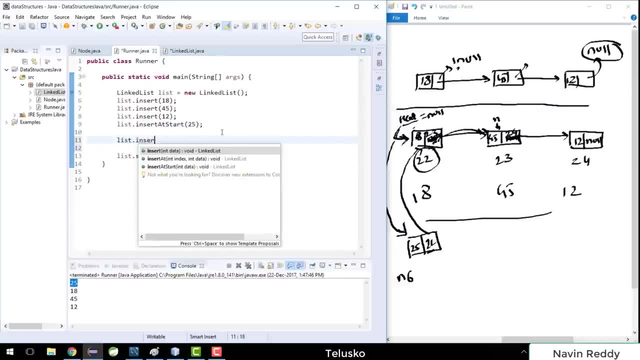 is the index value And then you specify the actual data. Now when you specify index value, maybe I want to insert a data here. So I would say list dot insert And I would say insert at At position 2.. Now index number normally starts with: 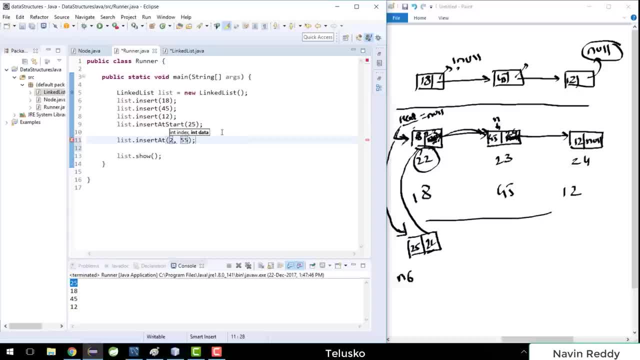 0. And we will say data is, let's say, 55. So I want to add 55 at location 2.. So when I say location 2, it is 0 location. So this is my 0th object now And this is the first. 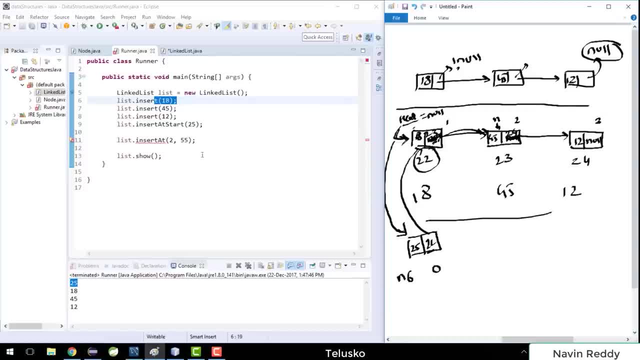 this is the second one and this is third one. So when I say I want to insert this 55 at, I want to add 55 object at index 2, which means here. So we got a new object and this will be 55 and this will have some address. So this object. 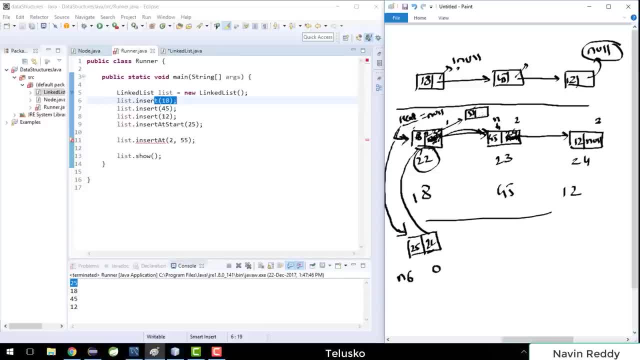 the first object will refer to the new object and the new object will refer to this one. So now this becomes 3 and this becomes 4.. In fact we don't have to number that, but then this is how you push. You have to push. 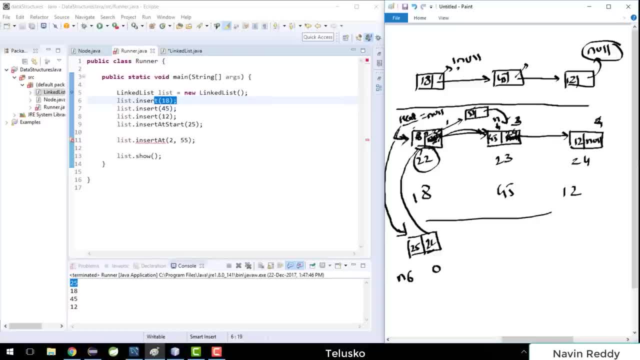 this one to the next location. So what you will do is you will just mention this node will change to this address and the new node which you have created will be will refer to the next object. Okay, now how do we do that and why are we getting error? 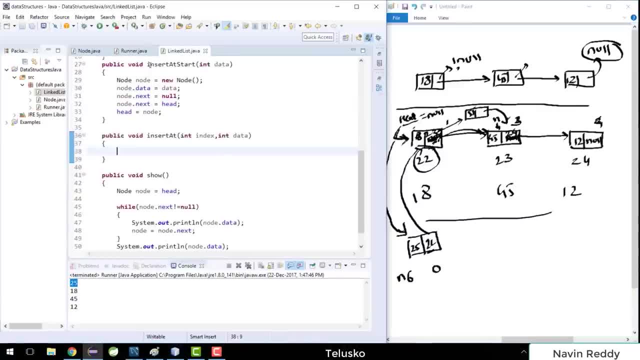 there, So I will go back to my link list. I guess I have not saved it Now. how do you mention that? So, to achieve that, what we will do is we will say: node node equal to new node, again the same steps, in fact, we could have copied. 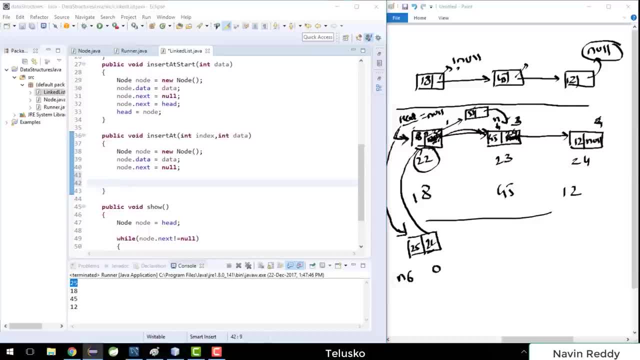 it. So I will say: paste. So this thing is for sure there with every insert. Now, in this case we have to traverse right, because we have specific index value. we have to traverse from that location to the index value and to travel we have to again start with the node, the head. 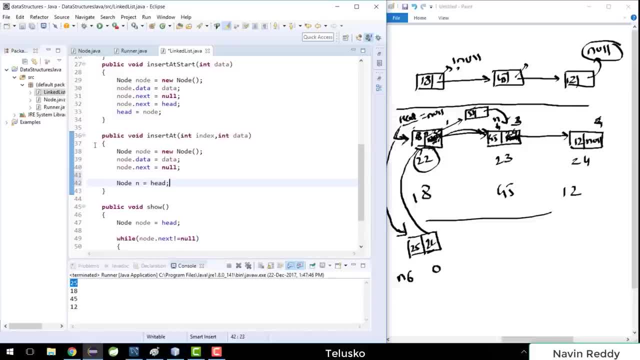 node. so I will say n equal to head. so remember, whenever you want to traverse, you have to always say node n equal to head. Now, how do we traverse now, since we know the index value? so whenever you know the value, it is always better to start with a loop. So 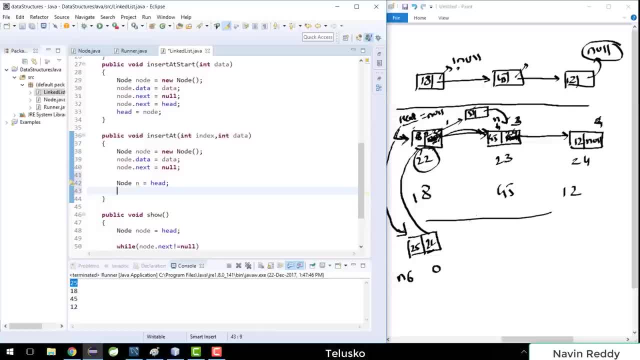 with that trace we have to go to this point. So if your index value is 2, you have to reach till 1.. So if index value is 2, you have to reach till 1, because in 1 you have to make the changes right. 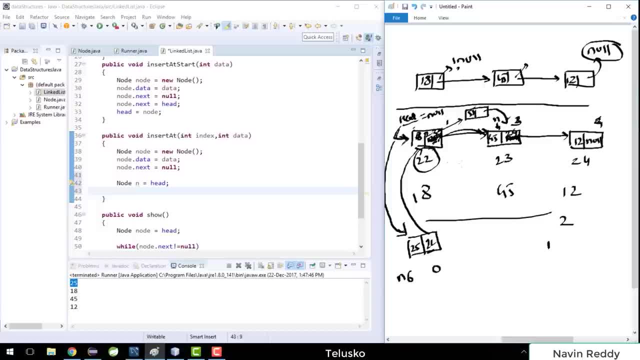 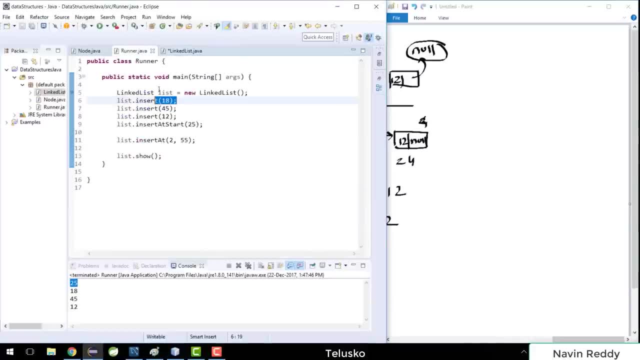 So if I say index value 2, you have to make the changes here. I guess this thing is not properly visible. let me just rewrite again, as I am very bad with writing and writing, So let me do that once again. So I got the first. 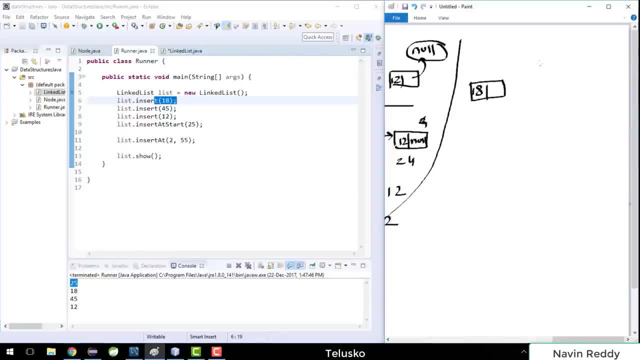 object here. So we got the first object, which is 18, and which is referring to the next object, which is 45, which is referring to the next object. let's say, this is 12 and oh, before that we got 25 right, because 25 is the first element. 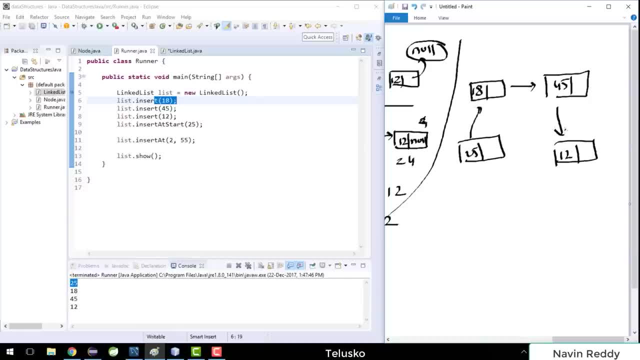 now. So 25 referring to 18,, 18 referring to 45, 45 referring to this one. now, when I say you want to count, when I say index value 2, it means this is 0. I have to start with 0.. This is 1. 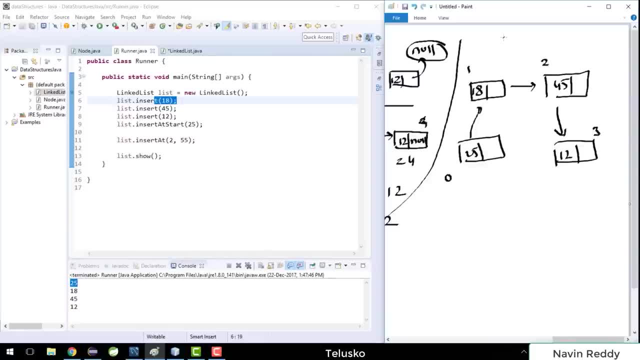 and this is 2 and this is 3.. Now, when you say 2, that means you have to get a new node here, somewhere here, and let's say the value is 55, so you have to reach till this node first. in this node you have to. 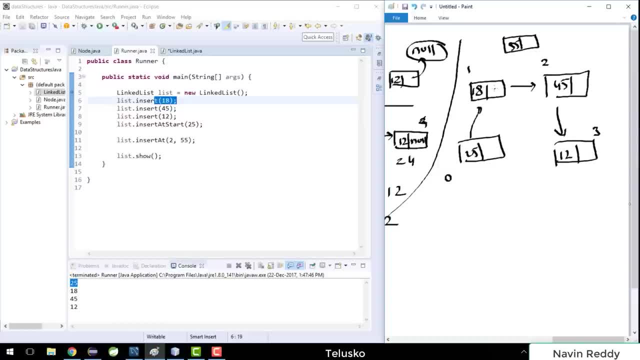 change the location from here, from this arrow to this arrow, and from here you have to refer this one. So first you have to reach till this point. now, since the index value is 2, you have to reach till 1.. How do we reach till? 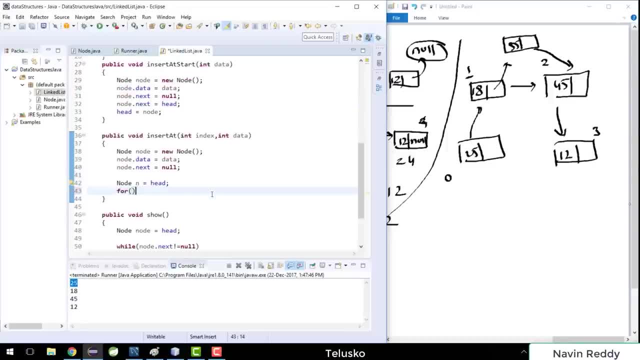 1 is by saying: let me just go back there. So we will use a for loop and in here I would say int, i equal to 0, and I would say i less than equal to index minus 1 and I would say i plus plus. 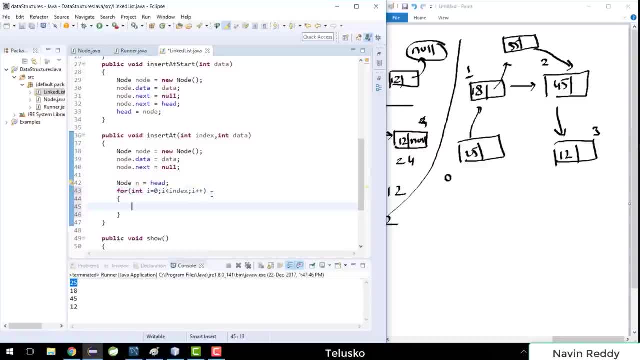 in fact not minus 1, we will say index. now, every time you traverse, you have to say n equal to n dot. next. that's how you traverse, right, ok. now there is one change: when you say next, that means we have to say minus 1, because 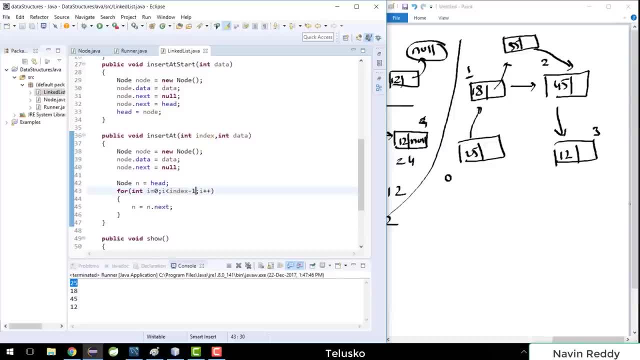 we have to reach here this node by referring next, because next itself is going for the next node. so you have to say minus 1, you have to come 1 back. once you reach till this point, you just need to change the address. right, you have to change the address of this node. 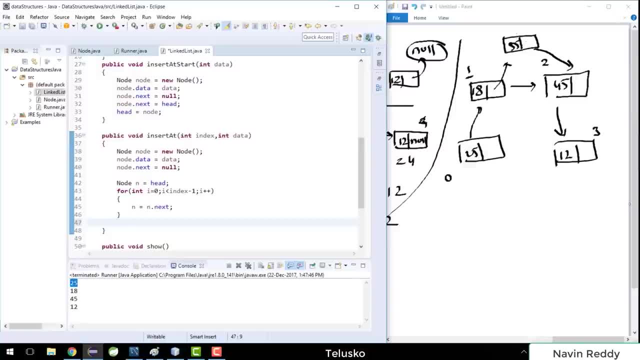 with the new node. but even before doing that, I will change the address of this node to this node. so this node, the new node which I have created, that is node. so this, in this current situation, this is node and this is n I want to have the value of. 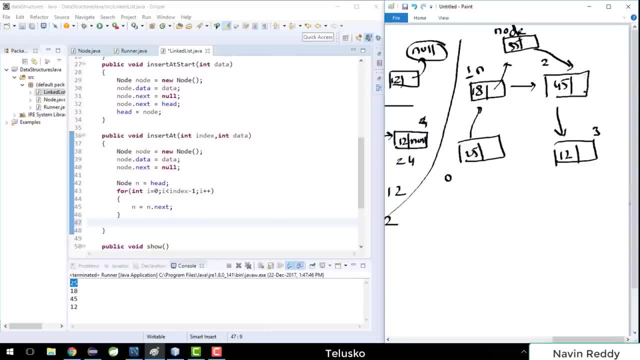 node next to the this value. now, to achieve that, what we will do here is we will say: node dot next is equal to n dot next, so n is this one. so whatever value, so whatever value is there here, will go into this node right, because this value is nothing but the pointer. 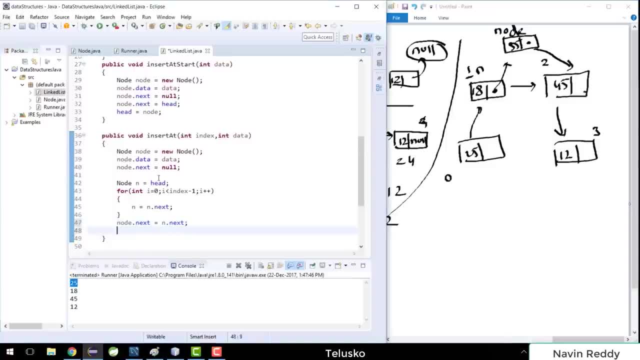 or the reference to the next node. ok, we have done that. now we have to update this value, so this node, so the 18th node, now will have the address of this node, and to do that we simply say n dot next is equal to node. and by doing this, 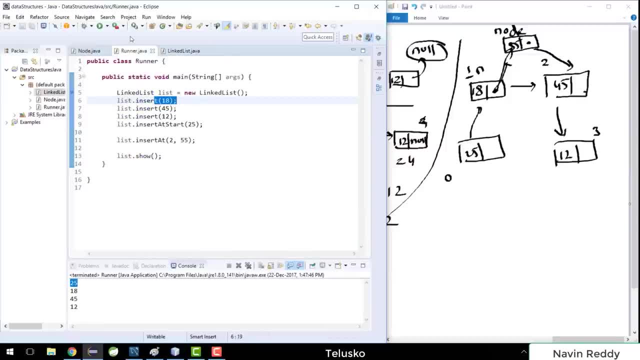 our job is done, let's verify. so I would say: insert at 2. let me just run this code and you can see we got 55 at 2. so 25, 18 and 55. is that simple? awesome, right? so this is how you add. 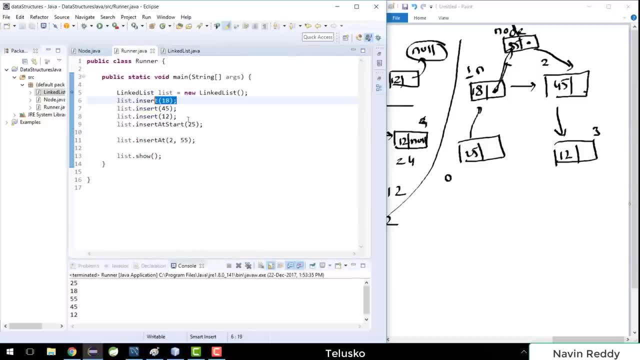 the element in between. but there is only one twist: what if I add at 0th location? because for 0th location it is a bit different, right? so if I run this code now, you can see it is adding at the first location. so it is not working. 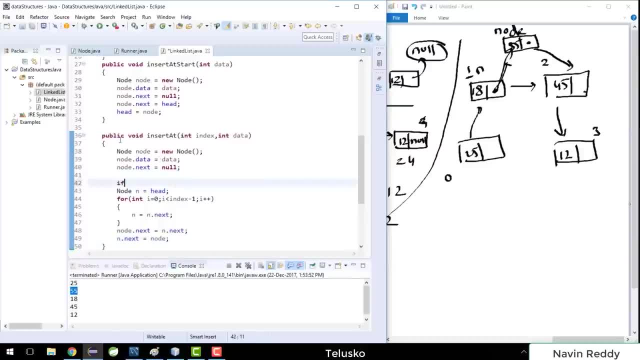 so for 0 we have to put a special condition here. so we will check if the index value is equal, equal to 0. what we will do is we will simply call, because see, when you say 0, it means you want to add at start, right, so you simply. 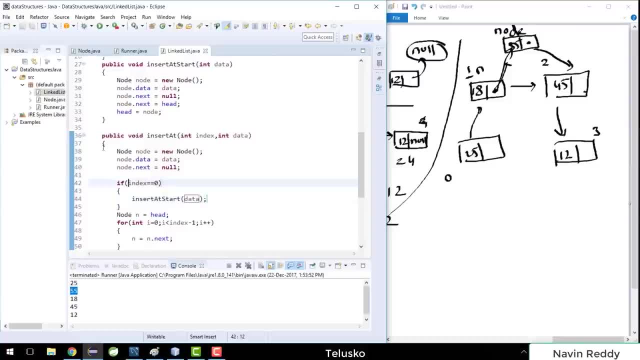 call that method. start by passing this data. so in case if the index value is 0, that means your intention is to start from the first location. so you have to say insert at start. so this is how you add the element at any location which you want. so 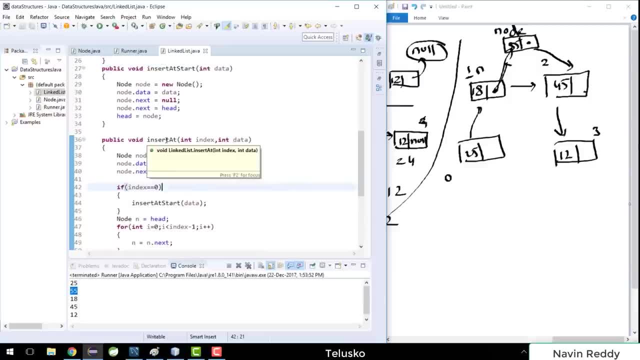 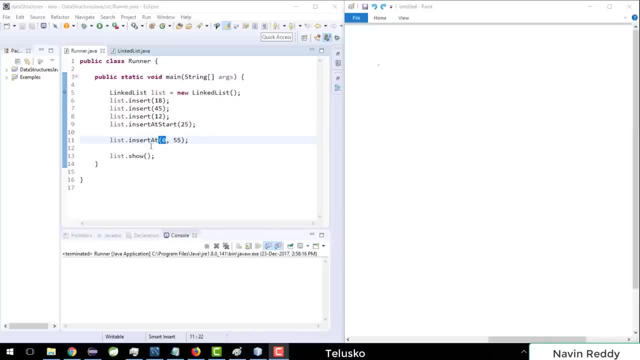 I hope you got the idea how to add at start and how to add at any location. so till this point we have seen how to insert data into list, how to insert data at the start of the list and then how to insert at specific index. so if you can see, we have. 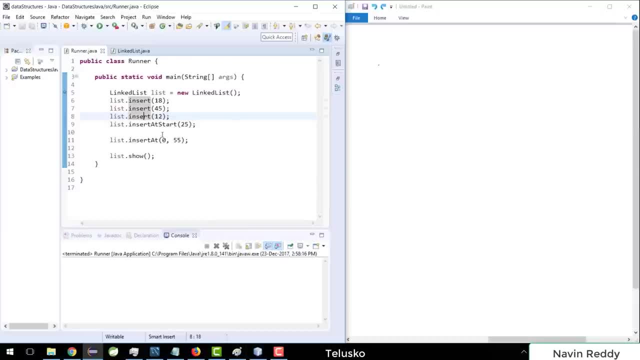 a value which is 18,, 45,, 12 and 25, and then we are also adding 5 or 55 at the start. so if I run this code, we should be having 5 elements right. but then I made a mistake. so if I run this code, you can see. 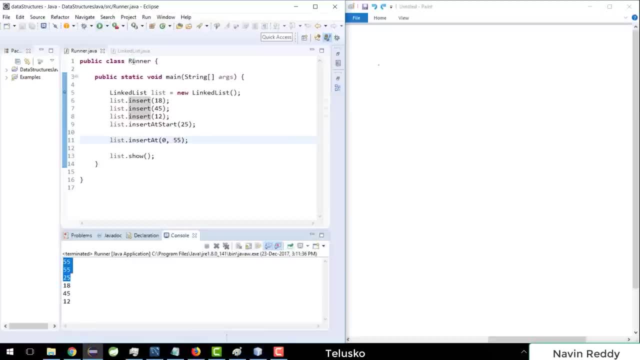 I made one mistake. I am getting this 55 two times. so what went wrong? if you can see the code here, we are saying, when you insert at the start, if the index value is 0, then you need to execute this code. that means we should not be executing the other. 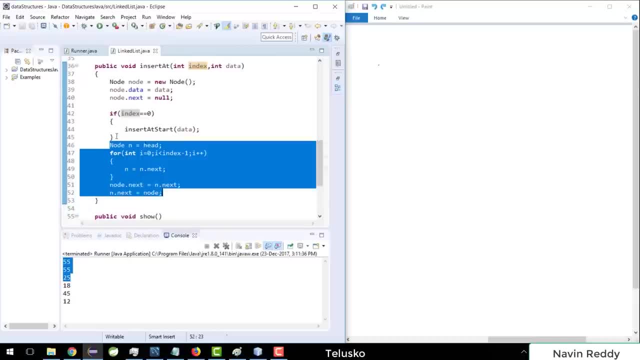 code as well, right, I mean, this thing is need to be skipped and we are not doing that and that's why you can see we are inserting 55 two times. so this code here should go into the else part which we missed in the last video. I will just put: 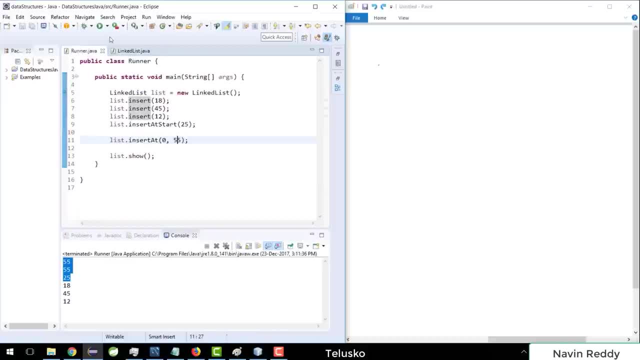 else block here, and after putting that else block, I will just go back to my runner and if I run this code now, you can see we got 55, only one. so yes, that was one mistake in the last video, so I just made some correction here, so there should be an else here. it's working now. 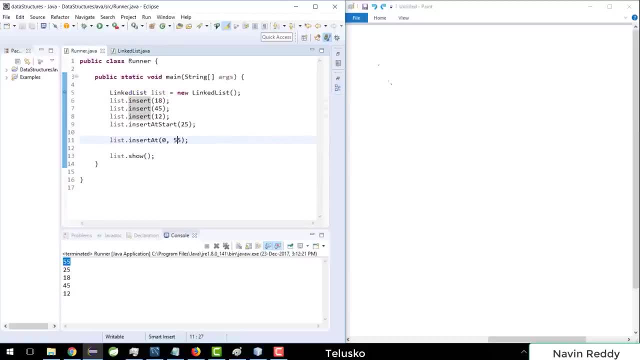 you can see we got 55. so just to draw here whatever we have done till now. so let's start with the first one. so what we are doing is with this line of code, we will create your first box here, and let me just write a box, which is 18. 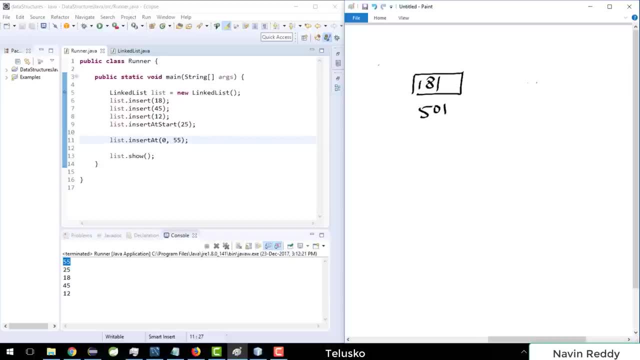 and let's give an address which is 501. that's my first address. let's have one more. so when you say 45, we got a second box. so when you add this list, you will get 45. here the value is 45. now let's say this is: 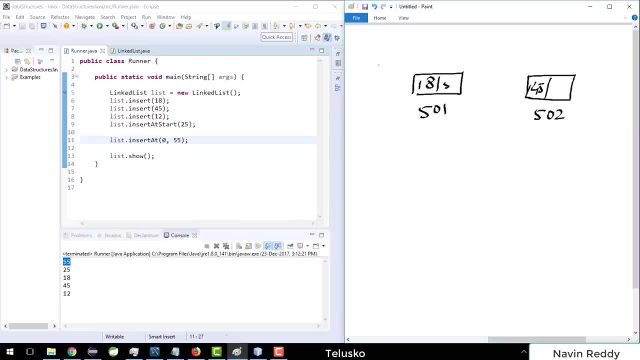 502. so of course this 18 here will have an address of 502, so it will link to this box. and then when we are saying, add 12, so we got one more box here which is 12, and let's say this has some address which, let's say, 503. so 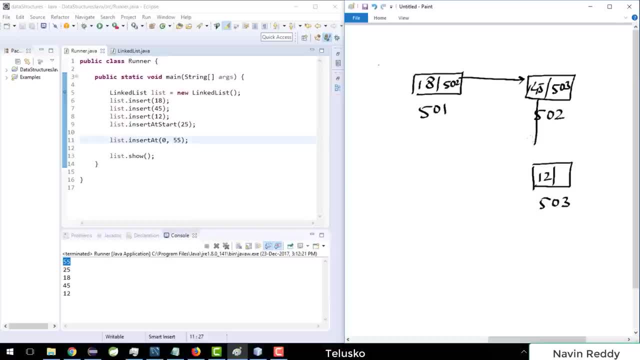 45 here will have 503 now, so we got this link here. we got one more which is 25, but 25 will go at start, so we got a new box here which is 25. initially we were having a head which was referring to 18 at the start of. 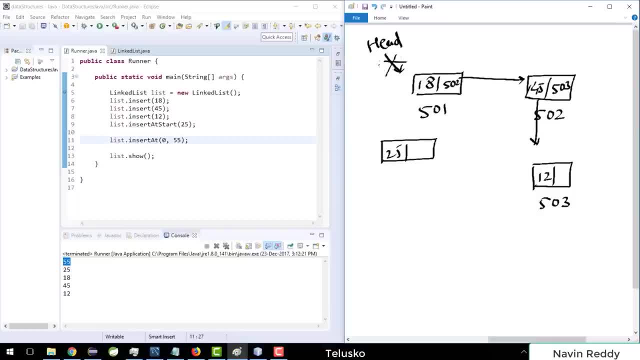 location. but now that head is not referring here. the head is referring to this new box 25, because we are saying start at the start, so this will have its own address, like 495. this is the address. it can go anywhere, it's not just when you. 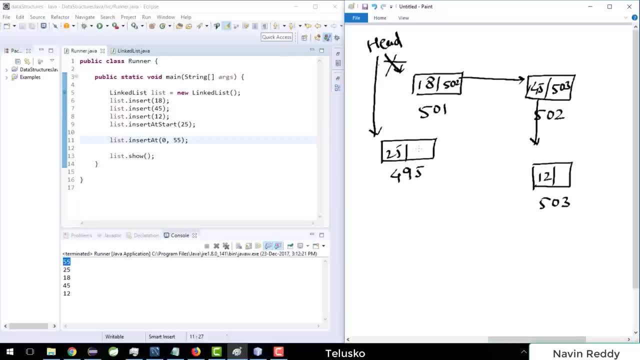 say it will add a start, it will have this value. it can have any value, maybe 595, maybe 695 or 795, it doesn't matter. now, here it will have 501, so this will refer to the next element. so the sequence is 25- 18. 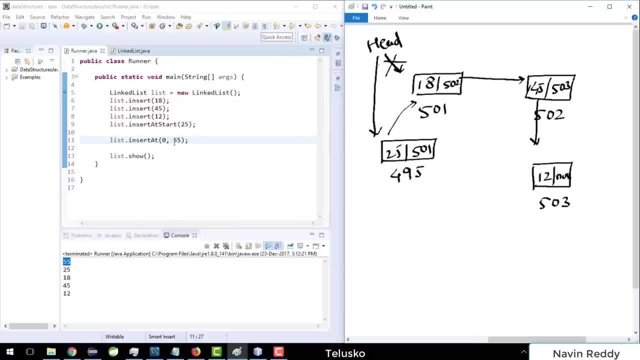 45 and 12 and of course 12 will have null, and then we have saying insert at 0 location. so we are adding one more element which is 55. so we got 55 which is going at and let's say, 55 has its own address. 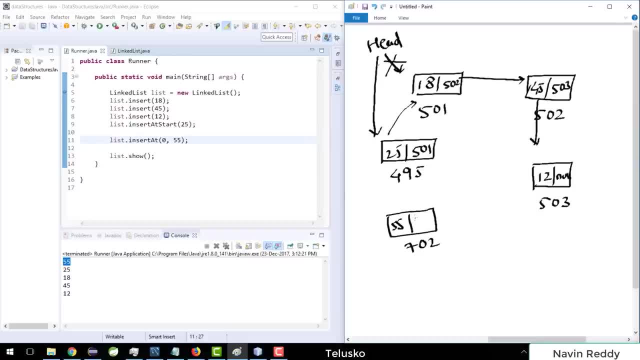 we will say this is 702, 55 will have 495, because the head value and then this will refer here. now head will not be referring to the 25. head will refer to this new location. so that's how you insert value in between or at the end. so we have seen all. 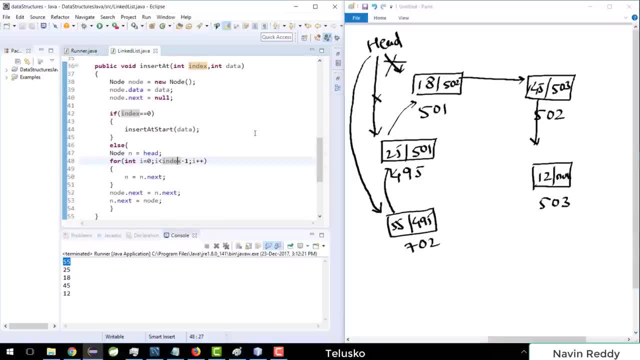 those stuff. the next thing which is remaining now is delete, right, so how do i perform delete operation? so let's say, i want to delete this 18 here, so i want to delete this 18 with index number 012, so i want to delete this index value. 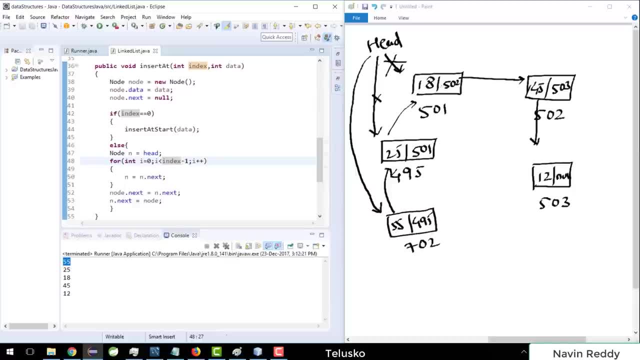 2. now how will you do that? so, when you want to delete this index value 2? so what we normally do is we just so? the only thing we have to do is just change this address. that's it. the only thing we have to change is change this. 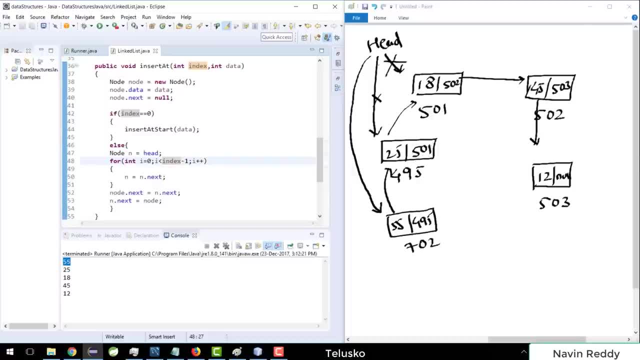 address. so here, instead of having 501, we can. we need to change this to 502. our job will be done right. so when you say this is 502, it will refer to the next node and will not be using this node anymore. so this is gone. 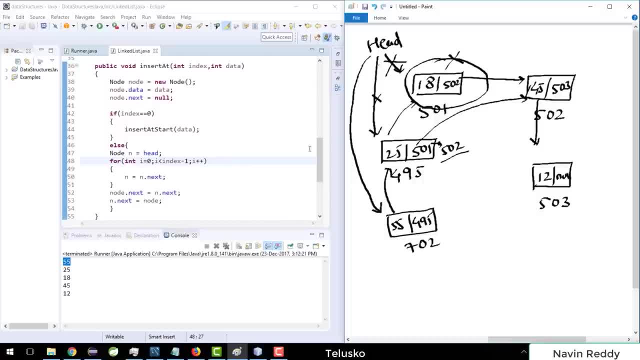 okay, now how do we execute that? so let's go back to our linked list and let's add one more method, which is delete. so before show here, i would say delete, public void, delete. and this will take a index value. so i would say index, int, index. 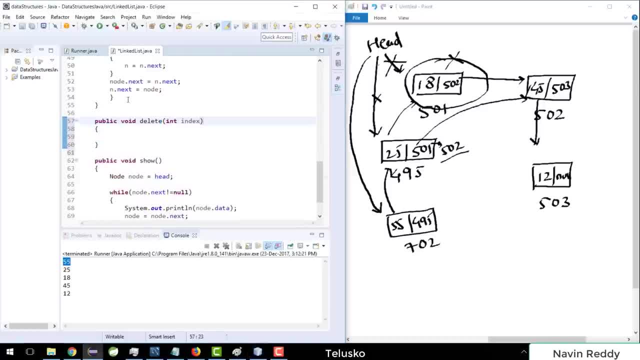 now, technically, the name should be delete at right. so it should be delete at, because we are specifying the index value. okay, now we have a special scenario here. what if you want to delete the first index? so if you want to delete this one, which is the first index here, 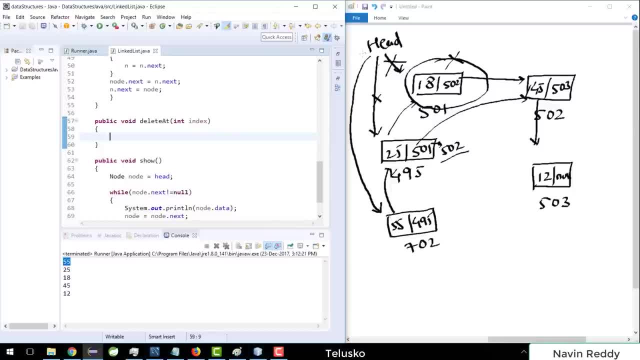 now, in that case, you just need to change one thing. you need to change your head location with this one. that's the only thing you do right. and how do we achieve that? so we say: if my index value is equal to zero, in that case i will change my head location. 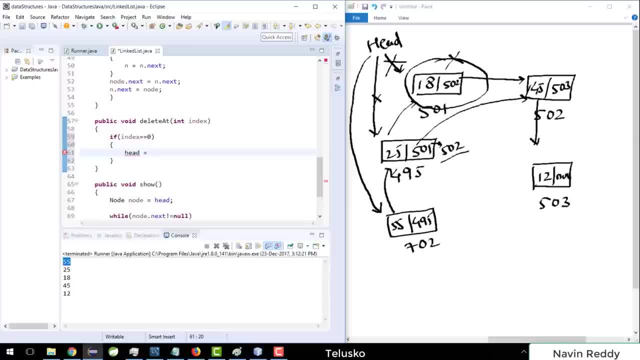 so the head location will change to the next node. and what is next node? it is referred with the head node dot next. so i would say head dot next. so head will become head dot next, and that's it. this is what you do when you want to delete the first element. 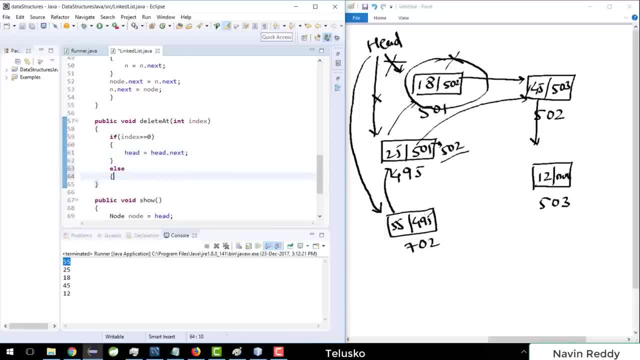 is that simple? but what if it's not a first element? so we'll go for else part again. and here we have to traverse. remember we, when you want to traverse, you have to do something. if you want to traverse, remember this- we were using a for loop or a while loop. 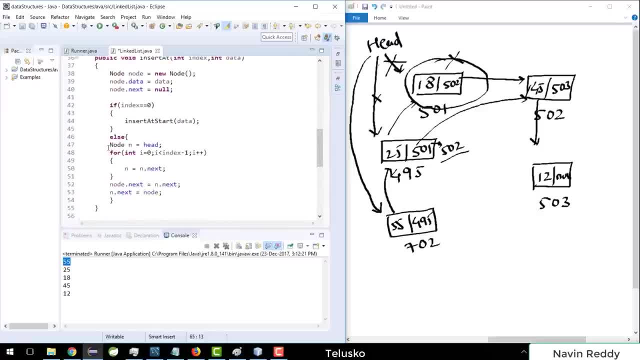 we will go for for loop because we are using index value, right? so remember this code here: the same thing from here to here. everything remains same. we have to traverse to that location, so let's go there, i will say copy and we can just reuse the code here. so 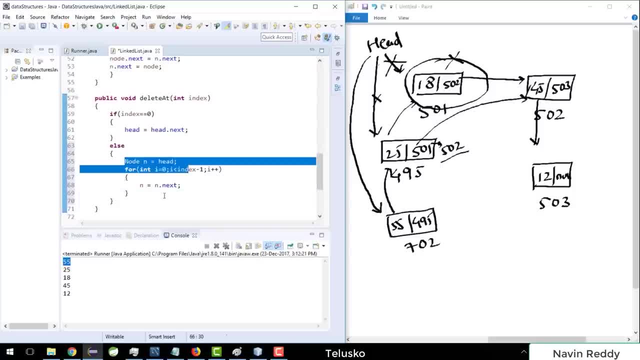 we are traversing right, so from from the head node we are traversing to that location. now, once you reach to that location, so now when you pass a value two here, so the index value when is two. so this loop will run only once right, because the index value is two, so two minus one. 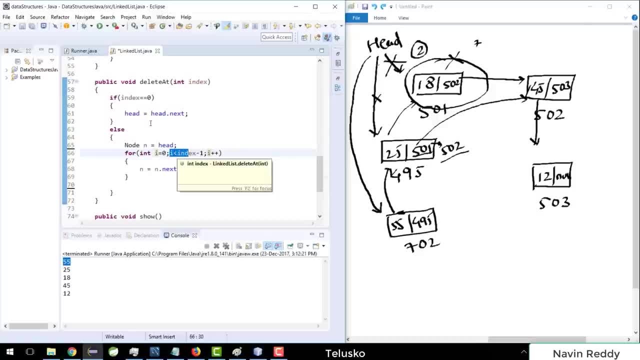 is one, and we are going till i less than one, which is zero itself. so this loop will iterate only once. that means the current end value which we are representing after the loop would be this end. so this one will be your n. so n is one now i. 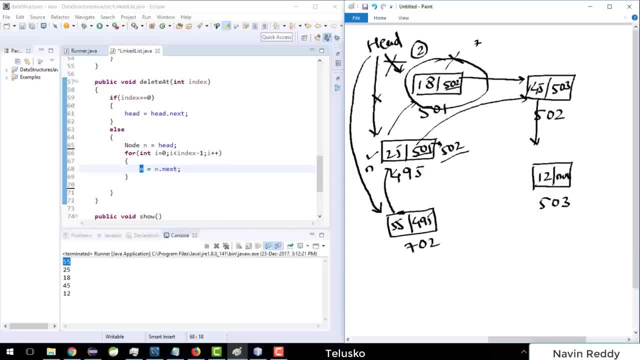 want this value, which is five zero two, because, so that, if i know this, five zero two- you can assign that value in this box, and the way you do that is by using this node in some temporary variable. so i will say that there is n one. so when i say n one, 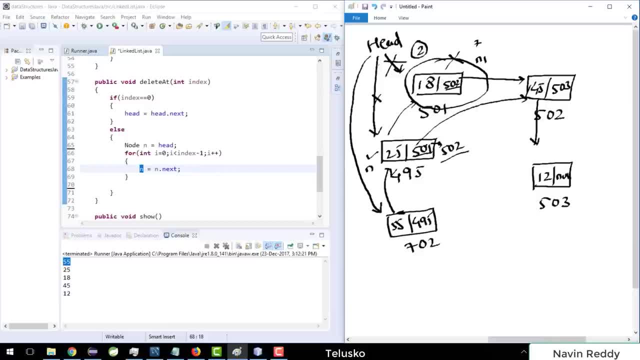 now i am representing this object and when i say n, i am representing this object or this node. so i would say, first of all, i want to assign n. one is equal to n dot. next, that's how you will get this reference. so if you want to, 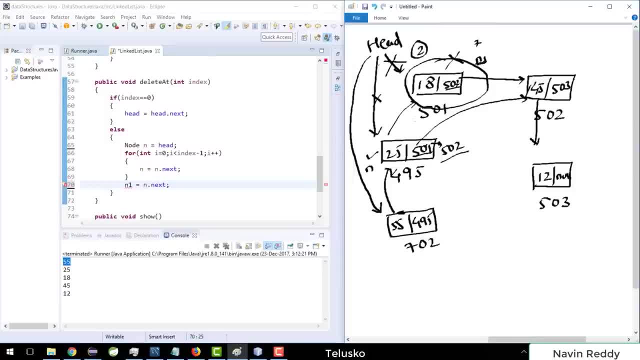 use this object here. if you want to make it n one, you have to say n dot next, because n dot next is n one, right, oh, but we don't have n one anymore, so we will say node n. i mean, node n one is equal to null, so that we can refer that. 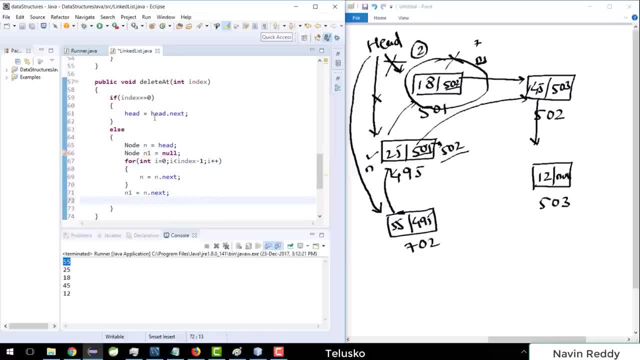 so we have to declare that object first. now, once i got n and n one, the only thing which you have to do now is the n object. so when i say n dot next, so the n dot next need to be replaced by n, one dot next, and it's very. 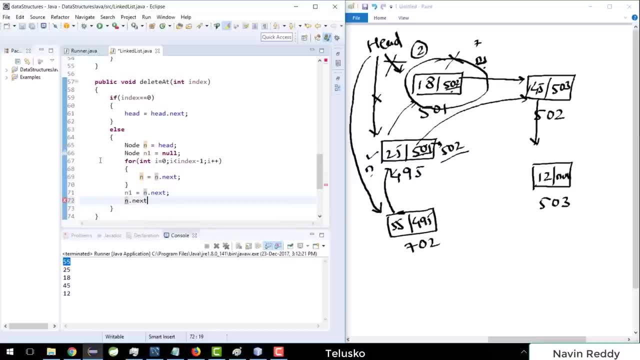 simple now. you can simply say: n dot next is equal to n, one dot next. okay. and then, once you got the value, you can simply say: system dot out dot println and you can print the value if you want. so just to verify if everything is working properly. you can delete the element which: 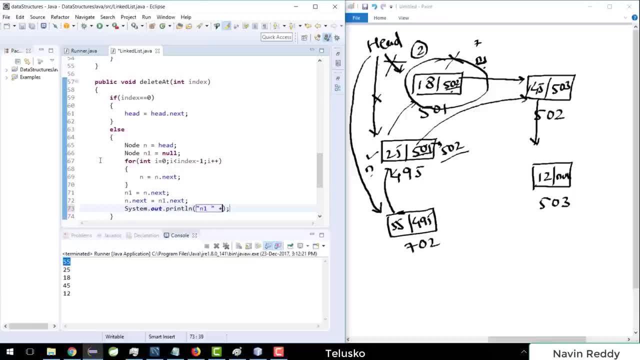 you want to delete. so i will say: i want to delete n one, because that's what we are doing. we want to delete n one, right? so we will say n one, and let's print the value of n one, which is n one dot data, so we will know at least which one is getting. 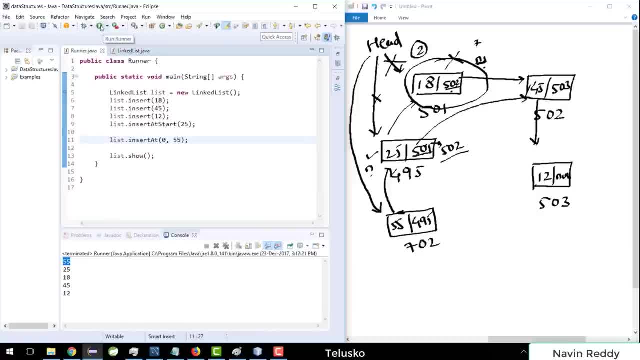 deleted. now how to verify this. let's go back to our runner and let's delete a value after some time, so it's at least dot delete. i want to delete the element at index number two, which is eighteen in this case. let's run this code and you can see after running. 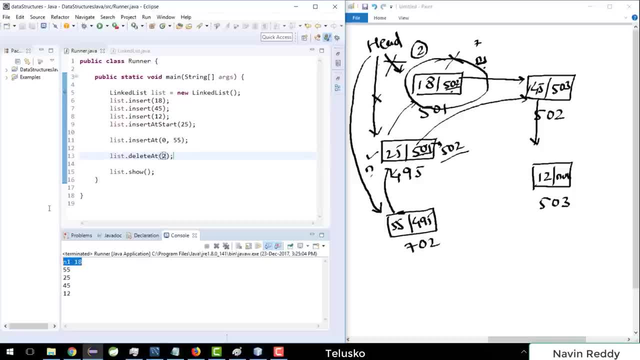 we don't have eighteen anymore in the list. yeah, this is getting printed in the delete method itself. if i don't print something here, even it will not print eighteen there. so, yes, we can delete the value just by using delete method. so we have delete at. it will be used to delete the. 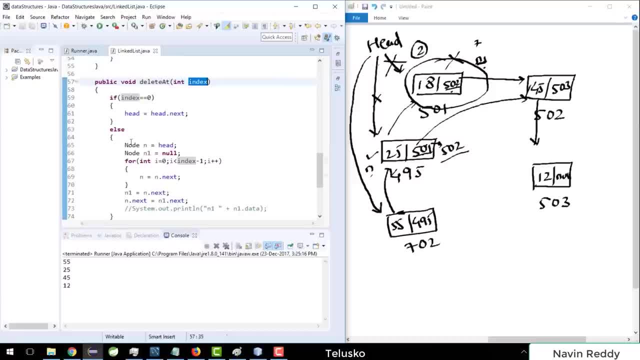 value at the particular index. so that is awesome. this is how you delete the element. the only thing we did here is we just changed the reference right. so this element address is changed by the new one, which is 502, not 501 in this case, and that's it. this is how you. 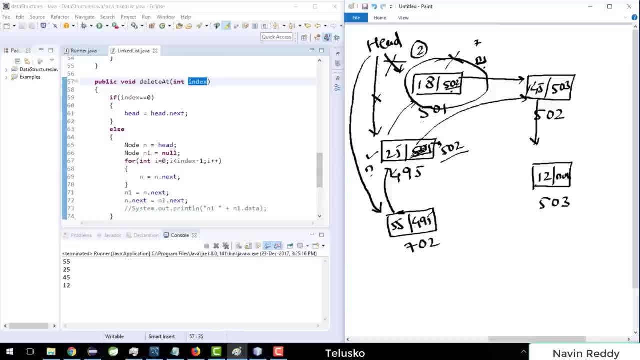 break the links. okay, there is one problem. this object is still there. it is deleted from the list, but it's still there. if you want to nullify it, you can do that. you can simply say n1 equal to null, so that it will be eligible for garbage collection. 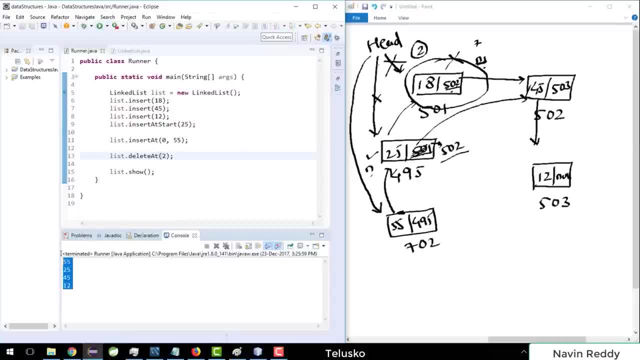 right. so if i run this code now, you can see we have removed eighteen and it is not there in the memory as well. it is eligible for garbage collection, so that's how you can delete this data. in this video, we will talk about stack now. what stack? 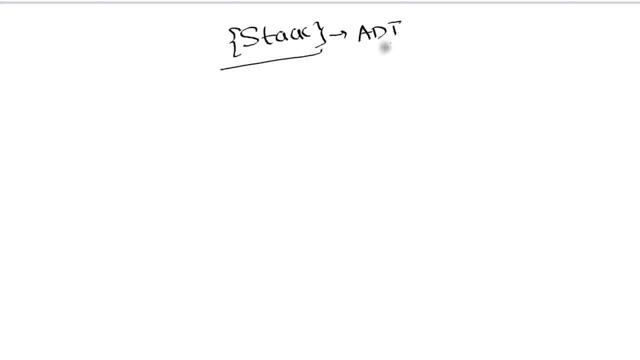 means now? stack is basically an ADT in data structures and, as you know, ADT stands for abstract data type. so when you talk about abstract data type, we only focus on the features it provides, but not the implementation. now, in stack, it provides you multiple features. when i say features, 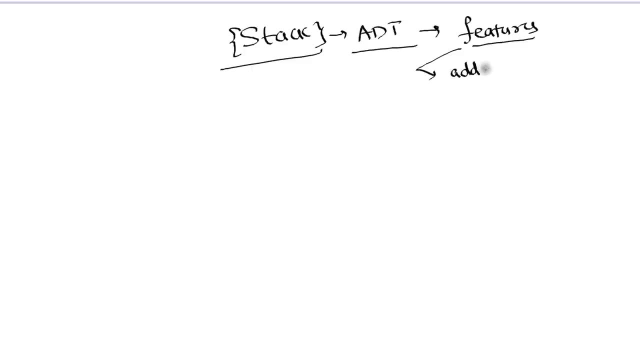 we have a list of features like we can add element and normally when you want to add element we use a term called push. you can delete the element using pop. so you can do that with the help of pop or you can. you can not say delete, but you can take out the element. 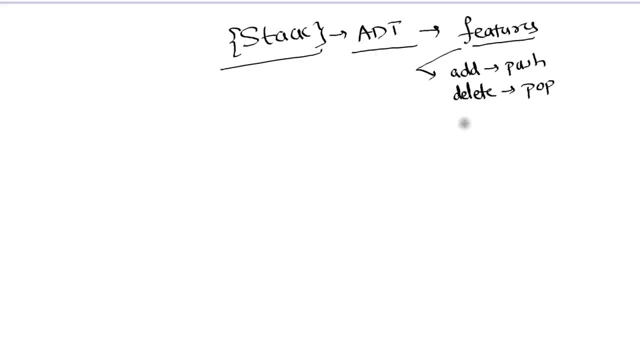 from the stack and then you can also look for the element. so you can find an element, the first element, and then you can do that with the help of pick- again, you will understand this in detail later- so we can apply a push operation, we can say pop and we can. 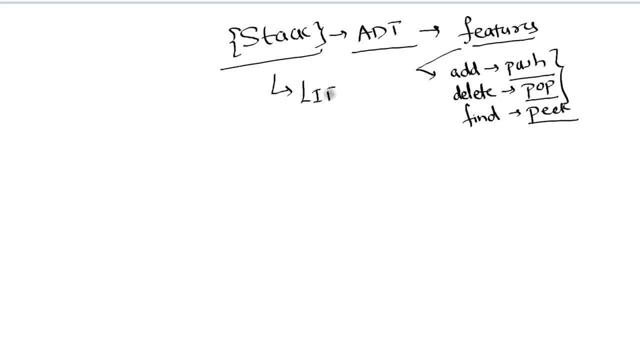 say pick stack. it supports a feature called as leave for, which is last in first out, which simply means whatever element you have inserted last, you can access that first. so leave for stands for last in first out. so whatever element you have added last, you can access that first. to explain: 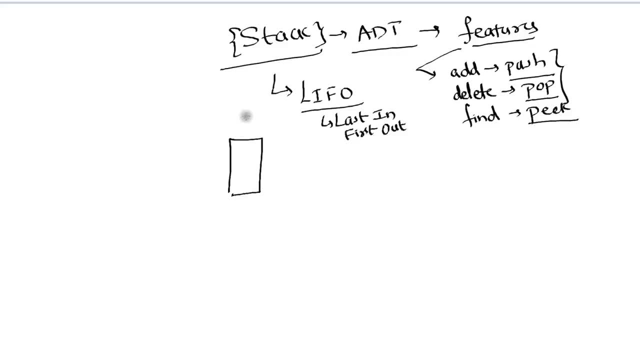 this. we will be having a stack here, so the last element you have inserted is the first you can take out and in stack you have only one entry point. so you have only one entry and exit point. that means this is the only entry and this is the only exit. so this: 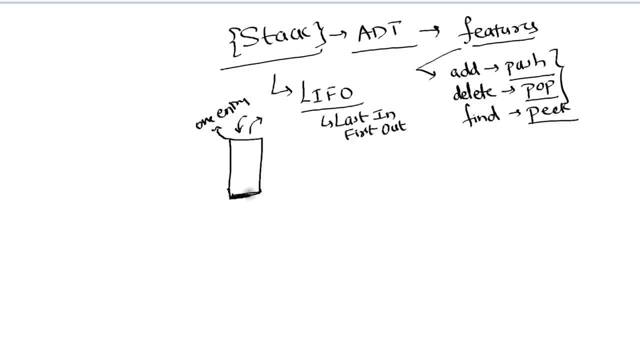 one will remain closed. you can apply a lock here, so this one will remain closed. the only place where you can enter the values is from one point from here, and you can take it out. so whatever element you have inserted last, you can access that first. but do we use this in real world? 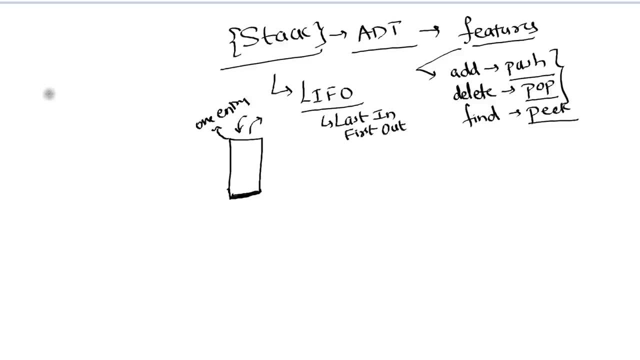 and the answer is yes. example: let's say: if you are working on a task. so let's say: if you are working on a project, it's a very big project, maybe that project is, let's say, A and that project will, maybe will take 6 days. 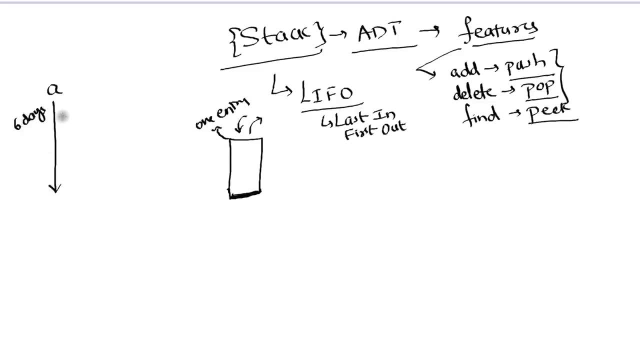 so it will take 6 days to complete this project and suddenly the old project or the old version which is already deployed on the server, it is giving you an error. now let's say you got a bug. now, at that point, what do you think? will you complete the entire A project? 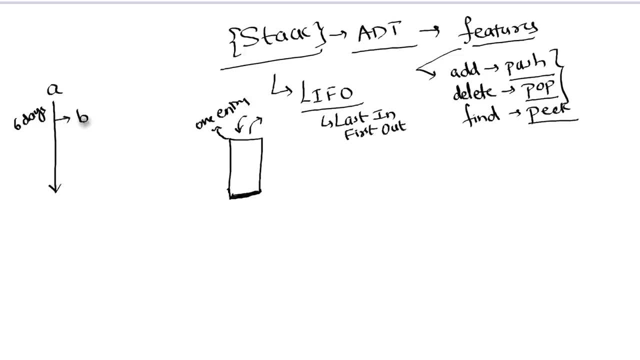 and then you will think about the bug, or you will try to fix the bug first, and of course a bug is something which a user is facing nowadays. so of course you have to fix the bug first and then you have to think about the earlier task. so in this scenario you will 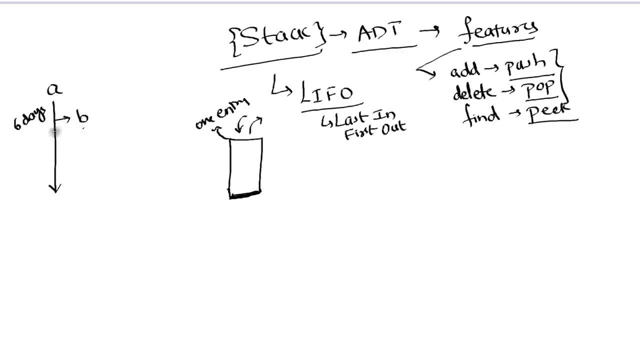 try to fix this bug. that means you are keeping your job A aside and you are focusing on B now. so you started working on B and you thought, okay, in next 3 to 4 hours I will complete this B, I will fix this bug. so you are keeping this task. 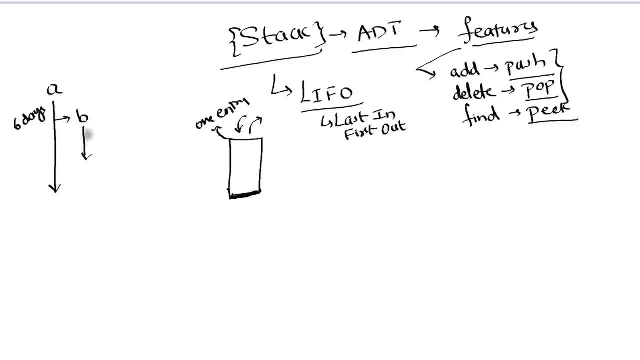 A aside and you are working on B now, and certainly that this is your lunch time now, so you are going for lunch, so let's say it is 1pm and then you want to have your lunch. you are going for the lunch now, so let's say that is. 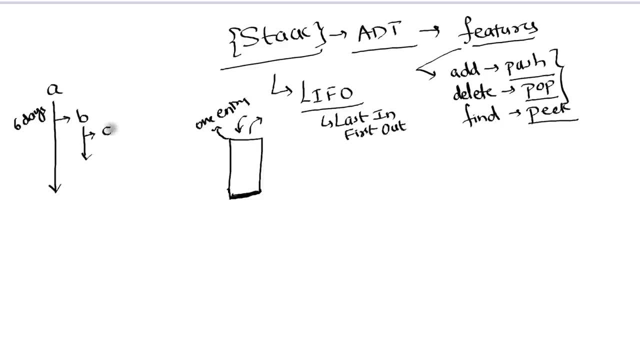 task C. so task C is your lunch time, and now you are having your lunch. so while you are having your lunch, of course you will not be working on B at the same time, because when you are having a lunch, you should do only one thing at a time. you should have your lunch. so when you are 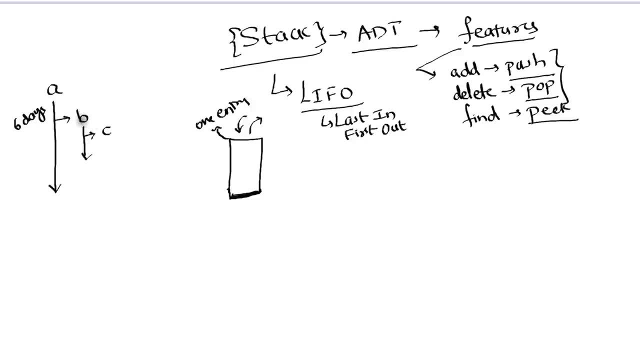 doing your lunch, you will not be working on B. that means you have kept B aside. now, once you complete your lunch, what do you think which is the first task you will resume, A or B? it's B, right, because this is the last task you have left. so when you say B, 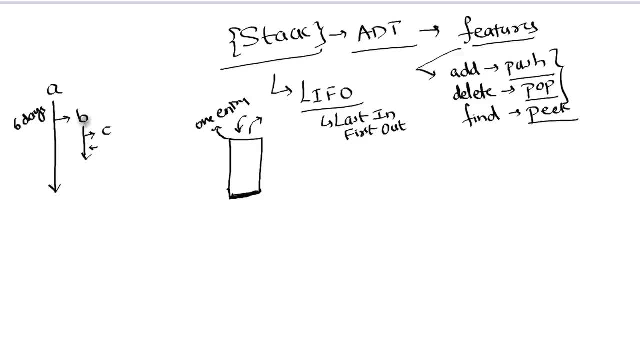 this is what you left last, so last in, first out. this is what you will resume, and once you complete B, then you will resume with your A. that is last in, first out. so the last task which you are working is the first thing you will resume. now do we use? 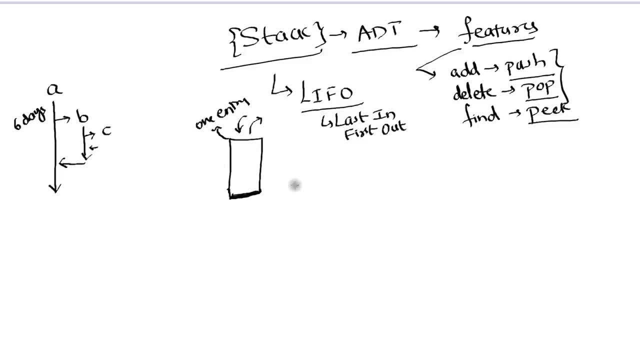 this in some other concept? yes, example, if you have a stack of books, so whenever you have a stack of books, what you do is the first book. so you will keep the first book here, then second book, then third book and then fourth book. so once you keep, 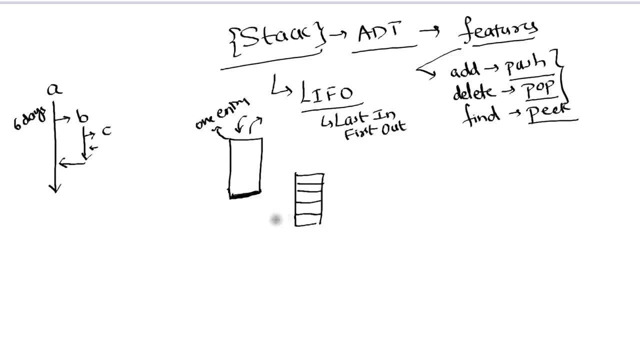 all this book once above other. the first book you are going to access is the last book you have kept here, right? so this is how your so. let's say, if you have kept one more book here, then this is the last book you can access. first, this is the book you can access. 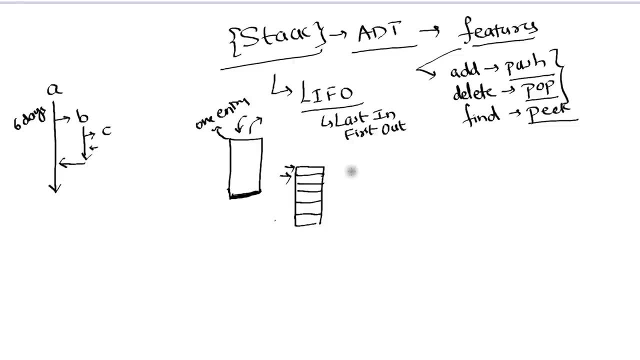 first, what about virtual world? so in virtual world as well, you know, when you talk about recent applications. so in windows we say alt tab. so when you say alt tab, it will show all the applications which you are working with. so when I say alt tab here, you can see. this is the first application. 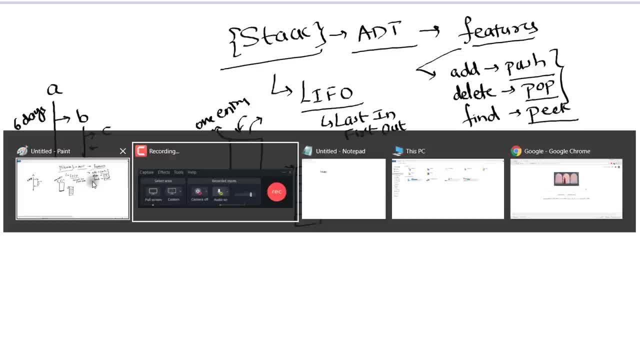 this is the last access application, so you can see that first, which is paint, then I got this recording software, which I have opened second last, and then I was working on a notepad- that's the third in the list- and before that I have opened my computer and before that I went to google. 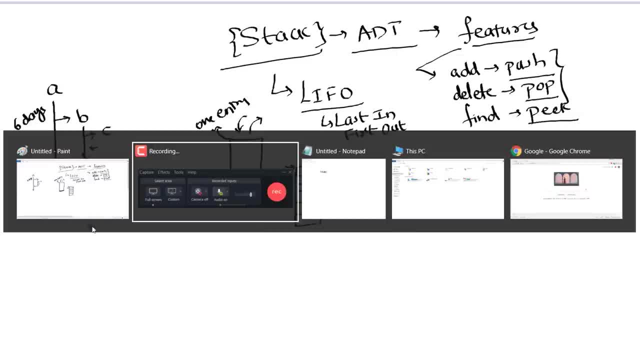 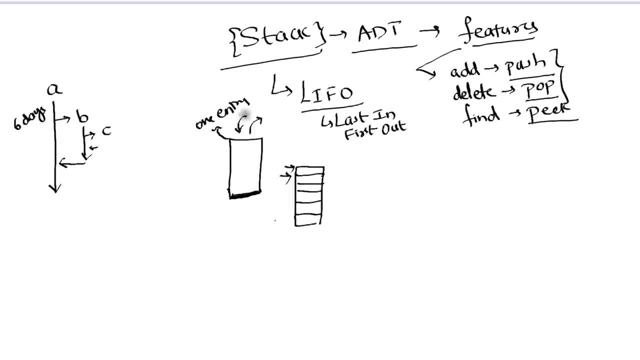 or chrome. so this is the, this is the stack, right? so the last access element is coming at first here. so yes, we use stack a lot of time in real world and in virtual world as well. so let's try to understand how do we work with elements. so let's say: 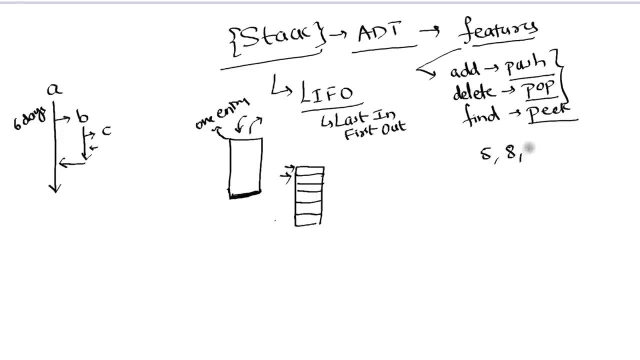 I want to store this 4 elements here. we got 5, we got 8, we got 3 and we got 2, so I want to insert this values in a stack. so what we do is we create a stack here and again if you want to insert the value. 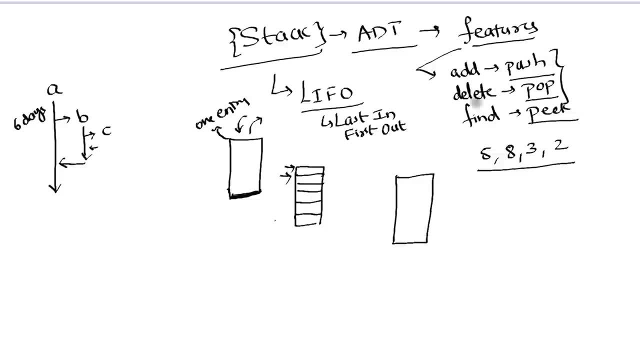 we will use push. so using push, you can insert the value. using pop, you can get the value, the last value, and using find, if you don't want to delete the value from the stack, you just want to see the value, you can use. peek question is: how do we? 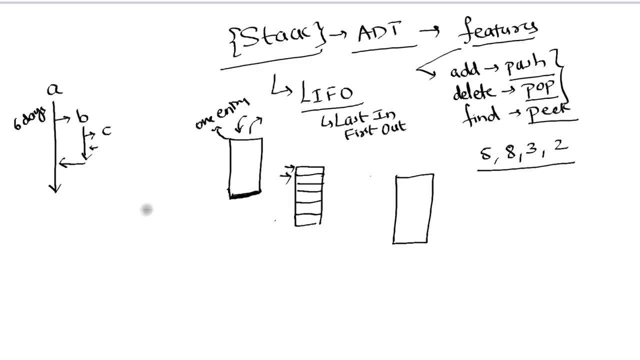 implement this. in fact, you will be seeing the implementation later. but then there are multiple ways of implementing this. we have the array way, so you can implement that with the help of array. in fact, in array as well, we can go for fixed length array, then we can go for dynamic length array. 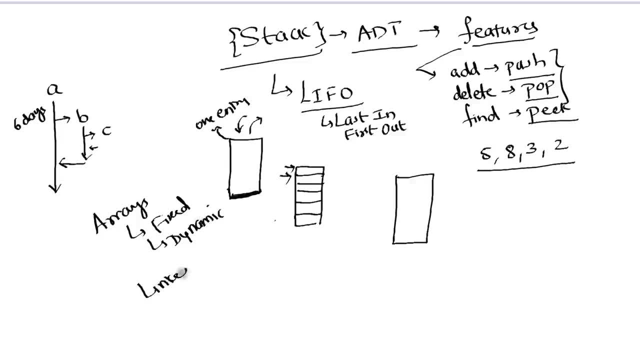 or then we can also go for link list, so we have different implementation. so we can go with the array implementation using fixed or dynamic length, we can go for link list. but doesn't matter what you go for. let's say, if you talk about array, so let's say, if I create an array of 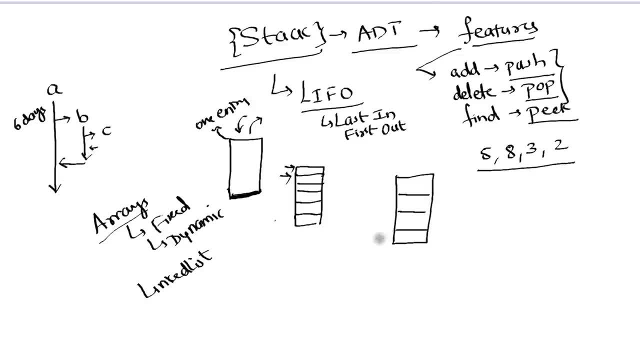 4 elements here, right? so we got an array of 4 elements, and this is: index value 0, index value 1, index value 2, index value 3. now how will you insert the value? so this is the only entry point and this is the only exit. 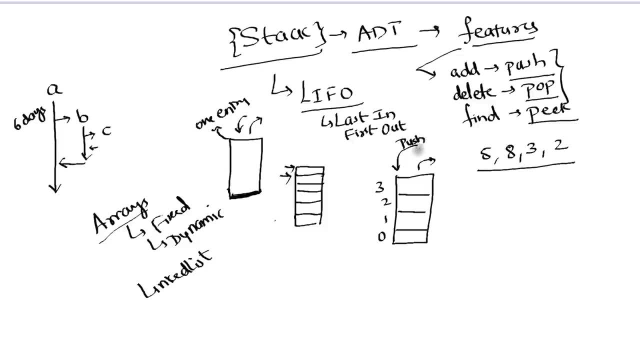 point right? so if you want to enter the values, you will be using a method called as push or a function called as push. in this push you will pass the value. so whatever you want to pass, let's say, if I say i, i will represent 5 or 8 or 3 or 2. 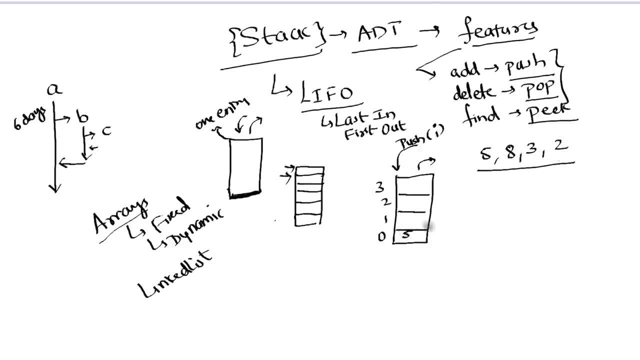 whatever you pass. so once you pass a value here, that value will be assigned to 0. so let's say, we got 5 here. then when you say 8, 8 will be assigned here. now, once you inserted this 2 value, or maybe let's say, add 3 as well, so we got. 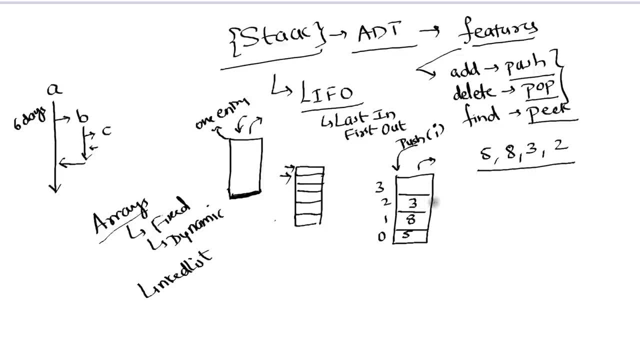 3 here now, which is the last element you can access. so if you have entered 3, this is, but how do you know which is the last element? so you can simply use a variable called as top. now top will have the. top will have an index value of the. 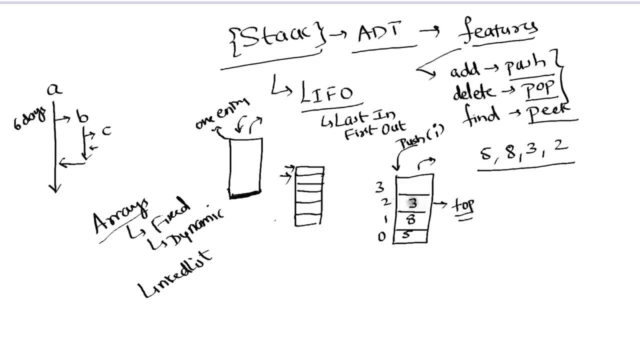 element, so index value 2. we have element 3. this is the top element and when you insert 2 now it will the 2 will go here. simple, right now. how about if I say pop, so when you say push everything going in, this tag will say 5, 8. 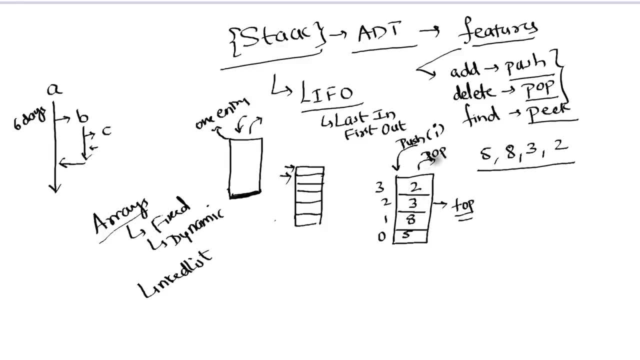 3, 2, so the value will go down and then, when you say pop, it will remove the first element, because when you say you have inserted 2, this is where you are representing your top right, this is the top most element. so this is the element which. 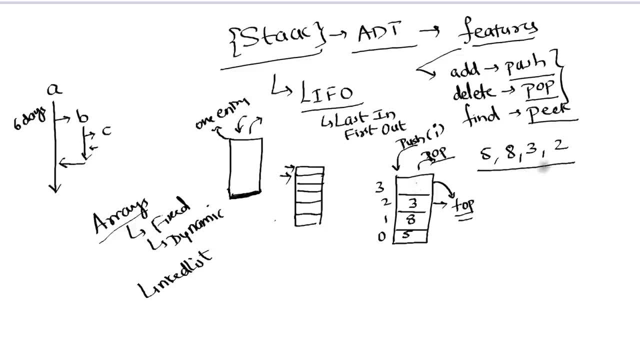 will remove first. so when you say pop, it will remove, it will remove this 2 and let's say after that: if you're inserting 12, so let's say after that. but after saying pop, you're inserting 12, so 12 will come here, because that's the last. 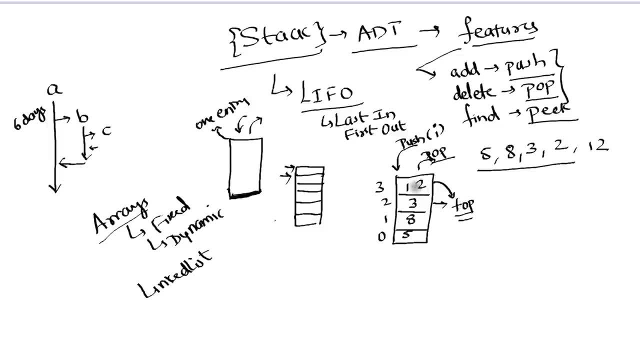 element you can access. so, again, that will go back to 2. yeah, when you delete this element 2 before it will go back to 3, okay, the top variable will go back to the index number 2, which is 3 in this case. so this is how you, you push and. 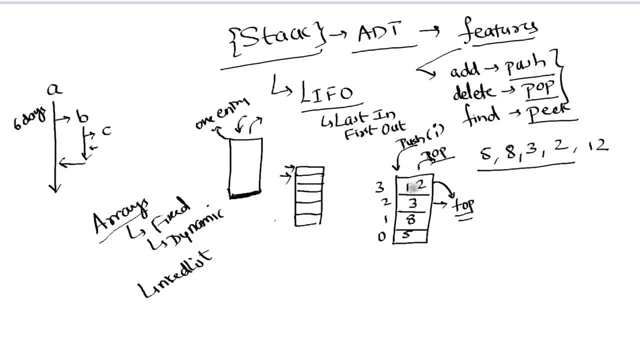 you pop, so the last element which is added is the first thing you can. you have an access, so when you say pop, it will delete the element. it will give you the element and to delete the element from the stack. but what if you don't want to delete the element you can? 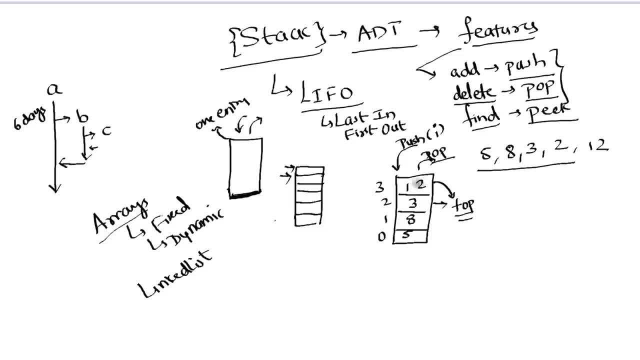 simply use find and use to use find. we normally use a function name as peak, so when you say peak at this point it will give you 12. pretty cool right now, let's say, once you have inserted all these values in the, in the stack and the stack. 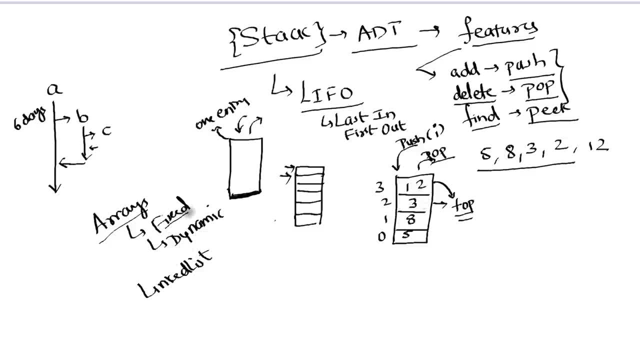 is full right, because the size of the stack is the same as the size of the element. so let's say I want to use lengthless, but let's say if I'm using a fixed length array, so if you're using a fixed length array here and if you have, 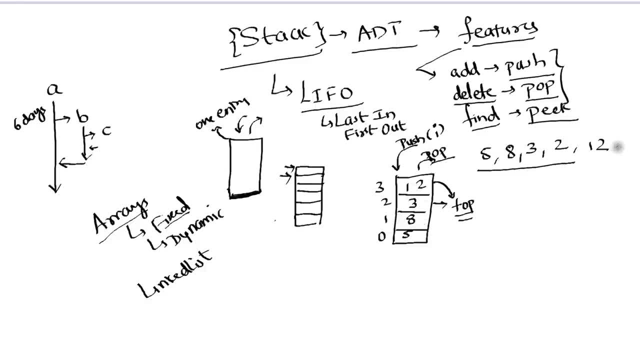 increased if you have crossed the limit of your stack, which is 4 in this case, if I try to add one more element. so at the end here, if I try to add an element which is one now the moment you say one, if you, if you try to add one, it will. 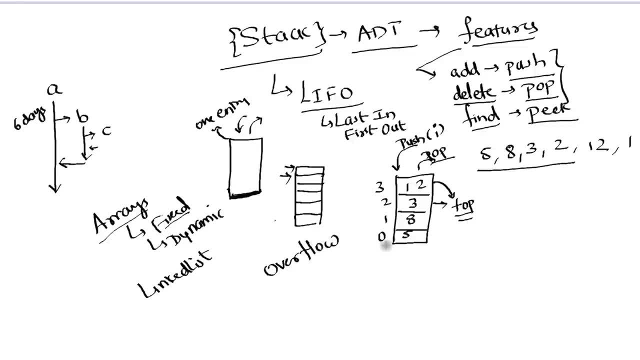 give you an error and that error is overflow error, because you are trying to overflow the stack. that's one, one, one case. so if you try to push the value and the size is full, it will give you overflow error. what if you try to delete the element, if you try to pop and 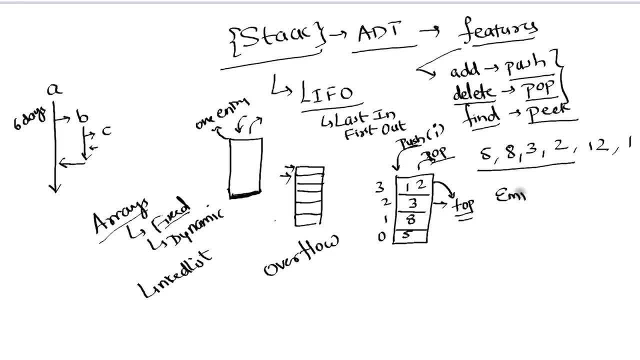 your. your stack is empty, let's say if you don't have any element here. so if a stack is empty and if you try to fetch value at this point, it will give you another error. so if your stack is empty and you're trying to pop, it will give. 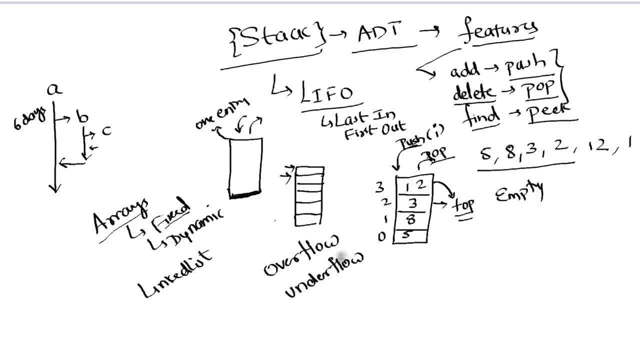 you error, which is underflow error. so underflow is when you, when you don't have the value, and try to pop the value from it. so that's how you have overflow and underflow concept. those are errors, basically, and there's one more thing that you need to keep in mind. 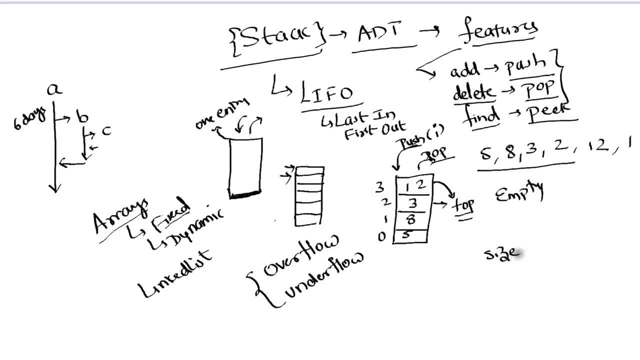 when you're trying to pop and peek. we can use some other methods as well or functions as well. example, we can get the size of the size of the stack using size method. you can also check if the stack is empty with the help of ease empty function. so again, you can. 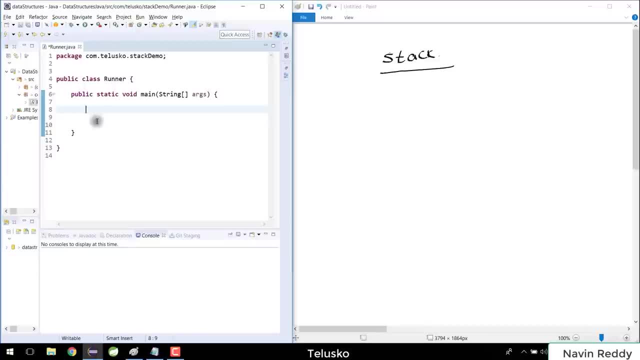 implement whatever methods you want, but these are the basic ones for stack and in this video we'll talk about the stack implementation using java. now, when you say a stack, basically stack is a class inside java. so if i simply say control space, it belongs to a packet javautil. 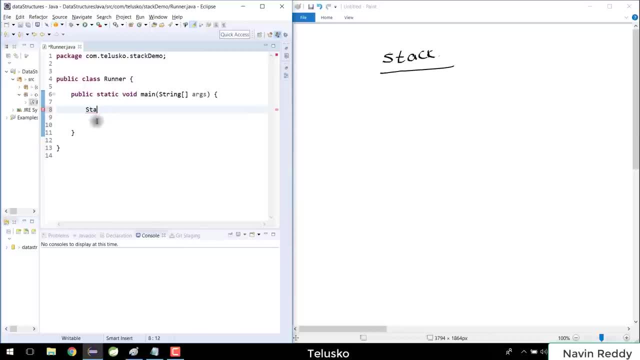 all the features of a stack here, but then why to use a inbuilt class when you can create your own? so i don't want to use the stack class which is inbuilt, i want to get my own class. so what i will do, i will right click here on the 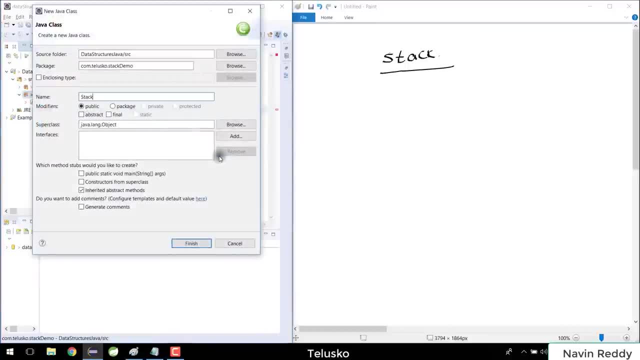 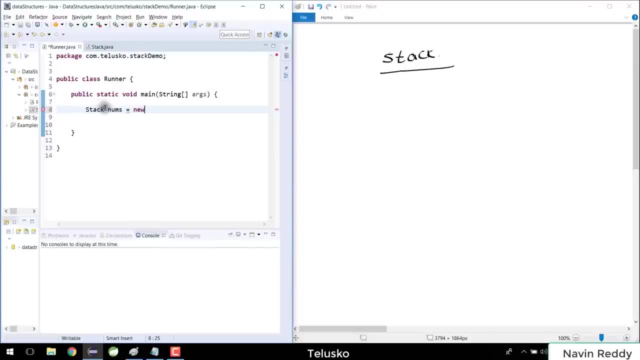 package, i would say new, and i want to create my own class and that class name is called a stack. so i have my own class here and here i will create object of stack. i would say stack nums equal to new stack. now, in this stack object, or the nums, 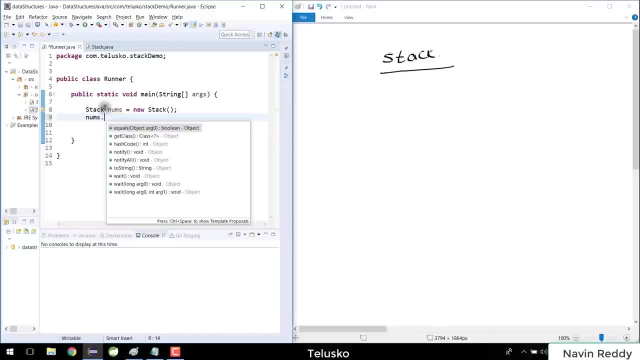 object. i want to perform certain operations. so when i say nums, dot, push, i want to push the element. i can specify any value here. if i say 15, so the first element should be 15, and then again i can push multiple elements and then i maybe i want to pop. 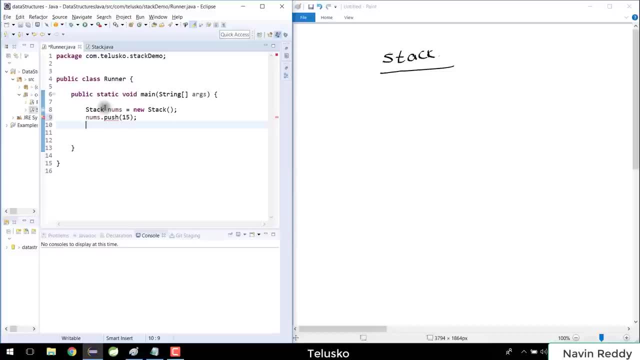 element which is taking out the element from the stack, or maybe i want to fetch element. so when i say stack, basically it has certain features. right, as we discussed in the theory session, we can use push, we can use pop on, we can use pip, so we'll be using, we'll be working. 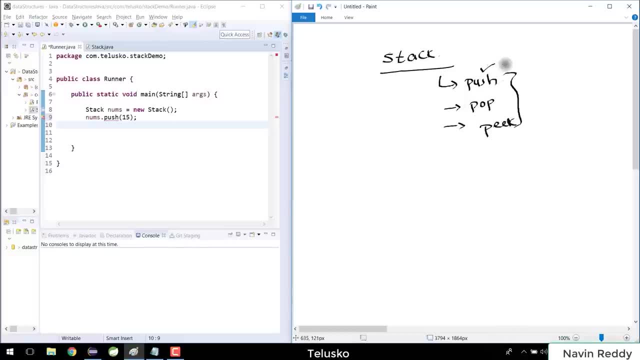 on these methods. so let's start with the first one, which is push. so in in the- if you can see, in our stack, we don't have any method yet, so let's create certain methods. so the first method is push. now to implement, push what i will. 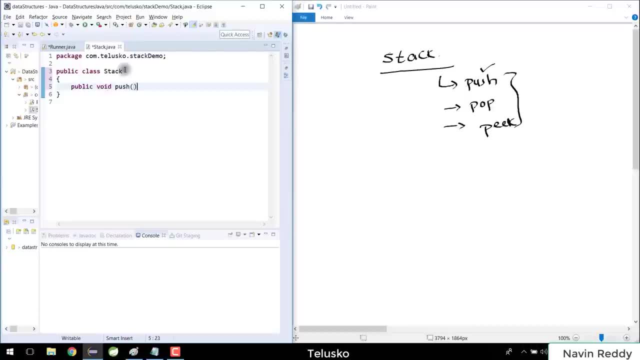 do is i will say: public void: push now, since we are adding the value, we are not expecting any value. so let's say push data, so we have to send a data and it will add data there. so now you can see if i go back. now you can push the. 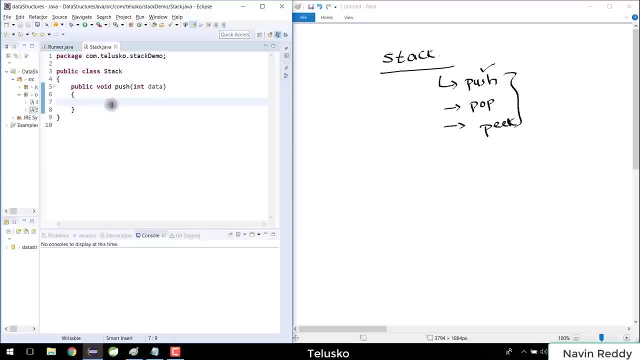 element and there is no error. but then what you will do with the push to make it work. first of all, we need to create an array, right? so we have to create an array and we have to also specify the size of the array. so let's say, if i say 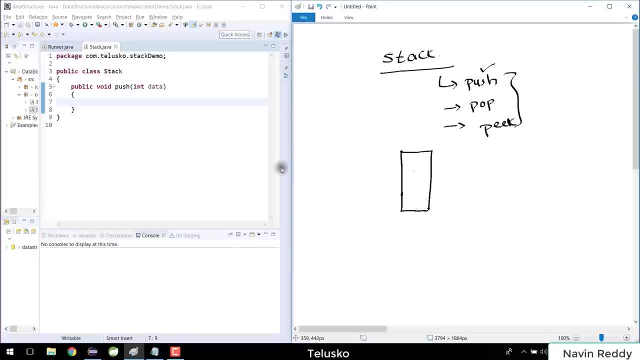 we have an array here and initially we'll take an array of five elements so that if you can work on five elements, you can work with a number of elements. so let's say, if i have the first one, then the second one, then third one, and fourth and fifth. so we have this five. 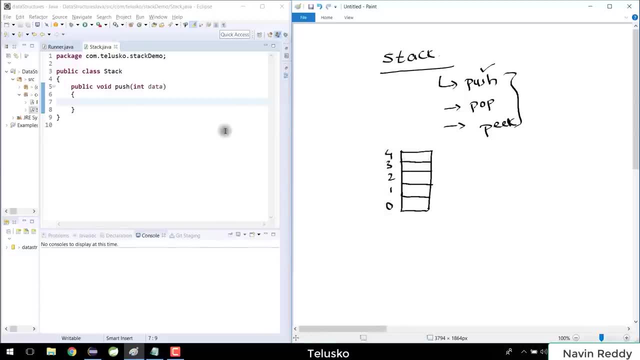 elements. here index number will be zero, one, two, three and four. now, if you want to add the first element, as we are doing it here, we are passing 15 right so that 15 will go to the- uh, go to element zero. so somewhere here we'll be having that. 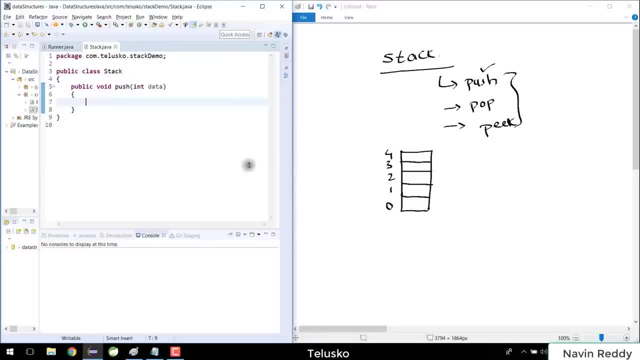 15, but then we don't have array yet. so even before you push the element, you need to create that array. so let's do that. i would say int and we'll say stack equal to or stack. it's an array, basically. so we'll say stack equal to. 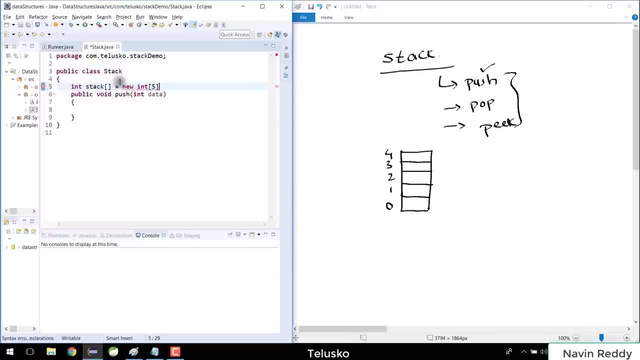 new int and the size of int is five. you can make it dynamic, you can. you can take the input from the user what array size you want, but time will, let's specify by by ourselves. so we are, we have created the array and now we can push the. 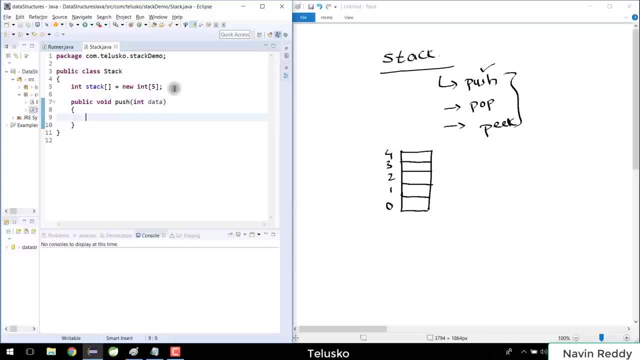 element, but kosher is where. so we'll say, okay, you have. when you say push, you will assign the value to the address location: zero, okay. so that makes sense. we can simply say zero, right here. right, so we can say stack of zero and you can assign the value whatever, whatever data. 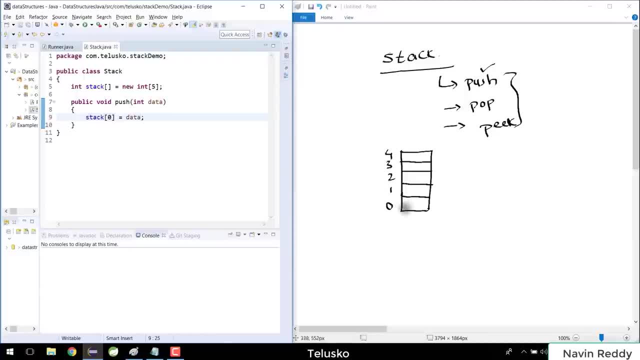 is coming. it's so easy, you can. that value, which is 15, will be assigned to the index value, zero. it is that simple. but here's a twist. the twist is what if i, if i want to add one more element, so if i say nums, so if i push another? 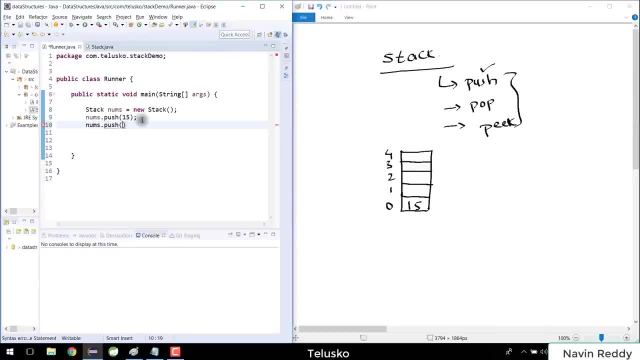 element. here we'll say: let's, i want to pass maybe eight. now we are passing two elements. right, we got, we got 15 and we got eight. now what will happen is the moment you pass eight here, the eight will be the value. eight will be assigned. 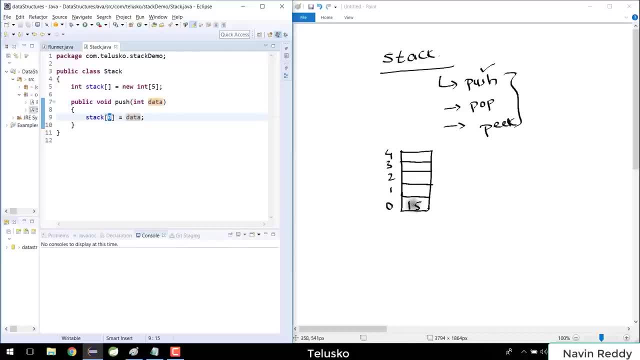 to zero again with the zeroth location. that's not what we want, because if you, if you, if you're on this code, the value 15 will will be replaced by eight. we don't want that. i want to assign value to one. that means we need to count it. 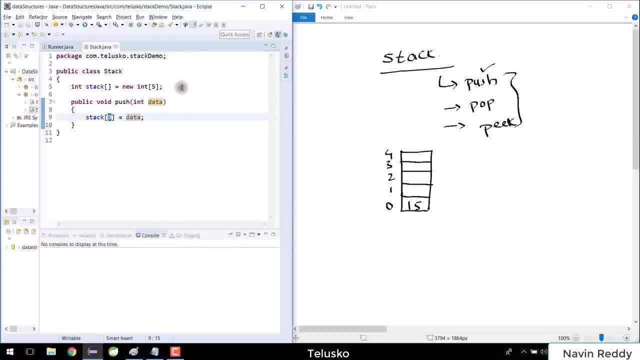 we have to use? we need to use a variable which will count the number, and maybe i will use a variable here which is called as top, and the initial value of top would be, let's say, zero. we can simply specify top here, right? so instead of using zero, we can say top. okay now. 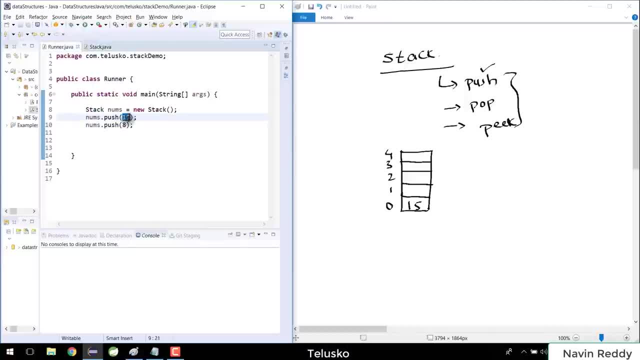 when the first element getting inserted. so when you insert 15, that 15 will be inserted here at this, at the top location zero, right? so we got 15 here. now if i send eight- oh, eight is also the value of top is still zero. so that's. 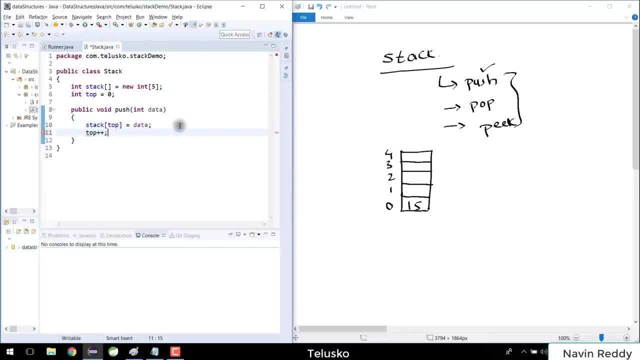 what we want to do. so that means, after doing this thing we have to. you have to simply say plus, plus. so every time you push an element you just need to increment the value of top, so that when you pass eight now, eight will be assigned to index value one, because when 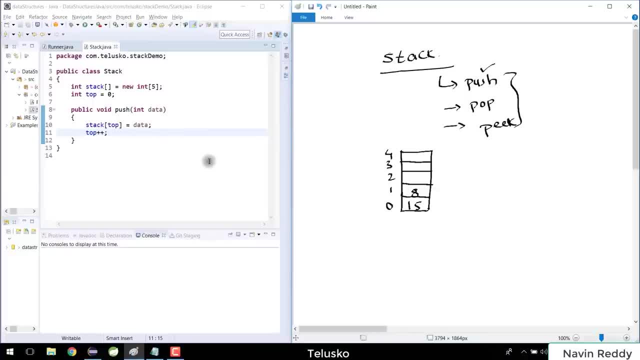 you pass eight, the value of top at that point is eight. so yeah, so that is how you push the element in the in the stack. okay, now next point would be: how will you fetch the element? maybe i want to pop the element, or even before, let's. 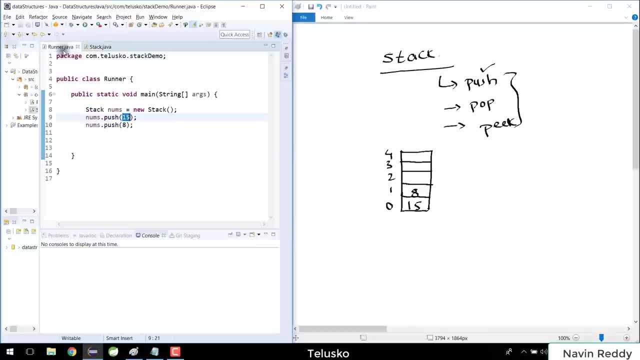 push all the element and let's say i want to print it. i want to print the entire stack. so after pushing two or three values, let me just push one more. we have a stack of size five in that let's say we have only three values. let's say this is 15, 8 and 10. i want to 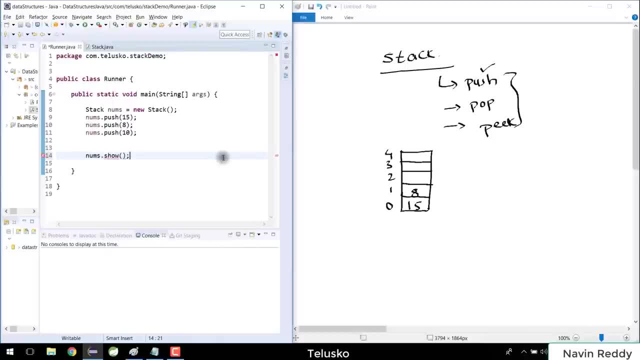 print the entire stack. so i will say nums, dot, show. so it should show the entire stack. but the problem is we don't have show method in the stack. so let's let's go there and say, hey, i want a show method here which will print the. 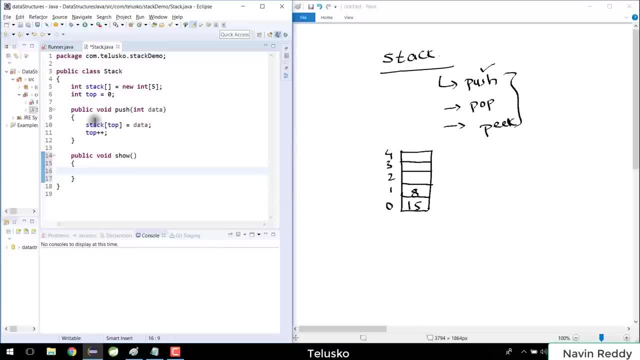 entire stack. now question arise: how do you print the entire stack? it's very simple actually. you can take a loop for loop here and you can say int, n, colon, tack, that's an array and you can print each value and you can print that value with a space. so i will say n and then i 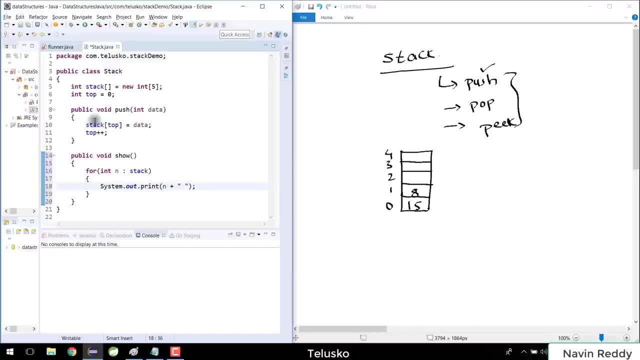 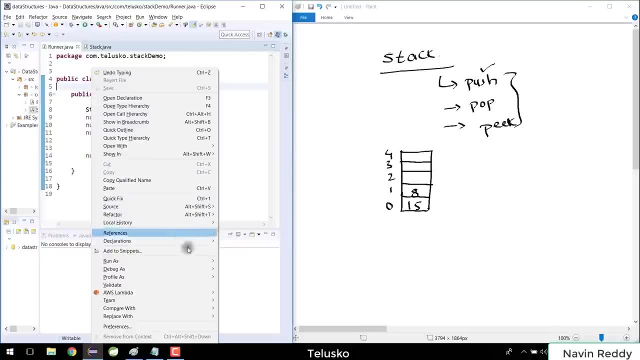 will print a space so that you know when you print all the value. they should be separated with us with a space. sounds cool. let's go back and what do you think? will it work? let's try. so i will right click here and we'll say: run as java. 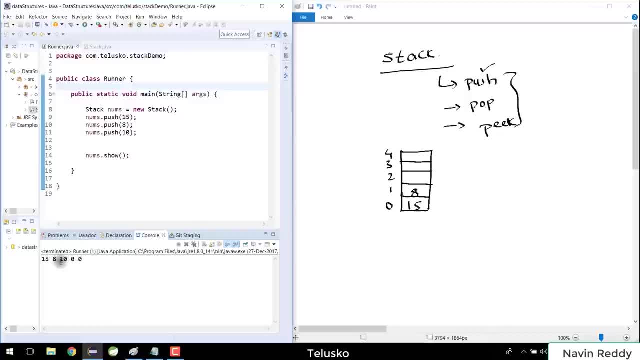 application and it worked. can you see that? we got 15, 8 and 10 and we got 0: 0. so yes, it is working. so stack is working. when you say push, but how about pop? i want to remove the elements now, is it simple? let's try. so, when i say pop, i 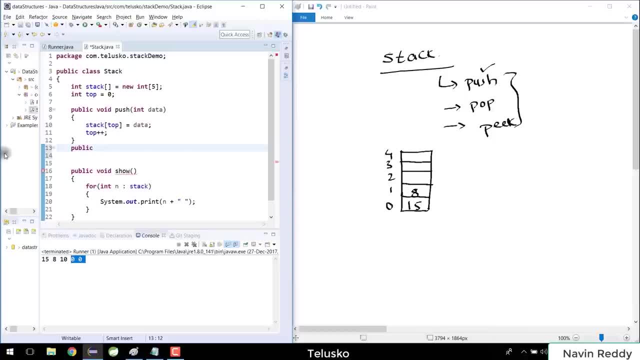 will simply say public, now pop will also fetch the value. so it will. it will remove the value from the stack and it will also fetch the value. so i would say int pop and this will not take any parameter. now, how will you fetch the value now temporary? we can say int data. 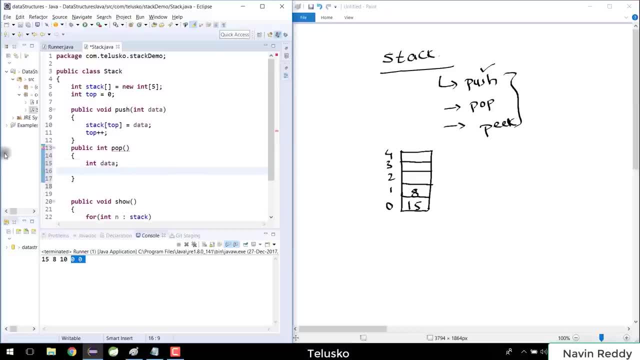 is equal to. okay, first of all, let's declare that. how do you fetch a data? it's simple, right? we can say: data equal. the data is coming from stack. now, the property of stack is if you have three elements, as we defined here, we have three elements, right, we have 15, 8 and 10. 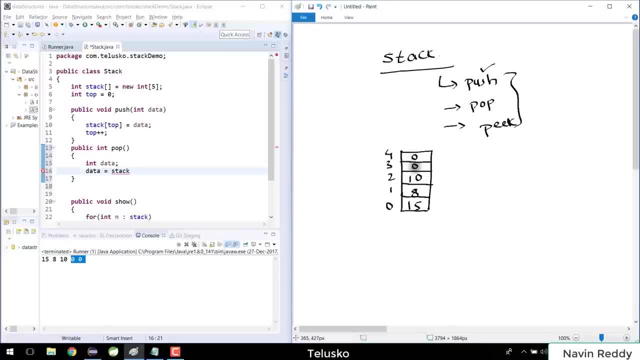 now, when you use pop, what do you think which element you will be getting? and by default, the value of 4 and 3 is 0, because that's how array works in java. the point here is, when i say pop, which value i will get. so it is done with the. 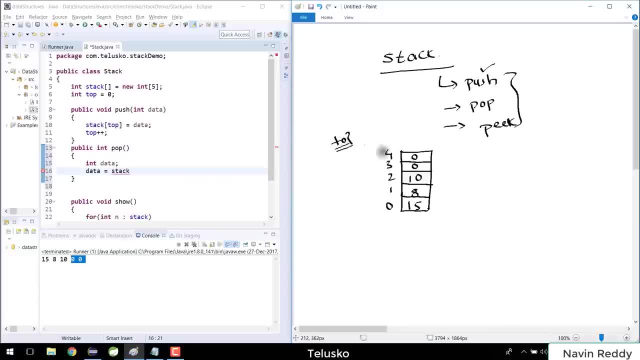 help of top. so we have a top variable here and whatever value we have for top, you will be fetching that value because you will always get last in first out. so the last element which i have added is 10, so the top referring to 10. now this: 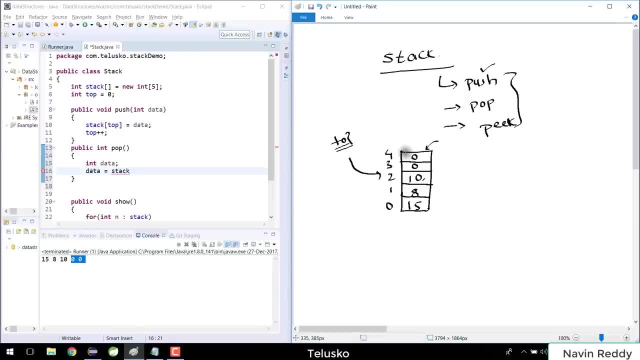 location. so it will give you 10, and the way you do that is by simply saying you will say stack and you will say top. now you will get that data quite simple, right, okay, now there, we have to do one more thing now, once you say you are, 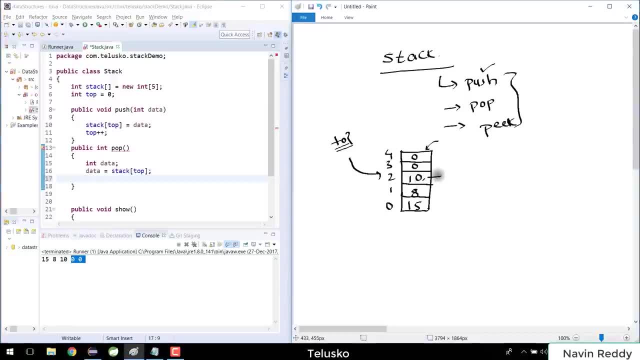 removing this 10, we will be making it 0. so i will remove, i will make this element as 0. and how do we do that? it's very simple. let's go back here and say stack of top is equal to 0, so we are making 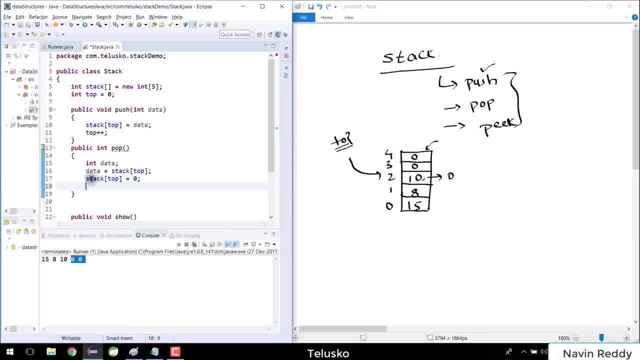 0, so that again you can make it 0, you can make it negative value for whatever you want, and then at the end we can say: return data. i hope it will work now. so let's run this code and you can see: we got. oh, we have not. we are not saying pop. 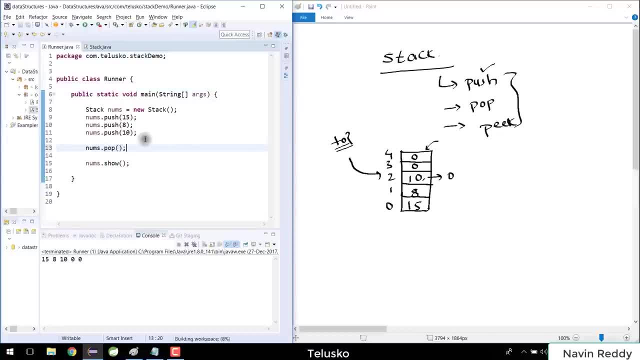 so we'll say nums, dot, pop. now it will delete the last data run and you can: oh, not working, what's wrong? what went wrong here? okay, so we are saying top, top, oh. okay, so we have to do one more thing. see, as you can see here, when i say push the 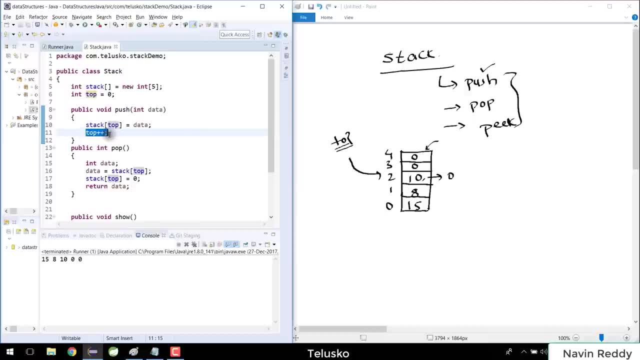 top value. so when i say push, first time it the top value become one. second time top value becomes two. third time top top value becomes three. that means it is referring to this value. we need to do minus, minus. we have to decrement the top before using it. so we'll say top minus. 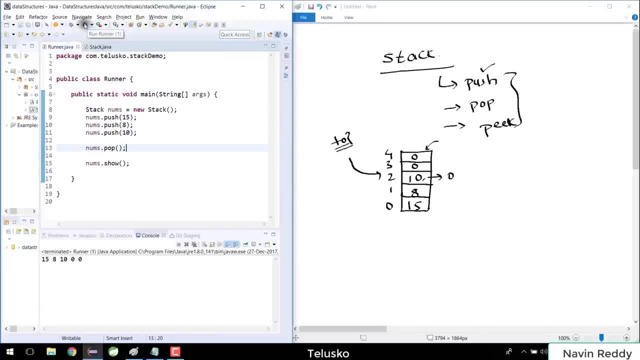 minus, is it? let's try, so i will. oh, i'm not even printing pop value, so whatever pop value i'm getting, i should be printing it right. so i would say: system dot out, dot println. i hope this will work. but on this code: oh, it worked now. 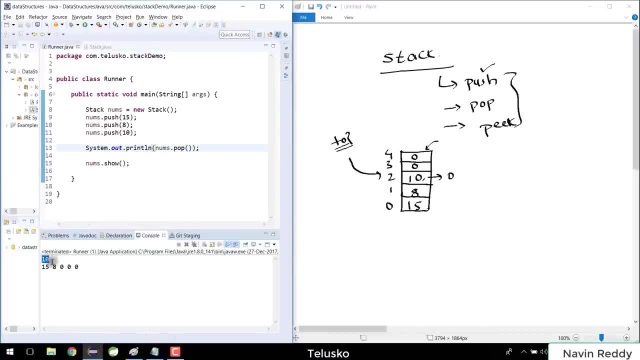 it worked. you can see that we are removing the value if we stand from this tag. and you got zero here, cool right. so that's how you use push and pop. now what else we can do. we can also implement peak here, and how do we do that? so peak. 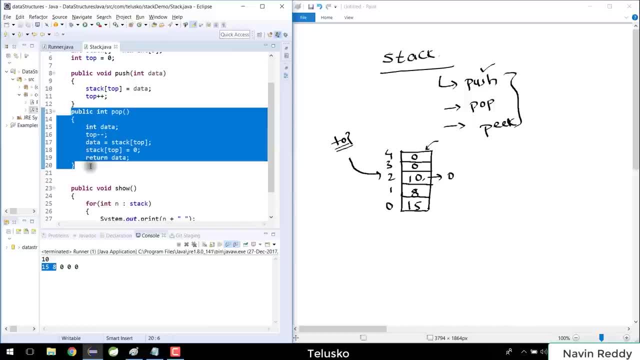 is very simple. peak is almost same as pop. the only thing is in peak you don't delete the element, so i'll paste it here and i will say: this is peak. okay, you will not do minus minus, because if you do minus minus it will- it will decrement. 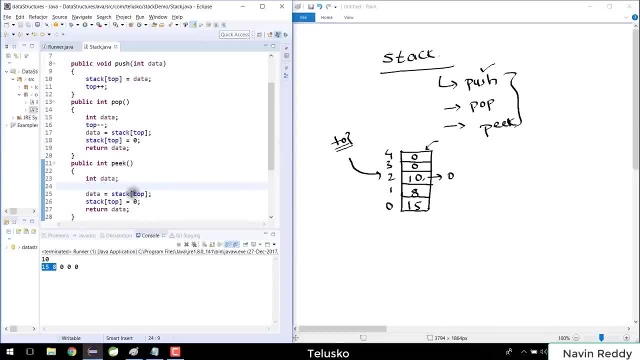 the value, but while you're fetching, you will be fetching the minus one of it. so it's a minus one and you will not delete the element. that's what you'll be doing. that's it. that's peak for you. after adding the: after adding value eight: i. 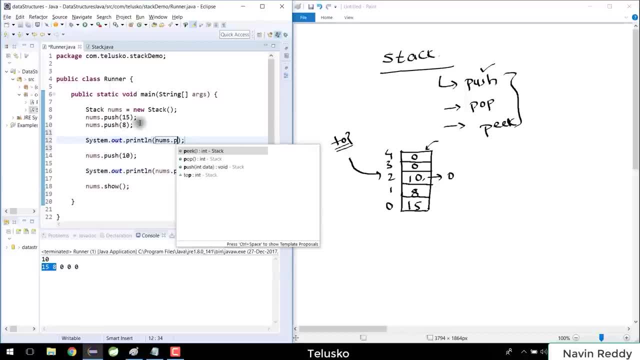 will peak. i would say nums dot peak. if i run this code now, you can see we got eight. so the last value which i have inserted is eight here, and then i'm pushing ten, then i'm popping ten and you can see. that's why in the, in the stack. 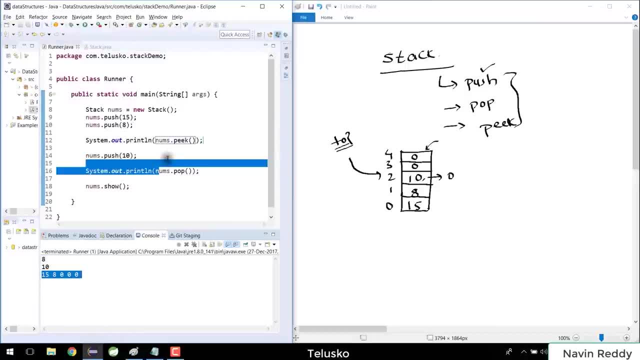 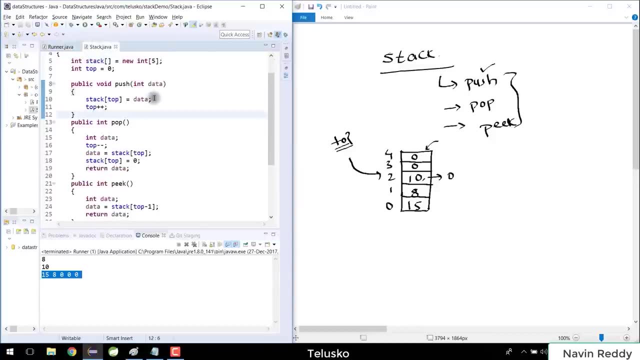 we don't have ten simple. this is how you use push, peak and pop and you will be able to increase the size and pop. what else we can do here? now? we can implement certain other methods as well. example: you can get a size of the stack. you can get, you can, you can make this. 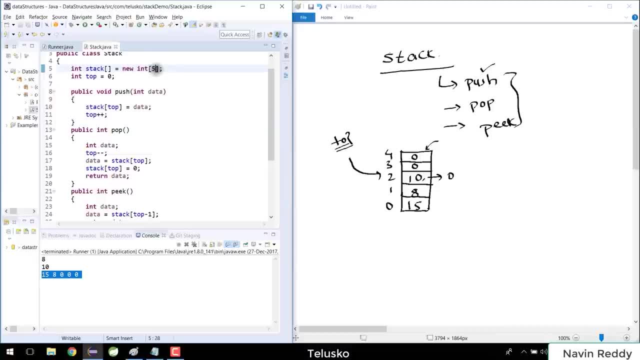 dynamic, instead of saying five, whatever size defined by the user. or very dynamic, which is every time you add the element, even if the initial size is five, you can. you can change it so you can increase the size on the go. we have talked about three methods. we have 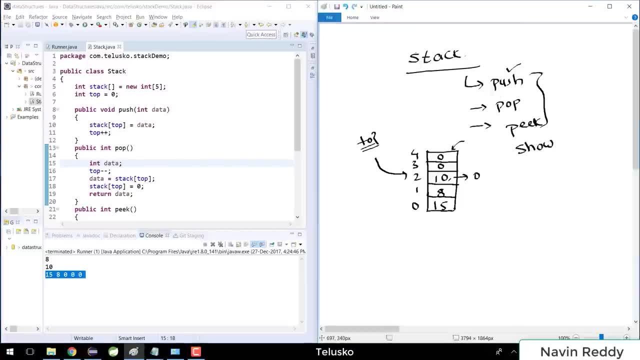 talked about push, pop and peak. in fact, we have also used one more function which will print all the elements of the stack. now, with this, we need two more methods. the first one is size. now, size will give you the size of the stack. and we also need a method called as is empty. 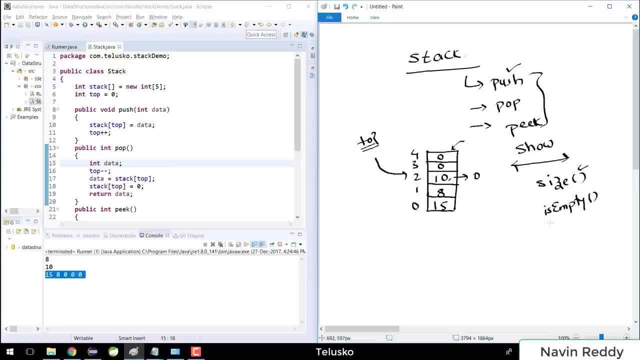 now is empty will be useful to check if the stack is empty now. why do we need that? that we'll see in in some time. but then let's implement these two methods first. now to implement this, let's go back here and i would say, in fact, 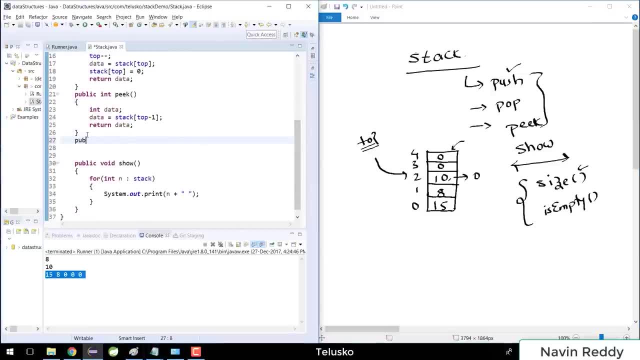 before, after this peak, let me first implement the method which is size. so i will get the size of the stack. so i will say public int. the method name would be size and here let's return top, because top will give the size right. okay, we have, we have a top variable. 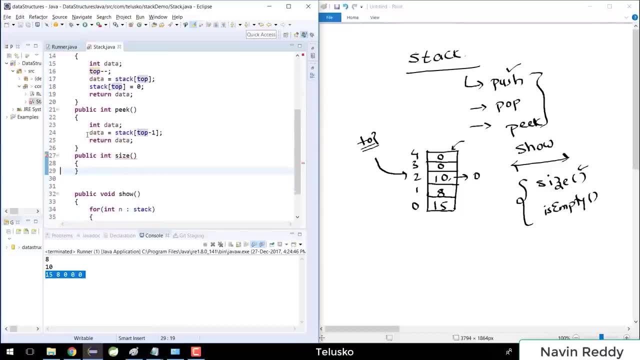 there. so when i return top, what do you think will it work? let's try. so i would say: go back and run inside run. so let me just not pop any element here so you can see we are pushing three elements and then at the end i want to print the size. 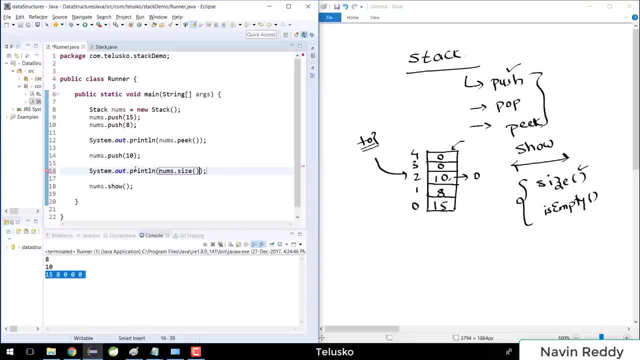 of the stack. i would say nums- dot, size. now it should print the size for you. let's run this code. and okay, it is printing three here, but you know you should also print the message. i would say size is and i will say sizes this one. let's run this code and you can see. 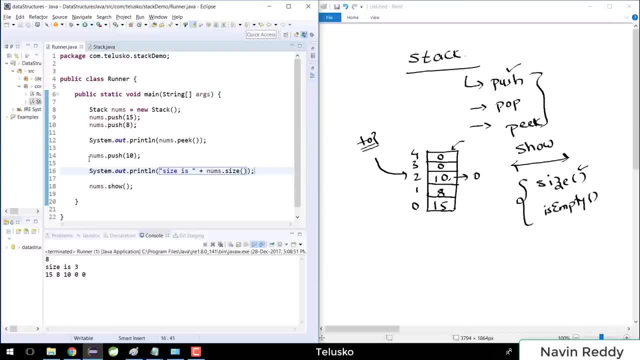 it say size three. that's right, we we are. we have three elements. let me just add one more and i would say the value is, let's say, seven and if i run this code it should say size is four. oh, that's working. you can see that it is working. 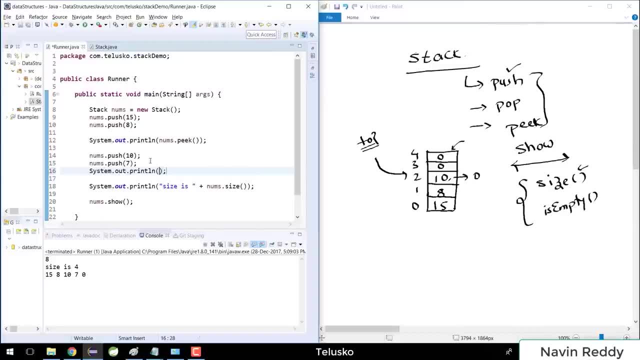 and after that, if i, if i remove any element, let me just say pop, i would say nums dot pop. of course it will print seven, the pop value. but what's the size? size becomes three. so it works right. when you push the element, it will increase the size. 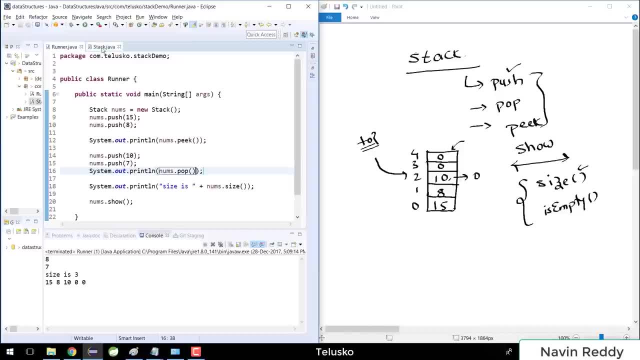 when you pop the element, it will decrease the size. that makes sense. let i want to implement one more, which is is empty, so i would say public now is empty is a method which returns a boolean value. so whenever you, whenever the method starts with ease, it always returns a boolean. 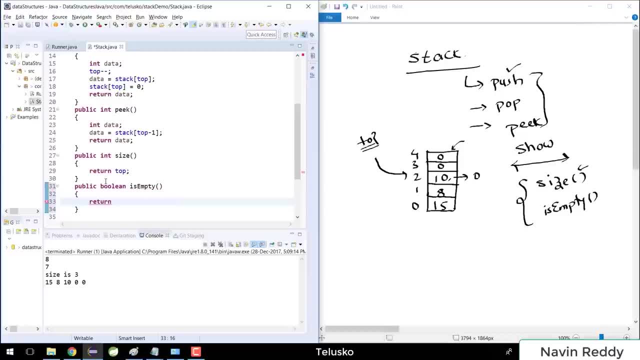 value i would say is empty, so let's return. if the top is or less than equal to zero, then we have to say it is empty right. so it is not zero, which is more than zero, it's not empty right. so let's go back to runner and let's, or we have 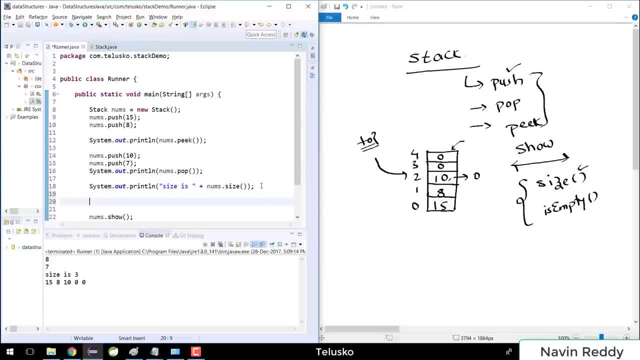 to check if it is empty. so i will check it here after everything. so i will say so. i would say empty status. i want to check if it is empty, we'll say true or false and the moment you do so, we have we have to say num start is empty, right. 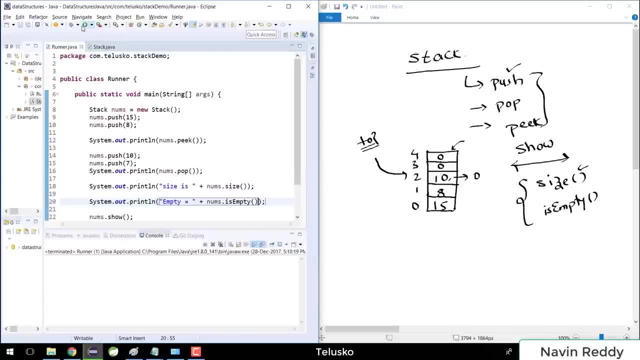 and of course it is not empty. so it should print false and you can see we got false. if i do the same thing before pushing any value and if i run this code now you can see it says true. and if i do the same thing before pushing any, 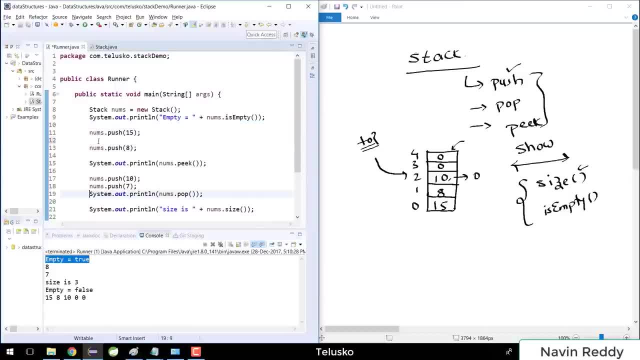 value, it says true. and maybe if i push one element here and after that, if i, if i pop and again, if i print is empty, it will. it will say true, right, because it is empty. so that's how we can implement these two methods, but what's the use of? 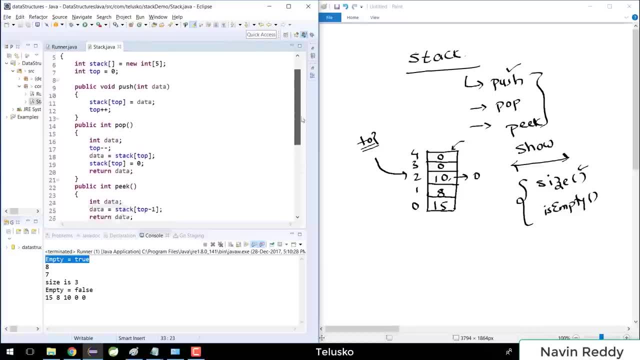 this. implementing these two methods, do we have any advantage? and the answer is yes. so what i will do is: uh, let me just do some experiment and let me remove all the extra stuff from here. i don't want to peek, i just want to push multiple elements and i don't want to do any of 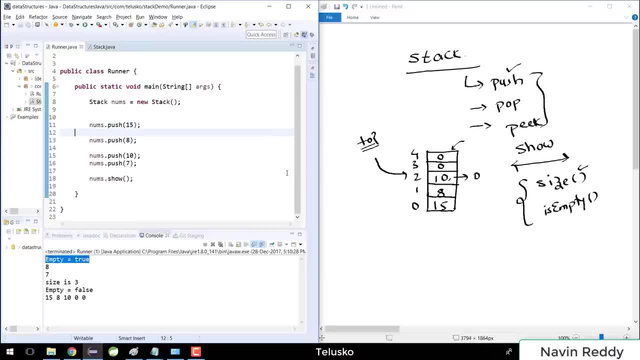 this stuff, let's. let's keep it simple. say i'm i'm only pushing elements and then while i'm pushing, i will push four elements. and if i run this code- so yes, we got four elements- what if i try to push five elements? will it work? let's. 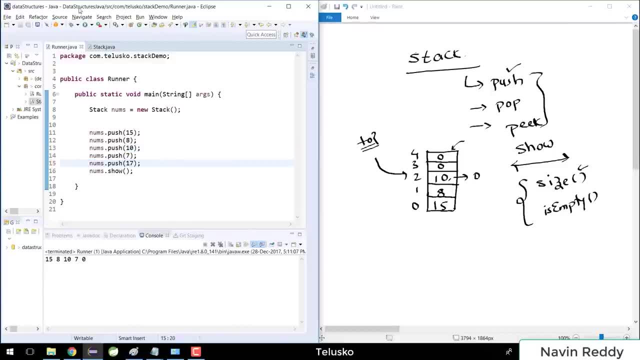 try, i would say 17. and if i run this code- and yes, it does work- what if i try to push one more and let's say the value is maybe 77? in this case, if i run this code, you can see we got an exception, which is array index out of bounds. 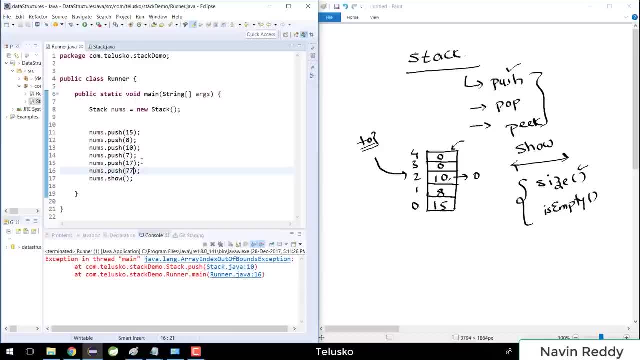 exception. it's full right because the stack is full. that means whenever you're stacking a stack is full, you should not be adding the value. you should print the message to the user: hey, the stack is full. how will you do that? how will you check if the if the stack is full and 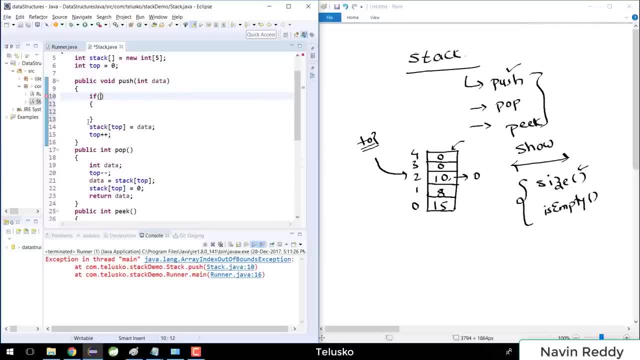 the way you do that. so every time you say push, so before pushing you need to check: is it full? how do you check if it is full? the stack value is five, right, the maximum size is five. so i would say, if top, if this is equal to equal to four. 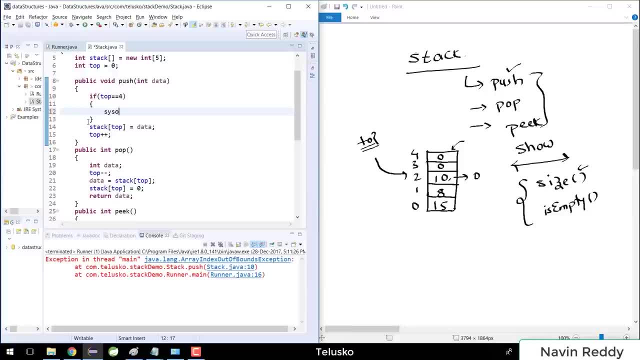 that means your stack is full, right. so if it is four, i would say stack is full. so i would say: system dot out, dot is full and this part will be executed in else part. okay, let's go back here, and after every push i will try to. 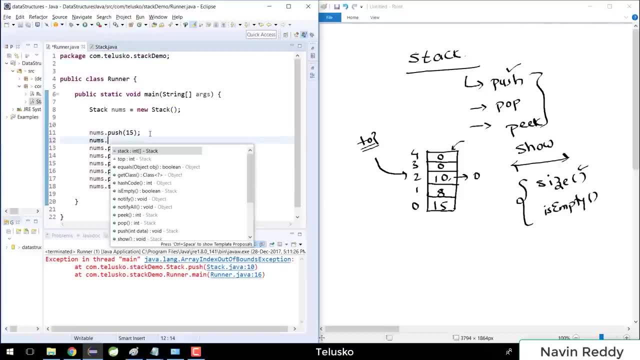 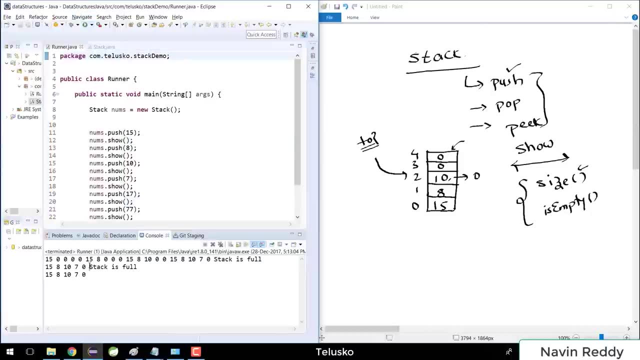 print show so that we'll know what is happening. so i would say num start show and let's run this code now and you can see. at this point it is saying stack of stack is full. oh my bad. okay, i guess i'm missing one more thing here after: 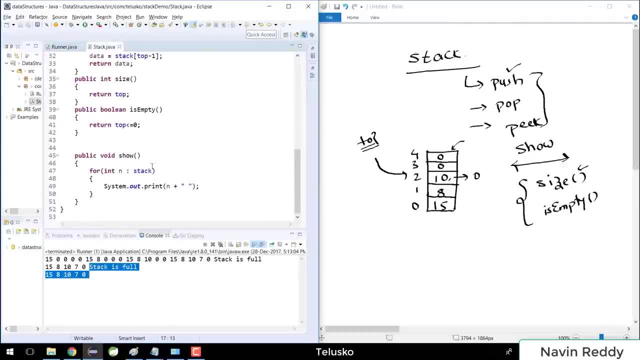 printing the stuff. i just want to print a new line so that every output i will get a new line. okay, so you can see it is. it is a stack. it is saying stack is fully. it's here here itself. because i just made a mistake. it should not be four, it should. 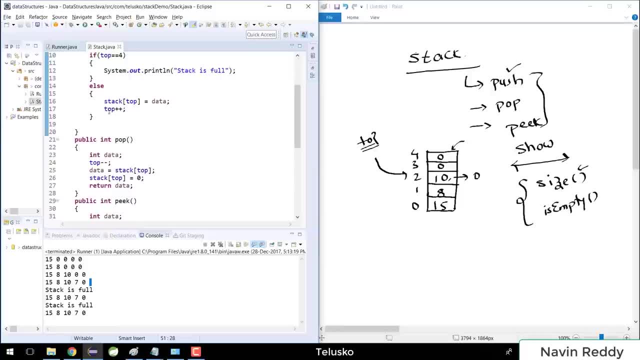 be more than four. why more than four is because every time you say push, you can see we are incrementing the value here. so it is not four, it is five. let's go back there and let's run this code and you can see that after this point it. 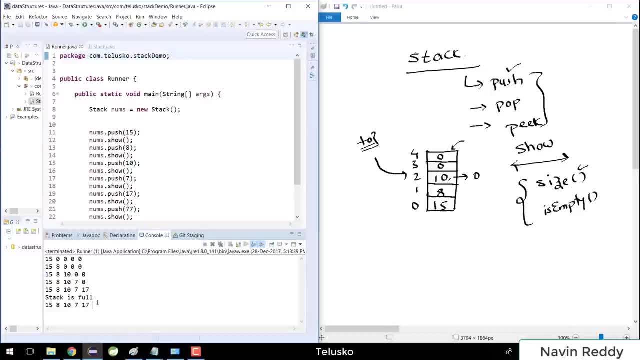 says stack is full, so it will not allow to push the element after this point, so that you can save yourself from the exceptions, right? so that's how you can check if it is full. now what i will do is i will try pushing all these elements and after 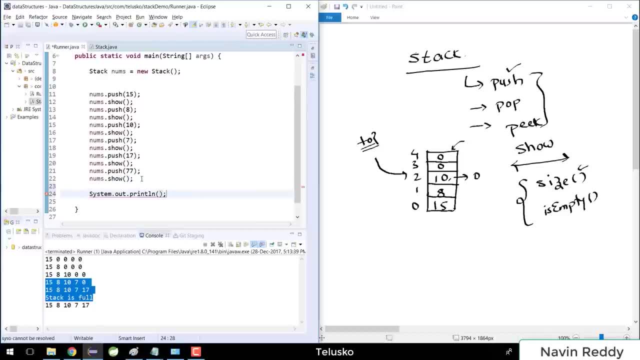 pushing this. if i try to pop the elements and i would say system dot out, dot println, i would say nums dot, pop, it will print. it will pop all the elements and not all it will. it will pop only one at one point. so i will run this code. you can see at the end. you 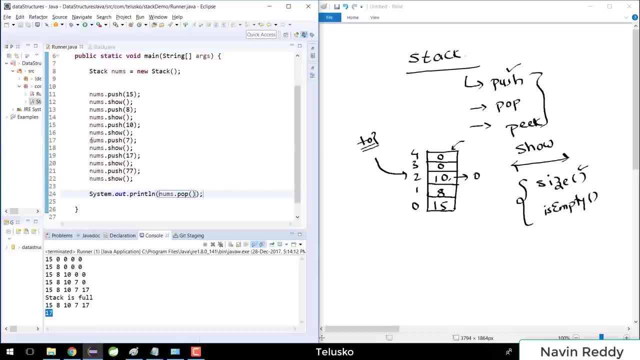 got only one element, which is 17. that's great. in fact, i will not add all this element. i just want to add three elements so that we can save our job. so i'm adding only three elements now and if i say pop, of course you will get the. 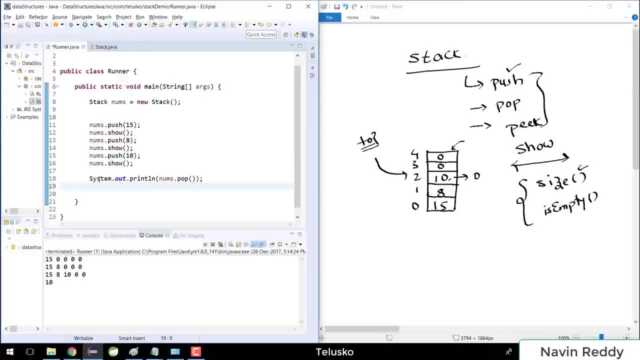 last element, which is 10. right, this is the last time which you have entered. i would say, pop two more times and you can see it will try to pop all the elements. so if i say print the size, i would say nums dot size. it will print zero because 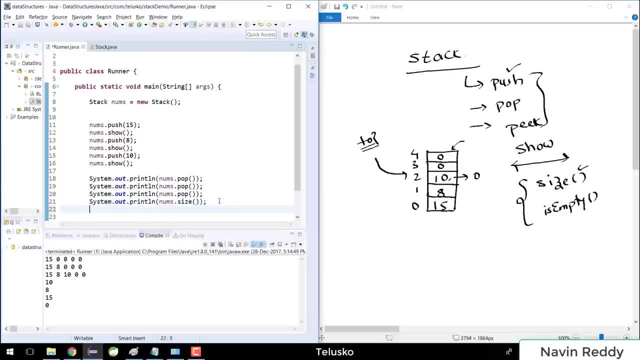 we don't have any element right, so you can see we got zero. what if? if your stack is empty now and if you try to pop now, if you try to pop, it will give you exception right, because you don't have that value before that, so you don't. 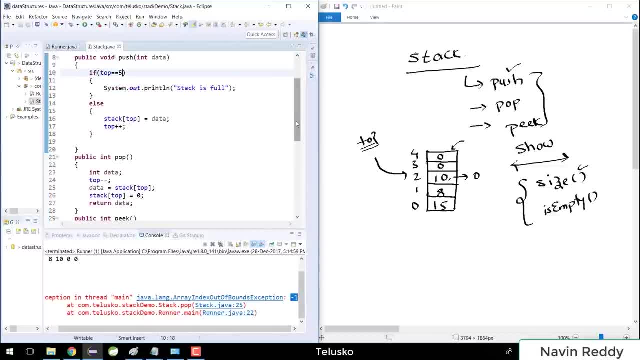 have any value in minus one. so that means you need to stop it before going, before popping the element. how do you check? so we'll say: if so we have to do is, if your, if your stack is empty, then you will not do all these things you. 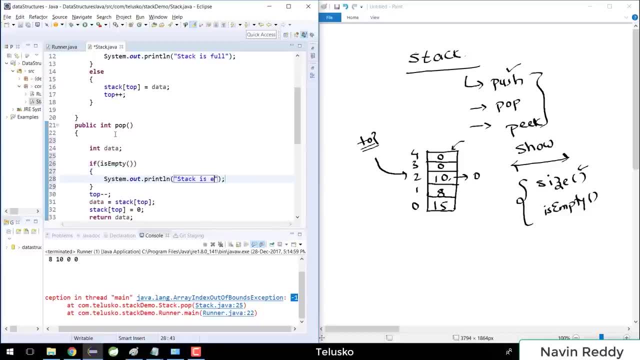 will simply print a message which is: tag is empty, otherwise we'll say else and you got the point right. so if i say tab and if i run this code now, okay, i hope it will work. there's an there's a problem here or data we have to. 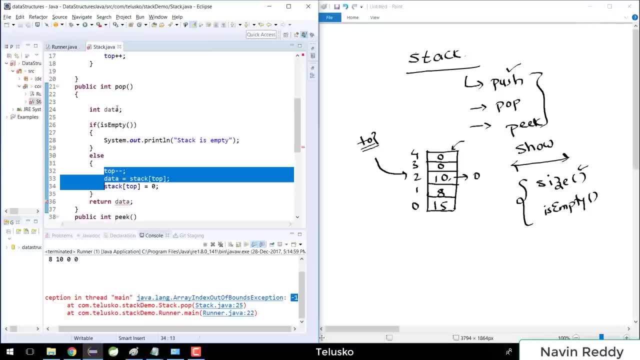 insure something. i would say: data is by default zero. that's a local variable, right? so before returning it, we have to assign some value. and let's run this code now. and it worked. you can see that it says tag is empty, so we have to assign some value. and let's run this. 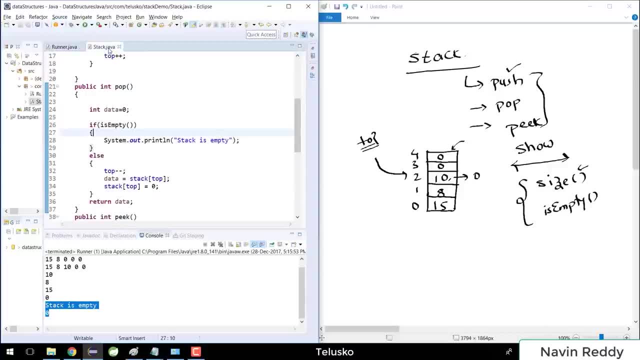 code and, let's say, tag is empty, so it will not give you exception. so we have to handle, we have to take care of all this element as well, right, so that's it. i hope you- uh, you understood what we have done. so we have implemented two things. one is size and 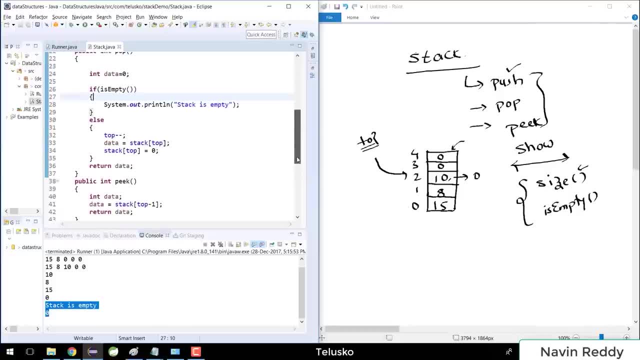 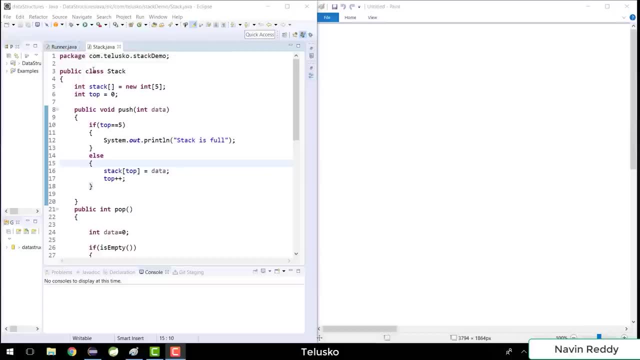 second is an is empty method. so using these two methods, we can. we can check if the stack is full or the stack is empty before performing any operation. we have seen how do we implement stack using a fixed size array. so, if you can see this example, here we have a stack class. 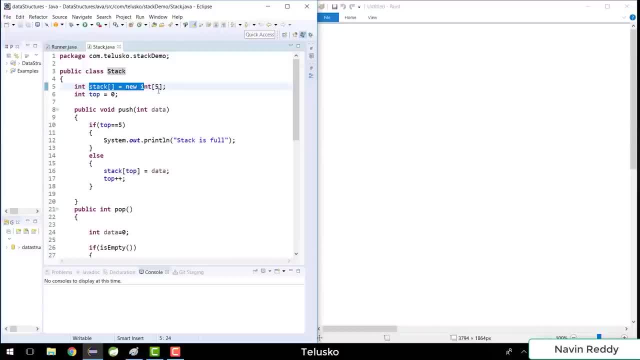 i'm creating a stack array or basically an int array of size five, and then we were able to push element, we were able to pop element, then we were able to peak, and then we were checking the size of the array and then is it is empty, and then we 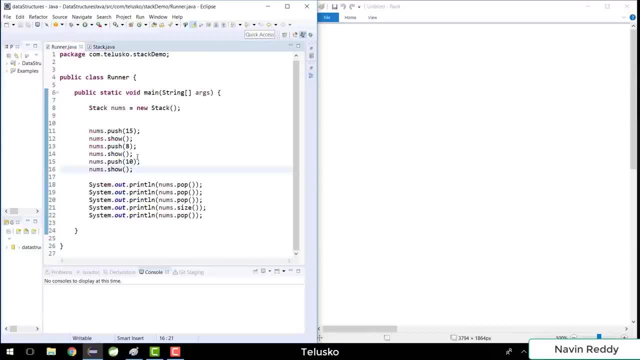 were able to print all the values and then, using this, we can perform the operation. the only problem here is we have a stack and that's perfect. we have a stack here and this tag does have a value, which is, you know, 15, uh, 8 and 10, but the problem is we. 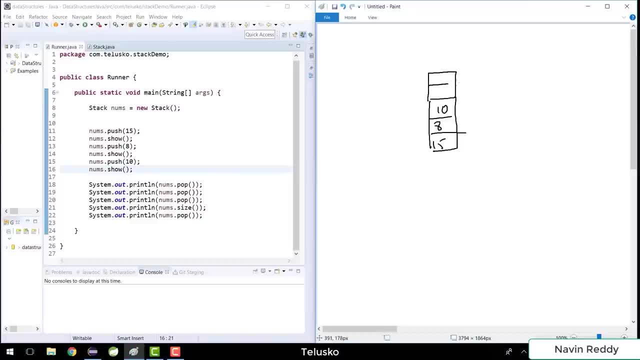 the size of this array is only five, which means the maximum maximum element you can go here is five elements. what if you want to go beyond that? what if you want to have a stack, which is, which is expandable? and that's where we have a concept of dynamic. 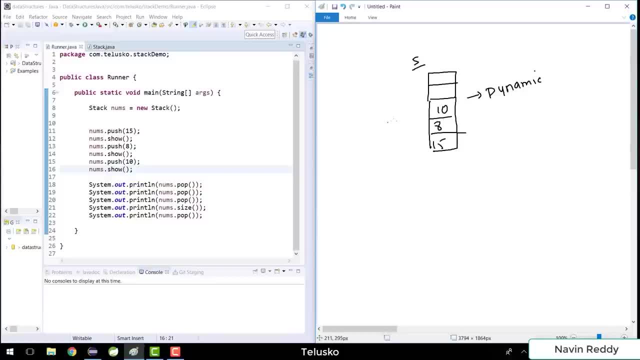 size array, but then how to implement dynamic size array. so what we are, what we want here, is the moment you say, uh, you have five elements, let's say, if you enter two more elements here, let's say three and six, and under that, if you try to add one more element, which is 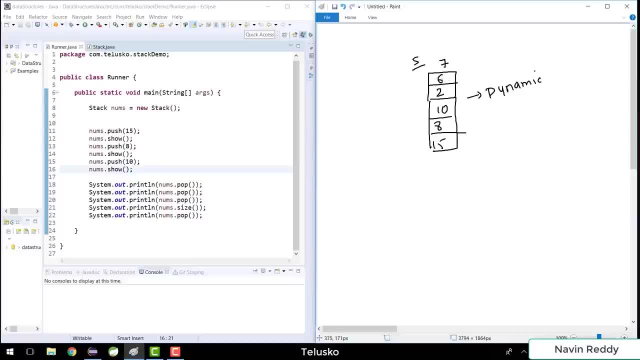 seven, and now, of course, we don't have the array size of size six. so i want to create a new array, so it should create an array of, maybe a new array using in which you will be having all these values. now, when you say a new array, so what? 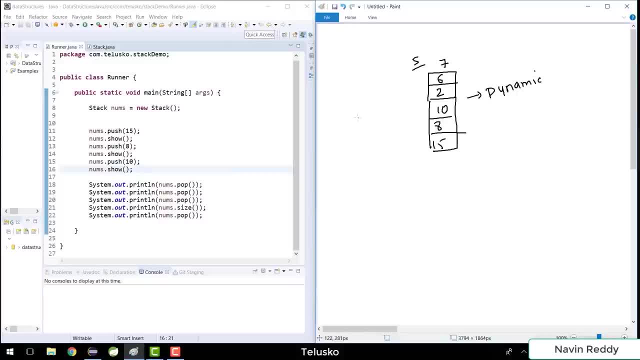 should be the size of that array. so i'm expecting the size of the array would be. so. let's say the current array is of size five. the next array should be of size 10.. technically we'll go with the power of two. initially we'll have an array of size. 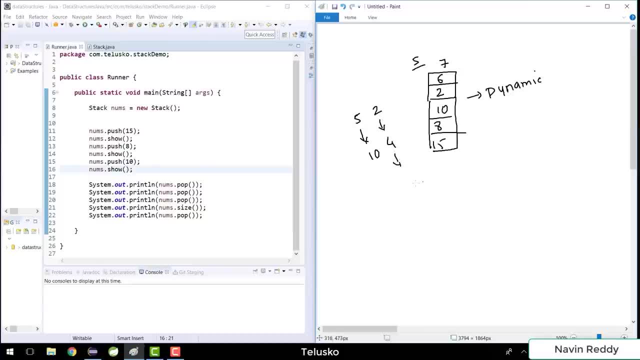 two. if you want to add more elements, we'll make it four. if you add more elements, we'll go for eight. if you add more elements, we'll go for 16.. this is what i'm planning for, but then how will you increase the size every time? so it's very simple. 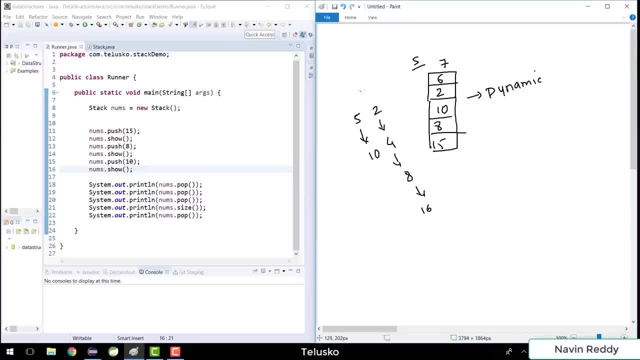 the current array is. so let's say, if you have a current array and let's name that array as stack, so that's your array, we will create a new array with a name. so let's say, if i create a new array with a name as new stack, now this new stack will be. 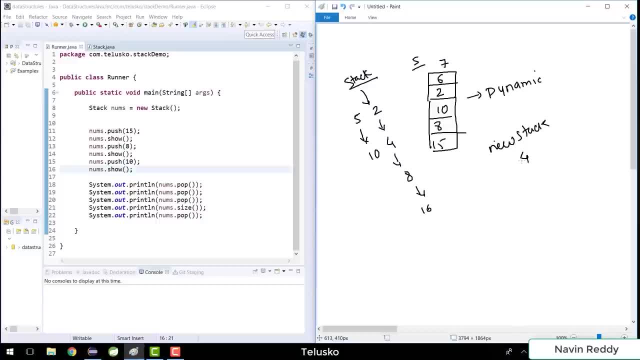 having a size of four. but the problem is we got the new array. what about us? just typically, we just create another stack to the AR- the values in it. so whatever value you have in this tag will be copied in the new array. that's what we want to implement. that's it, if you can do that. 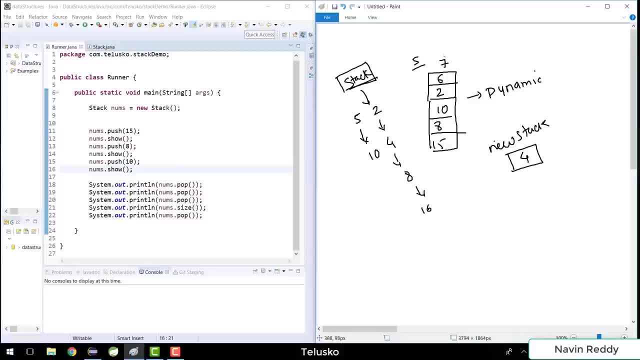 our job will be done. so every time you increase, you go beyond the limit. you have to simply expand your array. and okay, there's one more thing. what if you have a array size let's say 16? yeah, so as you add more elements, you'll be. 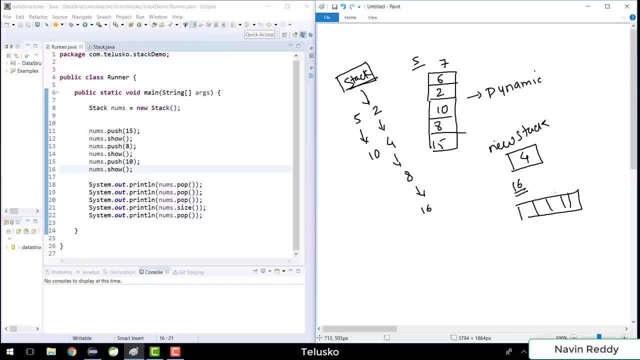 having an array size of 16 and let's say you have 16 values and then you are saying pop, pop, pop for maybe 15 or 10, 12 times. in this case, let's say, if you have only three elements now, so in total we have three elements and the size of. 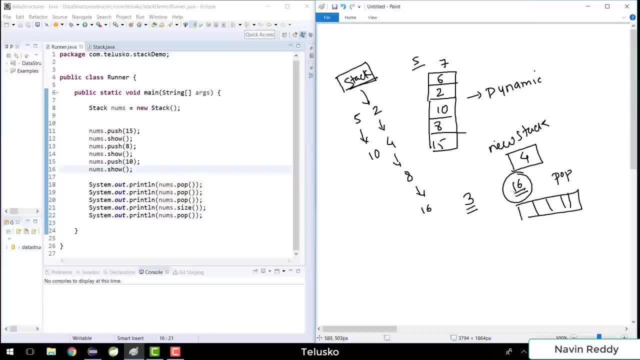 this array is 16, that means you are wasting some memory, right? or we want to have a feature where you can shrink the size. so we want an array. when you say that is dynamic, you want it to be expandable and you want it to be shrinkable. so we want to implement these two features and, if you can, if it is. 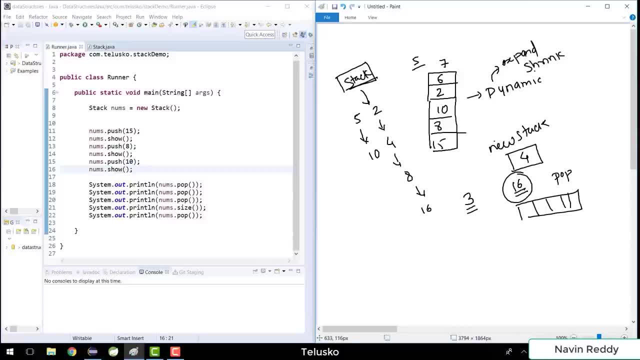 possible for us to implement these two features. that is what you are implementing, and if you want to implement these two features, that is possible for us to implement these two features. that is what you are implementing. so let's get started. so what I'm going to do here is, first of all, I want to 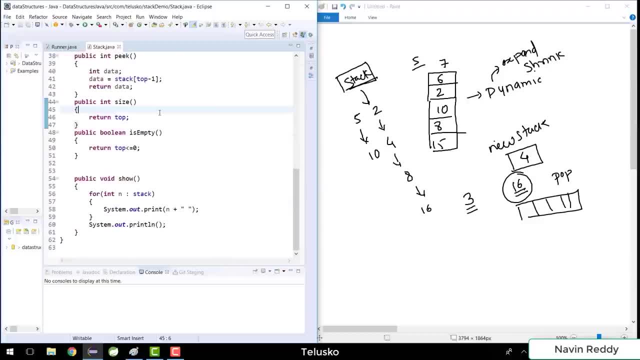 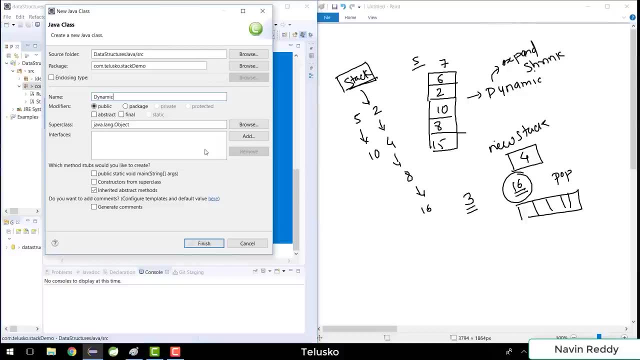 copy the exact code, because we will reuse the code here and I will simply copy this code. I will say ctrl-a- copy and let's create a new class, and then we call this class as dynamic stack. I will say destack. you know, that will then look. 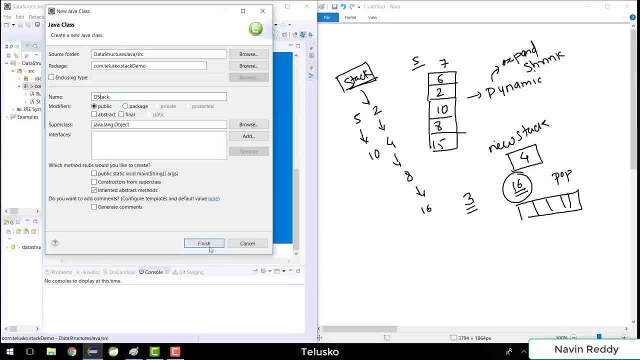 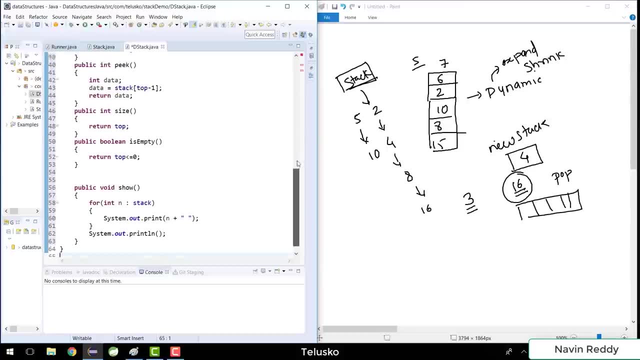 like a dynamic stack. we are making an image stack here, so let's say destack and we click on finish and in this tag class I want to have all those features. I will just simply paste it here and if i go back up there might be some issues. i have repeated the package. 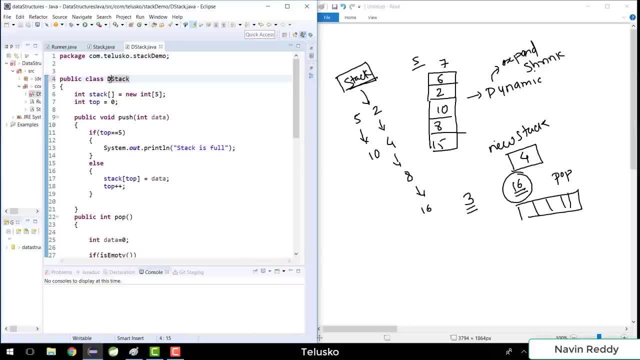 and the class name is this, this tag. okay, now, the first thing we need is: you know, we cannot simply create an array of size five. i want to create a variable with a variable with a variable name as capacity, capacity, and then, let's say, the capacity of this is two. initially, we'll have a capacity of 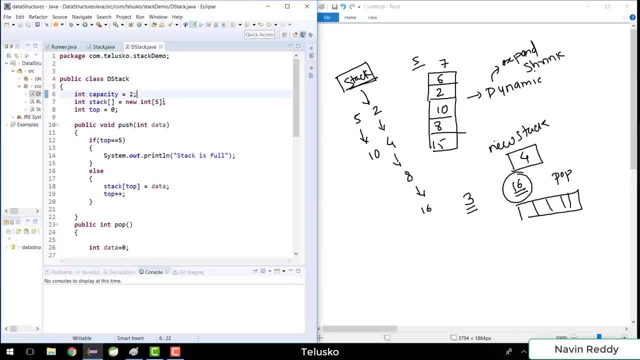 two, and then we'll go beyond that. normally we can go for a capacity of four or eight. that will make more sense because normally when you say you have a stack, of course you'll be having more elements. but just to make it interesting, you know, just to show you how it expand and shrink, we'll start with. 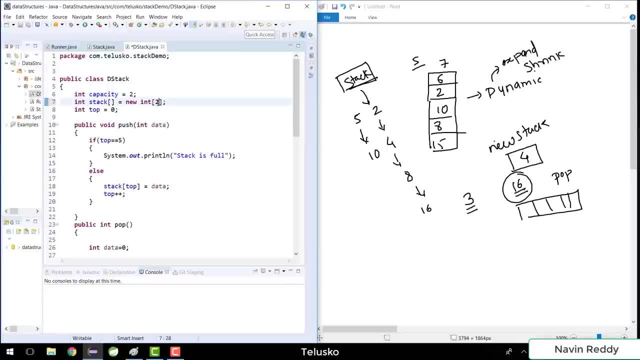 q. and then here, when you create this array, i want to say this is two. again, you can, we can, write capacity here, right? so you're creating an array of that size. initially, the array which you have is of size two. okay, that makes sense. now, of course, we will be having a method which is size we have. 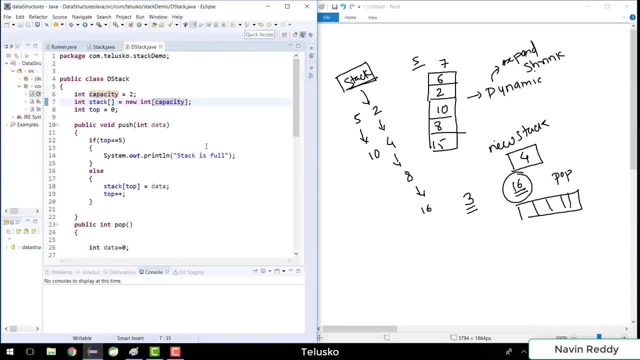 the element which is is empty. so everything will remain same. now what will change is the way you push. so when i say i want to push the element and i don't want to print a message which is stack of full, we don't have any option there. now. 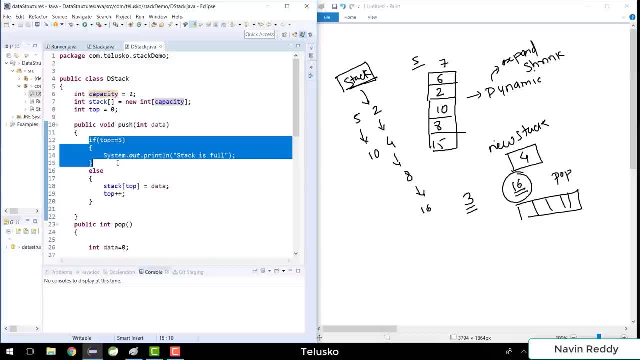 if you, if you, even if your stack is full, you want to expand the size, that means this code will happen, for sure, you will be able to add the element. the only thing is, maybe if your stack is full, so you need to expand the size, and then how will you expand the size? so i will simply call a function. 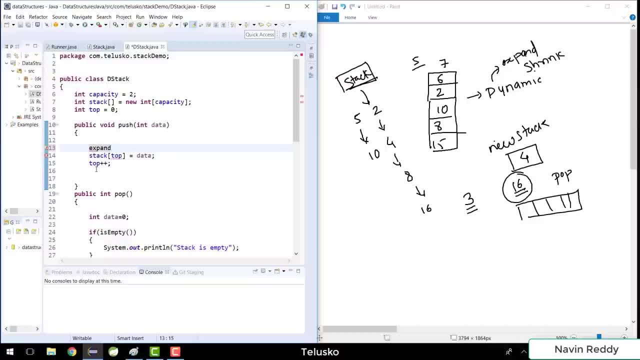 or a method here called as expand. but when? when i want to call a method which is expand, so only when your stack is full. but how do we know that when i want to call a method which is expand, i know if the stack is full? okay, that's a good question, right? so if the size of the of the stack 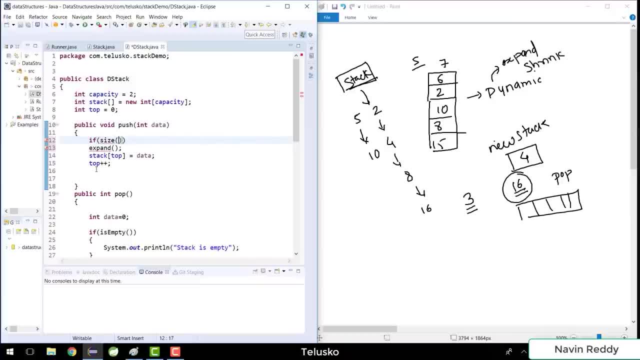 which is, say, size is okay. if i say size is equal to, equal to the capacity, then that means your, your stack is full. in that scenario you will expand, that's it. nothing much in that scenario will expand and anyway you have to do this task. but question arise what you will do in expand what? 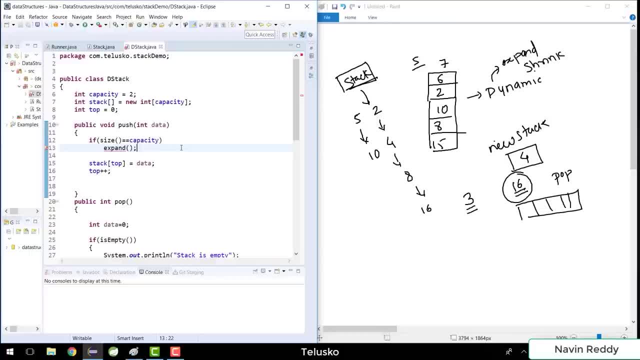 exactly happens in expand. think about it. what will happen in expand? so, in expand, what you do is we have to create a new array. that's the main idea, right? so let's say, i want to get a method called expand, which will be this method. here again, you can make it public or private, doesn't matter. uh, in this case i'm keeping 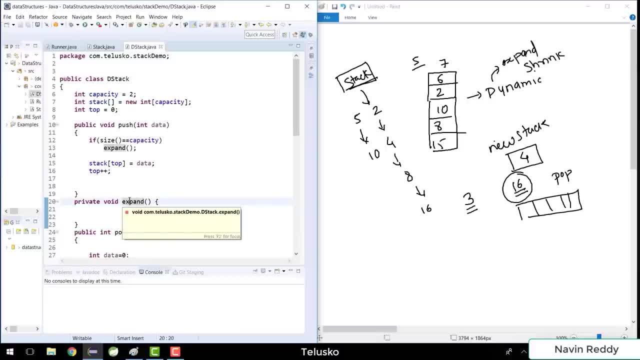 it private, because i don't want to access this expand function from anywhere else. i just want to use the expand only from the current class. so i will use expand and then the first step would be: i will use the expand function and then i will use the expand function and then i will use the. 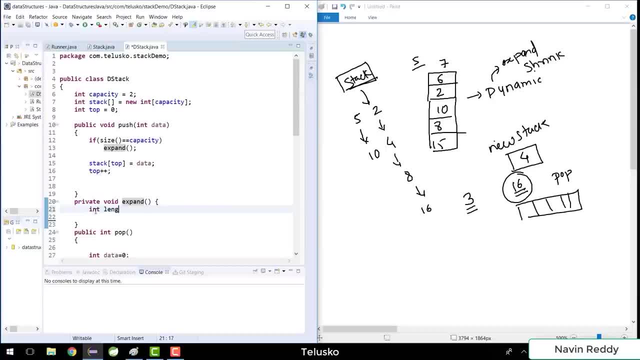 expand function, and then i will do it again to copy ahead and paste. now i will do thisśli za okay, now the size of the stack would be doubled, right? so if, if the current size is two, the next size would be four, right? so i would say ain't, and then i will simply say capacity, whatever value of. 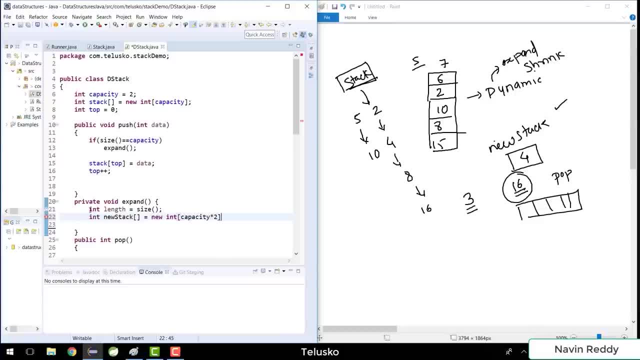 the capacity we have. i will simply say capacity into two, our job will be done. so we got new stack and then we are saying: into two, that makes sense. the next thing we have is: okay, so we got the new array. now we have to copy the element from the current array to the new array. now how do we do? 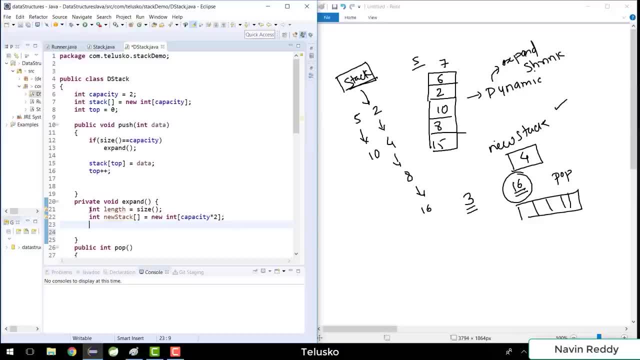 that, so we can run a loop here. we can use normal for loop. the best way would be to use inbuilt classes. again, it's your choice. okay, you can use normal for loop, but since i'm lazy, i'll be using some inbuilt classes. i would say system, i would say there's a method called as array copy. so 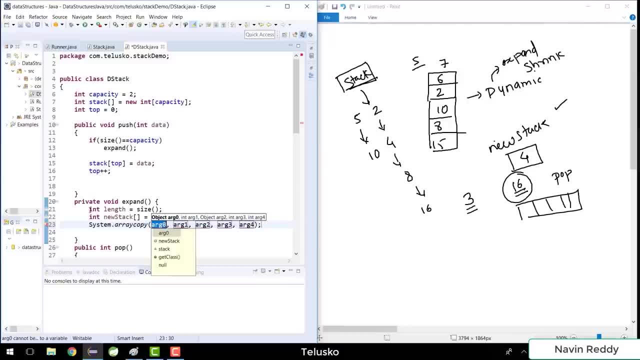 thankfully we got this method: array copy. this array copy takes five parameters. the first parameter is from where you want to copy. so i want to copy copy from the stack array which starts with index value zero. again, i want to copy the entire array, right, so we start with zero and then it will it. 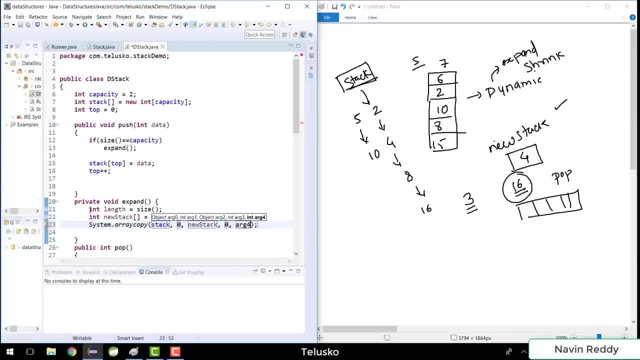 will get copied from the stack array. so i want to copy from the stack array which starts with, and it would be zero, and then how many elements you want to copy. i want to copy all the elements. i would say: simply say length once you have copied everything. so in new stack you have all the new. 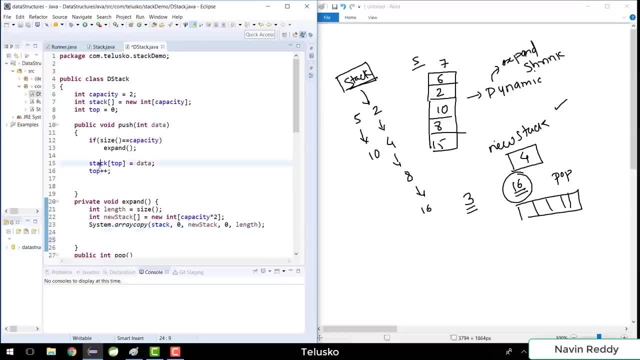 values, but then unfortunately, ultimately we are working with stack array itself, right? so, even if you expand the new stack, everywhere we are using the stack reference. so of course, we have to replace the stack reference with the new stack reference, so that everywhere else i'll be using the stack. 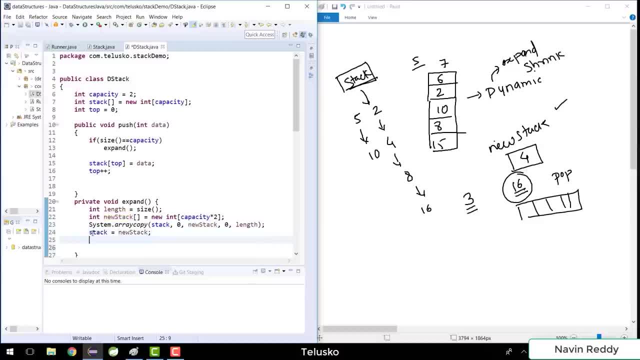 reference, which is replaced with the new stack reference, so that i can just copy the stack, a new stack here. Okay, so, once we have done with the stack and now, if you can observe, we have also increased the capacity. So I would say capacity is equal to the current. 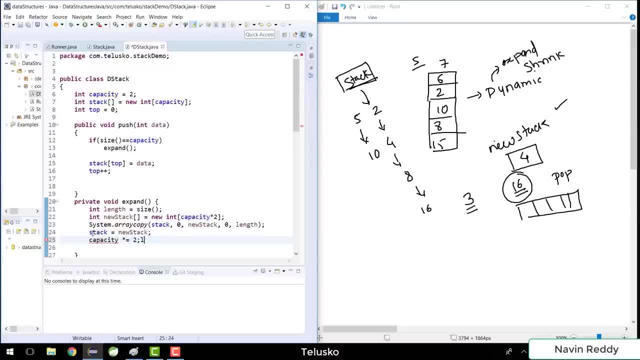 capacity into two. So I would say, I would simply say, into equal to two. So whatever capacity you have here, it will. we are just trying to double it. That's it. It's so simple. And now let's go back to runner. Now, instead of having the object of stack, let's say object. 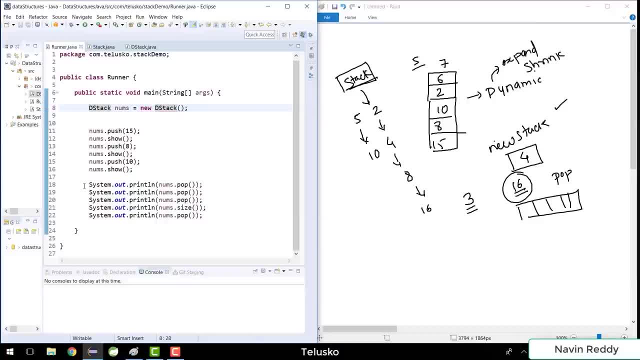 of this stack so that we will not get the exception And I will not say pop. this time I will only focus on push And every time I push the element I would say show, just to get the output. It's a copy paste page, So you can see I'm entering five elements. 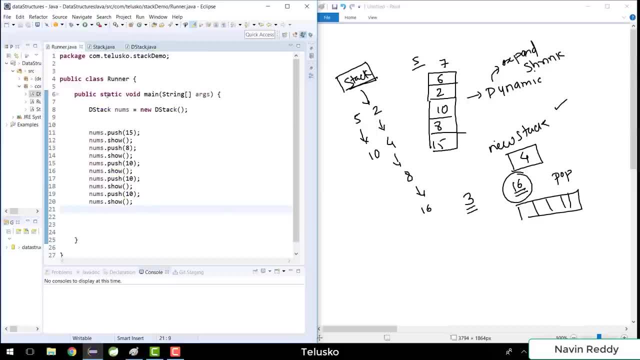 The size of the array which we have here is only two right, But still we are trying to print five. let's run this code, let's see if it is working. And it works. You see that it works. So initially we were having two elements. no problem, We added new element. 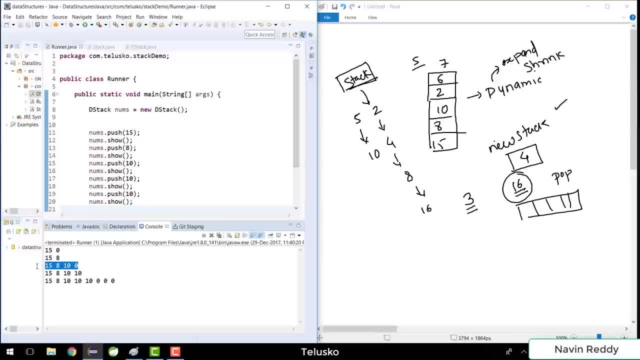 But then the moment you add a new element, you will see that the element is not going to be added 10.. Can you see that? it is? the capacity is not three, it is, it is four. In this scenario, we have added four elements And now, the moment you add one more element, 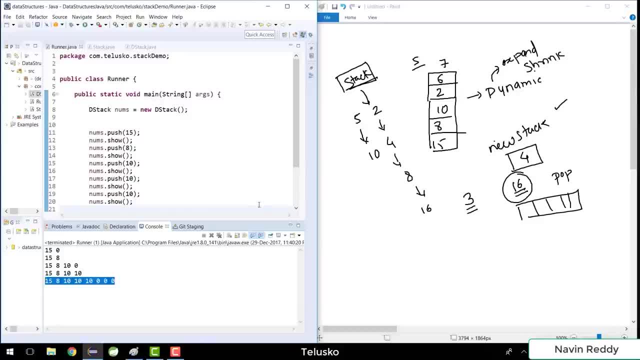 which is 10,. again, we got the element of size eight. So that's how it is expanding. Cool right, In fact, you can print the. you can print the value using size and you will get the exact size, whatever, or the capacity if you want to print. So that's how we are. 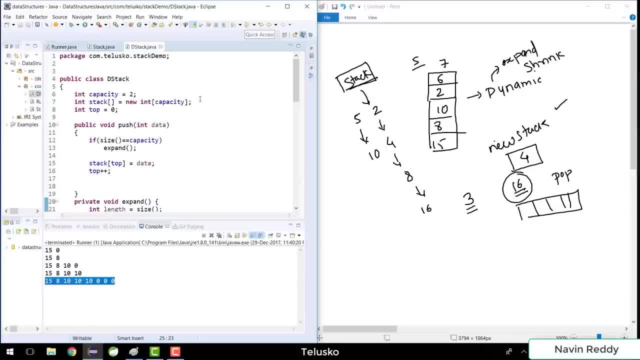 expanding it So simple. That's why you say it's a dynamic array. The next point would be: how do we pop the elements? Because I want to also want to pop elements. right, So I would say: pop is working. But then every time you say pop, I want to decrement, I want to shrink. Okay, first of all, I will. 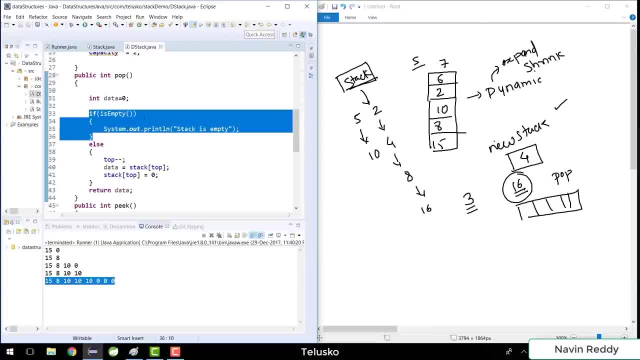 not say is empty. Do you want to check? is empty? Yeah, that sounds good, Is empty is a good checking. But every time I remove the element I want to shrink. So I would say: shrink Now. shrink may not work every time, But then whenever your size goes, okay when. 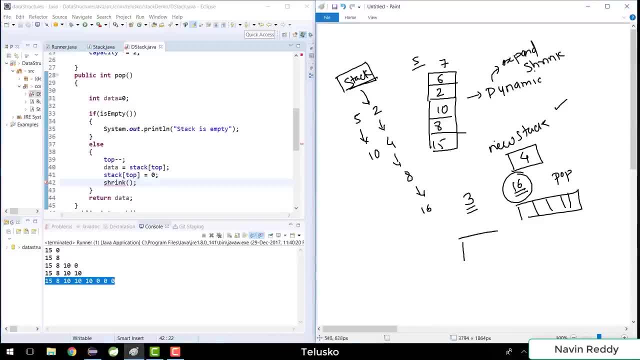 do you want to shrink? That's a good question. If you have an array of eight, or maybe you have an array of 16, the size is the size of this array 16.. But the elements you have, let's say, eight. at this point I don't want. 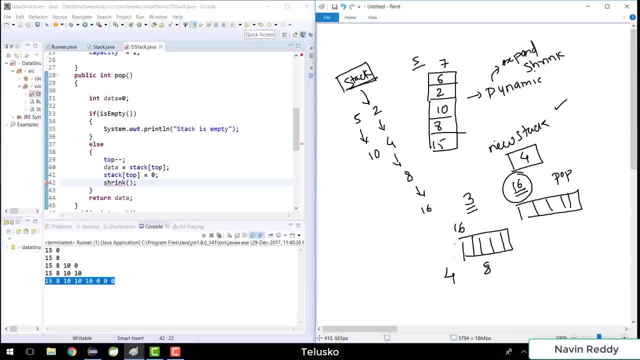 to shrink, But the moment elements goes on less than four. So let's say, if the number of elements is 123 or four, in this scenario I want to shrink it and I want to make it half, half of 16, which is eight. So even if I have four elements I want to make keep. 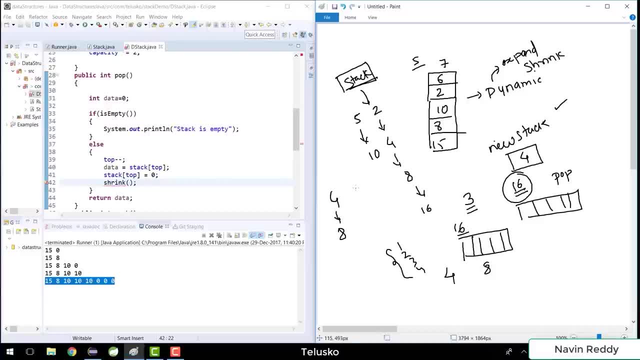 it eight. Let's see if I go beyond that, if I, if I, if I go below that, if I say I have one element, then I have to make it two And of course, before going for one, it will become four and then it will become two. So the idea here: 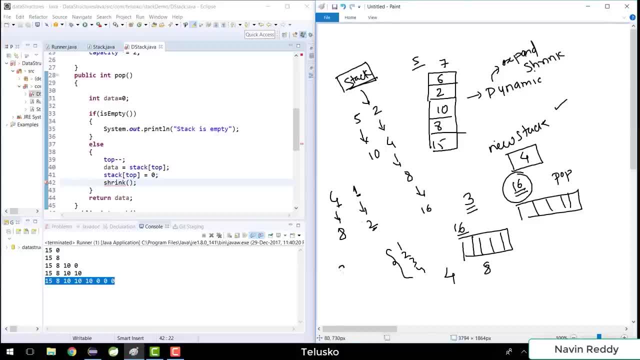 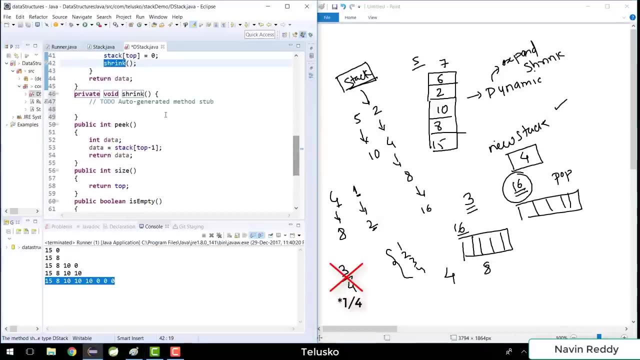 is, if the number of elements goes below three by four, we will make it half, So the size of your array becomes half. That's what we're going to do here in shrink. So let's implement shrink method. So I would say, click and create a method called a shrink. Now, inside this, 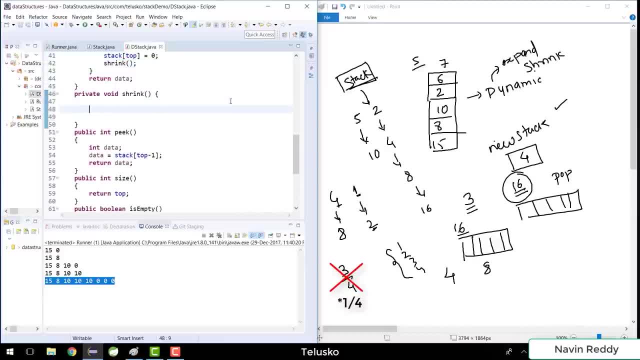 shrink method. I want to perform the following those operations. And how do we do that? Now, first of all, we want to know the length, because that's very important. So I would say length equal to size. And then, once we 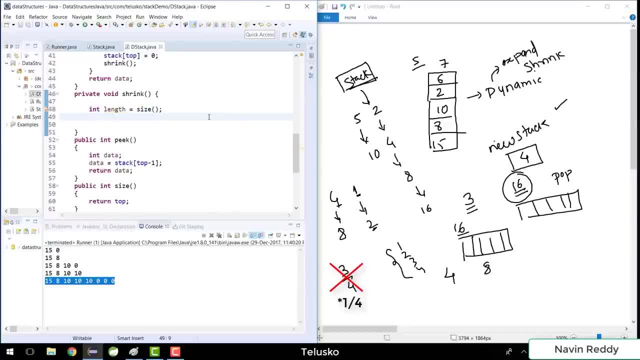 got the size here, or once we got the length, now how do you, how do you shrink it? How? first of all, how do you know that your array is? is the number of elements in the array is less than three by four? Now, there are multiple ways of doing this: formulas, we can use shift. 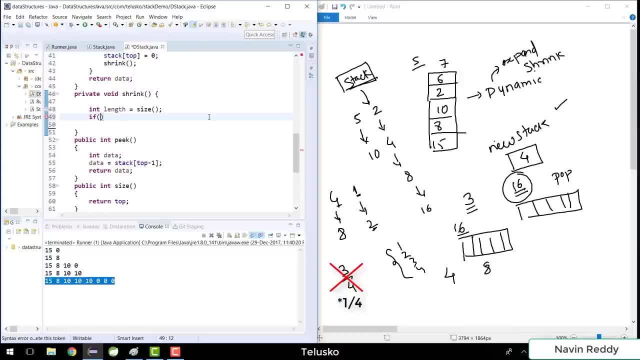 left shift array, I mean left shift arrows. you can do some mathematical calculations. you know, I'm Sims, I'm lazy. I'll be using the simplest one, which I love. So I would say: length is less than I would say capacity, because this, so the operation which I'm doing now, will give. 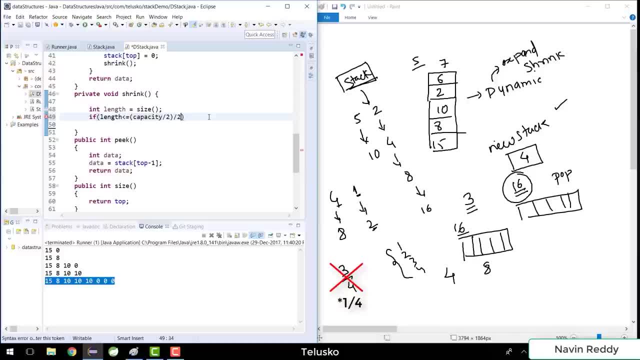 you half. So I would say, divided by two, it will give you half. And again, if I say divided by two, it will give you one for the one fourth. In this scenario, what I do is I want to reduce the capacity by half. So it's a capacity is equal to capacity divided by two. But then 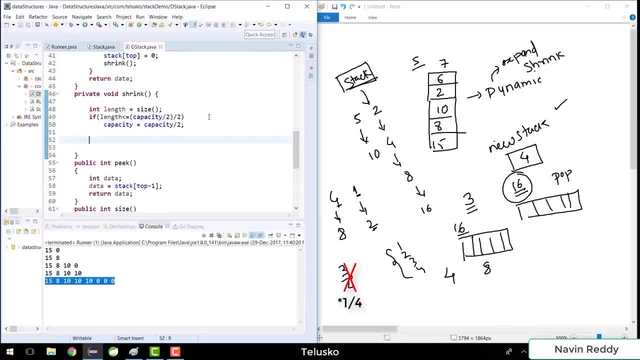 it's not just reducing the capacity, is also about creating a new array. That's important, right? So what I will do is I will get a new array, which is it's a new stack again, And the question is: what should be the size of this array? 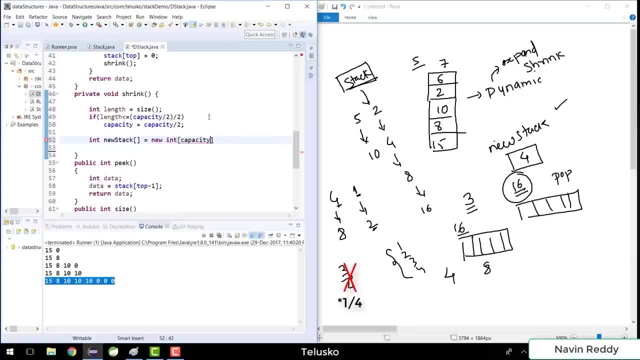 And you guessed it right, It will be the new new capacity, right? If you? if you, if your earlier array was of size eight, the new array would be of size four. So this is where you're doing it. you're dividing by two. Again, if you're thinking, we will be. 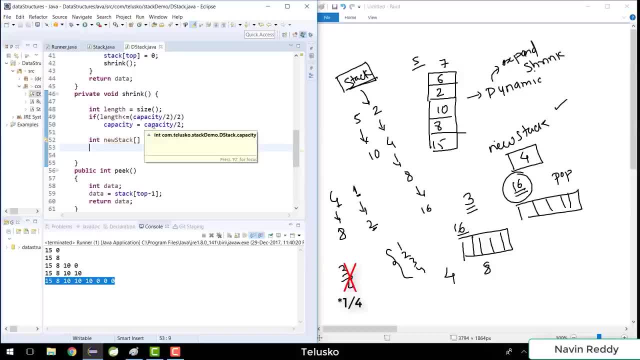 getting a point value. don't worry, this is a part of two. capacity will always give you part of two because we're expanding in that way. So it will not give you a point value. It will just create an issue for you. Now, once you've got the new array, the same thing. 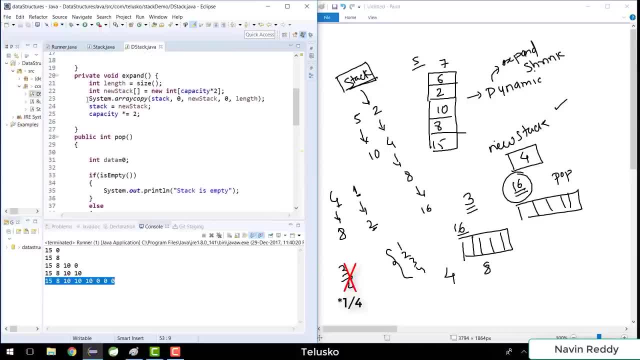 we can actually copy paste. you know, okay, I cannot say copy paste. I should be saying code reuse, that will make more sense. Go back here and paste And you can see we are critical new array, we are copying the elements And then we are saying stackable, the new stack. 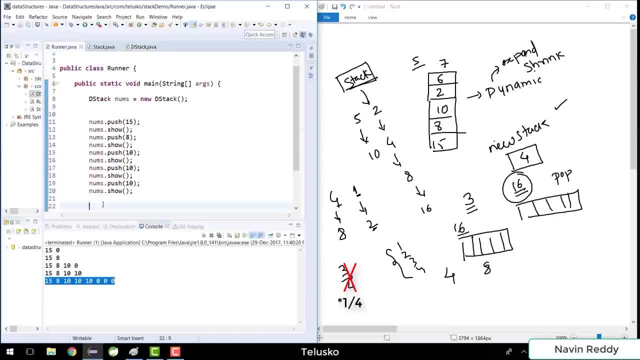 I hope it will work. Let's go back to runner And then at this point the size of your stack is eight. After that I'm saying pops. I would say I don't know, I don't want any value. basically say nums dot pop. it should remove the element. and then I will say nums dot show. 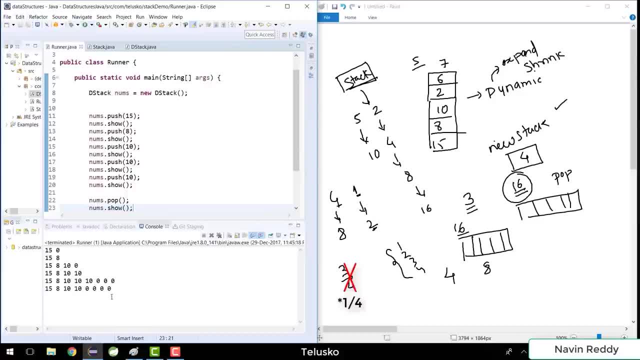 so that I will see the elements And look at the size. it has removed the element. let me just remove one more, In fact two more. just let's go beyond three or beyond two, it will go. let's go to two And the moment you have a size two, you see that the the 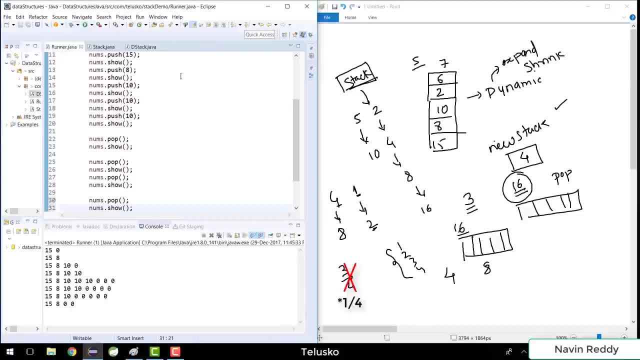 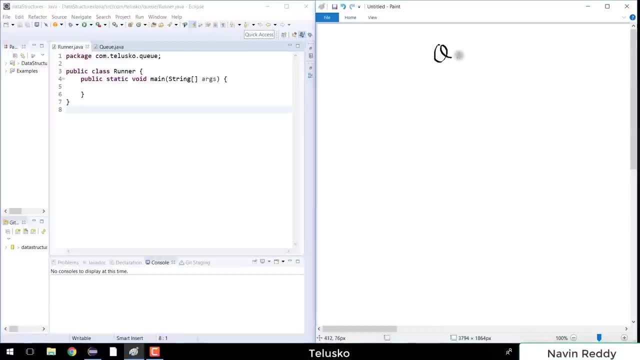 array is getting shranked, And if I go one more time see this, I see the other size. it is getting shranked. So that's what. that's how you do make it dynamic, And in this video we'll talk about queue. 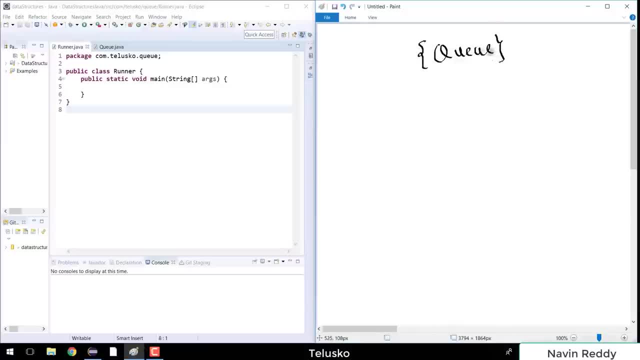 Now we have talked about linked list, we have talked about stack, and now it's time for queue. Now, queue is almost same as stack. The difference would be: in stack, we use a concept of li fo, which is last in, first out, And in queue, we use a concept of FIFO, which 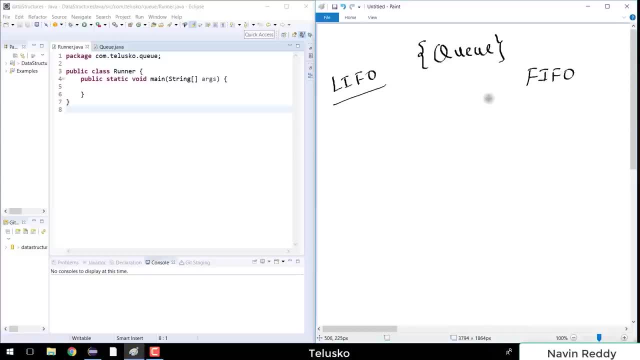 is first in, first out, which means whichever element arrived first will be the first one to go out. So it is first in, first out. Now, in real world, you can see that if you want to take a movie ticket, you join a queue right. So whoever- 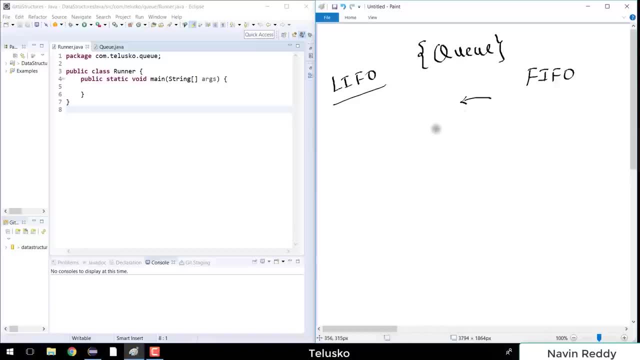 arrived first will get the first ticket In a queue. what we do is we have, let's say, we can implement this with a with a different concept. we will be implementing this with an array, So you can do that with the help of array or you can do that with the help. 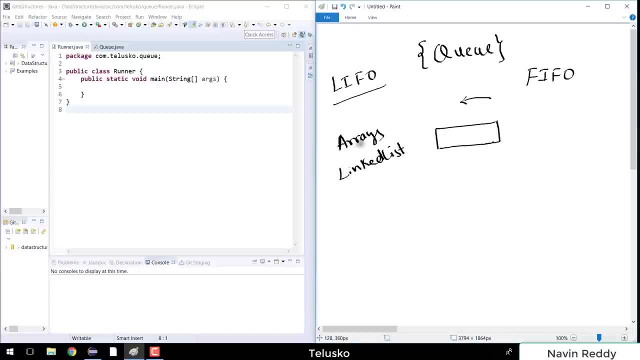 of linked list. In this example, we'll look at how do we implement that with the help of array. In fact, in array itself, we can go with the flat array or we can go with the circular array, But we'll see the difference. Now let's have the array of size four, where 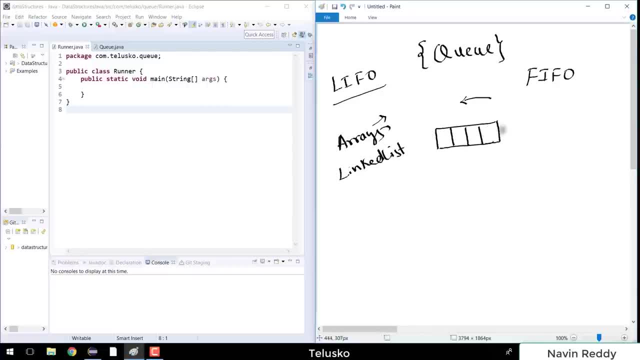 we have four elements In this array. you'll be having to end the end from where you will insert the value and the end from where you will take out the value. So this is your insert. So this is where you will insert the element and this is where you will take out the element. 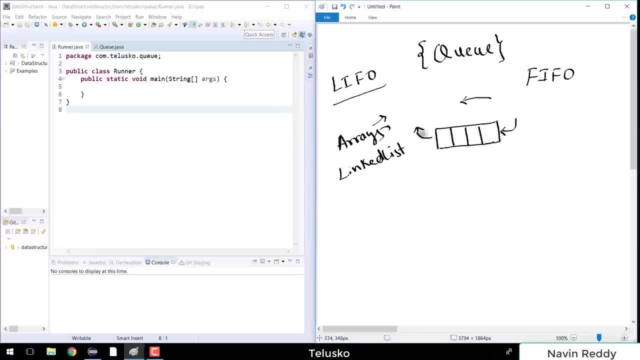 And that's why whichever element reaches first in the queue will be the first one to go out. Now let's say, if I insert a value five, so the five will be coming from here, it will go in this area, So the five will be saved here The moment you insert a new value. let's 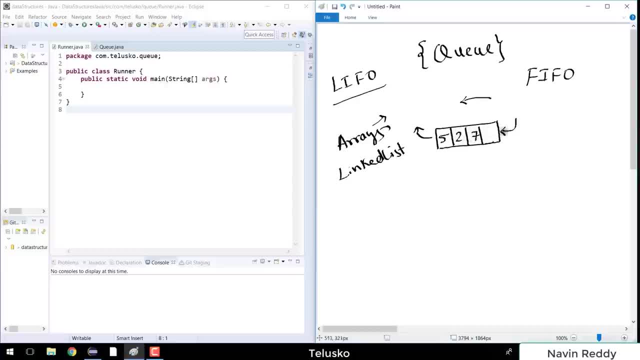 say two, it will go here. Let's say: if I insert seven, let's say five, let's say six, let's say it will go here. And let's say: if I insert three, it will go here. So this is how you. 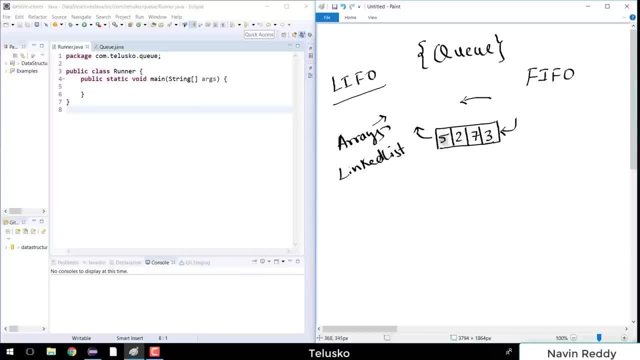 add the elements. Now, if you want to delete the element, so this is the first element which which go out. So five is the first element which go out, And then all this element which is two, seven and three. they will shift on left hand side, So two will come here, seven. 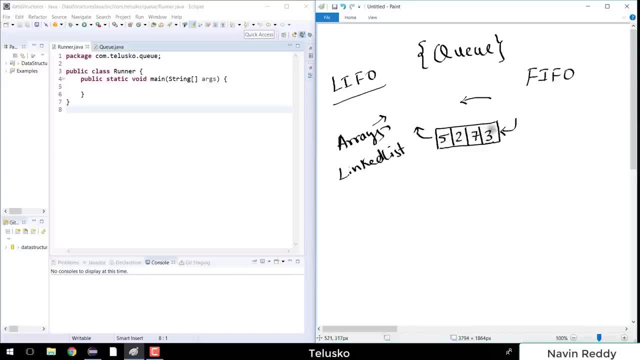 will go on the place of two, and three will go on the place of seven, And then you can add one more element at the end. That's what we're expecting from queue. So in queue basically we have two, and one is from where you will insert the value. 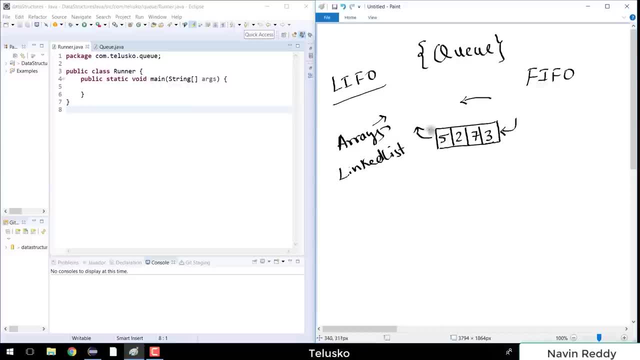 And from where you can take out the value. So you can call this, this area or this thing called as front, And this is the rear end from where you're inserting the value. Now in queue, we can perform certain operations, So you can insert the values and you can remove. 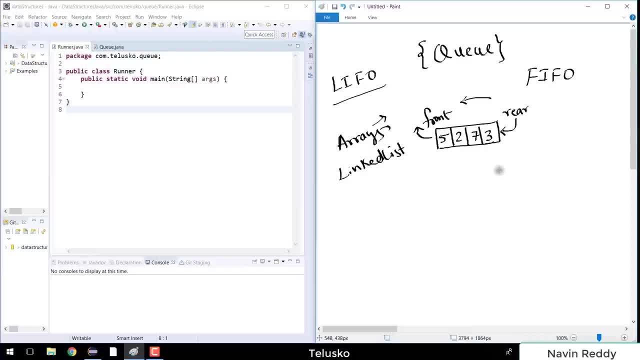 the values the way we did with stack. In stack we use a concept of pop or push, So push would be inserting values. in the same way, in queue we use a different term, So that term is enqueue. So enqueue is like inserting, or in stack. 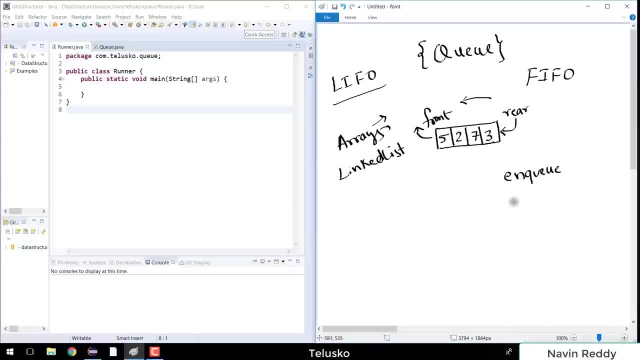 You can say push If you want to remove the element. we use a word called as dequeue. So we have a concept of enqueue. So you can represent insertion with the help of enqueue And you can remove the element with the help of dequeue. Now, of course, enqueue will take. 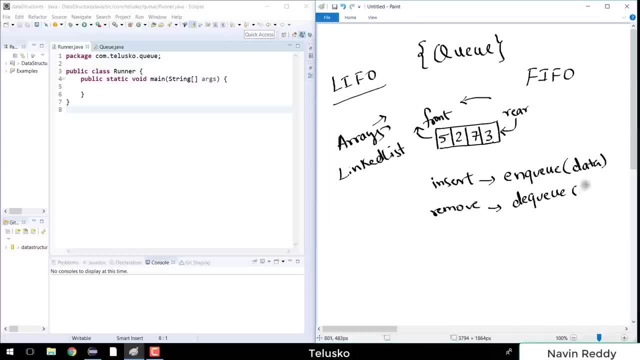 an element from you. So you have to pass a data and then dequeue. don't pass the value, but it will return your value. So let's say, if you say dequeue and your front is five, so it will give you five, But let's say after: after that also you're saying dequeue it. 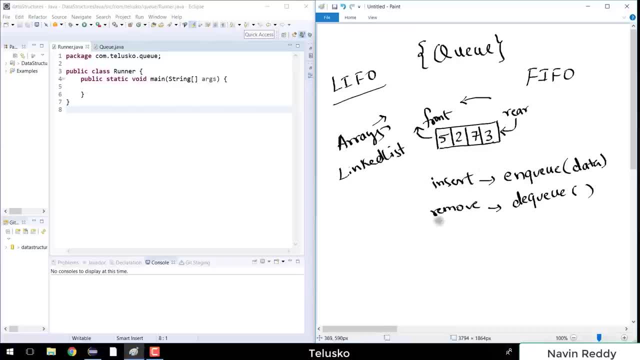 will give you two. So these two methods, we can implement some more methods as well. Example: we can implement a method of size, which will give you the size of the queue We can implement is empty if to check if it is empty. These are two methods we can also implement in this We. 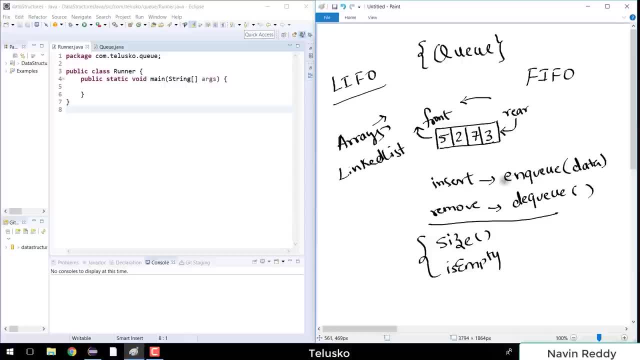 can also implement peak the way we did in stack. you can get the value which is going to be removed. it will not remove the value, but it will. it will show you which is the value which which is going to remove. Now, how do we implement this? So first step would: 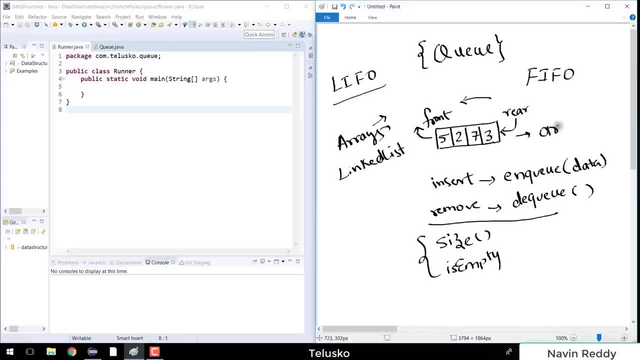 be. we need to create an array, So we have to create an array of size five. I love this number five, So I will go for the array of size five, and then I will try to add the element. Now how many variables we need here? So basically, we talk. 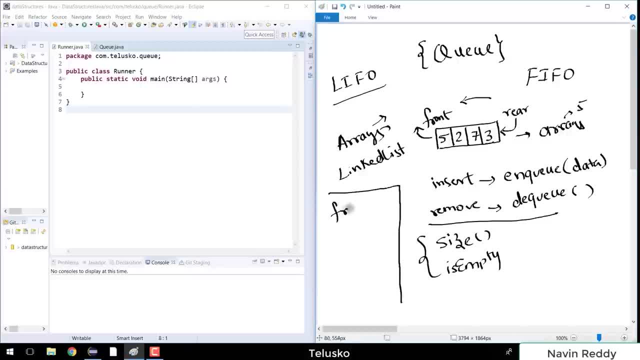 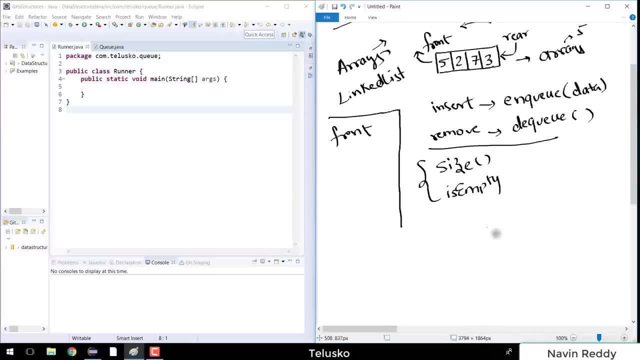 about this implementation. maybe we need a front variable which will have the index number of the front, Because every time so initially, when you don't have the value in this in the queue. so example, if I create another queue here and if I say the queue is of size five, so 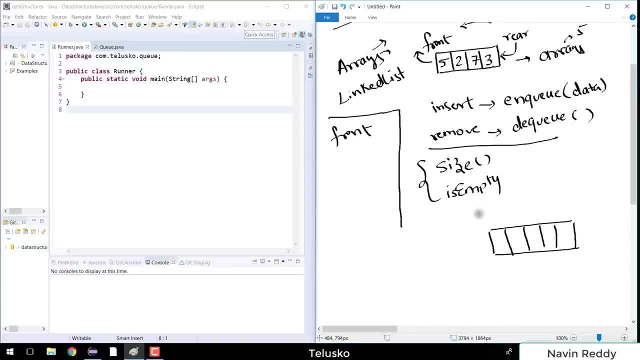 in a size of five. so when you what you don't have any element, of course the front and rear both will be not be referring here. but then the moment you add a value, front and rear both will refer to this value. so this is your front and this is your rear, but the moment you add more values, 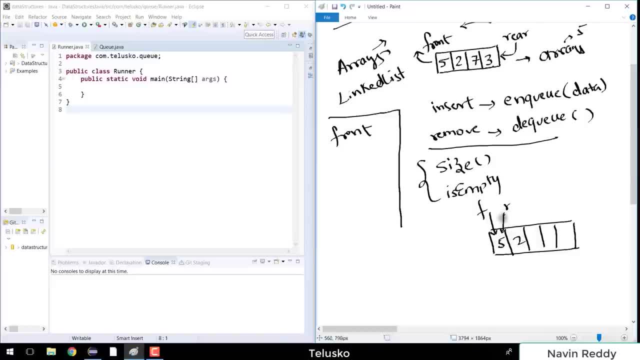 let's say, if you have entered five and then two, the rear will be pointing at this point. in fact, the rear we have to shift to this point when you insert two so that you can add three, so rear will shift here. so every time you add a value you will say rear plus, plus, and every time you delete the. 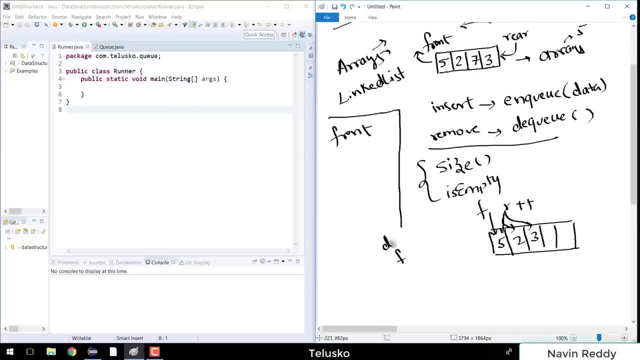 value, you have to say front plus, plus. so when you say delete, you have to say front plus plus, and when you want to insert you will say rear plus. we'll see the implementation and then you will understand what i'm talking about. so i will go back here in the queue and so you can see i have 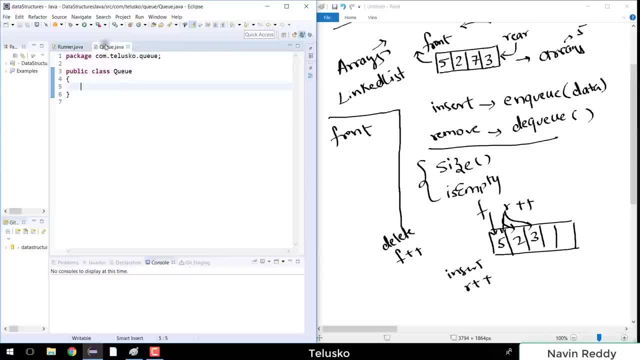 two classes. one we have is runner class. another we have is a queue class. i will go to queue and let's try to implement those methods. the first method we have to implement is nq. oh, before that we need to create some certain variables. the first thing would be: 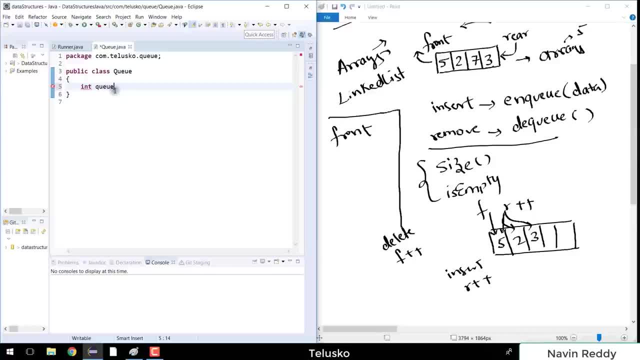 i want to create a queue itself. so i would say queue, and the size of this queue would be, let's say, five initially, or this is not what you do it. so you say new ain't, and you specify the size: five. you can make it dynamic, your choice, but initially i will go with the static one or fixed one, so that 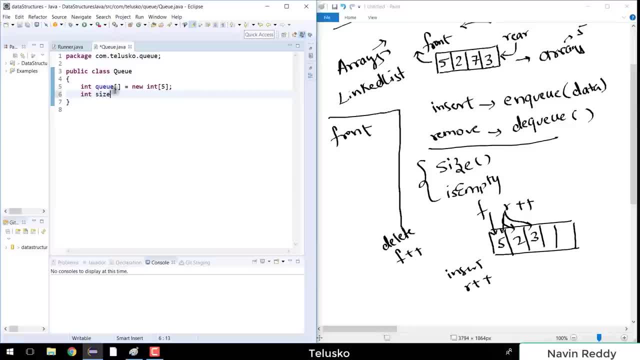 it will be easier for you to understand. and then we need three variables. we'll say size, one of the variable, then i need a variable which is front, which will refer to the front element, and then i will need a rear element which will only a variable which will refer. 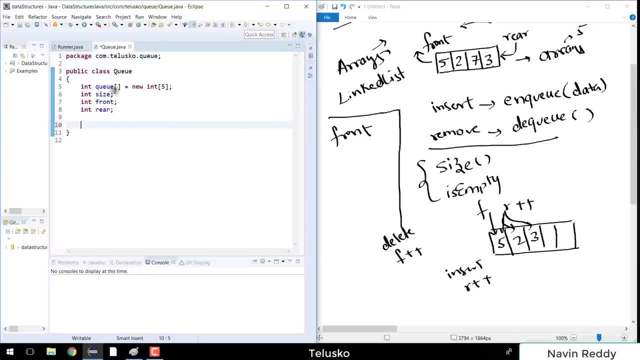 to the front element, and then i will need a rear element which will refer to the front element, and then i will need a rear element which will refer to the front element, and then i will need a rear element which will refer to the rear element. once you got these four variables and, of course, 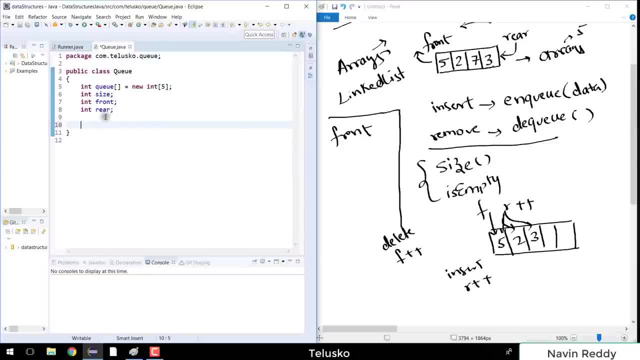 the value for this size would be zero, front would be zero or there will be zero, and then i will create the method. so the method name is public void nq. this is my method, which will take a int data and then i will try to insert a value here. now how do we add the data into a nq? so for 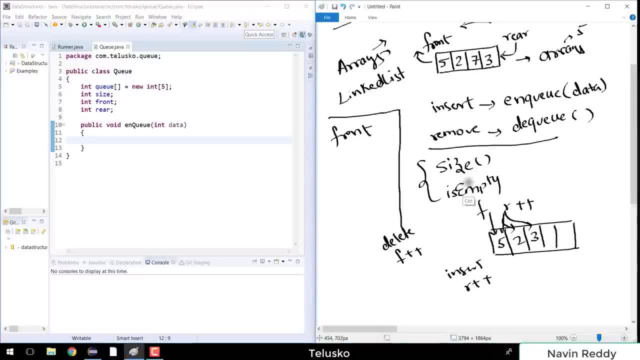 that i will go back to my this point and let me just make this an empty, empty queue. okay, so you can see that we got a empty queue here. so the name of this queue is queue itself. and now i want to insert a value. so let's say, if i'm inserting a value which is five, 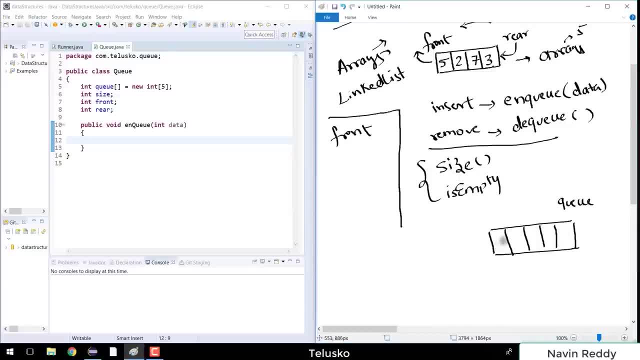 so in this queue, at the index value zero, i want to insert five. now, if you want to insert the value we use, a variable which is real and by default real has the value which is zero. in fact, front will be also referring to the first element as a at this point. so we'll say front is also zero. 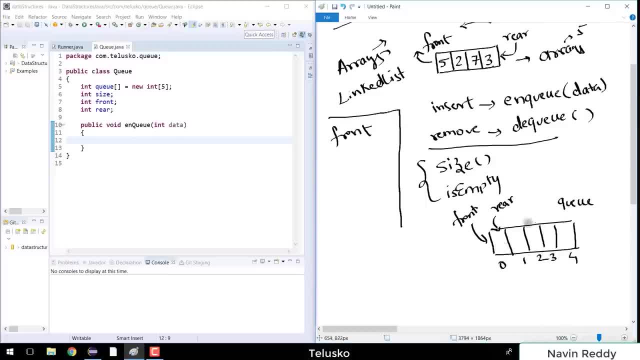 index number zero, index number one, index number two, three and four. now, front and rear. both will refer to the same element here at the end, now, the moment you add five. so at the rear end you're going to insert five. so at the rear point you have to insert five. now how do we achieve that? so in the 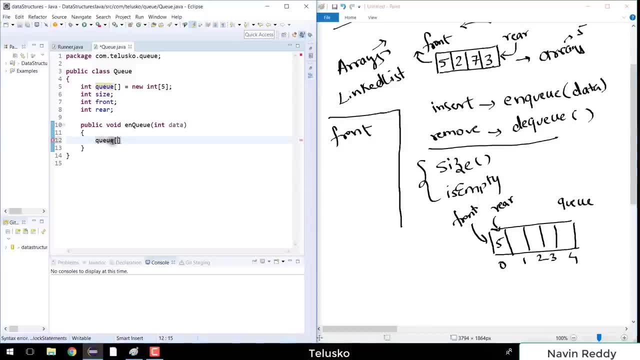 code itself, you will say: q of rear is equal to whatever data you are passing. so the data i'm passing is data itself. now, once you have added the value, you need to do one thing. after adding the value 5, you just need to shift your rear to the next location, which is here. and how do we do? 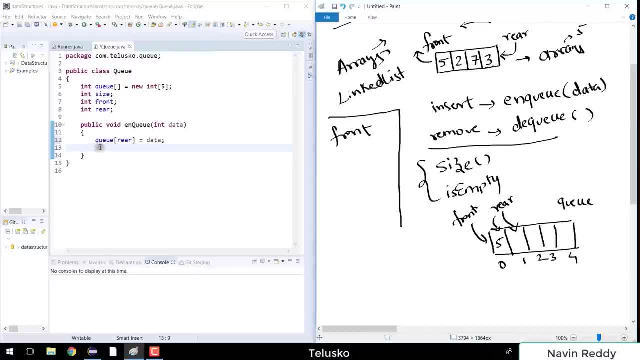 that. how do we shift our rear? it's very easy. you simply say rear plus plus. so you will say rear is equal to rear plus one. or you can say plus plus. that's fine. and then, once you have added the value or incremented the value, now also want to increase the size of it. right, so now the size is size plus. 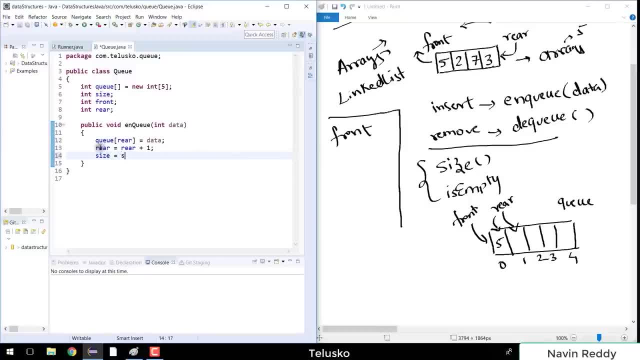 plus, because we are not. in fact, we can write size equal to size plus one, just to maintain the same sequence. so we have real equal to real plus one and size equal to size plus one. so every time you add the value, the size will increment. it's that simple time, and let's work with nq and then later. 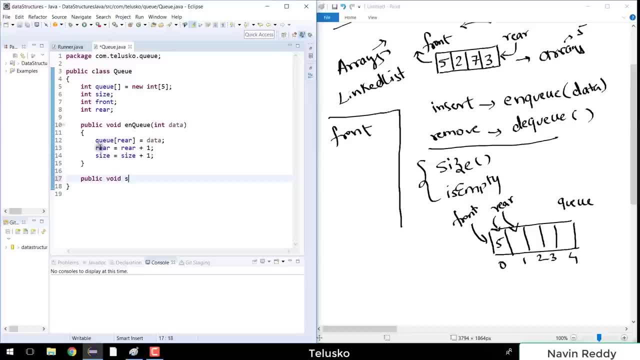 we'll work with dq. i want to see the element as well. so let me say, i want to create a show method which will print the elements. so we also need one more method here which is show, so i would say show method as well, and show is responsible to print all the elements. and in this show, if i want to print elements, it. 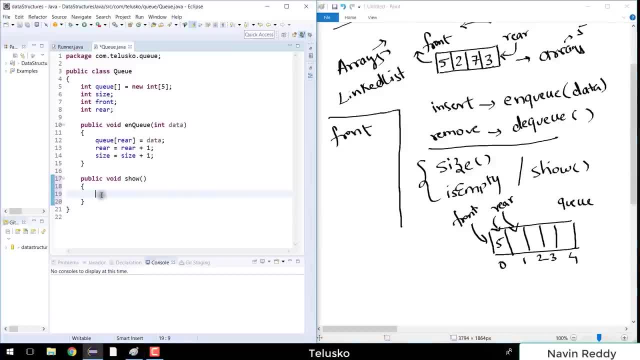 will print all the elements in the from the queue. but how do we do that? so what i will do is i will say for loop. i will start with zero initially and then i would say, okay, till what point we have to go. i have to have to go till size right, and then plus, plus, because the size of the array may be so. 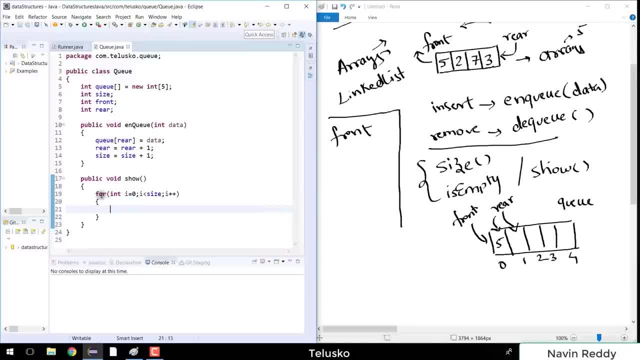 you have inside a three value, so the size would be three. so you have to go till i- less than three- and every time you go there you just need to print the elements. and the way you can print the element is by saying the value q of i, and then you will also print a space after that. and here i want to print. 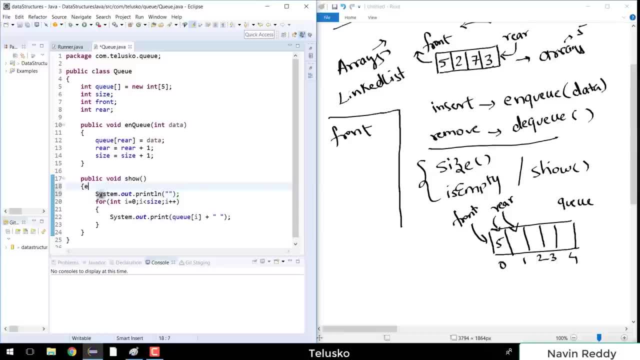 the elements. i would say system, dot out, dot print, and then i would say elements, elements, colon. so it will give you a good format of printing. i don't want a printer in there. that's it, it will work now. so we got nq, we got show, now how do we verify? so let's go to runner and in this runner, let me create. 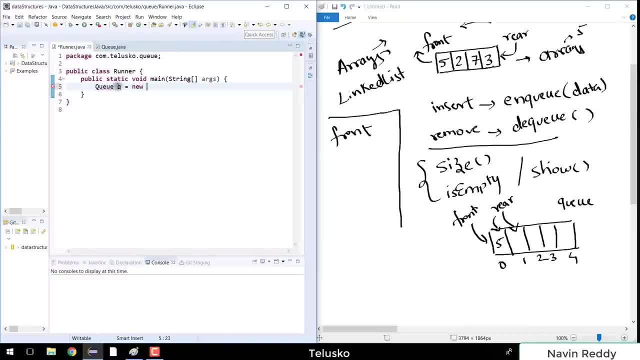 object of q, i will say q. q is equal to new q. i got the object which is q and in this q i will add the element. i would say uh nq. i want to enqueue the first element, which is, let's say, five, as we have. 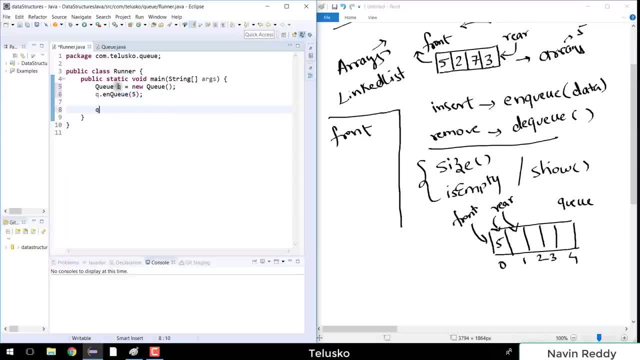 done here. now, after inserting five, i will just simply say q dot show. i want to see how many. and if you run this code you can see we got five. we got only one element. that's perfect. let me just add one more element here, and that would be two. in this case, i would say: 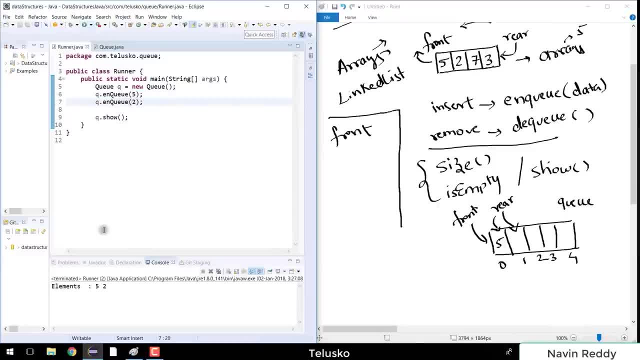 two here. and when you say two, if i run this code, you can see we got five and two. so every time you insert the value, it will, it will get added in the queue. but question arise: how will you remove the element? and what happens when you go beyond the size? let's say, if i inserted seven values, what? 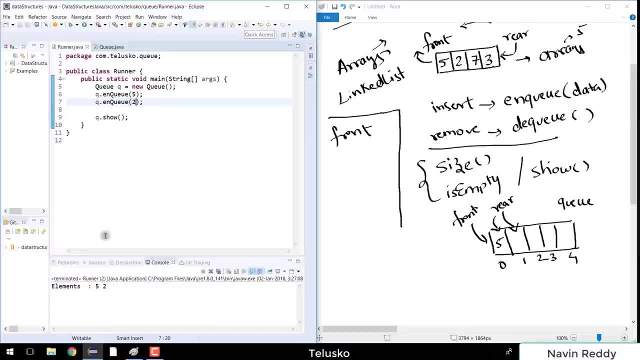 will happen and, of course, if you insert seven values or six values, it will give you a very error or the exception, which is array index out of bound exception. till this point we have only inserted the values. now how do we remove the values and how do we avoid the exceptions? 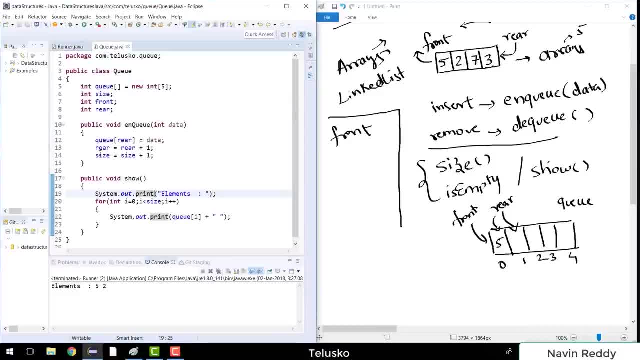 so let's try to delete the values. and how do we do that? it's very simple. just go back here and we just need to implement one simple method, which is dq, so i would say public, uh, it will return the values. i would say dq, and it will take. 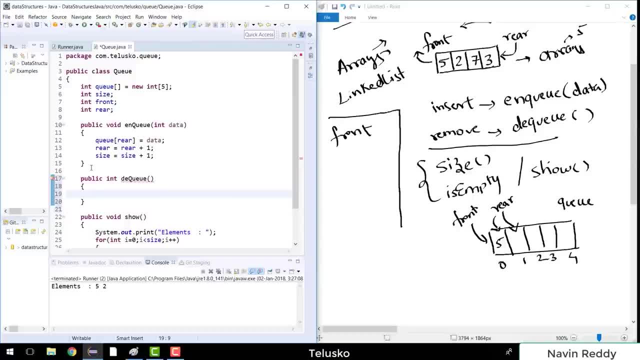 it will not take any parameter. now how do we remove the elements? it is simple, right. so just go there so say i have inserted two values. so we got five and two and let me just insert some more values. you know, i will just try just to explain this in a better way. i would say, i want to insert some more. 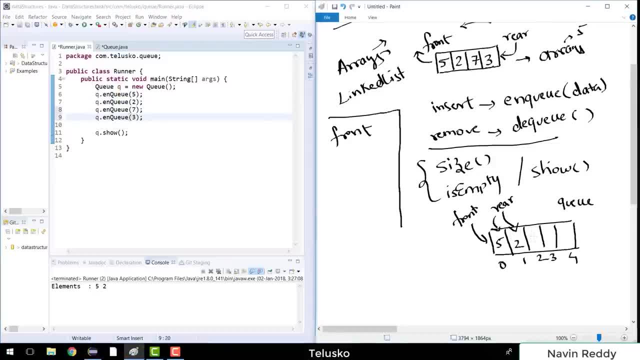 values. so in this list, in this queue, we got seven and three right, so we got these values. i want to say dq now. so the moment you say dq, what should happen is it will remove five from the, from the, from the queue, so it will remove this five. now, when you say removing the value, maybe you will. 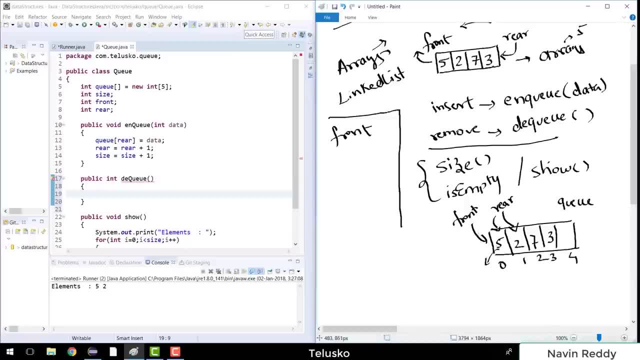 not remove the value. the only thing we have to do is we just need to move our front from this point to this point. so we just need to move our front, right, that's, that's enough. so i would say: hey, front, just go to two here. okay, that should work. i mean, we just have to increment our front. so 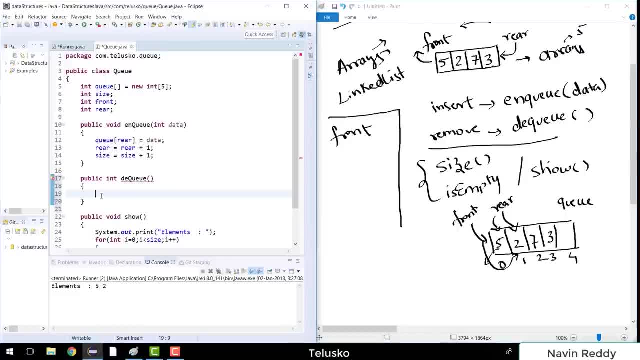 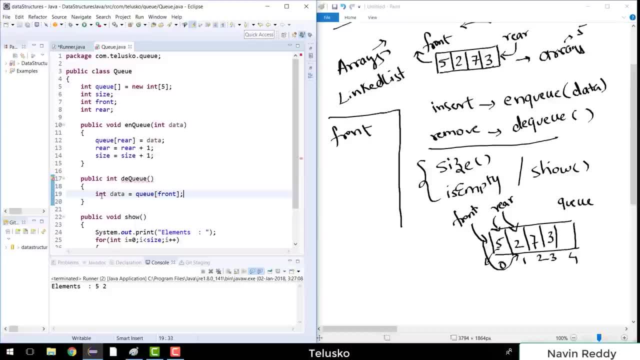 give me your value, so front will have. front will be index number zero, so it will give you the first element, which is five. that simple. and then every time you fetch the value of, we have to return the data as well. so we return the value here. but it's not just about returning value, we have to 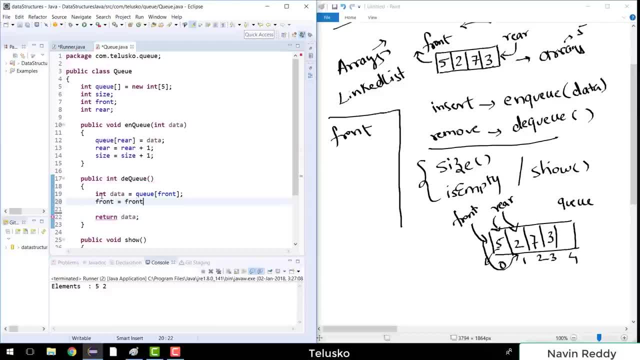 move the front to the next location. so how do we shift? we say front equal to front plus one. is that simple? and and once you do that, we also need to reduce the size of it. so we'll say size minus minus. we can say size equal to size minus one, just to keep the same syntax. yeah, so we'll say size equal. 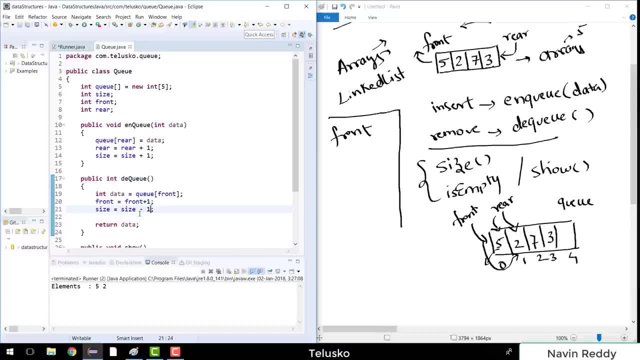 to size minus one. so here we are saying size plus one, here we are saying size minus one. that's it. it's so simple. let's go back here now. you can see we have inserted five values and before calling show. in fact, if i call show at this point, you can see it will print all those. 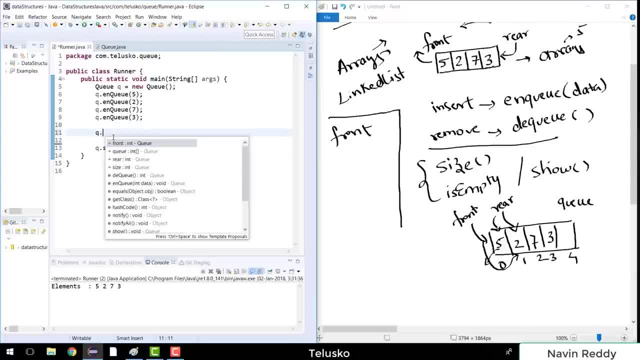 four values. but if i say dq, so if i if before i print all those four values, i can print all those four before saying show. if i say dq and if run this code, you can see we got five, two and seven. oh, we got a problem here. we are not able to remove the last element. we have removed the front as well. 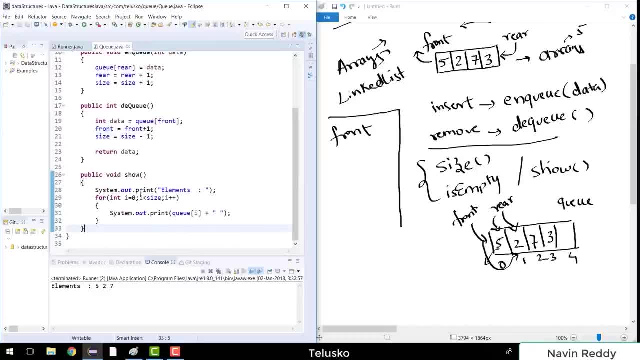 so this is some problem with the front. the problem is, you are starting from zero and you are ending at size. right, that's perfect. but then you cannot simply say i here, you have to say front plus i, because we are shifting the front as well. right, so you don't want to start from zero and you are 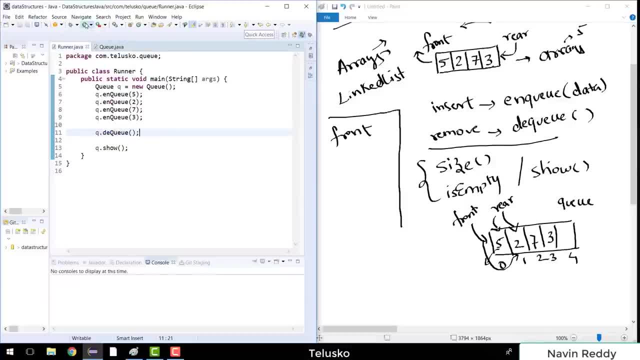 starting from zero. you have to start from front, and now, if i run this code, uh, you can see this is what we're expecting, right? we got two, seven and three. we are removing the element which is five. it's so simple. now, if i try to do this one more time, if i say dq and you are guessing it right, 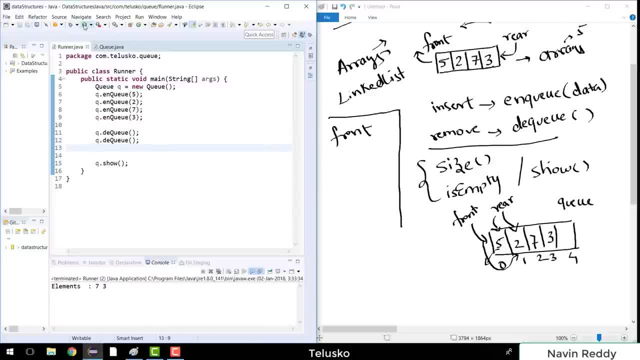 we will be getting only seven and three. so if you, if you run this code, you can, you can see we got seven and three. so this is how you nq and this is how you dq. now, after dqing it, what we are thinking is we only have two elements, right? so in an array we have 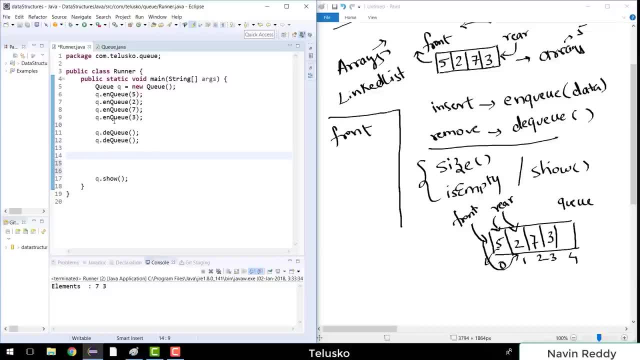 only two elements. but that's not the case. let me prove it. let me just add two more elements at the end. now, of course, it should work right, because in total, when you say dq, in total you have two elements and i can insert two more elements. there i can say: i want to insert nine, i want to insert. 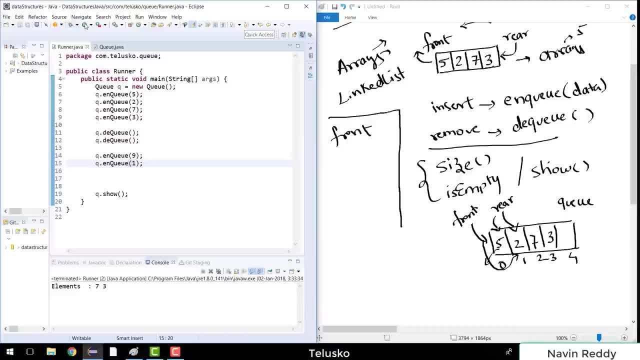 one. so this should get added right. but the moment i run this code, we got an error, which is array index out of bound exception. why? because even if you are dqing it, you are not removing the elements, shifting the pointers. in total, you have four values there. in fact, after these four values, 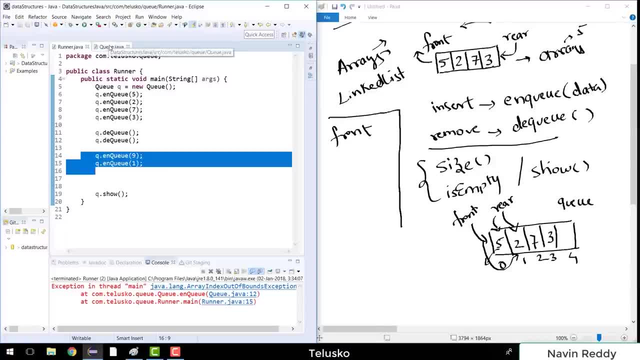 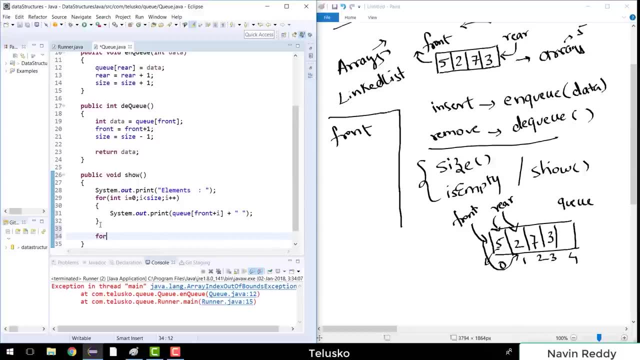 you are adding two more elements. just to prove my point once again, i will go back to this show and at the end, when i say show, at the end, after printing the values, i want to print the array as it is. and the way you do that is: we can use enhanced for loop or we can use normal for loop. 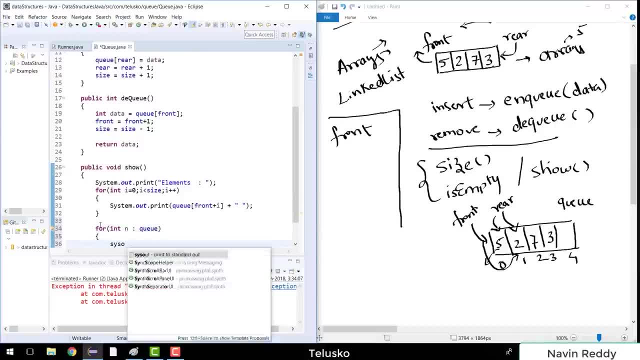 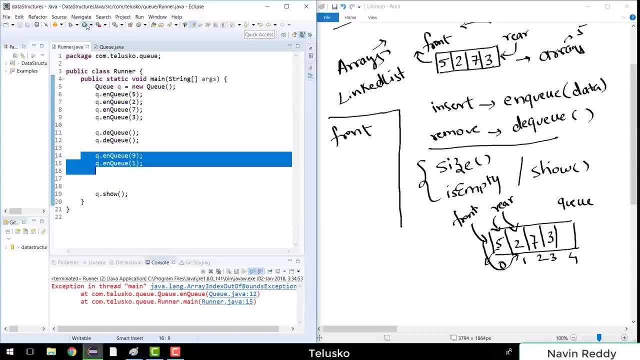 as well. i can say q and then i will print the element of n with a space there. now, if i run this code, you can see: oh, we got the exception. uh, let me just, let me just not do that here. i'll say comment and let's run this and you can see we are getting. oh, okay, i just forgot one. 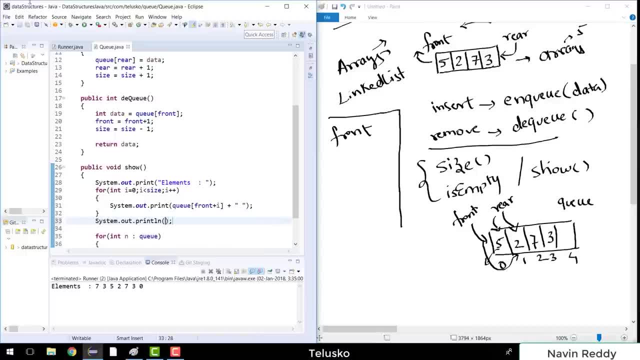 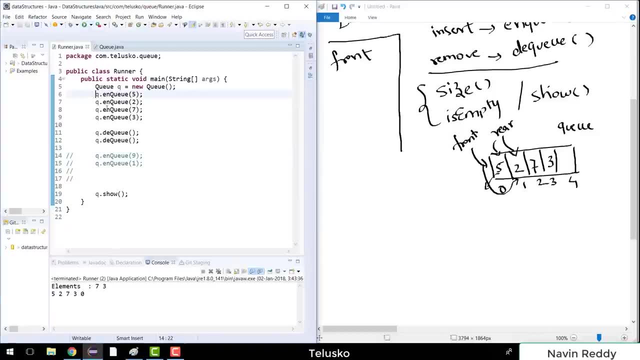 more thing: we just need to put a new line in between so that we'll get a difference. and if i'm this code now you can see. you can see it is working at this point because you are entering only four values and the size of the array is five. so you're inserting four values. you're trying to. 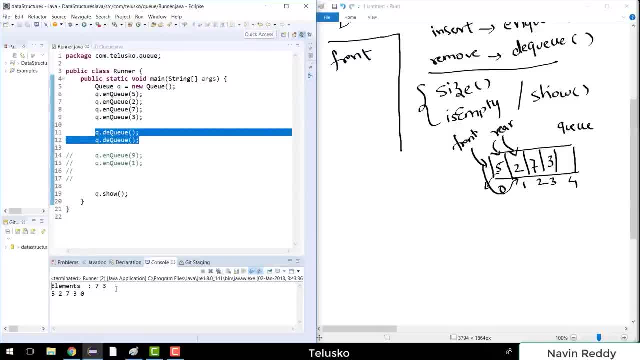 so in total you have two values which we are getting, but in array we still have four elements, and that's why, if you try to enqueue two more elements there, which means you are crossing the index value, which is four, five. so in this way, last would be four. right, but the moment you try to add, 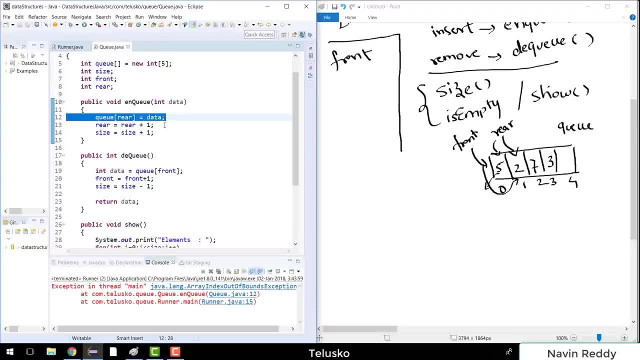 more elements, it will give you error and, as you can see, we got error at this point. you cannot go beyond that point. in fact, the exact error would be at here, because nine will be inserted, because we have space for that, not this value. the problem is arising because of this real value. 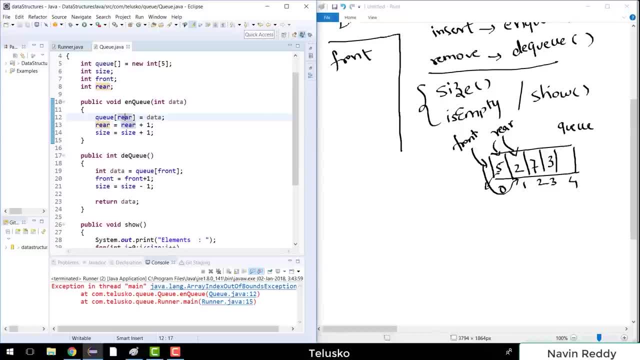 because if you cross the fifth value, which is this: one index value at this point is four, and after that the value for rear becomes five and we don't have any element after that, and of course the size of array itself is five. you cannot go beyond that at this point. what i want is i want it to go back. 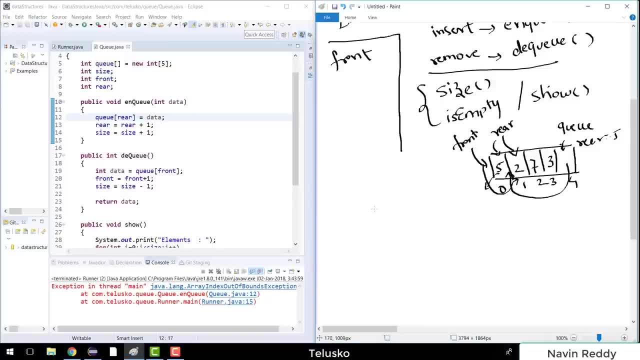 on this first one, which is you can imagine this array in not as a linear array but as a circular array. now, this is just a representation, so you can imagine we have an, a circular array, which we have. we have the first one, in fact five elements, uh, this third one, so four and five, let's say we have 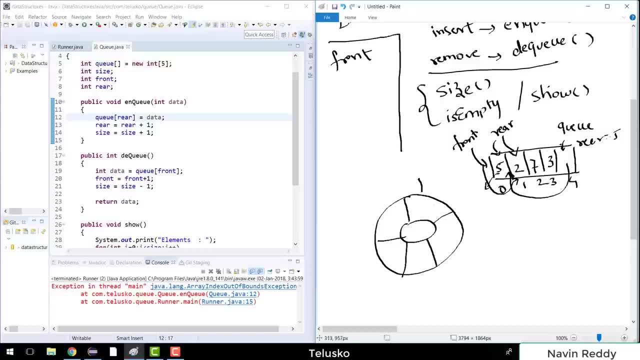 these five elements, so the initial, so the starting value would be here. so this is, let's say, imagine your front and this is your rear itself. every time you add value. let's say, when you add value five, it's here. the value will become two here, and then seven here, and then three here. now, if you try, 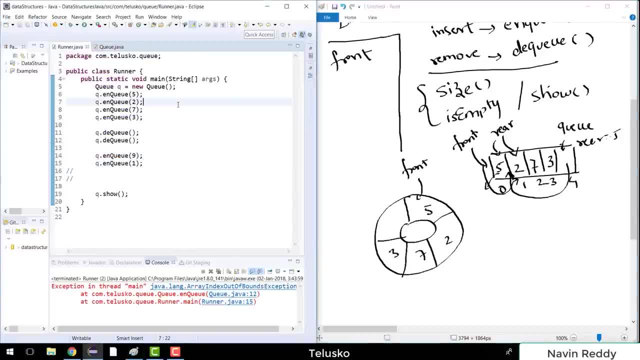 to match this with the runner. what we just have to do is imagine this is: index value zero and index value one, index value two, index value three and index value four. imagine this is how you work with, and then, after four, i want to go back to zero. uh, how do we do that? that's a question. so the moment. 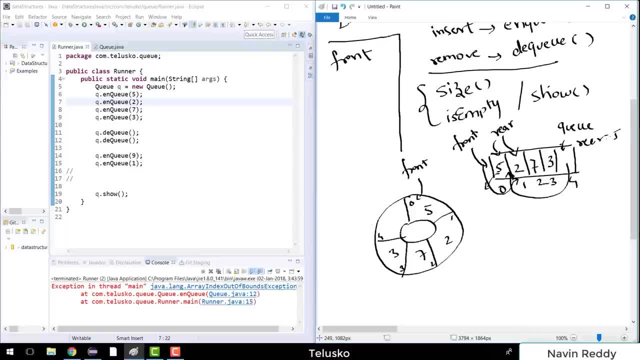 you add these four values, we have added those four values. and then when you say dq, it simply means you just need to shift your pointer right. so your front will be shifted to zero and one. so it will shift it two times and your front will represent the seven value here. so this is your front now. 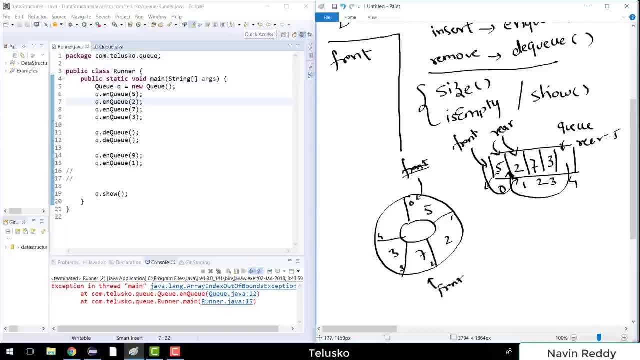 this is no more your front now. what about the rear value? so the air will shift here. so this is where your rear is now. if you add a value here, which is nine, it is getting added. what about this one? the moment you try to add one, it will try to go on index. 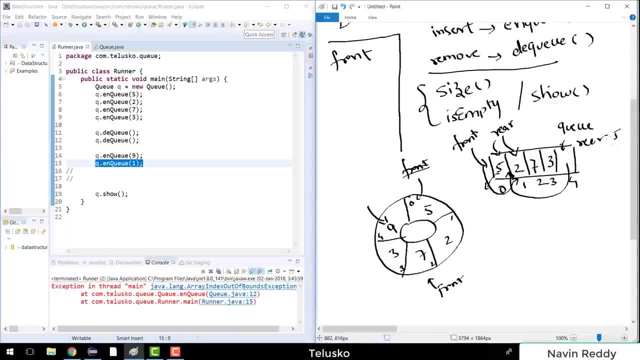 number five. we should not be going for index number five. we need to go to index number zero. that is where you call it as a circular array. so after four the index number will go to zero. that's it. if you can achieve that, your job is done. oh, now that's a question after four, how can you make sure? 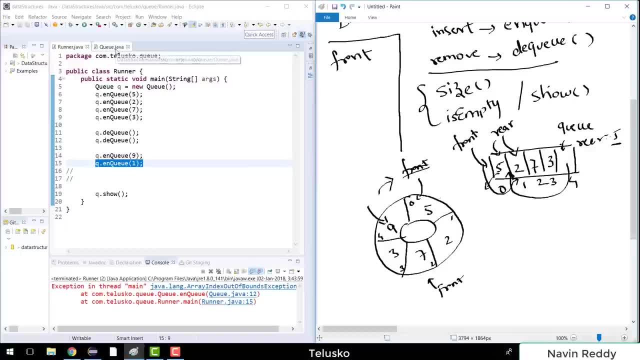 that your value becomes zero. um, okay, so let's try. now when i say uh, zero, so can i apply this operation? because when i say yeah, so when you say five mod five will give you zero, right, because zero is a remainder. so five mod five is zero. now, when your, when your real value is equal to one, one mod five is equal to one. 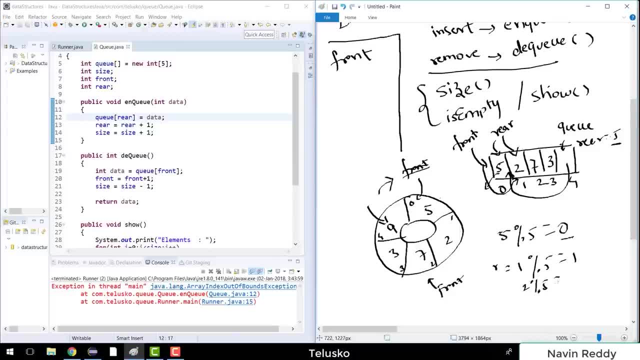 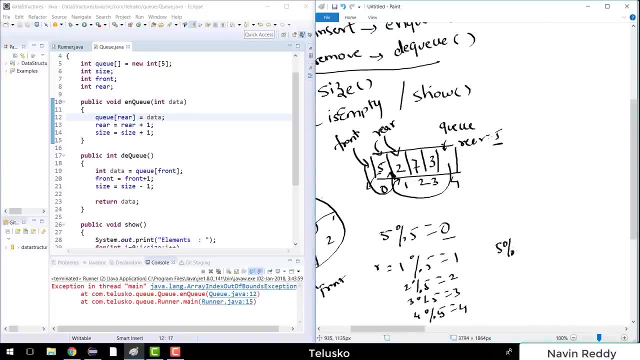 uh, when your r value is two, r mod five is equal to two, then three mod five is equal to three and four mod five is equal to four. and then here is a twist: now, if you say okay, now if you say five mod five is equal to zero, that's the beauty. we wanted zero right, and we got zero after that, when 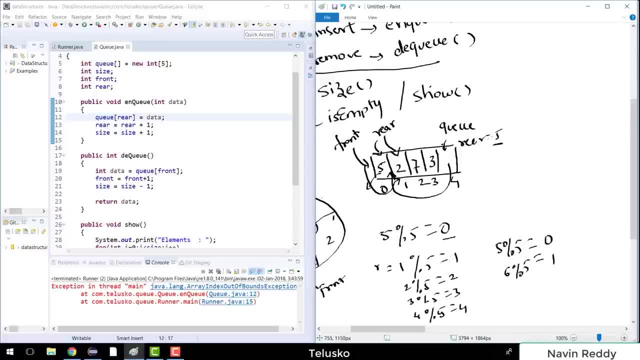 you say six mod five is equal to one. that means we are going to the same loop. so only thing that you do is every time you perform this operation you just need to do a mod of five. so if the size is five, you will say mod of five. 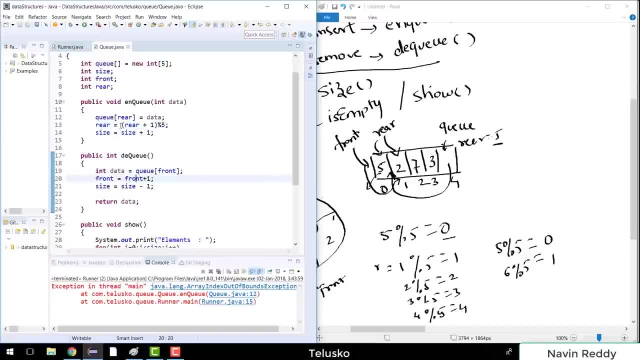 same goes with front every, because the front also should be in the loop, right? so you will say front and you will say mod 5, that's it. this is what you do now. if i run this code, it should work and you can see it is working. oh, it's not working. we still got an exception. but why are we doing in a perfect? 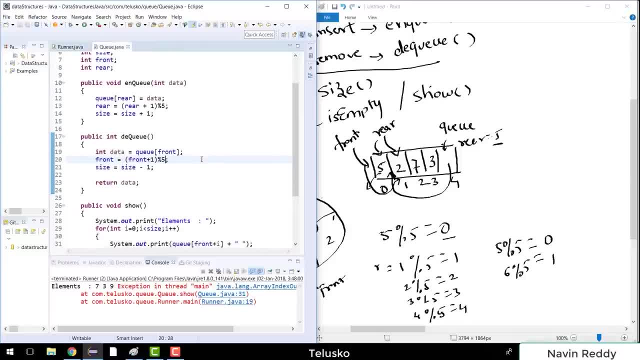 way? yes, we are, but it is giving you error while printing. i guess that's the issue. if i go back to runner, yes, the problem is because of printing. so if i go back here in printing as well, i need to run that operation. because you don't want to say front plus i. you want to say front plus i mod. 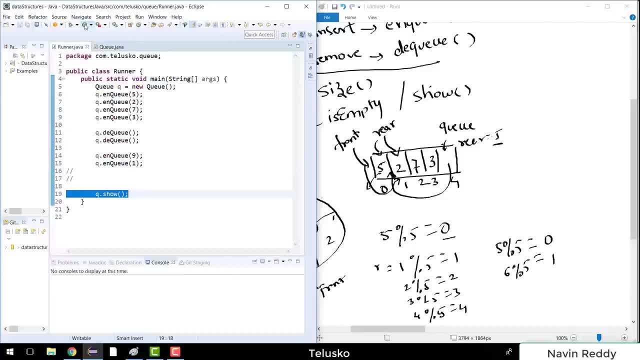 five, because i don't know the current value of front because it is going in circle. so i will run this code. you can see it is working. you can see we got the value, which is seven three nine one. this is the exact loop. can you see that it we got seven, three, nine and the next two elements. 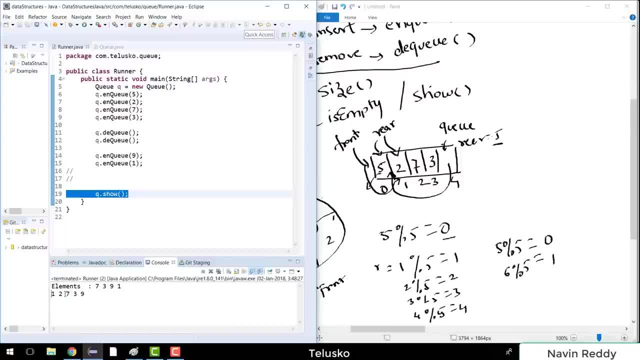 are coming here, which is one- i mean nine and one, this is two- is the previous element. it's so simple. that's how you can work with the circular loop. but we still have one issue: what if we try to add more elements? in fact, i will say copy and paste, let's see what happens. i'm trying. 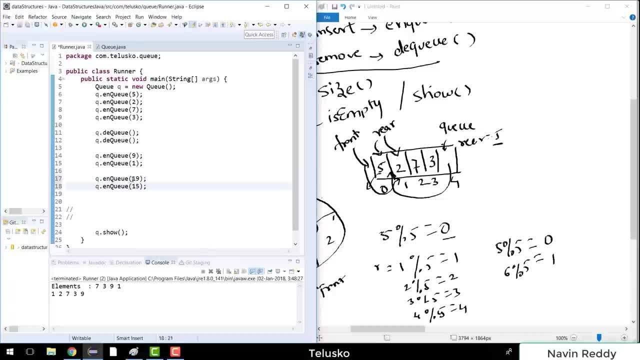 to add two more elements, which is 19 and, let's say, 15.. so we wanted the value here, which is 73. okay, these two values, because we are removing these two values. right, five and two because of dq. so these two elements and, uh, this four elements. in total, we have six elements. let's see if it is. 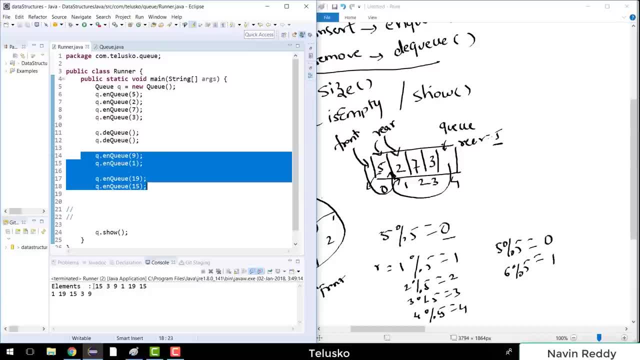 working. and oh, it's working. you can see there's no problem and your, it is getting increased. oh, that's okay. you see that the elements, the other size is five and we are getting six values. it's because of the loop. so till this point, we have seen how to add the element and how to remove the element from. 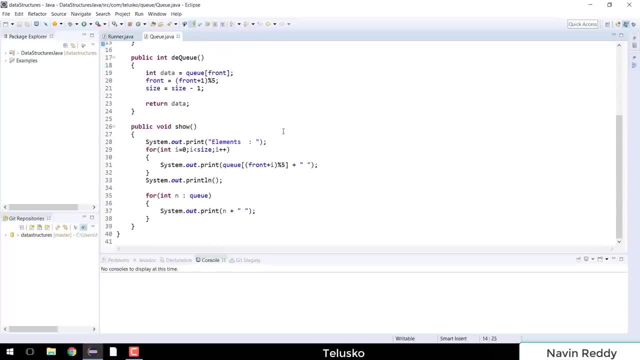 a queue. we are here to add some methods, some methods like size of the queue. then we want to know: is the queue is full? all we want to know is the queue empty? let's start with the two size method. or the size method. so i would say public, so we return the size, so i would say size, or maybe. 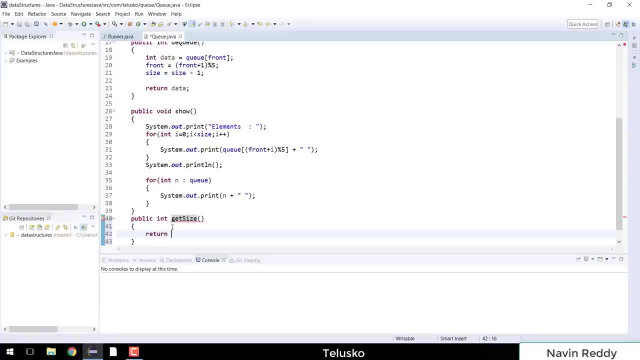 return is simply: it will return the value, which is size. that's it. we'll say return size. and now, if i go back to runner and after doing all these things, you can see i'm adding four elements and i'm removing two, and then again i'm adding four elements, so in total we have six elements there. 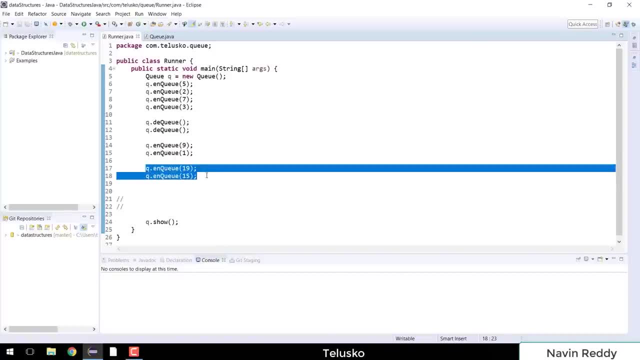 and unfortunately the size of our array is only five. let's remove this as of now. so you can see we have four elements here. we are removing two and then we are again adding two, so in total we have now. if i want to know the size, of course i want to print the values, but i also want to print the. 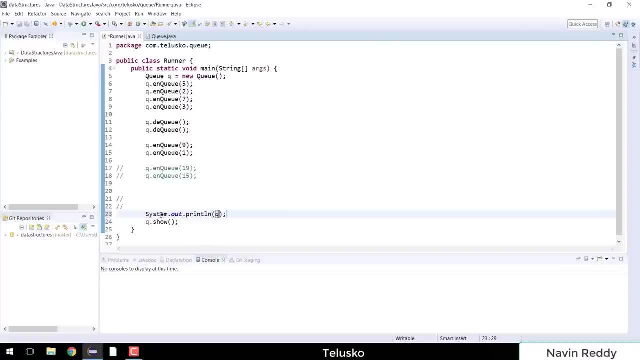 size. so i will, i will say systemprintln and here i would say: uh, the size. and then i will print queue dot, get size. so it will print the size as well. and let's verify if it is working. and the moment i run this code, you can see we got the size as four and that perfectly makes sense. 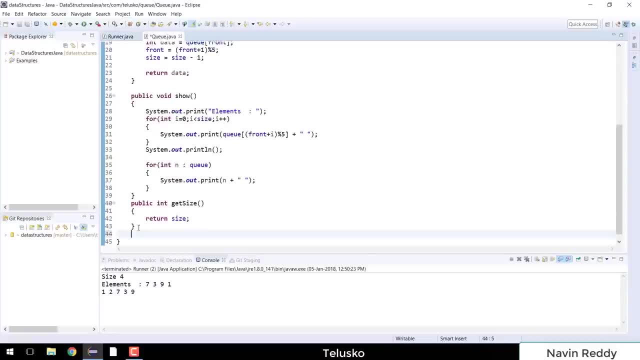 because we have four elements there. now let's use is full or is empty method. so i would say public. now how do you know if your, if your queue is empty? so i would say public boolean is empty. so the way you know that it is empty is by returning. 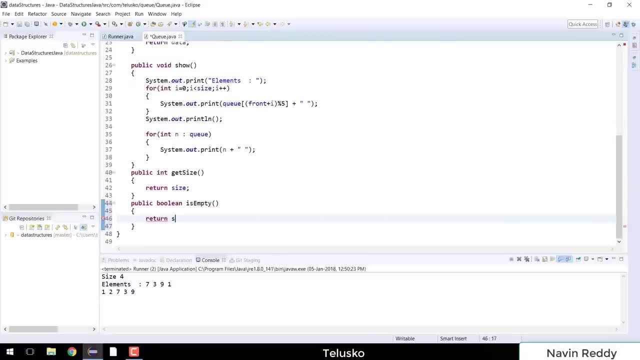 if the size is zero, so we'll say return size is equal to equal to zero. if it is zero, then of course it is empty, right? so that's what we are doing here now. how do you know if it is empty? so let's go back here and i will not add any element. i will not delete any, any element there, or maybe i will. 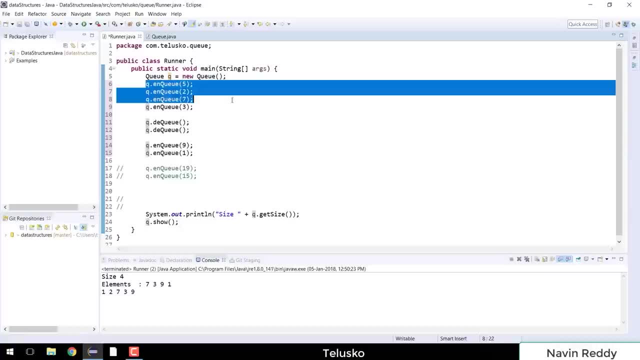 add two, i will remove two. let me just comment so you can see we are into and we are removing two system dot, dot, dot printer, and i would say q dot is empty. so of course it will point: uh, true, so if i run this code you can see we got true. but if you add a value and if you don't remove it, let's say if 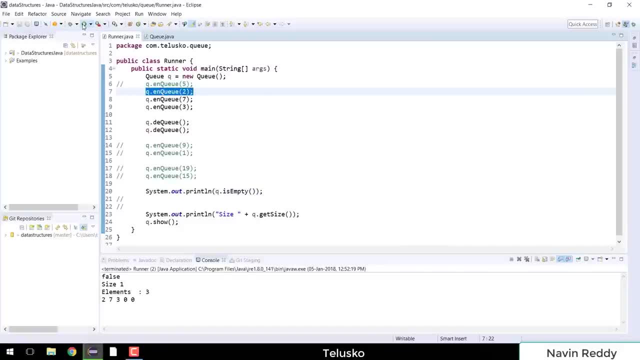 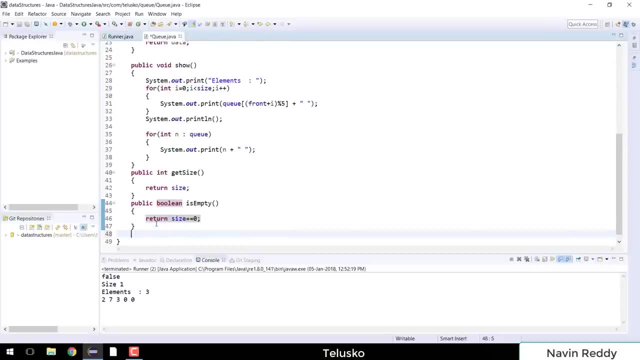 i uncomment this part and if i run this code, you can see we have one element there, so it will print false. so we implemented is empty as well. and now let's go for is full. so it's very easy. let's go back there and say public boolean is full and here we just need to return if the size is equal to 5. 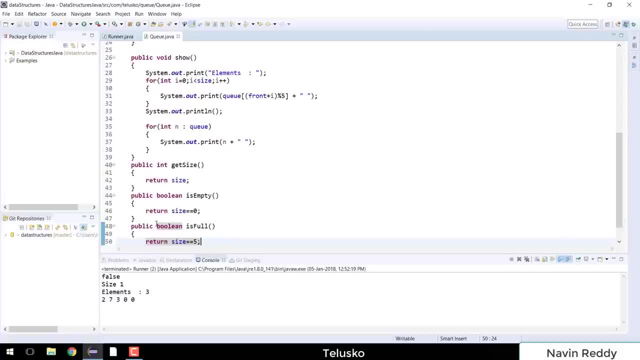 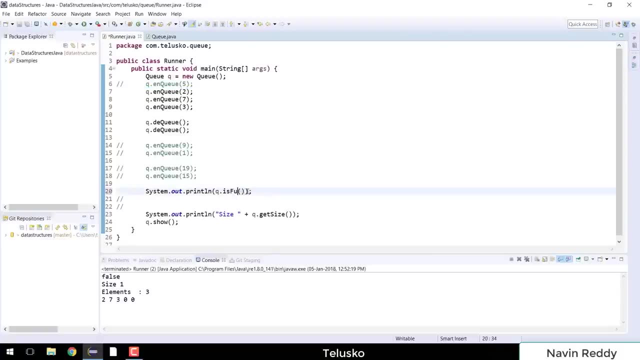 because the queue size is 5, so we'll simply specify size equal to 5.. in case, if you're making dynamic, then you can also use a variable there. let's go back here and you can check if it is full. so we have done with the empty, let's go with full and in full. what i will do is i will add some more. 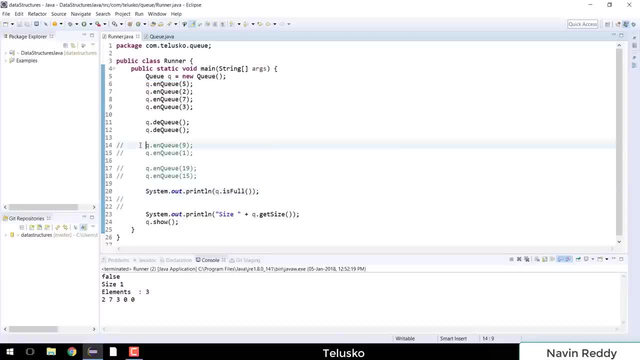 values. i will uncomment this part. and i will uncomment this part because i want to add five values and i don't want any any removal. so you can see i'm adding five values there. the moment i run this code it will say it is full, true. but if i add only four values, it will say it is full, true. 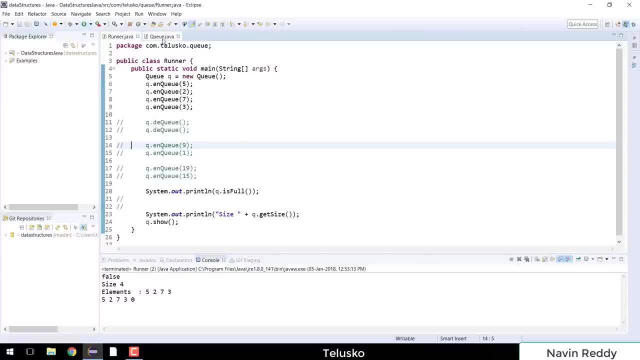 you can see it will print false. it is not full. so we have implemented: is empty is full and get size. now how it will be useful. now, instead of using size here, we can also use methods. normally this is what you do in java. you always use methods to get the value. so you will say: get size. 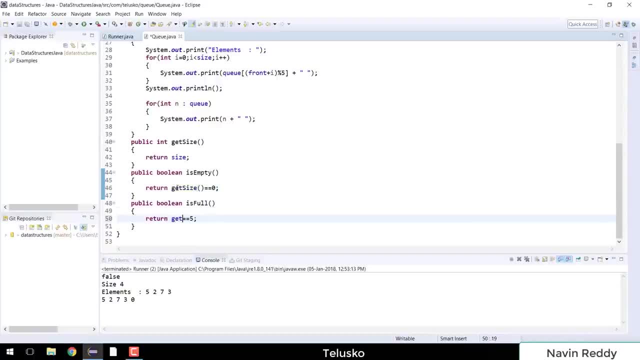 equal to equal to zero. or you will say, get size equal to equal to five. so normally we check with size. that's one thing. the next thing would be whenever you want to add the value. so before adding the value we have to verify: if it is not full, so we'll say. if it is not full, so we'll say. 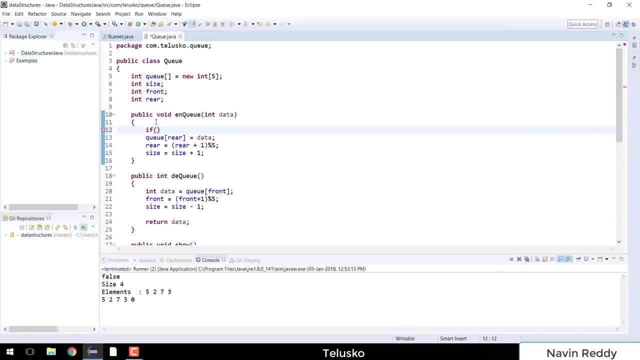 if we have to do, we have to do this only when it is not full. so if it is full, how do you know? if it is not full, so we'll say: is i mean not, is full, then only you have to execute this statement, otherwise you will print else message, you will say else and you will plant the queue. 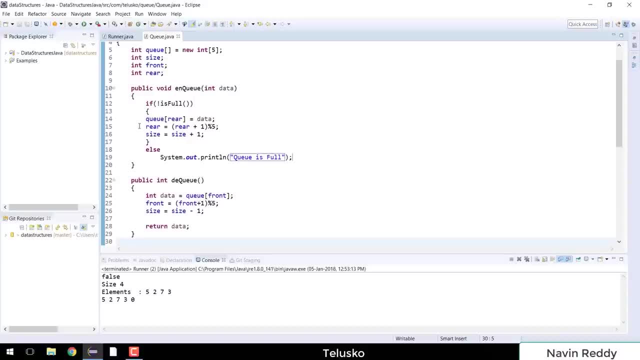 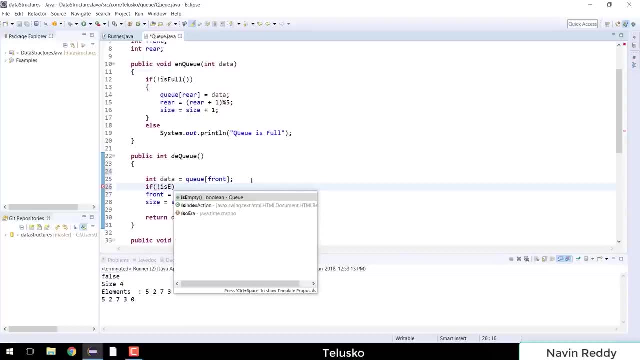 is full and here also okay, we have to just format the code to look at good. and in dq as well, we want to remove only when it is not empty, because if it is empty, then why what you will remove, right. so we'll say if is empty, and this code will be. 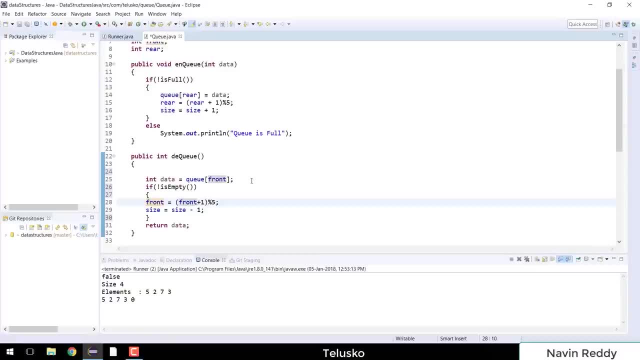 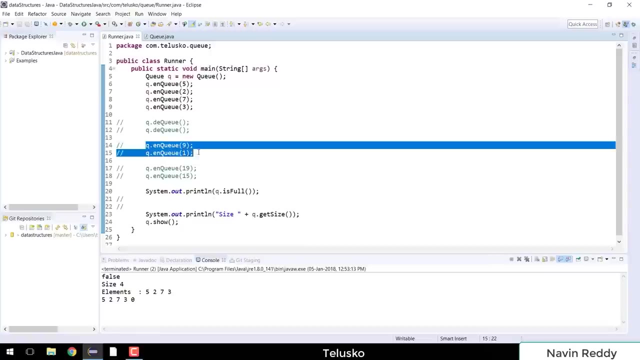 executed only when it is not empty, otherwise you have to print a message. i will say first of all this format, that, and in else part i will print: q is empty, simple, right. so here we are checking: it is full, or is it? is it empty? here let's go back to runner and i will try to add more elements now. 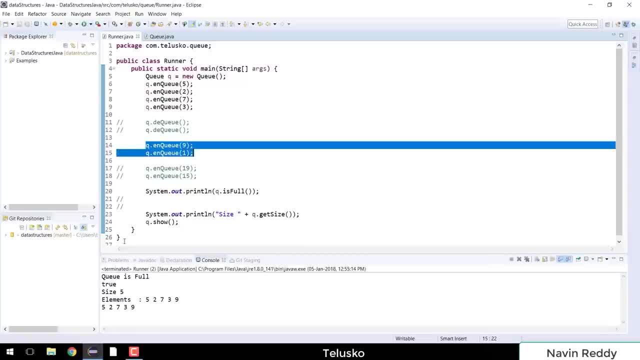 so you can see i'm adding six elements there and the moment i run this code you can see it will print: the q is full for this element here and the size is five and you got all these elements. so that means one is not getting added. now what if i delete the element, let's say, if i don't have? 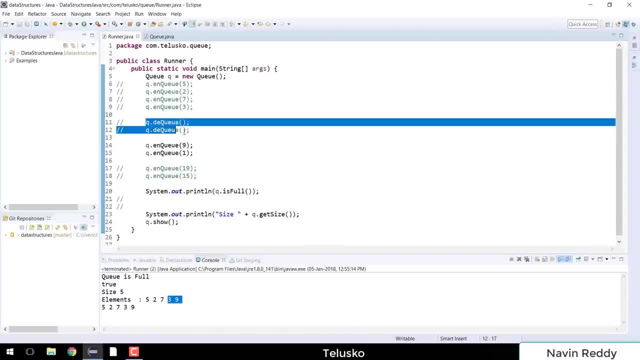 any element in the queue and i i'm trying to delete the element. so, of course, if the if you don't have any element, of course, how can you remove that? so if i run this code, you can see it prints q is empty. so in both scenarios q is empty. so yeah, that's how you, that's how you implement. 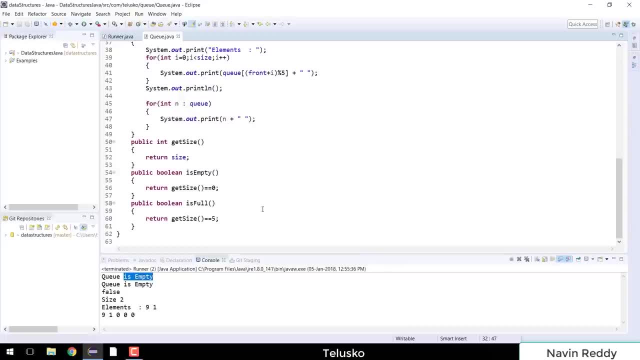 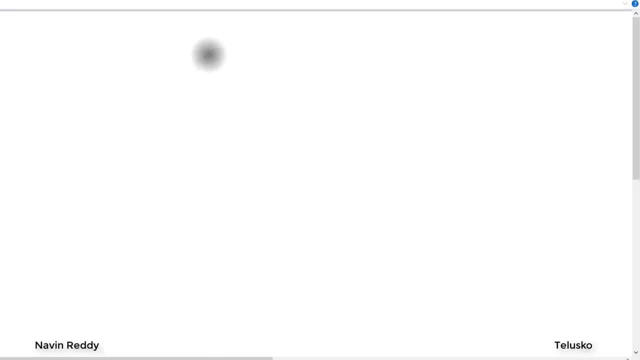 these methods. so let me recap: we have get size is empty and is full, and this will be used to check before adding the element and before removing the element, and in this video we'll talk about a tree data structure. now we have talked about linked list, stack and queue. 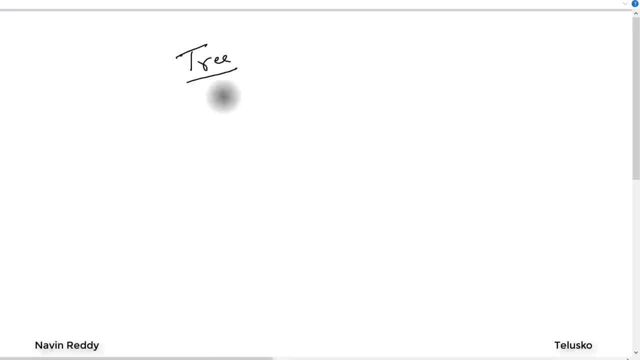 now, tree is another addt. now if we talk about tree, it is basically a structure where it's similar to linked list. you can say so in linked list. what we have is, let's say, if you have a node and you have b node, so what happens is a node will have a reference of b node, right, and then 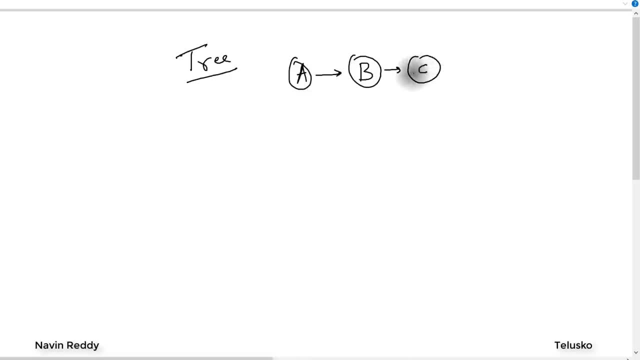 b node will have a reference of c node. so we have this in linear format. in tree what we have is we have the almost similar structure but then with a difference. in tree we normally create a structure like a tree, but you can imagine a middle image of a tree. 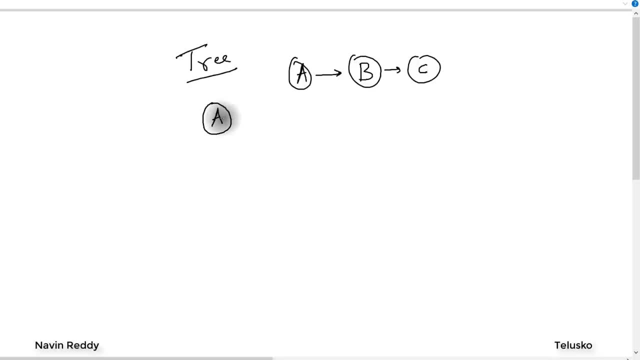 normally in tree, we have roots, we have branches, we have leaves. in the same way, if we talk about a tree here, imagine this is a root node, this is a root of the tree and this a, instead of having one reference, may have multiple reference. in this case, i'm getting three references. 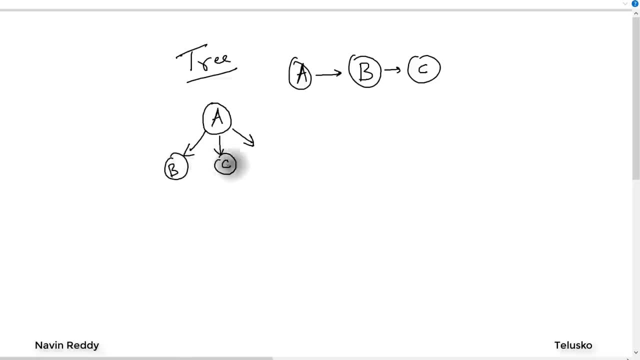 so a will be knowing about b. b will- i mean a will be knowing about c and then d. so after a we have these three nodes. maybe this c itself will have more, some other nodes, let's say we have x and here we have y, and maybe this d has one more. 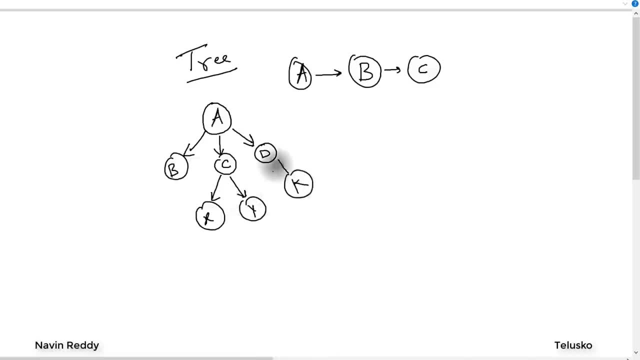 node here, which is maybe k, so k. so we have all this, all this nodes here. now this is the top most node, right? okay, everything, every box here is called as nodes, so these are nodes here and this are called as edge. so i would say this is edge, so we have this as node b, x, y, c, all our nodes, and 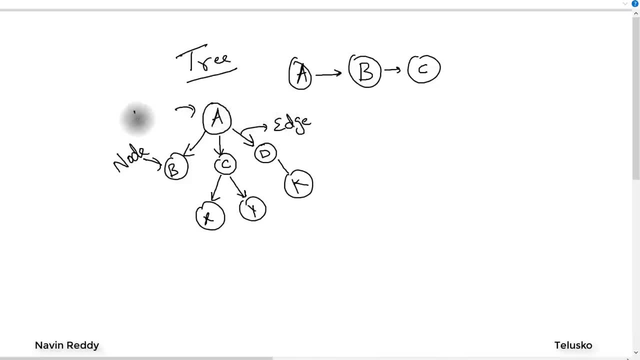 then this is edge, and the top most is called as a root node, because this is where your tree is getting started. this is your root node. now, if you talk about this a. so a has a node which is b, a has a node which is c and a has a node which is d. right, the same goes with c. c has x and y, but 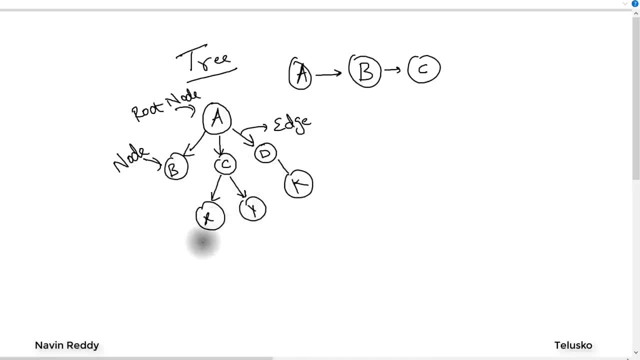 what about this k? what about this y and x? we don't have any other further nodes here and in fact b as well. we don't have other nodes. so this nodes are called as a leaf node because we don't have anything at the end of after that. so the top most is called a root node. this is where you will. 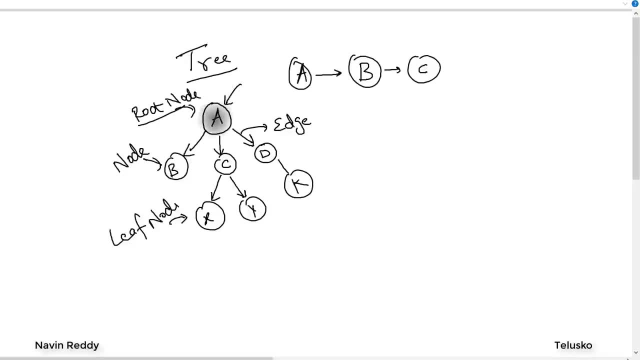 start your travel cell, if you want to store data as well, you will start from the root node and then you will go down, and down and down. so this is your node, and then the end nodes are called as leaf nodes. so these are normal nodes in between, but then a has a special name, which is root node now. 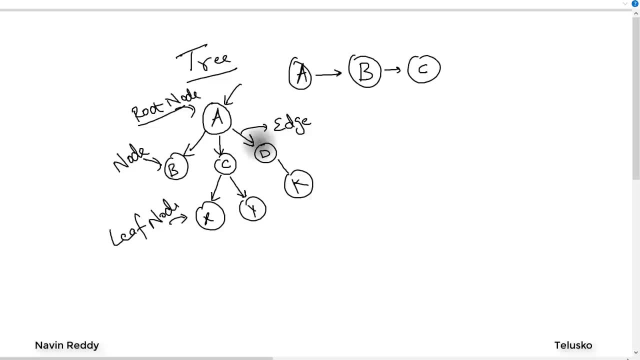 this is about tree. this is so you can represent this with different languages using java, c, c plus python. now, with this, we have a very special type of tree, which is called as a binary tree. now what this binary tree means? now, binary means two right, so if a node, so let's say, if you have a node which is 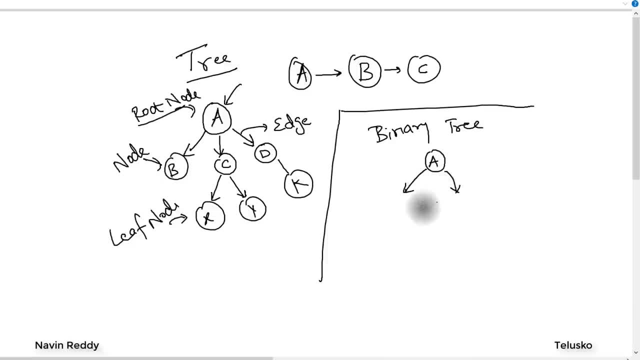 a and if this node has two more nodes like c or d, so maximum if you have two nodes, this is called as a binary nodes. so we have two nodes, so binary nodes, and that's why the tree is called as binary tree, where every node will have max2max two nodes. so either we can have a 0 node or we can have one. 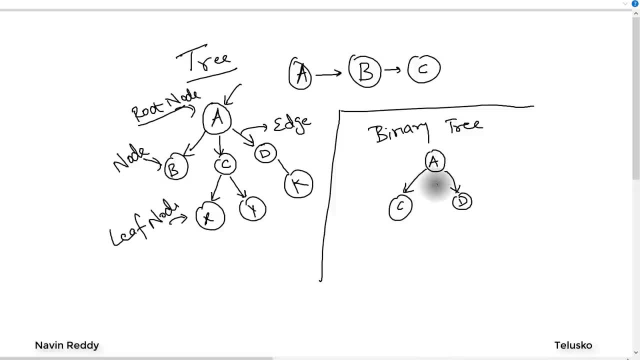 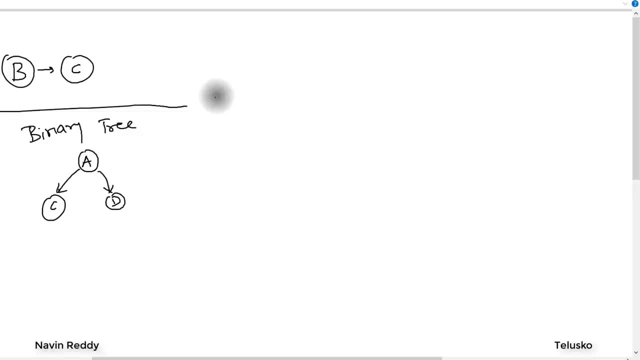 two nodes, not more than that. so this is how you represent your binary tree. now, in fact, in binary tree as well, we have certain, certain types. let me just write it here. so we have certain types in binary tree. so first one is strict binary tree. so we have the first one, which is strict binary. 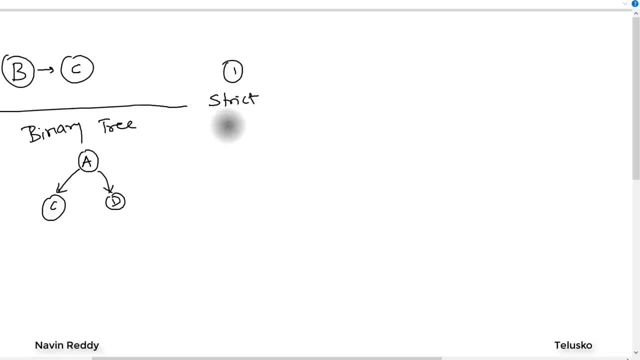 tree. now, what is strict binary tree means a tree where an every node will have two sub nodes or no children. so- and again we have one more term here, so the c and d are called as children's. so if i have a here and if a has two, which is c and d, then this is called as a strict binary tree in. 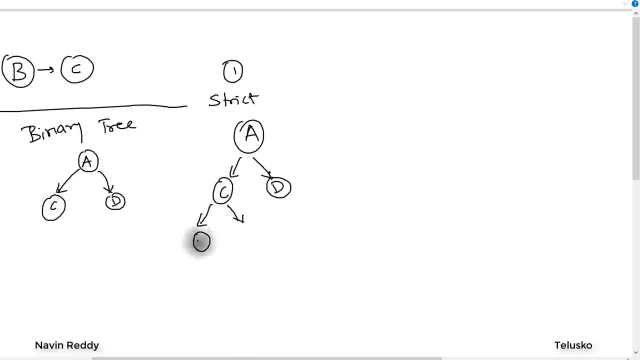 fact you can also have inside c, we can have two more nodes. let's say we have x and we have y. this is also a strict binary tree. now you might be thinking about d. so yes, so when it, when you say strict, it means either two or no children. so here you can see, we don't have any children to d. 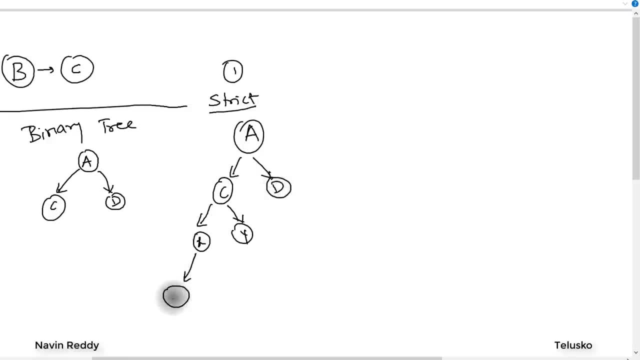 now, how about if i say we have, uh, let's say x has one more child. let's say k, now and that's another. this is not a strict binary tree, because we have only one element or one children node for x. so this is not a strict. so let me just remove that. so this is the first type. the second type we have is: 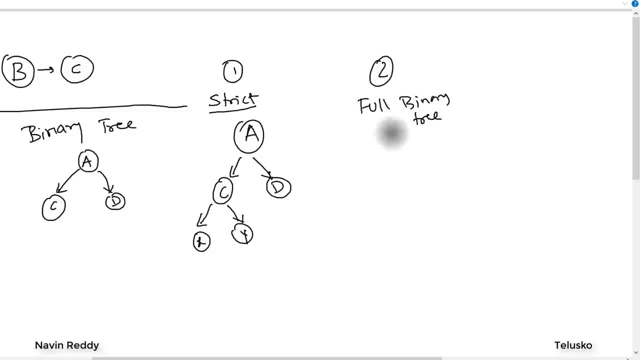 full binary tree. now, what is full binary tree means where you have a, you have a tree where every node either either has two. i mean they will be having two sub nodes. example: we have c and d again and d has two, let's say. let's say we have x and y and d should also have two more nodes. so 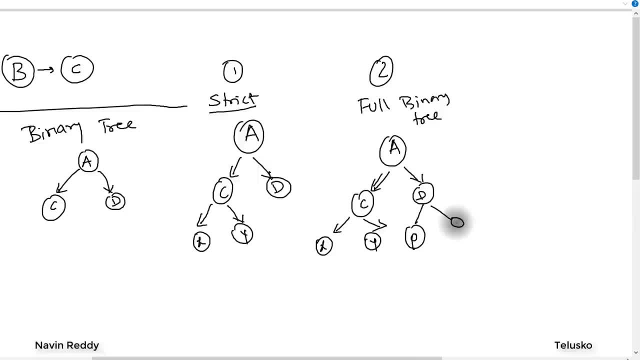 so that they will come on the same. so let's say we have p and q here, right? so we have d. also has two more nodes, which is p and q, so a has c and d and c has x and y and d has p and q. so all the. 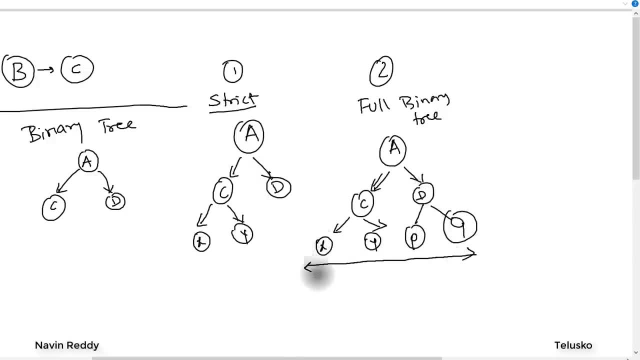 leaf nodes should be on the same level so you can see they are on the same level. so this is what you call as a full binary tree, where all the children are on the same level. so this is a full binary tree. the third one is called as a complete binary tree. when do you say a binary tree is complete? 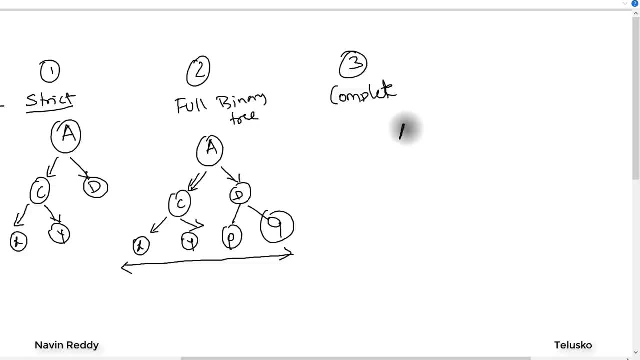 it's very simple: where you have a tree where all the nodes are on a level. so let's say, if i, if i define that c and d again, and here if i say x and y, and then we, so this is also called as complete binary tree because you have all the all the leaf nodes on the level. so let's say this level is, let's. 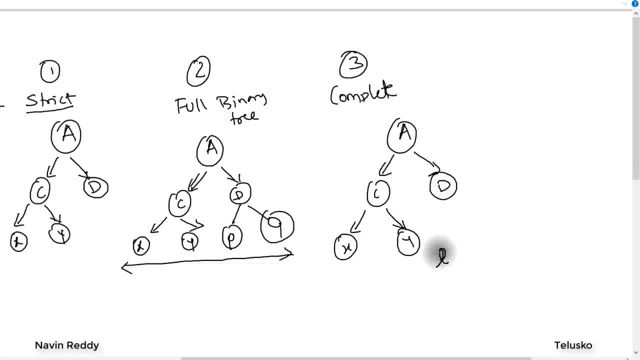 say i will, i will call this level as l, so either it should be on l level or l minus one. now, which means if you have one more here or two more here, let's say we have k and we have c now. this is not a complete binary tree, because the leaf node are on the are not on on l and l minus one, because if 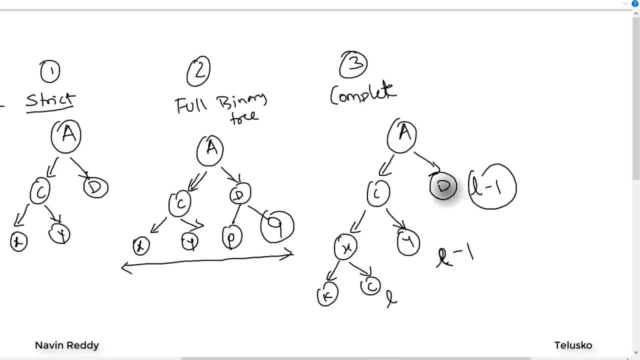 i say this is l, then this is l minus one, but this is this will not work, so there should be two more nodes here. then it will be called as complete binary tree, right? so this is not a complete binary tree. so if i undo so, this is a complete. 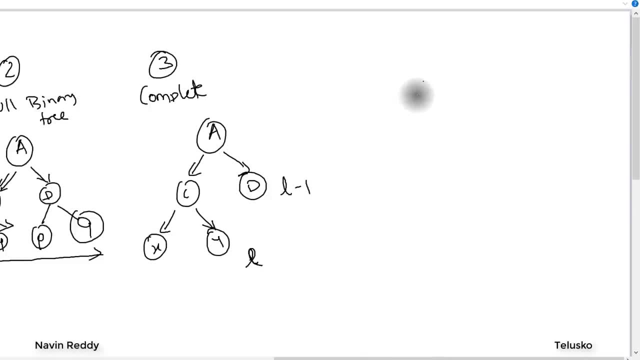 binary tree. so if i undo, so this is a complete binary tree. so if i undo, so this is a complete binary tree. so let me draw a simple, simple tree here. so if i say we have a and then we have b, we have c, and then we have: inside b we have d, we have e and inside e we have f and we have g, and then i 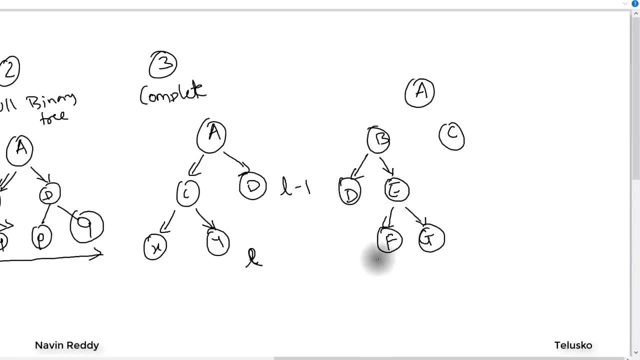 will draw a line here. so these are all my nodes, and inside this f also, we have two more nodes here. let me just draw it. let's say this is x and this is y. so now, looking at this tree, we have certain terms here. so again, this is a root node, right? so this is your root node, and this c, g, y, x. i mean x and y and d, those. 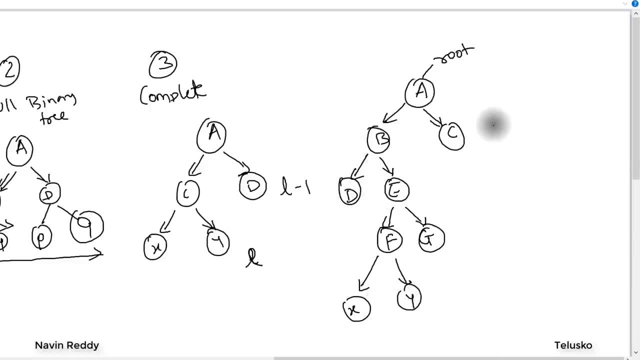 are your leaf nodes. now we have to remember two more terms, which is height and depth, now what it means. so depth means, let's say, if you talk about this e, so what is the depth of e? it is a, b and e, so that's a depth of this e. and what about the height of e? so height would be, it's the, the. 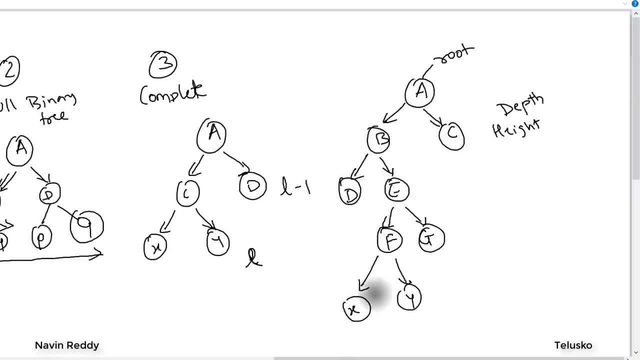 children's of e, so we have f and e. and then we have the children's of e, so we have f and e and we have x. right, maybe this x has two more, uh, two more, two more subparts here. let's say we have k and. 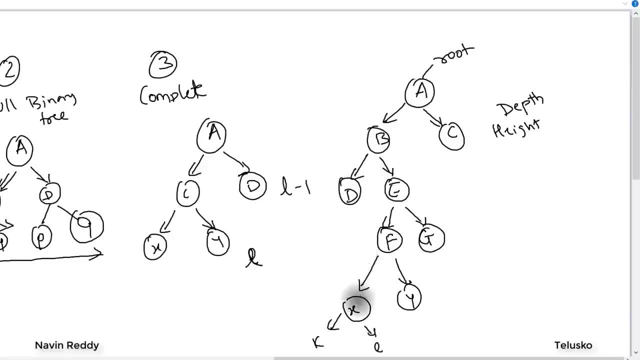 we have l. so now for for e, it would be f, x and k. so this is the height of e. so when i say the depth of e would be 2, so we have. so we have 2 because it is a and b, right. so a and b, those are the two. 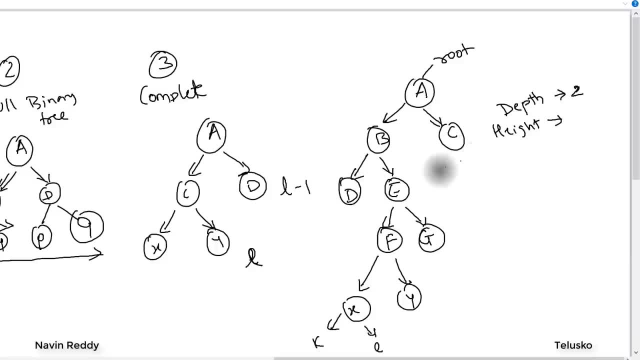 two, two nodes we have. what about the height of e? it would be f, x and k, so it will be 3, so it's three. now what about the depth of a root node? it's always zero, right? because this is the first element. so we don't have any depth. what about the height of a root node? is it? again, you have to say. 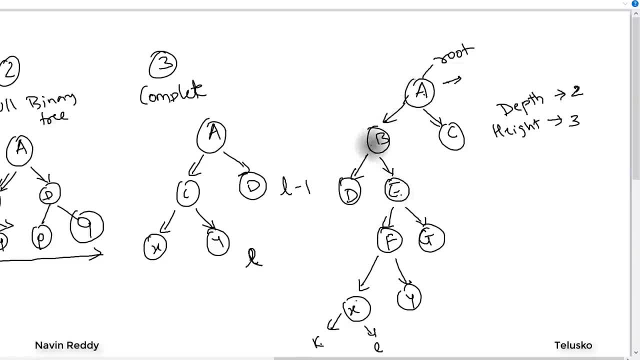 a, b, e. so we have to go for the longest one. so it is a, b, e, f, x and k. so it's one, two, three, four, five. so height of this tree is five. oh, that's a new term now, so we we know the height of the root. 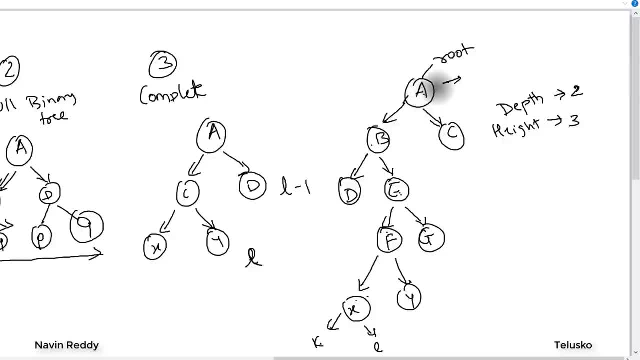 node right. so height of the root node is same as height of the tree. or you can say: height of the tree is same as height of the tree. so height of the root node is same as height of the tree root node. so that's how you. so we have this two. these two terms are important when you go for the. 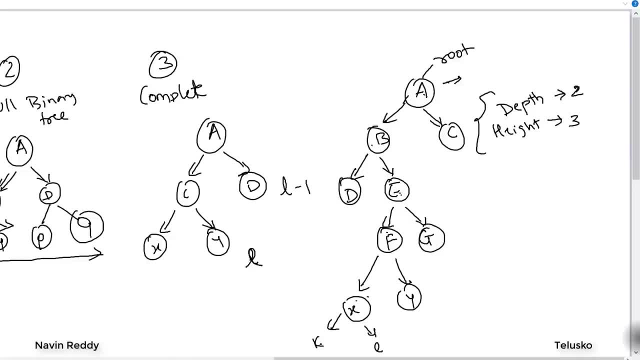 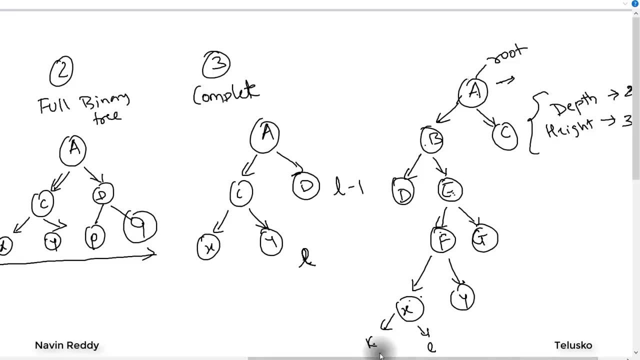 coding part. so, yeah, that's it. that's what your tree function thing is. so we have talked about what is tree. we have talked about binary tree. now we'll be doing the implementation of this using different languages. so i hope you enjoyed this video. let me know in the comment section in the 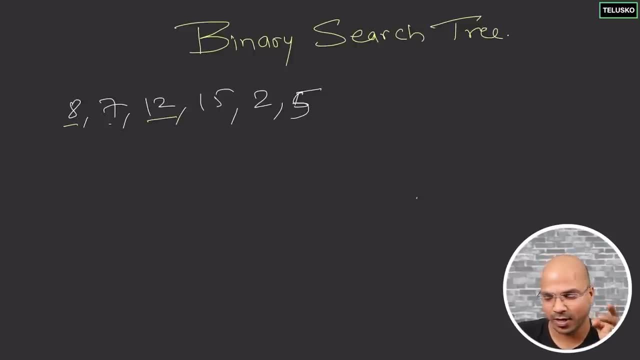 theory video of tree. we have talked about different types of tree and we, when you implement this, we are going to implement that with the help of binary search tree. now, what's the difference between binary tree and the binary search tree? binary search tree is a binary tree. the difference is the way you add values now in binary search. 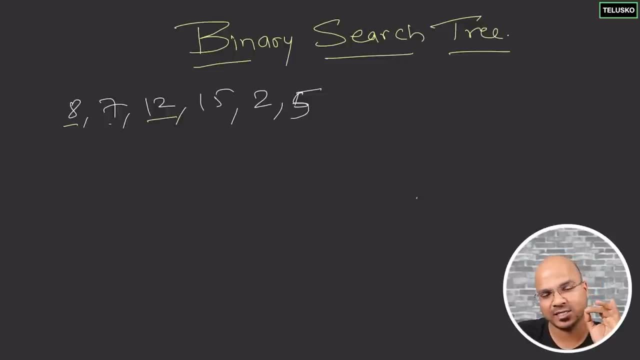 tree. what you do is you always make sure that the smaller element is on the left hand side and the bigger elements are on the right hand side. that means, if we talk about a root node, the elements on the left hand side of a root node will be smaller than the root node and the elements 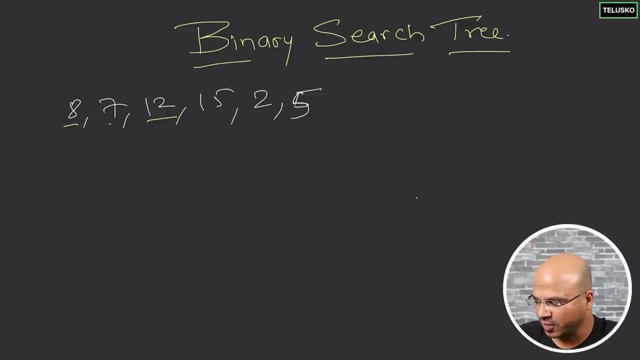 on the right hand side of the root node will be bigger than the root node. it's that simple. that means, when you try to create this tree, how will you do it? so let's say we have these values here. now, when you work with eight, eight becomes your root node. 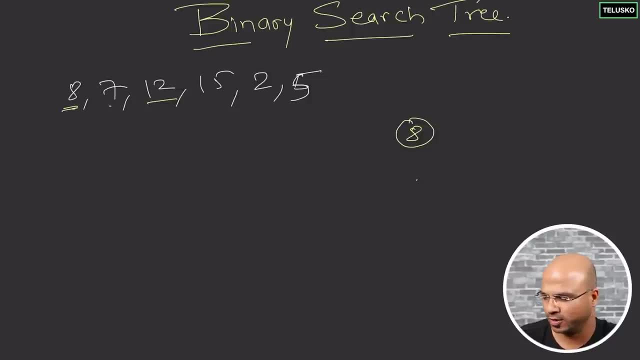 okay, that's so simple. you always get your first element. make it a root node. next you have 7. now 7 is less than 8, so it will go on the left-hand side. so that is a 7 here. then you got 12. now 12 is bigger than 8, so it will goes on the. 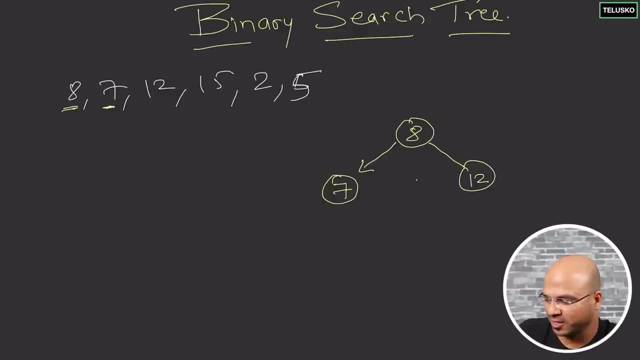 right-hand side. now, of course, for the root node. both the nodes have been covered. what about the next element, 15? where 15 will go? of course you cannot create a one more node here. that's not possible for the binary tree. so what you do is you travel now. way to travel left or right. now, 15 is bigger than 8, so 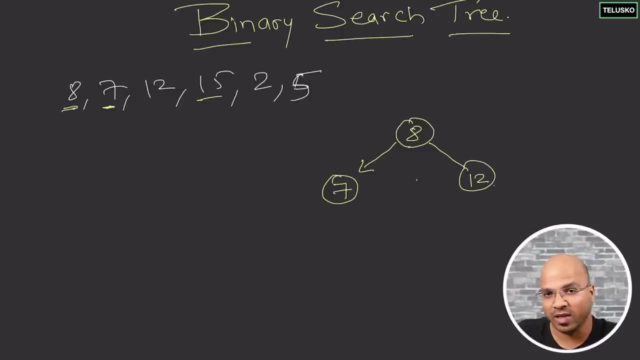 it will go on the right-hand side, but we already have 12 there. now 12 have an option of putting 15 left or right now. since 15 is bigger than 12, it will go on the right-hand side, so 15 goes here. next element is 2. now, 2 is smaller than 8. 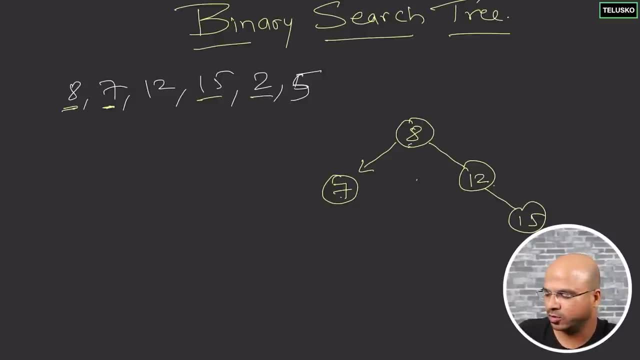 again, we starting from root node, so starting from 8, it is smaller. then it goes to 7. it is smaller. it goes on the left-hand side of 7, which is 2 here, because it is less than 7. next we have is 5. so we go on, we go to 8. it is smaller than 8. we go to 7. it is. 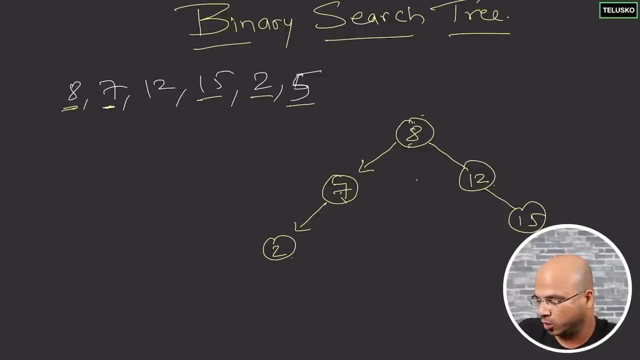 more than 7, we go to 2. it is greater than 2, so it goes on the right-hand side of 2, so 5 goes here. so this is how the binary search tree works. now, once you got the basic understanding, let's start the implementation. if I want to code, 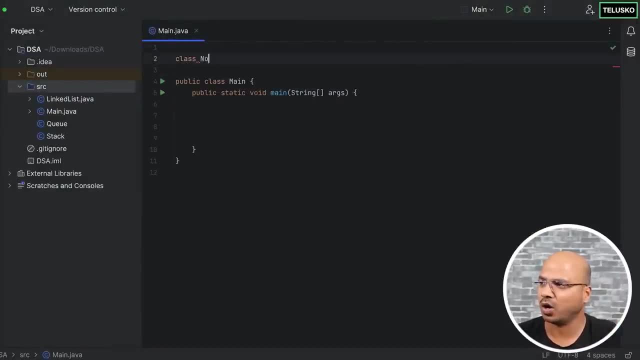 that first of all, we need, for sure we need- a class called node, right? in fact, I will not writing this here, let me just remove it. what I want is I want from my main method. basically, I want to create a binary tree. there are some inbuilt classes, but we're not going to use it. so let's say: 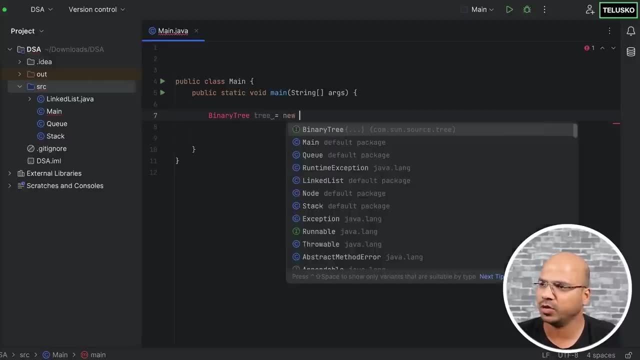 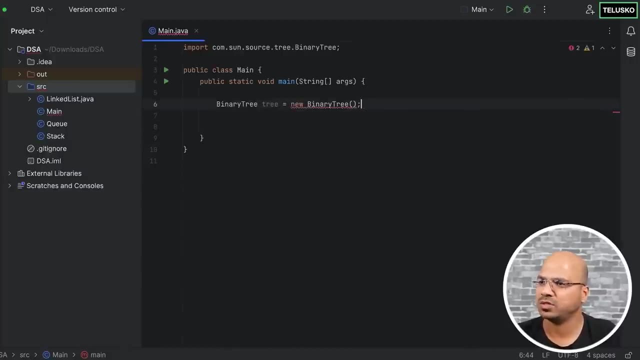 binary tree, and we'll call this as a tree equal to new binary tree. so we want to build a binary tree. okay, you can see we have some inbuilt methods. we don't want to use them, so let's use a binary tree. we don't have this class yet, so 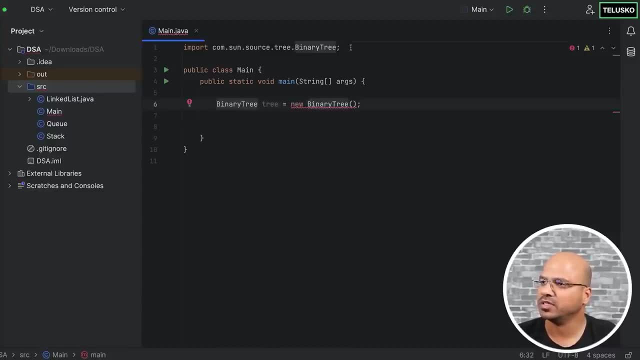 what I will do is I will just go back here and you can see it is importing this package. we don't want any inbuilt things. so if I go back here and if I say, hey, I give me solutions, more actions. I want to create this class binary tree in the 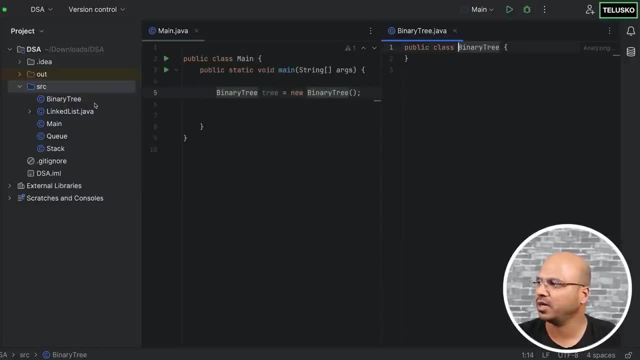 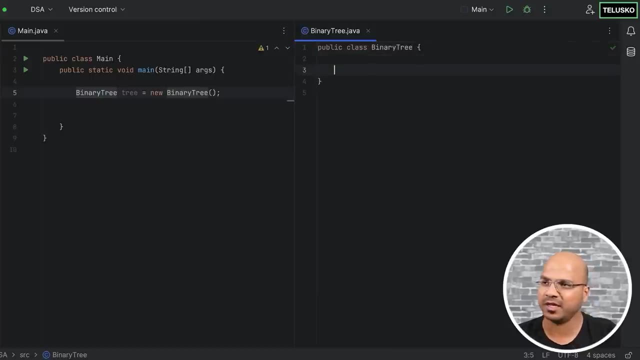 package and you can see we got it. I will just move this on this side. I don't want to see the project structure. so you can see, on the left-hand side we have a main. on right-hand side we have a binary tree. so basically in this binary tree I 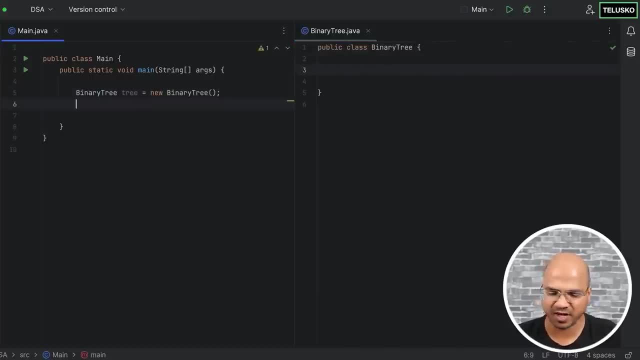 want to do all those stuff. now let's say I want to do stuff. basically we have to say tree dot. I want to insert value in this tree so I can say insert and I can pass a value, let's say 10. I don't know what values I'm passing here, or maybe I. 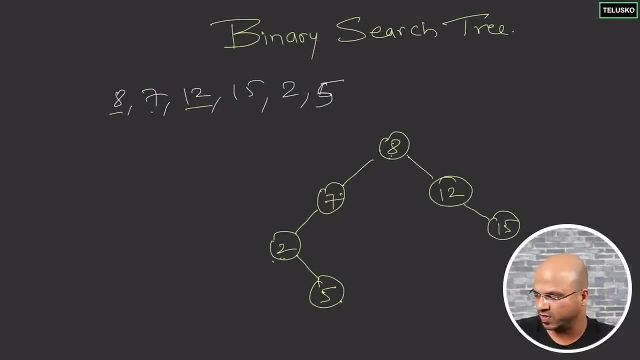 can? I can for the same value which we have in our node. so we have 8, 7, 12, 15, 2 and 5. let's add that, okay, but then until, fortunately, we don't have this insert, okay. so what we need to do is we need to. 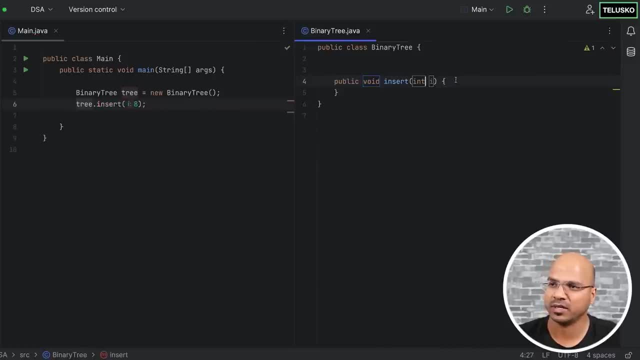 create this method called insert inside this binary tree and you can see we got insert method. okay. but when you say insert, that means we have to make sure that you're inserting a node. of course you are passing data here, but it should be added to a node, right, and we don't have a node implementation yet, so I can. 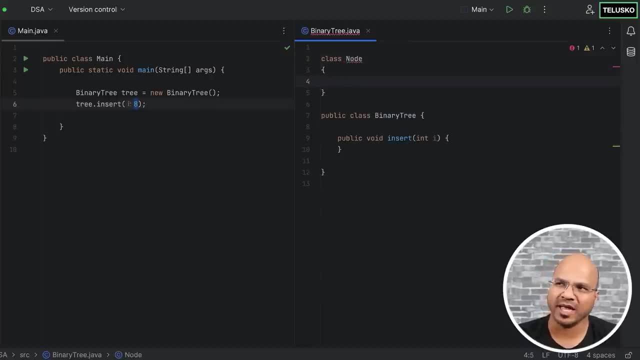 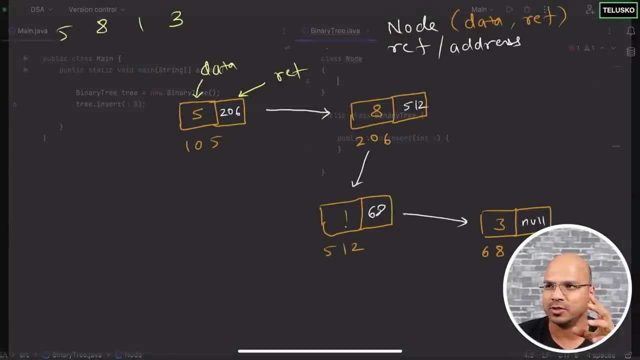 create a node implementation by saying class node. now what every node will have. now, if you go back to linked list, a node will have two things: the data and the next value. now, in terms of this node here, which is a tree node, it will have three things: data- the left node and the. 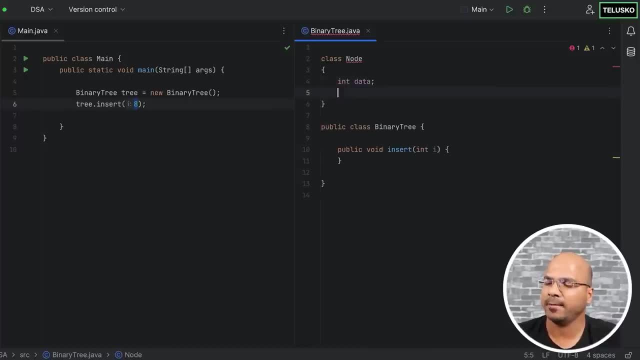 right node so I can say int data, then we have to say a node, because when you say right node, left node, they are itself nodes. right, let's first write left and then right. so yeah, so we got data, we got left node and we can, we got right node I. 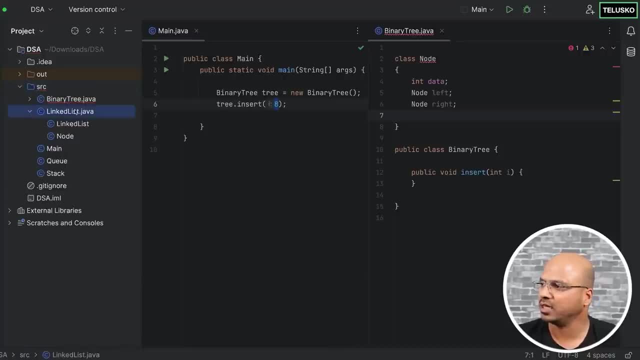 think the only problem is in some of the class. I think in linked list. we already have a node here. that's the problem. so what I will do is let me just move binary tree and this main to some other package. I will just move binary to the. 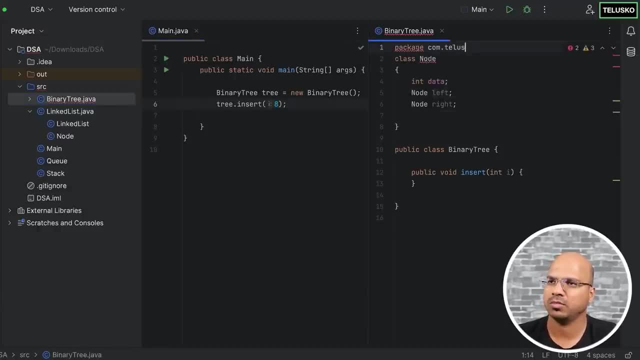 other package. it's a package comtelescopetree, so sometime you have to solve the problems in a go. you need to import the package from here now importing done. ok, so problem resolved. the problem was I was having two classes with the same name in the same package. I just moved it to. 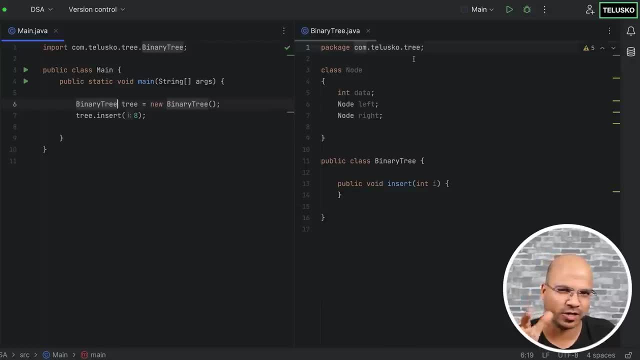 different package. ok, so now you don't have to do that. if you're just writing the binary code, you can just skip this line anyway. so we got a node and then we are referring to left node and right node. so that's node done. but also, what I'll do is maybe when I create a node I will. I want to have a constructor. 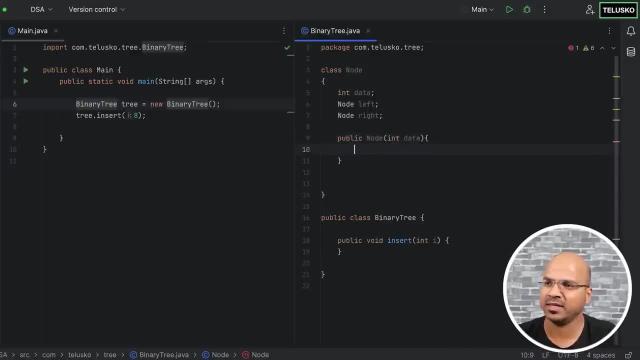 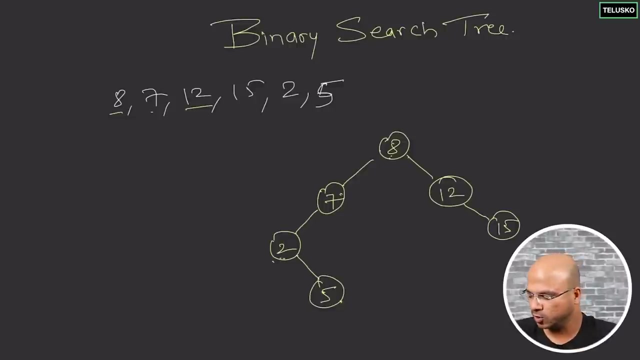 here which will take the data for me and I will assign that data. so I can say this: dot data to data and that's it. so we are basically done with the node concept. but how will you implement this tree? so, every time you want to insert the data in a tree, how will you do it? so if you say this: 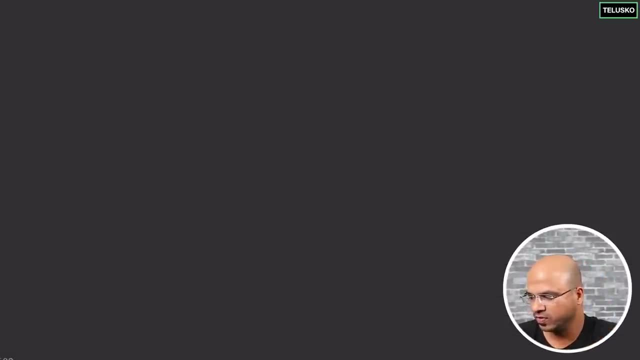 is a tree, of course we don't. let's say we don't have a tree here and let's go with the same value. I don't know what values we have, I can just use this copy: okay, so we got this value. so if I want to draw a tree, so let's say someone is giving you the value eight initially, so what you do is you. 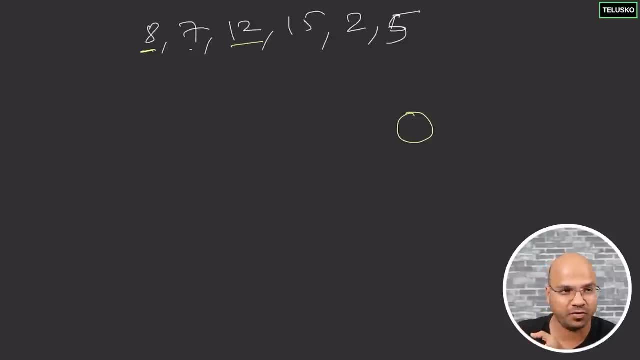 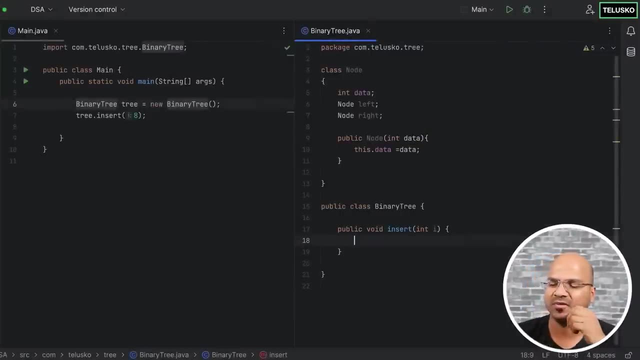 create a root node. now we know that we don't have a node in the tree, so basically the tree is empty. in that case, you will make this as a root node. okay, so how do we do that? so when you say insert, basically we have to create a root node- that means every tree need to know about only one thing, which. 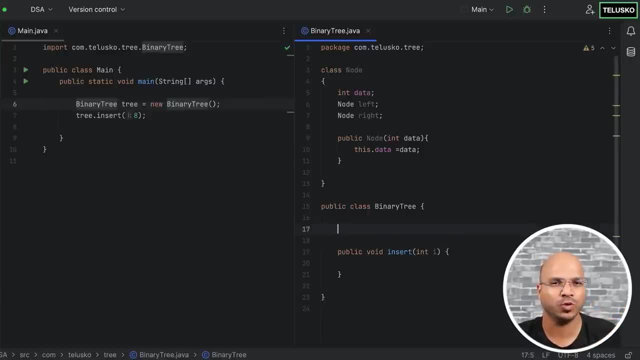 is a root node right. as I mentioned before, for a tree the most important thing is to know that the tree is a root node right. so when you say insert, basically we have to create a root node and then tree don't have to worry about other nodes. the root node will take care of the next. 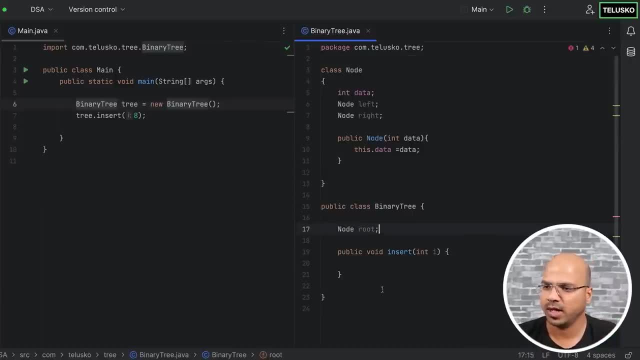 two nodes. so what I can do is I can say node root and then every time I create insert and then imagine that this is the first time. so what you will do is you will create your root node here, so you can simply say: root is equal to new node. that's how you create a node: just create the. 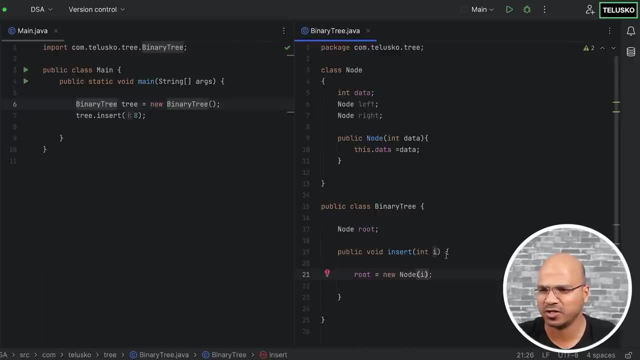 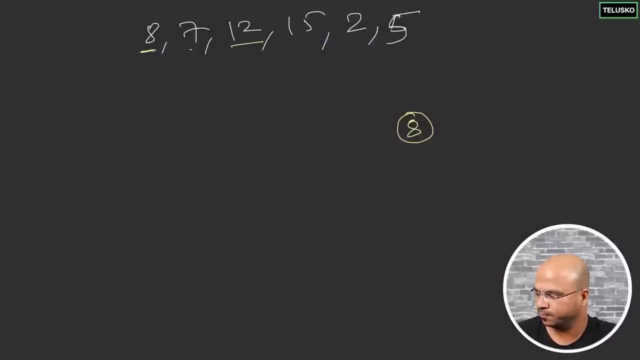 object and pass the data, and that's it. you got your root node. in fact, you know, instead of using this variable, as i, it should be data. it will make much more sense. so now, if you can see our code, this is the thing we have done. so we are going to create a new node and we are going to create 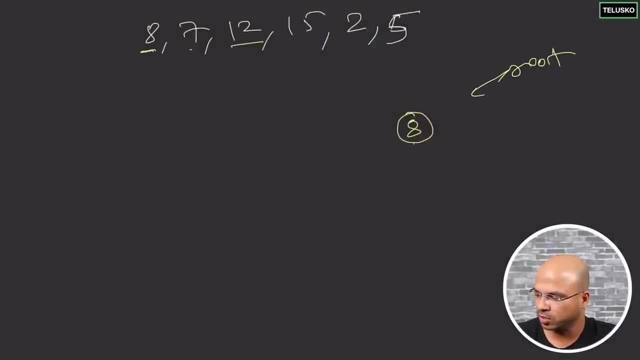 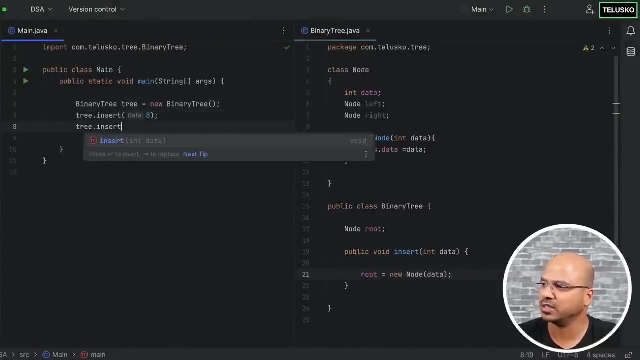 a new node. we created a root node called 8 and that's your root node, which looks good. but then what about if I insert one more data here? so if I say tree insert, I want to insert the next record. what's the next record? it is 7. so when I insert 7, where the 7 should go now? don't you think the 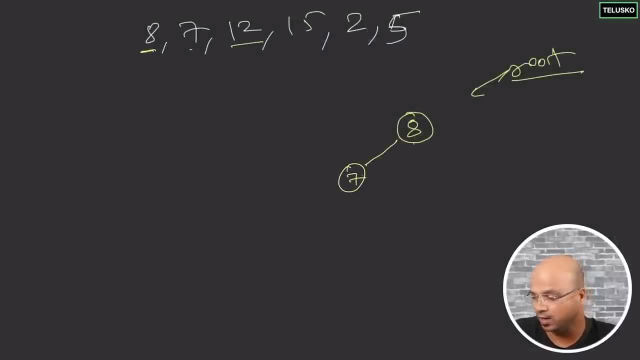 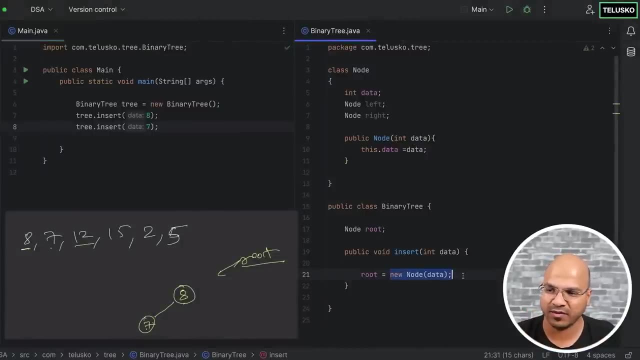 7 should go on this side is because we are implementing binary search tree. 7 is less than 8, so it should be on the left hand side. so when I say 7, it should create a new node. and we are creating a new node, but don't you think this time it's not a root node, it's a left node of the root. 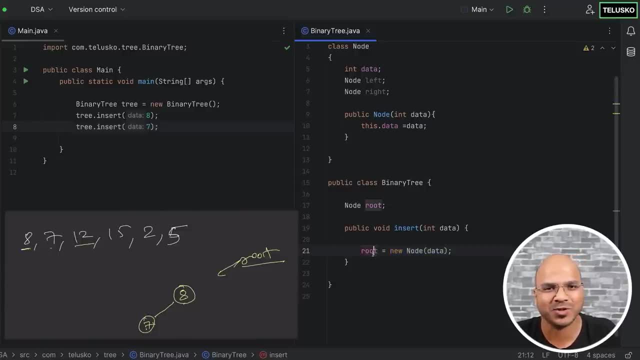 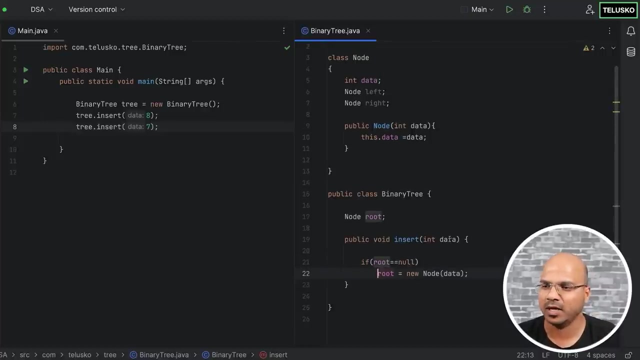 node. how will you do that, and how do we even know that this is not a root node? so in that case we need to do is we need to check: if the root is null, then you create a new node. I mean, then you create a root node. otherwise, you don't create root node every time, so root node will be created only once. 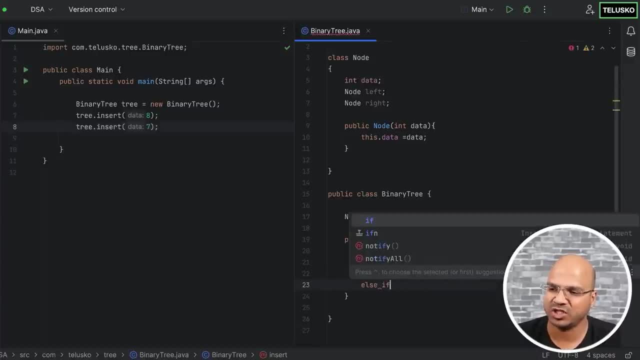 if the root is null, what else? if it is not null, then we can check for something else. now see if, yes, this satisfies, is because root is null till this point. when you before executing 8, but when you insert 7, we already have a root node, right, then we have to go for, if else. now the question: 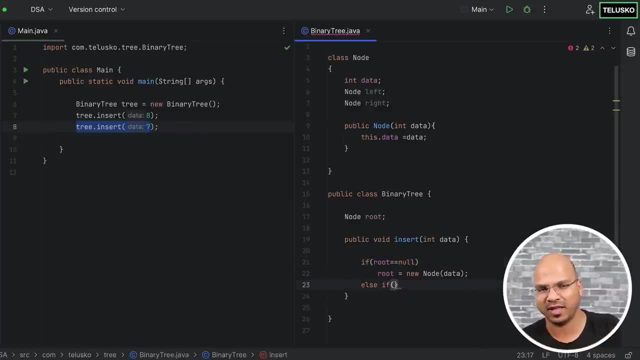 is now. we know that this is not a root node. we have to either go for left or right. so what you do is you basically check for data. if the data is less than root dot data, then you go on the left hand side. so when you say you go for left hand side, what you simply do is you say root dot left. 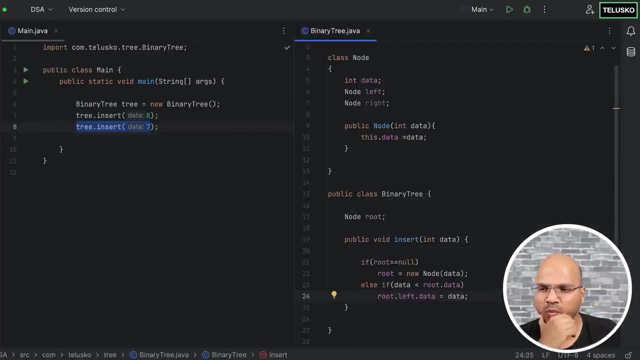 dot. data is equal to data. that's what you do. but then we have one little problem here, because this will work for this data, okay, so we will get new, new thing, but we are not even creating a new node, okay. so that problem is: we need to modify this to. 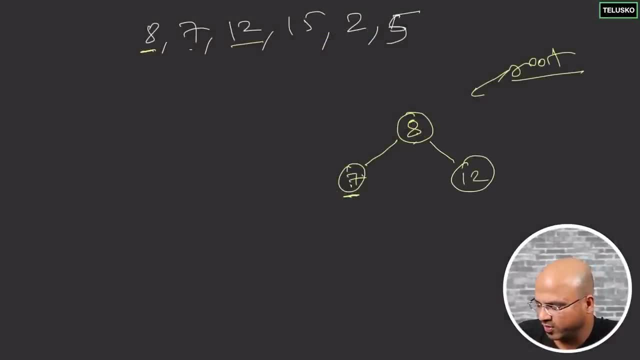 something else. why something else? let's say we have adding one more, which is 12, goes here, and then you add 15. now, by our logic, if the value is greater than root node, just add it to the right hand side. but 12 is already there, right? then we have to move to 12 and it becomes a right hand. 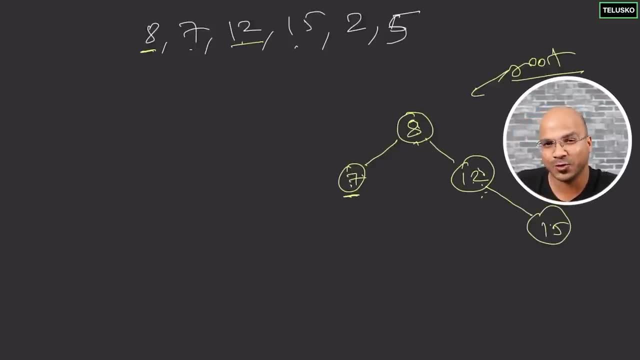 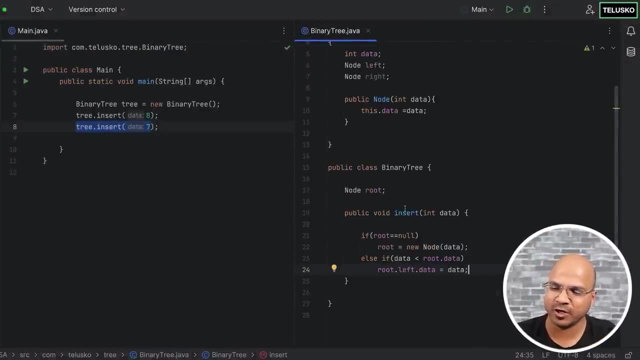 side. so we have to add a recursion here, and then we have to add a recursion here, and then we have to add a recursion here. so that's one thing. second problem is: every time you insert data we need to get a hold on root. you know, writing the logic here is not efficient way. what we should be doing is: 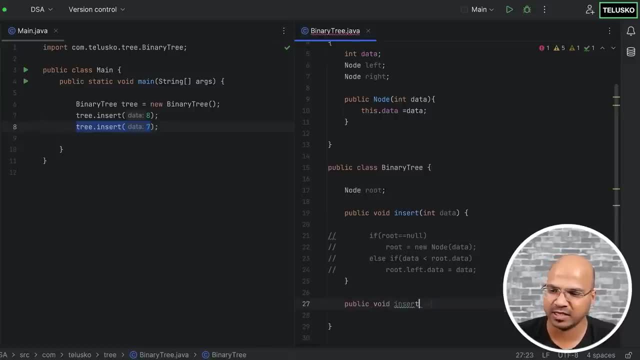 create another method which is called, let's say, insert, rec, and we'll say: this will take two things. because when you want to do recursion we have to get a hold on root element or root node. so that means we cannot do that in this insert, because the moment you use a recursion, every time you call the method. 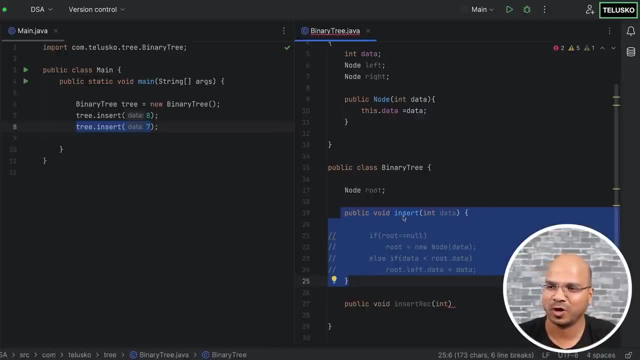 we need to get the hold on the node where you're calling this. so this will not work. but that doesn't mean we have to remove this. i will tell you in some time why. so basically, we have to say node root, comma data and here, okay, this should return a node because we are going for recursion, so it. 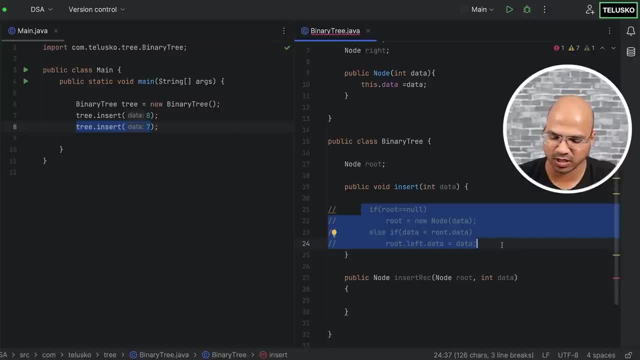 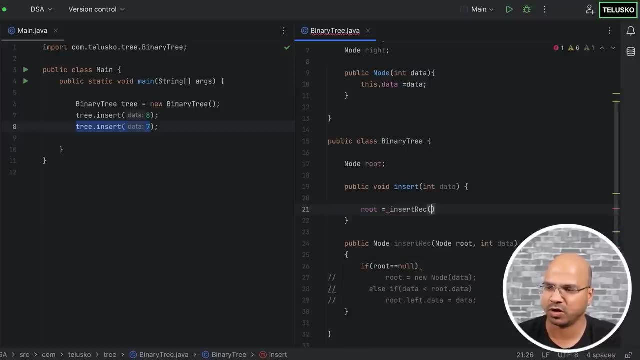 should return something. and now here, instead of doing all this logic, this logic should be a part of this, not this. so here we can simply say: root is equal to insert record, so every time you call insert, it will call insert rec in which you are passing the. 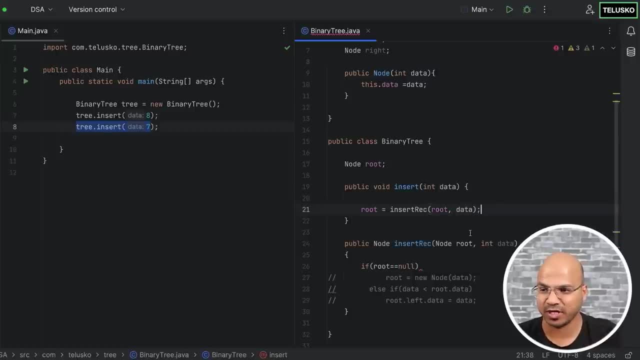 root node and the data. so when you say recursion, it will go into recursion. we will be using recursion on insert rec not on insert. so we have to change some logic here. so this is correct. when you say root, i'm only concerned about this part. so how do we implement this one? so when i say i want to, 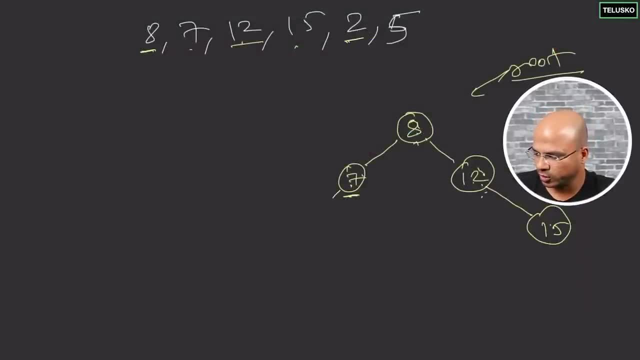 add element on the left hand side. so if you have, let's say, 2 now, we know that 2 should go here. but then we have to jump from 8 to 7,, 7 to 8 and we have to add a part in front to the right side. so 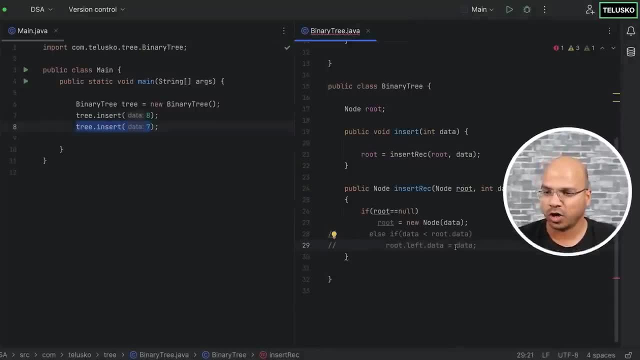 so now that we have set 2- so about that, all of this is done here. we will see very soon the value. that we'll see. here are the tokens that这就是用于我们想要新啥agem- 8 to 7,, 7 to 2.. That's a recursive process, right? So what you will do is let me uncomment this now. 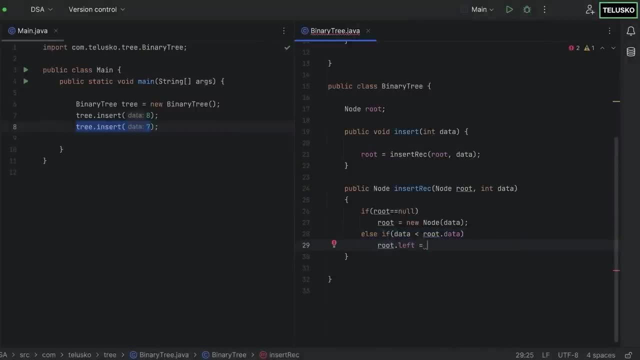 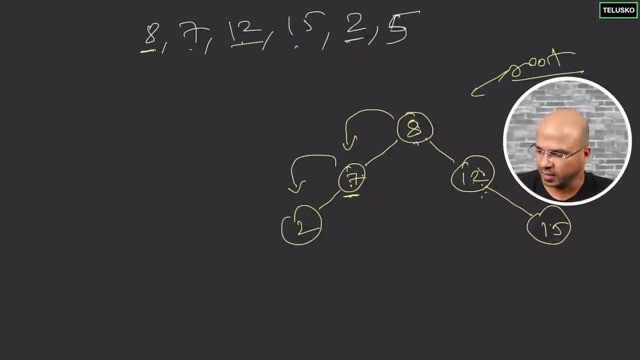 This is not how you do it. So basically, you say rootleft and then you call the function once again by passing the rootleft, because now we need to follow the tree right, As I mentioned before, when you talk about the subtrees. if it is not 8 left, then we have to consider this. 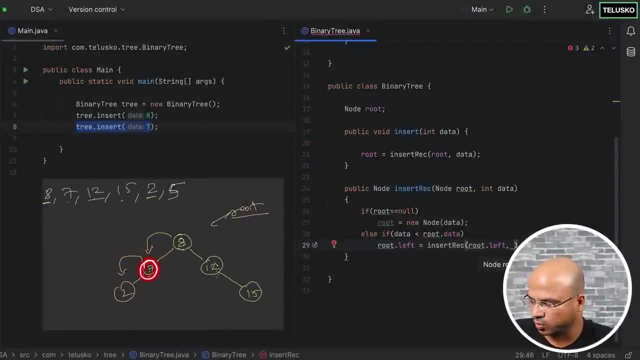 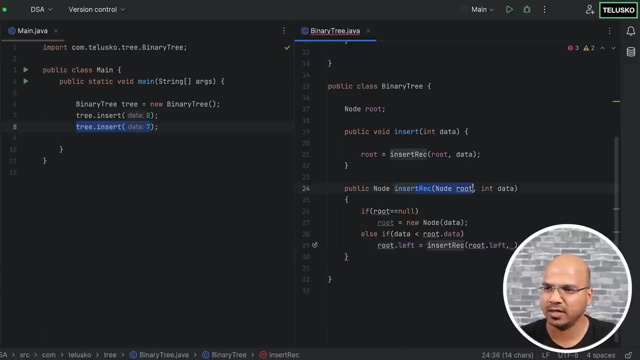 subtree. Now this 7 becomes your root. So how will you send this as a root? So you have to say rootleft. Now this becomes a new root. So when you call this function, which is insert rec here, this becomes your new root. And then you have to pass data as well, So you're passing data. 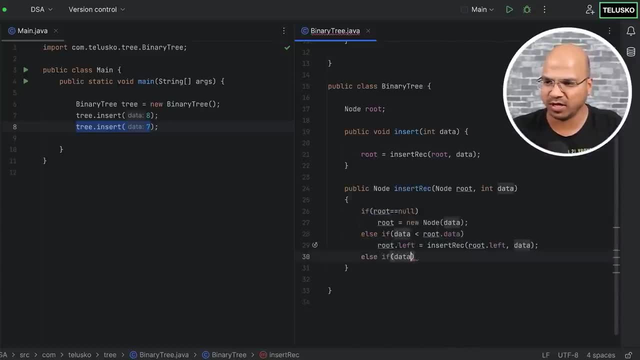 But what if this is not smaller? Then you have to go on the right-hand side. So I have to say rootdata. If data is greater than rootdata, then you do the same thing, but for the right-hand side. So I will say: paste here. So this should be right, and this should be right. And then at the 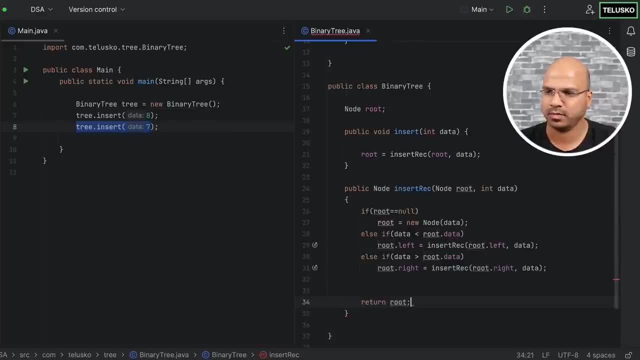 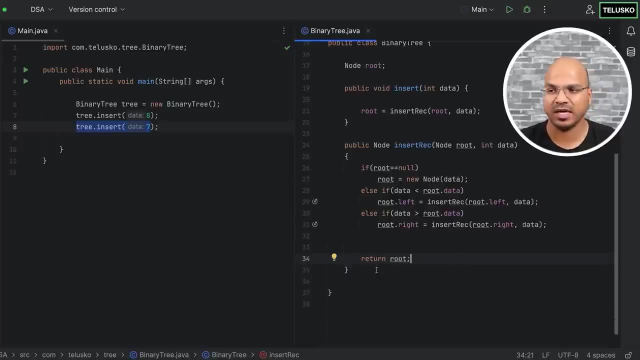 end. you know your root node, So just write it: return root. That's it. So this is the recursion call which we are getting here. So that's how, basically, you create a tree. Now this tree is created, But how will we know that this tree? 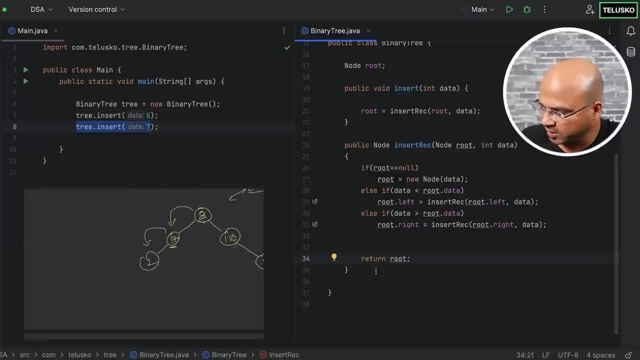 is created. We want to print also, right, And the way you can print it is like this: So if you want to print this tree, so let's say we have this tree here And this tree is created by the way we have. 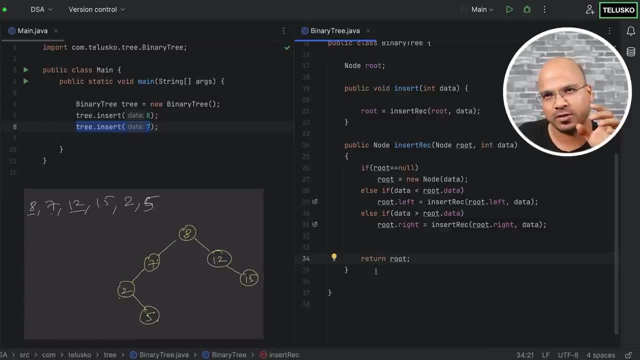 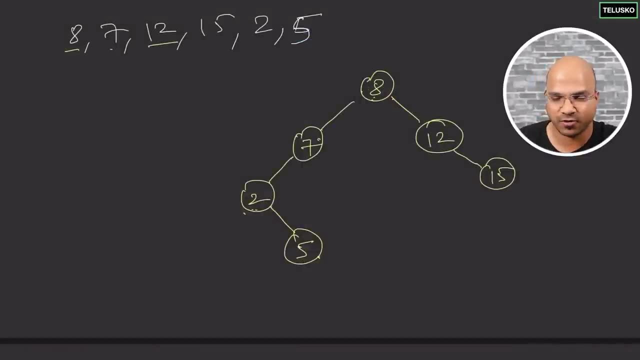 defined this example here. How will you print this Now? to print, we basically have to traverse or we have to travel to different elements here. The way you do this, you have to go to the tree. So what we do is we have different travel cell for tree. So when you talk about tree travel, 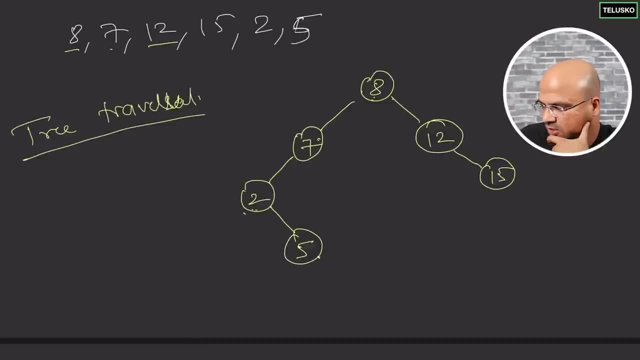 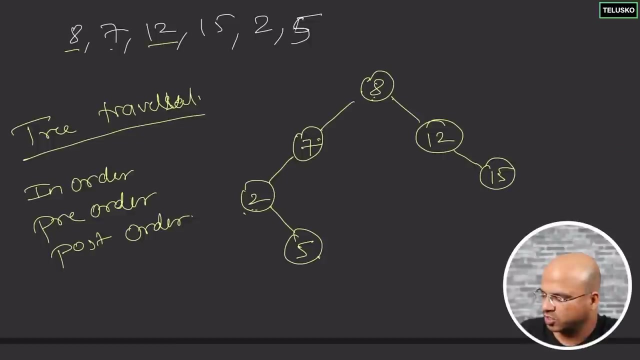 cell. we have to follow certain things. First, there are three options here. We have in-order traversal, We have pre-order traversal And we have post-order. The difference between these three is the way you print your root node. Okay, so when you talk about in-order, basically what? 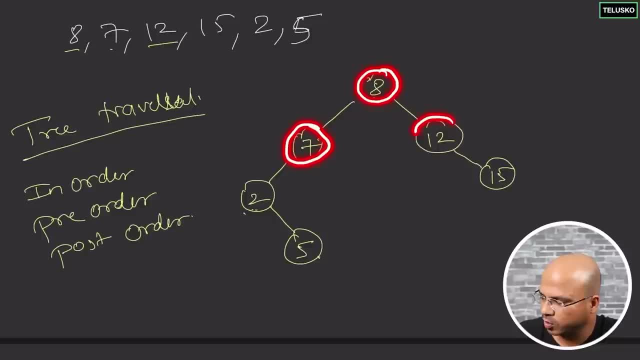 you do is you first go to the left, then you go to the root, then you go to the right. So which is pre-order? When you talk about pre-order here, you first go to root, which is 8.. So it will print. 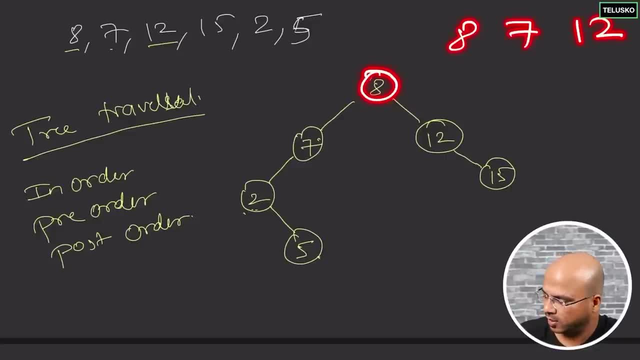 8,, then 7,, which is left, and then 12,, which is right. When you talk about post, it means first it will go for left, then right, then root, which is 7,, 12, and 8.. Okay, that's your post-order. 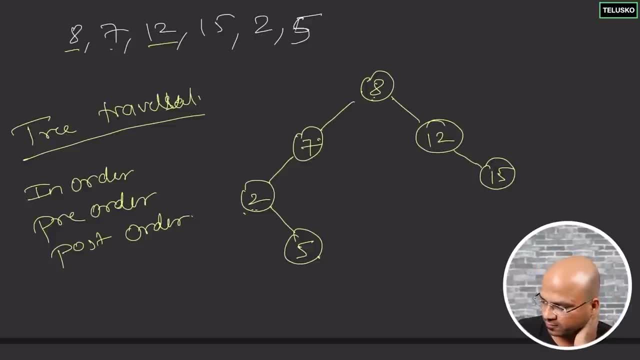 traversal. Here we are going to go for in-order. So in-order simply means: first you print the left one, then you print the- not exactly printing, but you go to the left one, then you go to the right one. So if that's your in-order, Now the way you can do that. of course this is also 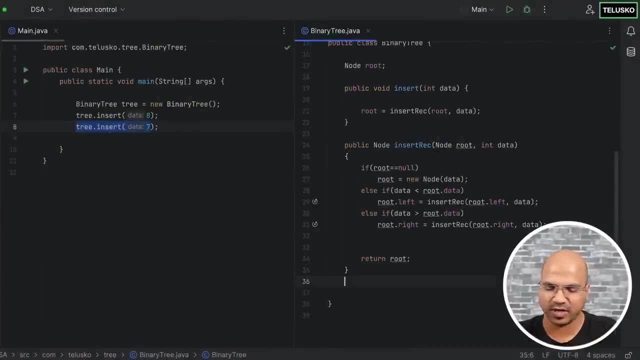 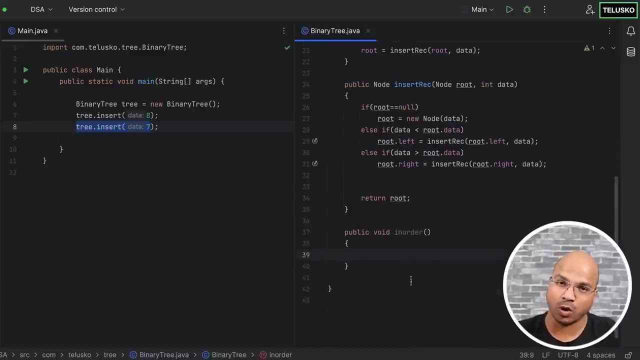 recursive right. So in order to do that, what I will do is I will create a function called public void in-order. Then you can work here. But then, since we know that in-order is actually, or traversal is basically a recursive operation, where you go to each subtree and print it or do some. 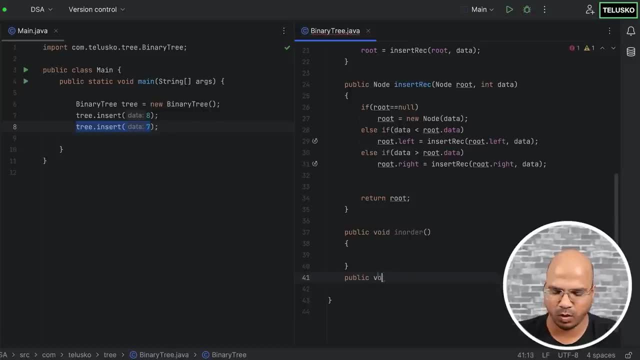 operations. For the recursion, I will create another method which is public. void is because I don't want to return anything, So I will say in-order rec. So we just want to print it. Now, when you say print it, how exactly we are going to print? 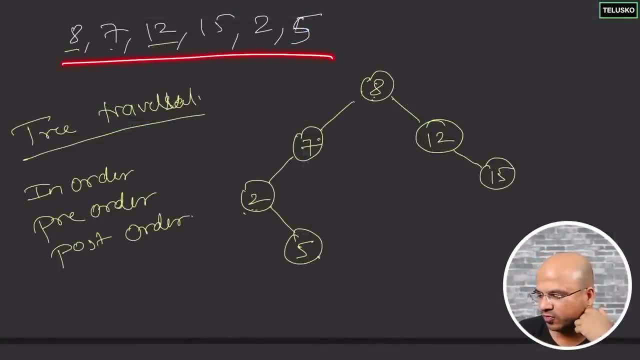 how we are going to travel this. Of course, the output will not be similar to the value we have inserted. It will have a different order. So what it will do is: first it will go for, it will print the left, one right. So when you start from here it goes to 8, but then we cannot work on the 8. 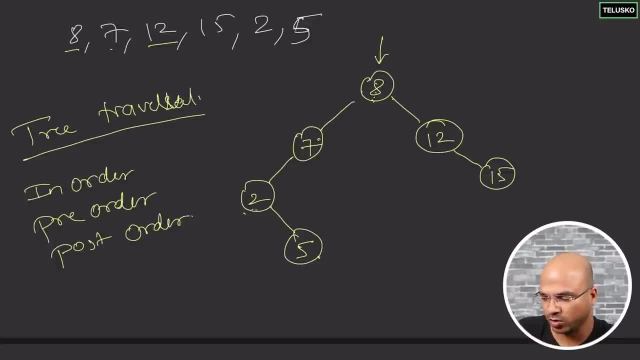 because that's an in-order. Then you go to the left one, because in in-order you first go for left inside left subtree And then from 7. also you can't print 7, because 7 becomes a root node, because we don't have any left here, right, This is empty. So in this case you will first print 2.. 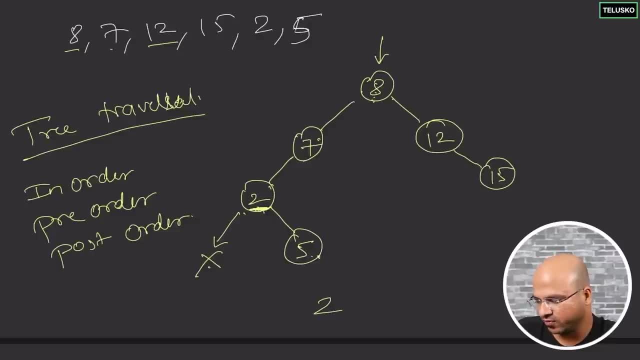 Okay, so you will go for 2.. But then you go for right. Since we don't have a left, we print the root node, because we are considering this subtree now. So you will print 2 and then you will print 5.. So here we have 5.. Then you go up, Then you print 7 because we don't have anything. So that's. 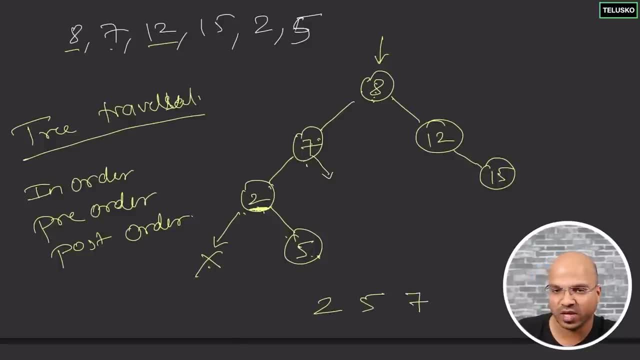 apparent for 2.. So we'll go for 7.. Then we print on the right-hand side. We don't have anything right-hand side, right, So this is empty. Then you go up, you print 8.. Then you go for the. 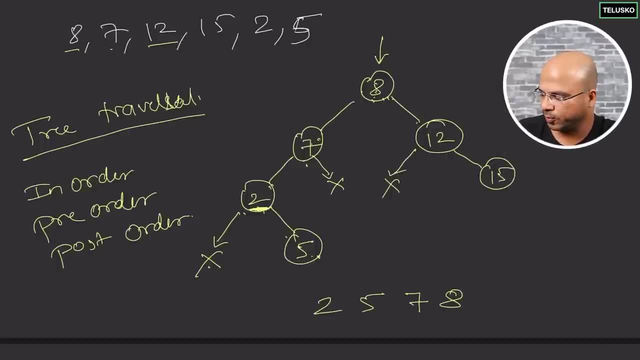 left-hand side. Right-hand side is 12. On 12 left we don't have anything, So it will not print anything, But you can print 12. And then you can go for right-hand side, which is 15. And if you, 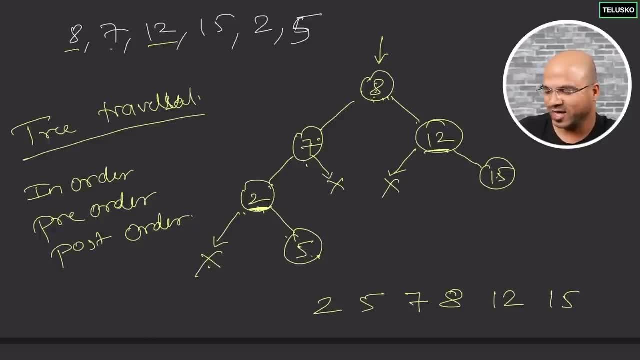 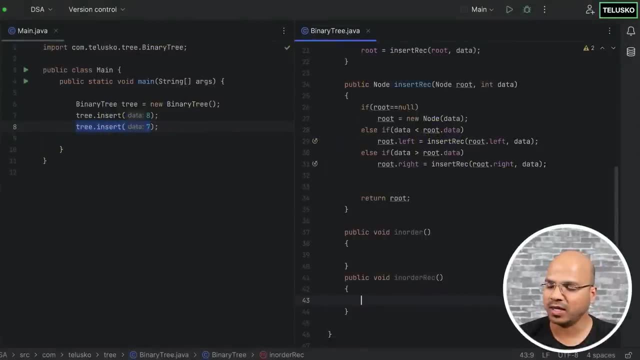 observe, you got a sorted values, So that's why we use BST, which is sorted values. It is easier to search as well. Okay, this is the in-order traversal. Okay, so let's implement this. So how do we do it? So first, we'll start from the left-hand side, But also we want to verify if the 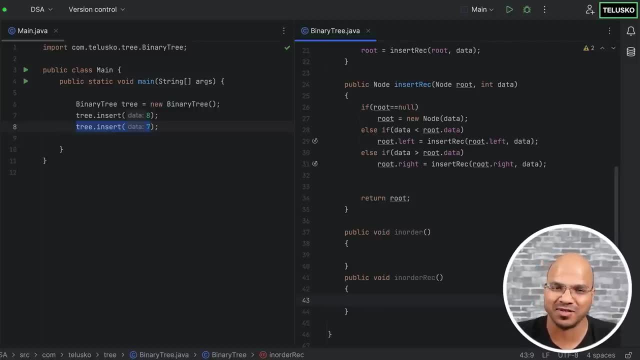 tree is empty. If the tree is empty, how will you print something, How will you travel And how do you know if the tree is empty? By using the left-hand side. So let's start from the left-hand side, using the root element, So we can simply check if root. But how do you know the root? 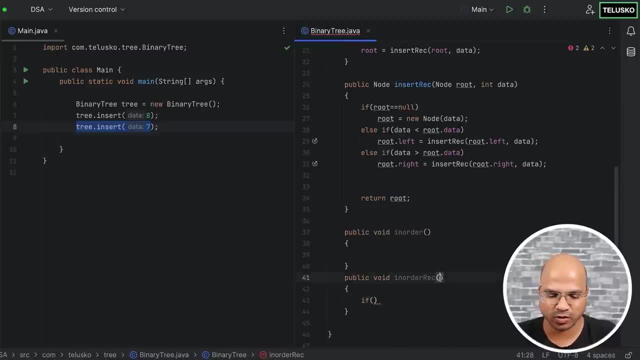 Because root will keep changing depending on the tree, right? So we have to also accept root here. So we'll say node is root, And then you check. If the root is not equal to null, then only you do it. Now. how will you do it Now? first of all, this is a recursive function, right? So basically, 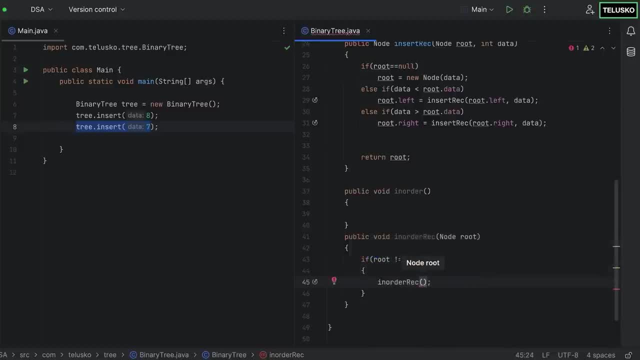 you have to call itself. So we'll say in-order right, And then you have to start from the left-hand side. So always start from left And then keep going till you find the last left element okay, And then, once you do that, then you have to go for the middle one. Middle one is root itself. 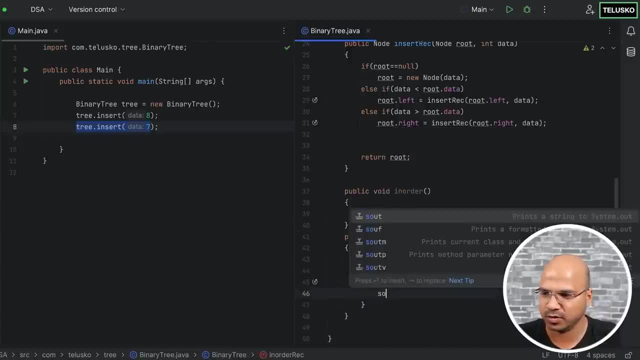 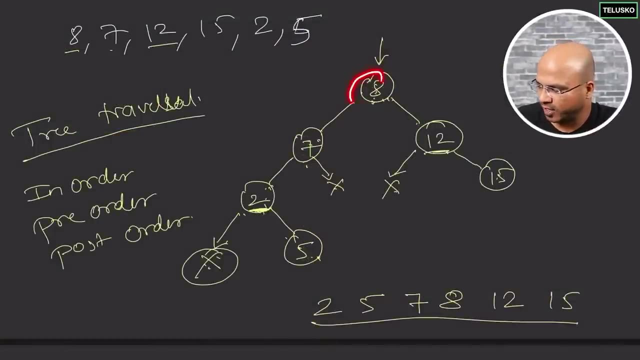 which we got here right, So we can print this value here. So I will say print. And if you observe, for every node, for every subtree, there is always a root node. If you observe, for 8,, 7 is left right, But don't you think 7 in this subtree is a root node? So that's the root. we. 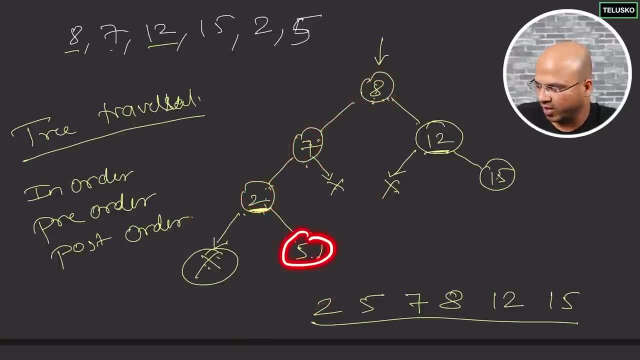 are printing. When you go to 2,, 2 becomes a root node. right, When you go 5,, 5 becomes a root node for their child, which we don't have. So we can print data here, So we can say rootdata And then 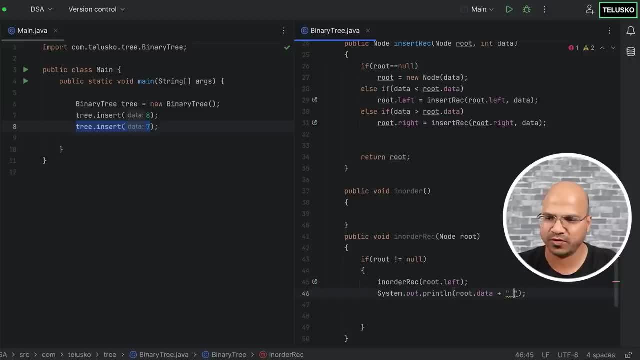 print a space in between as well, just to differentiate the values, And also I can skip the new line. Now, once you are done with the root element- of course, not just printing- you can do some other operations as well. Maybe you can add all the values, if you want, And then 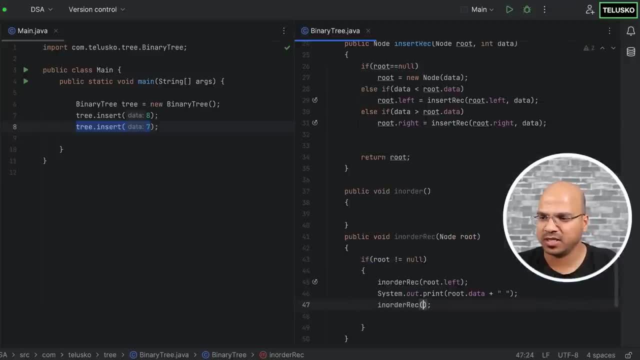 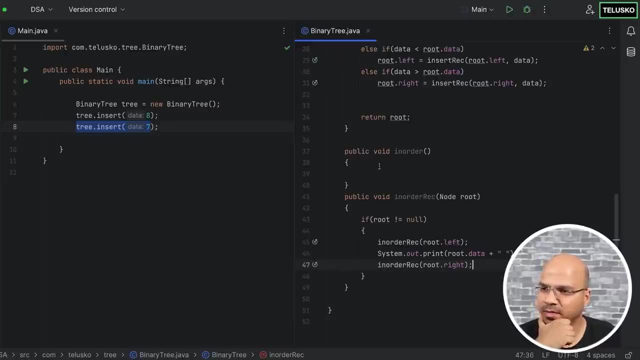 here I can say in-order, But this time you will go for rootwrite. That's it. This is how, basically, you print the values. But from in-order we have to call in-order rec By passing the root node. So you will call this only once in-order. So that means I can simply: 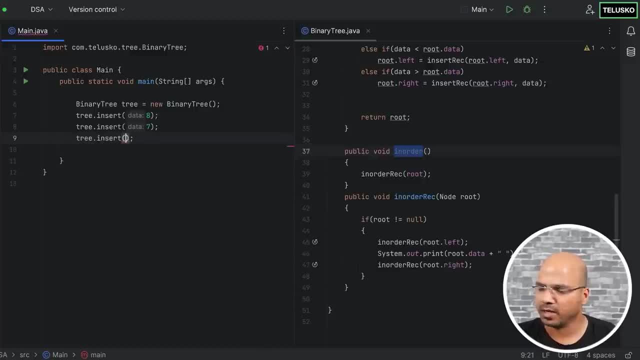 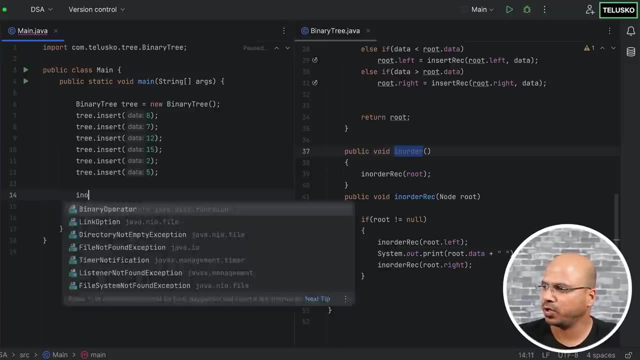 create a tree by adding values here first of all. Now, what values do we have? Let me just do that quickly. Okay, so you can see we have added all the values And now it's time for traversal. So I will just print in-order And it should do the job for us. Let's try. So we'll just run this.